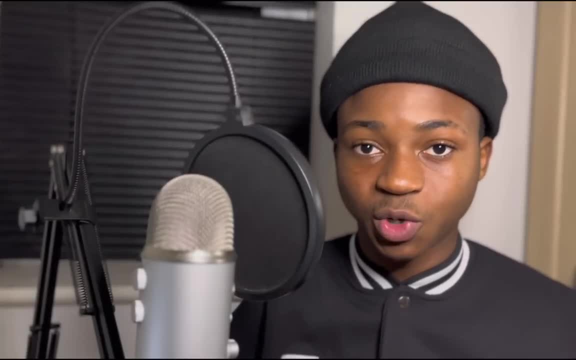 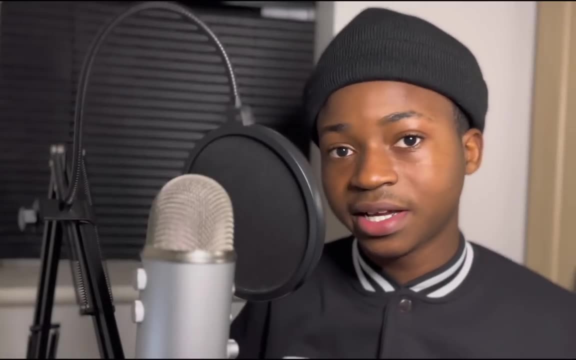 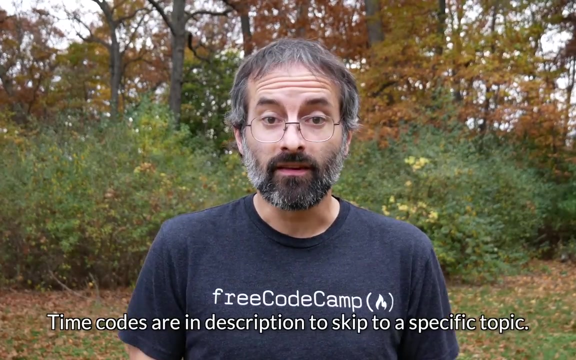 And I'm Tomi Toko and I'll also be teaching part of this course. I'll be teaching the JavaScript section and the backend web development section, And I'll be teaching the HTML, CSS and front-end web development sections. Before we get to the details, let me tell you more about some of the concepts in this course. 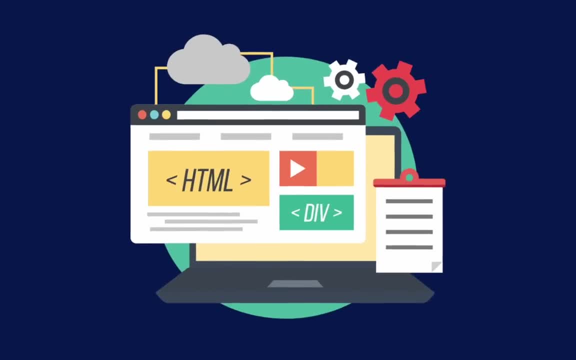 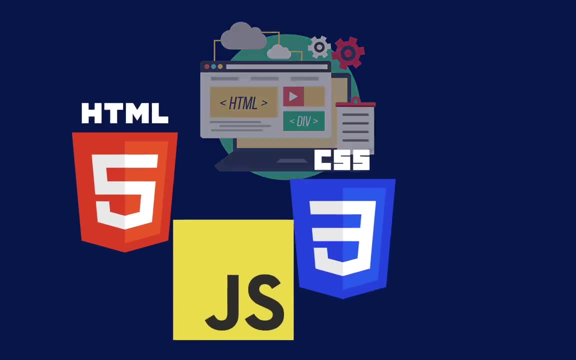 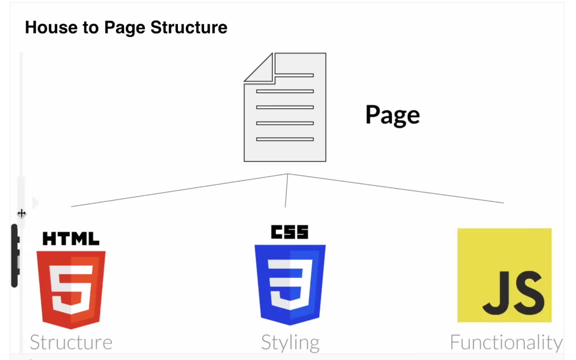 First let's talk about HTML, CSS and JavaScript. Every website on the internet uses HTML and CSS. Most also use JavaScript. In a website, HTML is the structure, CSS is the style and JavaScript is the functionality. Here's a great interactive diagram from code analogiescom. 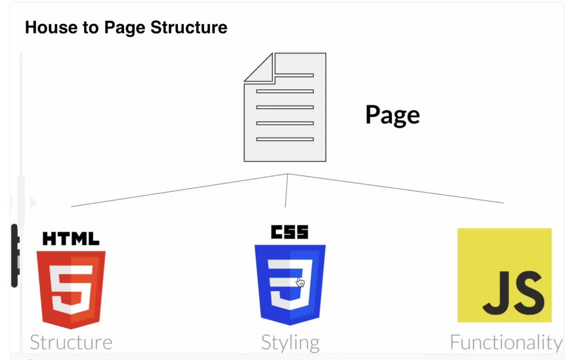 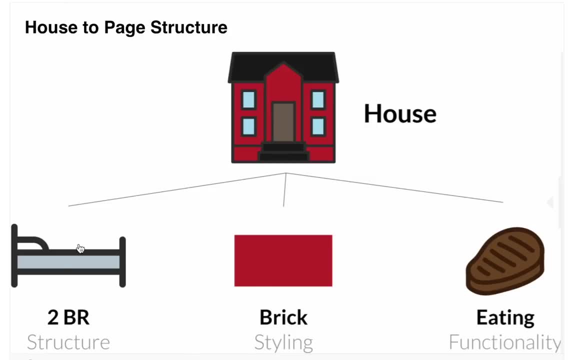 You can see we have the page, the structure, style and functionality, And if we move this slider so it's like the house. the page is like the house, So the structure or the HTML is like how many bedrooms there are, how many rooms. 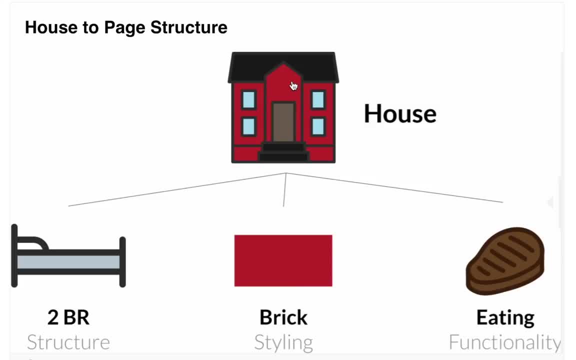 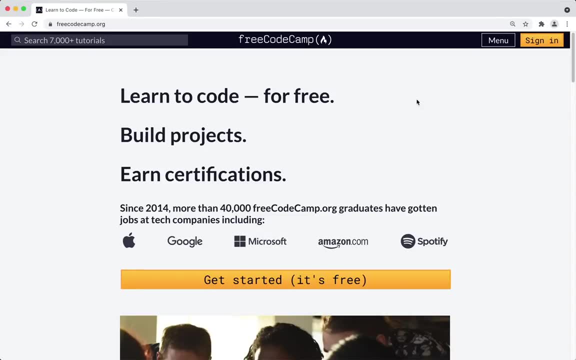 the CSS. the styling is like the color- the color of the brick here- And then the functionality. what you're doing like eating is the JavaScript. you can actually see the HTML that makes up any element on a web page by right clicking an element and then going to inspect. 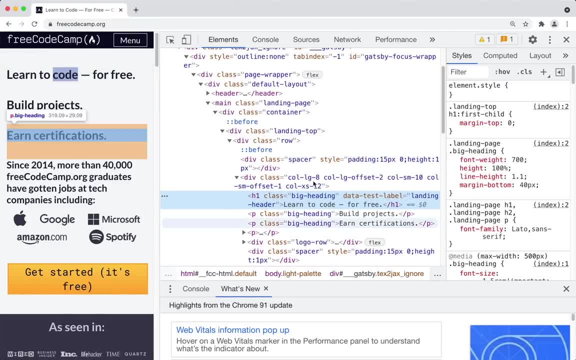 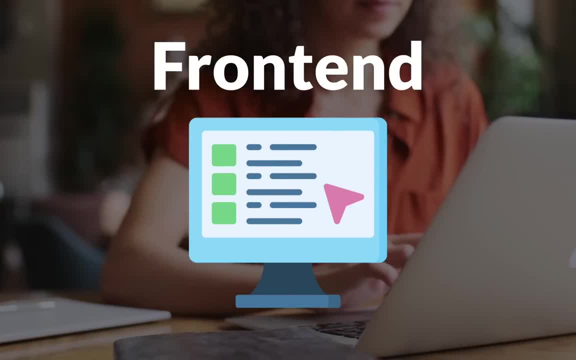 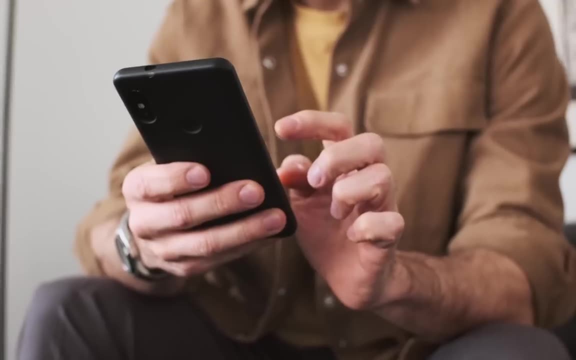 And this all this right here is the HTML. Now I'll explain the difference between front end and back end development. The front end of a website is the part that users can see and interact with. It's the part that all happens on the user's computer or device. 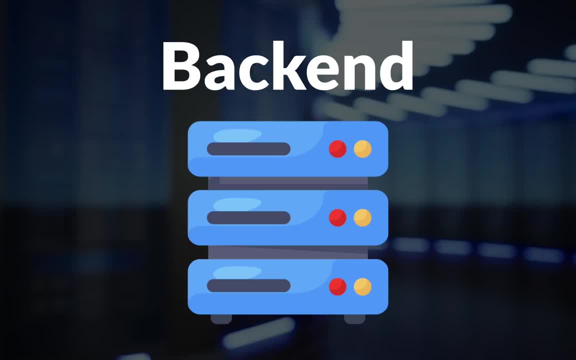 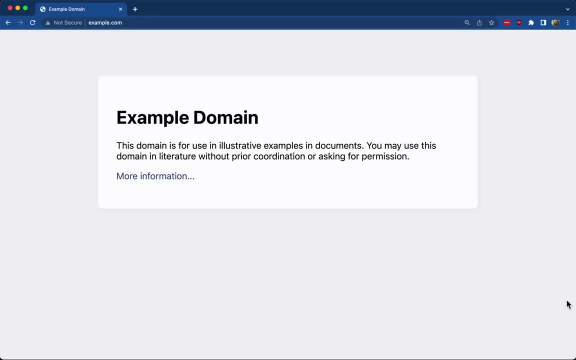 The back end is the part of the website that runs on the server and powers the front end. The back end includes the database, application logic and API. Some static websites only need a front end, But if a website interacts with the database or involves a lot of dynamic. 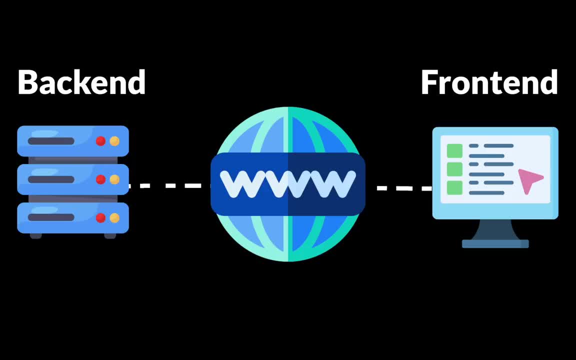 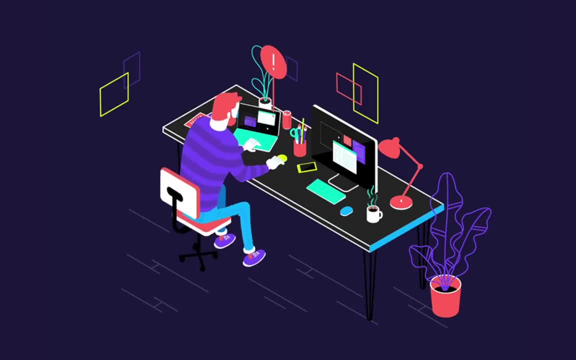 content, then there needs to be a back end server away from the user's device to do some processing before sending data back to the user. full stack development is just a combination of front end and back end development. By the end of this course, you'll have a better understanding of front end. 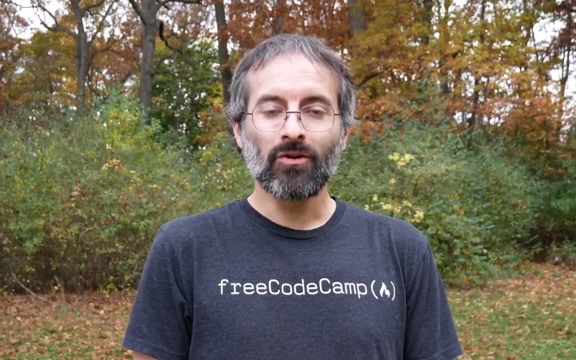 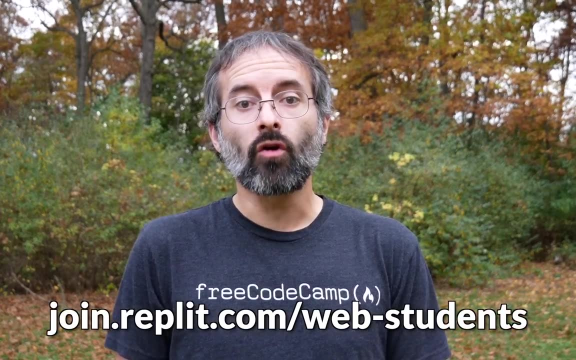 and back end development. Now it's time for you to start learning how to use HTML and CSS. Tomi will teach this section And before I pass it over to him, I want to thank replit for giving free code camporg a grant. 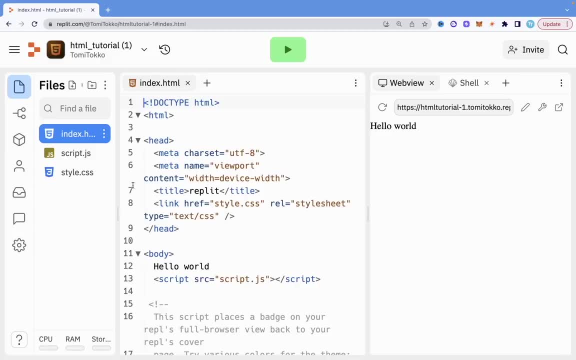 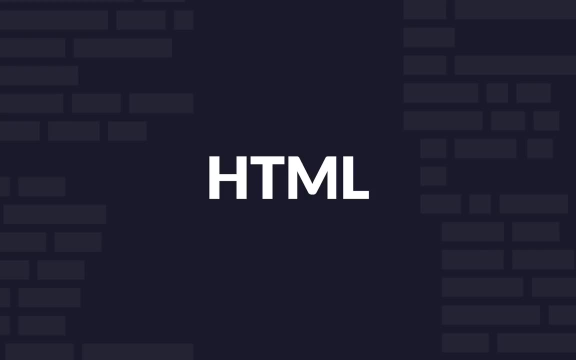 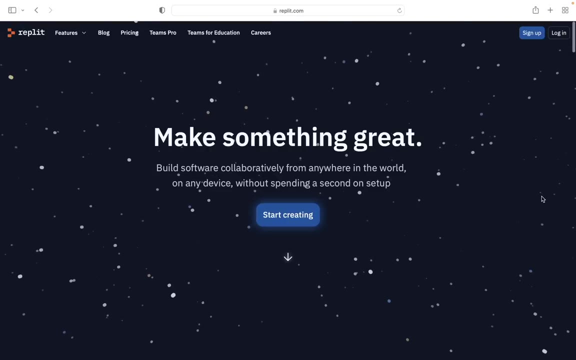 to make this course possible. We'll do all the development using replit, which allows you to write HTML, CSS and JavaScript all in your web browser. Welcome to this section of discourse. In this section, I'm going to be teaching you everything you need to know to get started building your own web pages using HTML. 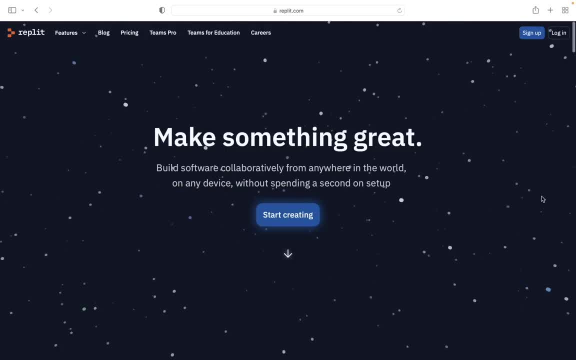 I'm going to be showing you what HTML is, why we use HTML and how you can build web pages using HTML. Now, in this course, we're going to be using replit for our coding And I'm going to show you how to set that up and how to do everything all from repli. 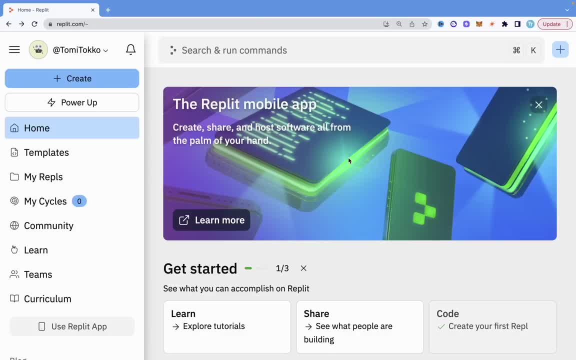 So the first thing we need to do is to go to replicom. So once you get to replicom, you're going to have to create an account and login. So once you log into replicom, it's going to bring you to this dashboard right here. Once you're in this dashboard, 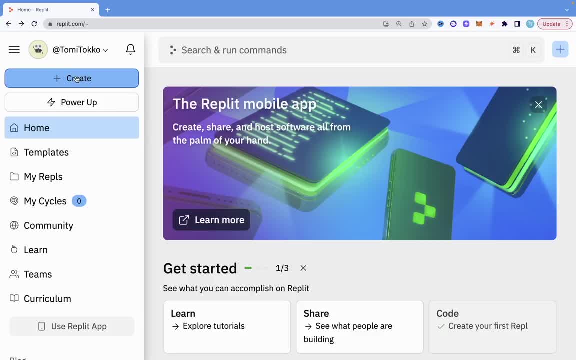 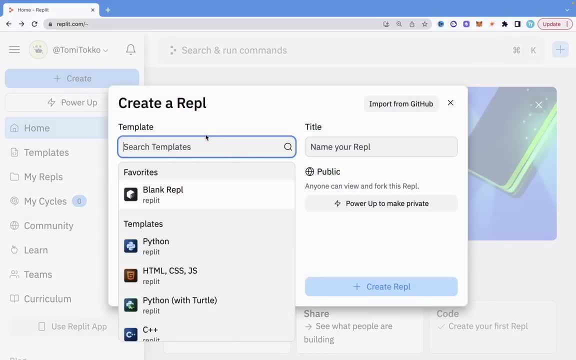 you're just going to come to this corner right here and click on this Create button, Or you can go to the top right corner and click on the new repli button. So what I'm just going to do is to click on Create and it's going to ask you to choose. 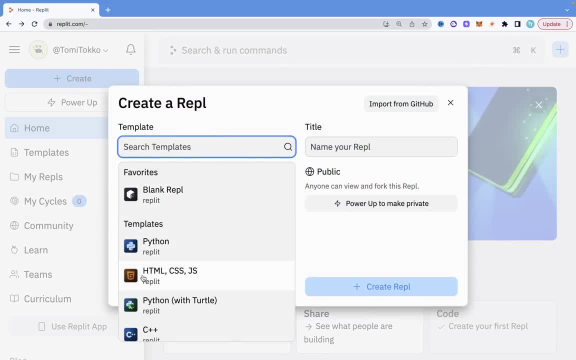 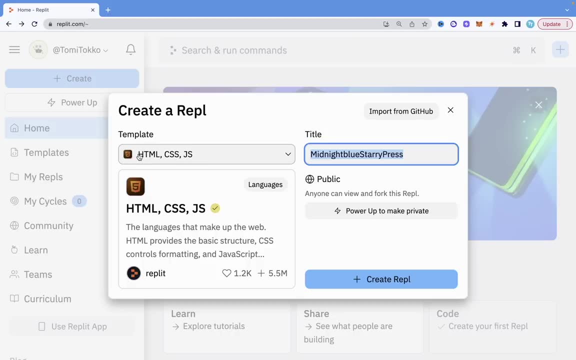 the language you want to use. So for this section of this tutorial, we're going to be choosing this HTML, CSS and JavaScript. But you don't need to worry about CSS and JavaScript for now, we're just only going to be using the HTML part. So let's name this HTML tutorial. 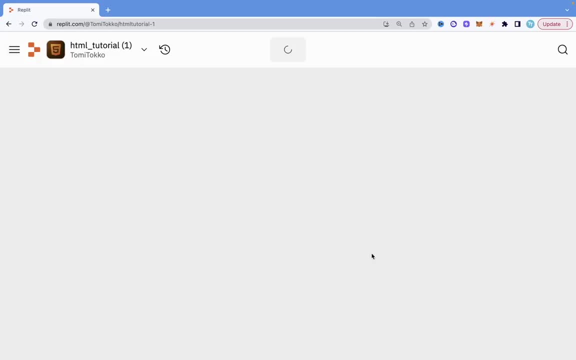 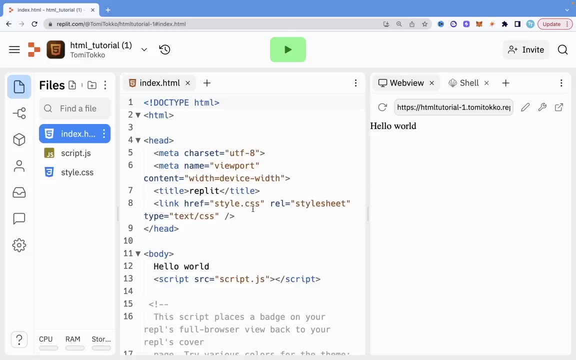 I'm going to create a new repli, So that is going to take a few seconds to create all of that for us, And once that is created, I'm going to show you what this is. So, as you can see, it's created this for us with like a boilerplate of code. 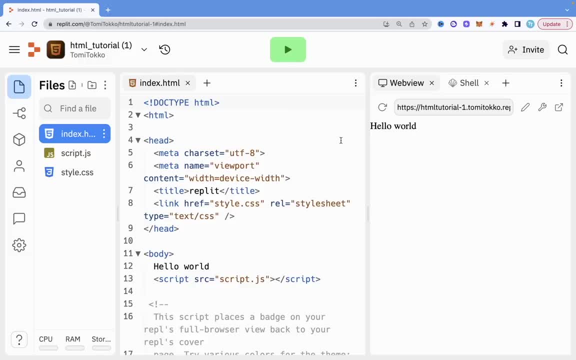 that automatically comes with this particular repli that we created. So what I'm just going to do is to quickly show you around repli, what it does and how we're going to use this. So on this corner you can see that it shows all the files that 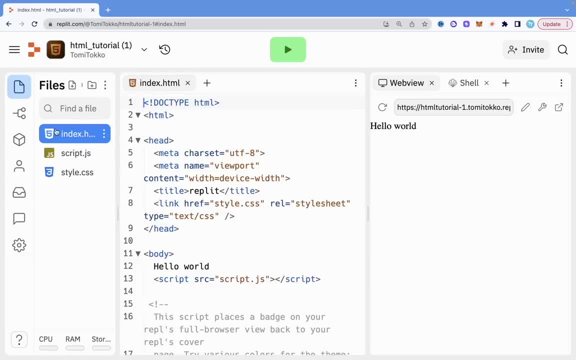 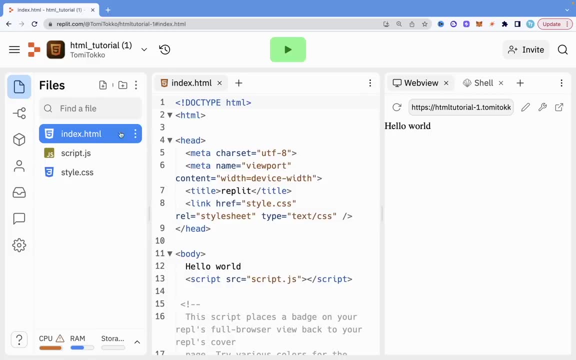 has been created. So, because we chose HTML, CSS and JavaScript, it created three files for us. One stands for HTML, one is for CSS and one is for JavaScript. But, as I said, for now I'm only going to be looking into the HTML part. I'm going to close that tab, just to. 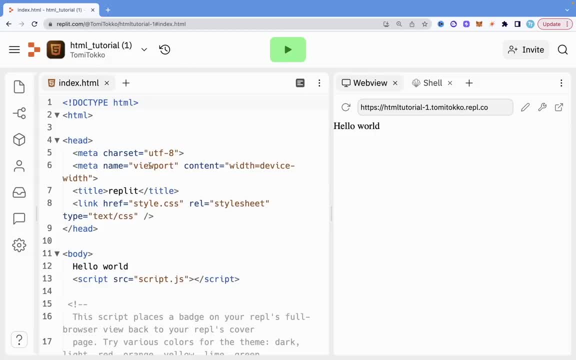 make sure that we have enough screen, And in here it shows the code base. So this is basically where we're going to be doing. the main coding is like our code editor, And at this right side it shows the output of whatever we are coding in you. But now that we have that out the way, 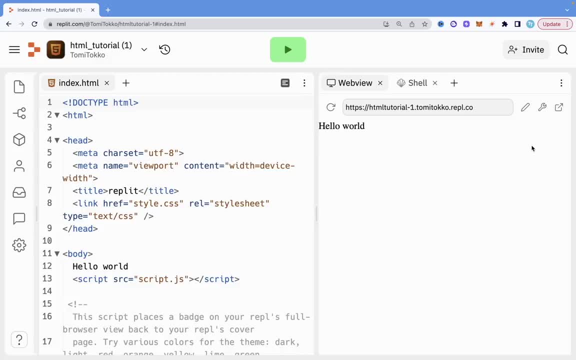 I wanted to quickly talk to you about HTML, So, before we actually go into coding, I'm going to to introduce you to what html is and why we even use it. so html stands for ipad text markup language, so it's basically a standard markup language used for creating websites and web pages. 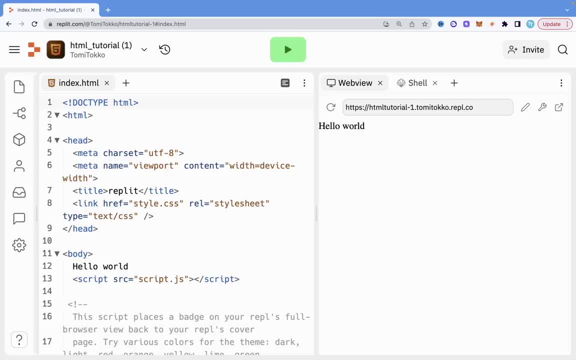 so html like describes how the structure of a website or a web page is going to look like. so any website you'll see on the web or any web page you see on the web, there is some html coding that has been done to build that. so html basically consists of different elements to make it what is. 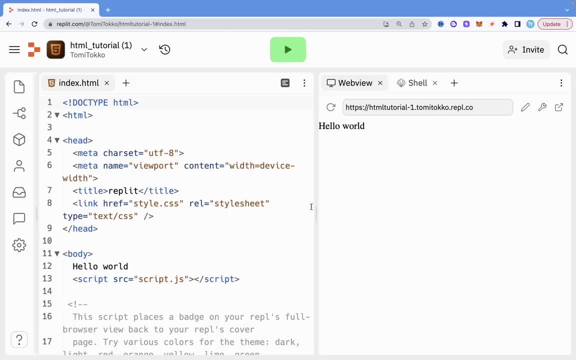 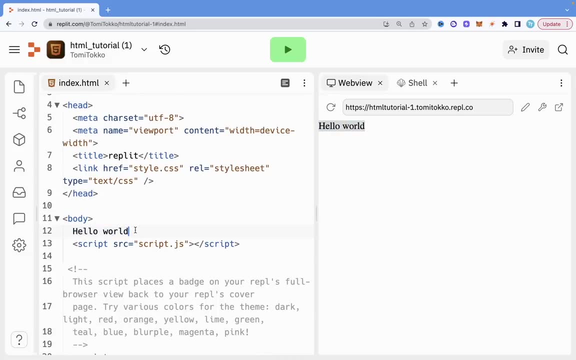 so, for example, if i come into this code, you can see that we have some hello world text being printed, and if you come into the code, you can see that that hello world text is right here. so this hello world text is under this element, name body. so don't worry about what all of this. 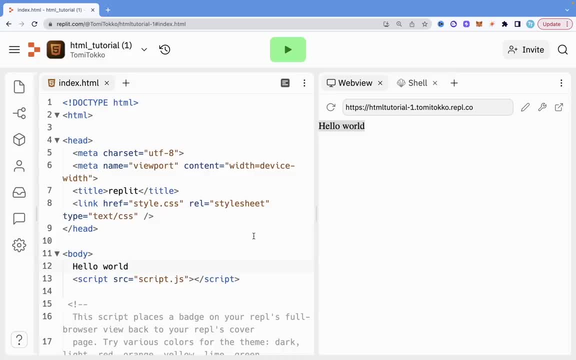 means. for now i'm going to go through all of that, but just know that html comprises of different elements, and now i'm going to talk to you about what all these elements are, the different type of elements that we have. so, first of all, i'm going to remove some text because we're not going to talk about them, for 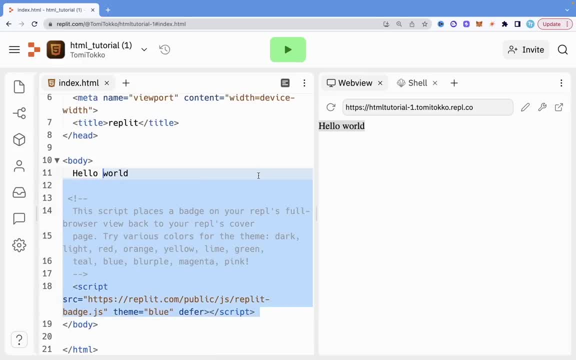 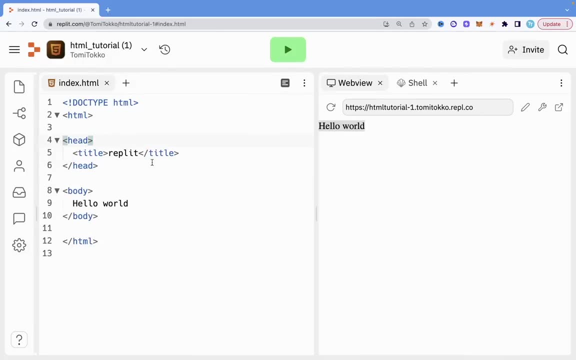 now i'm going to remove all of this script, because all of that are javascript and we don't need that for now, and i'm also going to remove this. so this is just a basic html code, right? so, as i said, there are different elements. so, for example, this doctype html is a declaring 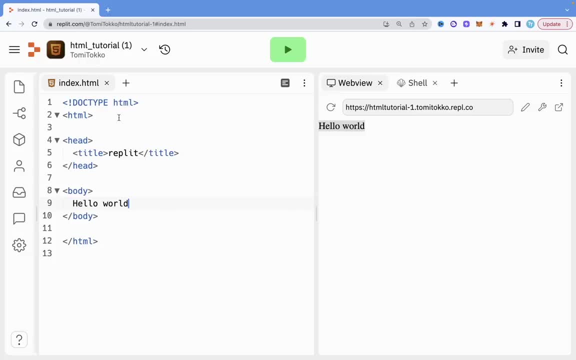 that defines this document is an html document. so this just tells us that whatever we're coding is an html document. and we have another element which is html right, and it shows the root of the html page. so this means that anything that we are going to be coding in this html file is going to. 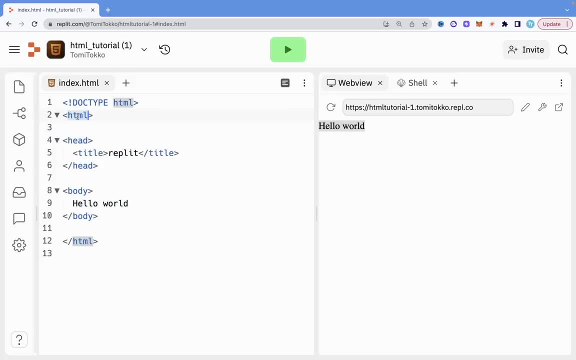 go into this html element, so we open it here and we close it here. i'm also going to talk about the structure of how we code an element using tags, so i'm going to talk about that in a bit, but for now, as you can see, we have this html. that is the root of the whole project, right, and 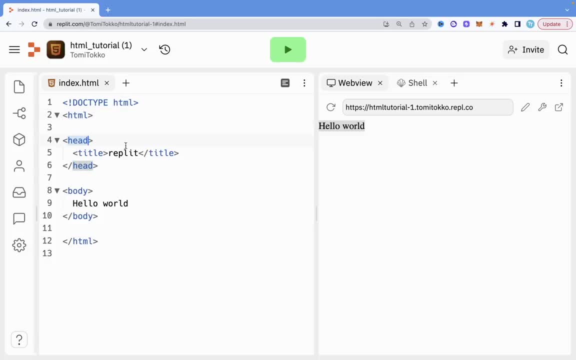 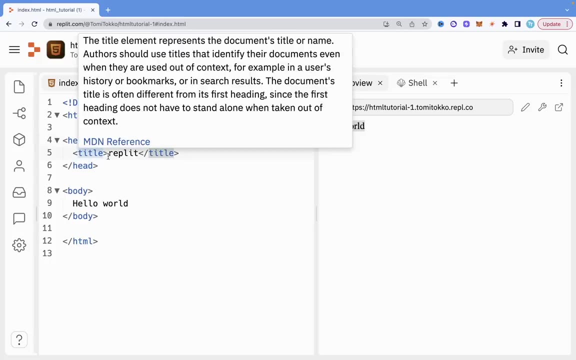 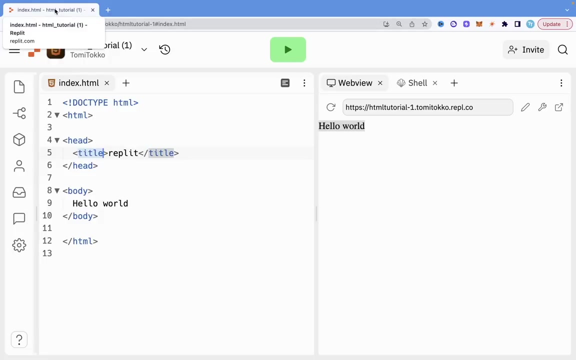 then we also have head that contains some information specifically about that html page. for example, under head we have the title: now this title is whatever you see on the browser. so on the browser right here where you see this indexhtml, that is the title of that page. 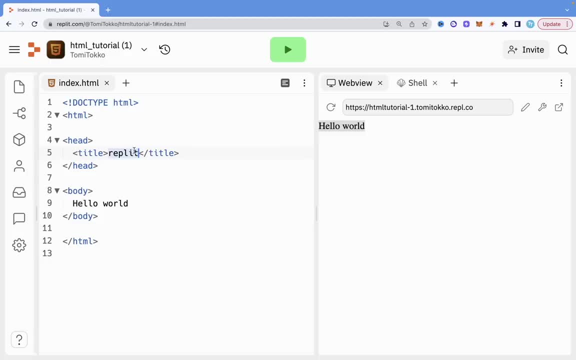 so whatever we put here is what's going to be shown here. so, as you can see, that basically is part of the structure of the whole web page, and then everything that is going to be in this section of this of the browser of the web page goes into the body element. so that is what the body element. 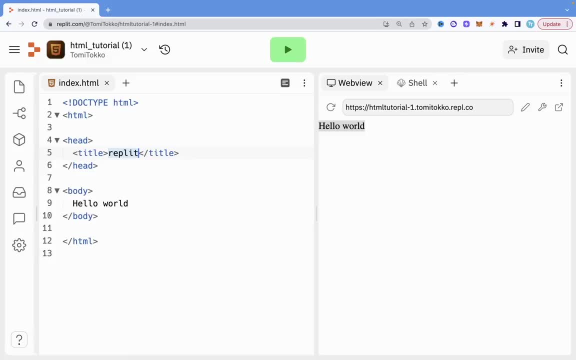 is for it's basically all the code that you're going to do is going to be done inside the body element, but let me tell you how we actually write this html element. so we write html element by defining tags and the content and the ending tags. so let me tell you what i'm. 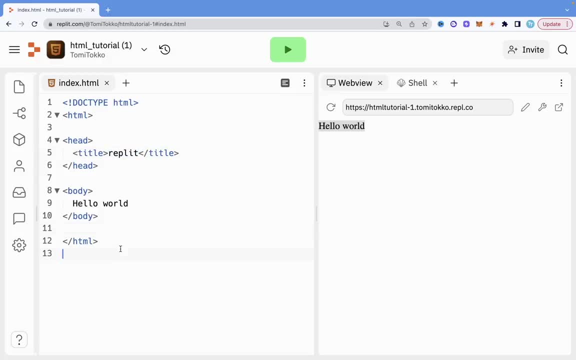 mean by this. now, i'm just going to close all of this real quick because we're going to have to start from scratch, so you understand it. so, for example, let's say we have an h1 tag, so this h1 is an element in html and is used to create like an adding text, for example in: 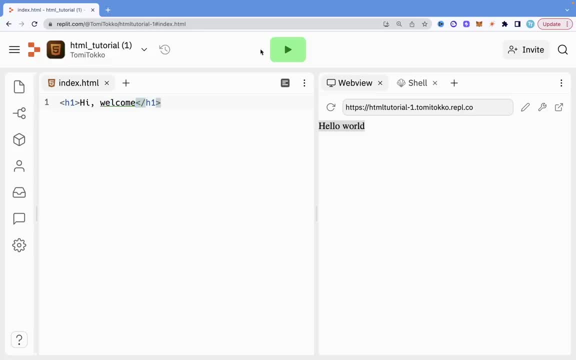 here. if i put i welcome and once i run that, you're going to see that it prints i welcome like an h1 tag. so that is what this h1 element does. but how did we write this h1 element? the first thing we do is to say we're going to open an h1 tag, so we're going to have two less than sign and greater. 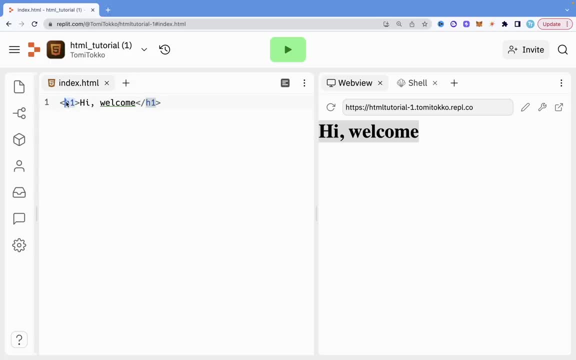 than sign, and in there we're going to have the name of that particular tag. then after that we're going to have the content that is meant to be shown in that element. after that we're going to close that tag. so this is how we close the tag. now let me show you another tag. there is an 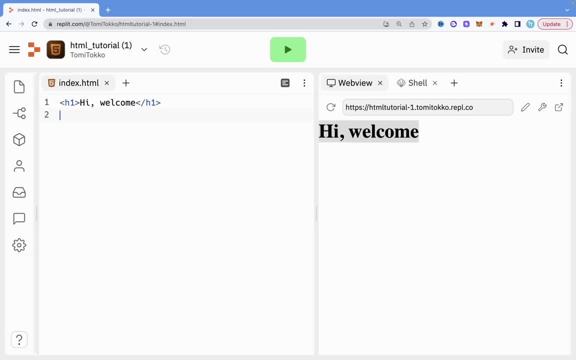 other tag that is used to define a new paragraph, and this tag is called p. so we have this sign less than sign. we put p, we close that automatically. replete ends the tag for us. but i'm going to delete that. i'll show you how to close it. so in here we're just going to put something like: this is a. 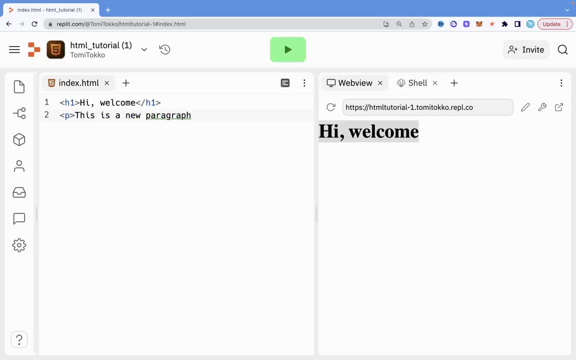 new paragraph and then we're going to have to close it. we close it by using the less than sign close it back. so this is how to open a tag. so it's something like this: we're going to say: tag once we close it. so this is basically the opening tag and then in here the content. 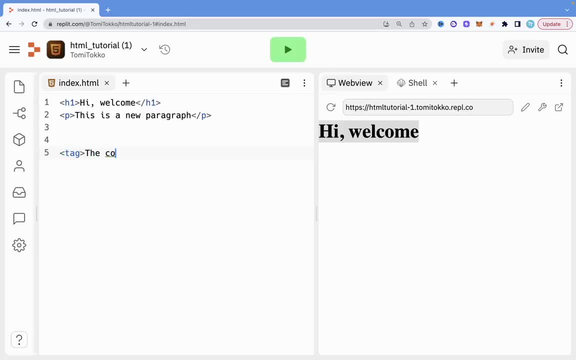 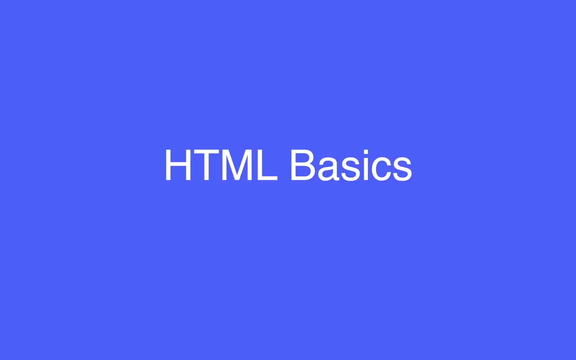 and then to close the tag. it's basically similar to this, but instead we have a slash, so what we can just do is to do less than sign slash replete automatically close that for us. so that is basically how to, you know, create a tag and elements in html. now we're going to be talking. 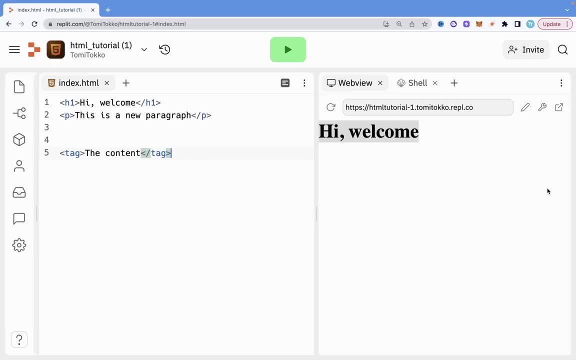 more about the basics of html, so basically, the structure that you're meant to follow when you create a new html page. so i'm going to get rid of all of this and let's start this from the beginning. so, whenever you create a new html page, you're going to need to create a new html page. 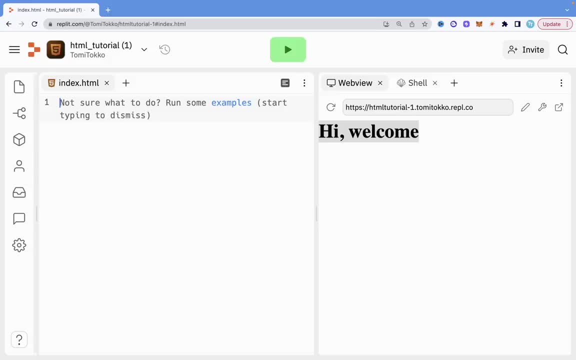 you must first define a doctype declaration. now, this shows the type of documents that this represents, so it allows the browser to know how to display the web page correctly. so what to do this? we just need to use the less than sign, because it is an element. so we do it the same way. 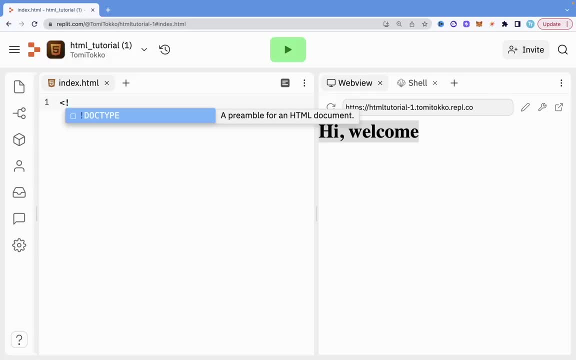 and then we use the app, this sign, and then we say doctype, and then we're going to specify the type of you know file that we're actually coding in, and this is html, and we're just going to close that. so this is the first thing you should do when you create a new html file. 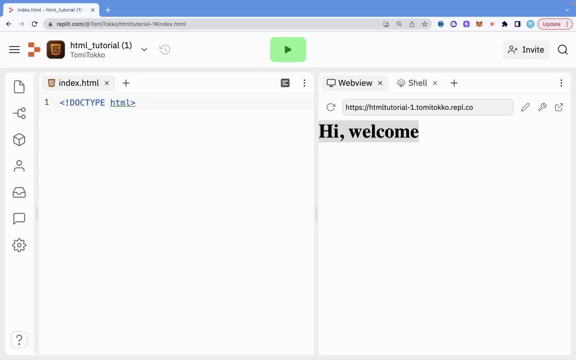 right, and then, once you do this, the next thing that you want to be doing is to create the html tag. so this html tag, as i said in the a while ago, is is the root of all your, of the all html structure, so everything that we're going to be coding. 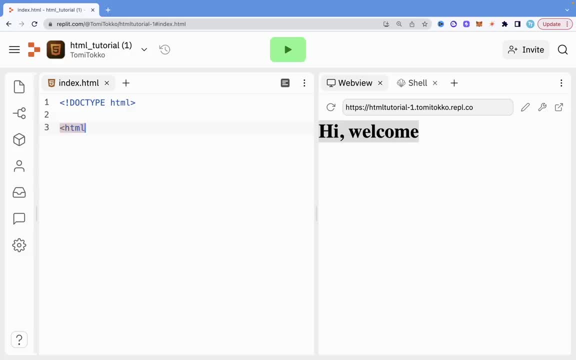 should be. inside this html tag we're going to write html and automatically replete, closes that for us. now, inside this html, there is something else that we need to have, and this is the body. so the body basically takes any visible code or any visible thing that we want to show on our web. 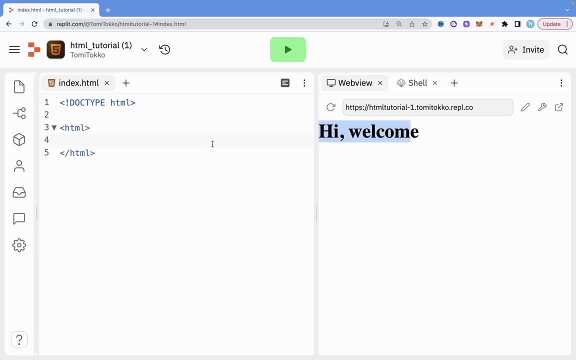 page. now, for example, this i welcome- should be under the body, for example, the. the code used to create the html code used to create this replete, everything that we see right here should be stored under the body type. so, right here we should have a body and, as i said, replete closes that for us automatically work. so anything that we're going to 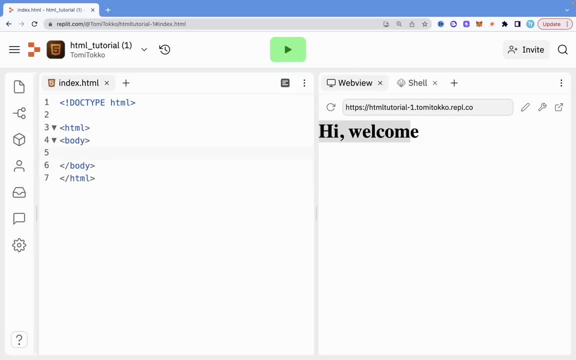 code should go in the body right here. so now i'm going to talk more about different types of tags, what they are used for. so we have the editing tags and they are mostly defined from their name to show addins. so we have the올 have them in a list from h1 to h6.. So in the a while ago I showed you how to create this. 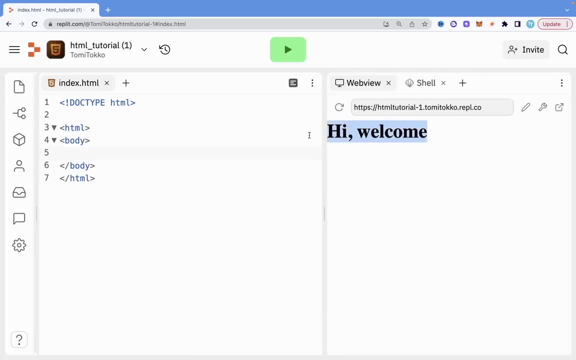 edit in using the h1 tag is editing that we see right here, So do h1. and then we close it and say first edit. Now, if we run that, you're gonna see that just going to print a show out the first edit. As you can see, it says first edit. Now if we use another, 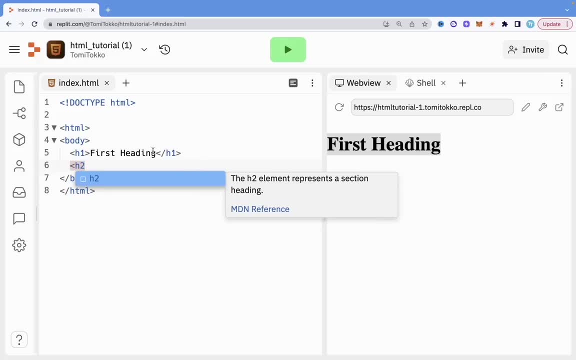 tag named h2,. this is also an editing tag, but it is smaller compared to h1. So if I say second edit and I run that, you're gonna see that it's gonna show second edding but quite smaller to this. And if I use another one, h3, I can say third edit And once I 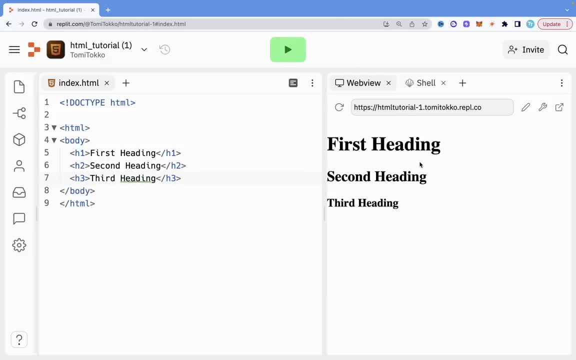 run that, you're gonna see that it's going to be smaller. So the size of the heading keeps descending right as the h1, h2. so as you ascend from h1, h2, h3 all the way to h6, the site keeps descending. so h1 is the biggest. so you can use this whenever you see fit in your. 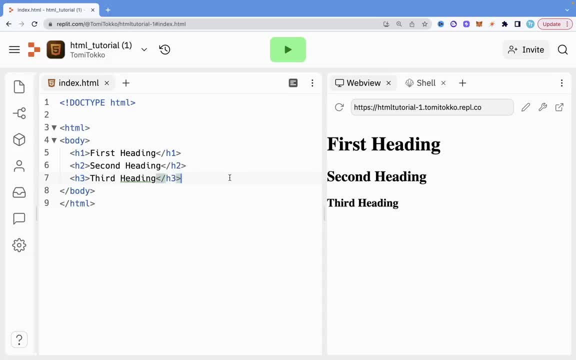 code. now. the next one i want to talk to you about is the paragraph tags. i talked about this briefly a while ago, but let me talk more about this now. so it's a very basic and simple tag. what it just does is it creates a new paragraph. so, for example, in your code, let's say you want there to be some. 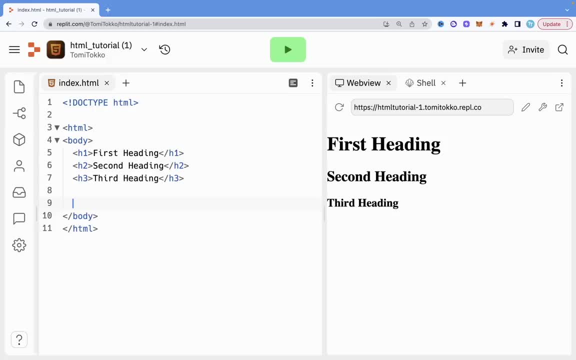 spacing between different texts or you just want to show like a new paragraph structure, we use the p tag. so once again, we use the less than sign, we put p, we use the greater than sign and in between this opening and closing tags we have the content of that paragraph. so we can say: this is a test. 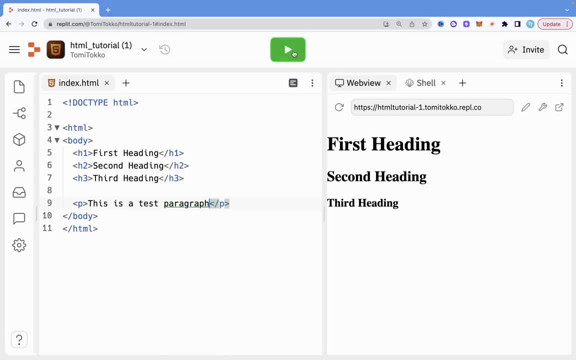 paragraph. so if i run this, you're going to see that, first of all, there's going to be spacing between it and this is a normal text. it's not an editing, it's not bold like this h1 tags. so, as you can see, just say this is a test paragraph right now, the next one i want to talk to you about. 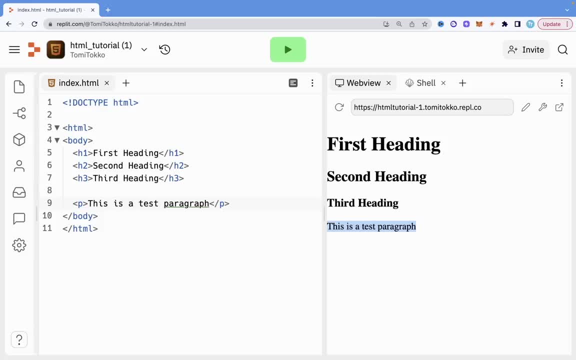 html links. so, for example, let's say, on this page, if i click on invite and it takes me to another link or another page, there is basically an html link tag that allows me to do this. now let me show you what i mean. so, for example, let's say, i want the user to say something like: click this link. 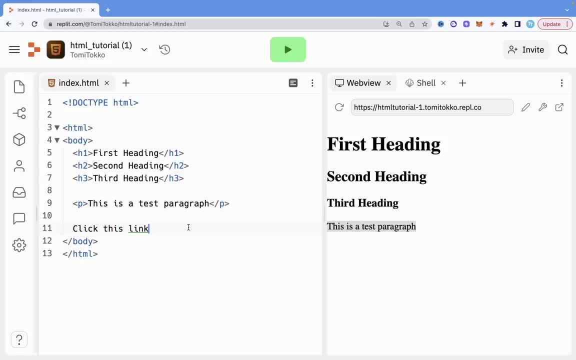 right, and once the user click this link, i want to take the user to, you know, freecodecampcom, or. or i want to take the user to googlecom. so what we can just do is to say i'm going to remove this real quick. we open a new tag, but this time around we're using an, a tag right, and then i'm going to close it. 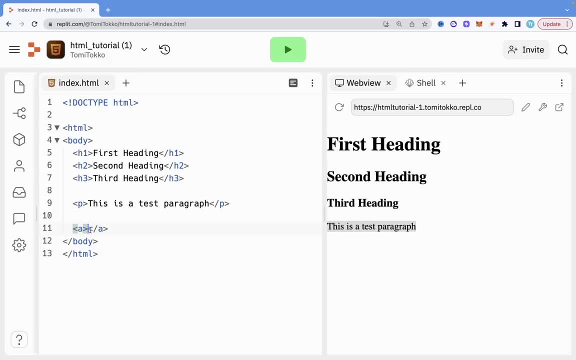 so once i close it, i'm going to have the content in here so i can say: click this link, right. but now there's something different with this. this is when i'm introducing you to what we call html attributes. now, if you don't understand this now, you don't need to worry, because i'm going. 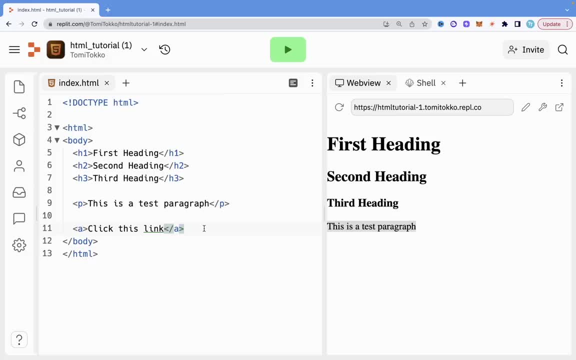 to have a whole section dedicated to talking about html attributes. so html attribute just shows me what parameters a tag needs to take. for example, this: a tag is used for redirecting a user to another link or sending a user to another page, but it needs to know what page it wants to send the user to. 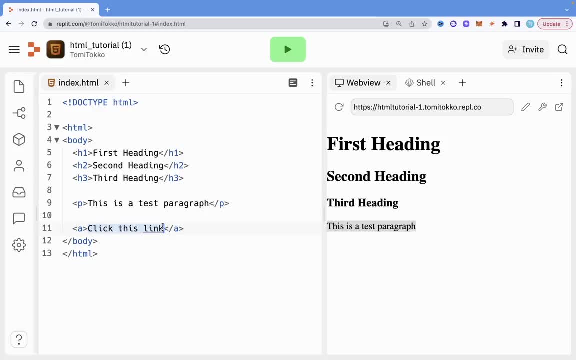 so, for example, once a user click clicks on this click the link, we need to specify the link that we want to take the user to, so it needs to have an attribute, and the name of this attribute is href. and this is how we input attributes in html tags, in the opening tag. 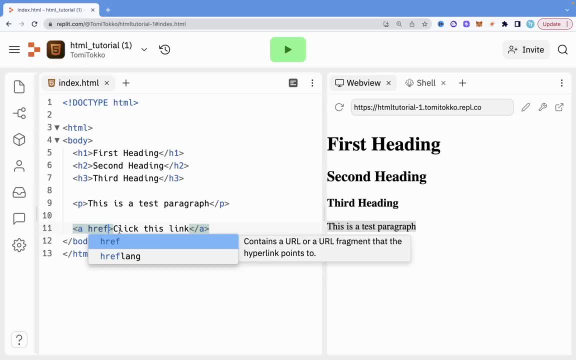 we leave a space and we type the name of the attribute and we say equals to and we use this quote. now, in this quote we specify the value of the attribute. so in this case, the value of this attribute is the link i want to take the user to right. so let's say i say googlecom. now, if i run, 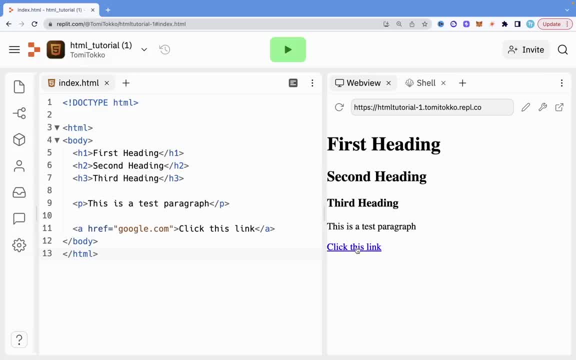 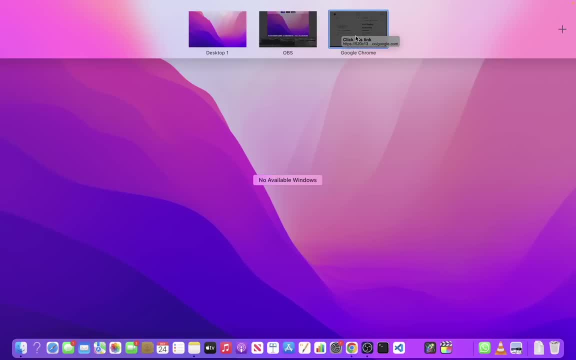 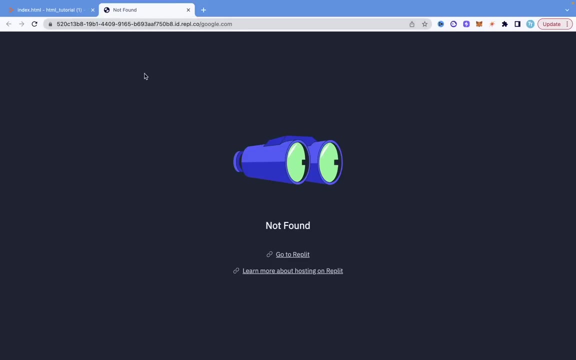 this. you're gonna see that we have like a blue color with satellite that is underlined, and if i drag this right here, so i'm just going to choose the link that i want to use to take the user to going to go back to that and let's see, i drag this right here. okay, so, um, it gives us an error. 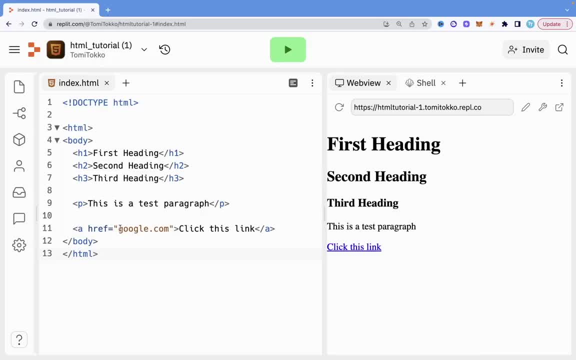 it says: replico slash googlecom. now, this is because i didn't define that is an external link, so it's thinking that is a link under this particular web page. so what you need to do is just to say https, so basically specify it as a new link on his own. so once i run that and it runs, 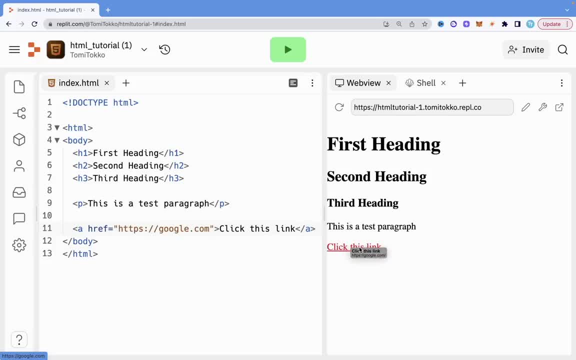 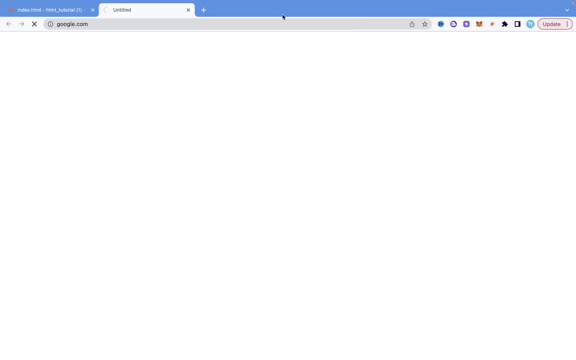 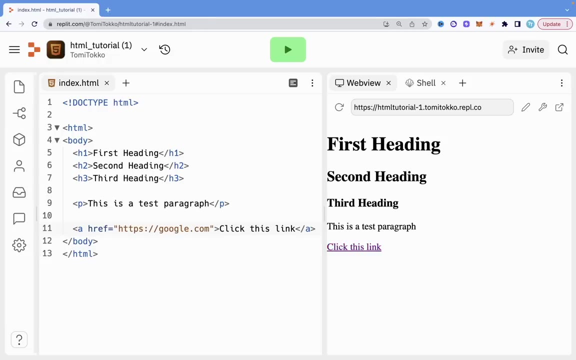 again. if i take this, if you look at the left bottom corner, you can see that it's showing me that i'm going to go to https, googlecom. if i take this and paste this here, it opens googlecom. so this, that is the basic way of creating a link. right and don't worry about the 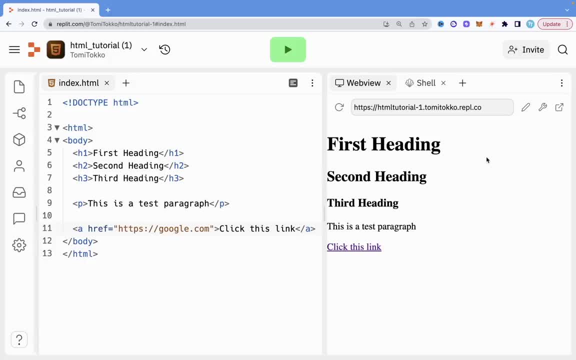 attributes for now. i'm going to talk more about that soon. now we are going to talk more about html attributes. so a while ago i showed you i used a simple html attribute to show the link that we want the user to go to once they click on this: click the link button or just click the link text. but now i want to talk more about what. 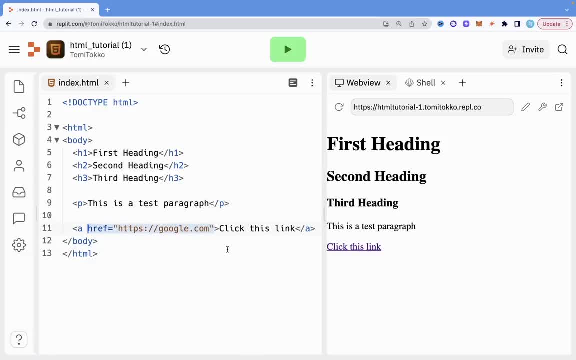 this attribute actually is why we use it, how do we use it and different tags where we can use this. so, as i said a while ago, the attribute basically gives more information about the element or the tag. so, for example, this a tag, it needed an information and that information it needed is the link we want to send the user to. so 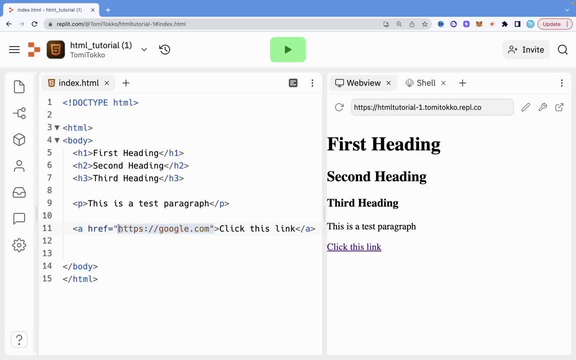 once the user clicks on, click the link, we want to send the user to googlecom. now there are other tags that actually need us to, you know, specify different things. that's when we use the html attributes. for example, we have the img, which is also known as the image tag, and this needs. 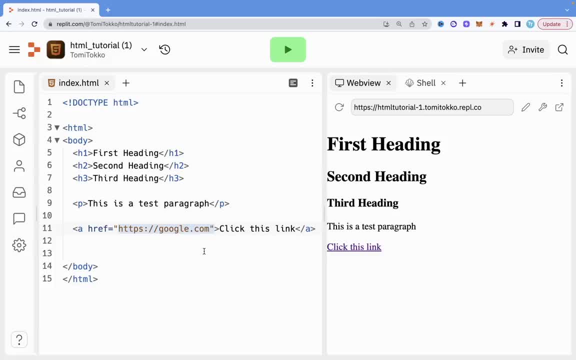 an html attribute that specifies where or the source of that image that we want to show. so before we go into that, let me quickly go through again how we, you, i will specify how we create html attributes. so, as i said, in the tag, in the opening tag, we write the name of the 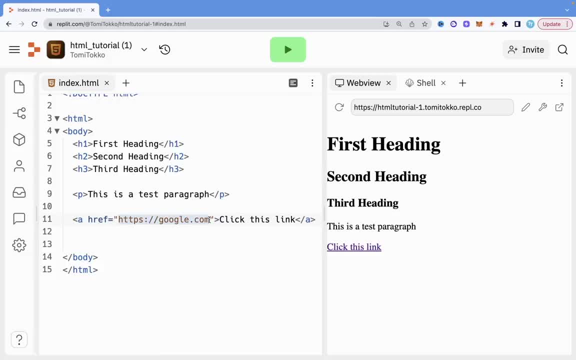 attribute and what the attribute contains. so basically, like the value of that attribute, right? so for us to do this now let's test it on another tag. so let me show you how we can display an image on your html page. so right here, we will show you an image that we can display an image on your html page. so right here, we will display an image on your html page. so right here we will. 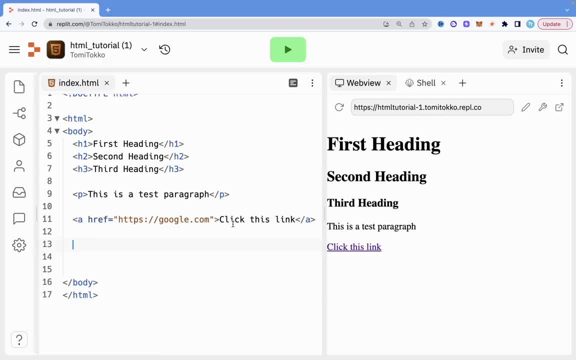 want to display a simple image, So what we can just do is to say IMG- right, And we're going to close this. So this image tag is: is a tag or is an element that doesn't need to close it. So you know how we close the P tag by using this slash. we don't need to. 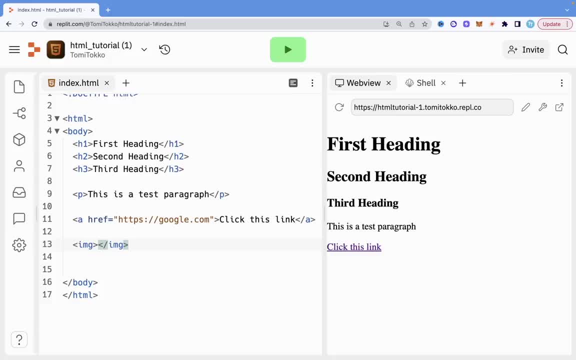 do that right here for IMG. And now? the reason why is because the IMG tag, or the image tag, doesn't take a value right Now. what I mean by this is like it doesn't showcase the value. the only thing it showcases is the image, So it just needs the source of. 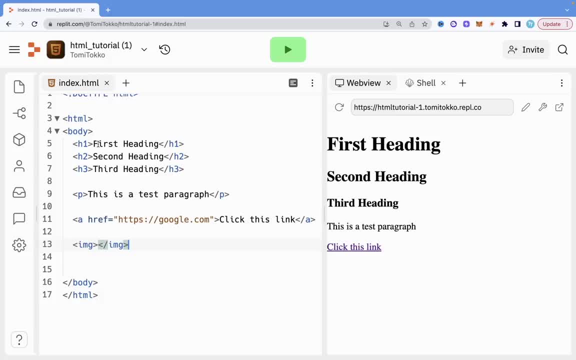 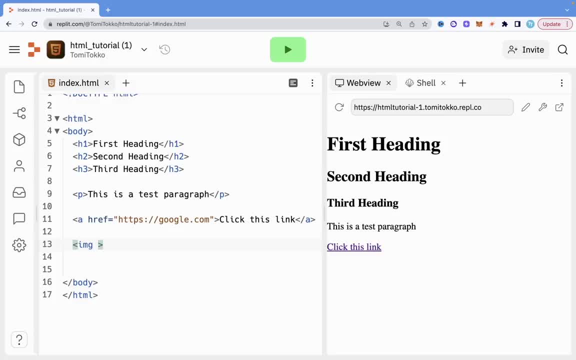 the image. So what we just need to specify is the source of that image. So we can do this similar to our way: Specify the link to this URL that we're redirecting. we're going to say SRC, So right now we want. 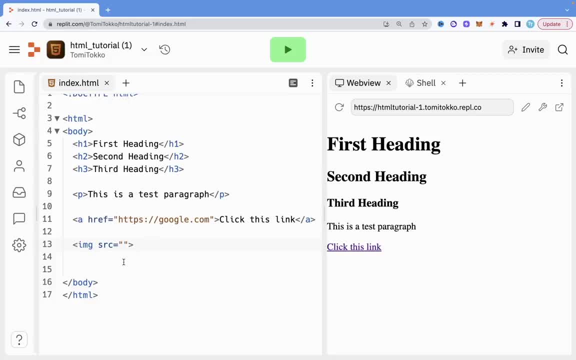 to specify the source or the link on where this image is coming from, Right? So, as I said, this is the name and India is going to be like the value of this source. So we can just take a random image, For example. we can, you know, take. let's see if we can. 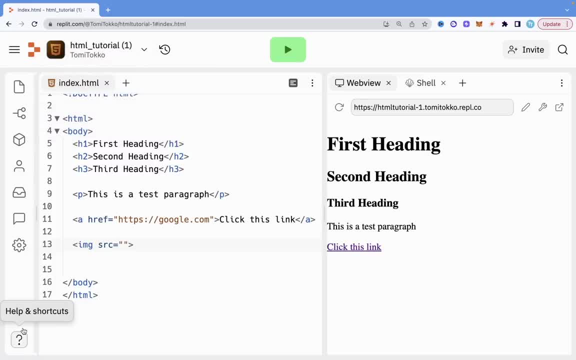 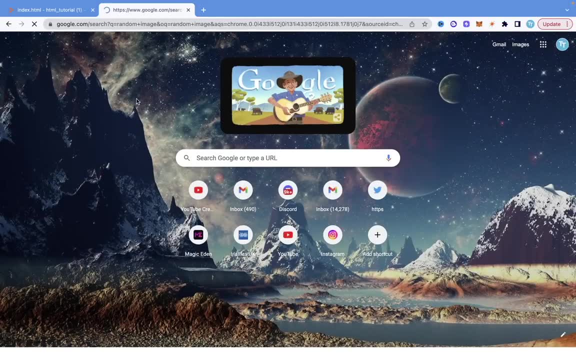 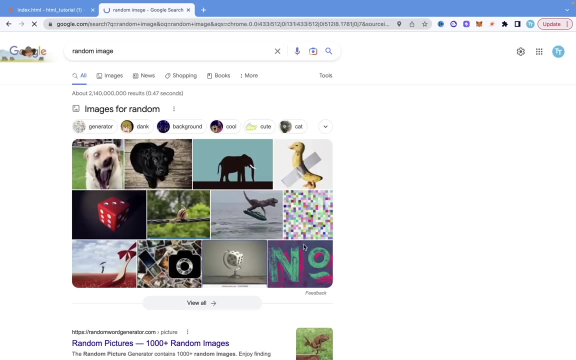 take an image from this page. We can take an image, So we can just go on. you can search random image And then in here we can take this dice image. I want to click on this dice image. We can say copy image. 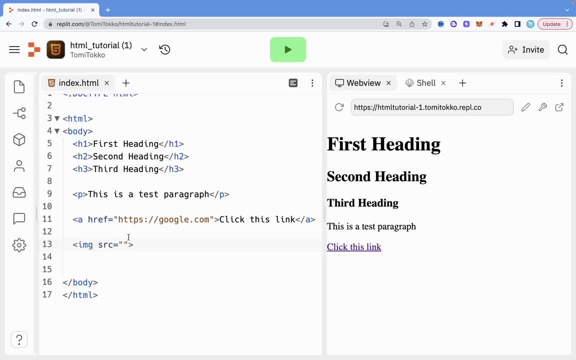 address. So now that we have that image address, once we paste this in here, that is the source of where that image is coming from. Right, If I run this, you're going to see now that shows that image right Now. obviously, this is a tag used. 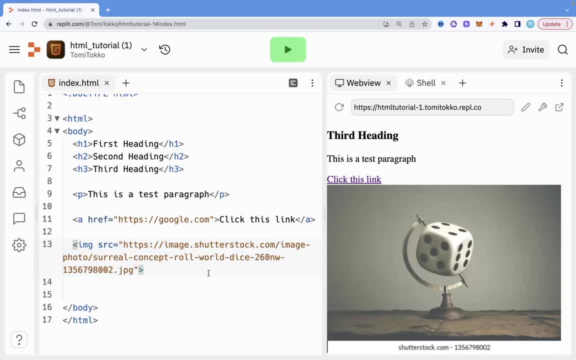 to show an image, And the reason why I said we don't close this tag is just because we don't need to write any text. That is why we don't like have a closing tag and put a text within it. So that is how we basically do that. very easy, very simple to do. Now. 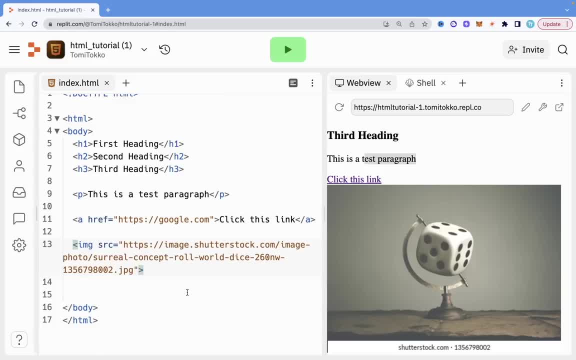 we can. a an HTML tag can have more than one attribute. right Now in here you can see that we have this SRC attributes. But what if we want to do more to this image? we need more attributes like: what if we want. 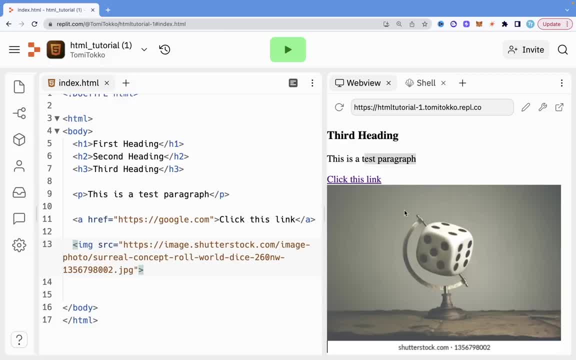 to change the size or anything. So, for example, we want to change the width of this image, I want to change the height of this image. So let's say, want to change the height of this image, right, And let's say we want to make it smaller or bigger. To do this, we're. 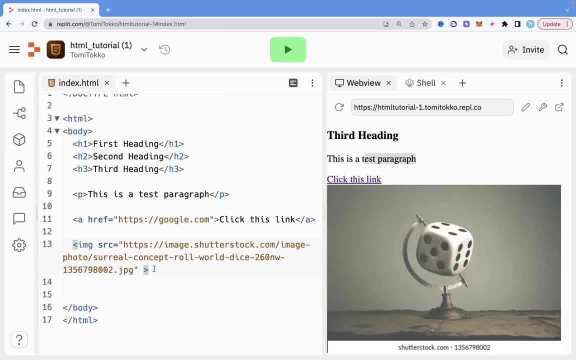 going to have to specify another image attributes, And this attribute is called it. So once again, we specify attributes by writing the name, we put the equals to sign and in here we put the quotes. Now, inside our quotes is where we put the value of that particular attribute. 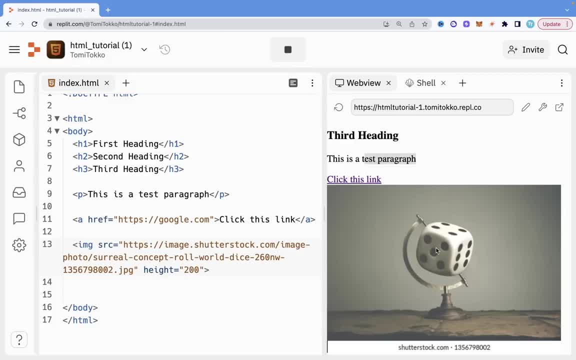 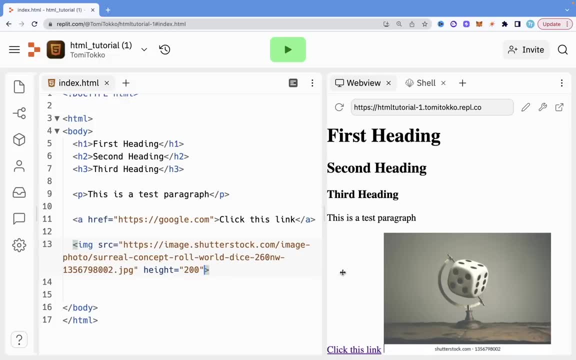 So let's say we want to make this 200.. If I run this, let's see what changes that makes to this particular image. you can see now that the image is shorter, And I can also do the same thing to the width. what if I want to reduce the width or increase the width? 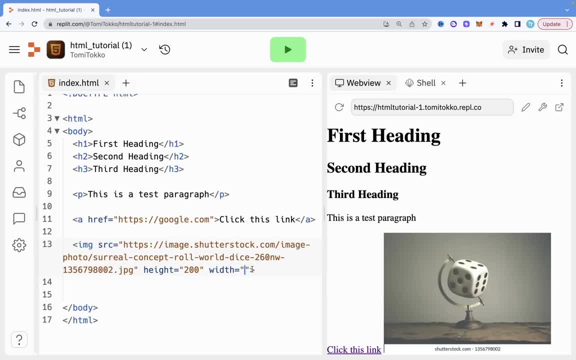 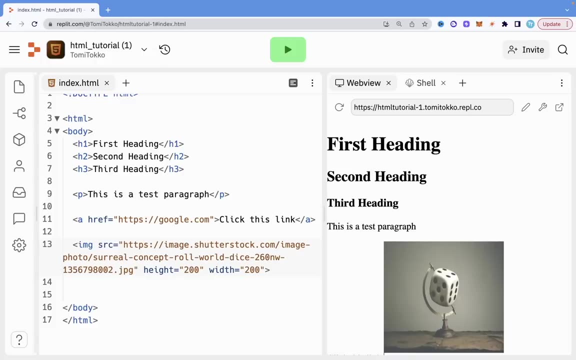 I'm just going to do with equals. then we put the column, The quotes, and then we also have the size. let's say the size is also 200. And we run that. So once we run that, you can see that the width has also decreased. So this is basically. 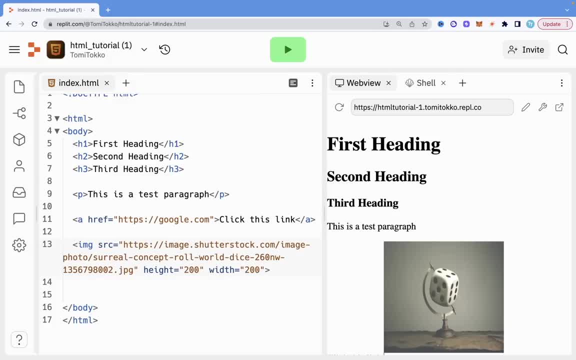 how we can do this, So we can also have another attribute called alt. Now this alt attributes basically tells us, like let's say, more information about this image. So let's say we just want to say the image contains a dice, right? 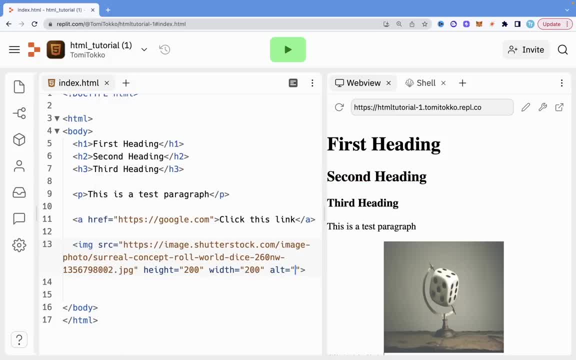 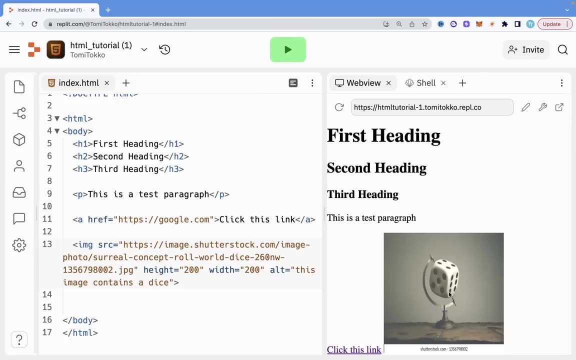 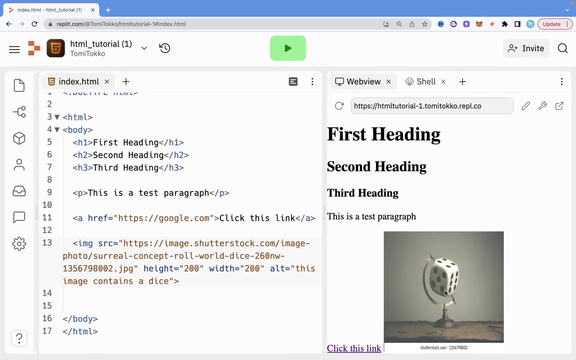 alt equals, put quotes and we can see something like: this image contains a dice. Now, once we run this, we're gonna see that this, as a description of this image, contains a dice. We don't see this right. But for example, if you go to the, let's say, you get the source. 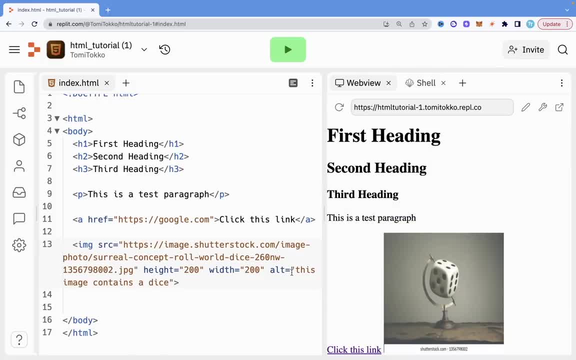 of this image Or whatever. once it's coming with a description, it comes with this auto description, which is: this image contains a site, a dice. Now, this is not what is shown to a user right, But this is basically part of the attributes of this image, So there are also various attributes. 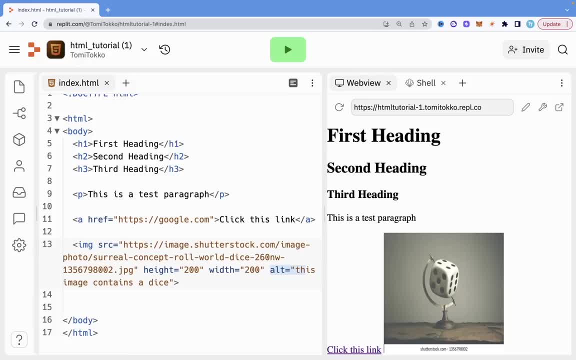 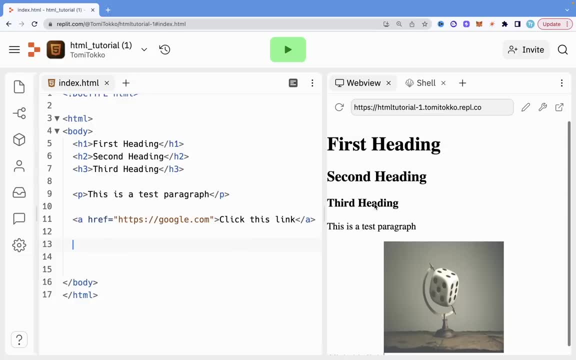 of different things we can use right And, for example, right in here where we have this paragraph. so let me just get rid of this image because we don't need it. So right here, where we have this paragraph, let's say: 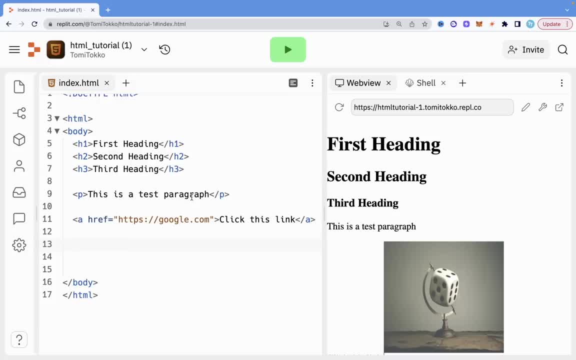 we want to show, like I don't know, maybe- another information of this paragraph. So something like: once a user clicks on this- right, I want to use our overs over this- we want to show that this is a new paragraph or something like that. We use a title attribute. 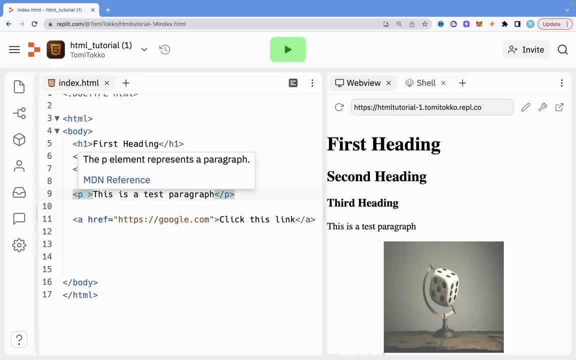 Now this is not really widely used, but just an example of what attributes are. let me say I say title equals this, So and I'm just gonna say test Once I run this, gonna wait for that to show. Okay, So if I come to this paragraph right here, you can see that when I over over this you 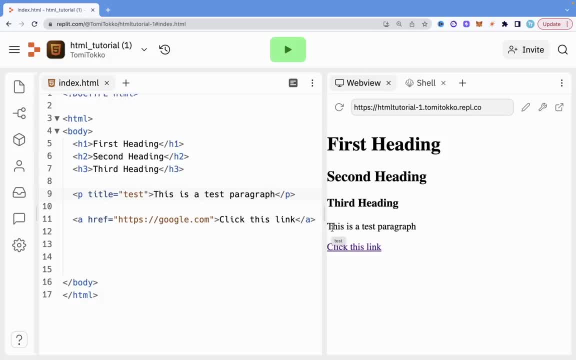 can see that there's a small button that comes up that says test. So that's just another useful attribute. Now, as I said, there are various attributes and it's very easy to make mistake while defining attributes, So you must make sure. let me go through it again. 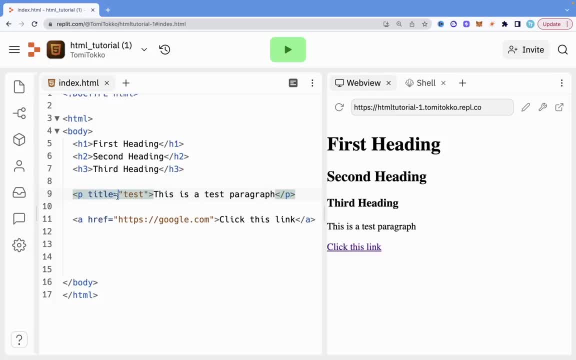 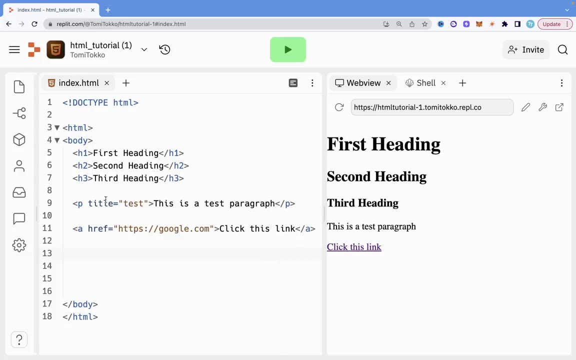 you must make sure that you have the name of the attribute. you put the equal sign, you put the double quotes And in there you put the value of that attribute. If you do that, you can't go wrong. Now let's talk more about HTML paragraphs. So in here I briefly talked about what paragraphs 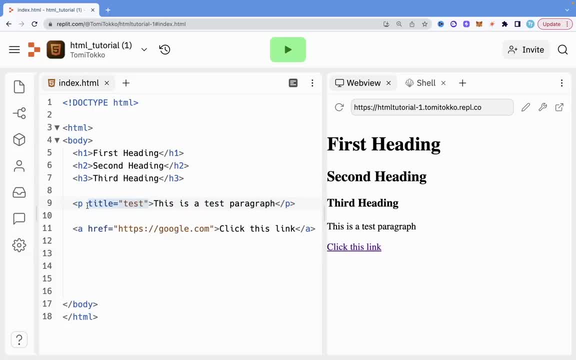 are and how we can use them. So, first of all, I'm going to get rid of this title attribute that I added to the paragraph. So, as I said, we talked about this paragraph right here, But now I want to go deeper into what these are on you know how they actually show in. 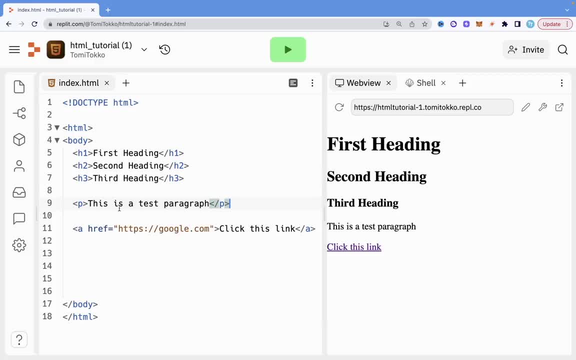 your web page Now, for example, let's say we're talking about HTML, we're talking about, for example, let's say, we have a paragraph right here And we write this like this is a paragraph, And first of all, let me just add this like this and put this year, So just. 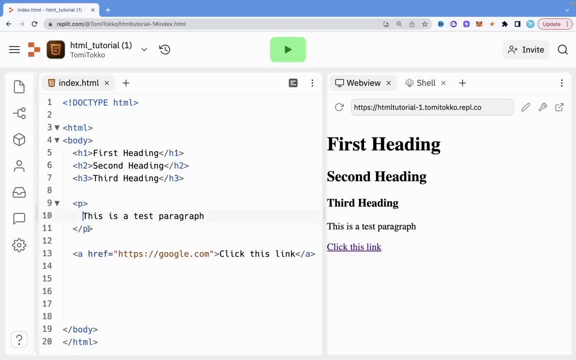 to make it a little bit more structured for me as the code to see. So I said: this is a test paragraph And I say something like: this is a new line. Now you expect that it should print it or you should show it here the way I typed it in here. But no, it's not going. 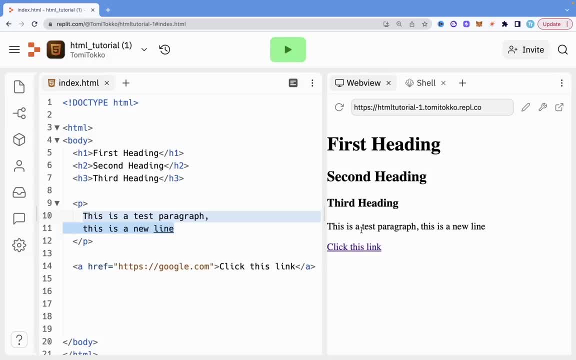 to do that now and you're going to see that it just shows everything on the same line. but most of the time, or sometimes i might not want to do this now, even if let's say i put: let me see, let's run this, and then once you print it, you can see that all the spaces are lived in from a to new. didn't show. 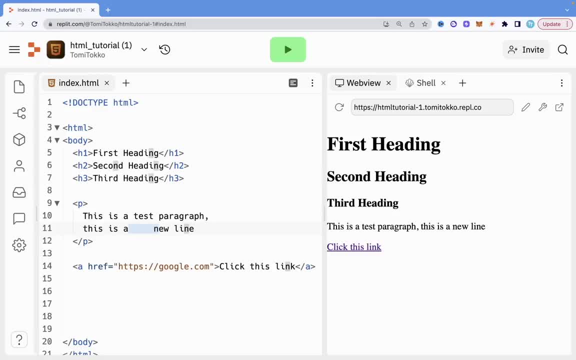 so none of this shows, and there are different solutions to this, because most of the times we might want to create a new line, we might want to, you know, do various stuff. so first of all, let me show you the first solution that we can add to this. so let's say we want to have a brick, right? 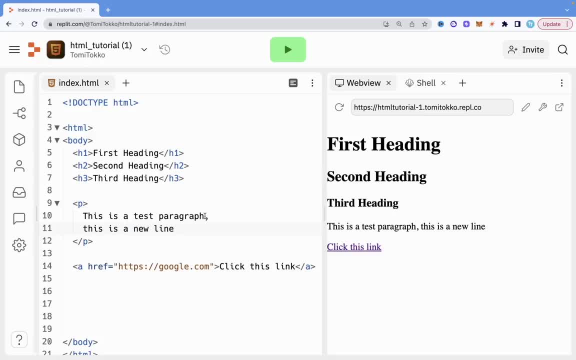 so, for example, in here we want a new line to be created, so we want this text to come to a new line. we can use uh, another html element called break. so it's short form for br, but it's called break. i want you to also use a table to say that if we want to change something here, we just need to do. 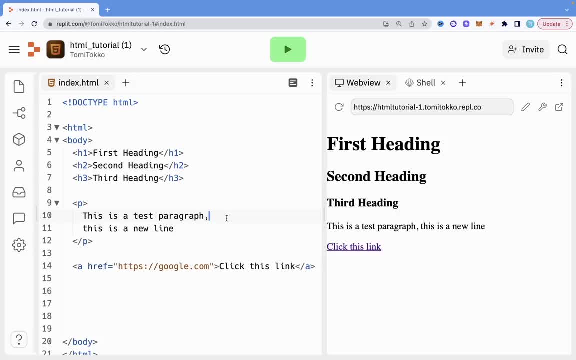 that on the right side of the table. we can't do that on the left side of the table. we can use another. this means is just after that, wherever we put it, it's going to break to a new line. so this is another html element that doesn't require a closing tag, and once again, this is because we are not. 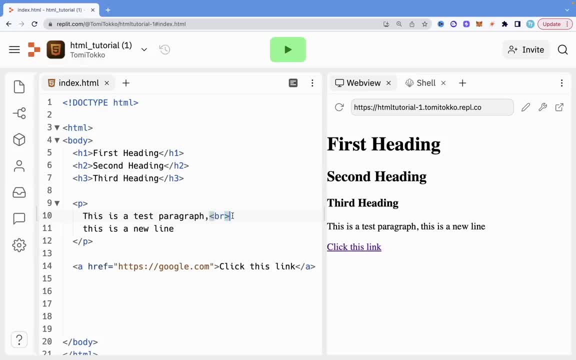 showing any content for it. it's just there to perform its own function. so once we specify this br like this, it's going to create a new line for us, so i don't even need to, you know, make this in a new line. once i just do break, wherever i put the break from, a new line is going to be created. 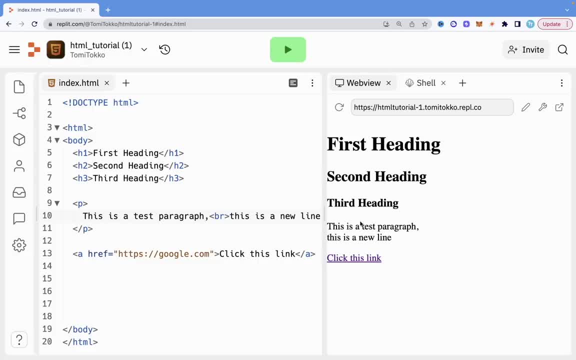 so now, once i run this, you're going to see that it says this is a test paragraph and a new line is being created there. now, that is one solution to the problem, but another solution or the solution i go with when i have this particular problem, don't get me wrong. break is very useful, you're. 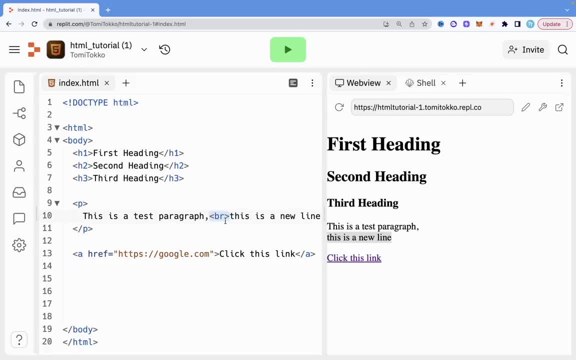 going to use it a lot when you're coding html, but for this type of problem i use the pre tag. so it's basically similar to the paragraph tag, but the difference is that the way we write our code, our text in here is the way it's going to be shown on the web page. so, for example, first of all, let me change this to: 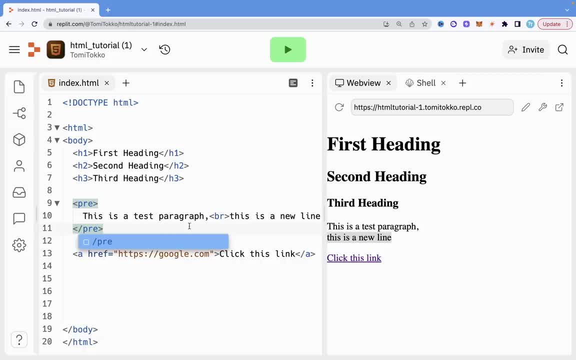 pre. i'm going to change this to pre, so i call it the pre tag. you can call it the pre tag or whatever you want to call it. so let me just have this on a new line and let me create a new line. i say: another line, yet another line and another line. 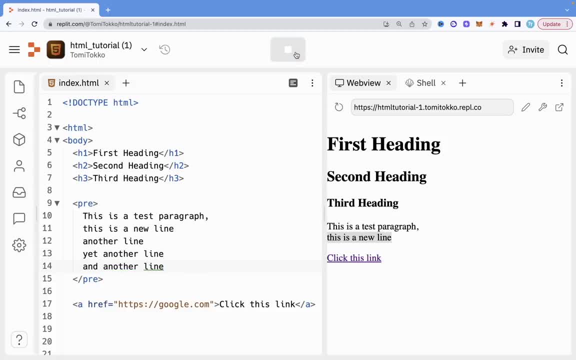 once i run this, you're going to see that the way i wrote this here is how it shows here. you can see that even with the spaces that are put in here is what is showing there. if i get rid of these spaces, let me get rid of all the spaces real quick. you can see that the way we put it in there is how. 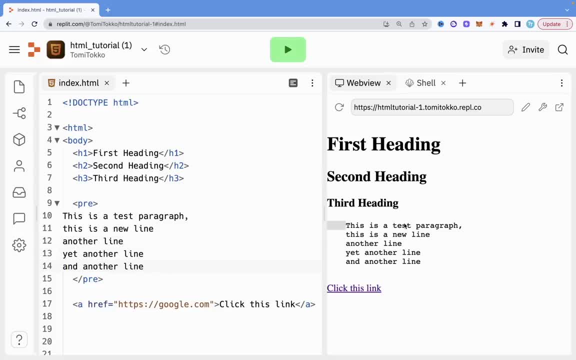 it's going to show for us. now. that is a solution to that particular problem. now let's see it run again. so i'm going to run this real quick. i'm going to wait for that to run. as you can see, everything has been fixed. so that is. 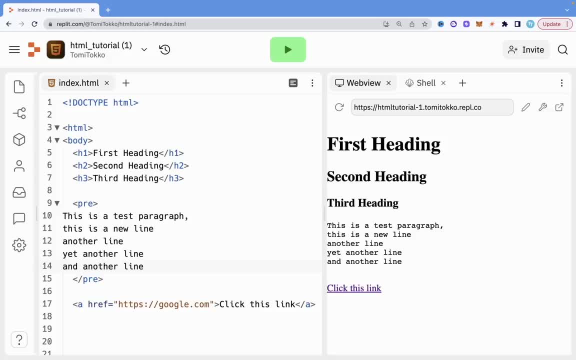 a way to solve that problem in a paragraph tag. now let me show you some other. you know elements that are going to be very useful when writing bare text like this, for example: let's say we want to have a line across this to, let's say, differentiate two different parts of a page. 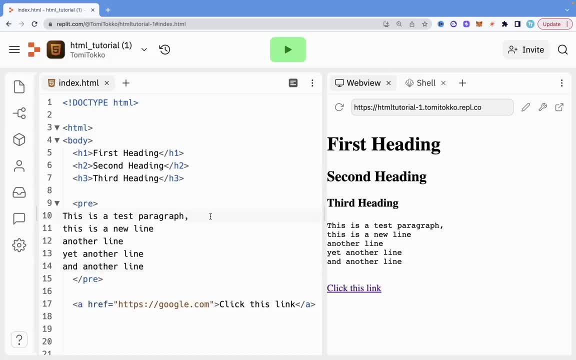 just the way we add the br tag. we're going to have a tag named hr, so this is the way we're going to add the br tag. so let's say we want to have a tag named hr. this tag is an empty tag once i just do hr right, it doesn't have a closing tag, it's just an opening. 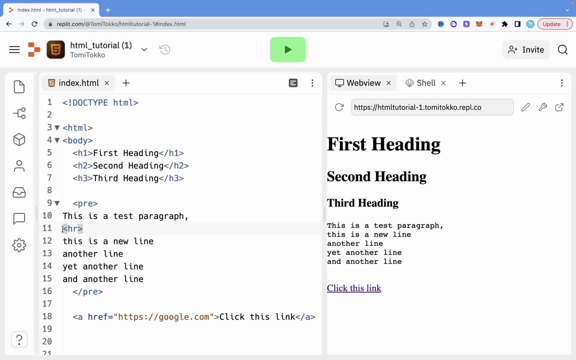 tag. from wherever i do that, hr, there's going to be a line, an horizontal line that is going to be ruled right here. now. let's run that and let's see what that gives us. as you can see, we have a line, it leaves a space, it continues. i can have it everywhere and just say, hr, i can do the same here. 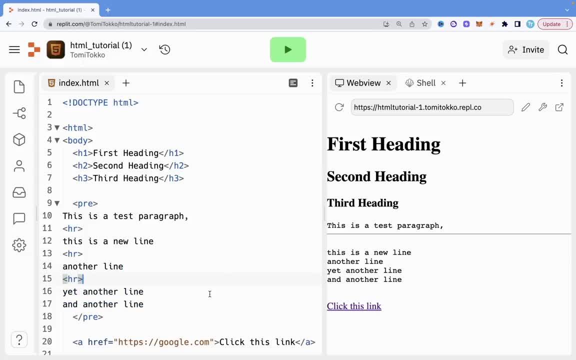 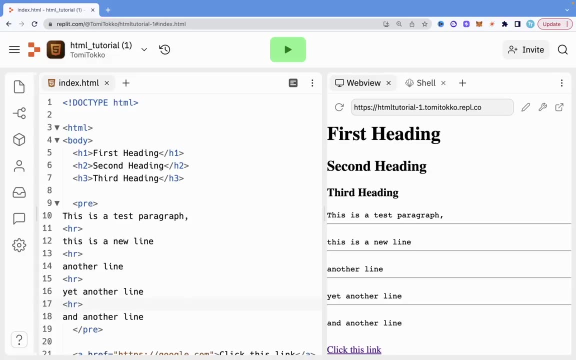 and say hr, and i can do the same here and say hr. so once i run this, you're going to see that lines are going to be created everywhere exact same way, the way we want it, as you can see, structured very well, the way we want it, and that's how to use an hr tag in your html code or whatever you want to. 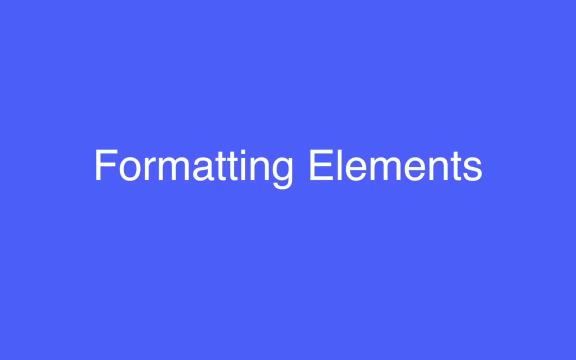 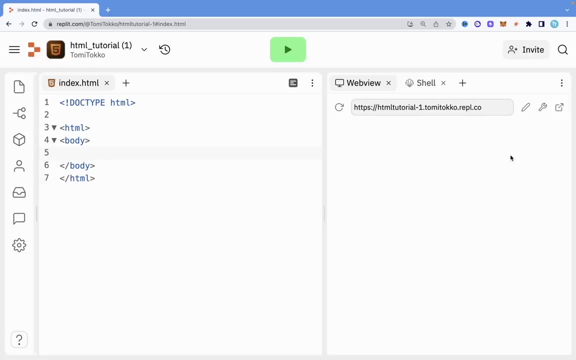 use it. let's say paragraph or another code. now we're going to be talking about formatting text or formatting elements in html, so we might want to show different text in different ways. for example, we might want a text to be bold, we might want a text you know to be superscripted. 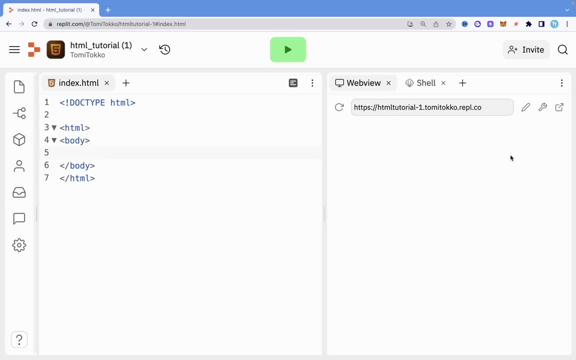 or subscripted, or we might want a text to look like an italic text. so for all of these, we need to format them to look the way we want them to look. so to format it, we need to use html elements, right? so, for example, let's say we have a simple, a simple text in here. that's. 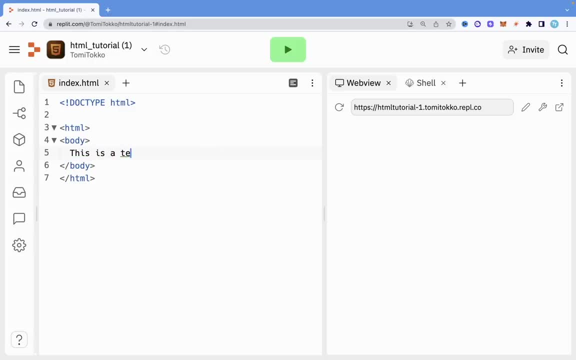 says: this is a text. so once we have a text that says this is a text, right here. if i run this now, make sure that everything is under the body element, as i said from the beginning. so it says: this is a text. but what if i want this to be bold? now for me to do this, i'm going to use an element. 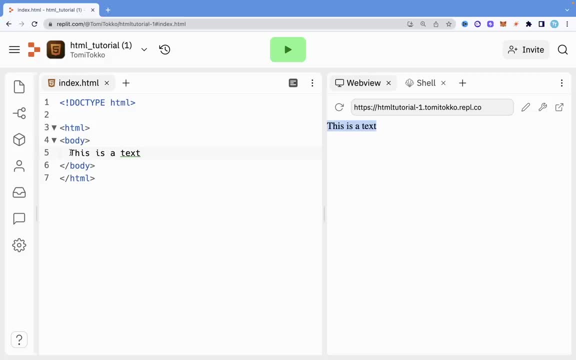 named b and that b stands for bold, so it basically makes whatever content is within it bold. so i'm going to cut this, i'm going to do b, i'm going to paste that in. so now, once i run this, you're going to see that that. 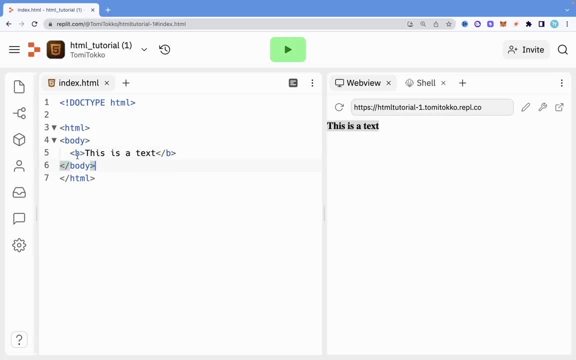 text is bold. so this is how you make a text bold: you open a tag, normally the way we do. you put b, you close that, you put the text in there and then you close the whole tag. so once you have that done and you run it, this should show: this is a text now. similarly, you can also use another tag named. 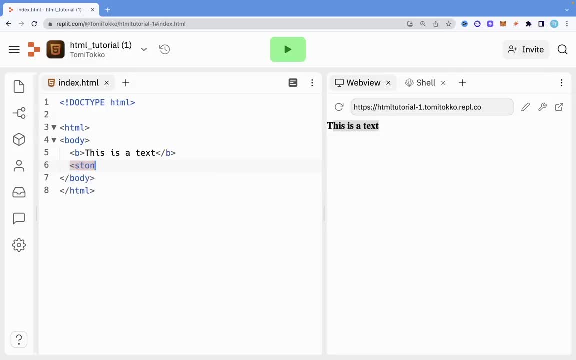 strong. so if i come here and i say strong, right, and i close it and i say this so strong, and once i run this, you're going to see that it looks exactly the same thing as this is another way for you to do that. so let's actually have a br tag here, and we've 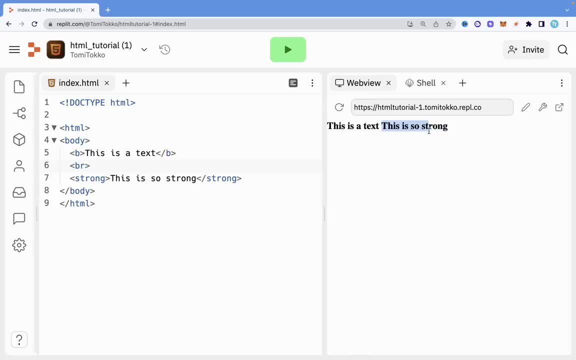 talked about what br does. it breaks the line, just so we're going to have each text we're having on another line. so let me run that and you're going to see that we have that on another line. so that is how you can, you know, use the strong. but what if? let's say, you want your text to show? 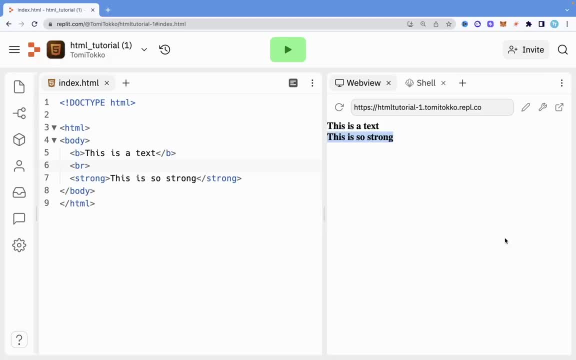 as an emphasized text. so, for example, we're going to use a tag named em, so let me say em and let me just say emphasize. once i run this right, you're gonna see that that text looks emphasized. it looks different from the normal text. so this is kind of going to show the paste pattern. therefore, i'm going to do: this with our strung: elizabeth, you can, you can send like this in that area. but let me tell you this: so, unfortunately, we give restoring to them and i can't give the string the size, because they say that either under the line. yeah, the thing that you want to do is you want to give extension to that line. 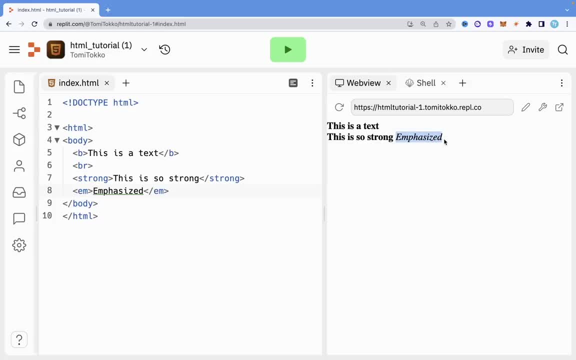 of like an italic text. so if you want your text to look italic, you can use this emphasize, or or you can use the i tag, and this i tag stands for italic. it makes that text italic. so once i say italic and i run this italic text, you're gonna see that it looks italic, right? 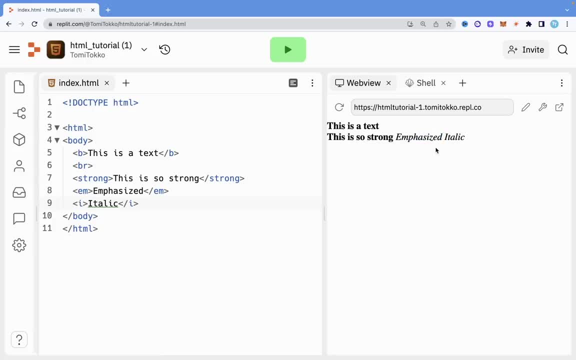 if you look closely, you can see the little difference between it, but they look very similar. so, instead of us having, let's say, a brick, you know, a break element after every single text, what we can just do is to cut all of this and then we can have a pre-tag. 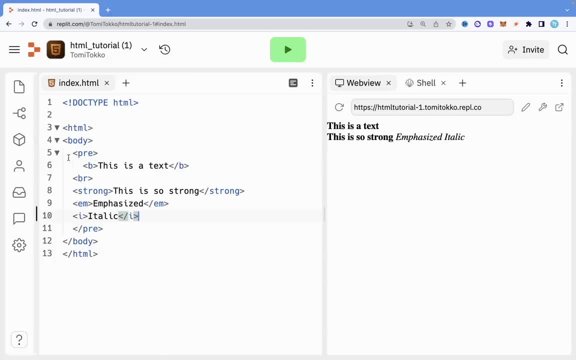 and this pre-tag. we can then paste all of that text in it. and then, when we paste all of that text in it, the way we put it here is how it's going to be shown here. so once i run that, you can see it says: this is this text and all of that. so it leaves the space for us. let me remove. 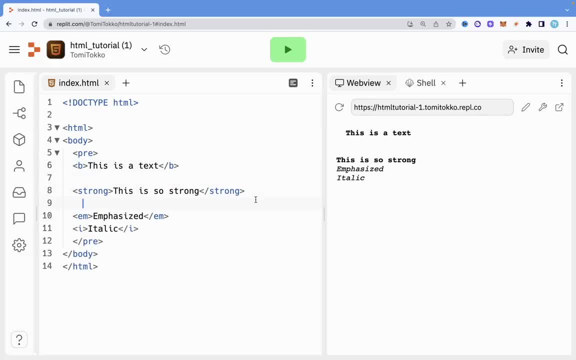 them this, and then in here we do this just to make it look better. so once we run that, that should show the text how we want it right? so once we've done with the italic, we can also mark a text. so let's say we want to do something like mark this, and then we want to have mark. 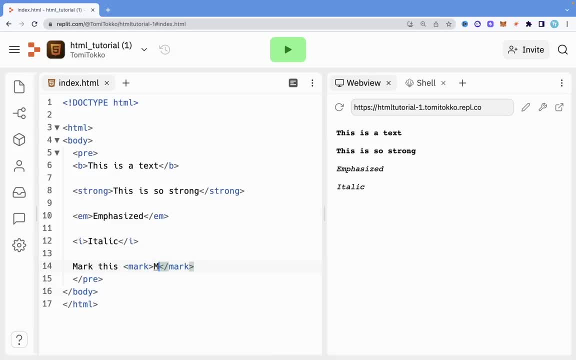 and say marked. i'm going to show you what this does. so, as you can see, it's i like that particular text for us, right? so it makes that text highlighted how we want it. so we can say, let's say we want to say this is an example or this is an important information, and then we just want to mark that. 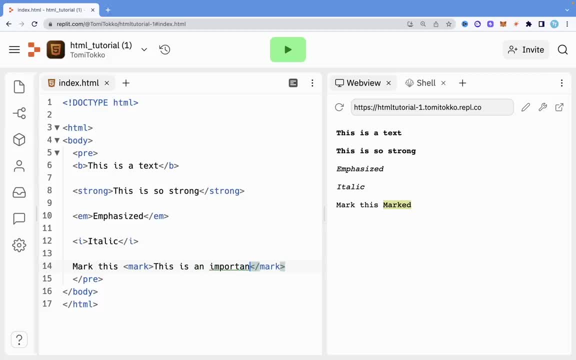 important information and important information run that you can see that it's going to show us that important information highlighted. so that is what the mark element does. now let's say we want a text to you know be cancelled out, for example, you know where you see, maybe on different web pages- and you see something like this is something you shouldn't do. 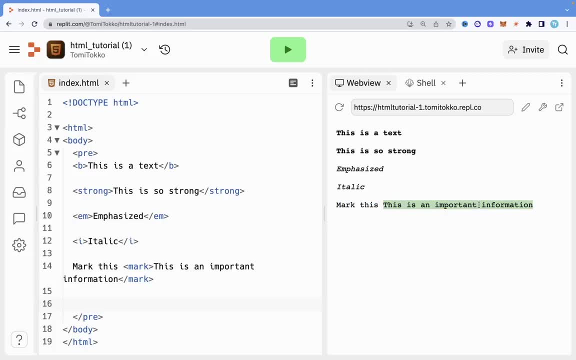 and then you see strike like a line stroking through it. that is the delete element. so let me show you what i mean. so let's say we have a text that says don't do this and we say delete and in there we say do it right now. once i run this you're gonna see that that do it as a strike through it. that is. 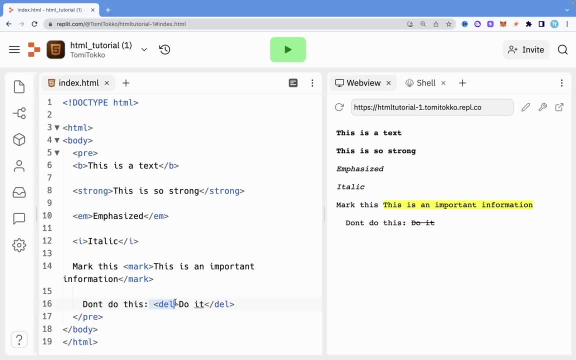 how that is done. if you see this anywhere on the web, it's done using- or you can do it using- this delete element. now we can also have an inserted text. so let me say ins right and say inserted, and if i run this, you're gonna see that it has this text like underlined, or basically highlighted. 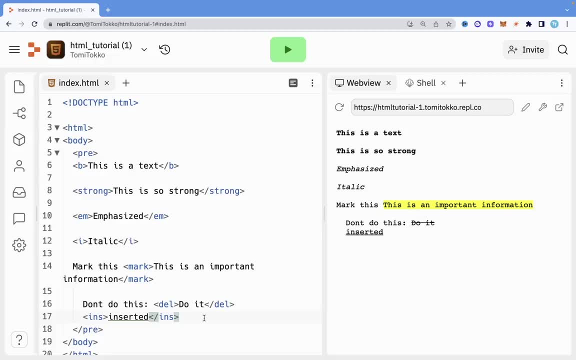 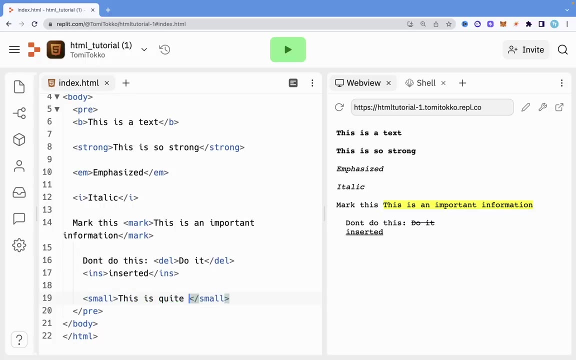 but not in this way, but it's underlined. now, let's say i want a text to be very small compared to what all of these are, so i can say small. i'm going to use a small element and say this is quite small. i run this. you're going to see that the size of this is smaller compared to. 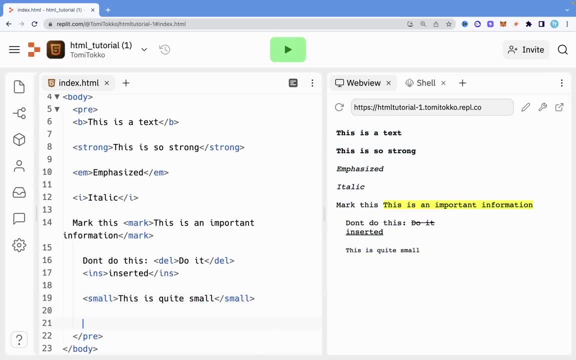 all of these texts- now the last two ones i'm going to talk about- are subscripted and superscripted. now, you know, in, let's say, chemical formulas, where we have something like oxygen, which is like o2, and we want o to show right here, and then we want 2 to show, but we want it to show like on the bottom. 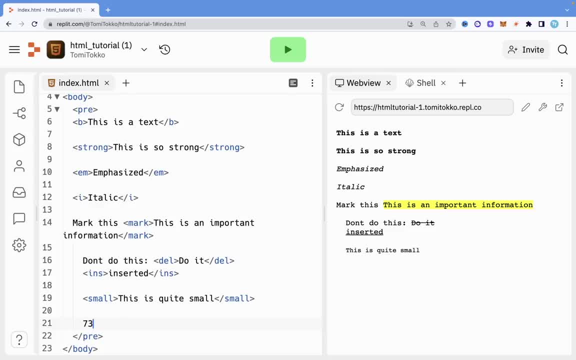 or let's say we have something like 7 raised to power 3. right, instead of doing using this sign right here, we actually want it to show raised to power 3 on there. so it's very easy for us to do this. so for us to do the chemical formula type, we can say o and then, where we have these two, 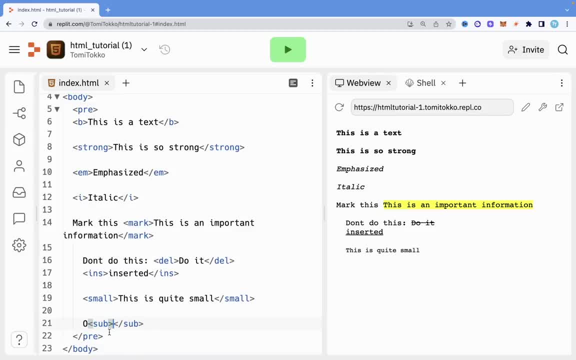 we're going to say sub, so this subscripted means that it should be on the bottom. i'm going to show you what that is. o2: i'm going to run this real quick and you can see that it shows two subscripted compared to o. now let's say i want to have 7 raised to power. 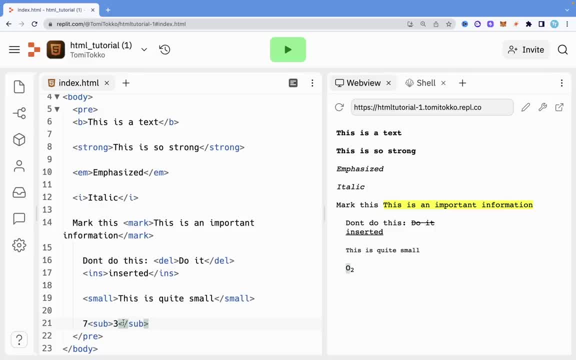 3. this time around. i won't use sub, i will use superscripted. i'm going to change b to p and once i run this you're going to see that it has 7 raised to the power of 3. we're going to quickly talk about colors in html, so i want to go more into like a little. 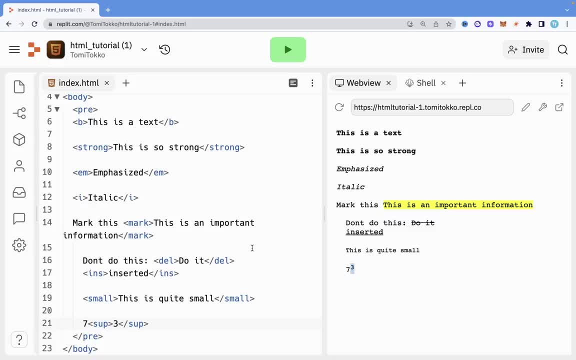 bit of styling of this text, of a particular element. so, for example, what i mean is, let's say, i want this text to, like, have a background color. or i don't want this text to be black, i want it to be, let's say, white or, you know, blue or whatever. now i can use the background color attribute. now let me first show. 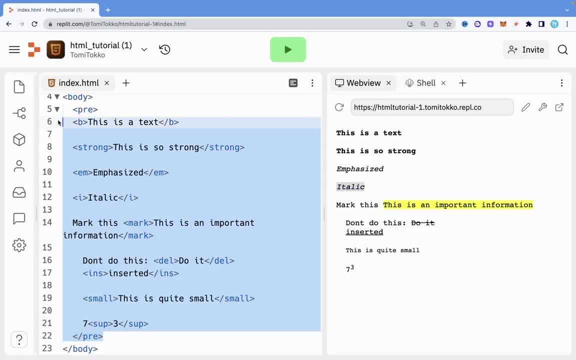 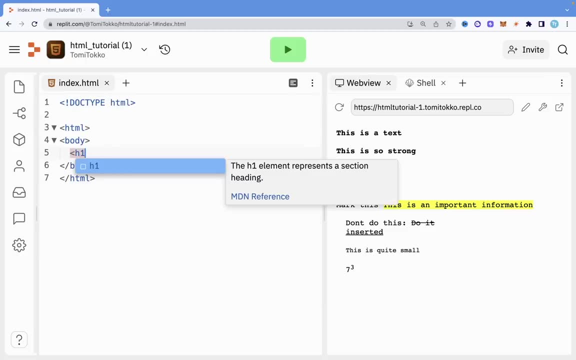 you what i'm going to do. let's get rid of all of this under the body tag and back in the body tag. what i'm going to do? let's say i just have a basic h1 right and i say this is my heading. so if i run that from now, you should see that i have a basic h1. 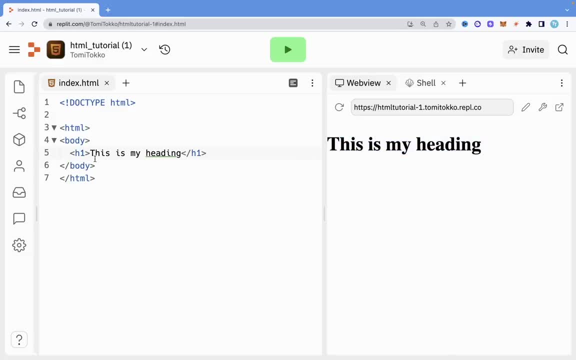 you know that i'm just going to print a basic. this is my heading right, so i'm going to have an attribute. so you know what an attribute is. it gives more information about that element, so we can have an attribute named style. now this style attribute basically gives us a 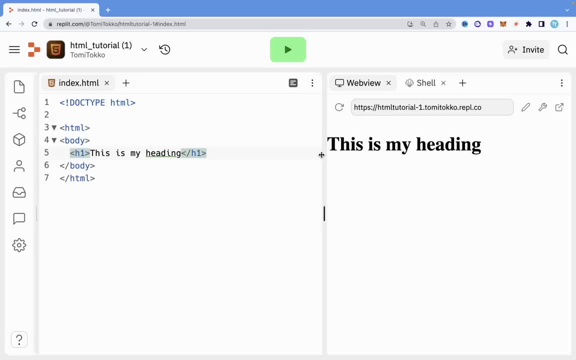 way of designing this particular, you know, element. so let's say i want this particular element or this text to have a color of, let's say, red. so i'm going to say style equals to, and double quotes right in there. i can have different things i want you to do, but we're 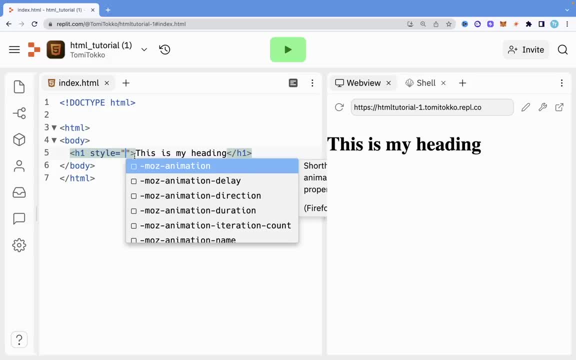 not going to go in depth into that for now, because that is more of like a css type of code which you don't need to know for now. but what i'm going to show you is how we can, you know, make it have a different color. so let's say, i want the color right to be blue. this is how i do it. i just say: 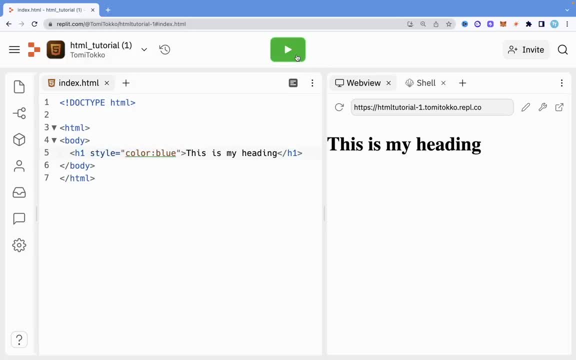 color column blue. now, once i run this, you know see that it changes that color to blue. now this is the simple way of doing this. it's very easy, very simple. you know there are various different like. i will call it like a styling command that we can give it. so this is a styling command in my words. so 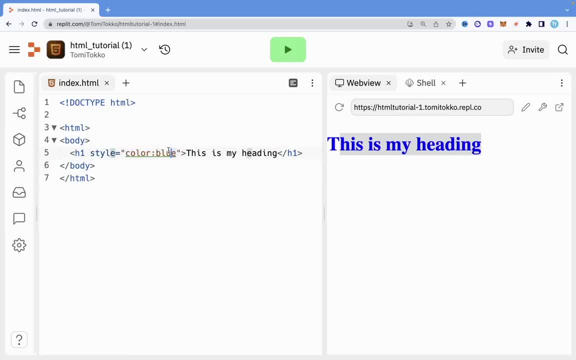 it's like by saying that the color of this particular text should be blue. now let's say we want to have another like, another style to it. let's say we want it to have a different background color on its own. now what we're going to do is to 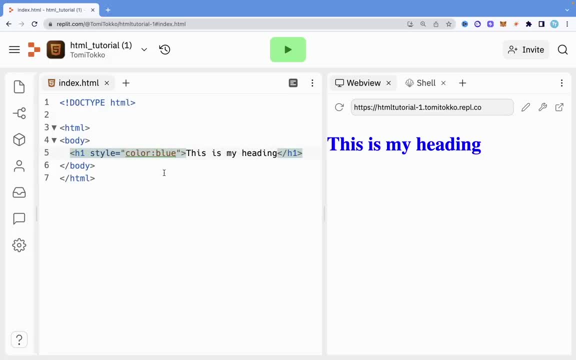 stop this or no, we won't say stop this, we'll end this by putting a semicolon. so this means that after this we can have another styling done in there. so what we want to do now is to just say background, and then we're going to do, i think, color, and now we can change the background color to whatever we 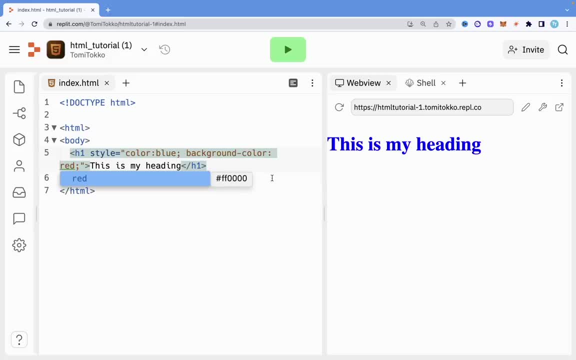 want, let's say, i want the background color to be red, right? so, as you can see, we say background color, we use the colon and then we use the value, right, so the value is red and we put this semicolon to, so that that is where it ends. 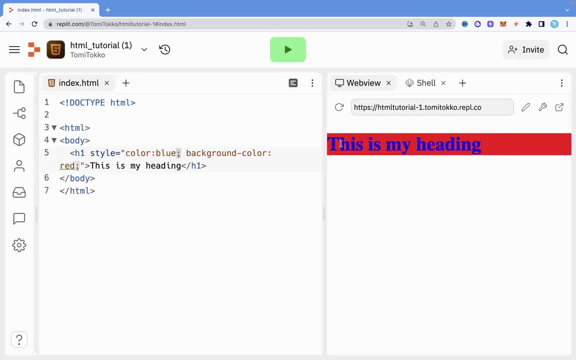 now, once i run this, you're going to see that only that text has a background color of red. now, that is the basic way of you know taking care of colors like that, and there are various stuffs where you can use like css code to style this like we can make this be in the middle. we. 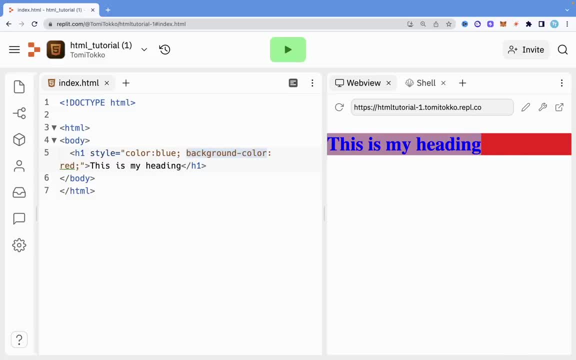 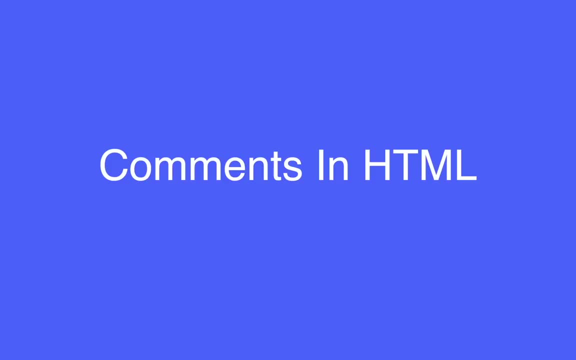 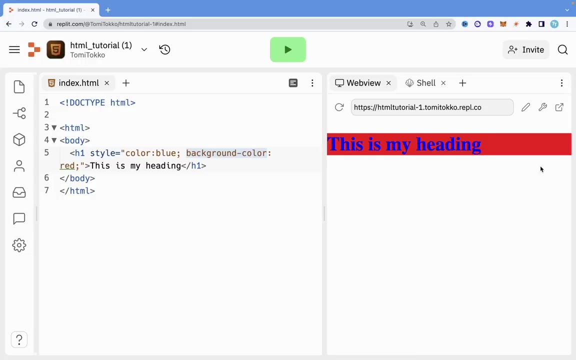 can, you know, do more stuffs, but we're not going to talk about that for now, so that this is just how you, you know, use colors in html. now that we've talked about colors, the next thing i want to talk to you about is comments in html. 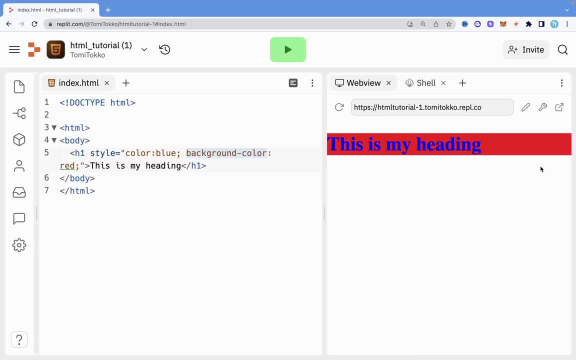 now, this comment is not just only a concept in html alone, it's a concept used generally in programming. so what comments does is that it basically makes a particular block of code not display in you know when your code is run, or something. now let me explain what i mean better. 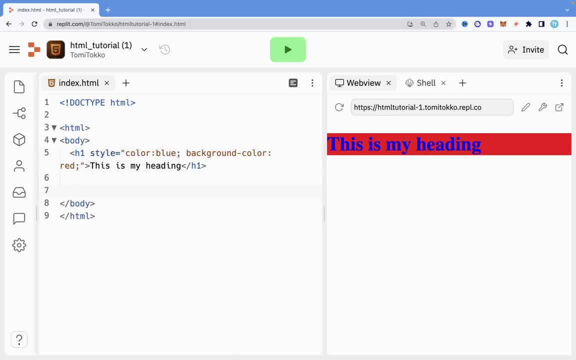 minutes, for example, let's say we have a text that is p and we say a text, so we, we don't want this to show because obviously, when we run this, this is gonna show in here. but we don't want this to show here, right, but we don't want to delete it. also, we don't want to remove it from there. what you can do. 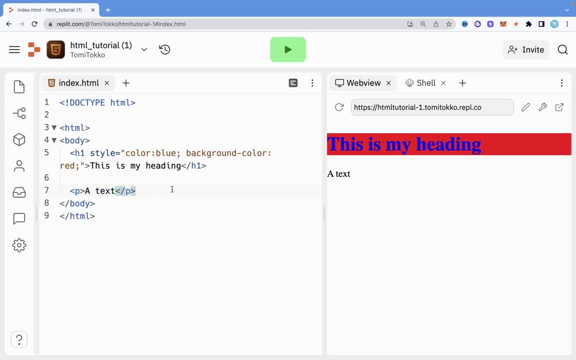 is to comments, that block of code or that line of code. now for you to comment, what you need to do is to use this particular่ syntax. Now just follow as I do. So we are just going to do is to say less than in a. 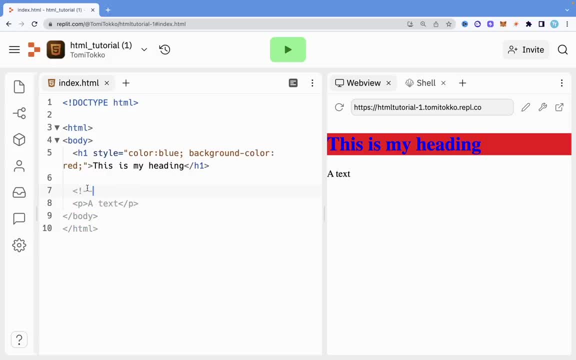 use the sign and then two of this, And then, after the code that you want to comment, you're going to close it by doing the same thing, except with the, the exclamation marks. So, as you can see what that is, it's basically grace this part out. If I run this, you're. 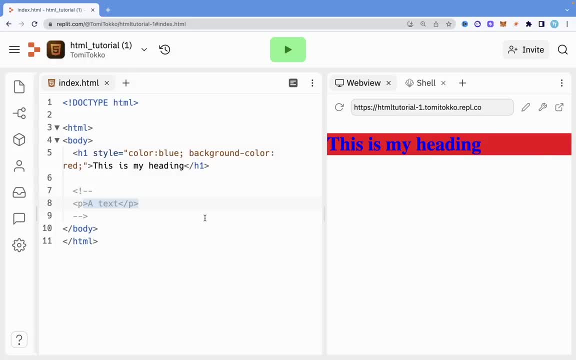 going to see that that part doesn't show. Now, this is a very good use of when we want to use comment because we don't want this particular part of the code to be run when all our code is run. Right, That is a very good use of comments. That is most of the. 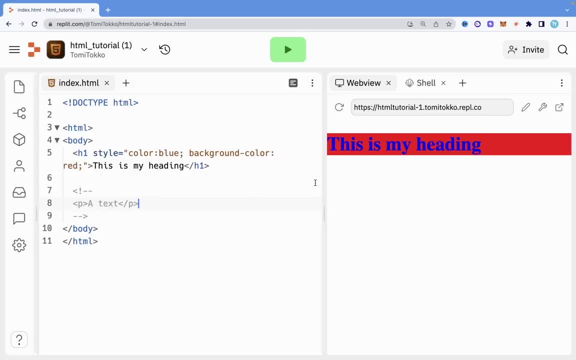 time why I use comments. The other reason you might want to use comment is to actually drop a comment on the code that you are creating. For example, let's say we want to comment and say the code below displays adding that as a blue color. right, We don't just want to write that in and see the code below. 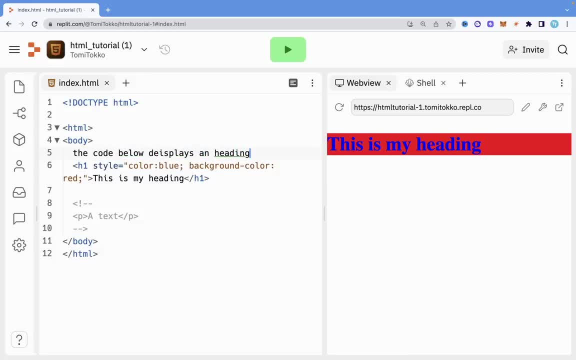 this place And Eden, right, You don't just want to write that there, Because if you write this, there is obviously going to show right here in our code. So let's say, we just want to put it in a comment so that whoever is reading our code we understand what we are. 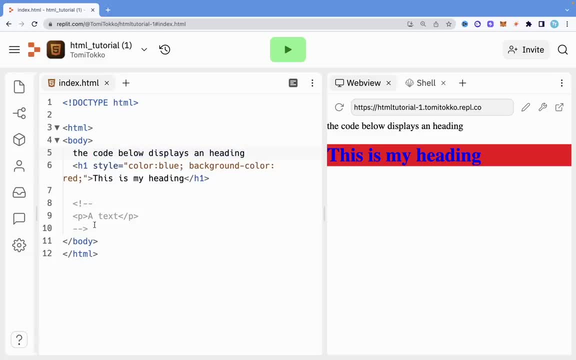 doing So. what we're going to do is to put this in a comment Now, just the same way we did here. we're going to add the same syntax and close it. So now, whoever is reading our code knows that this code here just displays an editing. If I run, this is not going to show with it, no more. 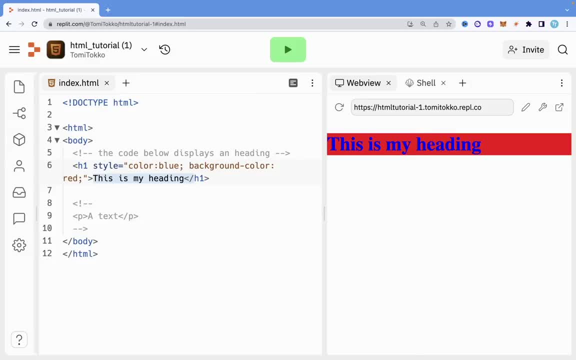 That is because it's only in the source code, right boys, not in the output, So it basically hides that content. Now you can use it, as I said, to hide a code or to stop a code from being executed when you run it, Or you can use it to actually drop a comment on a code. 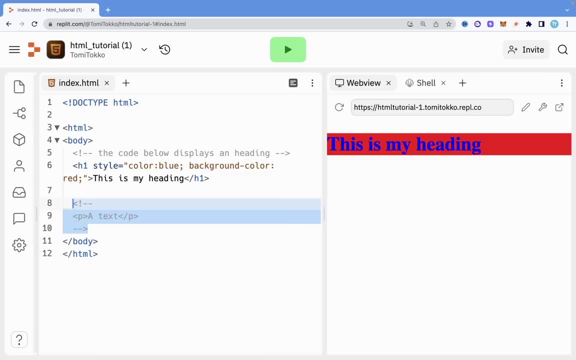 Now we are going to look more into links in HTML. Now, earlier in this course we talked briefly about links And now you can make a user click on a text on a button and it takes the user to a specific link. But now I'm going to go deeper into what they actually 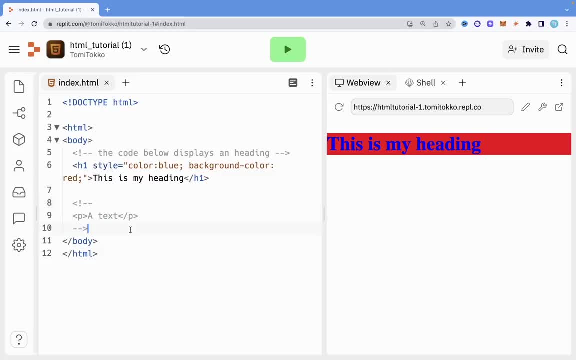 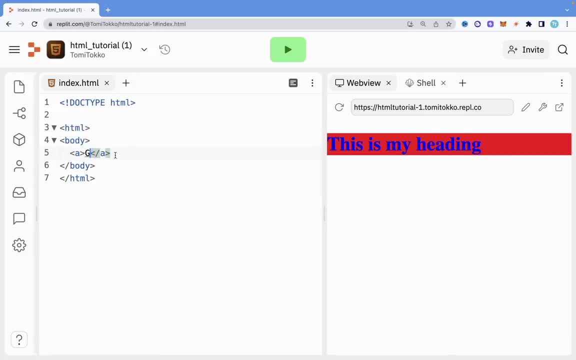 The first thing is we actually created the text page So you can do a close translation: go to site. let's say, go to site, and then we have an attribute named f- href, and let's say: we want you to go to, you know, https, googlecom. 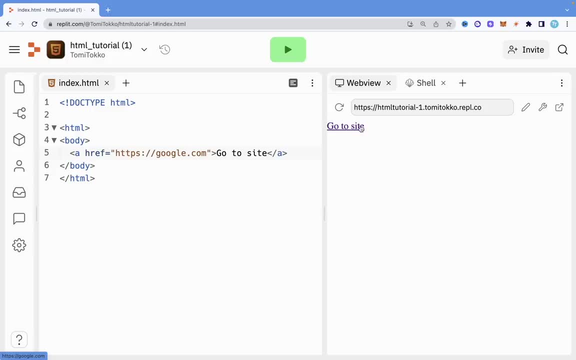 now, once i run this and if i just hover over this on the bottom left corner- left bottom corner- you can see that the link shows that is redirecting us to googlecom. so this is a basic way of just creating a link in html. so i'm going to talk more about like different things you can do with it. 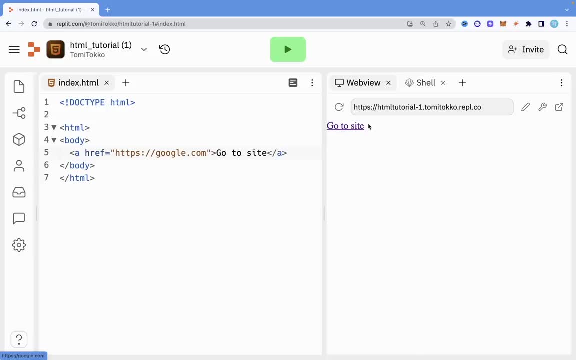 for example, if i click on this go to site, it's probably going to take me to the googlecom, but then it's going to go away from this page and take me to that page. but what if i don't want to do this? so you know, for example, on different blogs or different website where you click on a link, 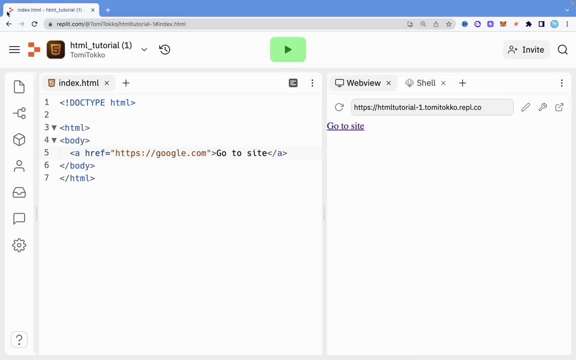 and it automatically opens a new tab with that link, so it doesn't close the tab that you are currently on. you can do that using an attribute named target. so if i say target right and i make the value underscore blank, now this is going to create a new. it's going to create a new tab for us. so let's say i run this. 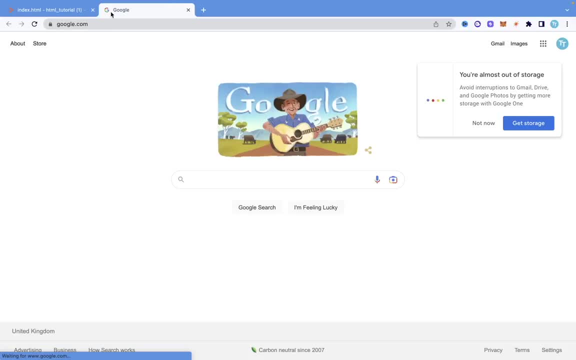 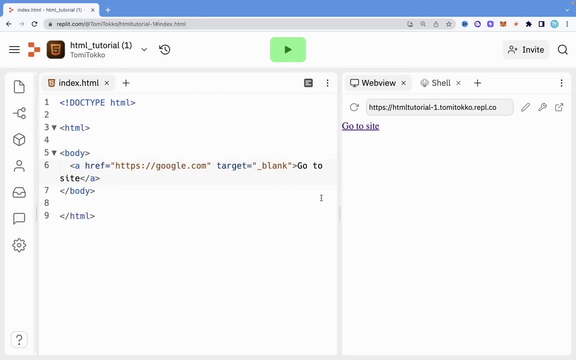 and then i say go to site. you can see that it opens it on a new tab. it doesn't like: go to that site from here. that is what that target blank does. this is very useful because sometimes you might, let's say, you're building an application that you want a user to. let's 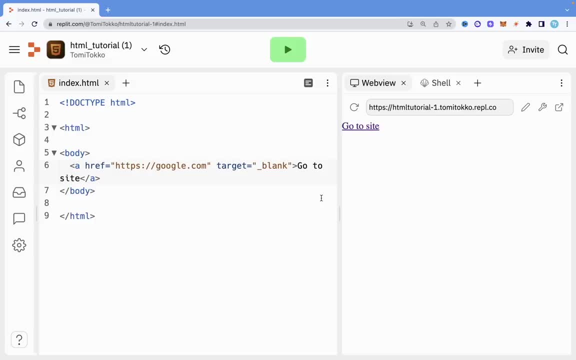 say, view something, but you don't want them to go away from this site, that they are in from your site because maybe there's some things that still need to be changed. this is a good use case of this target attribute. now there are two things called absolute url and relative url. now, if you remember, 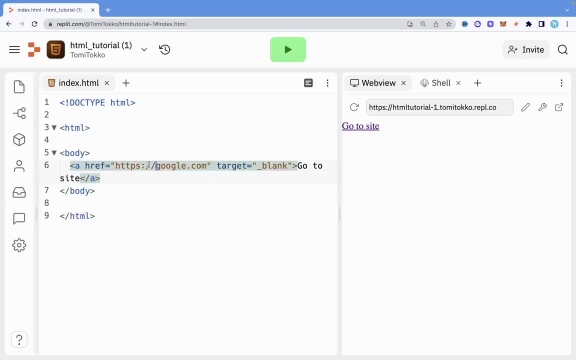 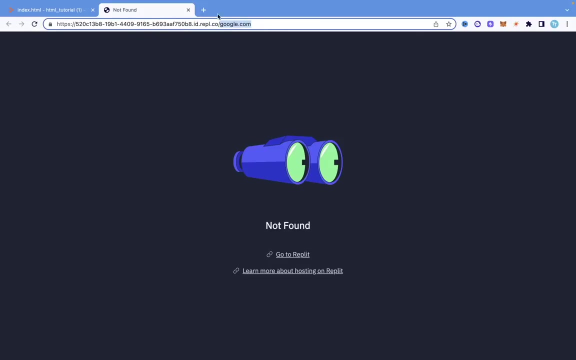 when i was trying to create a new link and i put googlecom right when i run it and i clicked on go to site. so let me just go to site. it's going to open a new tab. you can see what it's doing. it's saying: replico googlecom. now, this is because it sees this url, this link, as a relative. 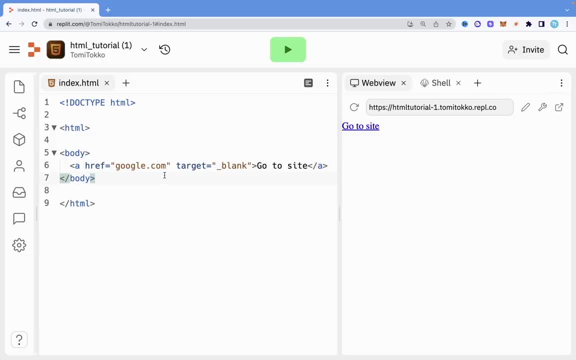 url. now, a relative url means that we are trying to link to somewhere else within this particular web page. so it's basically seeing something like, let's say, i just say slash um, slash go. so it's basically going to go to replicom: slash tome, to go slash all of this slash go. that is a relative. 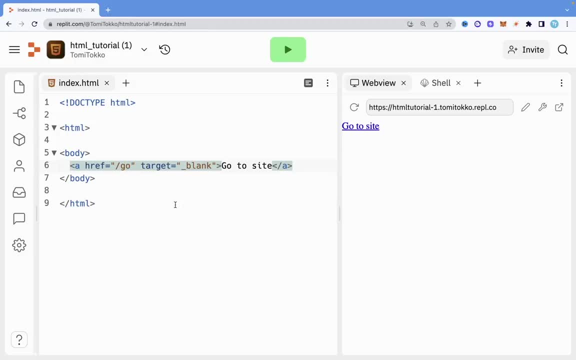 url is is just going to this particular url, this link within the local, you know the local application or the local website. well, let's say, we want to go to an external website, like the way i went to googlecom. now that is an absolute url. that is when we have to do the 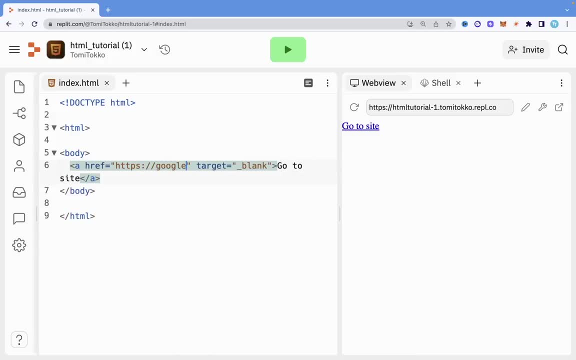 https right, and then we have to specify the site that we are going to. so now that is an absolute url. that is the difference between both of them. so we can also link to different things, like, let's say, we want to link to an email address. so let's say, we want to say something like: let's have an a. 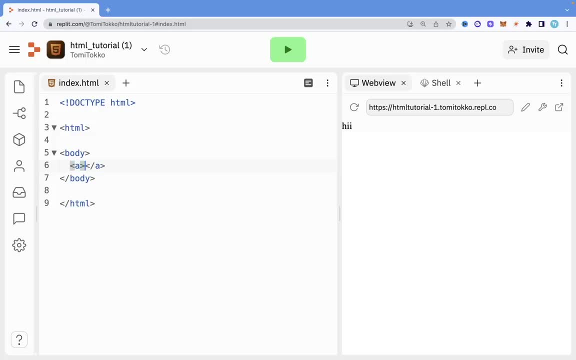 tag. i want to say: send me an email, and one that once the user clicks on this, it's going to like: open a new tab by sending an email to a particular- you know a particular- email address. first, to do this, we're just going to say href equals. now we are going to specify the link, what we need to 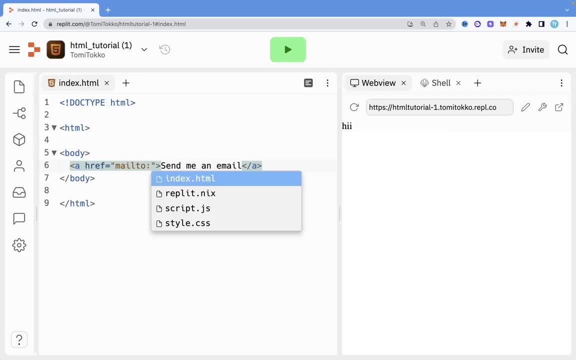 specify the mail to colon and then we're going to put the address so we can put sample at samplecom. so, for example, we run this right. this is going to show me send me an email and if i open it it's going to right. it says mailgooglecom refuse to connect, but it basically opened. 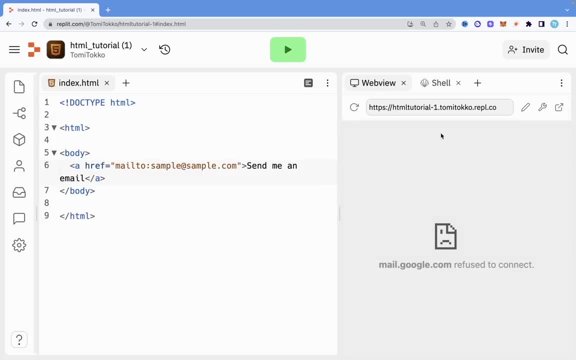 gmail and tries to, you know, send an email. so this is just not showing because we're under like this wrapper. but let's say you have your own website and you use this. it's basically going to open a page where you can compose an email to that email site. now we are going to talk about titles and 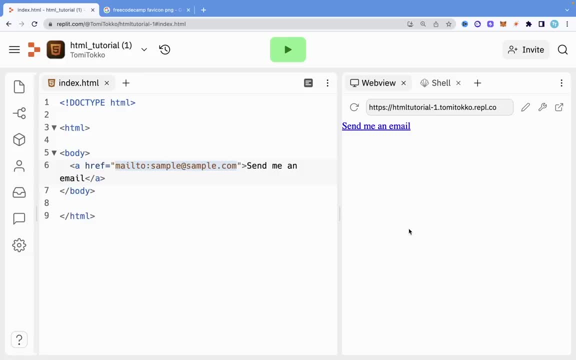 favicons in html, so a title is very simple and very straightforward. so what is it? what is it? basically? the text that is shown at the tab or at the top of the tab on a web page. for example, on this web page, you can see that what is shown is this indexhtml html tutorial replica, that is: 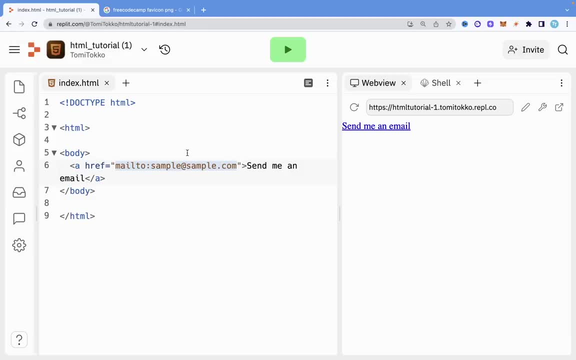 the title of this page. so for you to specify the title of a page right, you need to have an edge element. so, right after the html tag, we're going to have this edge tag right here and we're going to close it now. this edge tag basically contains different, you know- information about. 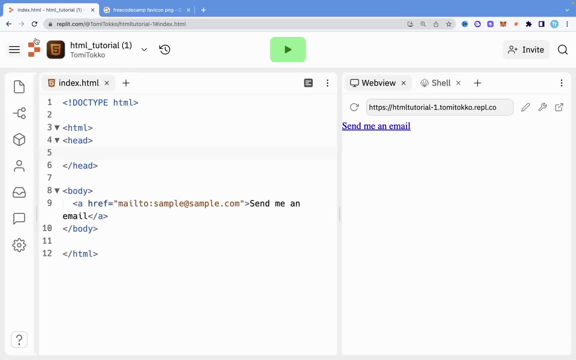 the page. some of it is information about the top corner, like the icon that shows here, which is the favicon, the title and some other information. but in this part we're going to be looking more into this title and this icon that shows here, which is also known as a favicon. so first let's look at the 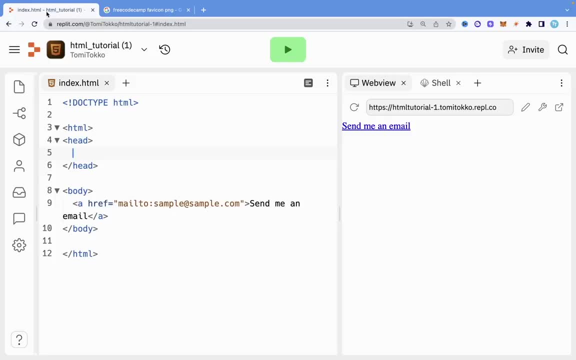 title. so, as i said, the title is the information that has been displayed in here. so for us to set the title of our web page, what we're going to do is to open a new tag and say title, and this title tag must be in the head element. so this is also another nested element, just like the way i talked. 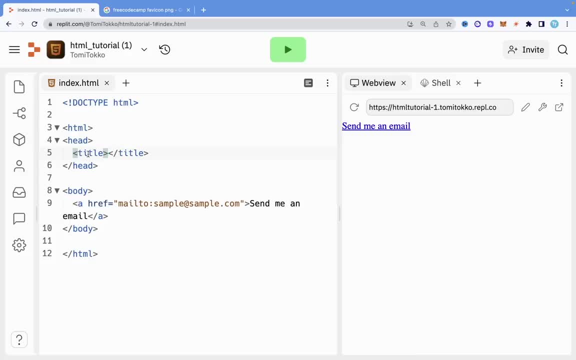 about previously. so now this title element must be under this head element. so what i can just do is my page, so i can say my page is the title of this particular you know web page. now, if i run this right, we're not actually going to see anything here, because this is just like a you know a demo of this, but let's say we have. 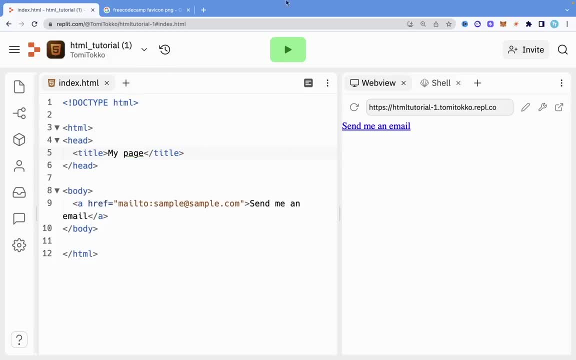 our website. we have our html file and we run it on our browser. here you're going to see that the text here is going to be that. now i'm also going to show you how to you know, create your html files on your local computer and actually run it on your browser so you can see, like this type of 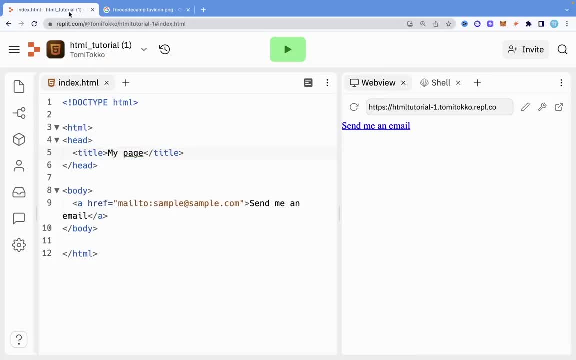 example. but for now, know that this title is what is being shown here, and the next thing we're going to talk about, as i say, is the favicon, and this favicon is known as the logo, or the image that is shown before the title on your page. so right here you can see i have this tab and you can see. 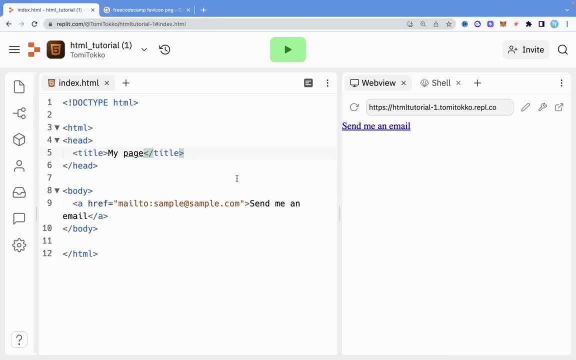 this google logo. that is the favicon. so to have the favicon, we're going to have the link tag right and then the way we close the link down is just to like that. we don't close it because it's similar to an image tag. we are not actually writing a text. 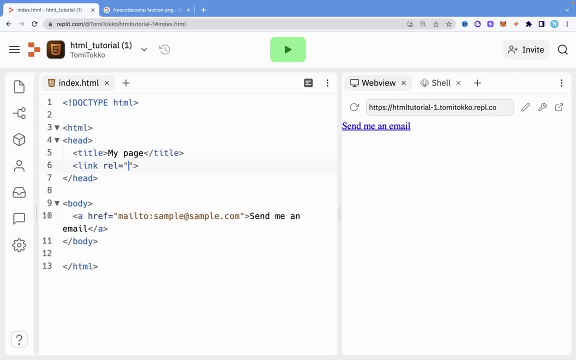 so in here i'm going to say rel, that is an attribute, i'm going to give it, and i'm going to say it's an icon, right, and i'm just going to say href, which is the link of where i want to get that favicon from. let me say, equals this? now, let's actually get that link. 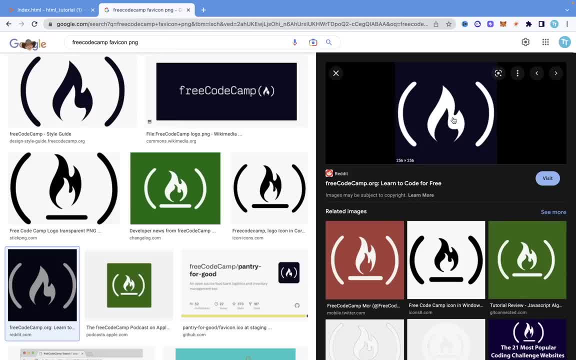 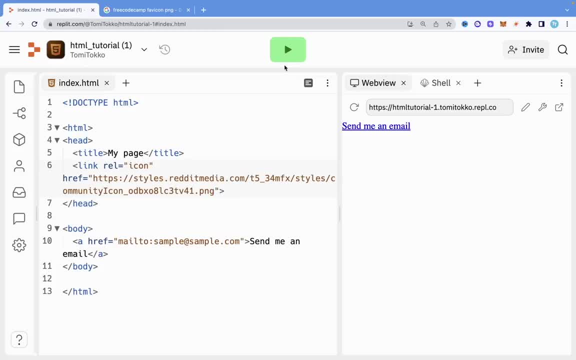 right here. i just searched frequent cam favicon, pmg. i got this and i'm just going to copy the image address. i'm going to come in here and paste it now. if i run it once again, this is not going to actually show here, because this is a demo of this, but when i show you how to, you know. 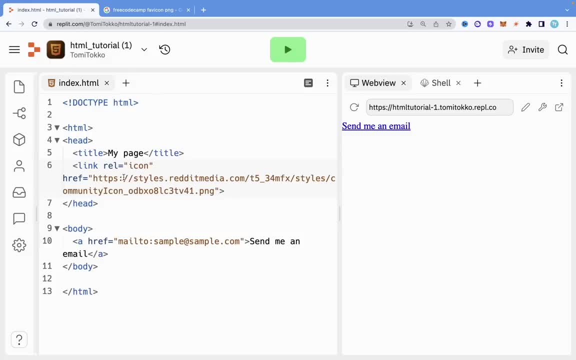 run your html file on your browser. you're going to see all of these details. but that is how to use a favicon and the title in html. now let's talk about tables in html, so a table where you can just basically represent data. i'm going to show you how to use a favicon and the title in html. 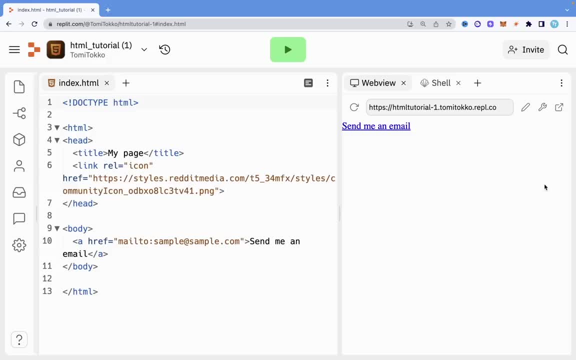 you how to create that right now. so, as you might have guessed, we're also going to use another element, and the element we're going to use this time around is going to be called table. so let me get rid of this right here and i'm going to get rid of this link right here. 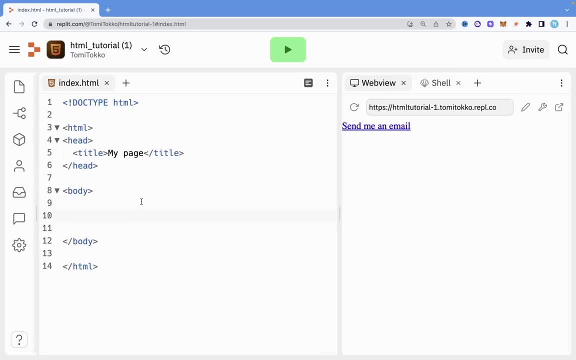 so, in the body, what i just want to do is to create a new table, so just a normal table, right, just a normal table, where we have the editing and then we have the datas that this table contains. so for us let's say table, and then we're just going to close it, just like that. and for us to now create like 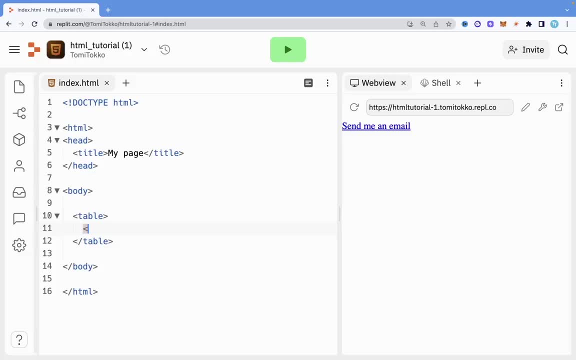 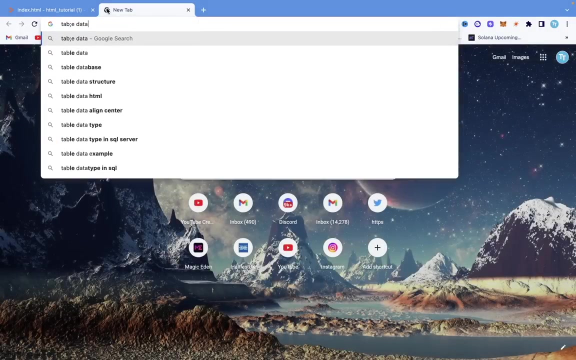 a new row. in that table we're going to use another tag named tr, so this stands for table row. so in this table row i can say something like: let's say: i want to have- let me visualize this. so let's say table data, let's look for images. 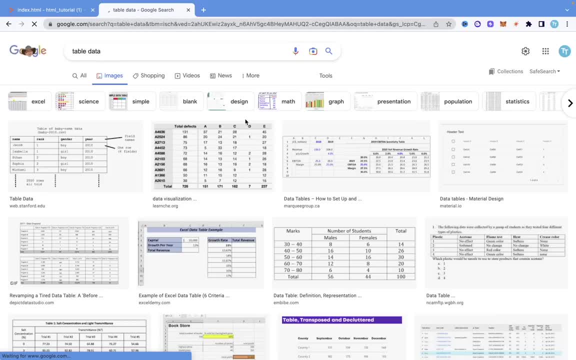 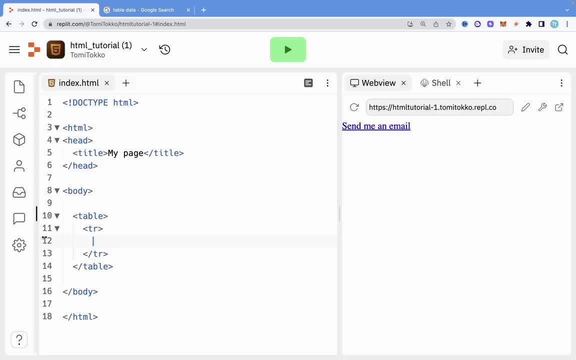 so let's make that table good. so now, for example, we have this right, so this is going to be a row. so what we just created right here, this tr, is a new row. right here i'm, let's say, i want to create another row to store all of this. 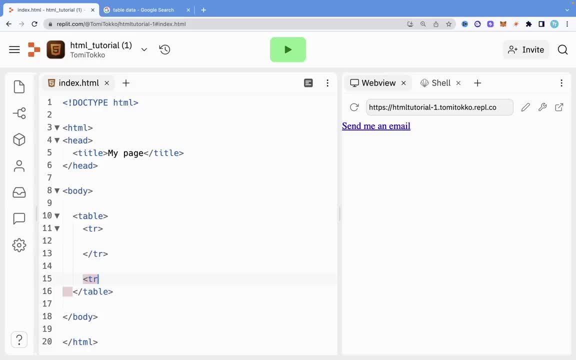 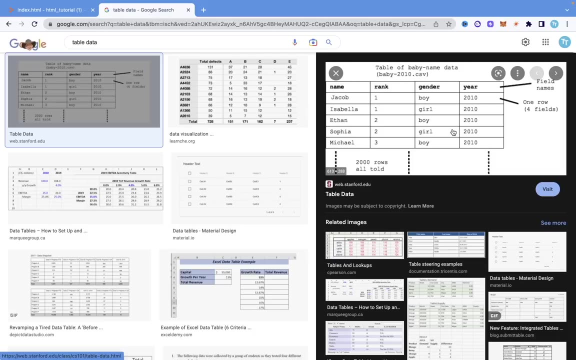 data under here. i'm going to create another tr, right, and i'm going to close that, so this means we have two rows now, so we can keep doing that for the amount of rows that we want. so what we can now do is that under the first table, we're going to create another row and then we're going to create 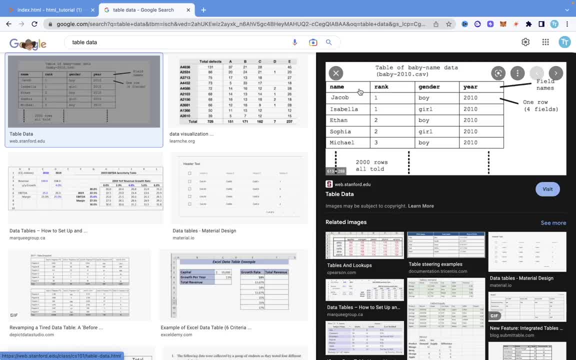 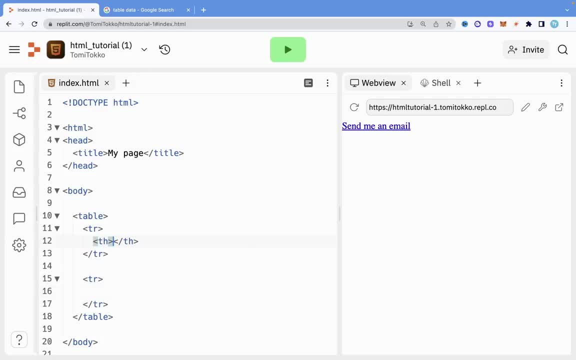 another table. so we're going to test row. we want to have the editing, so we want to say name, rank, gender and, yeah, all of this heading. so for us to do this, we're going to use the tag name th, which is also known as table editing. so that table editing, we're just going to do this real quick. 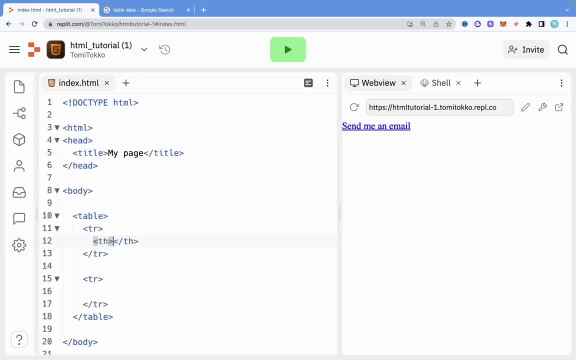 so this th is going to be the headin, so let's say something like name, so this is going to stand for name. we might want to have another table heading named age. and then let's say to say something like plus right. And then if I run this, you're gonna see what we have. 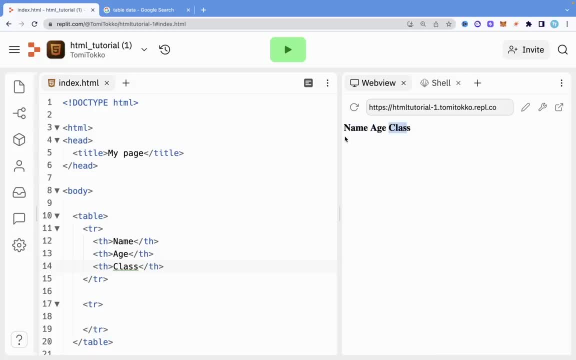 So you see that we just have name, age and class And let's say, on that, these. now I want to have a name like, let's say, told me and my age, and I might pull a class. So what I'm just going to do is I'm going to create a new row, as you can see, already did that here. 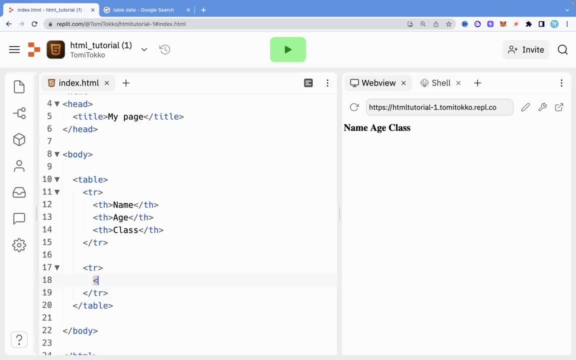 So now, instead of doing th, what I'm going to do is cd. So this means were adding a table data, not a table adding right. So you only use th when you have, when you specify the head of the class, So of that table data, but for the values we use td. So let's say: 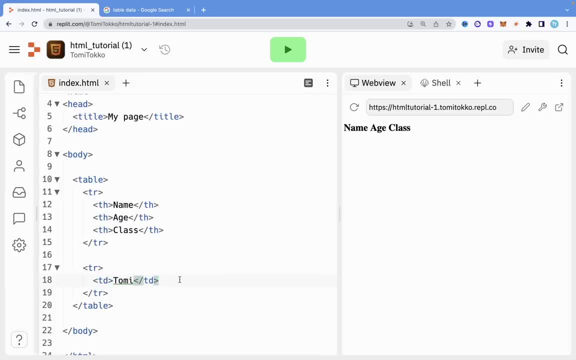 something like Tommy, And for the age is another TD and let's just say 18,, 19,, 20,, 21,, 22,, 19- let's just put a random age there and another td. let's get rid of that. let's use small letters. 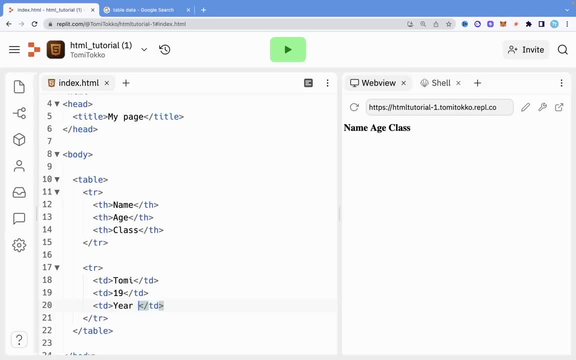 and it says class and we can say year- i don't know, year 20, 12- and then once we run that, you're going to see that we have this basic table that says name: tell me 19, year 12. now we can keep adding more rows. what we just need to do is to do tr and under tr, i'm going to have td. 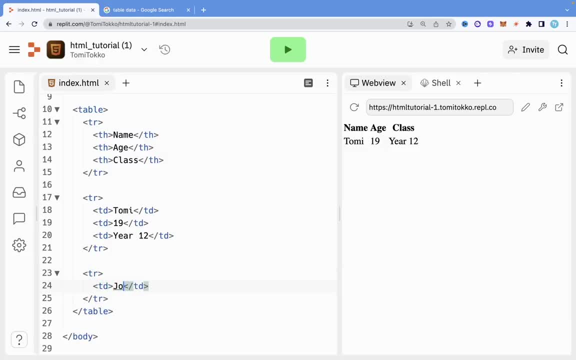 and i'm gonna. i can use another one and just say, john, i'm gonna have another td and let's say the age is 30 and let's say, um, he's in year 15, or something like that. and once i run this, you're gonna see. 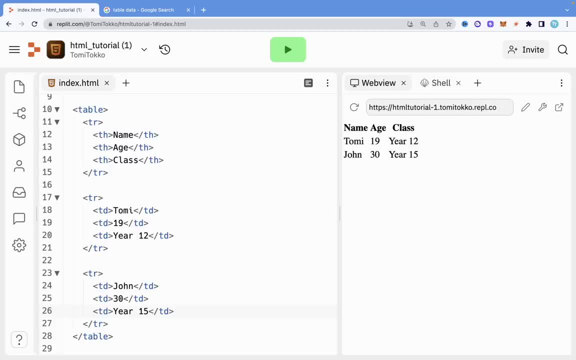 that we basically have a simple table that shows that. so, as you can see, it just shows the, you know. adding it shows the data which is tommy 19, year 12. it shows john 30 and all of that. so that's basically what we need to build a table: very simple and very easy. we make sure we have the 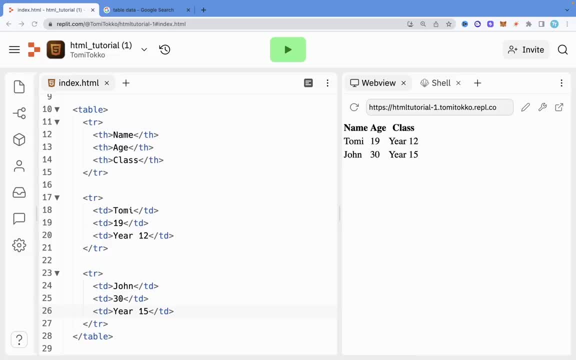 table class. we make sure we have the tr and then we make sure we have data in between. now let's talk about lists in html. so let's say we want to have a simple list right here that just lists, let's say a list of names, a list of years or whatever. first of all, let's get rid of 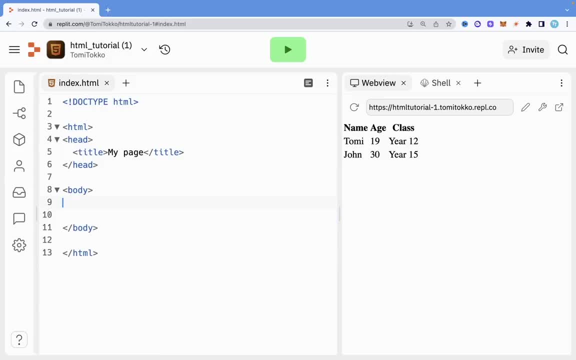 this table that we created. i'm not talking about that now. so what we're talking about is lists. so there are two types of lists. they are unordered lists and they are ordered lists. now, another list are the ones that just have like a simple bullet point mark between them, i mean before them. but 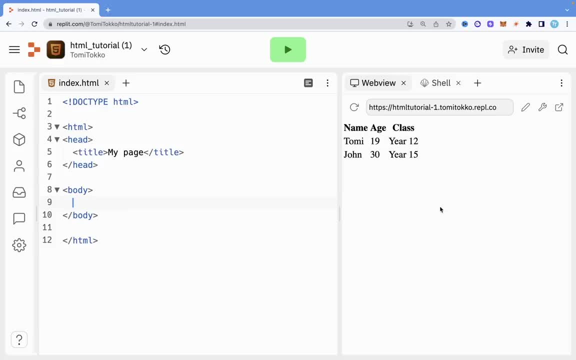 another list is listed from one, two, three, four, basically numerically. now let me show you what i mean now. for example, let's say we want to write an unordered list, we need to use a tag named ul. once we use the ul tag, we need to open and close that tag. i'm going to press enter and for us to. 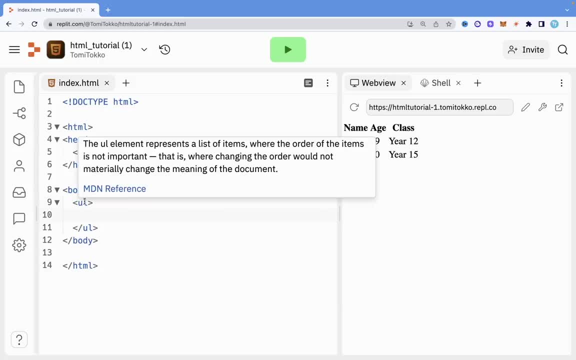 now add list. this ul stands for unordered list, so for us to now add elements in this list, we're going to have to use the li stands for list. am i going to say something like name one? and we can do the same thing. to have a second name- li- we're gonna say name two. let's have a third name, say li, i'm gonna say name. 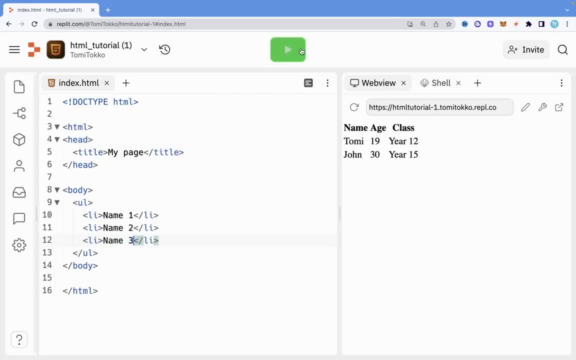 three. so, as you can see, we have three different names. if i run it, you're now gonna see that we have name one, name two, name three. now this is shown, listed, but it's not ordered. it doesn't have one, two, three, four, five and so on. if we want it to be ordered, like to show in ascending order. 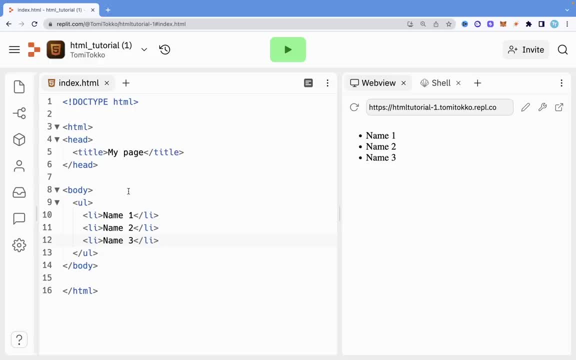 then what we just need to do is to simply change this ul to ol and this ol means ordered lists. so if i change that right here and i run this, you're now going to see that they have numeric numbers before them. so if i keep adding and let me say another list and i say name four, 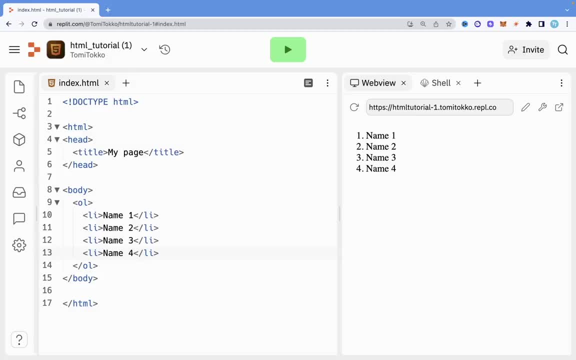 it's automatically going to add four as a number before that. now they are also more to least like. for example, we can show a description of this name. if we want to do this, we need to change this order list to description list, so this description is basically allows us to show more description on each list if we want to. so what we're going to? 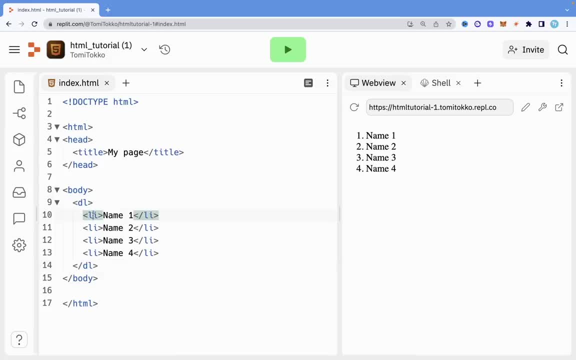 do now is we change that to description list and let's say, on the first list, we want this to be dt, not li. that's the difference. we're going to remove all of this real quick, and under that, let's say, we want to have a description of this name, one we're going to use dd. 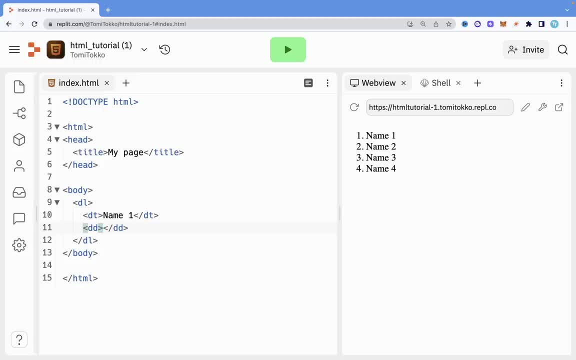 and let's say something like um, let's have like an asterisk and say: this is the first name. now, once i run this, you're going to see what it shows us. so you see that it says name one and under here it leaves like a space and it says the description of that name. we can add another one. 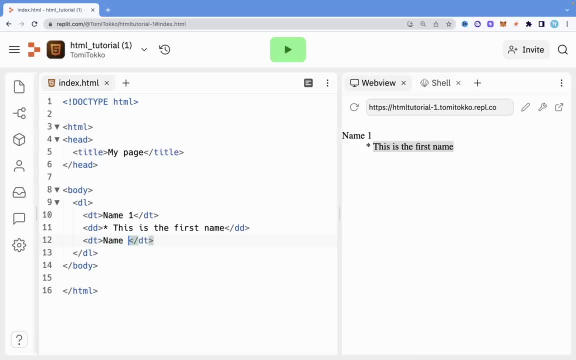 and just say dt and just say name two. and now, to show the description of this, we just say dd and we can have the asterisk again and say this is the second name. now, if i run this, we're now going to see that we have name one. 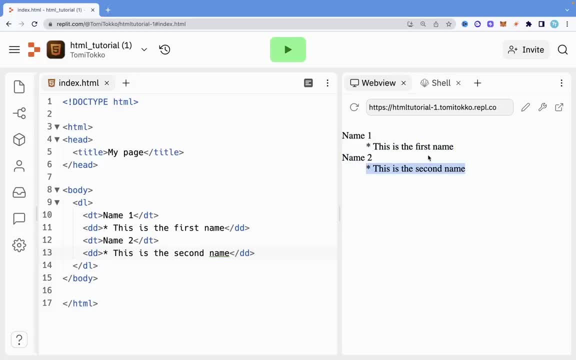 we have the description, we have name two and we have the description. now let's look into block element and inline element. so the difference between block and inline elements is basically this: so a block element always starts on a new line and the browser automatically adds some space. 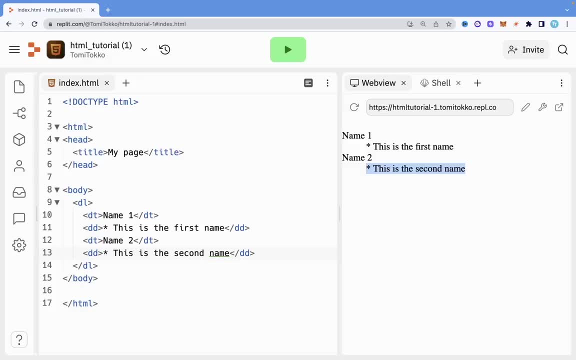 before and after the element. but for an inline element. the inline element doesn't start on a new line, and it doesn't. it just takes the space that it needs. so it doesn't, you know, have a space before it and after it. so there are examples of block elements and a div is one good example of 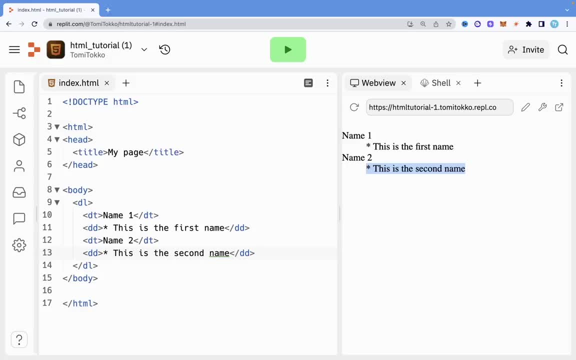 block element. now let's quickly talk more about this div tag. so div tag is written like this: the iv and it's closed. so most of the time is a wrapper or is a tag where all other html elements are contained with. so let's say, we want to group, like our whole application or our web page into different. 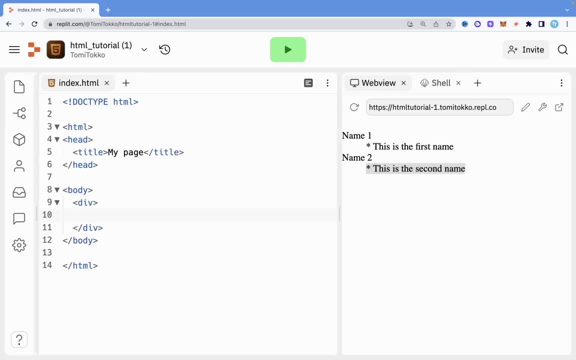 sections. we can use a div tag to do that. so, for example, we have this div tag and i can just say something like h1, first div and after this i can just say: i can just have a b tag in here. i can say: this is bold. 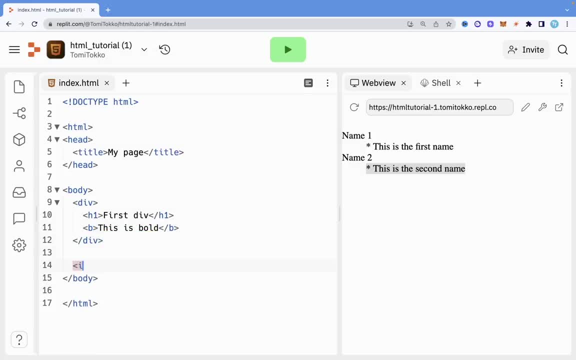 right, and i can then have another div tag just to separate that. now it's just. this is wrapping all of these elements in it, and this one we can have an h2 and say another one, and for b we can say i. so if i run this, it's basically just a normal text that prints this, but it wraps it into these. 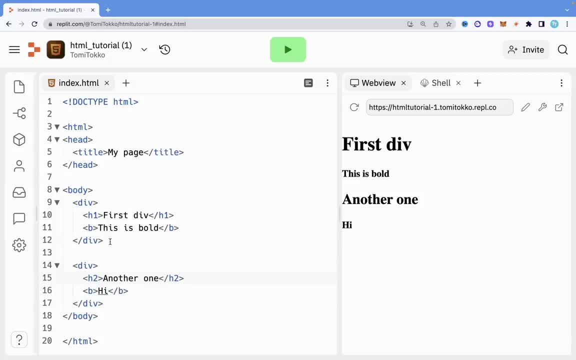 div tags. now we can use different things to. you know, know these div tags like, for example, i'm not going to use this div tag. you can see that if we have a duplicate div within here, you can divide this div tag, but even though you all have kahumas inside it and say double. 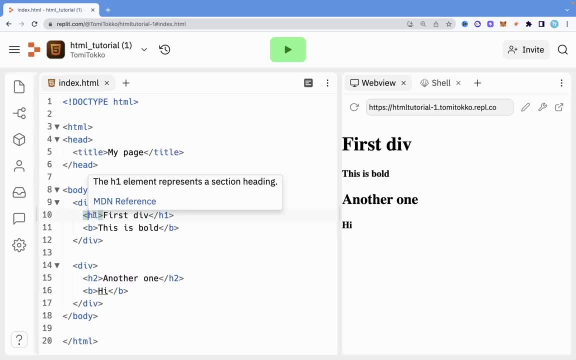 div tag position. just because it is the first div, we can make a div for a component like this, e I could release this in another youtube or youtube design suggestions or videos, but i just want to know, honestly, what's the name of this? yourself for this. okay, so this hll one longer div. 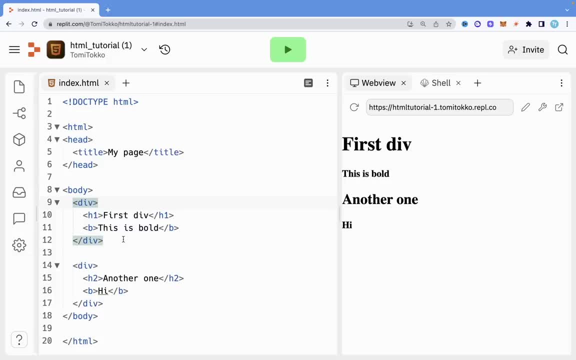 is our first div that you see, and this is the first div that becomes part of the different humanity. anything here is changed, and let me tell you what i mean. so we're going to use a style attribute- we've talked about this before- and let's say we use color and say that we want the color to be. 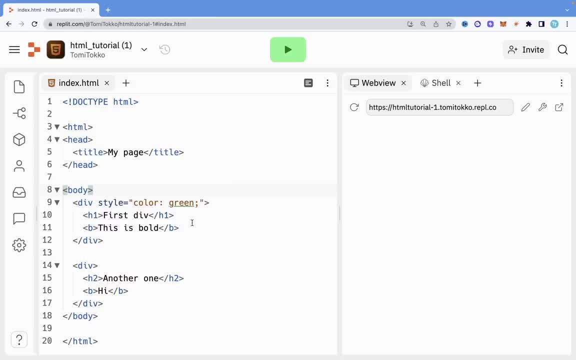 green. now, once i run this, all the elements in here are going to have the green color. right, i can also change the background, the background color, let me say blue. now, once i run this, all the elements in here- we have a background of blue and not the other one. you can see, now that we're able to, 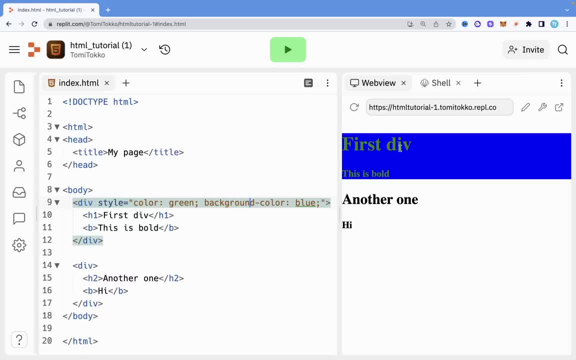 actually like separate different sections of our code and give them different attributes. so i can do something similar here and say that style and i want the color to be red. so, and i can see, i want the background color and i want this to be something like purple. 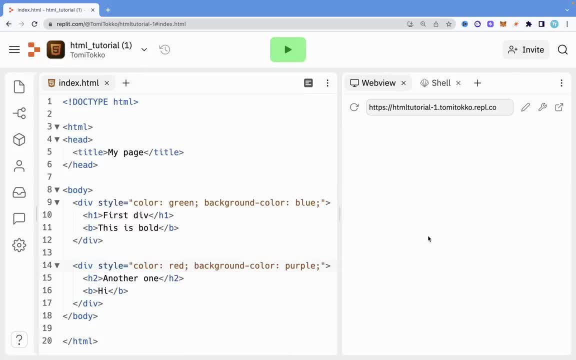 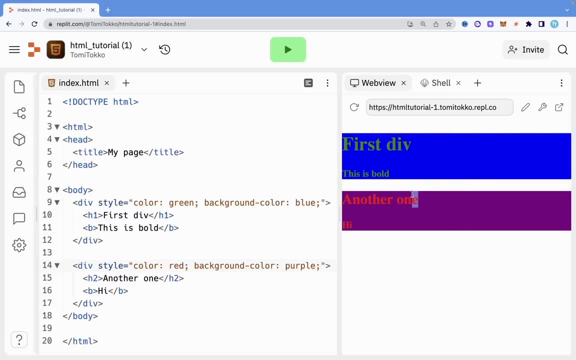 now let me run this and see what it gives me. you can see now these are two different sections. this has a different color and a different background color. this also has a color of red and a totally different background color, and that is what div class is, and you can see that there's a space. 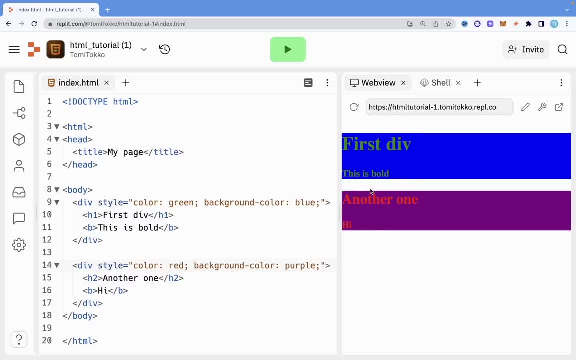 between and after that particular div class, space between and after that particular div tag. so now there is an example of an inline element. as i said, it doesn't take us as much space as a div tag and it doesn't start on a new line. so an inline element, an example of that, is something like: 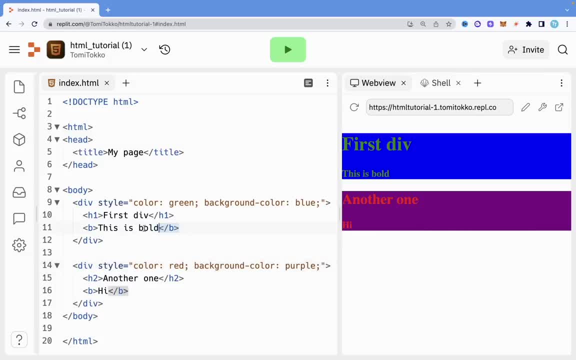 an a tag, for example, or a b tag. this b tag now is an inline element. this means that i can basically, let's say, just have a normal p right and say this is a text, and in there i can just have a b tag and say bold one. 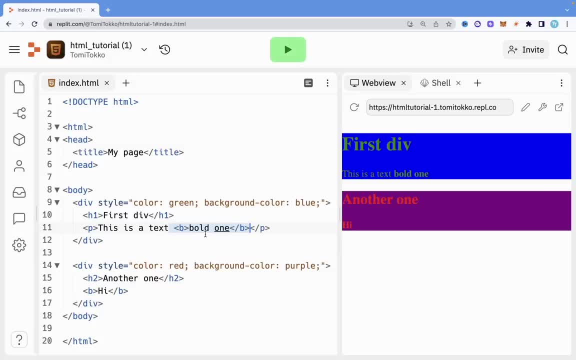 so it can stay within a text. it can stay wherever you put it. it doesn't really need to be separated on its own compared to a div tag. so that's the difference between a block element and an inline element. so there are various examples of block elements, like a few that i can see on top of my head are like: 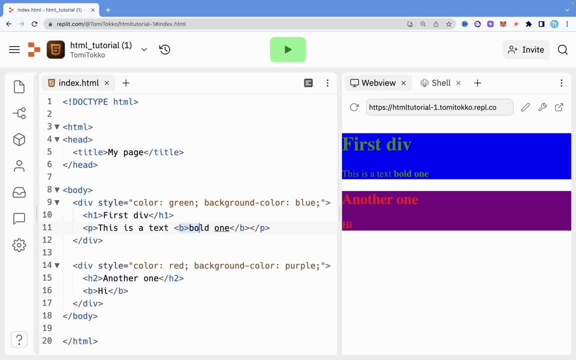 you know hr, like div, as i said, you know like pre um, ul, you know section and there are other elements like that. and for inline element, we have the a tag which we just which we used earlier. we have the bold tag, uh, we have image tag and various small. so this is basically the difference between those two. 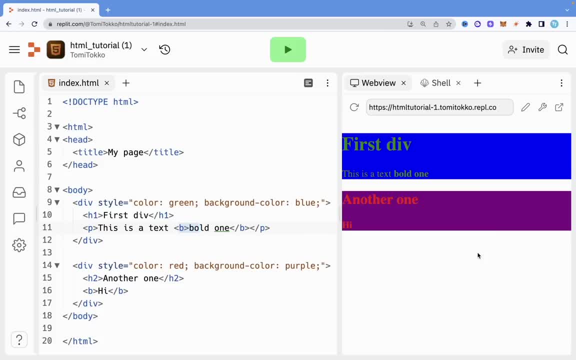 now let's look into iframe in html. so an iframe is used to show a web page inside a web page. so what i mean by this is using an iframe. we can have like a box that shows another web page in our own web page. so let me show you how to do this. it's very easy and very simple. all we just need to do is to: 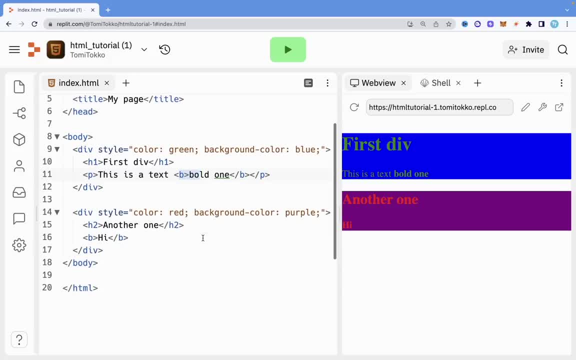 use the syntax. so we're just going to come here, we're going to get rid of all this d and i just want to say iframe, we're going to close it now. it's going to take some attributes. the first attribute is going to take is the source. so once it takes the source attribute, this source attribute. 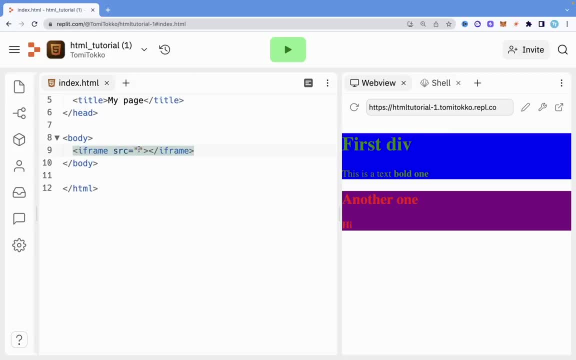 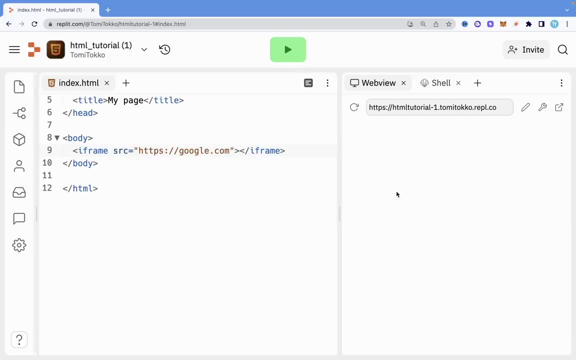 is the link that we want to show in here. so let's say, i want to show googlecom, so this is going to show googlecom in here for me, so that it is that easy to do. and once i run this, you're going to see what it shows. you can see that it creates a box. it says: 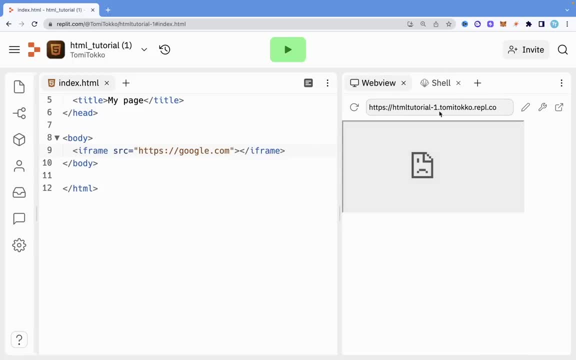 refuse to connect. that is probably because of this replay um page, but normally once you use this iframe, as you can see, it's trying to connect to googlecom. so there are more you can do to this iframe, more things like you can, you know, specify the height, the width of what, how big you want this? 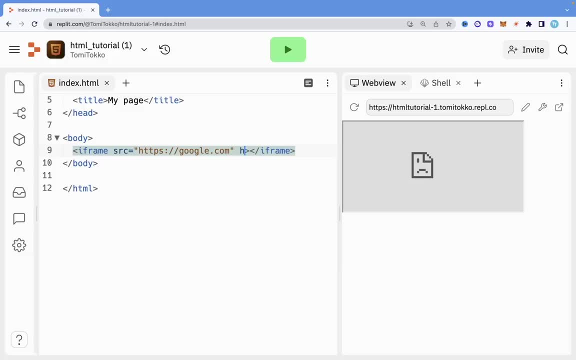 to be. so i'm going to give you more attributes and say height, and let's say 100. if i run that, you're going to see that it goes smaller. and let's say i also give it a width of 100, and if i run that, you're going to see that the width also goes smaller. so i can. 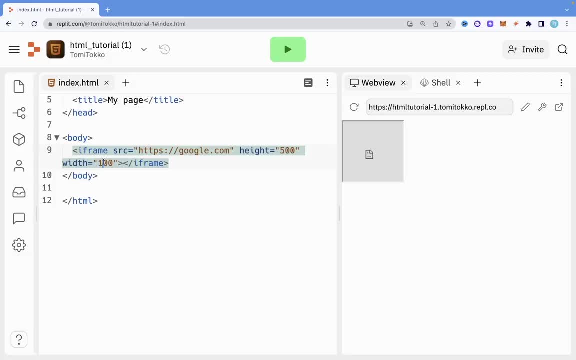 increase it however i like. i can say this is 500 and i can say this is 500.. so if i run that and i'm going to see that we have a big iframe right here. so that's how to create a very basic iframe for us. now you can also remove the border. you know this line where you see we can do that. 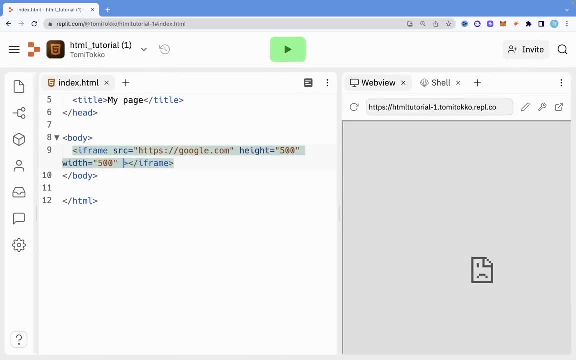 so to do that, we are going to use the style attribute. we've talked about this style attribute before. be easy to you know, add some styling to that particular element. so now, what we're just going to do here is to say: border. now this brother, is basically the line that we see. 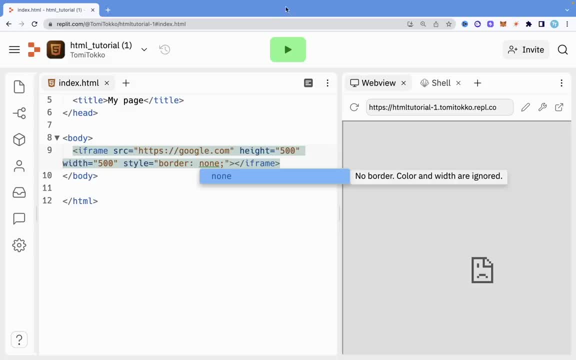 right. here i'm going to say: border equals non. if i run this, you are now going to see that there is no lines there. The lines that were shown before are gone Now. let me just make this quite smaller so you can see that very well. Now, if I run this, you're gonna see. 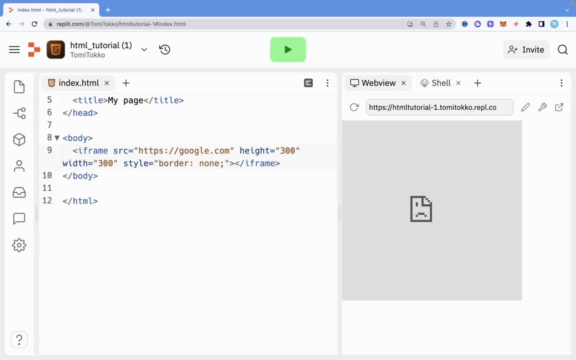 that it's just a square. there's no lines on that. So that's a very basic way of how to create iframes in HTML. Now let's look into symbols in HTML. So let's say we want to display different symbols, like, let's say, the pounds sign or the hero sign, or we even want to. 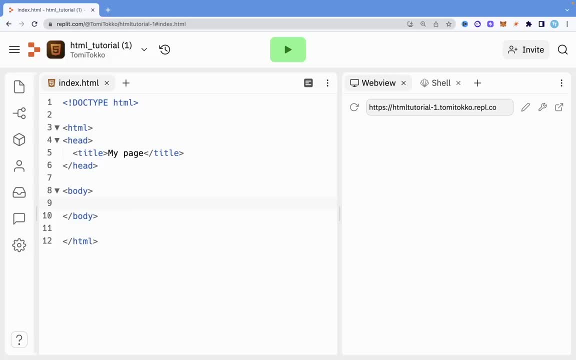 display more symbols like the copyright sign, you know, card sign. I'm gonna explain what I mean in a bit. So if you want to display all this stuff, there is a particular, you know, syntax that you have to follow in HTML. So, for example, let's: 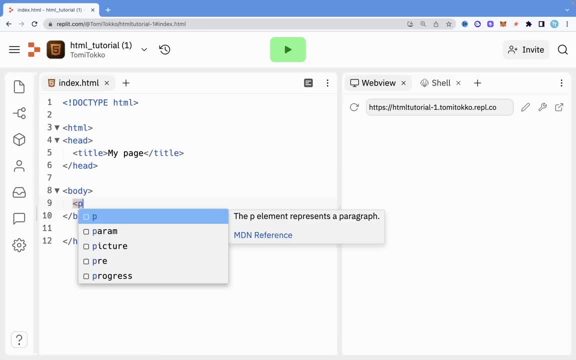 say, in this body I have a p-type. I'm just gonna say: this is hero sign. So I now want to display this sign of the hero's currency. For me to do this, I'm gonna say: and So I'm gonna use this and right here on my 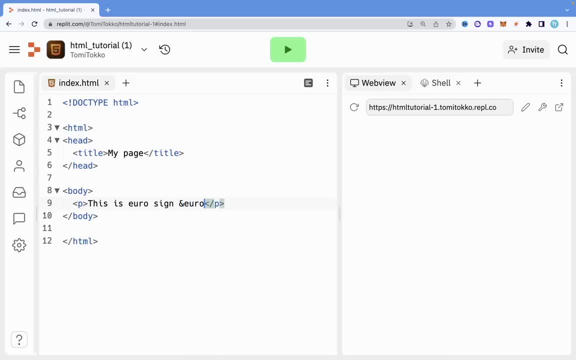 keyboard and I'm gonna say hero. Now, if I run this, you're gonna see that it displays the hero sign. for me That didn't display the hero sign and that's because we didn't have the semicolon, So we must make sure we have. 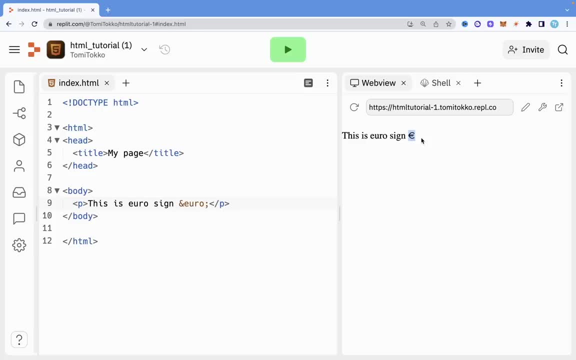 a semicolon. Now you're gonna see that it displays the hero sign. Now there's more and more that we can do, and I'm gonna go through most of them. So, for example, let's say we want to have you know something like the copyright sign. 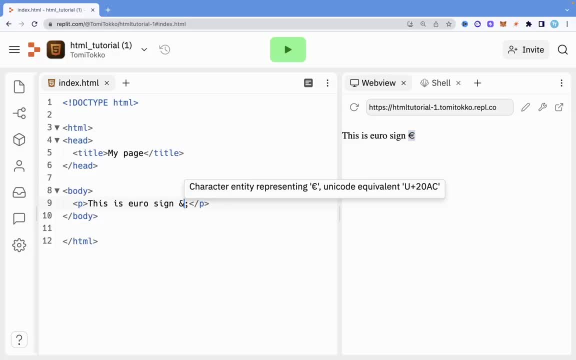 So the copyright sign. what we need to do is to do and, and we're gonna do hashtag and we're gonna do 169.. Note that it must end with this semicolon, If not, it's not gonna work. So once I run this, you're gonna see that we have the copyright sign. Now there's a. 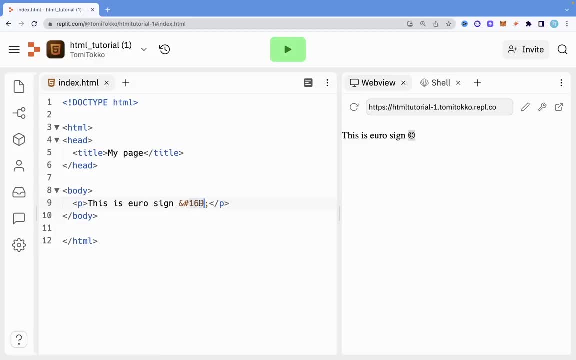 lot like we can have. the registered sign is similar to this, but it is 174.. And once I run this you're gonna see that we have this R sign. So we can also have, like the, you know, the signs on a card, like the spade, the R to the diamond and all of that. So for 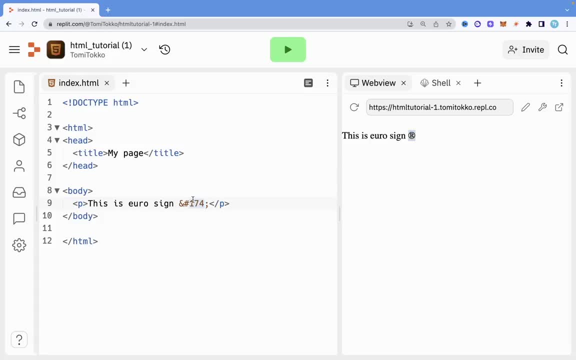 us to do this right here. let's say, I want to have the spade sign. I'm just going to have 98. To four, and this is going to show the spade sign on a card. as you can see, And if I want, 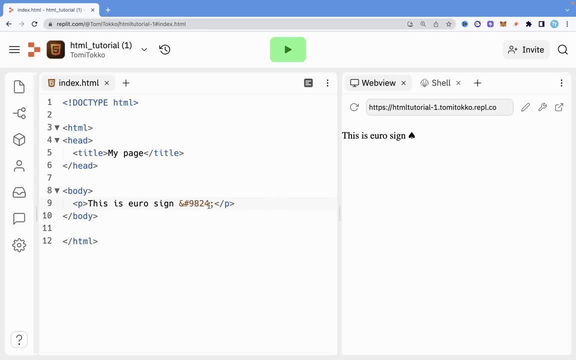 to have the clubs, I'm going to do 9827.. Right, that's going to show the clubs. And let's say I want to have the art, going to do 9829.. That's going to show the art. And if I want, 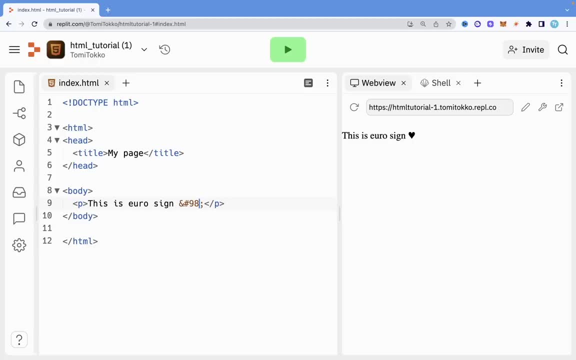 to have the diamond. I'm going to do 9830.. Once I run that, we're going to see that. that shows that for us Now there is a lot like let's do one more, for example, like a trademark, we're going. 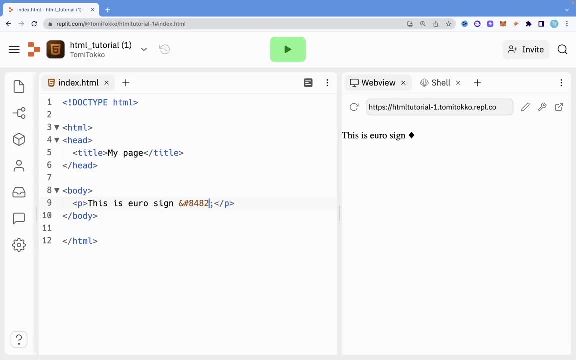 to just change it to 8482.. Once we change this, you're going to see that we have the trademark sign TM. So this is just a basic way, basic syntax of you know showing symbols in HTML. Now there's a lot of you know all of these and you don't have to know this off. 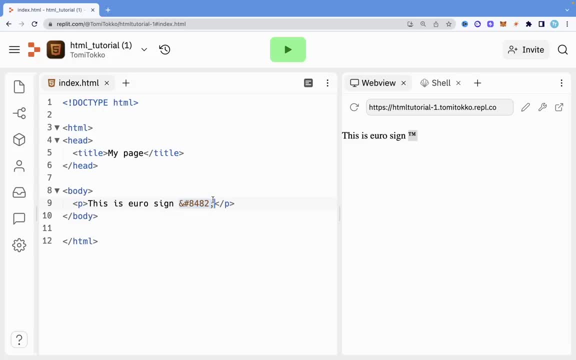 by heart. you can just search on Google. HTML symbol for displaying the- you know the pound sterling sign. Oh, this, This is displaying the pie sign. anything you want to do, you can just search on Google. I don't advise actually knowing all of these off by heart. So that is what. that is how. 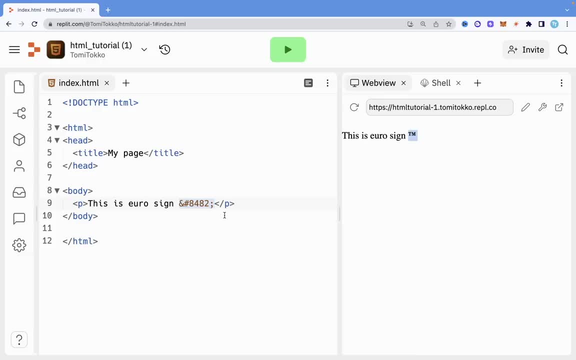 to you know, create symbols or show symbols in HTML. Now let's talk about forms in HTML. So a forms is a way you can collect input from a user. So when you collect input from a user, these forms are mostly sent to like a server for. 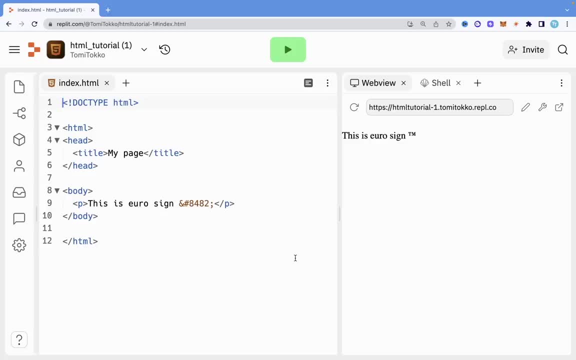 you know HTML processing or whatever the data is needed for, For example. let's say you go to a website and you want to log into the website. you're going to see that there is a simple form where you fill in your username and your password, then you click on Submit And that data is. 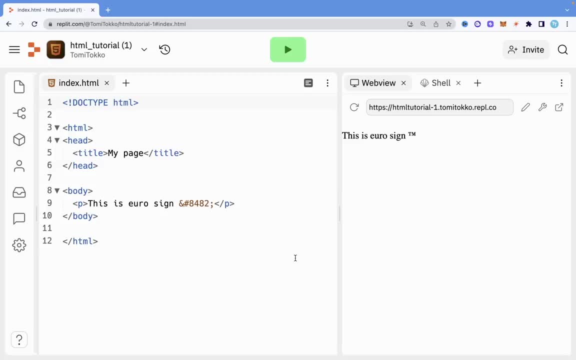 being sent to a server that checks whether your username and password are actually in the database of users. So the basic reason why we have form in HTML is to collect data from user. So let me show you how we can implement a form in HTML. So the first thing you need 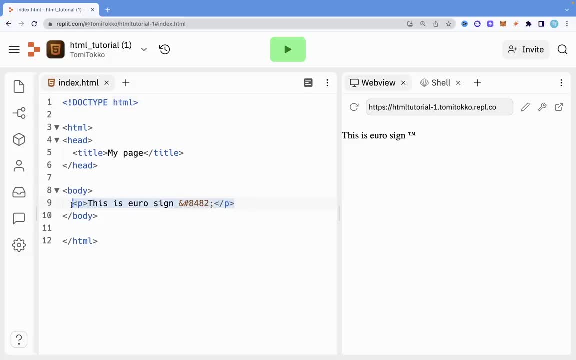 to know is the form tag. So I'm going to remove this and I'm actually going to just start by saying form And when I close it, it's going to close by itself. So now this form tag is. HTML now knows that we're trying to create a new form, So it's going to have like 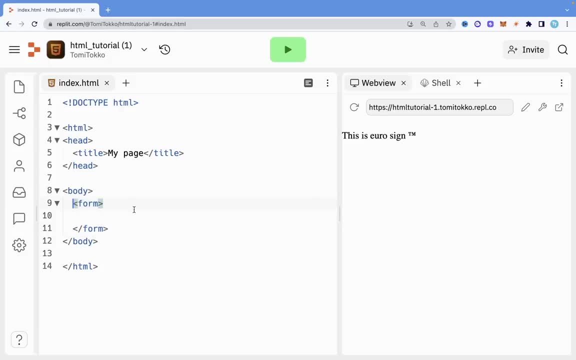 an input, like an input bar, where a user can input you know something? But now there are more to just this form than only the, the, just the element. So we need to have the input element also. So the input element is used to display what type of form or what type. 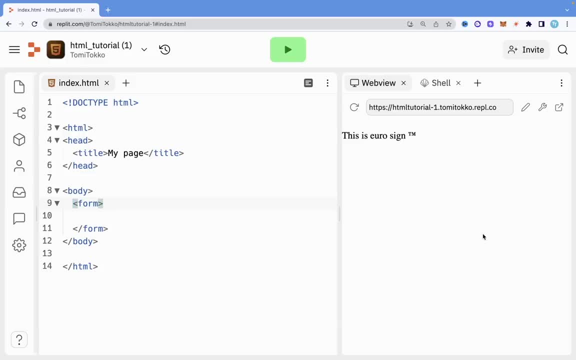 of data we want to collect. So, for example, let's say I have inputs, this is how we type input And then we close it like this: right, And what we can just do is to is going to collect various attributes, But the most important one is this: So I'm going to set it to input. 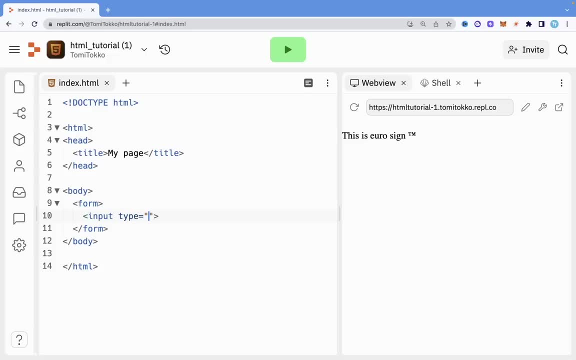 And then we close it like this, Right, And what we can just do is to is going to collect various attributes, but the most important one is the type. As I said, it shows, or it specifies, what type of data we are trying to collect. 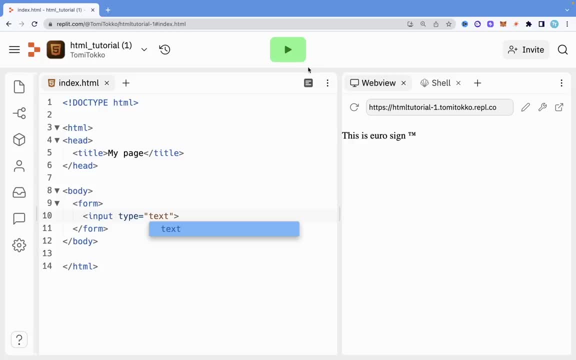 So let's say I just want to collect a text, I'm going to input text in here And I can run that. So once I run this, you're going to see that we just have this simple bar right here where I can input a text. right, I can also have an input that, just you know, collects. 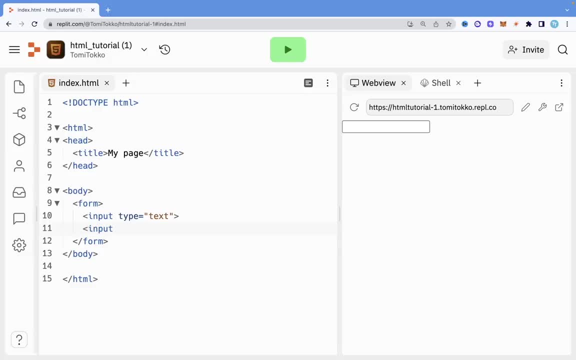 numbers. So let's say input type, we can say number. if I close that and I saved it, I run this. You can see now that we have these two buttons here which can help us increment and decrement the number. So this only collects numbers. So we this basically tells us like: 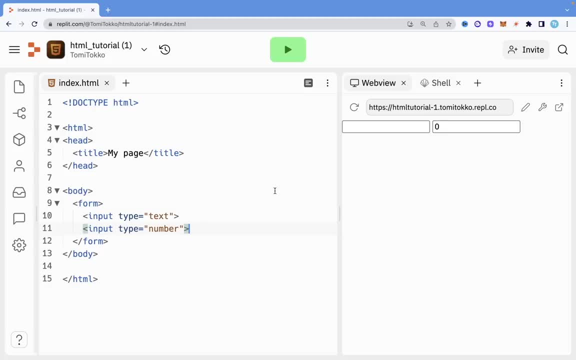 what we actually want to, you know, input, what type of data we want to input in here. So let's say we want to input a text. So let's say we want to input a text. So let's say So. let's say we want to input a text. So let's say we want to input a text. So let's say 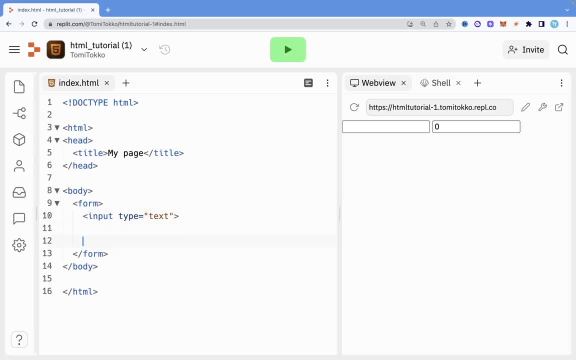 first of all, look into this text field very well Before we go into the other fields. I mean this text type. So, for example, whenever we have an input right, we must always have a label beside it, So right here where we have this bar. if we don't have something saying: input your name or 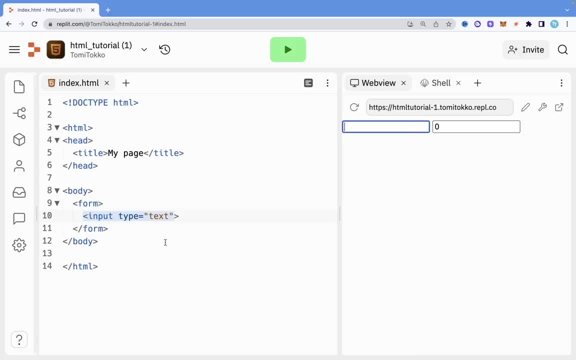 name or username. the user is not going to know what to input. That's where the label comes in. So we have a label And we close that label And here we can just say name. So here, where we have name, we can now say input type text. So I can run this And you see it just. 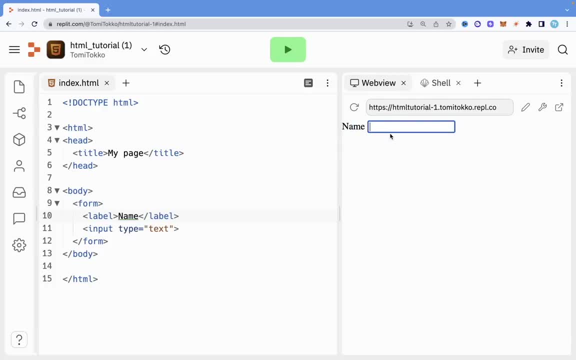 says name and it has the bar beside it. So let's say I want to leave a space and I want this to be on the bottom. I can just add a BR tag And I can run this. So you're going to see that it's now on. 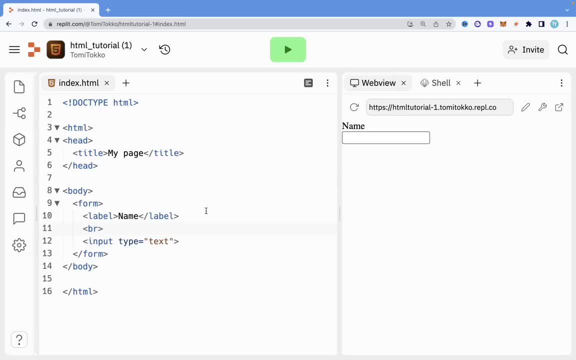 the bottom. But now the name need, the input needs more stuff than just you know the type, like we need to know the ID and the name of that particular input. So whenever a data is being sent from this HTML on, from this HTML form, right it's been sent using the name of that particular. 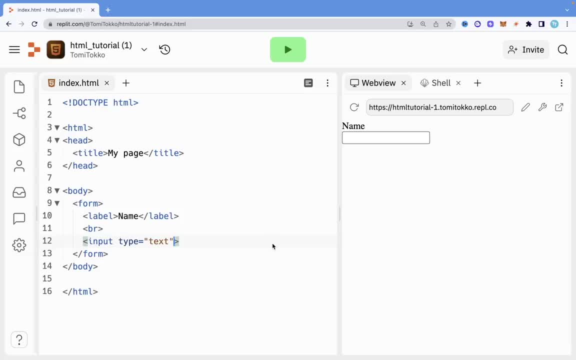 input. If there's no name, there is no way a data can actually be collected by the server. So we need to specify the name right of this input. I can just say the name of this input is username right And we also need to specify like an ID. 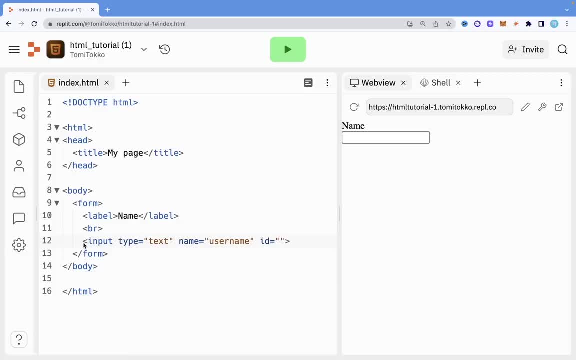 Now we use this ID just to be able to recognize or to be able to refer to this particular input within our HTML page. I can also say: the ID is something like username. I can give it the same name. Now for this label. I want this label to actually be linked to this particular input. 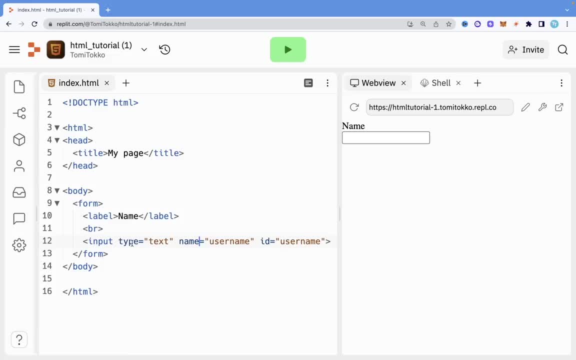 because, for all I know right now, they are just two different elements. But what I want to do is that I want HTML, this our you know code, to know that this label is for this particular user input. So for me to do that is fairly easy. I'm just going to need to. 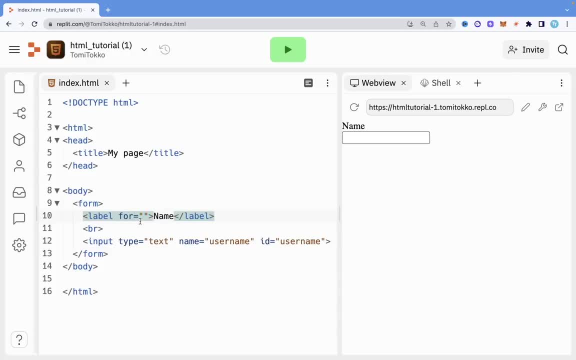 have an attribute here that says for- and we're going to say for- username. You see, we said that by using the attribute that we already, you know, defined here. So if we run this, that is not going to make much of a difference. But now we know that this label is for this input. Now let's do the same. 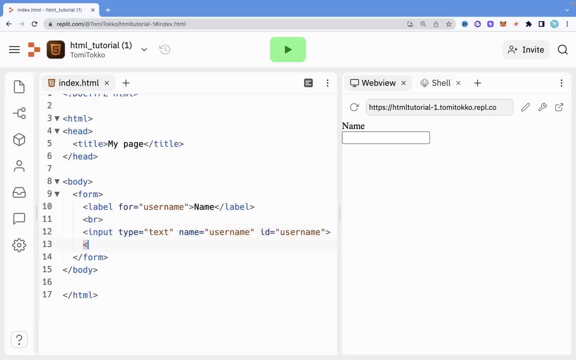 thing for let's have another form. We just have a Br. let me have a label going to close the label. Let me say you know H, and let me just say school Right, And I'm going to have a four, But for now I'm just going to leave it. 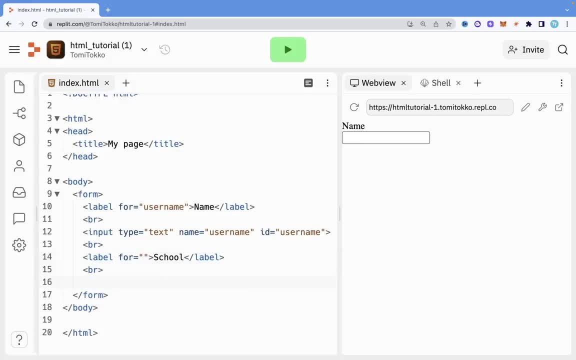 blank. Let's quickly create an input for that. Let's say input, and then we're going to have a type, and the type of that input is also going to be text and let's give it a name of school and also an id of school. 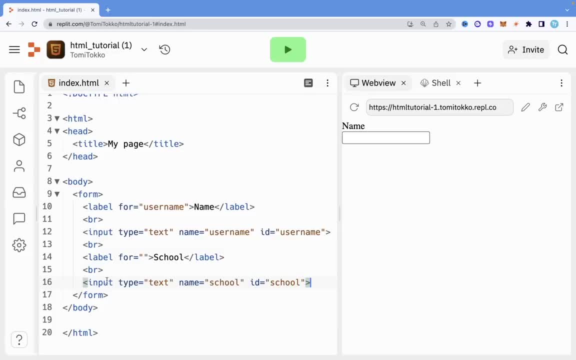 now i'm gonna say this is for school. now, once i run this, i'm gonna see that i have another particular field right there. so that is the basic way of doing that. now let's look into another type of input. like we've talked about text, but what if we want to talk about, like another type, like 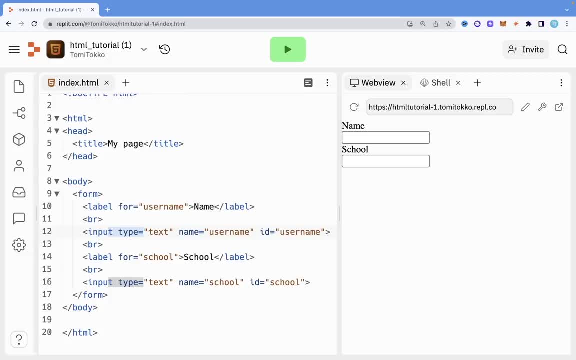 let's say check boxes, right? so let me come in here and i'm just gonna remove this particular input, so this input where it says type text. i'm gonna change that text to check box and i'm gonna give it an id of username, same username and let me just say the value. 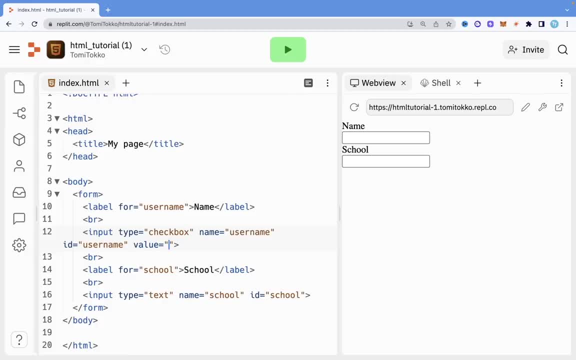 is something like: um, let's just say tommy, so i want the user to check if you know, this is its value and i can just give it another one and say, right here, i can just remove all of this, right, and i can just have this and copy it. so it's basically the same thing but with a different. 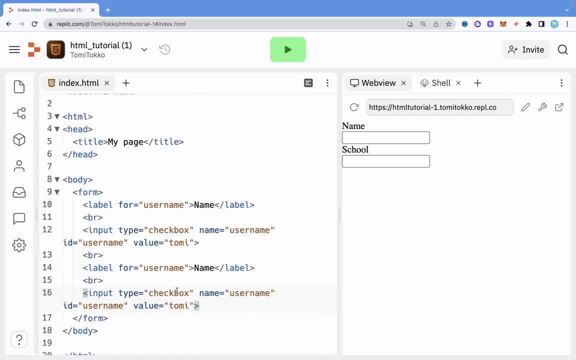 type. so now i'm gonna say name. this is another username. we can say username two, username two and let's say team. right now, if i run this, you're gonna see what it gives us. so you can see that it gives us name and it also gives us name. so what i want to do actually is right here. i don't know. i've told me. 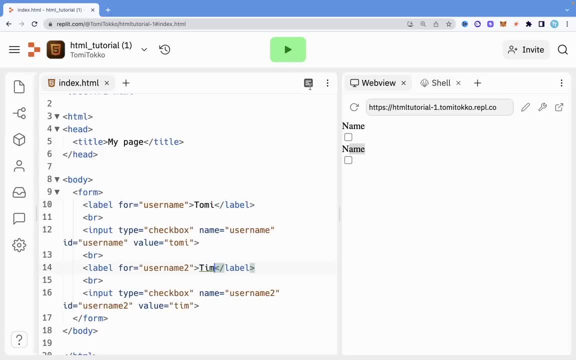 and i want to have team. so once i run this, i want the user to click which one is your username. is your username told me? then tick it. is it team or is it both of it? you know? then tick any of it right so that that is fixed right there, and what you just need to know is that whenever the value 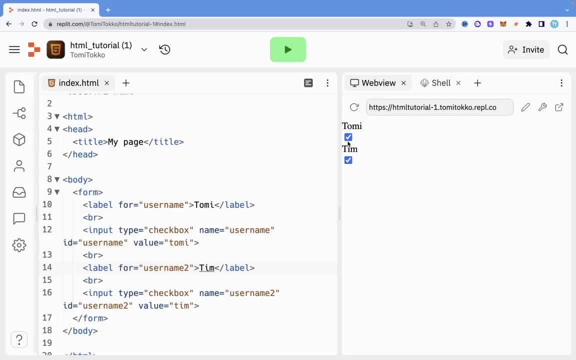 is being sent. for example, if a user ticks tommy or it takes both of it, the value that is being sent is not this value that shows here. it's actually the, you know, the value that is specified as an attribute in here, right? so whenever a user clicks on submit, we're also going to talk about. 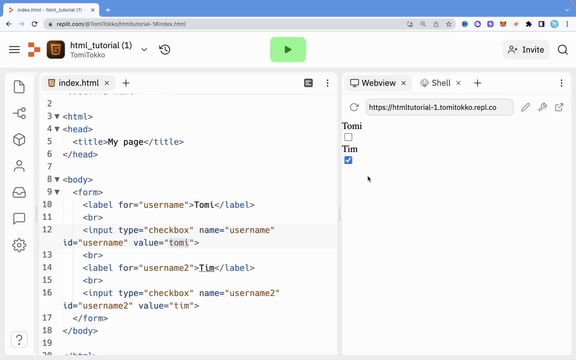 the submit button soon. when a user clicks on submit, that all the data is going to be taken from here and sent to whatever server we want it to be sent to. but the value that is actually going to be sent is this value that we specified here. now we can do exactly the same thing for like. 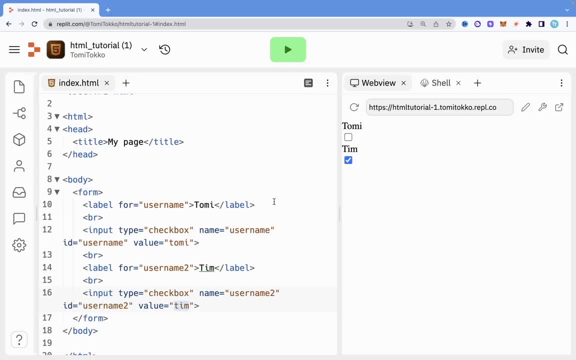 radio buttons. so very similar to what we just did. but what we're just going to do is, instead of checkbox, we're going to say radio. instead of checkbox, we say radio. if i run this now, you're going to see that it prints tommy, but this time around it is like a radio. 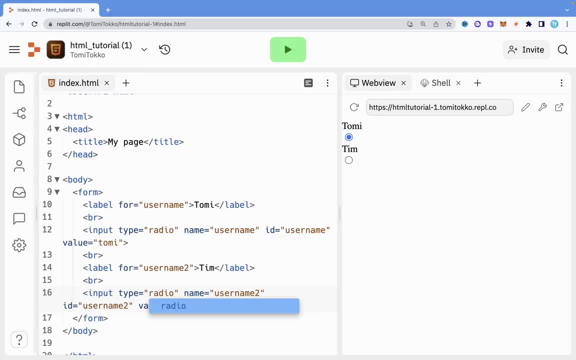 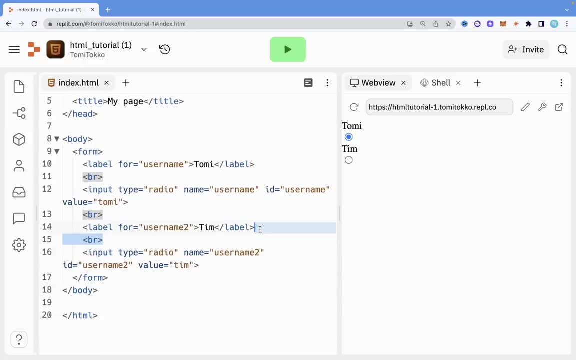 button. so that is fairly easy to understand, right? so the next thing i want to talk about is actually submitting this data. let me remove this right here and let me remove this br. let's just make it look good so it doesn't look confusing. now, once we run this, this should just. 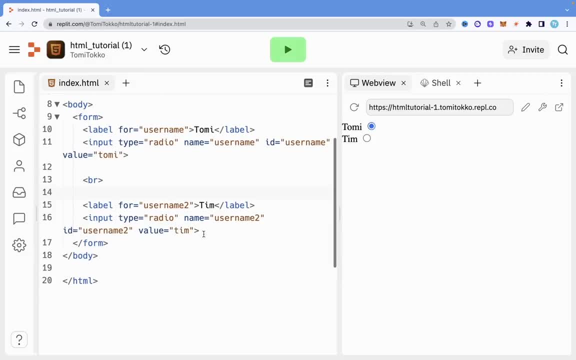 have it beside it so we can pick with the one we want. now that we have that, i want that whenever a user now clicks on submit, you want, actually want to submit a button. this is the easiest what we just need to do. let's first have our br tag right here so it doesn't collide. we can just we're. 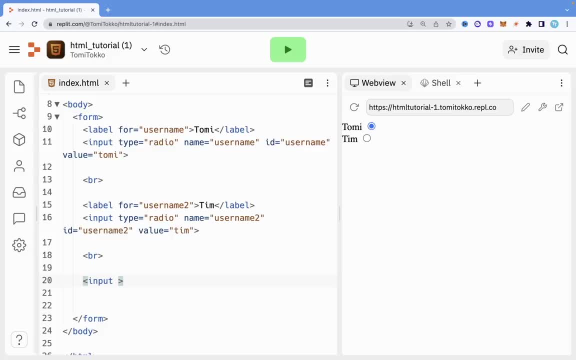 just going to have another input, but this time around what we just need to do is to say type submit. once we say type submit, HTML knows that we want to have the submit button. that means the button that, whenever a user clicks on this, is sending all those data or those inputs. 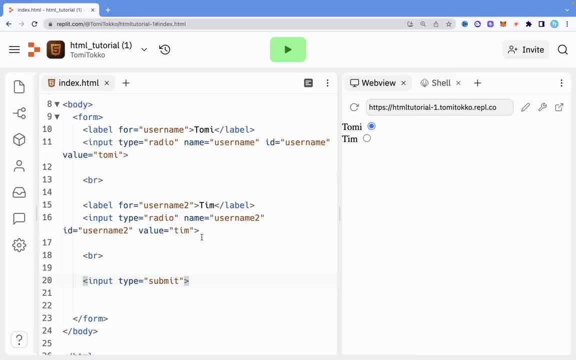 somewhere. but now we also need to have a value. let me run this first and see what it shows. you can see that it automatically writes submit step. but what if I don't want this to be submit? let's say I want it to be, you know, send. then I can do. 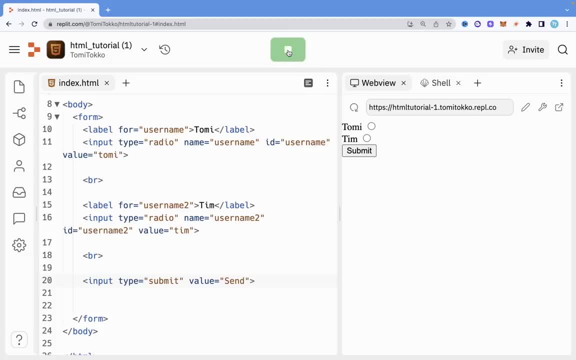 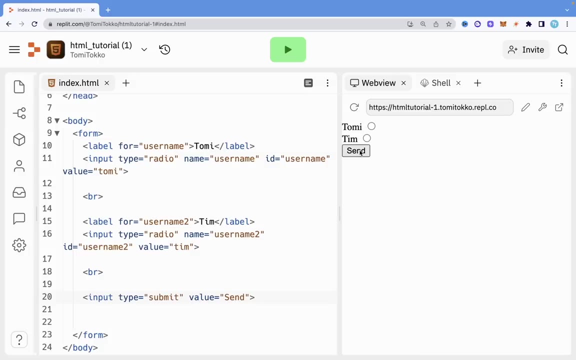 value and I can say send. if I run this, you can now see that that submit button has been changed to send. now that is how easy it is for you to do that. but now where is this data actually being sent to, like when we use? remember i said for this radio and checkbox, it's not actually this tome that is being sent. 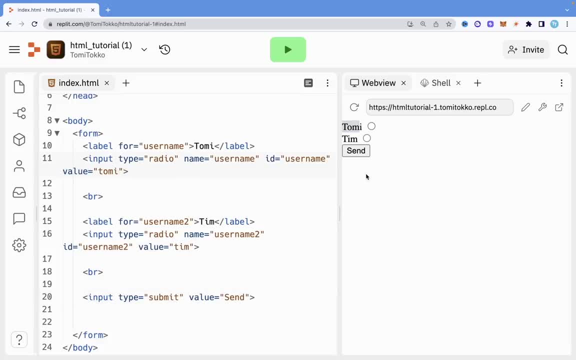 is the value that we specify there. that has been sent. but when we click on send, where is it being sent to? now, this is when we need to add an attribute to the initial form. now this attribute is called action. this action will tell us where the data is meant to be sent to. we are going to 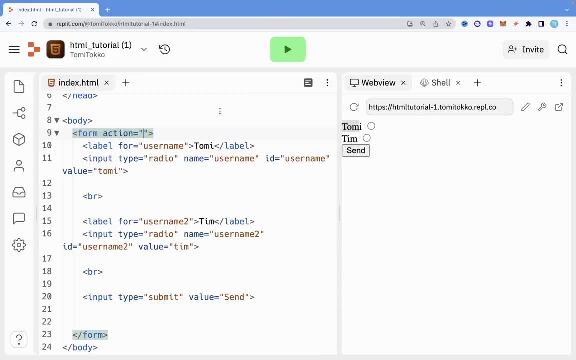 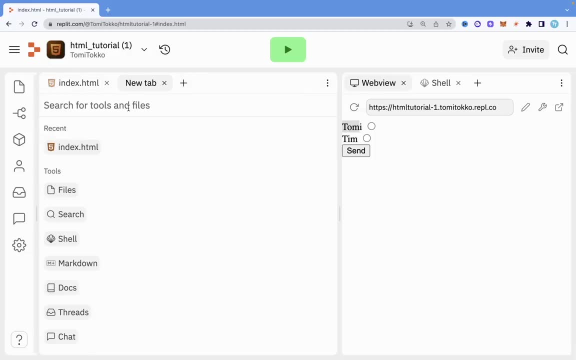 say: action equals. now let's say we want to send this data to another page. imagine we add another page like let's say something like um, um, formhtml. right, we can create that and we want this to be sent to that formhtml. once we hit send, that is going to be sent to formhtml, basically. so you. 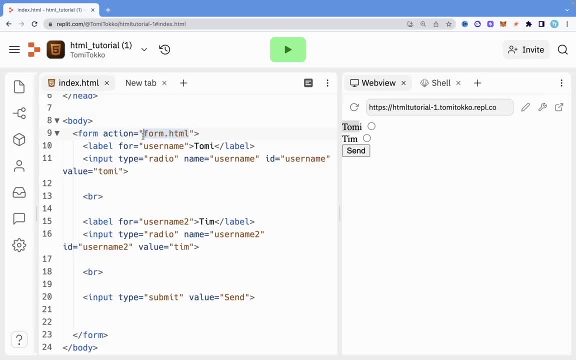 can also like send it anywhere you want to send it to. let's say, you have a web application you are building and we can say we want to send it to. like slash receive. you know you can do anything you want to, but this action basically is specifies the place or the url or whichever link is getting that particular form or where you want. 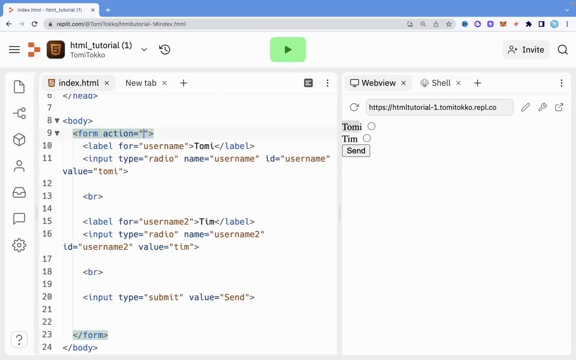 to send that particular form to. so that is fairly easy, and that's how to easily do that, the first thing we need to know. let's go through what we just did. so the first thing that we did was to create our form element, and then we created different labels and inputs. i showed you the 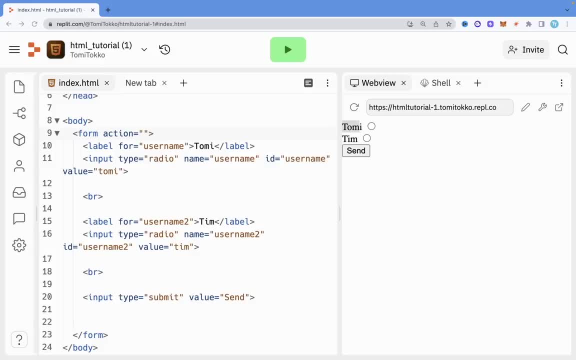 types and i showed you how to use the submit button. and once you have the submit button, i also showed you how to add the action so that you actually know where it's going to. but now that we know where it's going to, right, where we put in this action, let's say from that html, we also want: 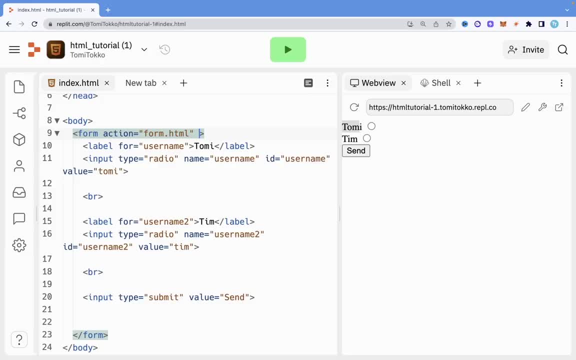 to know what method is being used to send this data. now you don't need to know the details of what i'm about to say, but there are basically two methods that we can use to submit a data, and it's called get and post. so when submitting a data, you can choose to either submit it using 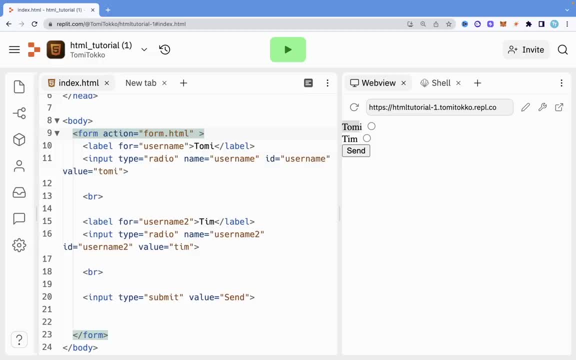 get and post. you can learn more about that, you know, on youtube anyway if you want to know. but for example, you can just specify method equals post. so let me just show you the the quick difference between get and post. when you are sending the data using a get method. 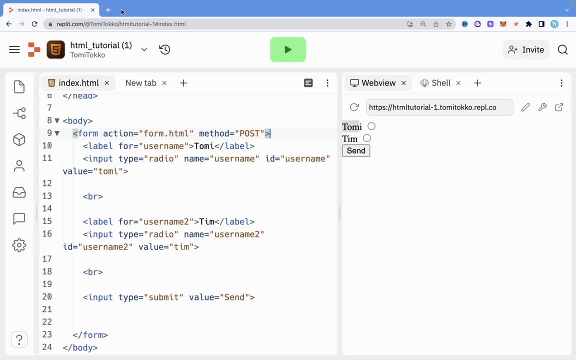 all the details of the data that you are sending is going to be shown in the url bar. for example, if i search something on google and i hit enter, everything i searched- the keyword i said- is going to be shown in the url bar. right, that's when you use a get method. we've used a. 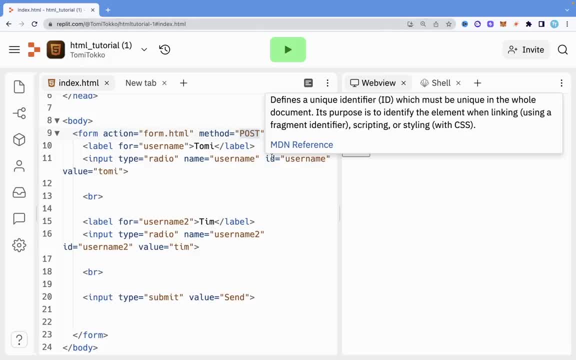 post method. it's not going to be shown. there are also just a lot of differences between the two, but that's just one difference that you know i can use to easily explain it. so you're going to pick whatever method you want to use to send this data. you can use post or we can use get. if you don't use. 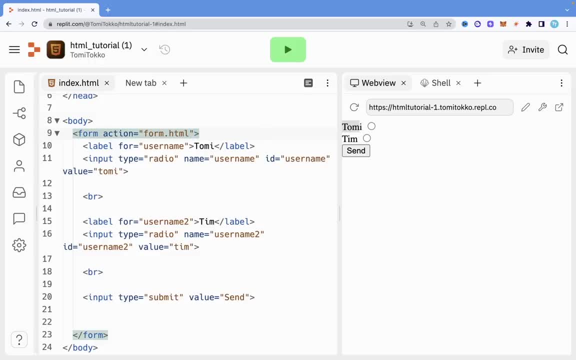 any method. imagine you don't specify any attribute right here as default, html is going to use a get method to submit that data, but for us let's just specify it so we can say get. so it's that easy. you just need to. you know some. you need to specify the method, the action, so that everything works perfectly. 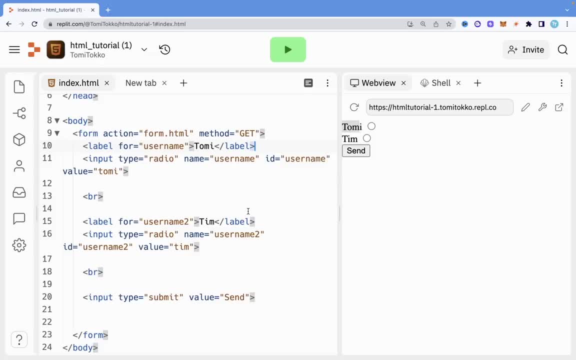 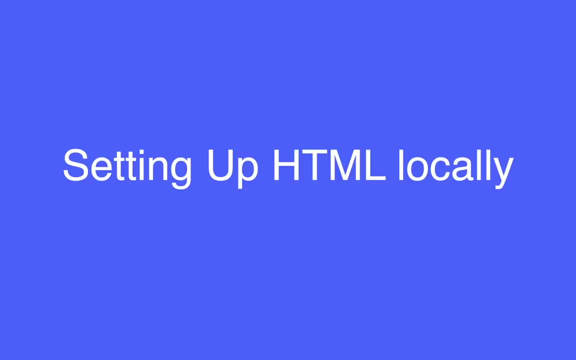 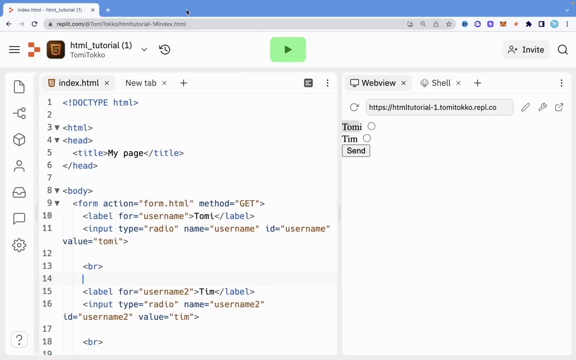 so i hope you understand everything we did about this html forms. it's fairly easy and you know. i hope you were able to follow along. so earlier in this tutorial i said that i was going to show you how to actually create an html file and run it in your browser, so i'm going to show you how to do it locally on your computer. 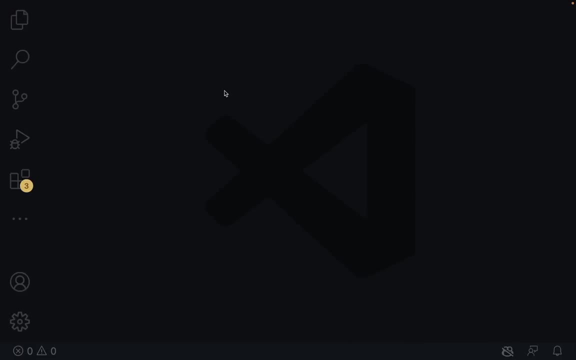 so what you need to do is to open a code editor. right here i am in fujia studio code, but you can use any one you want. you can use sublime text, you can even use a notepad. anything that can make you write code and you are comfortable with you can use it. so once you have your code editor opened, i'm just 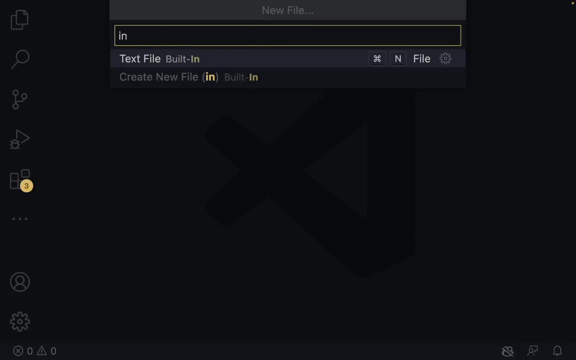 going to create a new file right here and let me name this file indexhtml. now, whenever you're creating an html file, it must have thishtml extension at the end. you can name this whatever you want to name it. let's say: test you know, whatever you want to name it. let's say: test you. 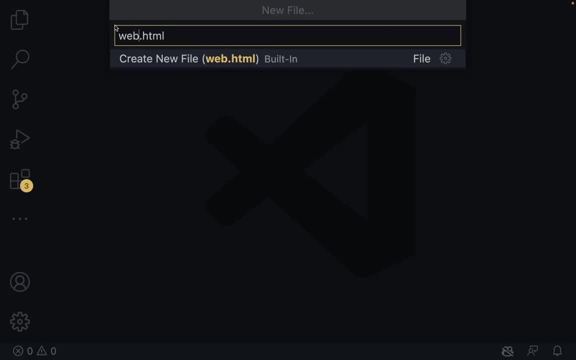 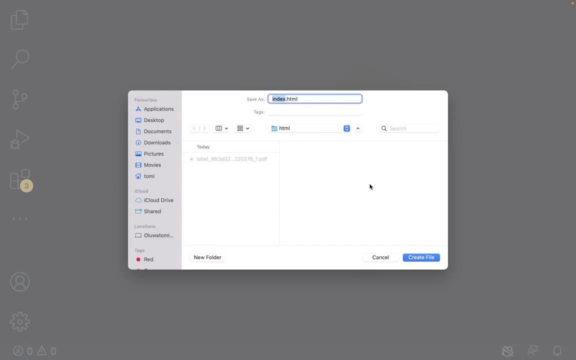 know, let's say websitehtml. you can name it whatever you want, but it must have thishtml at the end. i'm going to create that file and i'm just going to create it in this particular folder. now that i have this file created in here, i cannot code anything i want to code. 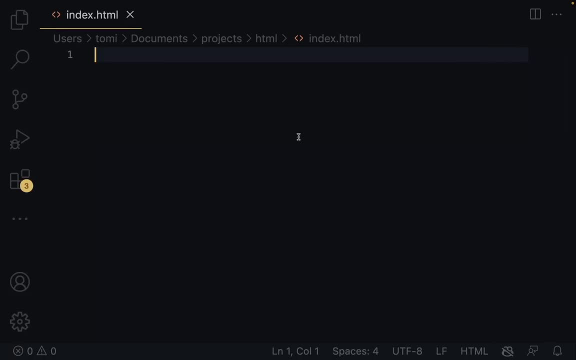 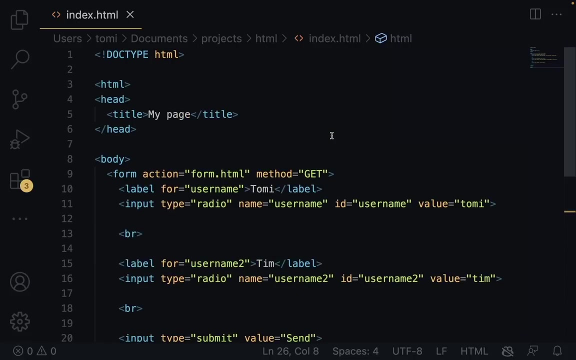 so let's say, i'm just going to come here and copy all of this code that we did here and i'm going to paste it right. so once i have this code in here, i've created all my html. everything i want to do now, what i can do is to now run this on my browser. for me to do this, i'm 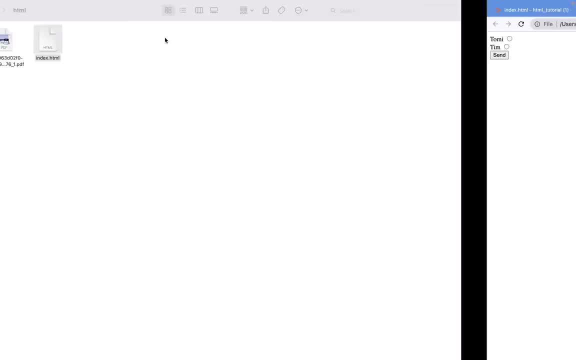 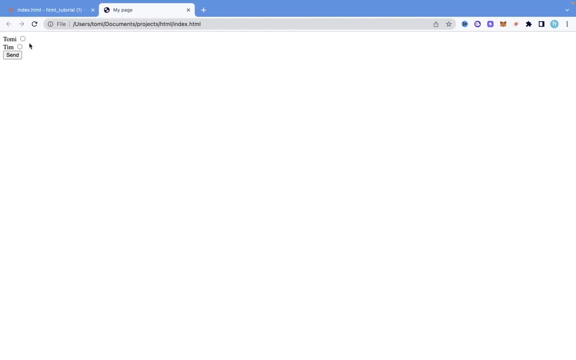 going to come into the folder where i created that and i'm just going to open indexhtml. so automatically, when you open that indexhtml file, it's going to open it on your browser and show you the result of what you are coding. so earlier i talked about the- uh, the title, so we tried to. 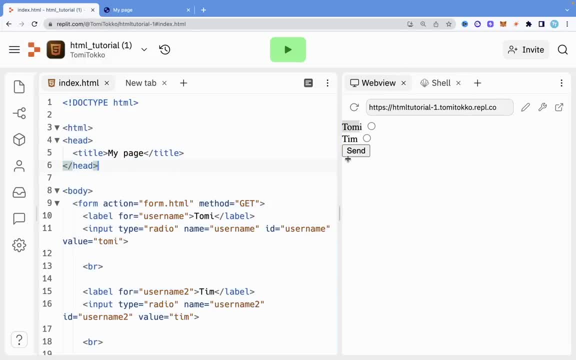 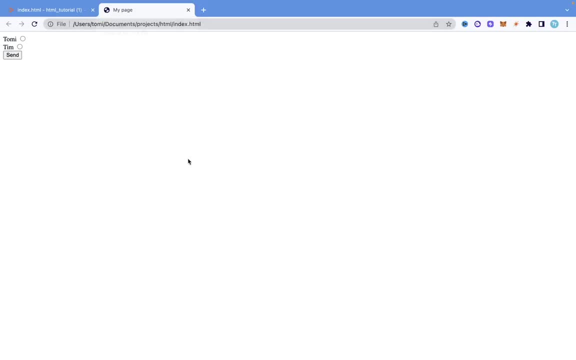 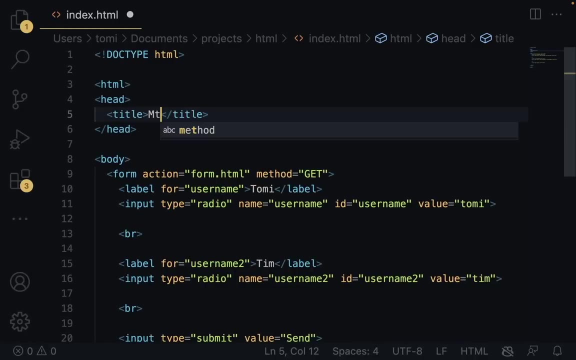 create a title here. but it wasn't showing just because we are using like this browser right here and not an you know an actual page. but now that we have the page, you can see that this, my page title, is showing. now, if i go back to this, you know code and let's say i change this to test title. 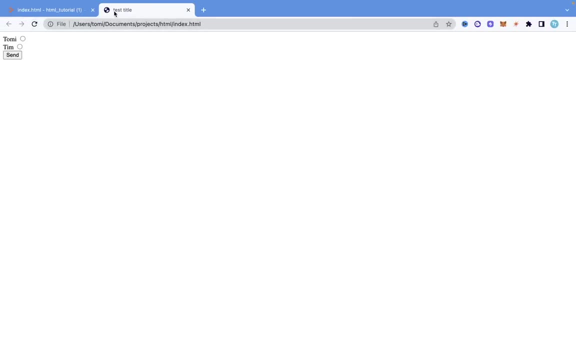 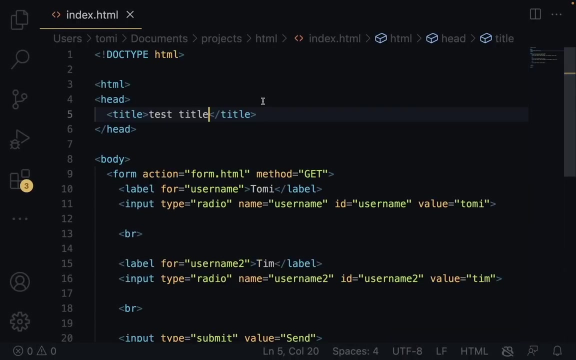 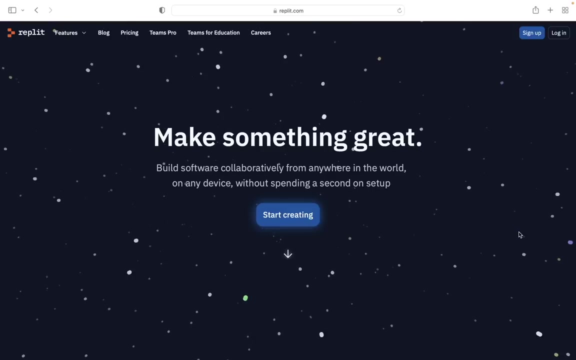 and whatever i change in here, once i refresh you can see that that title is now test title. so that is an easy way of actually coding, you know, html files, or doing it locally, then showing the result on your browser. in this section of this course we're going to be looking into css. 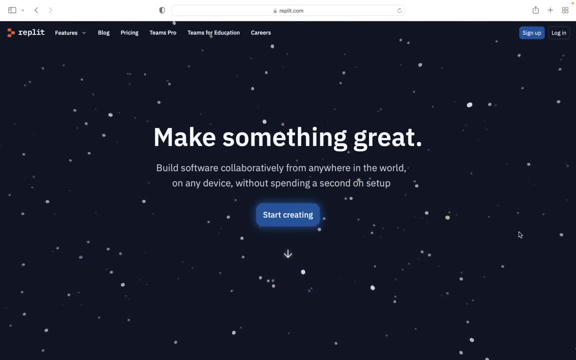 so css stands for cascading style sheet. now, what it does is that it allows you to add styling to your html page. now i'm going to take you from a beginner's level to a level where you can confidently use css to style your html code and without wasting any time, let's actually get. 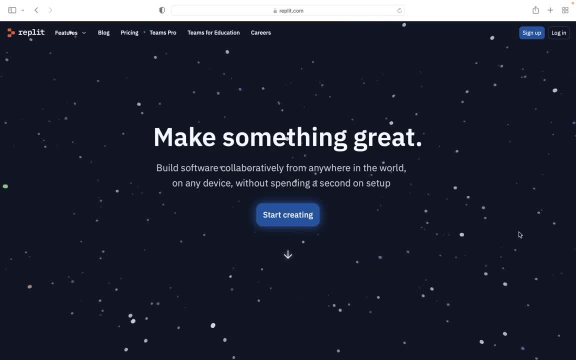 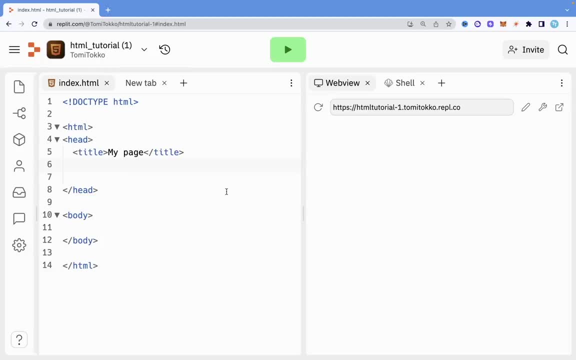 straight into this section. so here you go, we have our alive. so happens here. so now we know that css is what we use to basically style everything we do in our html. so but how do we actually- even you know- create a css file? how do we let that css file be linked to? 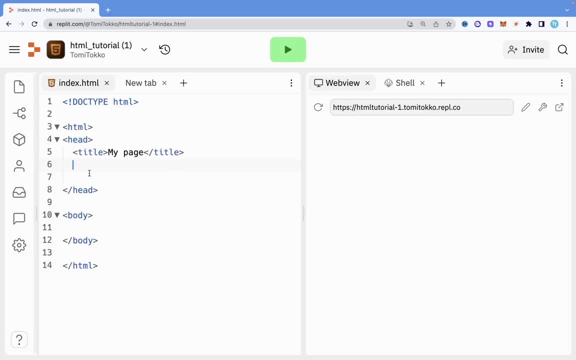 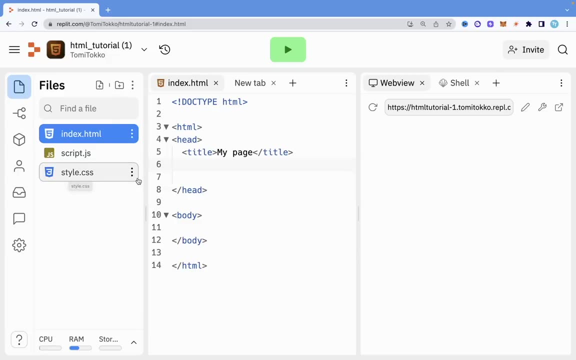 this particular html file. i'm going to show you how to do that. so, first of all, to create a css file, you need to create a file named stylecss. so first of all, right, we're using repli, so repli automatically created this file, these three files, for us. but right now we're going to be looking more. 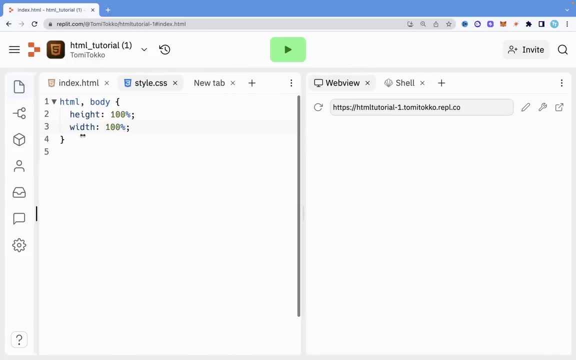 into this stylecss. i'm just going to drag it over here. so stylecss is basically a css file that we're going to be using on this html file right here, so you can name it whatever you want. you can name it. you know maincss, but whenever you're creating a css file, it must have thiscss. 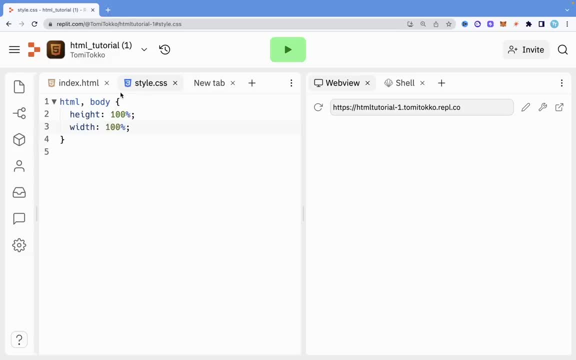 extension to it. so now that we know that we have that, how do we actually connect this css file to our html file? so we're going to create a css file and we're going to create a css file to this particular html file right here now. this is very easy. we're going to use a html element. 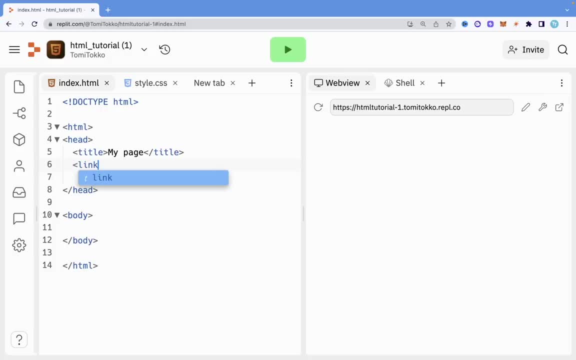 called link. so right here we need to say link and we're going to close it like this. that is how we close this time, and it's going to take two different attributes. the first one is going to be real and that is going to say that this is a style sheet that we're linking to. we're going to 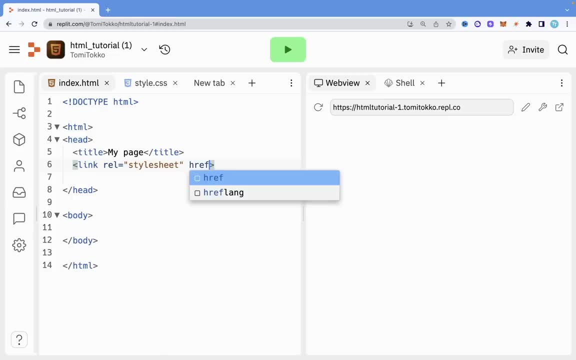 say style sheet and we're also going to have to say the name of that style sheet or the link to that style sheet. so right now we're going to say that we're going to say style sheet and we're going, right now we're just you're going to use the name of that particular css file, because on this, 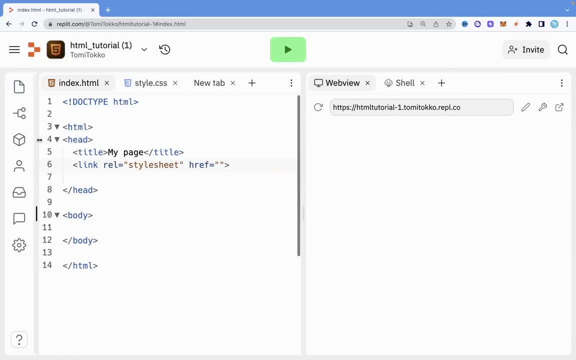 repli. right, all of these are under the same folder, so we can just simply say the name of the file instead of saying, you know, folder slash, whatever, because we have it in the current folder. so i'm just going to say stylecss. now, once i say this, anything i'm any css i code in here, or anything. 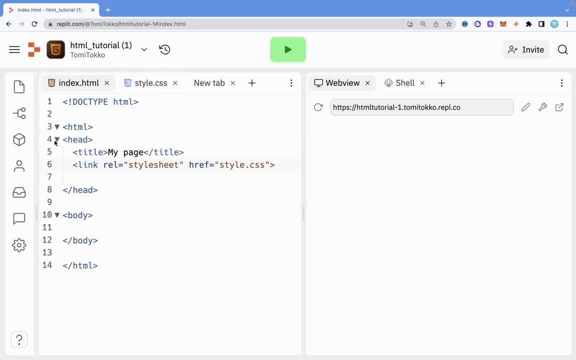 i try to do in here is automatically going to be added to this particular you know page. it's going to be effective now. now that you know how to do that, i'm going to start straight into the main css. so i'm going to talk about, you know, the css syntax like: how does it even work? how do we even start? 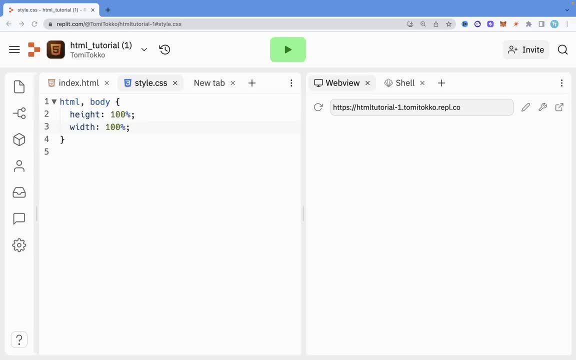 coding in css. so to write code in css we need to know two things and they are called the selector and the declaration. so, as you can see right here, automatically repli has this basic css code and what this does, right. so this html right here, as you can see, 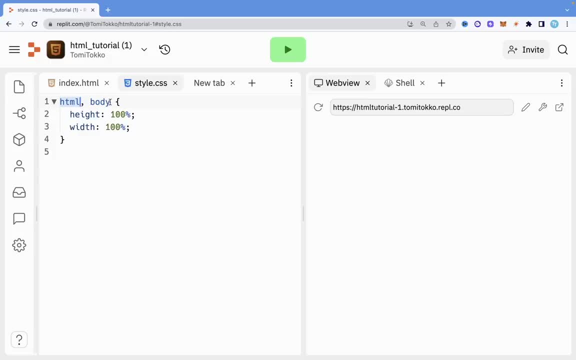 it is the selector. so first of all, i'm just going to let me just remove this html. i'll just have body. don't need to worry about that comma for now. so we have this body right here and that is a selector. and then all of these were saying the height of body should be 100. the width of body. 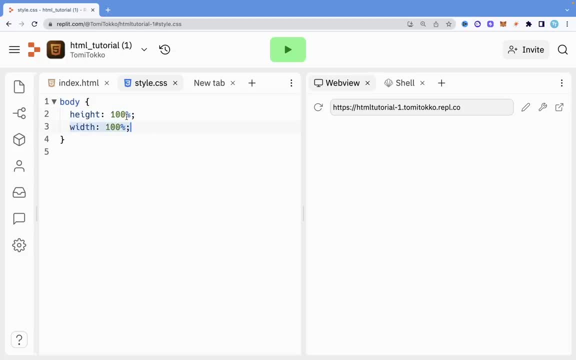 should be 100. don't worry about the details of what this does for now, but let me just introduce you to how we write code in css. so this is the selector right and this is the declaration. now this means that this body, we want, whatever we are doing inside here, to be affected on this body element. so what this is going to do, 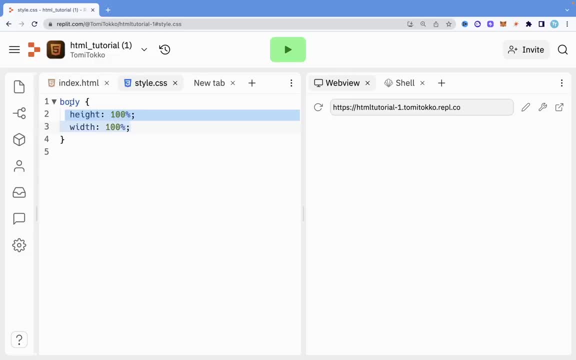 now is going to go into whatever html is linked to it and it's going to look for a body element. so it's going to come here and it's going to look for this body element. right, once it sees this body element, it's going to say: whatever we do inside these brackets, we want to have it been affected. 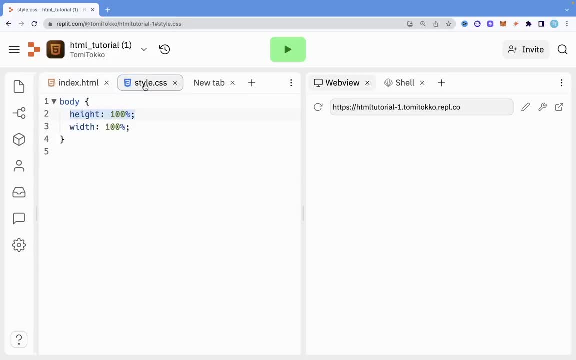 on this body element without wasting any time. let me show you how to do. you know our first change, so let me just get rid of this and let's actually do something. so i'm going to use the body again. let me say body. this is how we write a css code. so we say the element right, that we want to change. 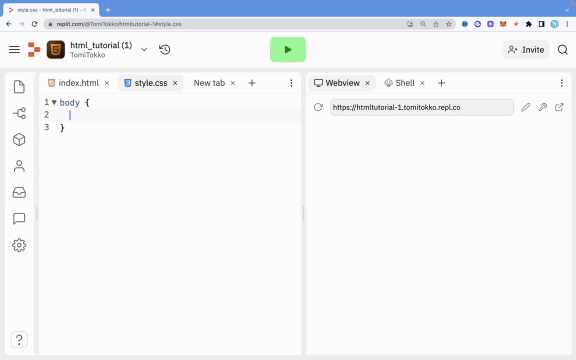 and then we use these curly braces and you press enter. now anything you do in here is going to be affected with the html or whatever file is being linked to it. so now our same body. now there are different declarations. the declaration can be: we want the color to be, you know, red we want. 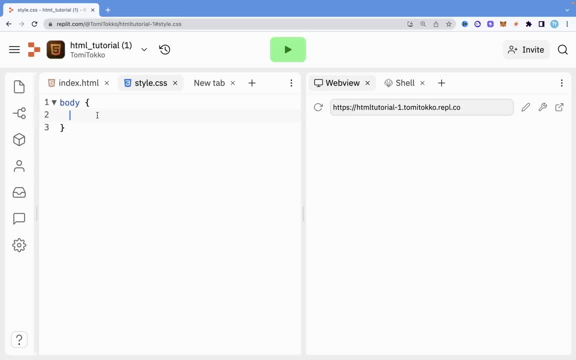 the color to be, you know, red. we want the color to be, you know red. we want the color to be- you know this. whatever font size in there to be- you know, 15- we can do a lot of things. i'm going to go through all of that in this section of this course, so first of all, let me just show you how you can. 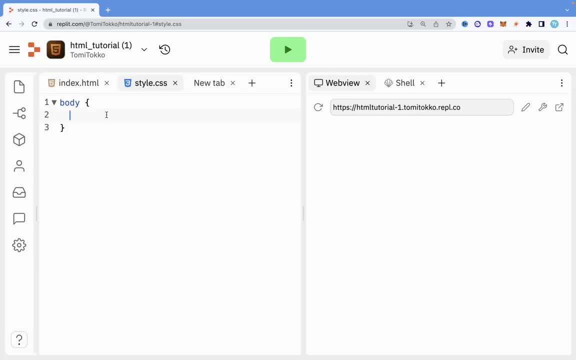 change the background color of the body to be, let's say, blue or red. so first of all, you know that this body is where all the code goes into. that means everything we're going to be coding in our html is going to be under this body, the visible part of the web page. so now we want the. 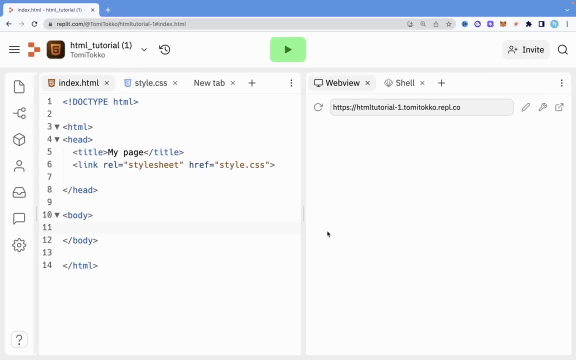 visible part of the web page to have a background color of, let's say, green, let's make it green. so what we're going to do now, we're going to say body. now, whatever we do in here, which you should know now, is the declaration we're going to say background. this is how you. 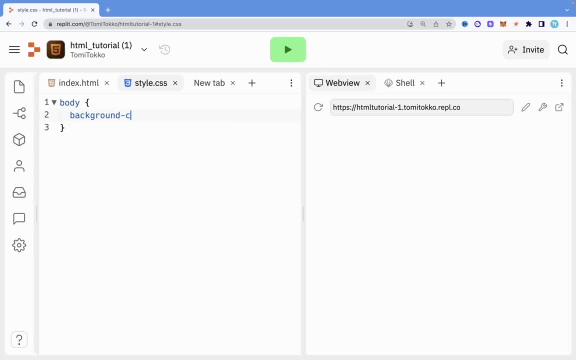 change the background color, background hyphen color, and we want that to be green, and then you must add this semicolon. now, the reason why we must add this semicolon is so that we can have another declaration right here. let's say, i want to change the font size. i can write something else if you. 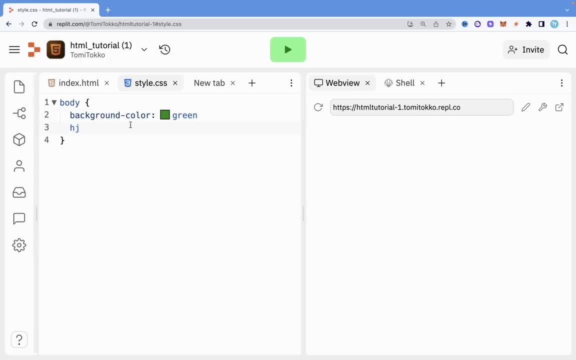 don't add that semicolon, going to think that whatever you add here is still part of this first declaration. so you must add the semicolon to end that declaration. so this is how you do it: background color, which is what we want to change. you put a colon and then you put a value. so think of this as a key and this is a value. 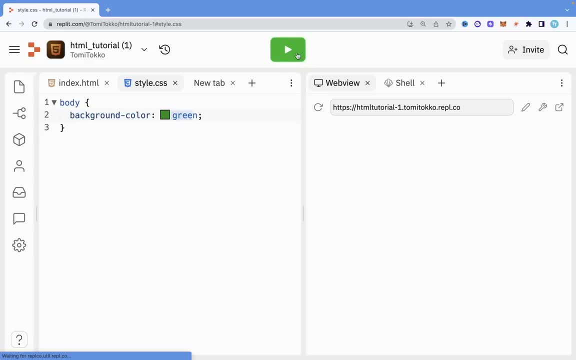 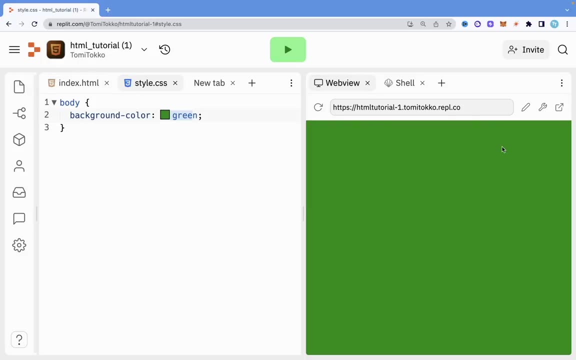 now let's run this and see. so we're going to run this. as you can see, now the background color of this is green, so it is effective immediately. now let's check what if let's say: i remove this, right, i'm just going to delete this. that means this html page is not linked to this stylecss. 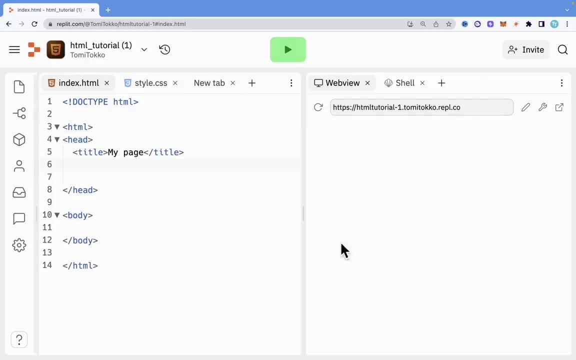 now, if we try to run it, you're going to see now that it doesn't show us a background color of green, no more. and that's just to show you that, no matter what you write in your css page, if you don't connect it or link it to your html page, it's not going to be effective. so now let's remove bring. 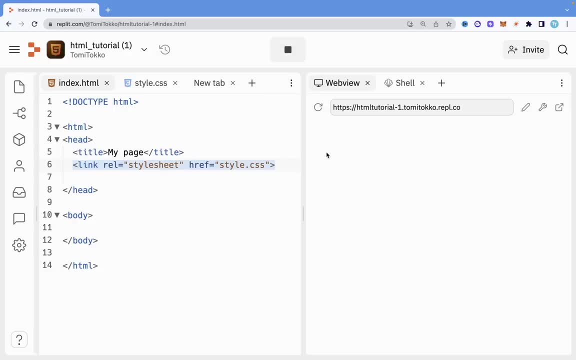 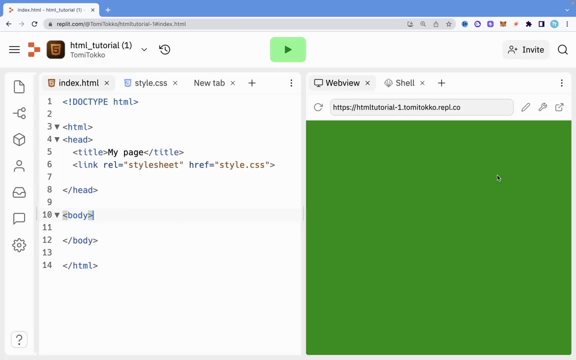 that back, and when we run this again we should have the background color as green. now let's talk about comments in css. so when we're looking into html- earlier in this course i talked about comments in html and in there i talked about what, why we use comment, what it is. 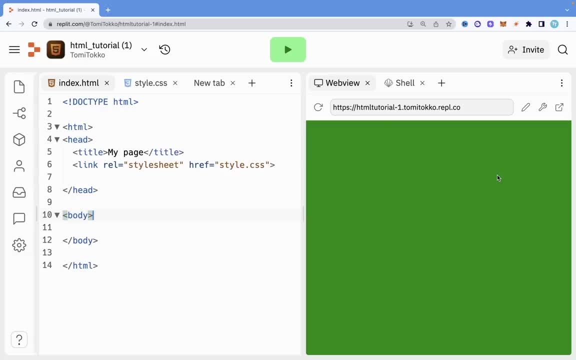 and you know how we can actually code that in our file. so in css is very similar to html. the motive for using a comment is you might want to explain a bunch of code, or you might want to just remove a part of a code that you don't want to be run. 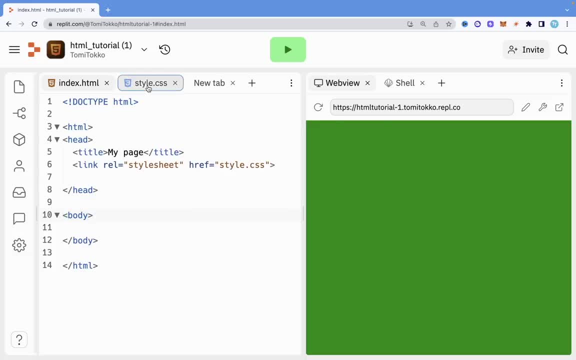 when your file is run. basically, let's say, i have this css file here, so if i comment out all of this body, the code is still going to be present in this file, but it's not actually going to be effective, so it's not going to be run by the browser. so let me show you how to add a comment right here in css. 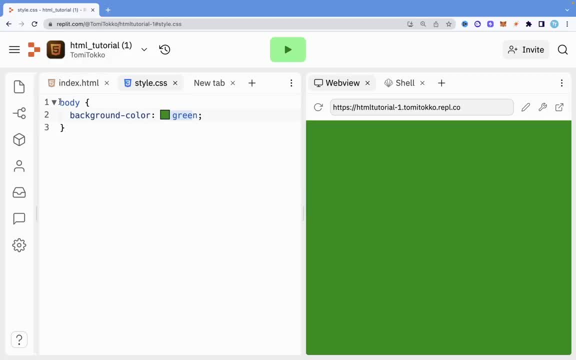 so we talked about it in html, but it's quite different here. so let's say i want to explain what this you know code does. i can add a comment, and to have a comment i'm going to have to use the forward slash, then i'm going to use the asterisk sign and here i'm going to write my 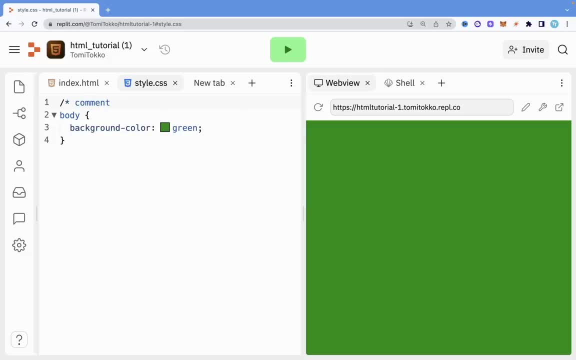 comment. let me just say comment for now and then for me to close that comment, because right here you can see that css still sees this as a normal code. due to the colors, i'm going to leave a space asterisk mark and i'm going to use the forward slash again. now you can see that that part is. 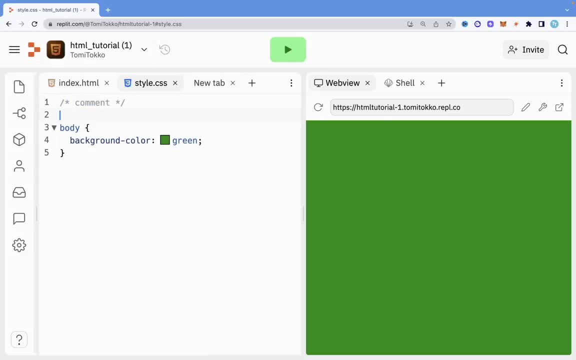 grayed out. you can see that the color is gray. so this just shows that this is a comment right here and i can just write something in here like: changes the background color of body, right? so that is explaining this code right here. now, that is a one use of you know, comments. you might also want to use a comment like, let's say: 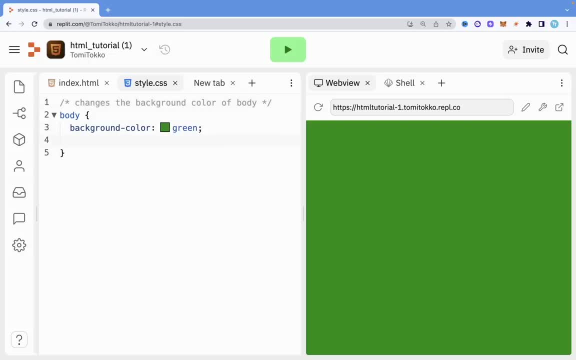 we have another thing that just you know. let's say another declarative or something like that, and it has a value. right, and i might just want to comment this out, i can do it exactly the same thing. i'm just going to have the forward slash, i'm going to have the asterisk sign. 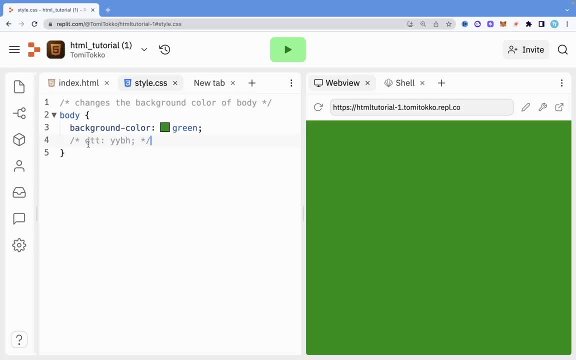 right. here i have the asterisk sign and the forward slash again, so that part is still going to be in this code, but the web browser is not going to run it when you actually run that file. so that is. those are the main two uses of commit, but apart from just using it to you, 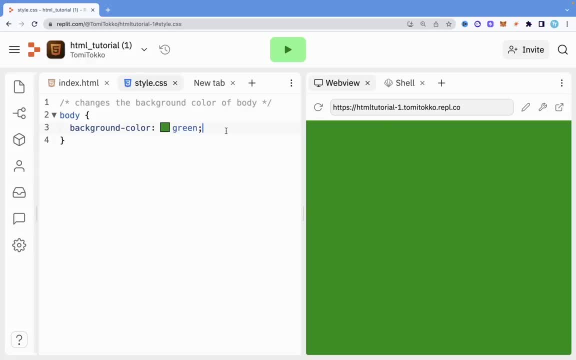 you know, adding it on top of like, let's say a code, you can add it somewhere else. let's say we have different- you know- declarations right here. let's say we have second declaration, third declaration. that's just an example and we want to explain each declaration by themselves so we can have the comments right beside this particular declaration. 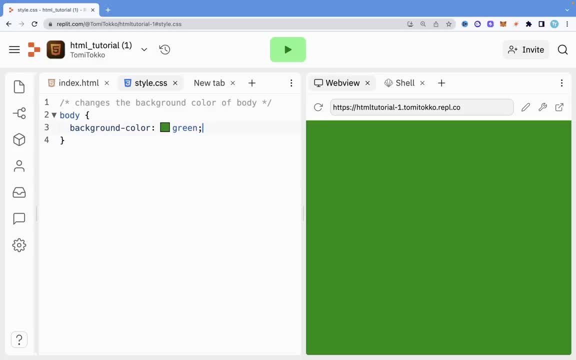 let me get rid of this. so right here i can just have a comment here that says: you know, change to green. so for me to do this i have to add the forward slash steric sign. and right here i have to do the same thing. i'm just going to do asterisk sign and forward slash so you cannot see that that part is grayed. 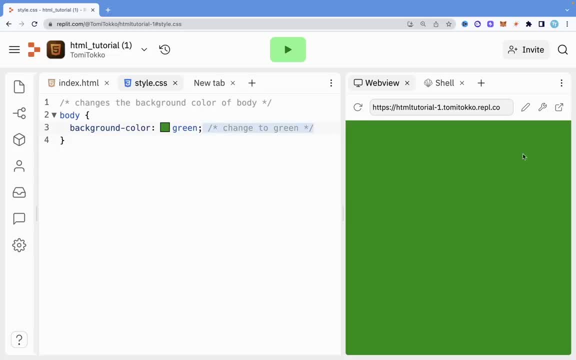 out. let me just make this something like this: so that is now a comment, right? so that's the easy way of you know using comments in css. it's quite easy, like when you're learning programming. well, you're going to notice that if you learn other programming language, each programming language has 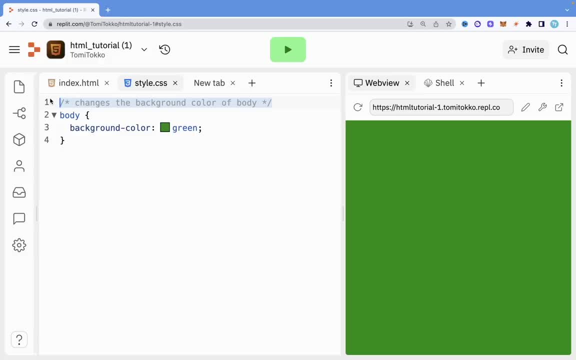 a different way of writing comments, but the motive behind using comments is the same in all the programming languages. now you can also have multiple line comment, for example, instead of just having one straight line, i can create a new comment right here and i can just say comment: aha, i can go to another line, continue writing the comment. 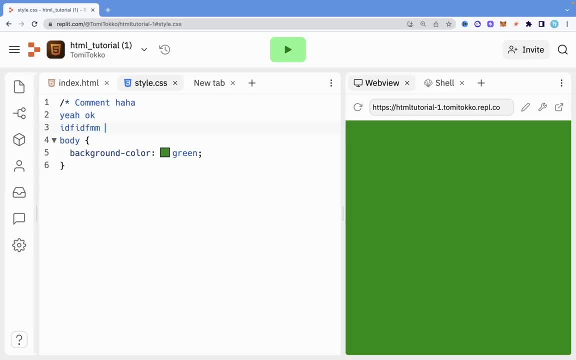 here. okay, just something random, and then i can close it right here so you can see that all of that been commented out. so it doesn't just have to be a straight line. so that means i can even comment out all of this code. you know, you can basically be very flexible with your comment, you can do. 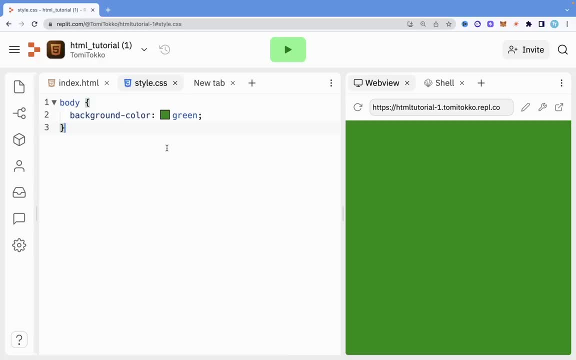 whatever you want to do, so that is a very simple and basic way of using comments in css. now let's talk more about selectors in css. so earlier in this course, i told you about how the syntax of css work, um that this is the selector right here and this is the declaration. 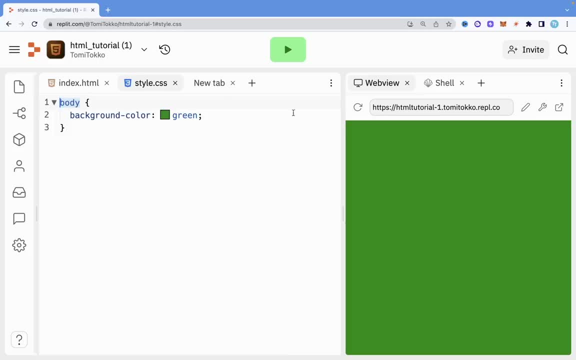 but now let's look more into how these selectors actually work, how we can pick different elements from html and style it. so see, the css a little is divided into different categories. but first of all i'm going to break down in, i'm going to break everything down. 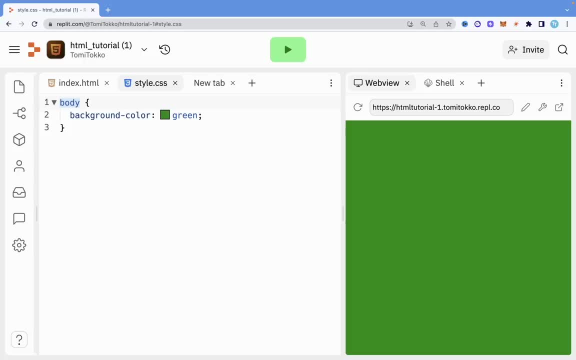 right now. so once again, css selectors. they're basically used to select html elements that you want to style right. so it's very easy. the first way to just have a selector is to come into your html and look at the. let's say, we have an h1 right here. i we want to look at the element right. 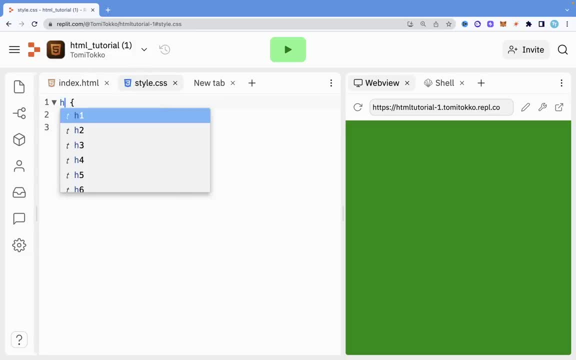 and then we're going to come in here and just write the element right there. we can just say on h1 tag: we want the background color to be green. so we've basically selected that h1 tag. very easy and very plain. now we can select an element or we can decide to style a text or 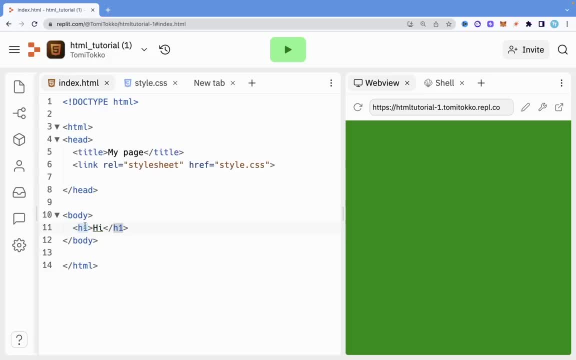 something else without selecting the actual element, we can select an id in that element. so remember, when we add, when we did a form and then we add an id as an attribute. now you can have an id, not just only in a form input, you can have it on. 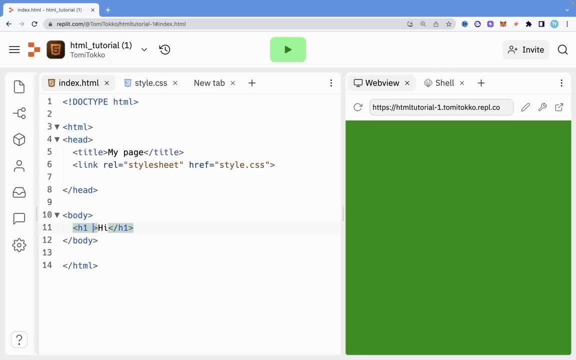 any html element you want. for example, i can add this id and say: the id is welcome, message: welcome. so now that i this has an id of welcome, right, i can come in here and then select this, all these particular elements, just by the id. so what i need to do to do this is to 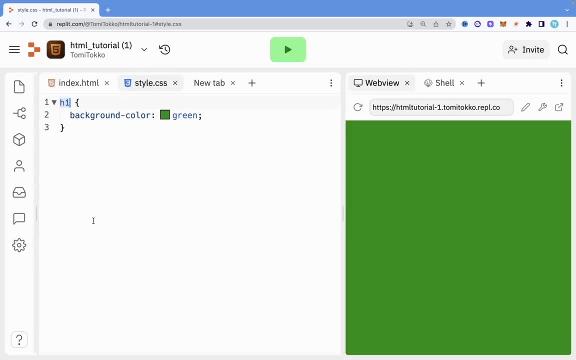 come in here and instead of just writing it directly, i need to write hashtag. now, once i put an hashtag, css automatically knows it's trying to select an element by identifying its id, so what you just need to do now is to write the name of that id. 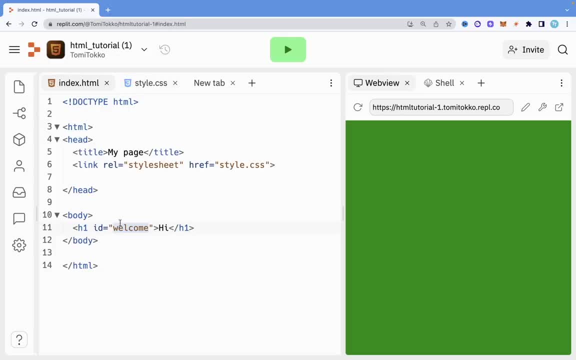 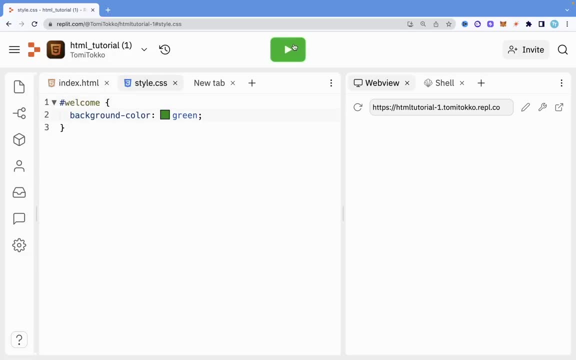 now css is going to go into this html file and it's going to look for an element with the id of welcome, and then it's going to make the background color green. now let's run this and let's see what it gives us. boom, you can now see that the background color of that old element is green. 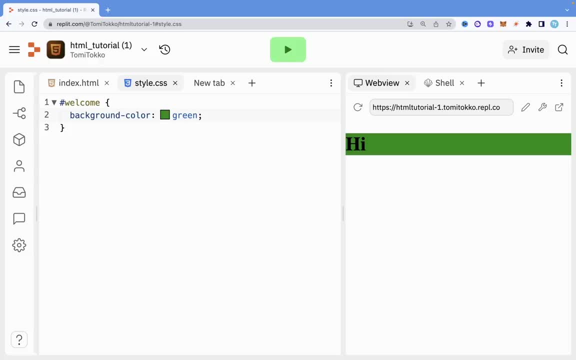 so that's a very simple way of using an id and this is also very- you know, very- useful. now let me explain a use case. for example, let's say we have two different h ones and this one says tommy, and if i run this, you can now see that only i is as an id of green, i mean as a background color of green. now imagine: 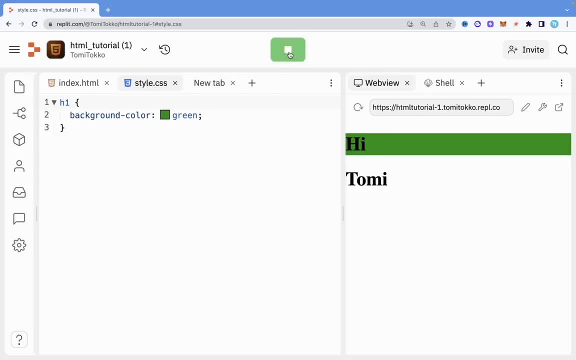 i didn't use an id and i just use h1. this is going to affect every single h1 tag that we have here, so it's going to have all the h1 as green. but what if i want just i to be green or just tommy to be? 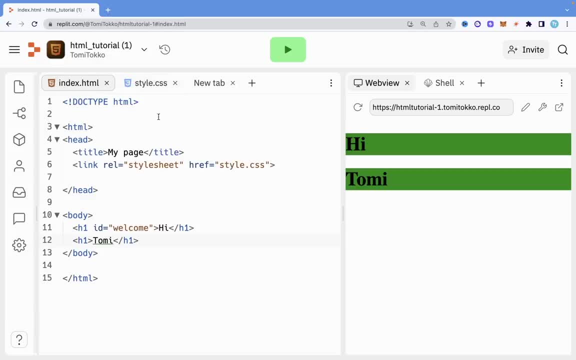 green. that is a use case of using the id to select it, because the id is unique to every single element, so that is also very, very useful. so now, that is one way of doing that. let's run that again and see everything is working. another way of selecting an element or a text or whatever you want to style, is to select it. 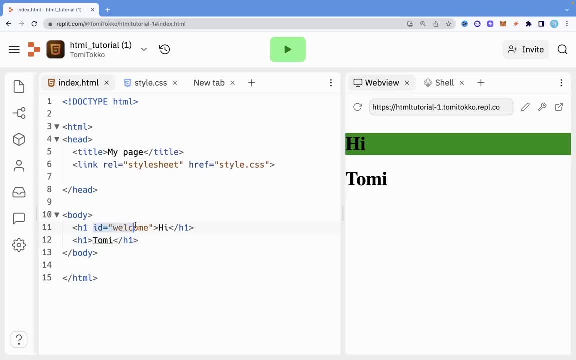 by the class. so there is something named classes in html and this class is also an attribute right. it also identifies a particular element. so once you have a class in an html element, you can then use that to select that particular element and style it. so, just the way we have an id, we can. 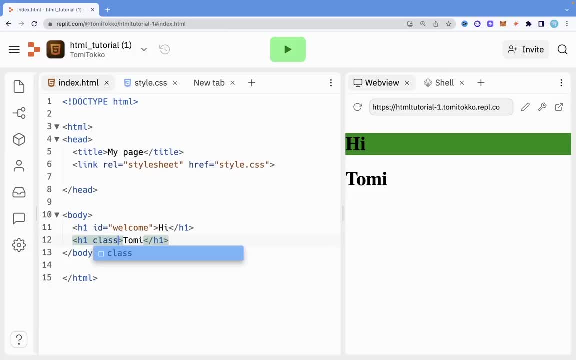 have a class here, just the normal way. we write html attributes, you write class and then you give it a value. so let's say this class. we want this class to be something like heading, so that is the name of this class. so now we can select just this class and say we want to style all of this. 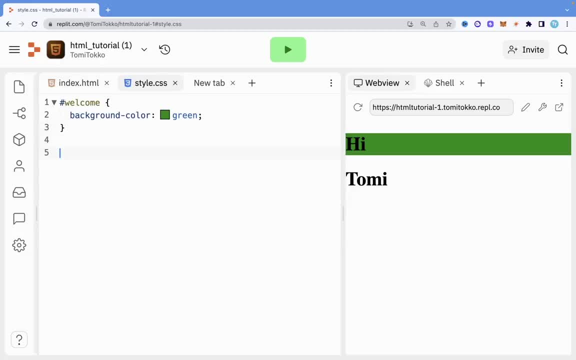 for you to do that now. let's actually actually just create another. you know declaration, selection and declaration. so for us to do this now. we want to select this particular element using its class, so we're going to do dot heading, so this is the selector. when you see dot, something that 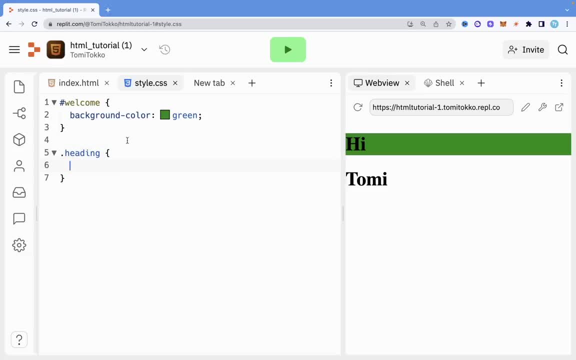 means we're selecting an element based on its class. so this means we're trying to select a class and this is the name of the class, and now we can just say we want the color of whatever is there to be blue, and we can use a semicolon to stop that. 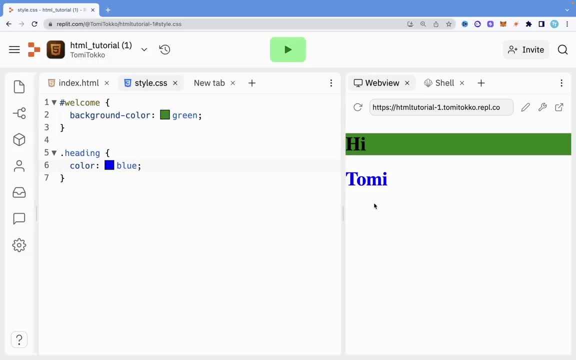 now, once i run this, you should see that it has a color of blue, just this one, and that is because it has been seen, or it has been selected just by the class. now, this is very helpful, right? so you can also do like more advanced stuff with this. for example, let's say there are two different. 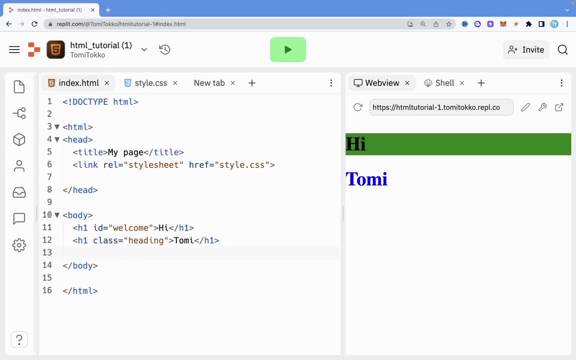 let's say we. there are two different elements. that has a class of eden. so let's say we have p and this, just say tome small. or let's just say tome again, and this also has a class of eden. if i run this, this is: 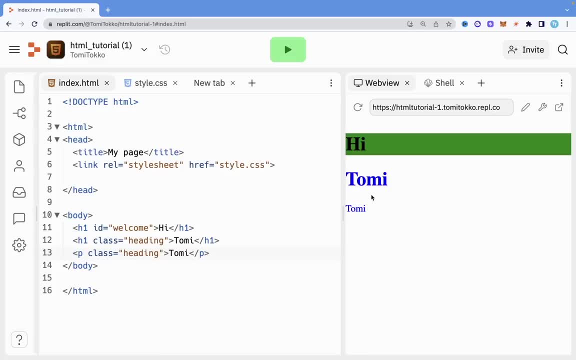 going to show a smaller to me, but it's also. it is also affected because we selected it by the adding. so anyone that has a class of adding is going to have this blue color on it. but let's say we just want to say just the h1 tag that has a class of adding should be blue. so that means 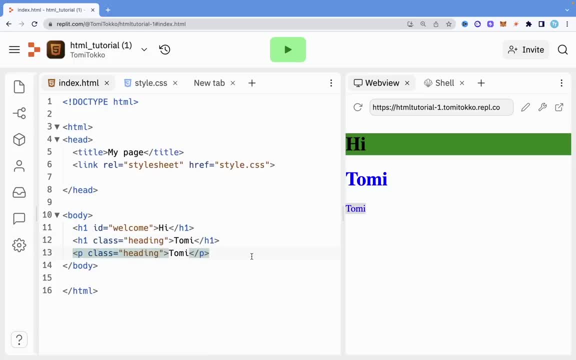 we don't just want to get every single element that has a class of adding just an h1 tag that has a class of adding. now for us to do this, what we're going to do, right here, beside the dot, we're going to say h1. so now what this is going to do is that it's going to go into the h1 element and 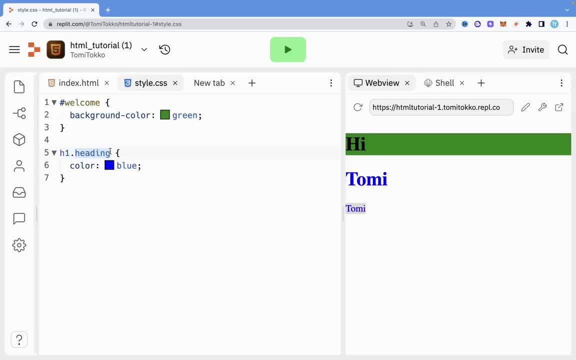 it's going to look for any h1 elements that has a class of adding. now, if i run this, you're going to see that that p is not affected. no more, this is just black or this is still blue. that is a very good- uh good- example of how you can do this. now there's also 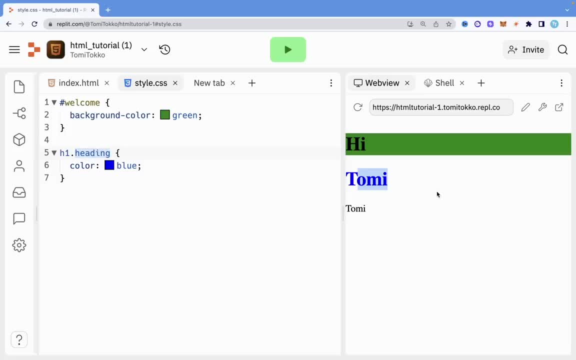 one more thing, and this is the universal selector. so the universal selector is basically a selector that affects every single element in the html page. so let me show you what i mean. so let's say, i want every element on this page to just have a color of red. every single element should be red. 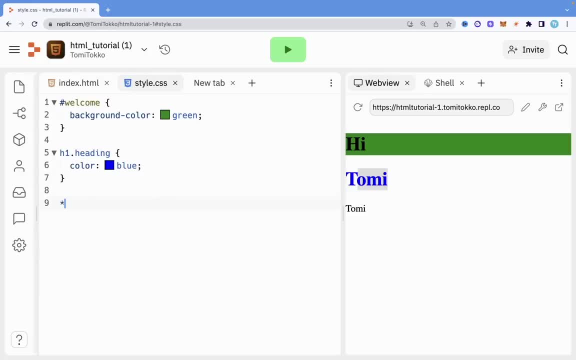 for me to do this. i'm going to use the asterisk sign. if i use the asterisk sign and have my curly braces normally like this, this means that whatever i'm writing in the html page is going to affect every single element in the html page. so let me show you. 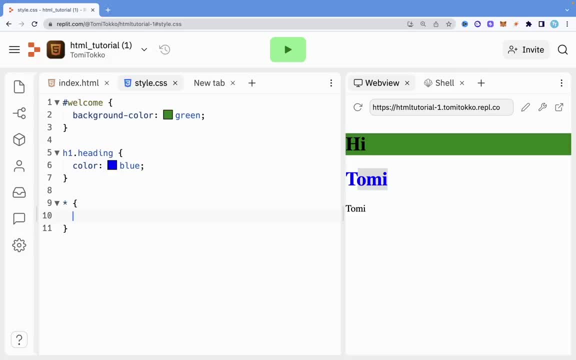 here. it's going to be affected by every single element, with no one left out. so now i can just say color, i can say purple, so let me just get rid of this. and now let me run this, so you're going to see that every element on here has a color of purple. 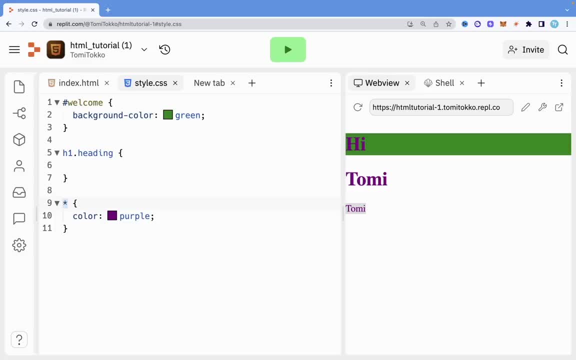 that's because we use this asterisk sign, also known as the universal selector. now, this is, you know, a very good use case, because you might just be building a page and you want that page to, you know. let's say, all the text should be in the center. 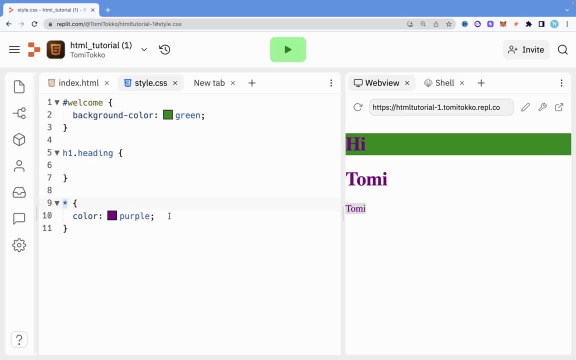 you can use this to do it right, so that is a very good one. so the last one i'm actually going to talk about is the grouping selector. remember, when we first started this css video, there was like uh, html and body, something that was written like this, and i got rid of one because i said: 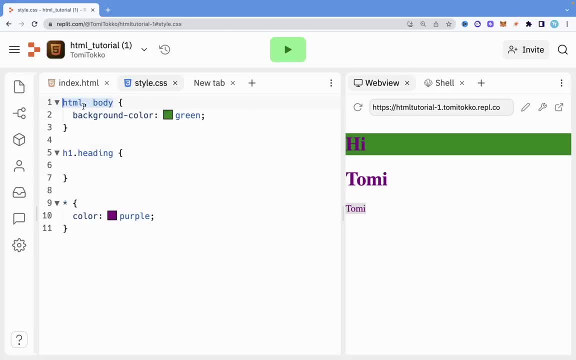 we're going to talk about that later. so now what this is is called the grouping selector. so let me get rid of all of this right. and let's say i have an h1 tag, an h1 selector, that says you know color, and let's say green. and then i have a p tag, a p selector, that says color green also. 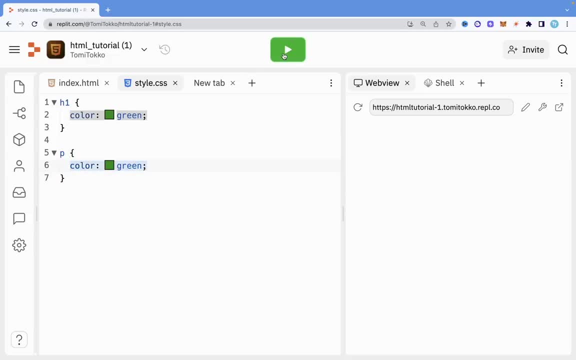 right. as you can see, i'm just repeating the same thing. if i run this, it's gonna have green, all of it, h1 and this is p. now i'm repeating the same particular, you know declaration for two different elements. now, instead of having to write all of these because, let's say, i have 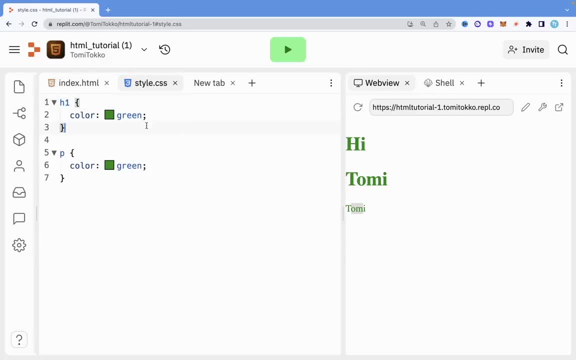 lots of elements and i want all of them to be green. i and i have to start writing h1- color green, p color green, you know, b color green, strong color green. we don't want to do that. you can actually just come in here, have a comma and say p. so this means that for the h1 and p, 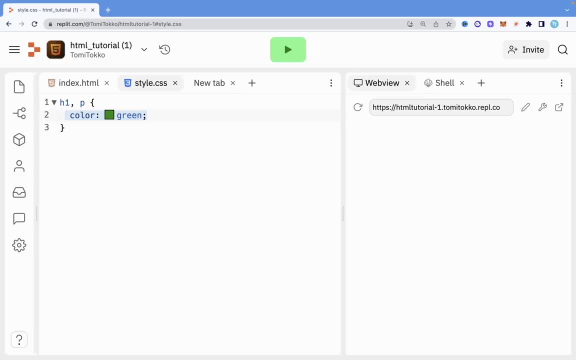 say p, it doesn't matter. i want p color blue, and if it is green i can edit my position. or h1 color green and it's time equal to p color in general. but that is not necessary because this, especially though it's going to respond like this and it will work, and happy like this that we actually 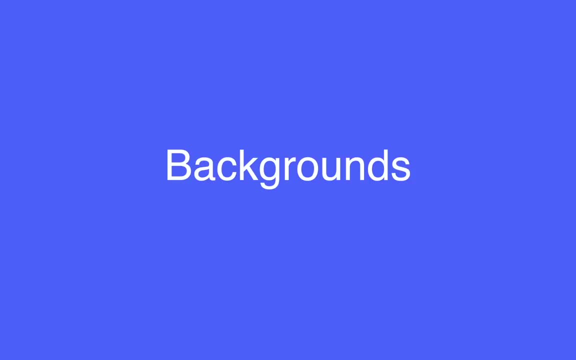 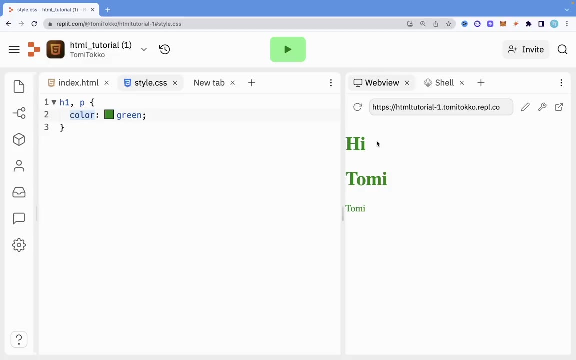 need not to exceed b, and we want to have done the same thing with all of this. you see, after i turn this on, that's like it doesn't really matter, is right now. i'm just going to askize the background color and say stars. so let's say i am going to do that too, and exactly like that. 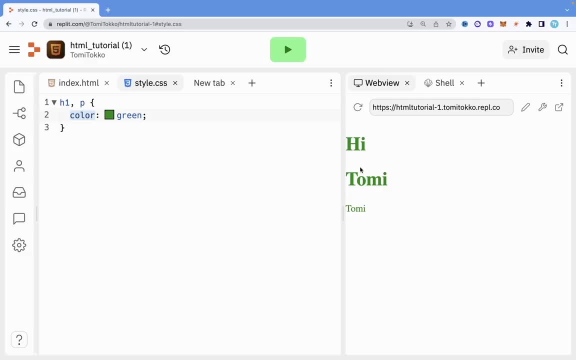 what you see here. you should have actually a background that might be a green, even red, and then you could actually banish the background, just to show you that you are gonna do this by�os in backgrounds in css, so like we can make a particular element, have a background color. 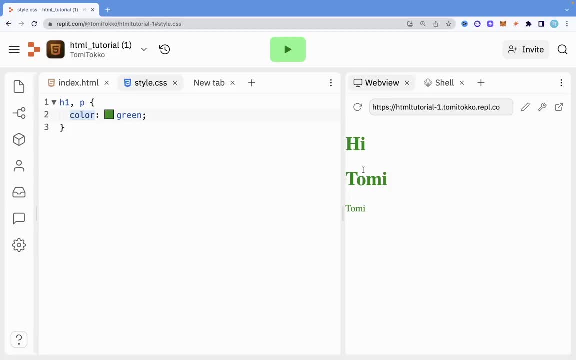 we can make that element have even a background image. so let's say we just want this part to have, like, a background image, where an image will be the background. or we can just make the whole page to have a background image. so there are, you know, lots of other stuff we can do and we're going to 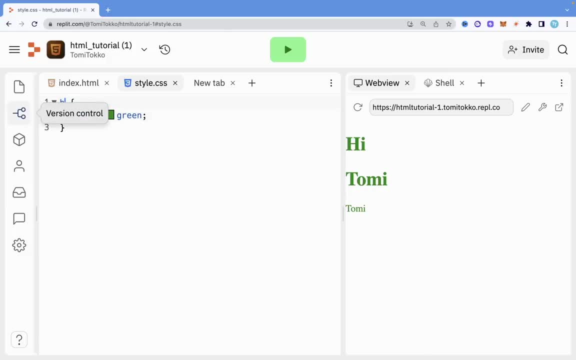 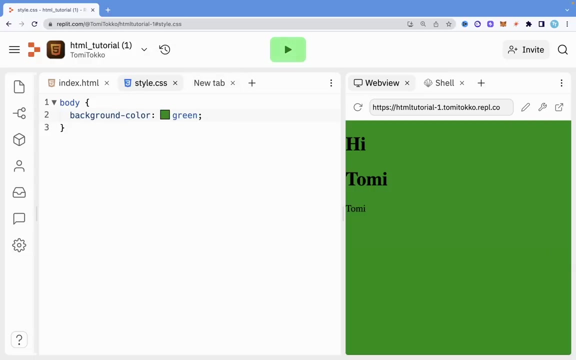 talk about them now. so first of all, let's just make this the body right, and in here, instead of just saying color green, we actually want to say background color. so, similarly to what we've done before, and once i just click on run, the whole background is going to be green. that is very easy. 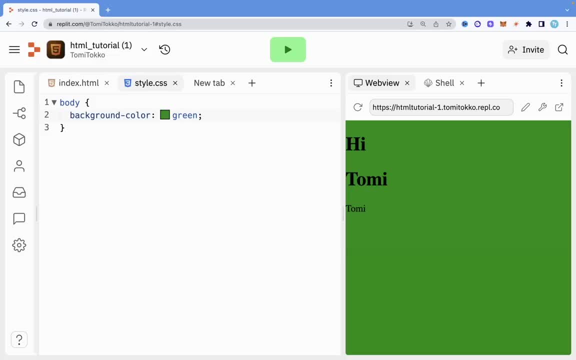 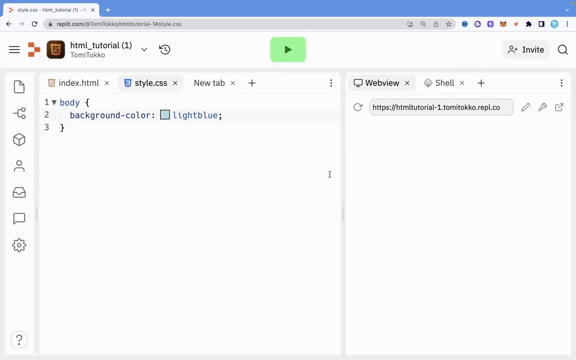 and simple, right, but there are also more stops we can do than just this. for example, instead of just having green, let's say we want to have blue, and instead of just having a normal blue, we can say we want it to be light blue. if i say light blue, you can see that it's going to be light blue. 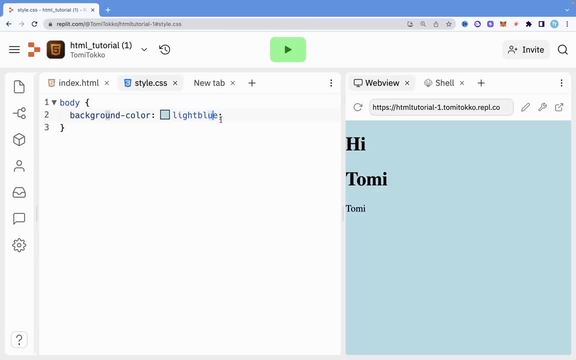 compared to the normal blue. so there's a lot of stuff you can do and i like repli because it automatically just gives you a lot of suggestions. once you say blue, you see all the blues that it has. so you can also go online to search like: what color of blue do we have? you can see medium slate. 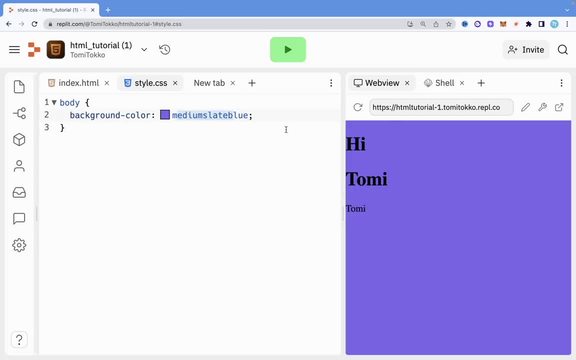 blue. you can run that it's going to be that particular blue color. so you can go online and search all css colors or css acceptable colors. you can see a list of it and you know you pick which one you want to pick. now, that is one right. 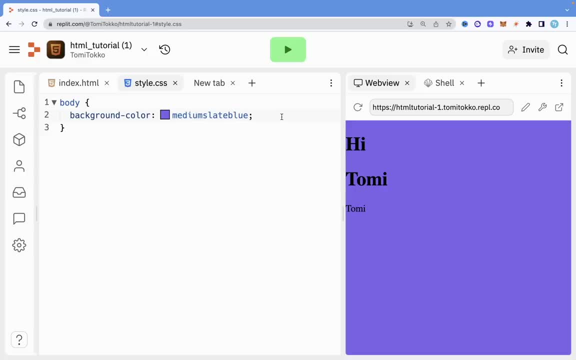 and there's another thing we can do by adding an opacity or making it more transparent, basically. so there is a opacity declaration that we can add and it's going to make this, you know, a bit lighter, a bit more transparent for you to do. this is very easy: we're just going to say opacity. 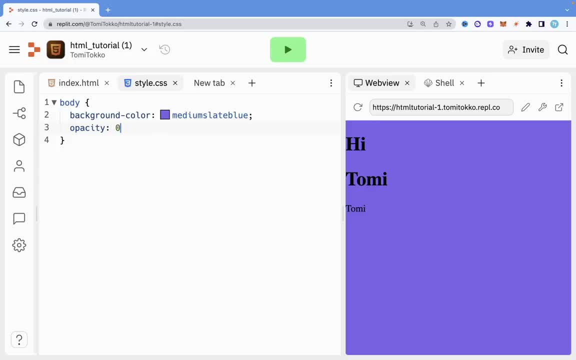 and let's say we want it to be 0.4, so you can make it all the way from 0 to 1. that is the range. so the lower the value, the more transparent it's going to be. If I say 0.4, you're going to see that it's quite. 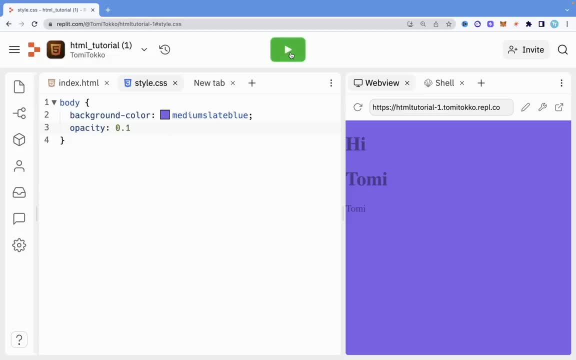 transparent. right, But let me say 0.1.. You're going to see that it's very transparent. But what if I just say 0.9?? You're going to see that it's opaque, very opaque. So you can do that, And 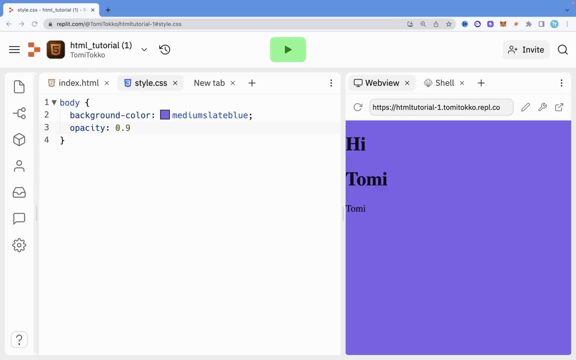 now, that's how to just have a transparency on your background colors. Now let's just go straight into talking about background images. So, for example, let's say: I don't want this to be a background color and I want it to be an image. So, since we know that we've already selected the 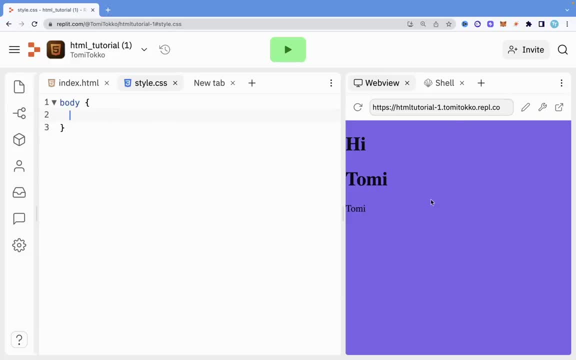 body. now, if we add anything, it's going to affect the whole page. Now, let's just do that real quick. Now for us to have a background image quite similar, instead of writing background color, we just change our color to image. So I'm going to say background hyphen image And now we're. 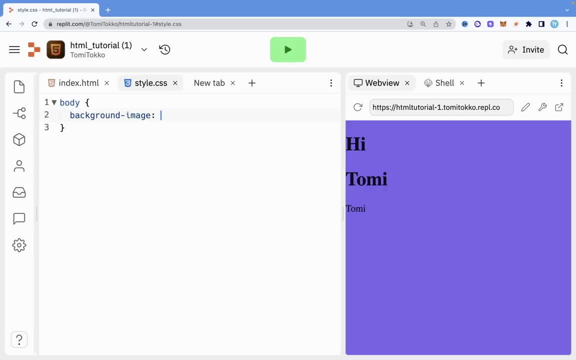 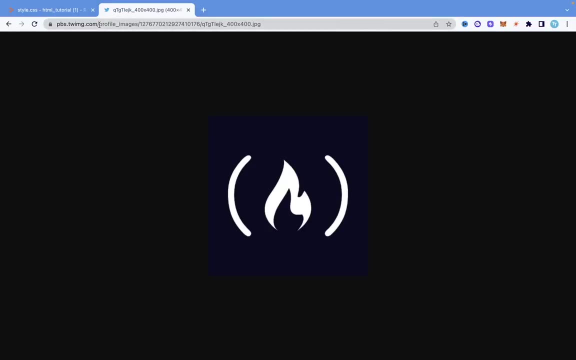 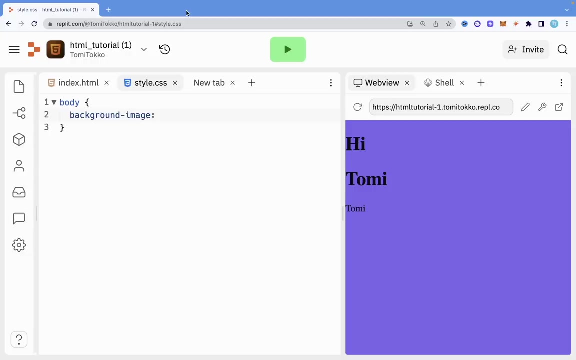 going to have to specify the URL where we want this image to come from, right, The source URL. So if I I have a link copied, I'm going to paste that. So that is the link right there And it just opens the an image of the free code camp logo. So I'm going to just copy that again And I'm going 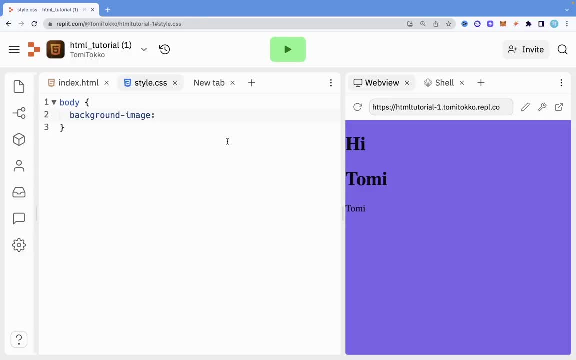 to close that. So, since we know we have the URL to that free code camp logo, what we just need to do now to tell CSS where to get that image from is, to say URL, And then we're just going to have brackets, we're going to have the codes And in that codes we're going to paste the link. 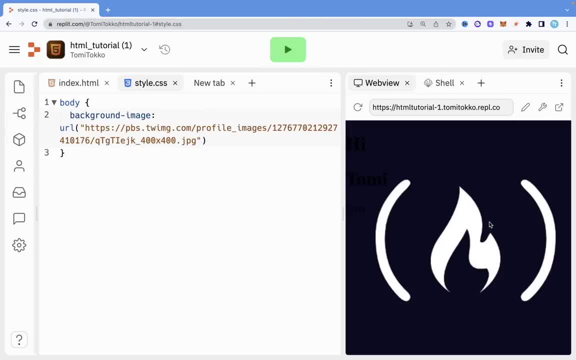 To that image. So if I run this, you're going to see that the background of this is actually that free code camp image. So, as you can see, the text don't show. but they actually did. They don't show just because the background is black and the text is black. So now that we know CSS, what we can. 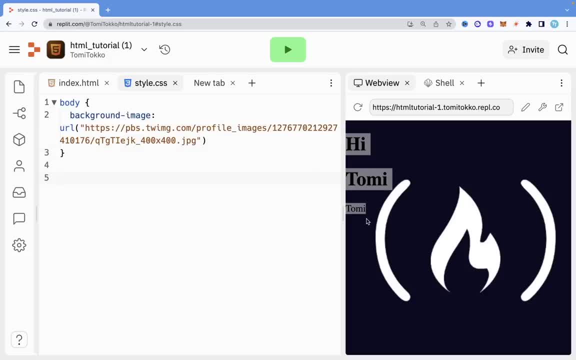 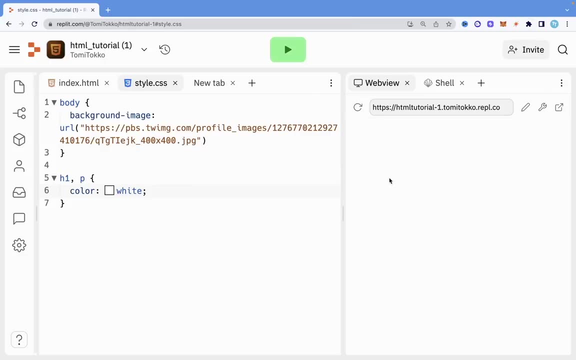 just do is to say: you know, this is h1, and P. we can say h1,, we can use group selector h1, p, And then we can just say: we want the color to be white. Now, once I run this again, the text should show exactly. so you can see that that. 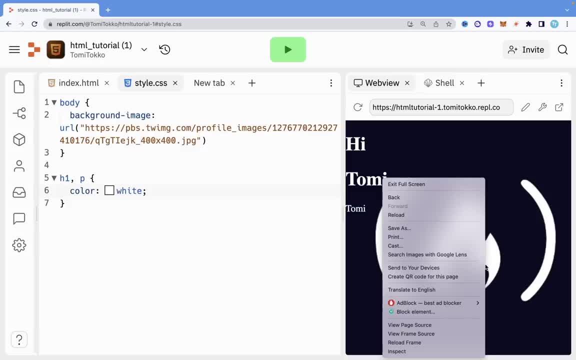 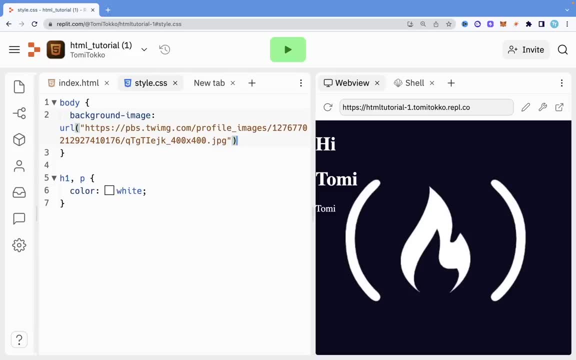 works. This is just the background image. this doesn't really have any effect on it, But this is the text that is still showing. The next thing that we want to talk about is the background position. So, for example, let's say, we just have a background image that you know is very small. 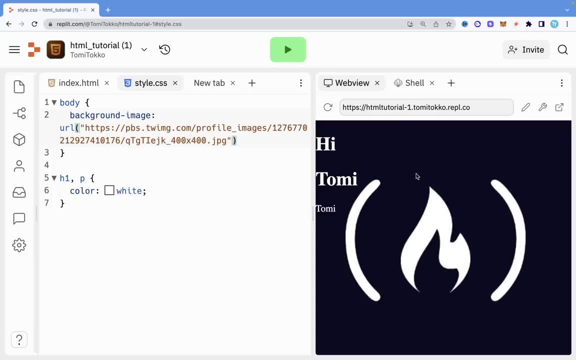 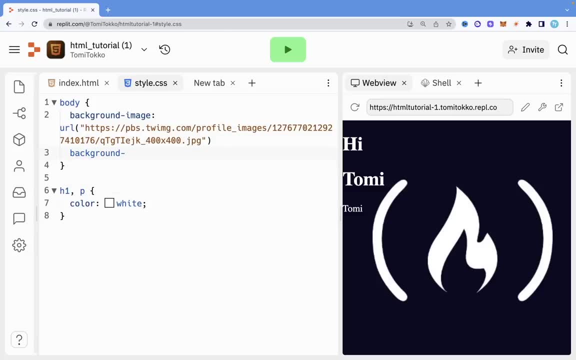 and it just stops here right, We can have a background position and say we want it to be at the top right corner. So we're going to do background hyphen position. We can just say we want the position of that to be. 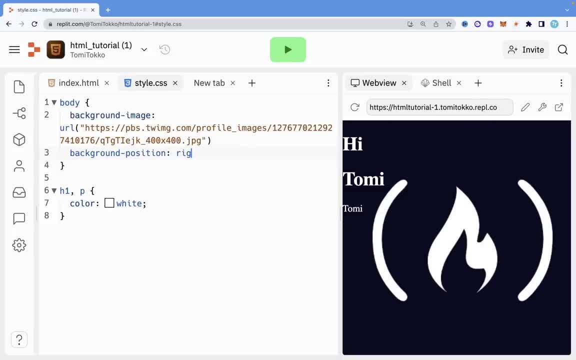 at the top right, So we can say right, want it to be at the right, and then we're going to leave a space and say top. So this means that it's going to be at the right corner, but the top of that. 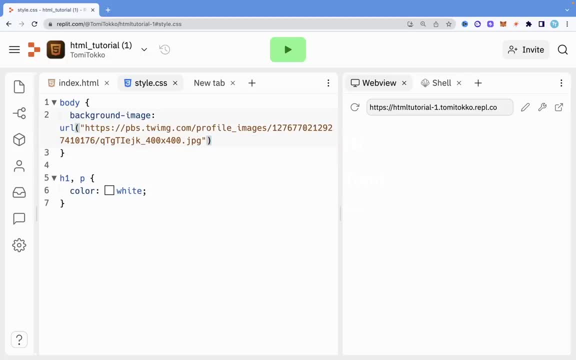 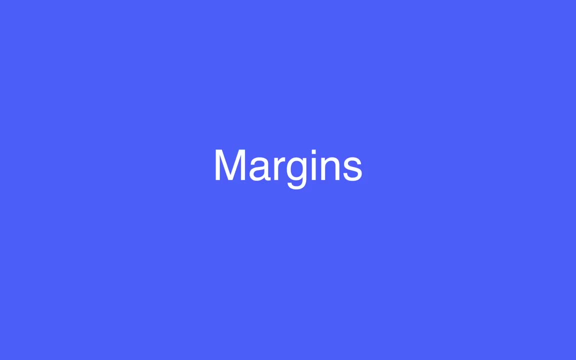 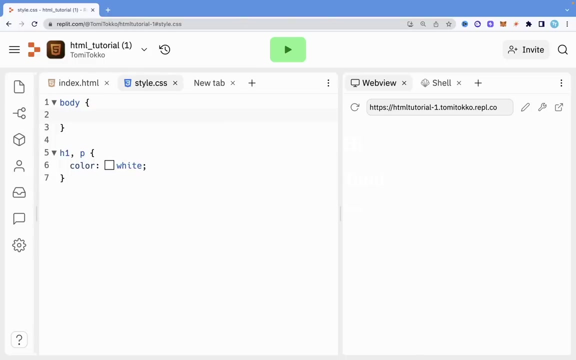 right corner. So that's what that does. So, now that we have all of that, that's the very basic way of, you know, having background images in CSS. Now we're going to look into margins in CSS. So margins are used to create spacings around. 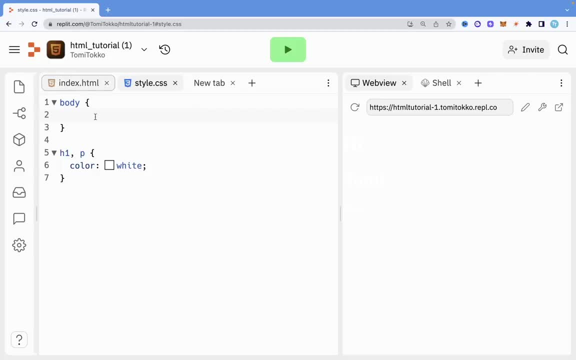 elements. So, for example, when I have this, let me change the color of this to black. I'm going to run this So it should show the text. let's say, I want this p tag to have a margin of say well. let's say i want this tag to be somewhere around here instead of just from the beginning. 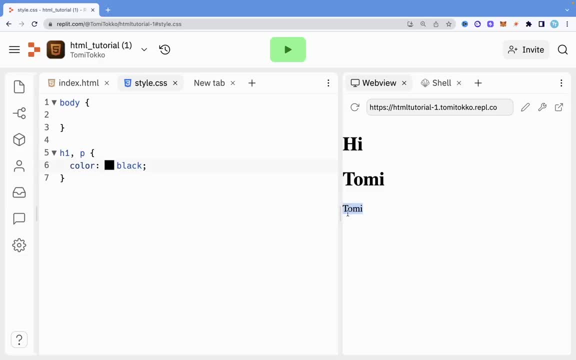 i want it to be here. that's when we use margin, so we can specify the like space we want from the left side, from the right side, from the top. i can also bring it down and i can also, like, take it up. so that's what margins does. it basically allows you to create like spaces around elements. now, 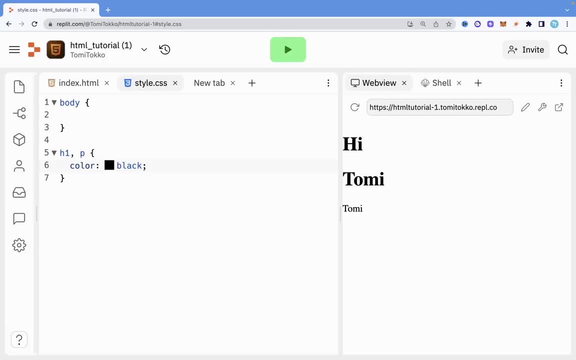 there are different ways we can specify the margins. so, as i said, we have the margin top, we have the margin right, we have the margin bottom and the margin left. so each of that are just used to specify the spacing for wherever we want, if we want it to be, if we want there to be. 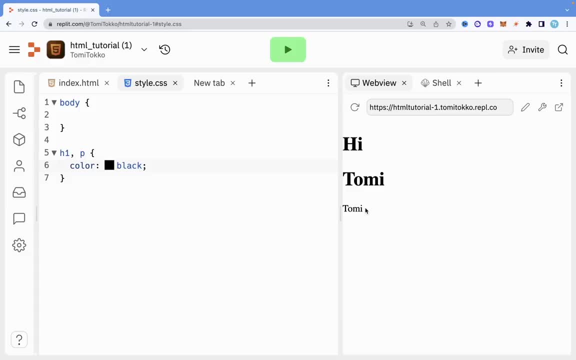 a space at the top. we use the margin top. we want them to be a space at the right. we use the margin right for the bottom, margin bottom and for left margin left. so now let's just go straight into this. so i'm going to remove this h1 and we're just going to have p, so automatically it has a color of. 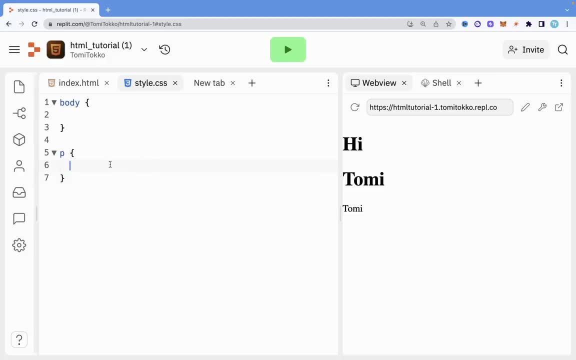 we don't need to write that. so what i can just do now is to say margin- is how i write it? hyphen, let's say left. once i say margin left, then now, when i want to give it a value- now there are different values we can give it. we can specify how far we. 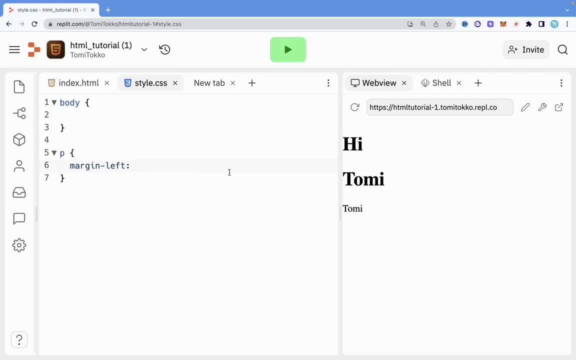 want it to be like in in actual numbers, like i can say 20 px. now, if i run this, you're going to see that once i run it there's going to be a space on the left. you can see that it moved a little bit. so you can keep going like that with numbers right. all right, i can say what? 50. now if i say 50, 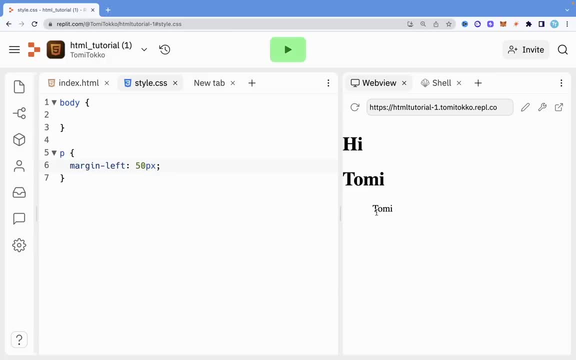 and i run it, you're going to see that it's going to move again a little bit. so that means i've created a space of 50 px from the left right. i can do the same thing on the right, the top and the bottom. so that is one way of specifying a value. another way i can specify a value is by using 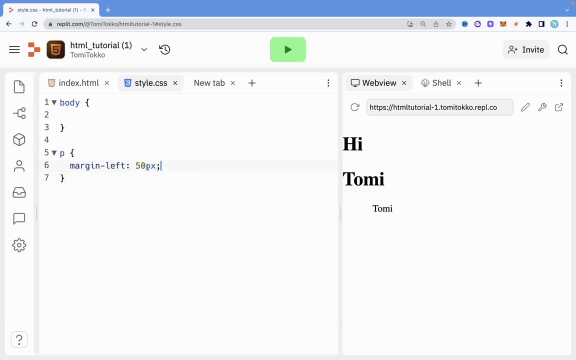 a percentage. so i can just specify it by saying: 50 percent you, and once i run that you're going to see that it has it in the middle. so what it? what the percentage does is that it calculates the whole width of the you know element and it puts it in like from 50. 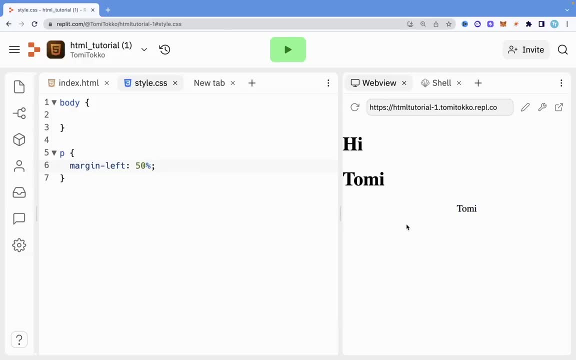 so this side is 50 of this whole width, so that is why we have it there. so that is for the percentage. what i can just do now is to actually show you what more i can do, like i can say, instead of having 50, i can say 50 px. 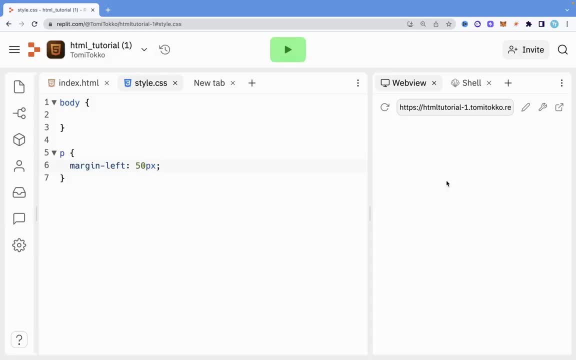 on the top. Now I can see that a little bit. there's now more space here. now i can also do the same thing and say margin, right, so i can specify it, for this was just for the left. if i run, it is going to have space in here. i can. 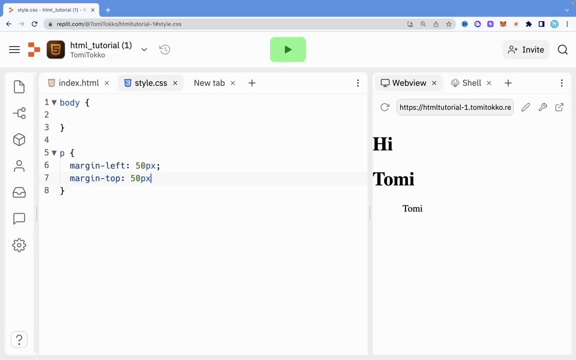 also say i want there to be margin on the top. If i say margin top and i also say 50. Now, if i run this, our going to see now that a yes, my 왶 came down a little bit, there's not more space Here. now i can also do the same thing at the same margin. 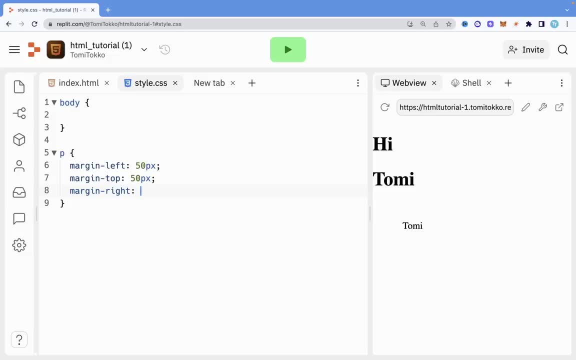 Right now, if i run this right, i say 50 px. right, so i'm saying the margin right, you have 50 px, not going to really show any difference, because there's nothing is actually, um, like moving from relative to it. like, for the left is moving 50 px relative to this, border from the top is moving 50 px relative to this. you know this. 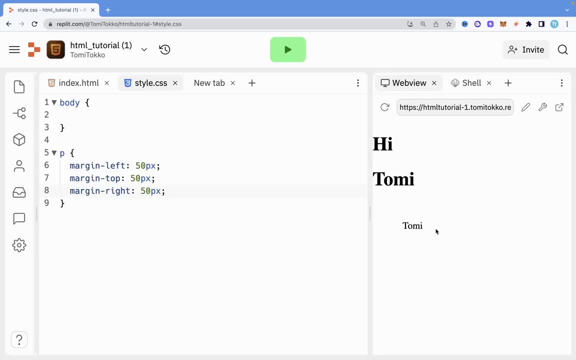 h1 tag, but there's nothing here, so that's why it doesn't really move, right. but i can also say margin bottom and i can say 50 px. now, once again, it shouldn't move. that's just because there's nothing is moving relative to this right. so it does how it's going to be and once we have that, 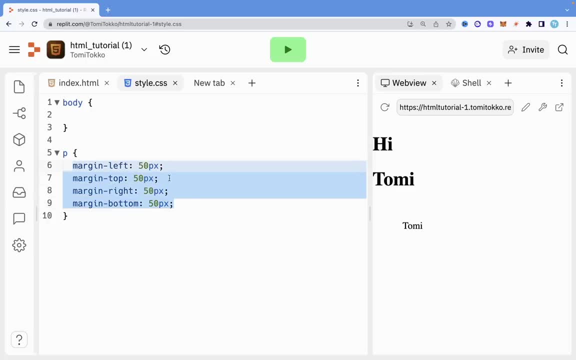 we basically know that we can specify what particular you know side we want it to move from. so, instead of writing all of this right here, you can see that this is quite a lot of code. just you know, to make some spacing you can actually compress all of this into one. so what i mean is that, let's say, i get rid of all of this. 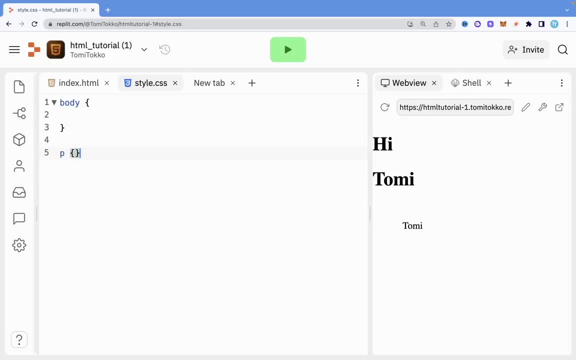 i can just actually make this one. so i can say margin and i can say it's going to have a value of, let's say, 50 px, 50 px, 50 px and 50 px. so what this does is that, instead of having to write, 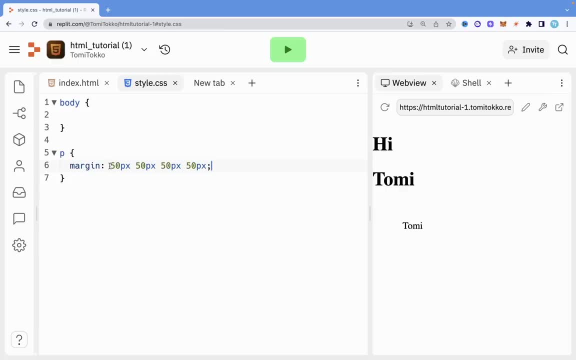 margin, left margin, right, all of that. it just uses this to say this: first 50 px is the top margin, this second one is the right margin, this third one is the bottom margin and this is the left margin. so you can compress all of this into just one line. 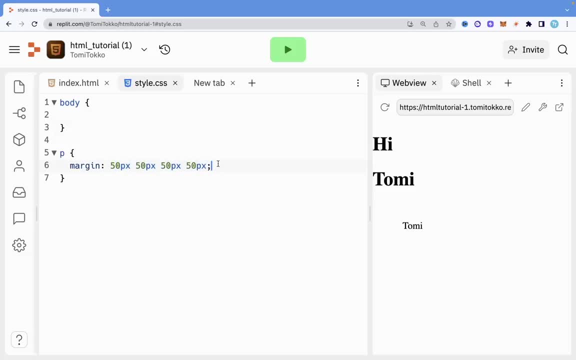 of code, or css, automatically knows what this stands for. so you should also know that the first one is the top, second one is the right, third one is the bottom and fourth one is the left. so if i run this, you're going to see that there is still some spacing. the same spacing as the same margins as we set before. 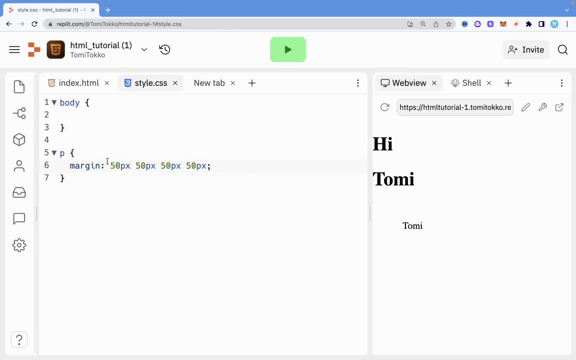 now, that is for you know, if you want to specify four of it. but let's say you just want to have three margins. now what does this mean? this just basically means this represents the top, this represents the right and this represents the bottom. so i'm going to run this and you see that we still 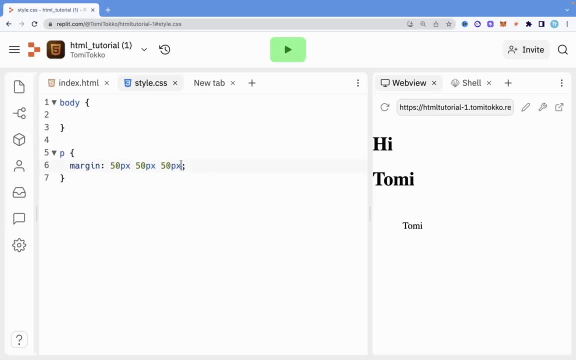 have the same thing. i can do exactly the same thing and just have two margins, and you should have guessed by now. this just basically represent- but this is quite different. right, this represents the top and the bottom margin right, and this represents the right and the left margin. so that means it's basically the same thing as. 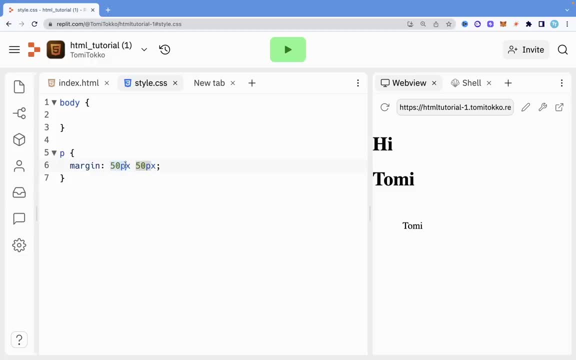 saying 50px four times, because this 50px represents both the for, the top, and for and bottom, and this is the right and left. if i run this, it's going to be the same, obviously, and you can also just have one margin. if i have just one margin, what this does is that this 50px represent all of the four. 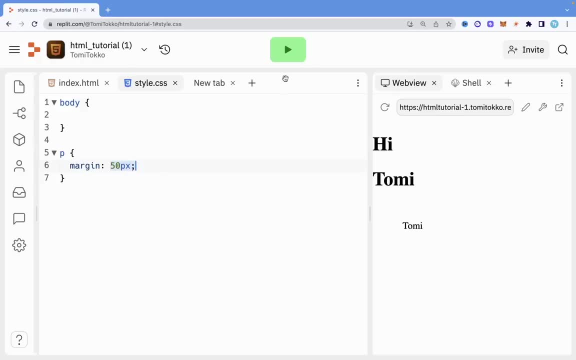 margins. so top right, bottom left, this 50px represents it, and once i run this you're going to see that it basically has that the way it is. so there's also one more way we can specify margins. we can say inherit. so let me explain what this inherits does. so if i come, 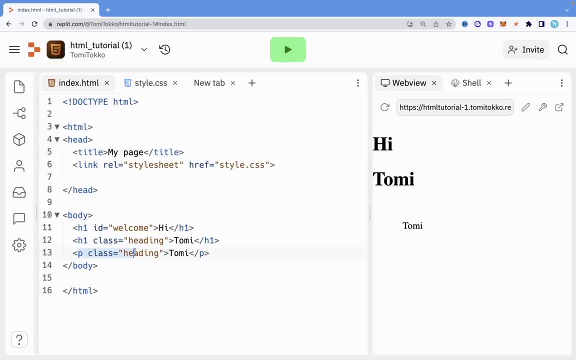 in here and let's say i have this p right under, let's say, a div tag. if i have this p under a div tag, right, uh, let's just say something like a b tag. so let's say this b, this p is under this b type, and i come in here and i'm i actually, you know. 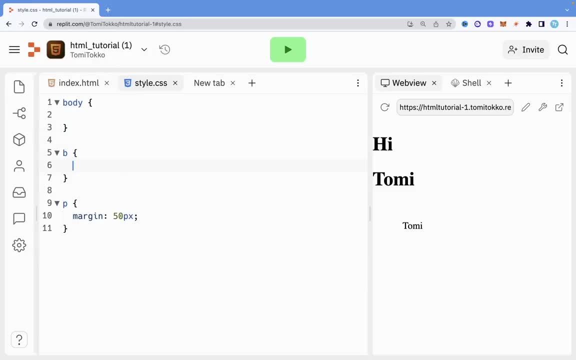 style that b tag and let's say i say margin top is something like 50px, let's say 60px, 60px. so since this p tag is under this b tag, that means i can inherit- right, i can inherit this margin from that b tag. 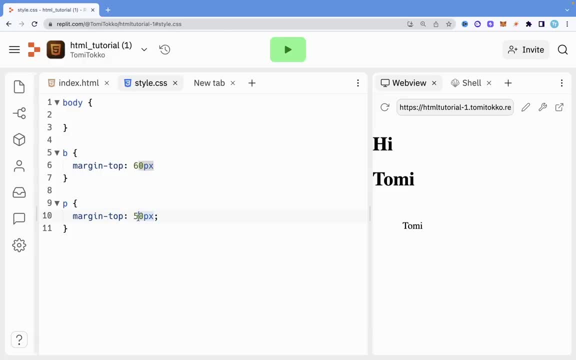 so if i want to specify margin top and i don't want to actually like start writing, i can just in input inherit and once i input inherit, it's going to have the same margin top as this b and when i say inherit, what css is going to go into, is going to go into html and it's going to look for. 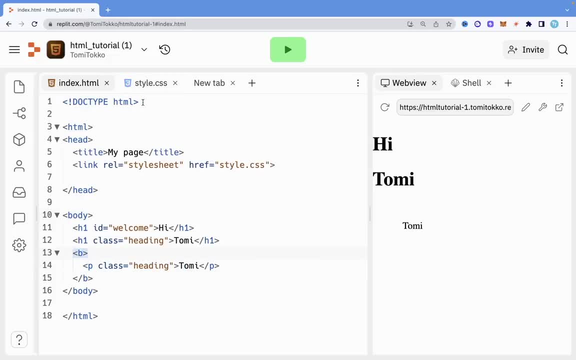 the tag that this is under. so, since it's under a b tag, it's going to come back in here and see the margin top on that b tag and it's going to do the same thing for this. now, if i run this, let's see what it gives us. 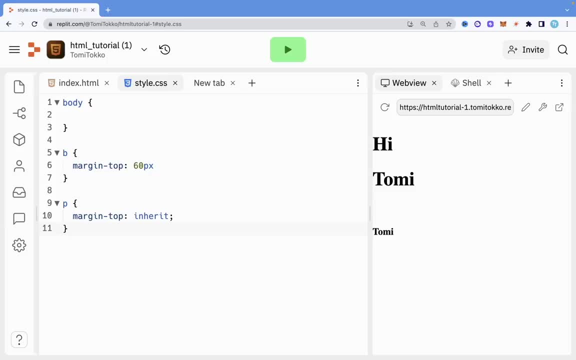 you can see that we only have a margin on the top. so that is a simple way, or basic way, of using margins in css. now we're going to talk about borders in css. now what i mean by borders is basically like a wrapper for a particular element. so, for example, if you want there to be like a 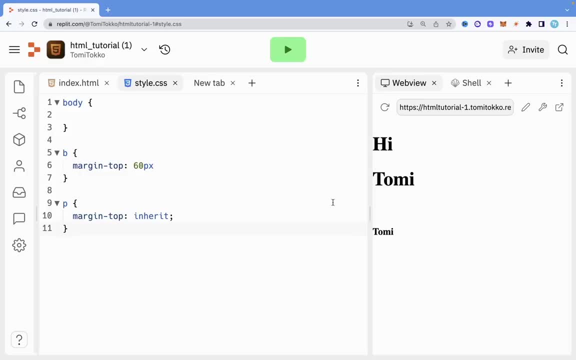 square on this element. that's when we use a border. so, without wasting any time, let me just show you how we actually use borders. so there are different styles of borders. you can have, uh, or just a simple rectangle wrapped around this, or you can make it dotted, or just dashes. i'm going to show you what we're going to do to do that. 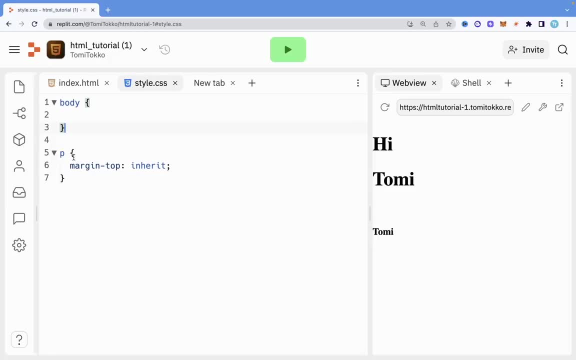 so i'm going to get rid of this b and on this p type. what i'm just going to do right now is i'm going to say i'm going to get rid of this, i don't need this, and i'm just going to say border style. 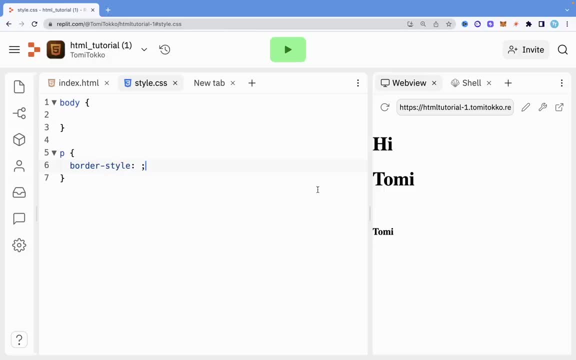 now, once i say border style, css now knows that i'm trying to put a border around this particular p tag. so now there are various styles. i'm going to talk through every single one of them. so let me first put dotted. now, once i put dotted and run it, you're going to see that there's a border around this. that. 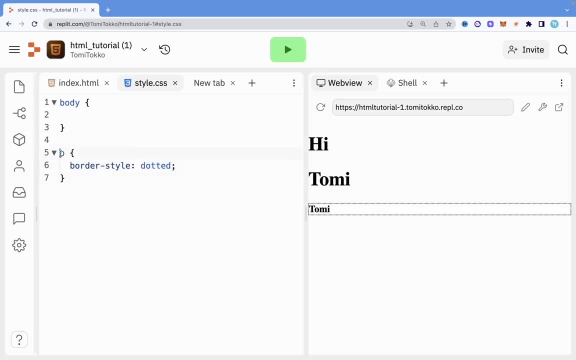 is dotted. now, that's a simple way of doing that. actually, let me just change this to the h1, just so you can see it better. so now we are talking about the h1 tags. good, so, as you can see, that is what it does. very simple. now there's a lot of different styles that we can use, and i'm going 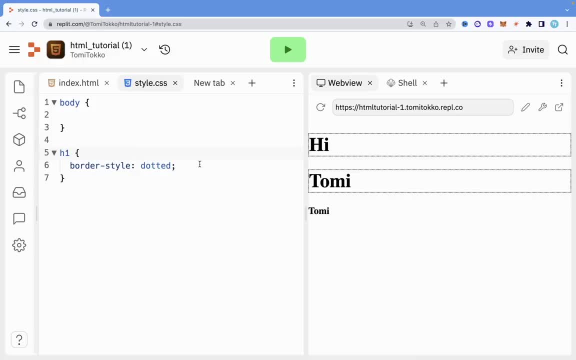 to talk about all of them right now. so the first one is dotted. there's another one named solid. so if i change this to solid and i run it, you're just going to see that it's going to have a solid border around it, a normal square. it's not dotted, it's just a normal line. so if i didn't explain, 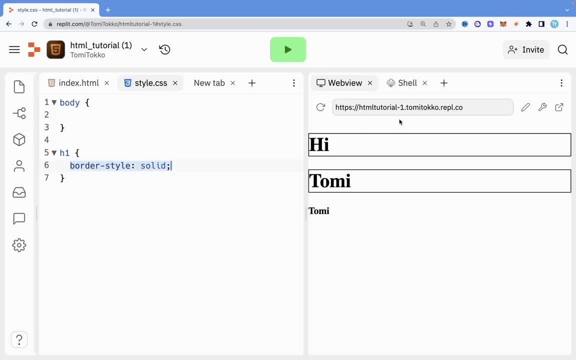 this border style. it's just a way to to actually put a border around this particular element, and then we can see that this particular style, this particular style says or asks for us to put the value of the style that we want. so, before we put dotted, now we put solid. so this is what this solid. 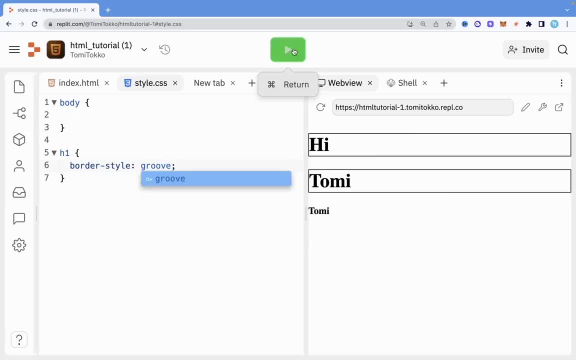 brings if i put: let's say i put there's another one named groove. once i put groove and run it, you're gonna see that it basically shows it, but like more slimmer, just a normal line, and is more fade compared to the solid. now if i put dashed, 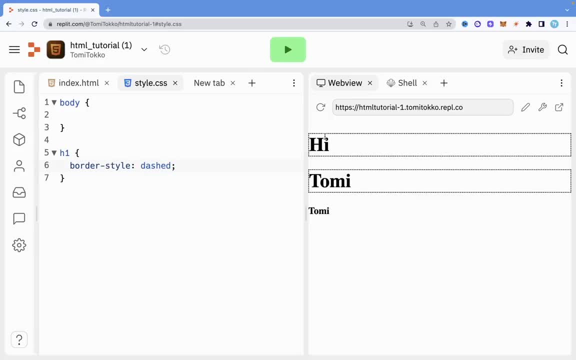 and i run dashed, you're gonna see that it's not dotted. it's like a dash dash, you know, with spacing between it, and i can also put double just going through what you can use as your border. so if i put double it's similar to groove, but let's say more thicker than that. now i can also pull. 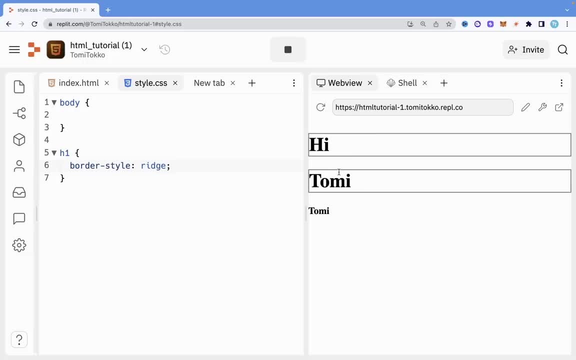 reach if i pull ridge and run it, you're gonna see. that is how that looks like. there's another one named outset, outset and inset, and once i run this outset, as you can see, it basically gives you, like this, a lighter of this particular, you know, element. and once i say: 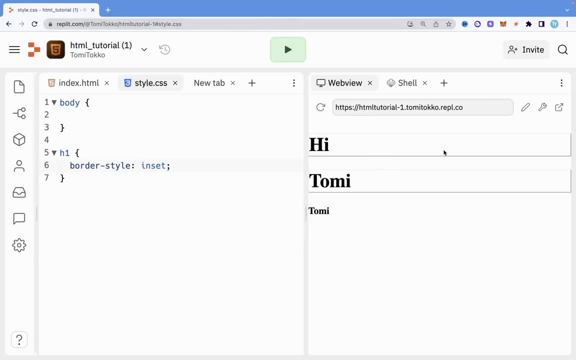 inset and i run inset, you're gonna see that it's just the opposite of that: the top are thick and the other parts are not thick. so what if let's say, you don't want to? uh, you don't want to, you want to the border. you don't actually want to have a border. that's when you just use none. 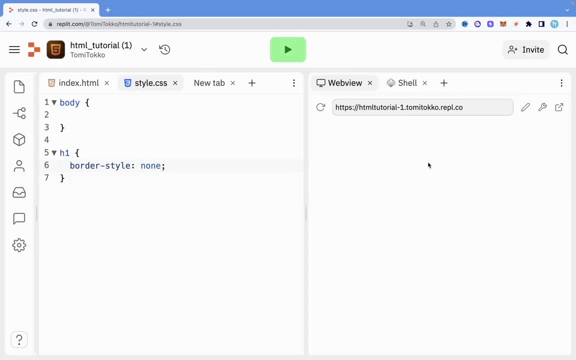 if i run none, you're not going to see any border. it's just going to be there, right? unless i want to have a border, but i don't want it to show. it's basically give you the same result as none, but this is hidden. so it basically like has a border, but it's not showing. now, once i run that, 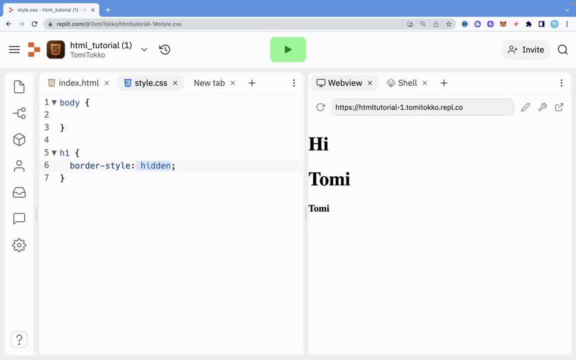 you see that nothing changes, and that's just simply because we use hidden. now let's say you want to mix different types of borders, like, let's say, you want the top to be dashed, you want the bottom border to be solid, you want this part to be double. you know, we can do that. what you just 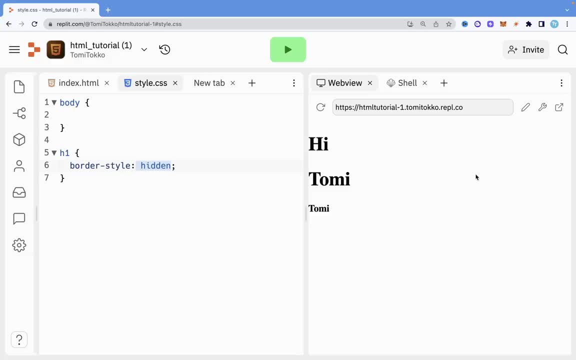 need to do is to basically specify what you want. so, for example, the right here, where we have this hidden. what you're just going to do is to say you can say dashed, double dotted and solid. now you've run this, you're going to see that each of these stands for different ones, so i'm just going to 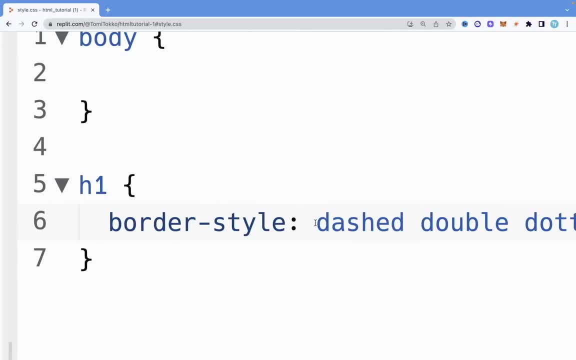 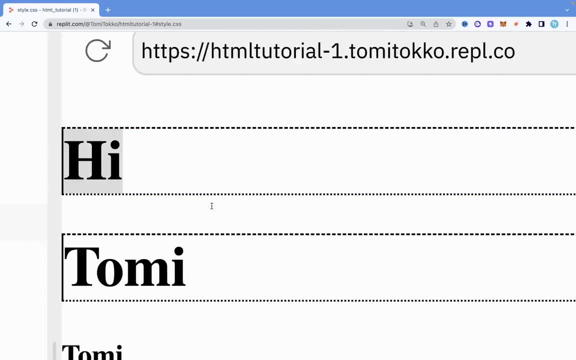 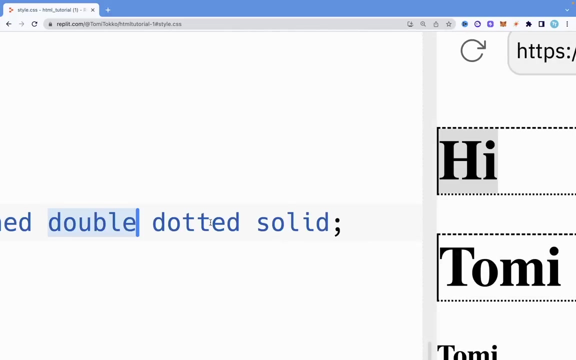 expand this right here, just so you can see it. so you can see that the first one which is dashed is right here. that's for the top, and this, uh, double, as you can see, is the one right here, double is the one right on the right, and when you say dotted, that represents the bottom, and 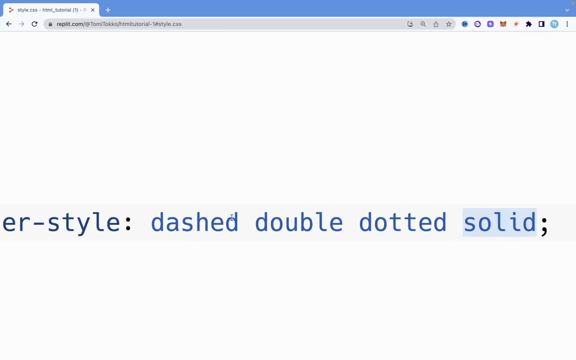 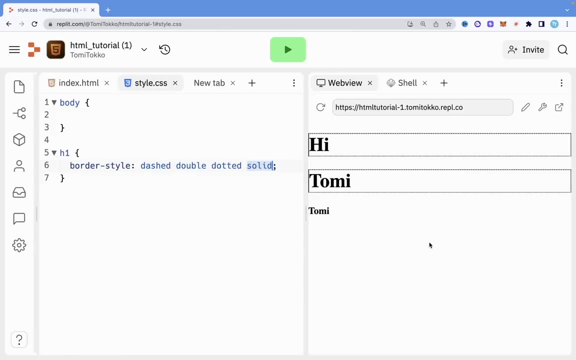 you say solid, that represents the left. so this is right, bottom left. so that's just how you can mix different ones together if you want, and once you know how to do that, that's basically the basics of actually, you know, inputting a border in uh, in css. but yeah, more to that. like what? if we actually want to be more flexible with this, what? 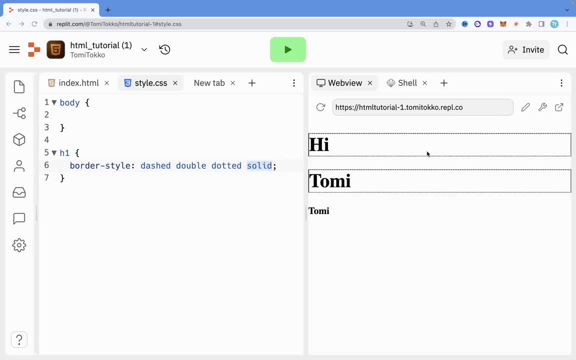 we want to be more dynamic with this, like we want this to be like our own design. so, for example, let's say we want the width of this to be larger. so first of all, let me just change all of these to solid. and now let's say i want this to have a. 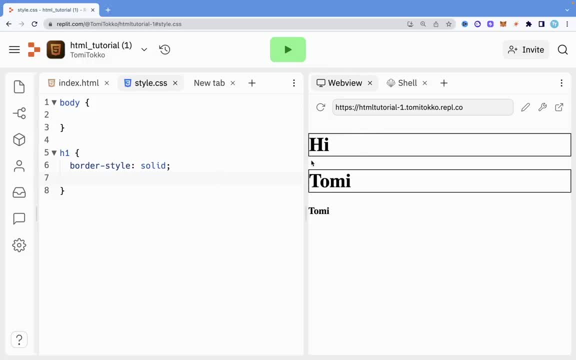 width. let me first run that so you can see the output of that. and let's say: i want this to be quite bigger, like i don't want it to be this small. i can say border hyphen width and i can say 10px. if i run that, you're gonna see that this is quite thicker. i can change that to, let's say, 6px. 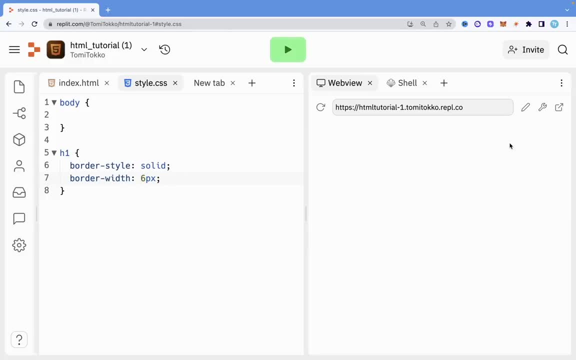 just to reduce the thickness. as you can see, it is less thicker. so that is one way of giving a value to the width. there are other ways we can also give values. just the way when we were dealing with margins, we could give value with six, with numbers. we could also give value with inerrity. 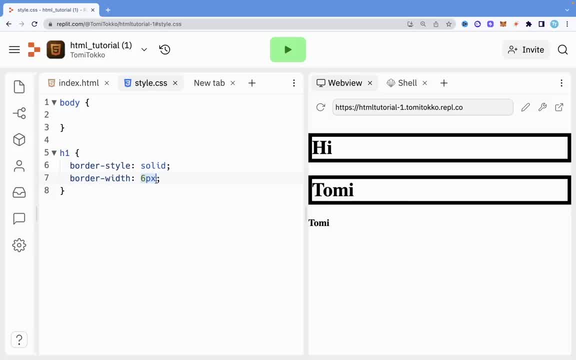 and all of that, but in this one we can give value to the width of the width, of the width of the width, give values with the x And we can also give values with. you know the rate, like, for example, I can say medium. Now, if I say medium, this means is going to be thick meat, you know. 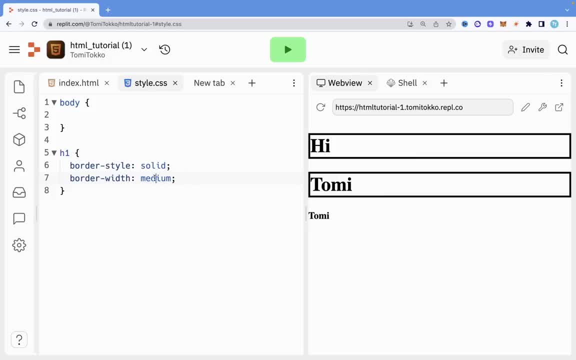 medium, And we can just also say thick. if I say thick, it's just going to be very thick, That's what it is. So you can use that to basically specify the- you know the width of the border that you want. It's very easy. But what if we want to actually just specify? 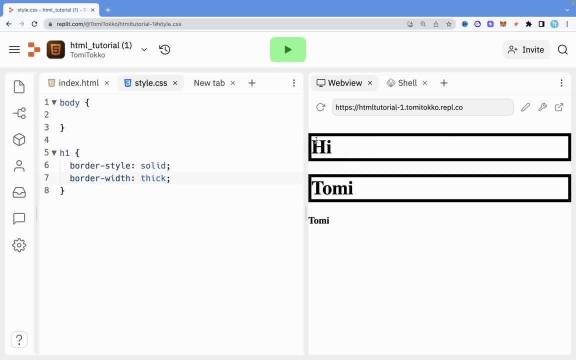 different side widths. like, let's say, we just want only this part to be five px. they may want this part to be, you know, 10 px. they want this part to be 11 px. we can do that And the first thing you need to do just the way we could mix different styles. we can. 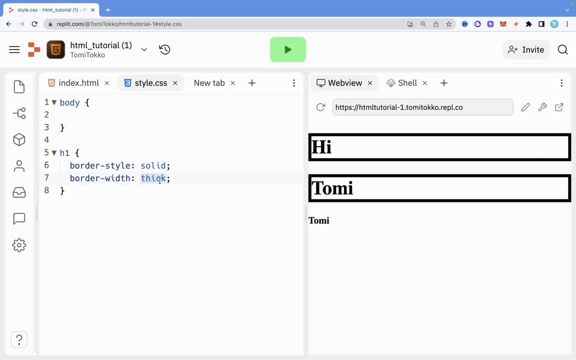 also mix different width. So what we're going to do is we're going to specify for the top. we can see the top should have 10 px. And then we're going to specify for the right. we can see the right should have five px. are going to specify for the bottom. 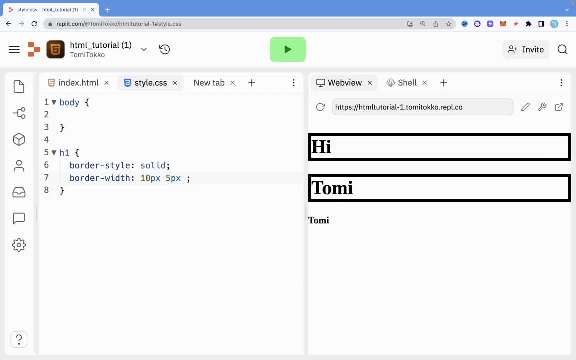 part and say the bottom part should have, let's say, 11 px, And then for the left part we can say: each you have 22 px. Now, if I run this, you're just going to see that is a mixture of different width in the borderlines. So that is how to do that. But you can also split. 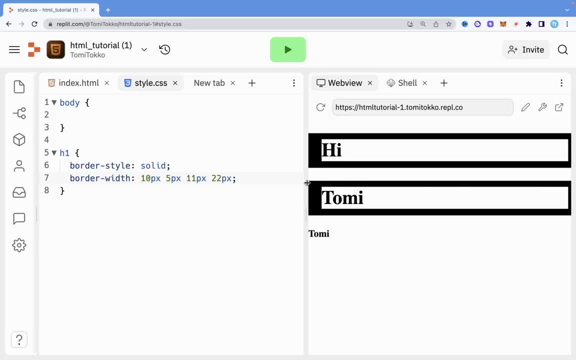 it evenly. So, for example, you can imagine, I have just two different- you know- px, two different sizes put here. what this is going to do is that it's going to take this 10 px and input it for the top and the bottom, And it's going 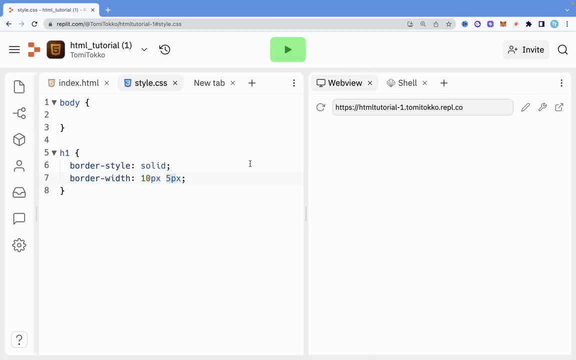 to take it five px and input it for the left and right. it's going to split it evenly, So, as you can see left and right as five px, top and bottom as 10 px, And that is a very simple and basic way of doing that. Now, after specifying the width of what we want, we can 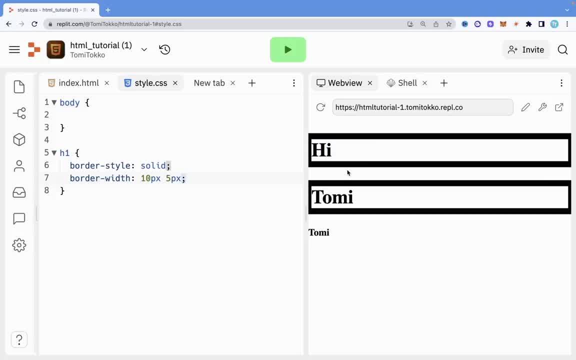 also add the color. Let's say: we don't want this to be black, we want this to be, you know, you know- green. we want this to be purple. What you just need to do, as you might have guessed, is to say border color. And once you say border color, you can just directly give. 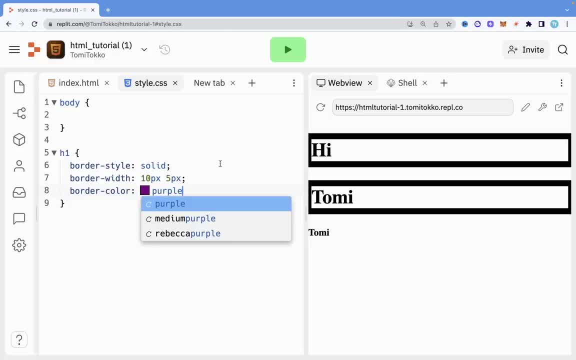 it the color that you want. You can just say purple And once we say purple, we put a semicolon. If we run that, you can now see that it has purple. Now, once again, we can have a mixture of colors. like we can want the top to be green, we can want this part to be purple, we can 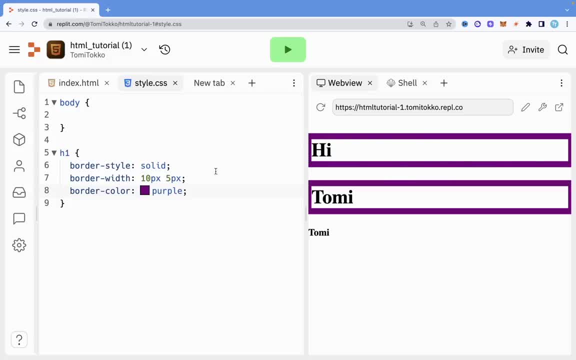 want this part to be violet. We can want this part to be black. Now, we're going to do that right now. So we're going to say the top part should be purple And let's say the right part should be blue. right, 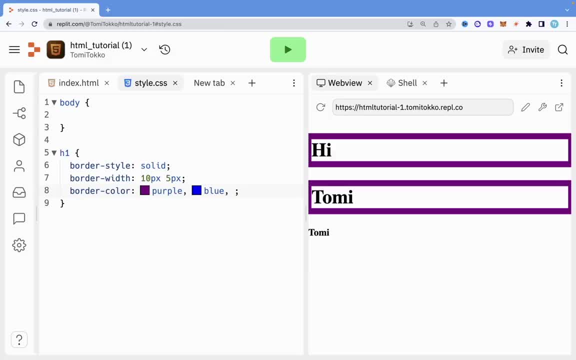 side, And then we're going to say the bottom side is going to be, let's say, green, And let's say the left part should be red. If I run this, you're going to see the each should have a mixture of different colors, though. 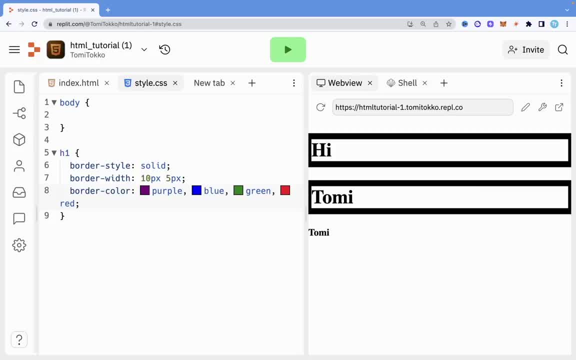 Okay. The reason why that gave us an error is because there shouldn't be comma in there. So what you just need to do is, when you're specifying different values, you don't actually use a comma I'm going to remove. get rid of this comma. Get rid of that. Get rid of that Once. 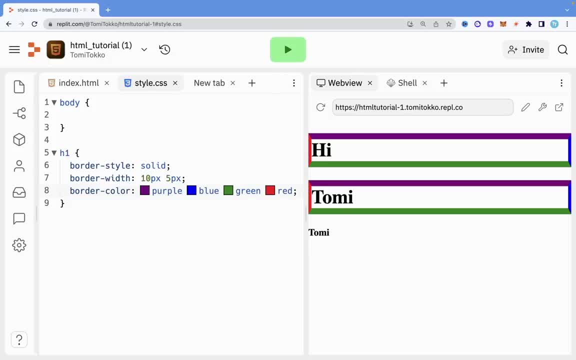 I run this. you're going to see that there's a mixture of colors, As you can see all the borders as different colors within them. So you can see that that is also, you know, very easy to do. So, instead of also just having, like this style for everything to be solid, we can basically 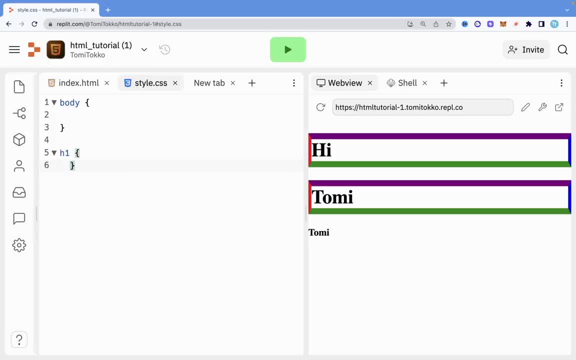 I'm going to remove all of these. or we can just say something to style like only the top right. So for example, I can say I want border, I think top I've installed. So for this you know. instead of saying you know before, we basically compress everything into a box. 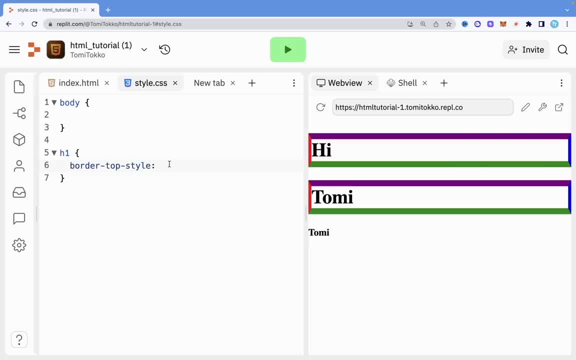 we basically compress everything into a box And that's basically what we're going to do. I'm going to do that. So, instead of saying you know before, we basically compress everything into one. when we say border style, and we could say dash, we could say you know solid, we could 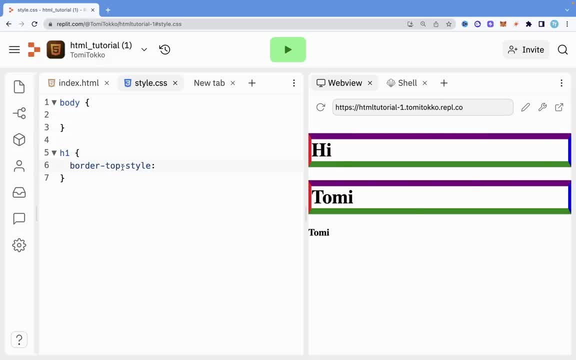 say dotted and everything is just going to be split. but let's say you just want to have each of them differently. you can say this should be dashed and brother, i think you know you can say right style. you can say dotted. you can also say border hyphen, bottom style. 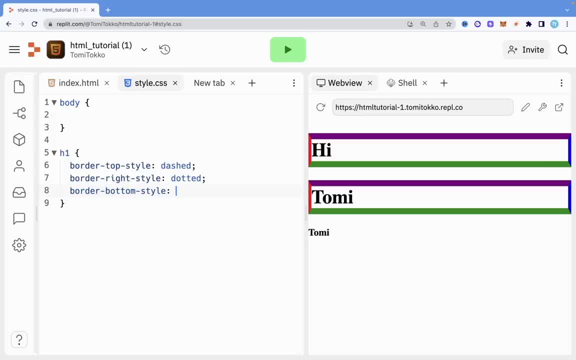 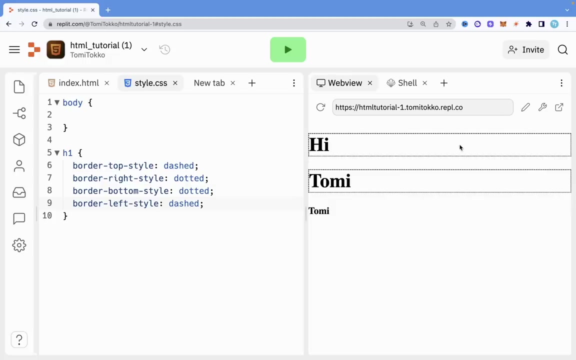 now you can just say: you know you can give it the same thing. let's say dotted also. and let's say border hyphen left style. we can just say dashed. now, if i run this, you're gonna see that it's basically gonna have different. you know ones like this is dash and this is dotted. this is dashed and this is dotted. so this: 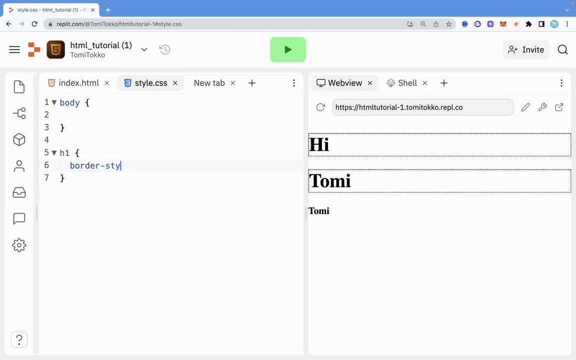 is a long way of doing it, but the way i said already, when we did style like this and then we specified different ways by saying let's say dashed, and then we can just say dotted, you know. so this is, you know, for the top two, the top and bottom, and this is for the top two. 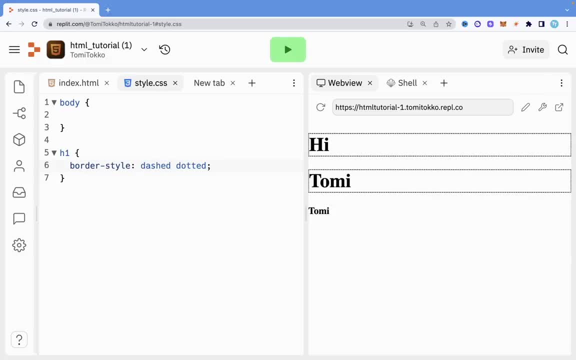 and then we can add theDessentialStyle Christianity engines and then we could just the left and right. so this is the shorter way of doing it, like see how compressed that is now. so i also highly suggest that you do that instead of actually going to do every single thing you know. 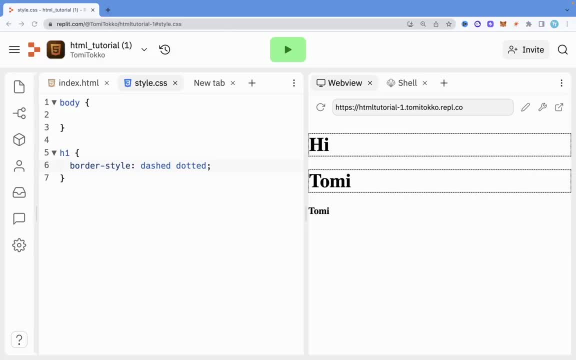 one after the other, so that is also a good one. so, for example: so let's say you want to have a border, but you don't want the border to be a square. you might just want it to have a border on the left or on the bottom, on the top. now what you can just do, very simple and straightforward. 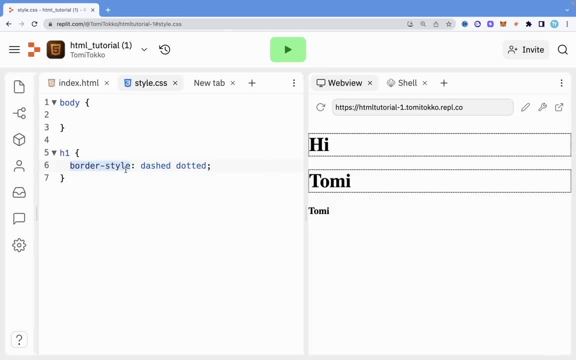 you can just say border for that bottom and let's say dashed. now, once you run dashed, you're just going to have a border on the bottom and it's going to have dashed. we can change this to border left and it's just going to have a dashed border on the left, like this. good, now you know when we specify. 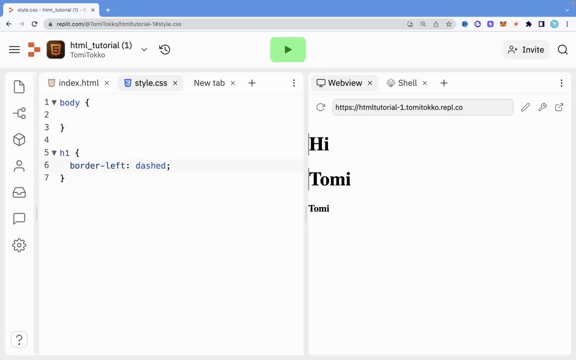 the border button. i mean when we specify the border style, the color, you know, the size and all of that. we can just do everything at once, like where i have border left. instead of saying border left, then i'm now going to say border colored and border width. what i can just do is 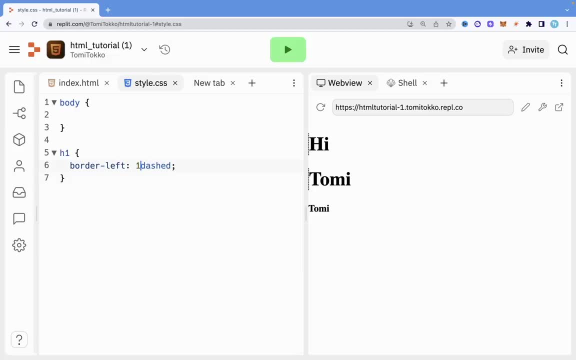 to first say the width, so i can say the width should be 10 px. then i'm going to say the style and then i'm going to say the color. let's say purple. now what this does is that it allows us to just comp, compress, every, all those code we're going to write into one line. so, instead of writing 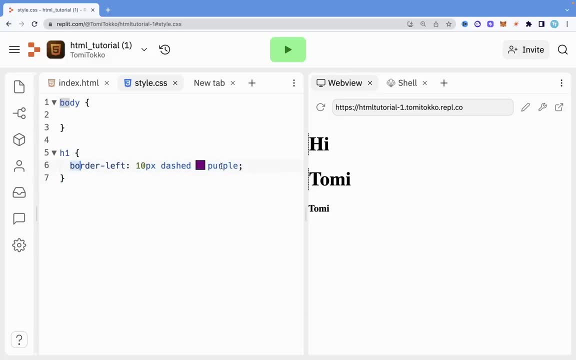 border width. to have the width, we can just have it here and instead of writing border color, we can just have it here. if i run this, you're going to see now that we have a left- you know- border of all of this. so if i don't want this to just be left, i can just remove this, you know. 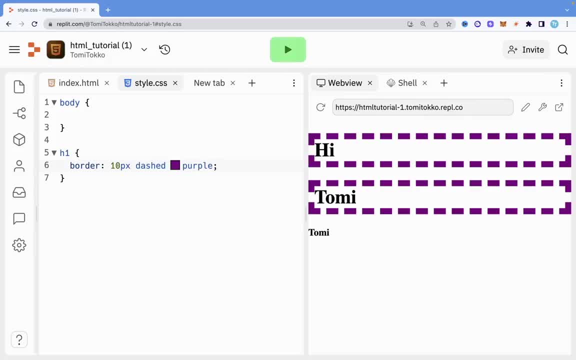 and now the old border is going to have all of this, so that is very easy and straightforward. now the last thing we're going to talk about is putting rounded borders. so let me change this back to solid. and when i change this to solid, let's see. 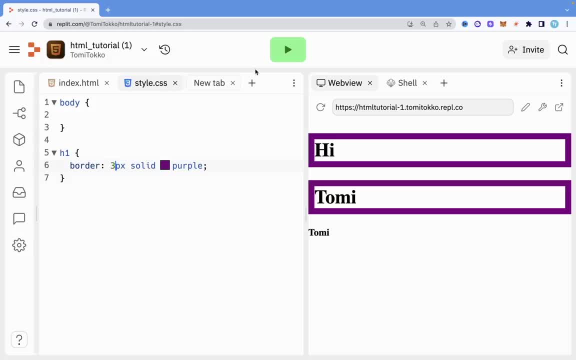 cool now let me change this to something like three. just want it to be smaller. cool now. what i want to do is to make this border rounded. so if you look into this particular repeat page, you can see that this basically has a border that is rounded, or, as you can see, on these edges they are not squared like the way this border is squared. 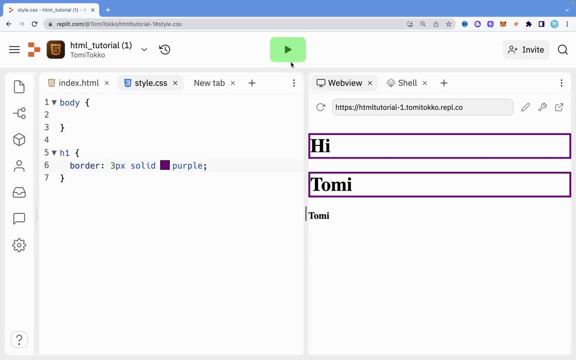 these edges are actually curved, so that is a rounded border. i'm going to show you how to do that on these edges very straightforward. what you just need to do is to say border hyphen radius. so now you're going to specify, or, you know, write, how curved you want it to be. so let's go with 4px. 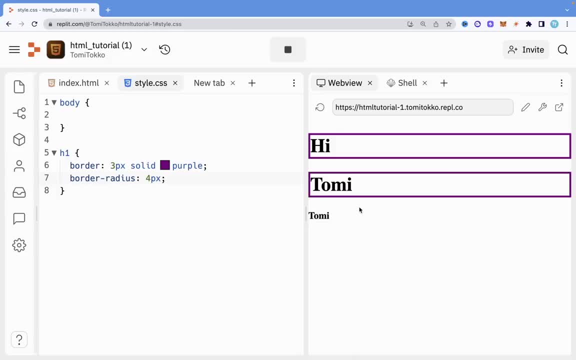 so let's go with 4px. we want it to be that curve and i run it. you're going to see that it is curved for px, let's say 10 px. it's going to be very curved, as you can see. it is very curved, so the more you increase it. 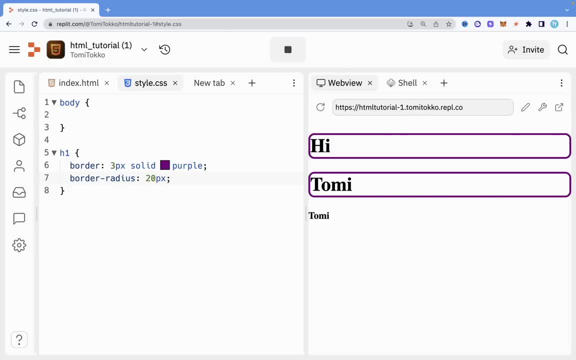 the more it curves. if i run it as 20 px now, you can see that is more curved. so that's basically how to do that and i hope you understand everything now about borders in css. now let's talk about css padding. so padding is used to create like a space around an element or 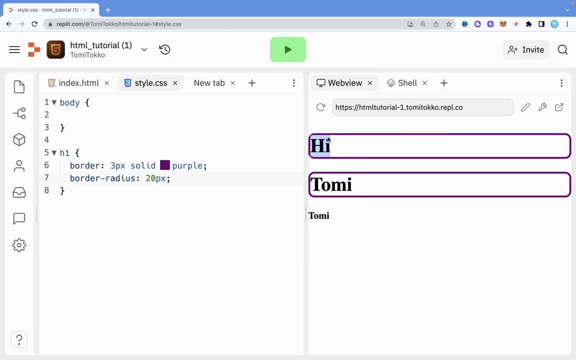 text inside any border. so, for example, let's say we have this eye right here and let's say we want to create a space, like we want there to be more spacing on top here and below here and also on the left. that's when we use padding. so for us to use padding is very easy. for example, we already 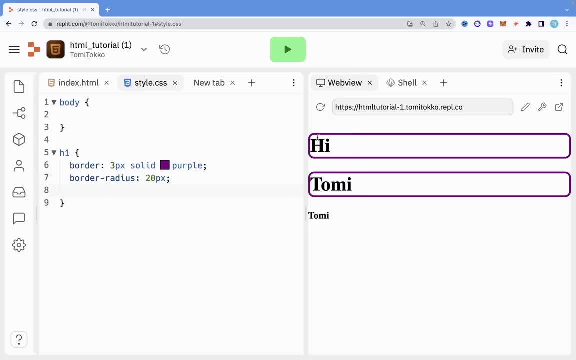 have this border right here. now. let's say we want there to be space on the top. what you just need to do is to say padding- i've been top that easy and now we're going to specify how much we want the space to be. you can say 40px and then once we run this, you're not going to see that there's. 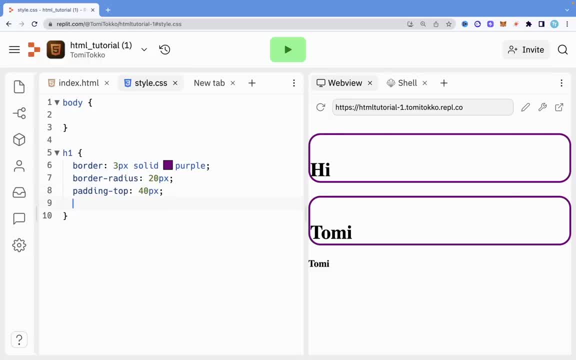 going to be a space on the top of 40px. we can do the same thing by saying padding left and let's just say 40px. once you do that, there's going to be a space of 40px on the left and then you can also say padding. you can say bottom. 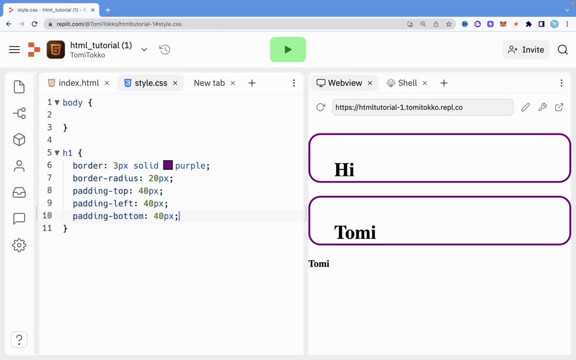 and then there's also going to be a space of 40px on the bottom. so, as you can see, that works and you can also do the same thing. you know, for the right side you can just change this bottom right here to right, but when you run that, 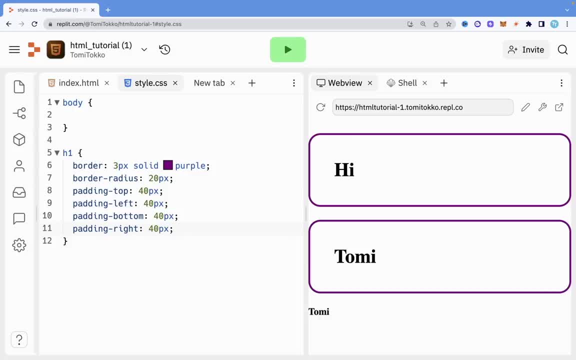 doesn't really make any difference because there's already a lot of space here. now, instead of having to write all of this. you know top, left, bottom right- you might have guessed just the way we did everything for border and for margins. when we are doing margins, you can just say padding and then we can just specify. let's say, 40 e x 10 px. 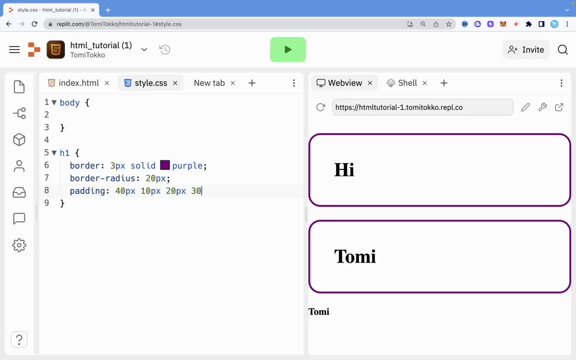 20 px and 30 px. so once you say all of that, this is basically: the 40 px is for the top, the right is for 10 px and 20 px is for the bottom and 30 px is for the left. now, if i run this, you're going to see that that is going to work perfectly. 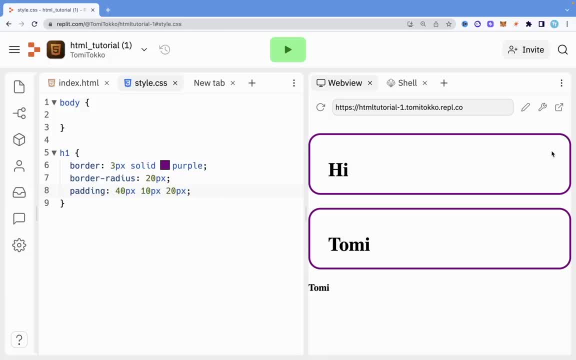 now you can also do the same thing by, you know, removing one. when you remove one, this just simply means the top, the right and the bottom. now, if i remove the second one, what this is going to do is going to split it evenly, so 40 is going to go to the top and the bottom, and 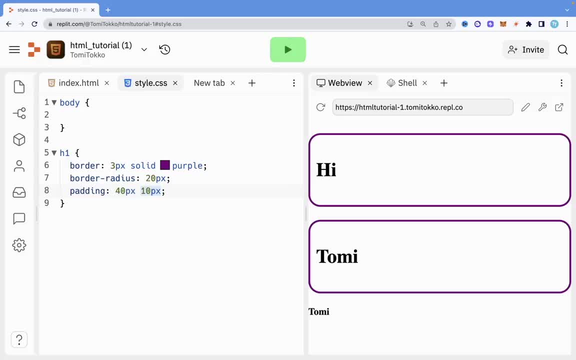 this is going to go to the left and the right. if i run that, you're going to see what that does. so that works successfully. now let's say i just have 40 in here and i run this. what this is going to do is that it's going to let the left have a padding of 40. 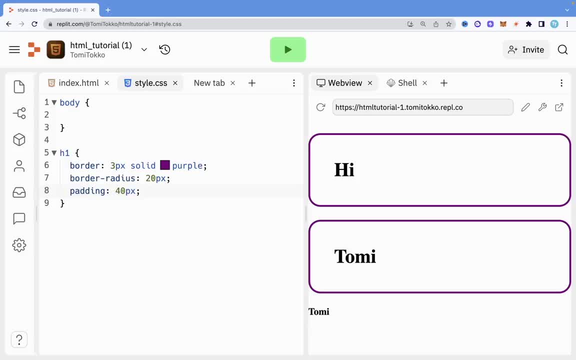 top 40, bottom 40 and right 40.. so just the way we've been doing, for you know, border for margins. that's the exact same thing that happens here. so i hope you understand what is padding and why we even use padding. now let's talk about height and width in css. now, the item which is 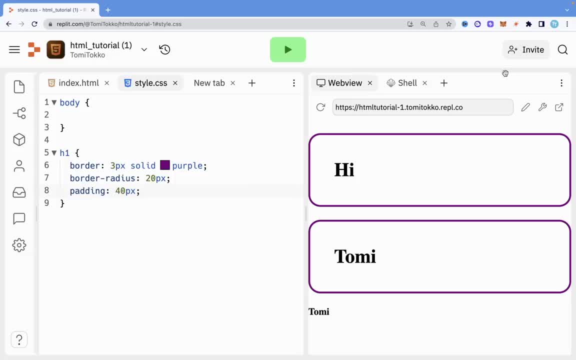 just used to set the item width of a particular element. so let's get rid of this, all the borders, and let's just run this normally. so let's say we want this eye to have like a, not the actual element, but you know, around the element, the space around the element, to have a i 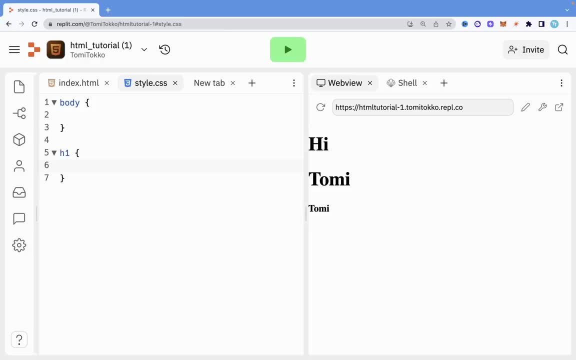 it of. you know, let's say 60 px, what you need to do is just to come into h1 and say height. you can say i and say 60 px, but once you say that and you run it right, obviously you might not see any change. okay, you can see a change now. this is the reason why we see a change is because 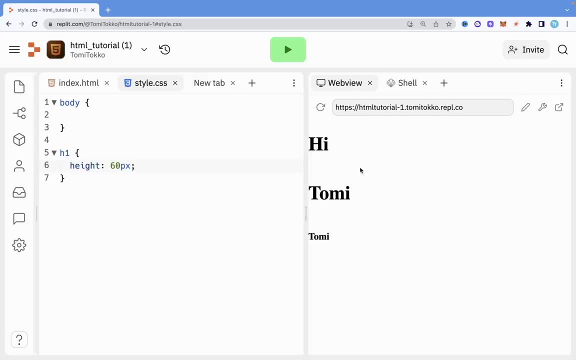 there is now an height of 60 px around this, so this starts from after that. that's how you can see base in these two. so for us to actually see it visibly more, let's set a background color. so when we have a background color of purple, 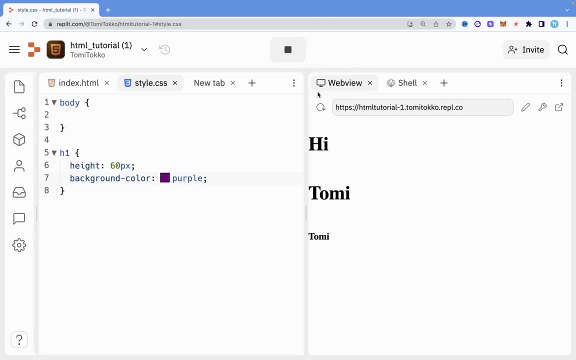 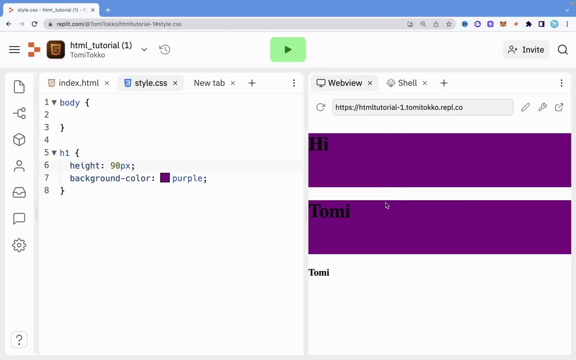 and i run it. you can see where is it. this has a background color of purple. now the height of this is 60 px. i can change this to 90 px and when i change this to 90 px, you can see that it now has a bigger height. so this height is basically the height of you know. 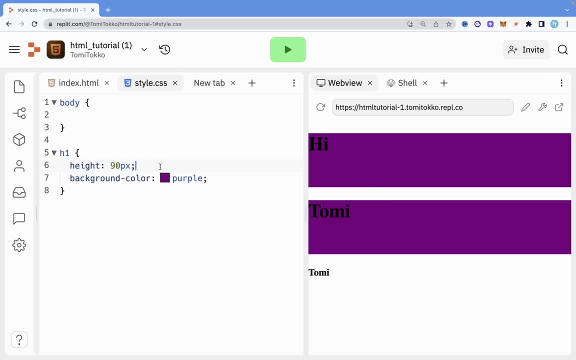 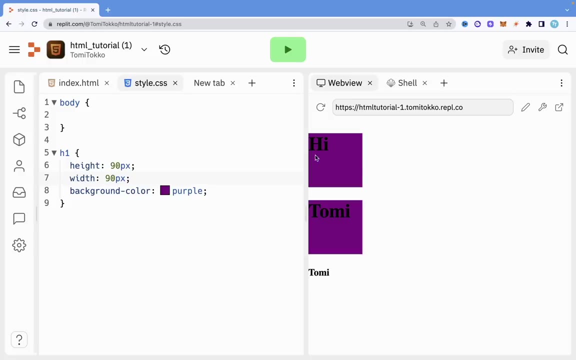 everything around that particular element. now we can also change the width. and let's say, i want the width to also be 90 px. now, if this width is 90 px and we run it, you're gonna see that the width was reduced drastically. but let's say, i just want this width to go all the way from the. 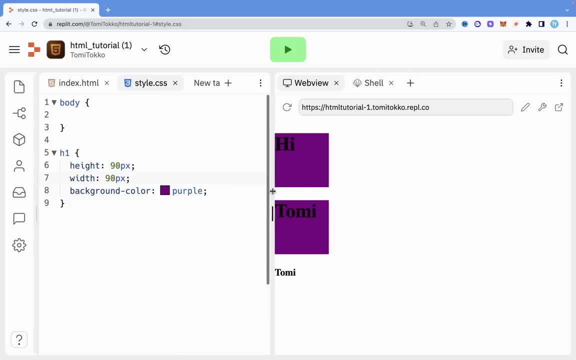 beginning right from here to the end of the page. for me to actually get the end of the page, because obviously i i might not know how large any body screen is, so like for this screen i don't know if the end of the page is 200px, even if it's 200px for another. 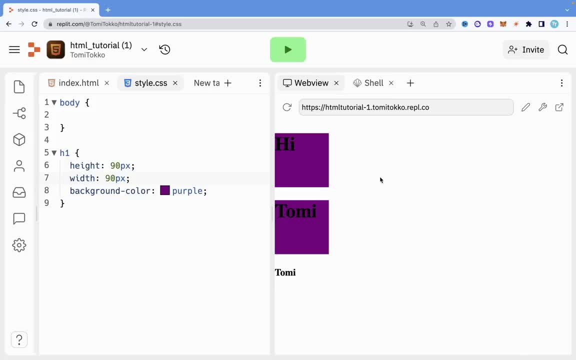 screen it might be 500px. so for me to get rid of that problem and let it just be all the way to the end of the screen, what i just need to do is to use percentage. so when i use 100 percentage on represent, it's not going to be calculating it based on pixels or px. what it's going to. 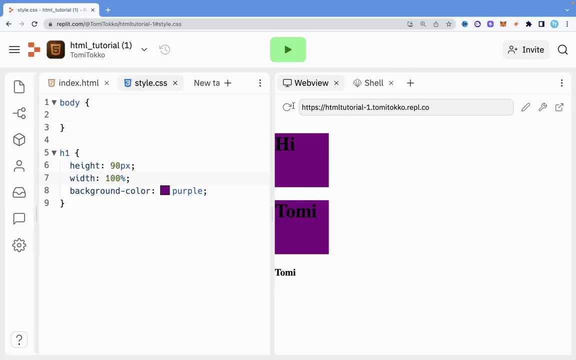 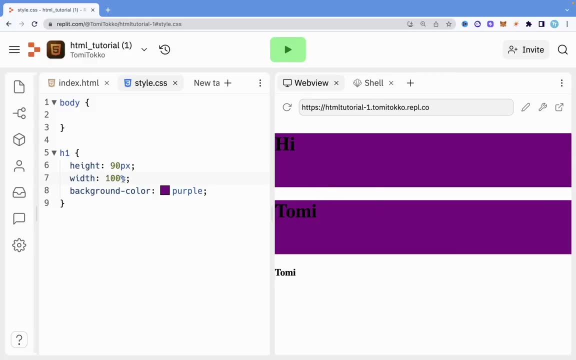 calculate it based on is the percentage of that screen. so now, once i run it, you're going to see that the width goes all the way to the end of the screen, so it calculates the 100 of that screen. if i change this to 50 of that screen, then you're going to see that it only stops at half. 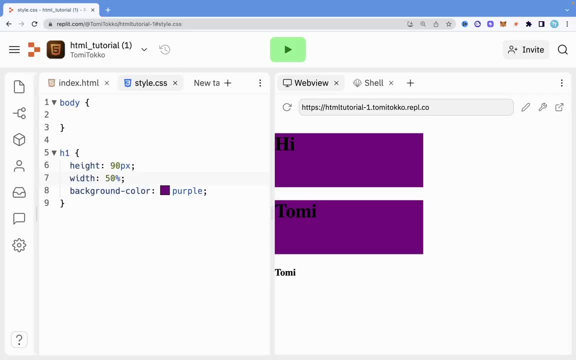 of that screen right here. so that is a basic, you know thing about height and width. now there's also something called max width and the max width is just used to set the maximum weight of an element. it's that easy. so what you can just do now is: right here i can just say max. 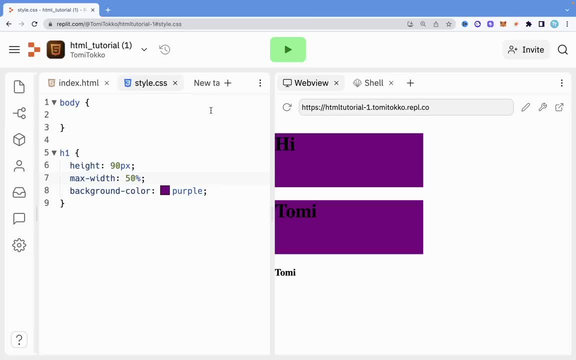 i think with if i say max width and i run this, it basically just set the maximum width of that element. it doesn't really make any change. that is noticeable. but now we know that the maximum width that that element can have is 50 of the screen. now we are going to talk about outlines in css. 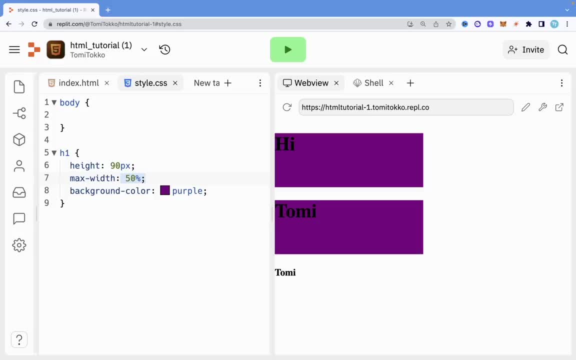 so what outline does is that it draws a line outside the border in an element. so, for example, we have this border in this element, right? if we add an outline to it, it basically just draws a line outside the border of the screen. so if we add an outline to it, it basically just draws a line outside. 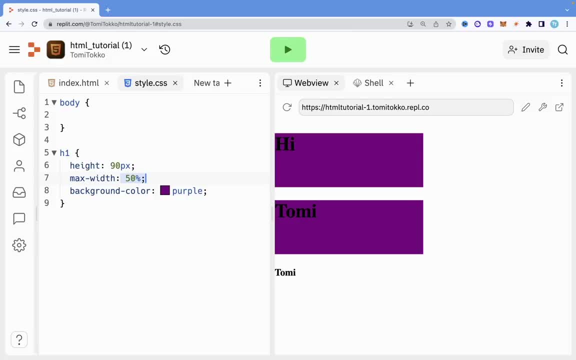 that particular border and what it does is just it. it just makes that element stand out. that's basically the main reason of an outline. so very, very similar to how we define, uh, borders, that's how we also define outlines. so let's say we have this border right here. actually we don't have a. 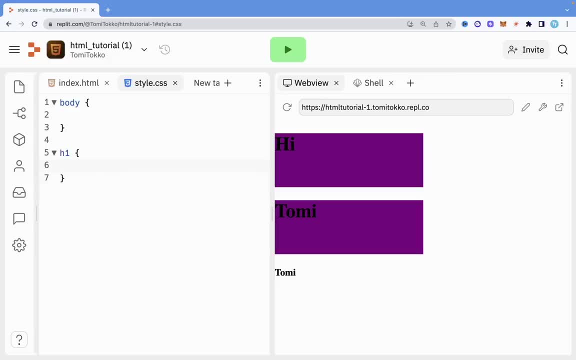 border. this is just a normal background color stuff. we can just get rid of this and i can say outline style. so when i say outline style, just the way we say border style, that's how we say outline style and i just want it to be normal solid. now, if i run this, you're just gonna see that it has a basic 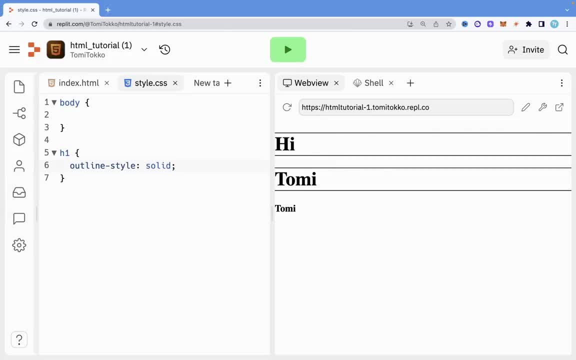 you know outline of solid. so it's very basic. you can change this to dashed. once i run this it's gonna be dashed, you know. you can change it to basically whatever you want to change it to. so that is the basic. you know concept of outlines. it's very easy. we don't need to, you know. 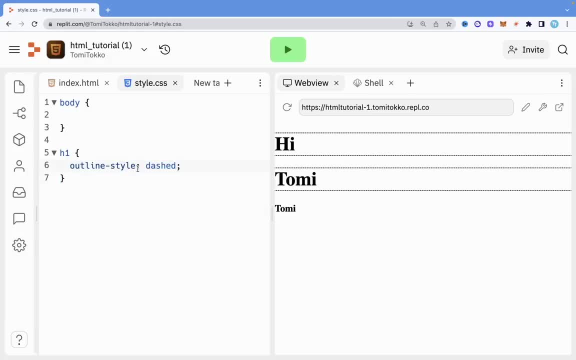 you don't need to have to put a border or whatever. you can use an outline or a border, or you can even use both. For example, let's say we have border right here. we can say border. And let's say we just say it's two px, we can say it is, let's say, dashed. 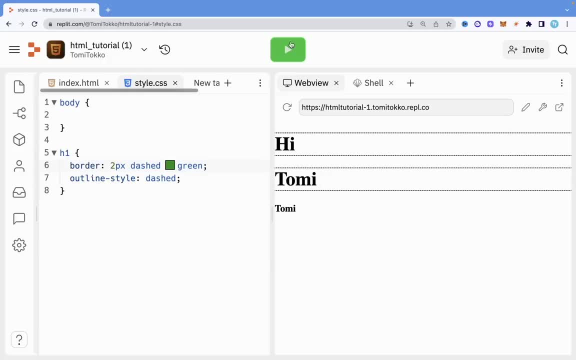 and we can say it is green. So if I run this, you're going to see that we have our border normally, but then we have an outline after it. let me change this to solid instead of dashed, So you can see that we have. let me just make this a little big. you can see that we have this dash. 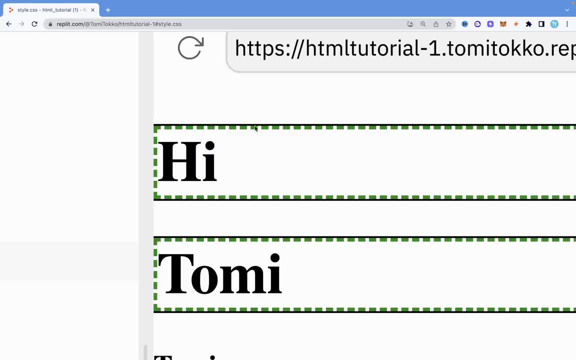 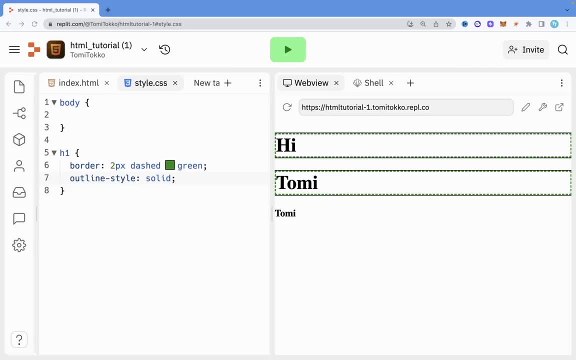 right here this dash border, but outside that we have this outline. So that's what an outline does: it just makes the element stand out or it wraps around the particular element. So it's very easy and, you know, very straightforward. But you can also do something. 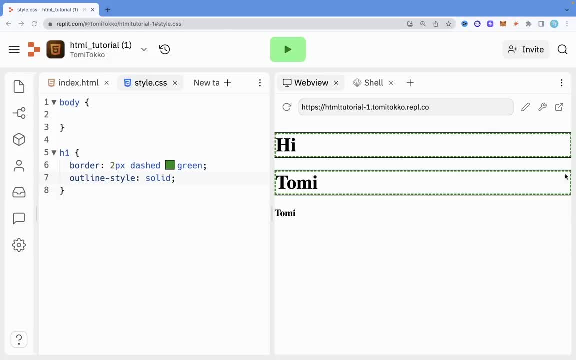 something to get a space between the outline and the border, And that is called the outline offset. So what you just need to do is to come here and say outline, I think offset. So once you have an outline offset, let's say 10 px. 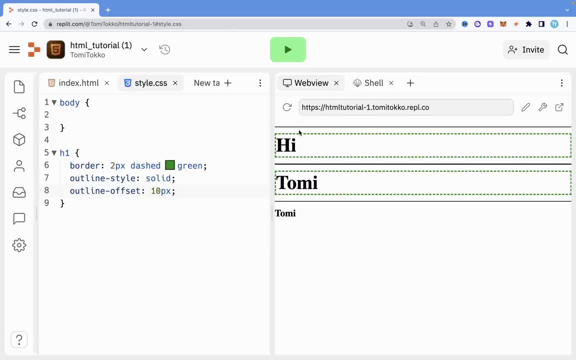 That means we want a space of 10 px between the outline and the border. So that is what it just does, right here. This is the outline And this is the border. There's a space of 10 px. So that's how straightforward outlines is. very easy, Okay. 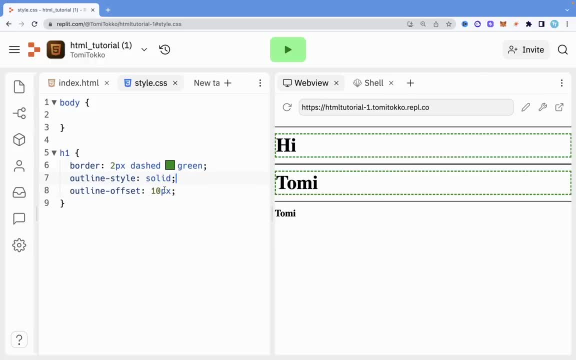 so this is the how we basically define outlines in CSS. Now we're going to be diving deeper into texts in CSS, So I'm going to show you everything you need to know on styling texts in CSS. I'm going to get rid of all of this real quick. Let me just run. 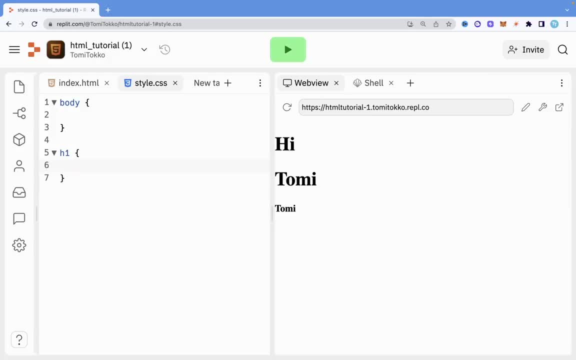 that again. What we're going to do first of all is to talk about how to style the colors of a text. So if you select an element and in that element you declare a color and give it a value of, let's say, blue, 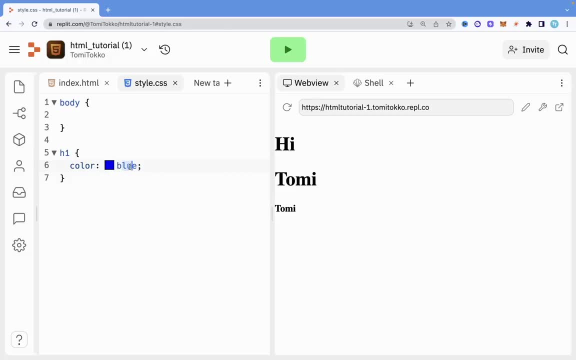 that is going to give the value, the color of blue, to all the text in that element. So that is the easy way of changing a text in an element. Now, we've talked about this. you know previously a lot And this is just emphasizing on that. So whenever you just say: 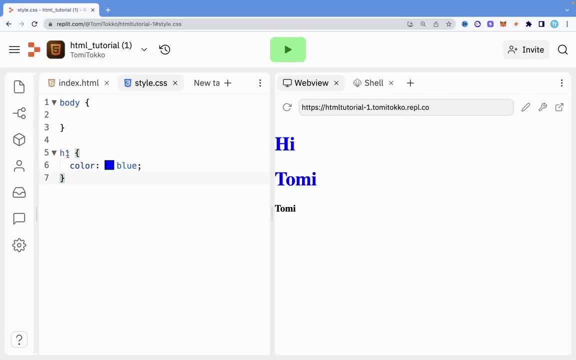 color and you give it a value, it's going to look for all the text in that particular element and change it to blue. Now you can also, you know, talk about the background color of a property, But that's basically the background color of that text, but not of the text actually that. we've also done this. you can. 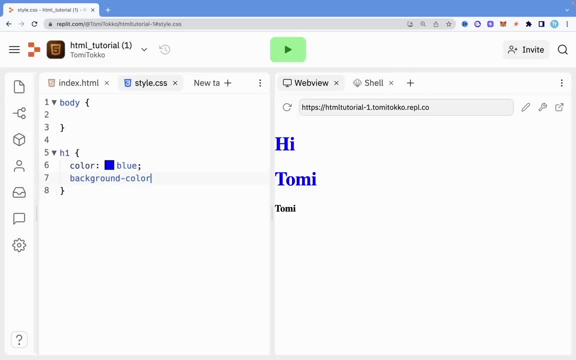 just say background, I think color. And then, when you say background, I think color, you can just simply say: you know red and it's going to give it a background color of red. Good, That is easy and straightforward. Now the next thing I'm going to talk about is alignment. So I'm 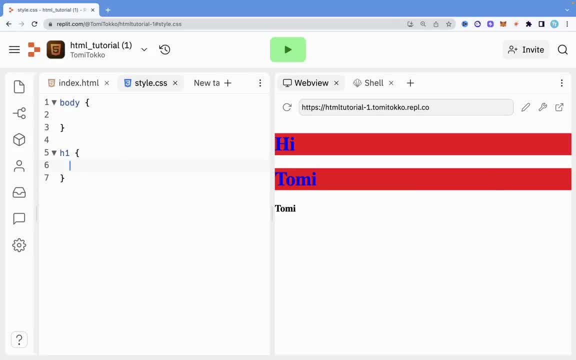 going to get rid of all these colors. don't really want to talk about the colors again Now. what I want to talk about is the alignment. So what I mean by the alignment is to show how aligned the text is. So, for example, if I want this text to be in the center or instead of being at the left, 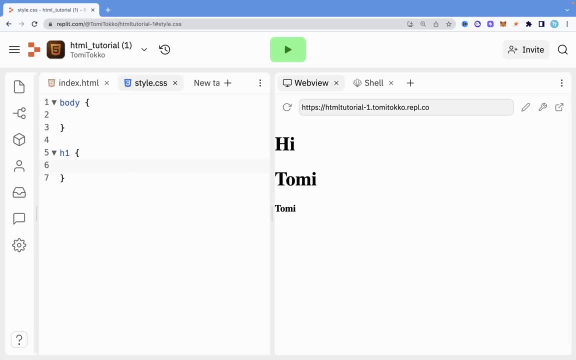 I want it to be on the right. That's when I use text alignment. So for me to align a text, what I need to do is to come into the text element that contains that text, And what I'm just going to do is to say text hyphen align. 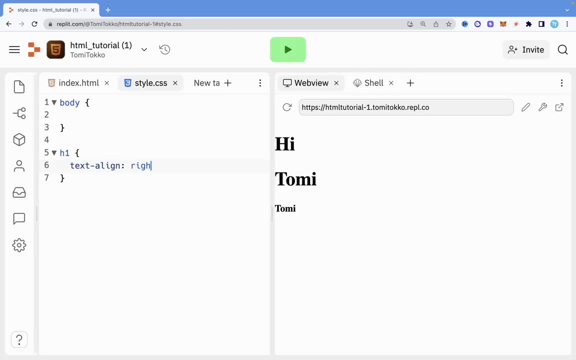 Once I do align, I can say right. I can specify three different things: left, center and right. If I say right, you're going to see that all the h1 tags, the text in them, goes to the right. If I say center, 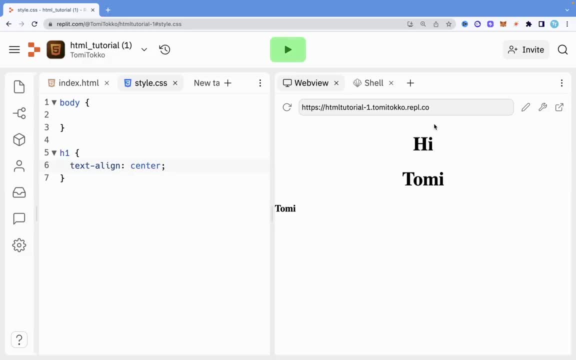 you're going to see that they automatically align at the center right. here I can say left, but that is just going to be default. So as a default, if you don't give it a text alignment, it's just going to be at the left. So if you also align it to left, 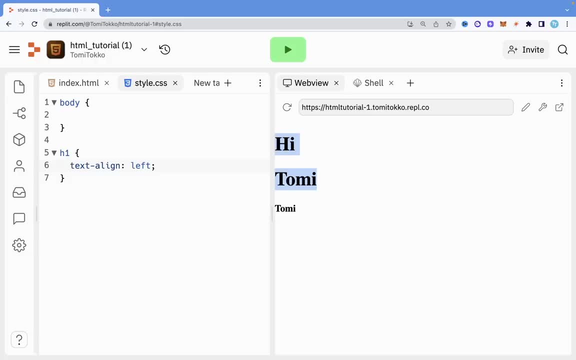 it's just going to be right there where you want it. Now, if I say justify, let me change this to justify And I run this Now, when you run it with justify, it doesn't really make any change. But if I come in here and let's say I change this, 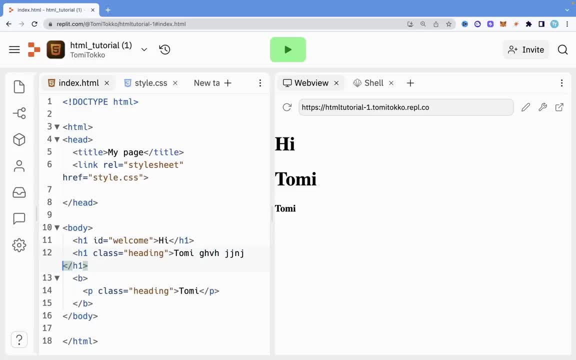 to random Text And I run this. So what justify does is that justify basically stretches out each line so that every, every line has like equal width and length. So what this means is that if we have- let's say we have- a full text here, and then we come in here and we say text align should be justified. What this is means. 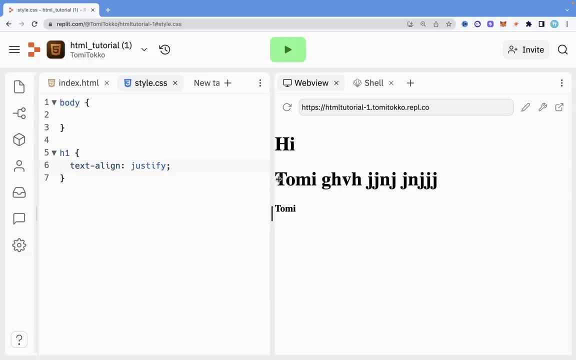 that it basically makes sure that this particular text wraps around the whole length of the screen. That is what justify does very easy. And after talking about justify, the next thing I'm going to talk about is text align last. Now, what text align last does? I'm going to change this to hyphen last. 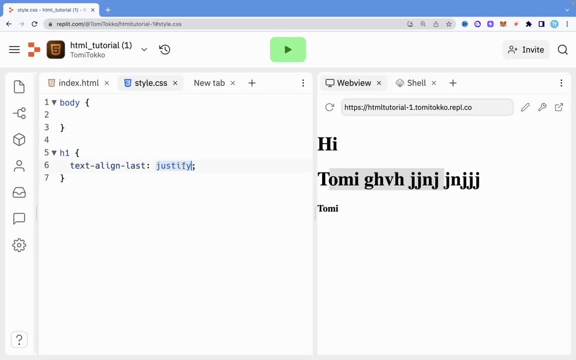 What text align last does is that it basically aligns the last line of the text. So, for example, if I say center, right. So if I say center and then I try to run this, you can see that it aligns that because this is the last line of the text. That is why it aligns. 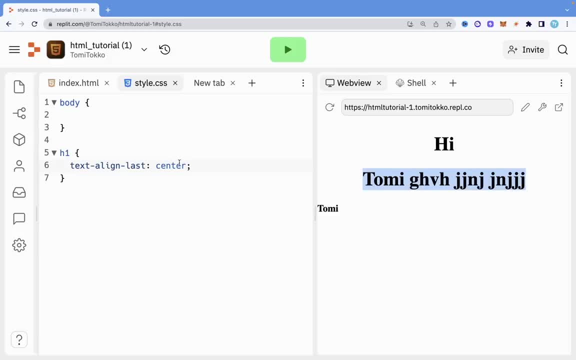 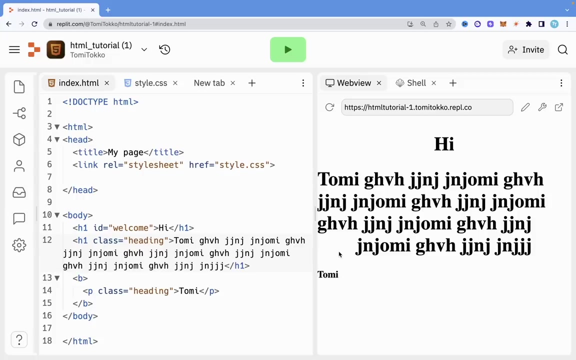 this at, you know, the at the center. So, for example, let's say I just have, let me just copy this And just keep going like that and I run it. So you're going to see that all of these from the left, but only the last line aligns at the center. so that is what test align center does. 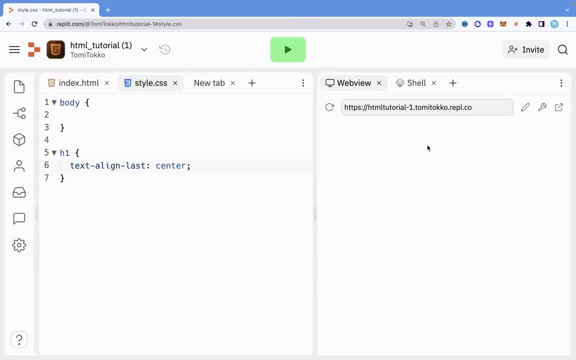 i'm just going to remove all this and put it back. the reason why this also that eye also aligns at the center- is because it is also the last line, even if it's also the first line. so that is what the test align last does. you can make it right, you can make it left, you can make it whatever you want. 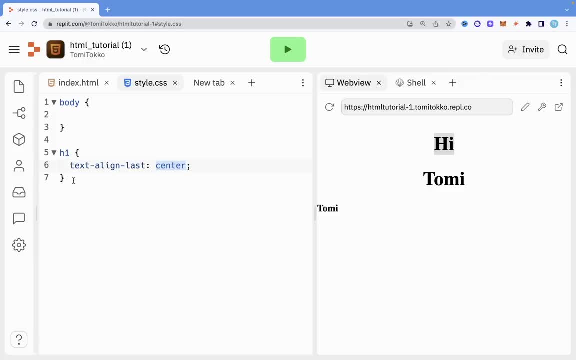 so i'm also going to talk about vertical align. so when i say vertical align, i'm going to change this to vertical, i think align. so when i say vertical align, what that does is that it basically aligns that vertically. so, for example, let's say that we have 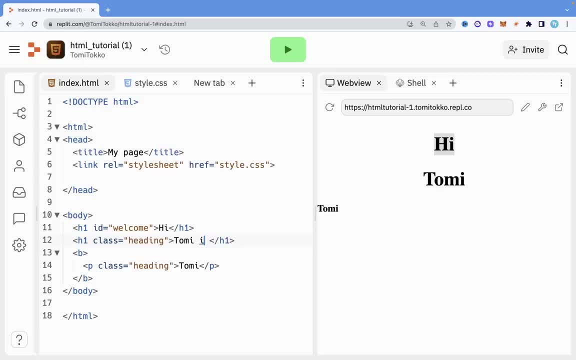 this is tommy is a guy, and let's say that this guy has a p tag. oh, now let's make it a b tag, just so that doesn't start on a new line. and then let's, you know, give it like an id of, or not, a class. yeah, we're gonna give you an id and let's just say: this id is something like: 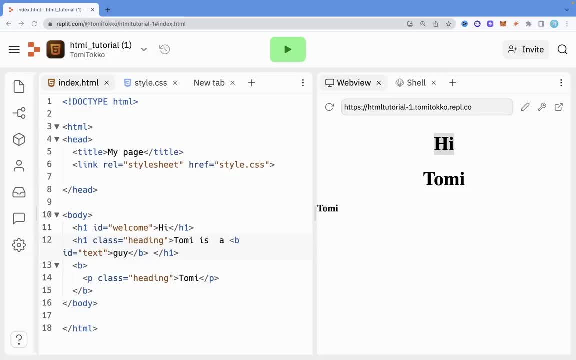 um text. so once we give that that id, well, we just want to actually let us give it an id, let's use a class attribute so that we can just look at that from there. so once we give this a class, what we can just do now we give that a class of text, you know, copy that text and i'm going to come in here. so 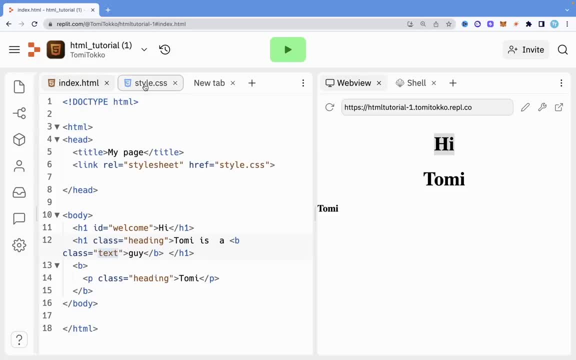 i'm just going to say h1. now i'm going to say b dot text. so right here, now, what i'm going to do is to come in here and i'm going to say the dot text and i can just say b dot text. you have a vertical alignment of, let me say, top. 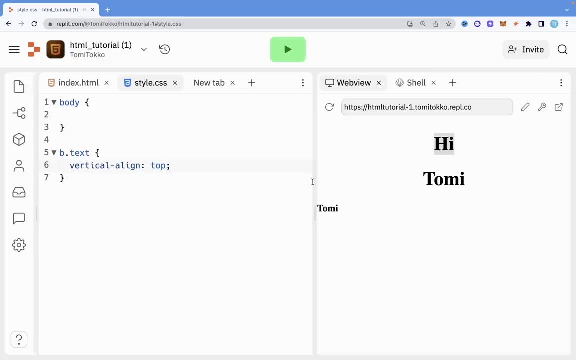 now if i run this, you're gonna see. i'm gonna wait for that to run. so it says tommy is a guy, so that doesn't really make any change. that's just because it's. uh, the size is the same as the h1, but let's say this is actually like smaller. 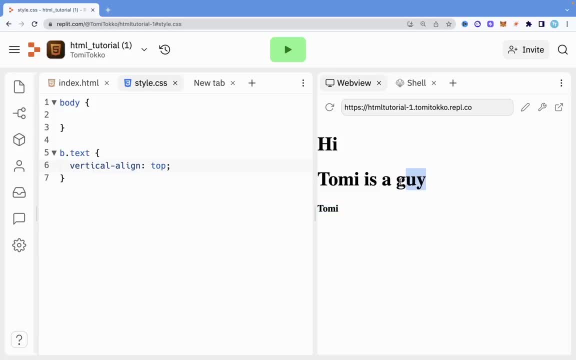 like this p: right here we it's. once we make the alignment go to the top, it's basically going to just shift all the way to the top right here. but because this guy is the same size as all of this, so when he tries to shift to the top it basically wraps around all the- oh you know, the whole margin. 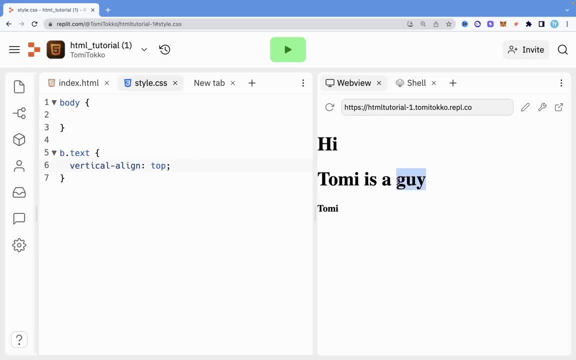 of this particular text. but, for example, let's say you have a smaller text, or let's say this a is smaller, then it's going to go up to the top a little bit. so that is what that does. so now that we know about the vertical text alignment, the next thing i'm going to talk about- 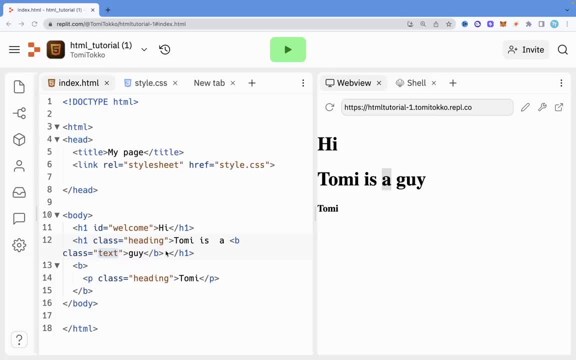 is text decoration. so i'm going to get rid of this ob. i'm just going to run that again and i'm going to come back in here. so right here, where we have text decoration, so what you can, what text declaration does, is that it it adds a line. 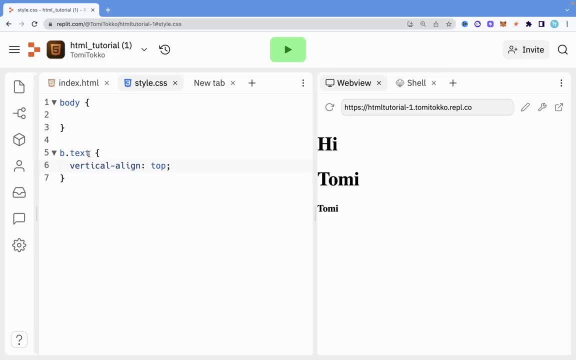 to a text, very easy, very simple. so right here, where we have h1, what i can just do is to say text, decoration line, hyphen line, i can give a value and say underline. so if i say underline, this is just gonna have an underline under the, it's just gonna have a. 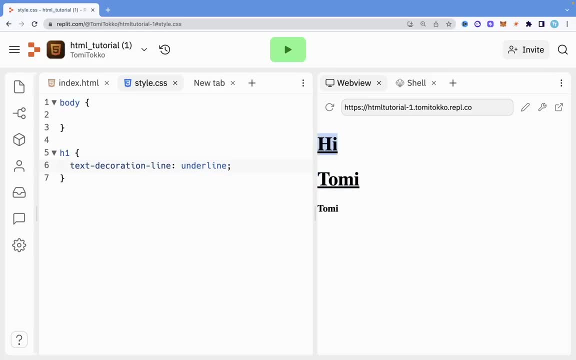 line under the text. that's what that does. now there are different ones and i'm going to try them now so we can say something like line true. once you say line 3 is just going to strike a line across the text so you can see there's a line striking across the text. if i say overline. 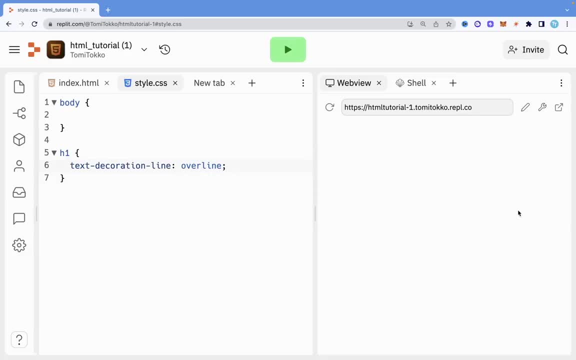 as you might have guessed, there's going to be a line on top of that particular text. now you can also add two different decorations together, like i can have an overline and i can have an underline. if i have both of them together, that is basically going to have one on top and also one on the bottom, as you can see right there. 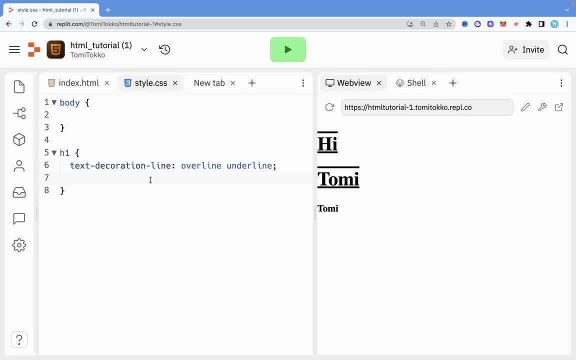 now we can do more. we can actually, like you know, say the color that we want for that decoration line. so we can say text decoration color: let's just say green. once we say that and we run it, you're gonna see that, just the color of that. 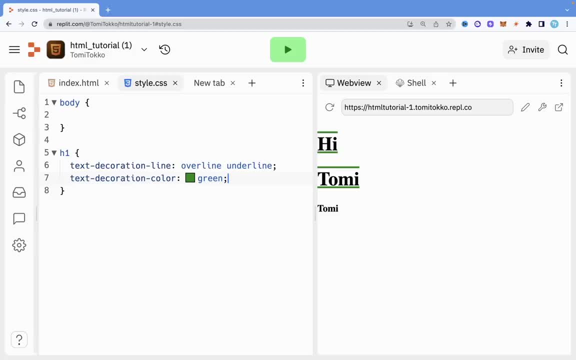 line is green and not the text. as you can see, it changed the color of that line to green. another thing we can also do is to specify the style of this line, like what if we want this line to be, you know, dotted or dashed, or solid? what you just need to do is to say text decoration. 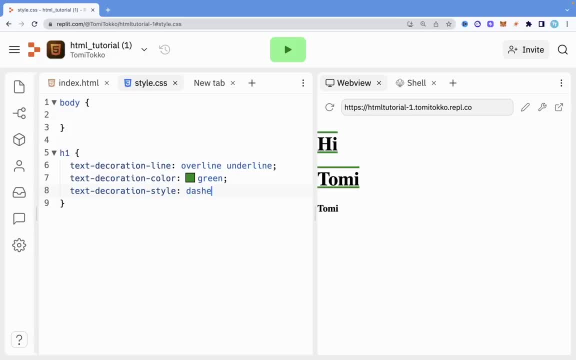 style and i can say dashed. once i say dashed, this line is gonna be dashed. so i can also, you know, change it to double and i can also change it to dotted. you know, i can use basically any style, just similarly to what i use in the borders, so that is dotted. so what i can also do now is to specify the thickness of 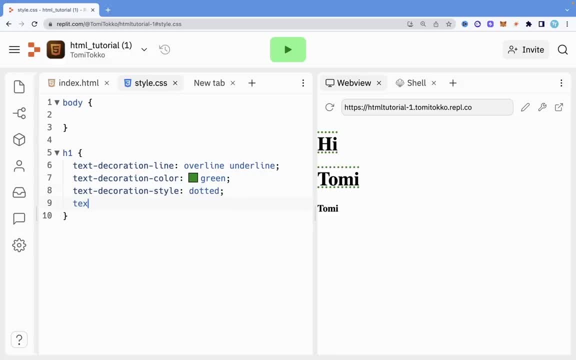 that particular line. so we're just going to say text decoration. i'm going to say thickness. now we're going to use pixels. we can say 10px and that is just going to give it a thickness of 10px. as you can see, it's quite thicker. if i say 90px, you're going to notice that. 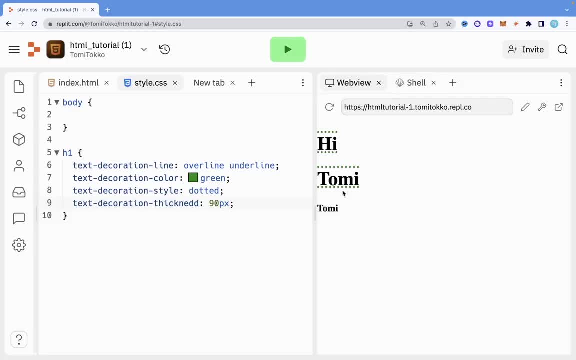 very well. so, okay, this should be ss, so you should notice the thickness there. that's a lot. so if i say 10, let me just go back to 10. you can see that that is 10 px. so now, instead of having to write all of these, 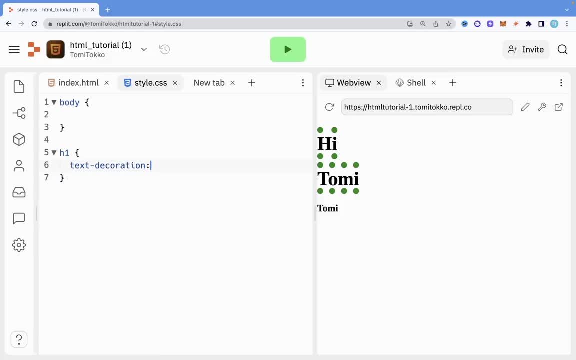 i've used come. i've used a few different styles. i mean, i've used color to write and then i've changed the font happening and so all of these styles are showing up in my text next. so that's it and i'm going to go back to my text. i'm just going to go back to. 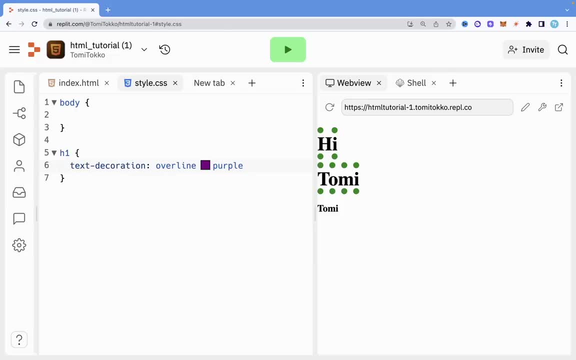 text, and then i'm just going to go back again and i'm going to change the font to the one that i wanted to do here, because i think that this is the one that's going to have the best look. let's say, if i want to go with this color, i'm going to go with this color, so it's okay. 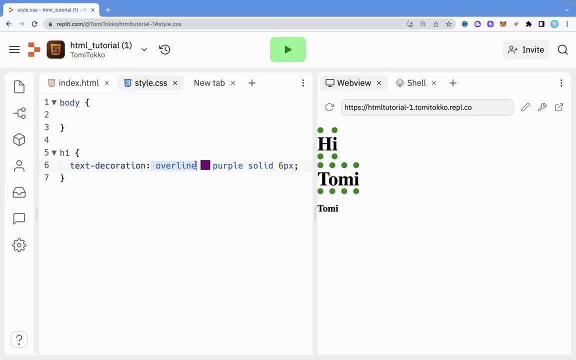 i'm just going to change the color of the text. so this is going to be the color that i want for the text. you first specify, you know, the one that you want, the line that you want, the type of line, and then you're going to specify the color, then the style and then the thickness. so once i run, 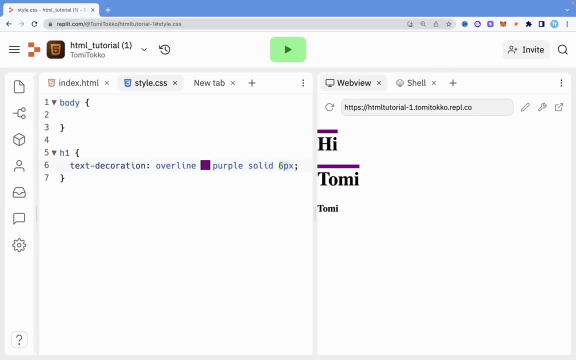 this. now you're going to see that that works perfectly. there's also something else that we can do. we can just basically say text decoration, we can say none. now this text declaration none has come very handy, especially when i'm building, like pages with html css, for example. let's say, we have a link and i'm going to show you this right now. so right in here we are. 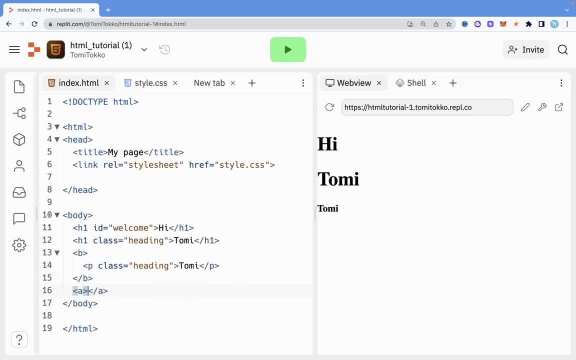 going to have an, a link, and i just say link and let's just say href and that goes to hashtag. if i run this, you're gonna see that it automatically has this underline right there, right? but what if i don't want that line or any decoration on this? what you can just do is to come here and say: 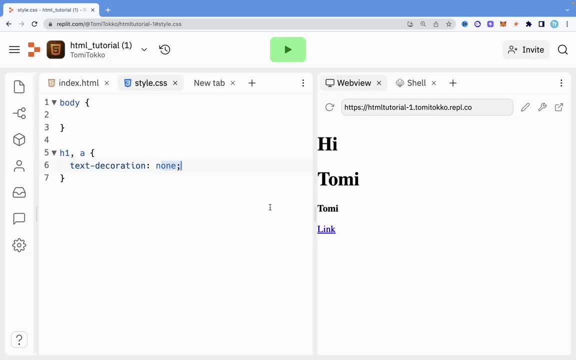 an a tag. every a tag should have a text decoration of none because, as you know, automatically it has this underline decoration. but once i say no decoration, you're going to see that it doesn't have that underline, no more. but the link still works perfectly. so that's a you know very useful. 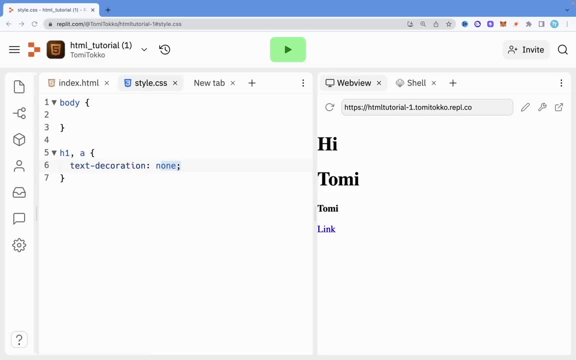 tip that i've used a lot, and now we're going to talk about text transformation. so text transformation is basically transforming the text. you can make it uppercase, you know, lowercase capitalized. you can do a lot of stuff with the test transformation. so what you can do now is 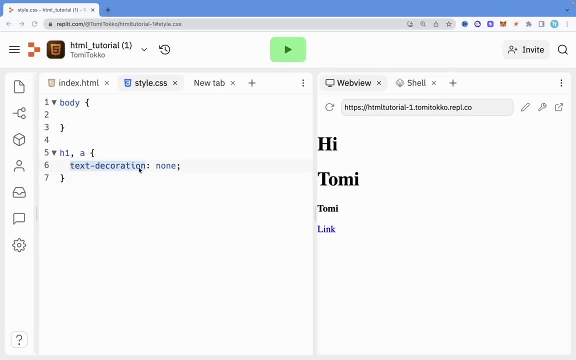 you just say, let's say text, i'm gonna come here and type text, hyphen transform. so what do i want to transform me to? let's say i want everything to be lowercase. so now you're going to see that all of these texts are going to be transformed to lowercase. i can want it to be uppercase also. 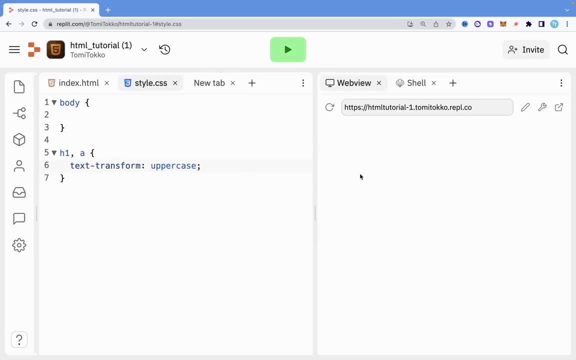 and once i run that, you're going to see that this is all uppercase. now i can also change this to car vitalize. now, what capitalize does is that when we have a sentence, every word in that sentence starts with uh, an uppercase. so if i come in here and let's say, tommy is a guy now, every single word. 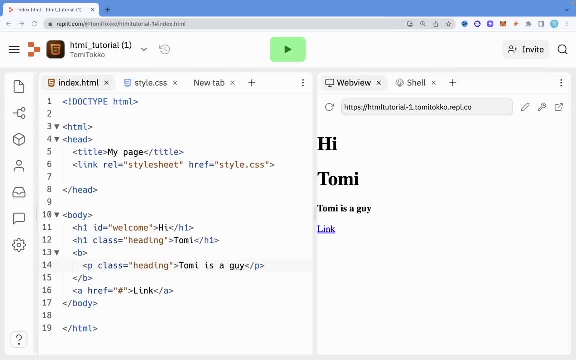 on. it is going to start with an uppercase. so okay, this tom is a guy, belongs to a p tag. so and the okay, what we can just do is to come here and add that p tag so that it affects it also, so as you can see every single word in that p tag now. 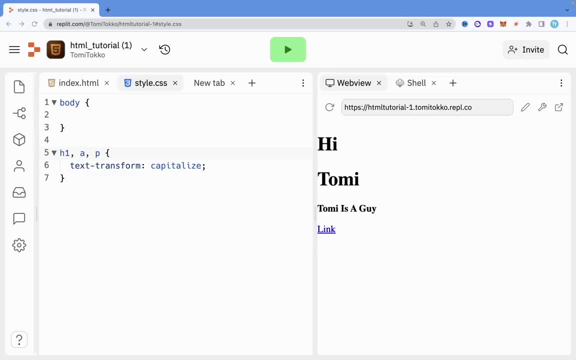 basically, as starts with a capital case. now the next one i'm going to talk to you about is text indentation. so let's remove all of this and let's say we have a sentence like this and we want it to start with a paragraph or something like that. what you just need to do is to say text indent. 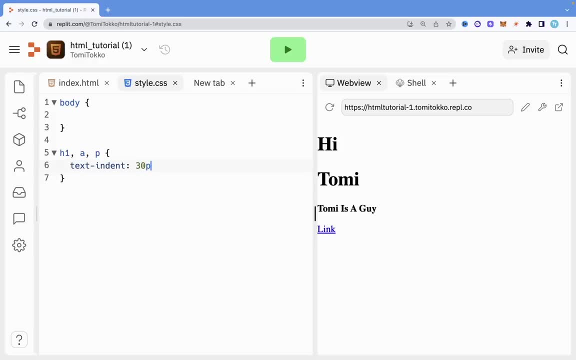 and we're just going to say something like, let's say, 30px. once i say that you're now going to see that all of this starts, you know, as a space before it. so that's a very simple way of you know showing then to your text. so, and i hope you understand that, one more thing, the last thing we're going: 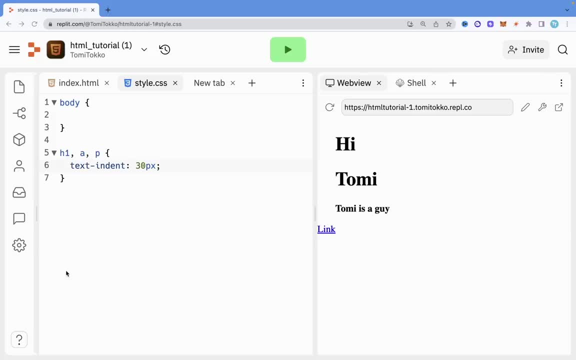 to talk about now in this old text is the letter spacing. so, for example, let's say you want there to be more space between each letter. what you're just going to do is to say letter spacing. so once i run this letter spacing and now i'm going to see that there's going 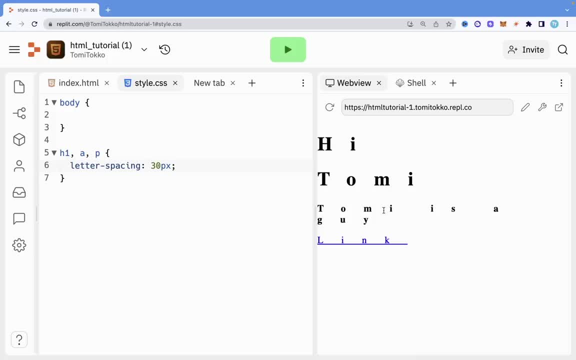 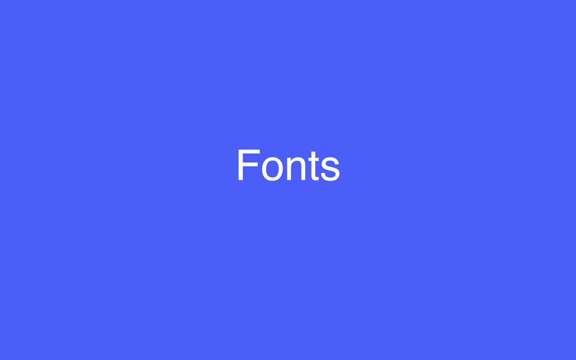 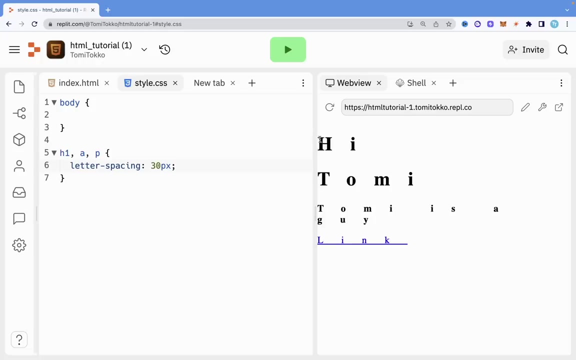 to be a spacing of 30px within every single letter. so that is how the later spacing works. now i hope you understood everything we talked about concerning text. now let's look into fonts in css. so front just basically allows us to change how the text looks. 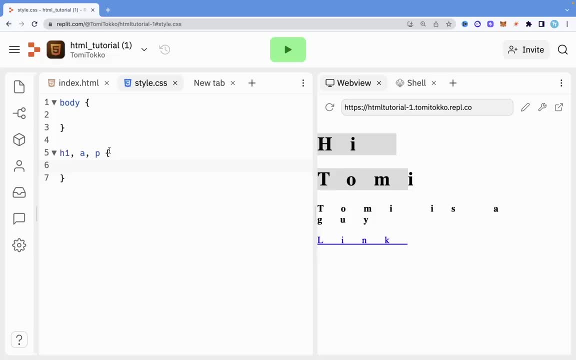 like, let me get rid of this spacing letter spacing and just have it back into normal. so i'm also going to get rid of a, just want it to affect h1 and p. so what we can do now is to actually change the font of this text. so for me to change the 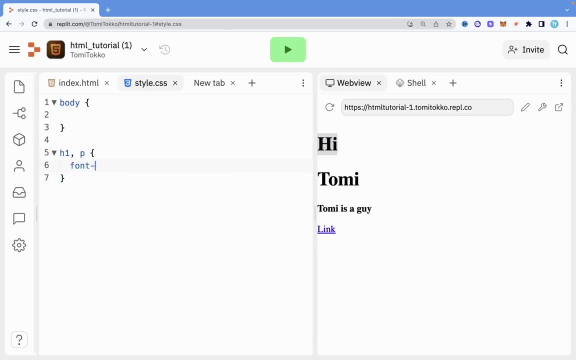 font of this text, i need to use something called font family. now there are there's a lot of like fonts you can use, and you can easily search google to get the list of css fonts that you can use, but i'm just going to test a few ones now to show you. the first one i'm going to test is ariel. 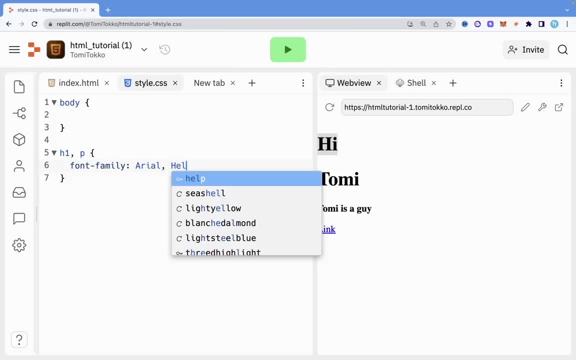 so i can say to use- i'm going to say ariel, command, command. so it should give us like a vertical, and that is under the sans serif front. so once i run this, you're going to see that the font of this has changed to ariel. you can notice that it is now a different font, so i can also 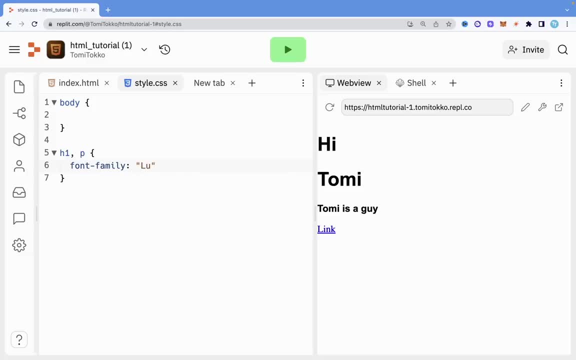 change these to, you'll see the console. so that's a font and you don't need to know all of this on of your head. everything is available for you on the internet. so where i can say new, and then this is under mono space. if i run this, you're gonna see that that changes the font to. 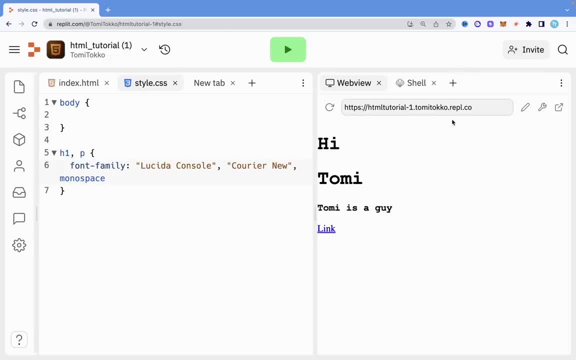 that particular font. so it is very easy to change the font and you know it's not that complicated. all you just need to know is you know the name of the font. so i'm just going to comment that out. and the reason i commented that out is because 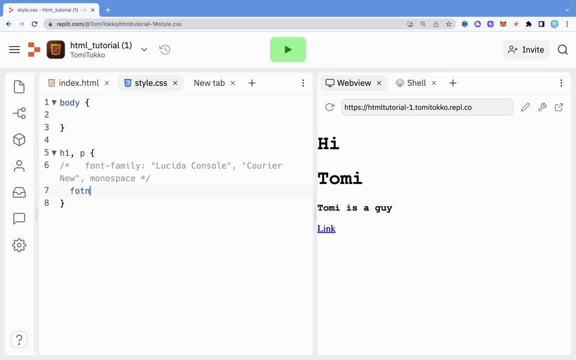 now i want to talk about font styling. so i can say font style and i can say that this style should be italic. if i say this style should be italic, it's just going to make the text a little bit slant. so that's just an italic tile. so this is. 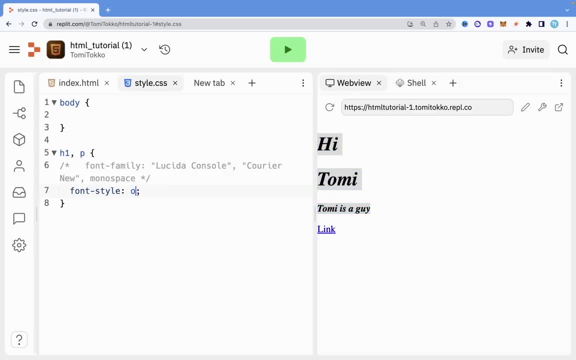 basically a font style named italic and i can also change it to something like public. once i change that to oblique, you're going to see that that is oblique, very similar to italic, and now i can just have it as normal. if i have it as normal, it's not going to change. 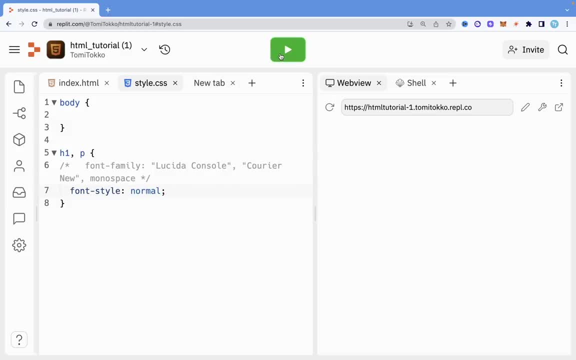 nothing. the style is not going to change, just going to be the same way that it is. so the another thing i can do is to affect the font weight. so i'm just going to say font hyphen weight and if i say font weight should be, let's say, bold, and that font is going to be bold. 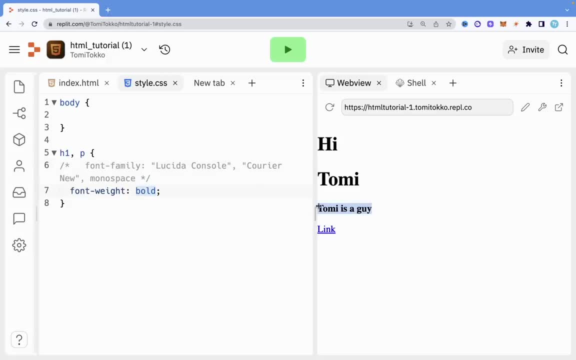 if i say font weight should be, as you can see, there's a p tag, but it's now bold. you can say: font weight should be normal and that is just gonna be normal. so that is how easy it is. as you can see, this was an h1 tag and an h1 tag is always bold. 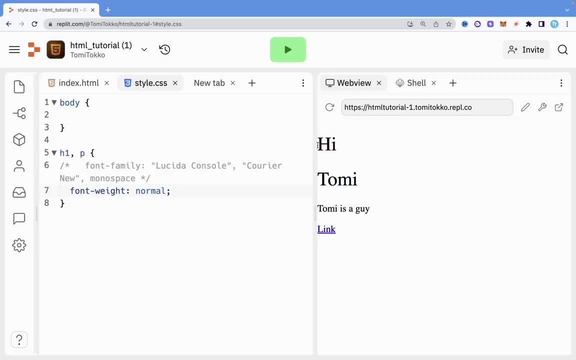 but because i told you to be normal. now, as you can see, it's normal that bold is just normal. and the another thing, the last thing i'm gonna look into is talking about the font size. so the font size is basically giving it like the text size. if i say size and let's say i say something, 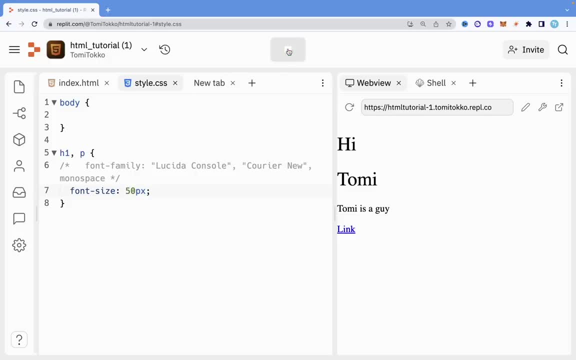 like 50 px and i click on run, i'm gonna see that this is gonna be 50 px, so this is that huge. so that's what it just does. you don't need to over 10k. what you just need to know is that it changes. 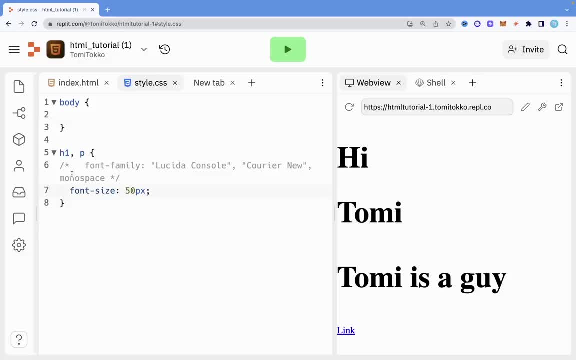 the size of that particular text. now, the way we change this size using px, we can also change the size using em. so what we can just do now is to say, let's say, 50 em is actually a lot. if i run this, you're going to see that it is massive. so actually that didn't show. yeah, you can see how. 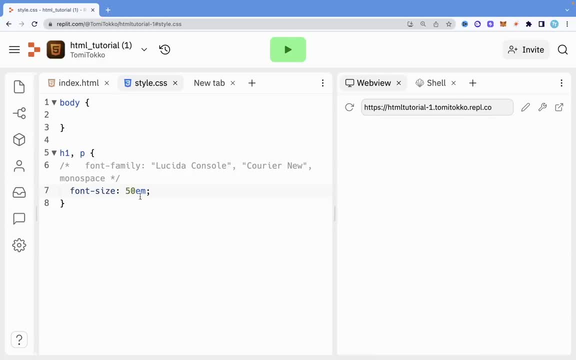 massive it is. so i think 16 pixels is equal to 1 em. so basically, this is like 50 times 60 in pixels, which is going to be, you know, let's say, 50 multiplied by 16, so we're basically saying 800 pixels. so that is why it is that huge. so, but let's say something like you know, say: 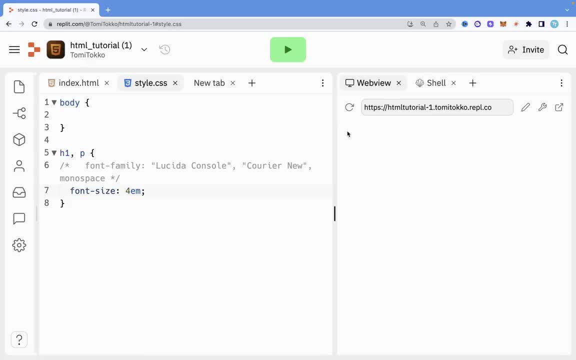 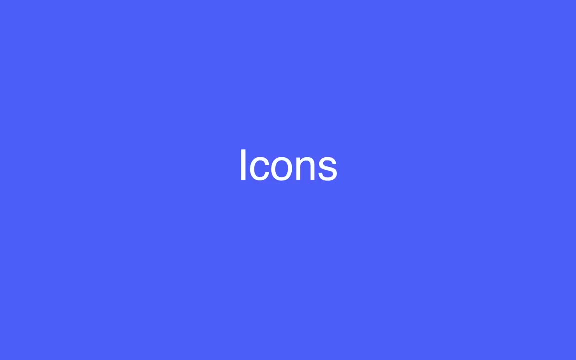 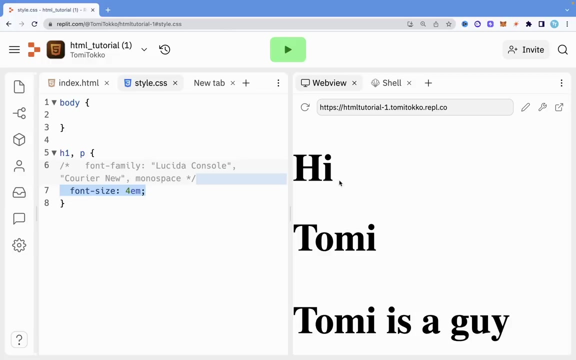 4 am and then if we run that, you're gonna see that it is that huge. so that is how to deal with fonts in css. now let's talk about icons in css. so, for example, let's say: i want to show like an icon, let's say a cloud icon. 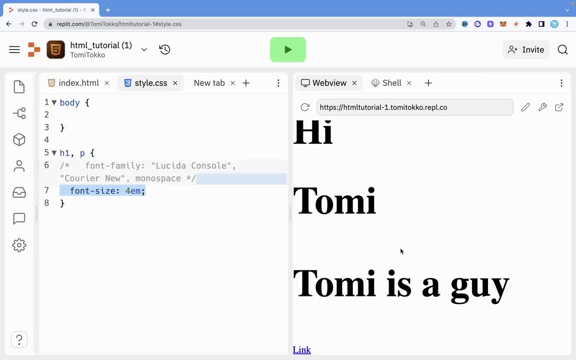 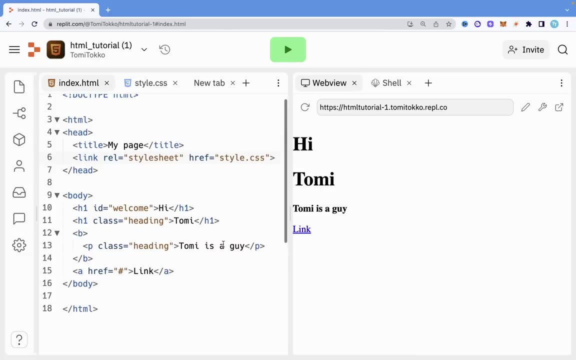 or, you know, a computer icon or any icon. how do i actually show that now we are actually going to use like an external source? so let me just get rid of this to make the text normal back, and i'm going to come into html to actually do this. so what you need to do is to go into your 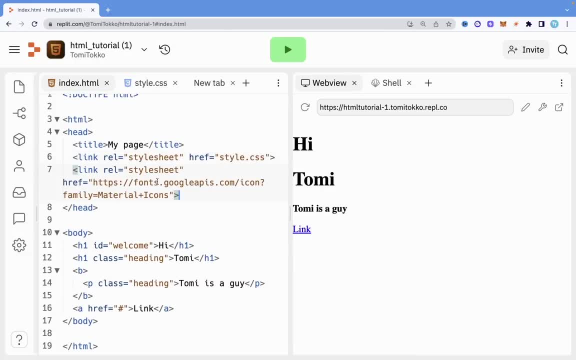 editing element and paste this in there. now you don't need to know like weird what this is, but what it is just is that it basically linking a particular style sheet which is an external css file from a google api. so google product, provided like a css, allows us to just make icons very easily. 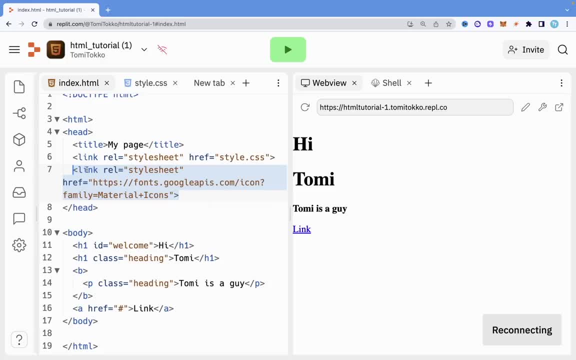 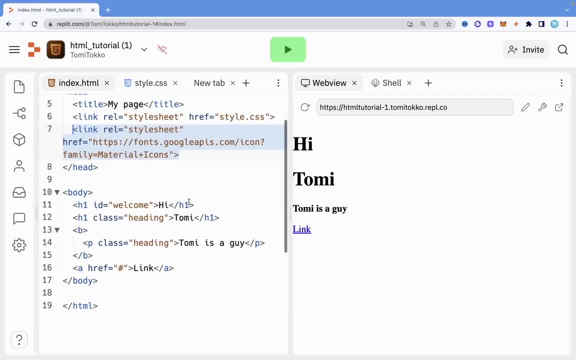 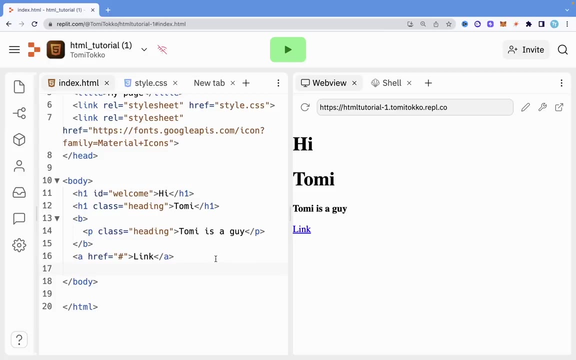 so what you just need to do is to paste or write, type in this particular code in your editing element and once you type that in your head element, what you can now do is to come into your body. and when you come into the body and you can see that this is the place that you want the icon to be, wherever you want that icon to. 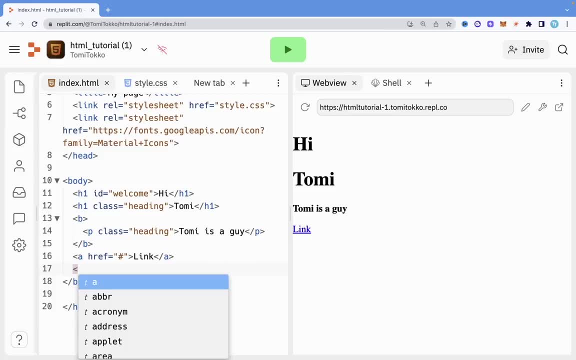 be now. you need to type it or you need to write that you want the icon to be at this place. so we're just going to say we're going to use an element named i and we're going to close it like that and that i is going to take a class of materials. so we're going to say equals to 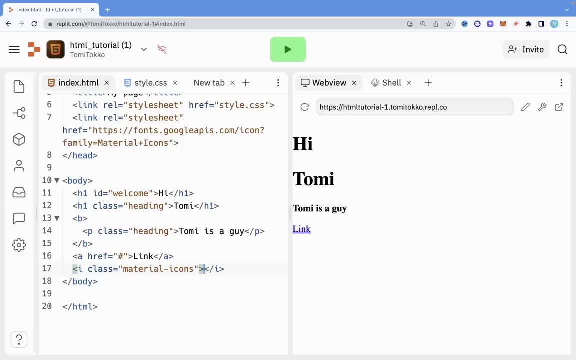 material, i think icons, and now we are now going to write the, if you want, to providing the image with the same values as if it were. i going to show this row that i like, or this guy, or we are going to show the image, not with the. 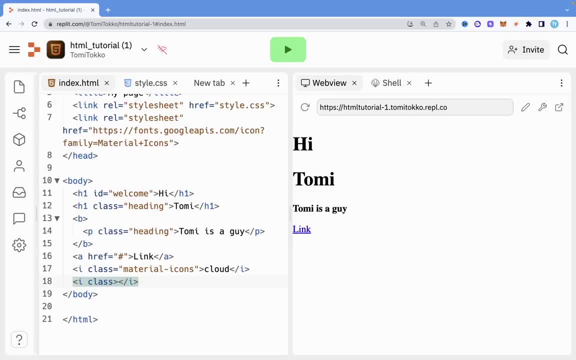 character in text, but with the other icon that we want to show. so if we want the cloud icon to show, we're going to say cloud, we can do the same thing to have another icon so we can say i. exactly the same thing. we're going to say class and they're going to say equals and 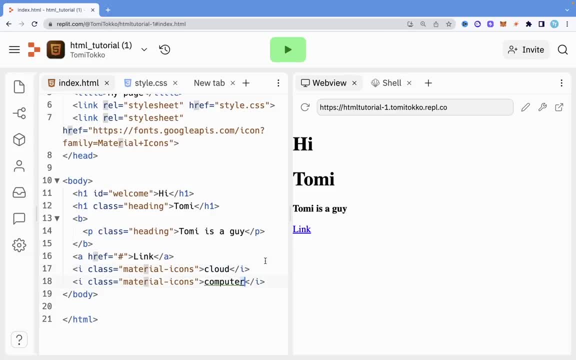 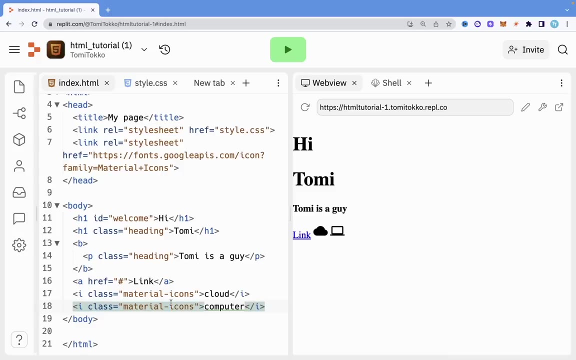 they were just going to see materials icons and computer icon show. now, if i run this, you're going to see that two different icons are going to show. this is a cloud icon. this is a computer icon. that is a very easy way of doing it with google icons api that it provided for us. now we can keep going. let's just copy and paste this. 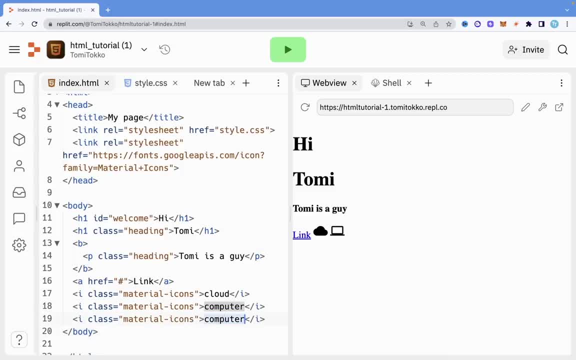 what we just need to do is to change this actual value. so let's say we want traffic icon. if i hit run, you're gonna see that it gives us the traffic icon. now there's a list of icons you can see. you can just also, like you know, go over to the google icons page and look at the. 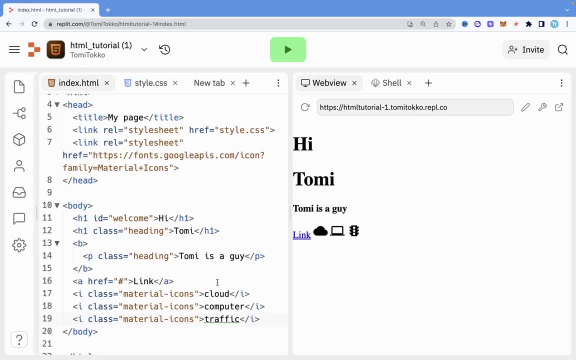 list of icons that they provide. so that is basically it about icons in css. now we are going to talk more about designing or styling tables in css. so right now, the first thing i'm going to do is to just create a very basic table. so right here, i'm actually going to 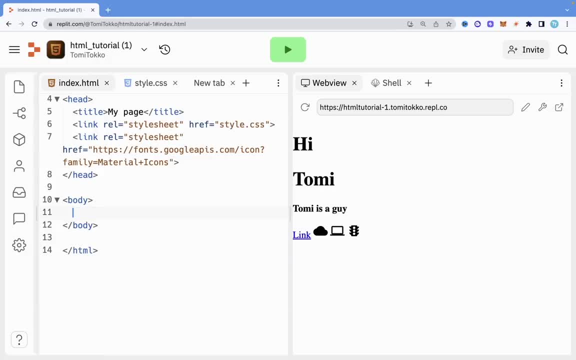 get rid of all of this. we don't need all of this for now, and also of this. so right here i just want to create a very basic table. we've done this in the html section of this course, so now we're just going to have table and then we're going to have 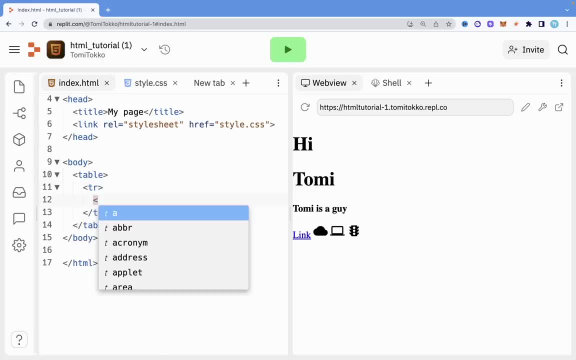 the tr, and in this tr we're going to have the adding. so let's just say name and let's say h. so those are the add-ins. and now i'm going to have another tr, another table row, and right here i'm going to have a td, which is table data. so let's have one name as john and let's say john is you? 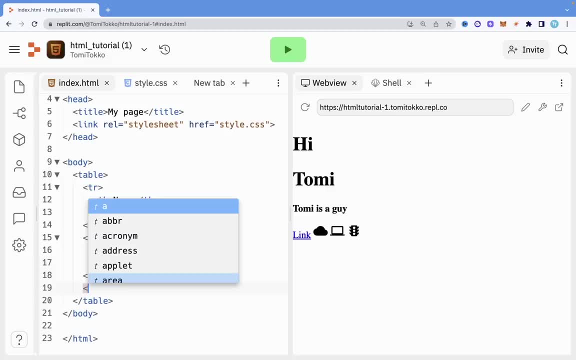 know 15.. and then we're going to have one more table row, so tr, and let's have a td, and let's just say tim, and let's say tim is 19.. so now, if i run this, this is just going to show me that basic. 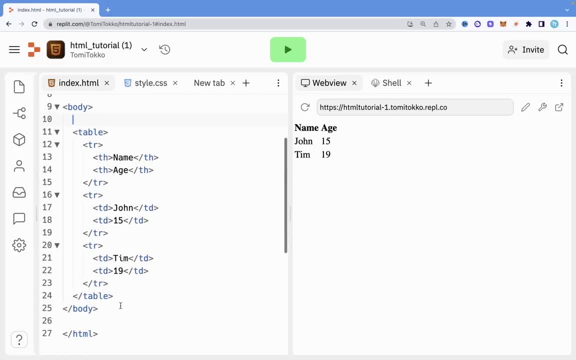 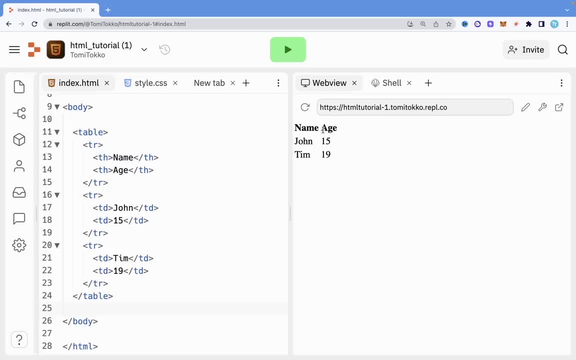 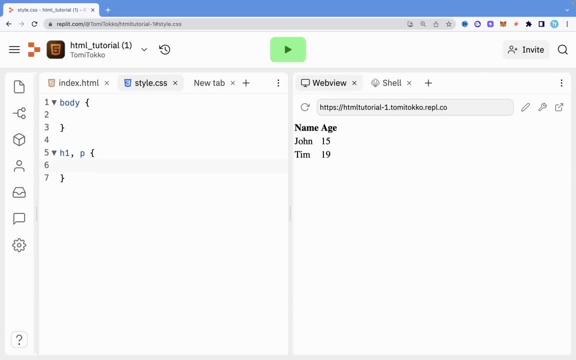 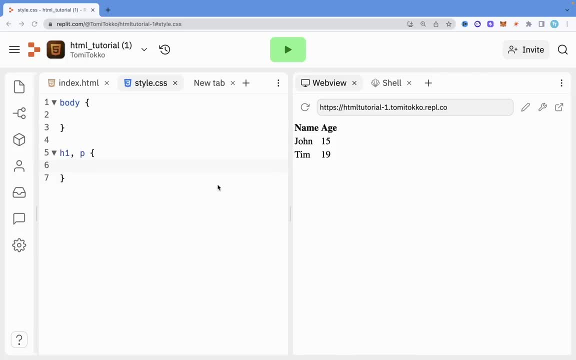 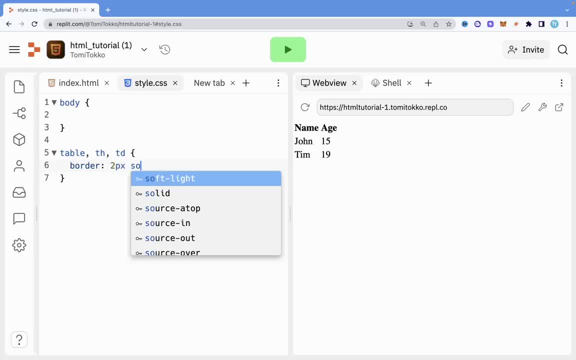 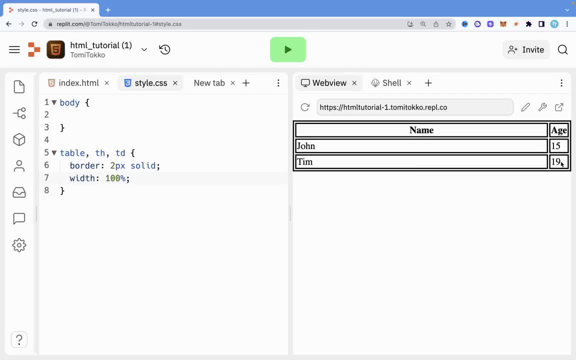 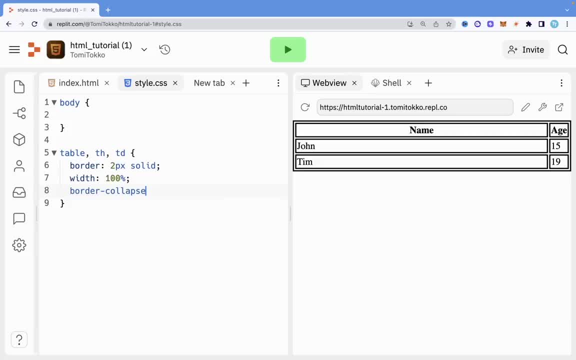 collapse. So once I collapse this and I run it, then you're gonna see that everything basically as one line, which is very good And this is what we want. So that is, you know, the first step in actually designing this table, So we can make this less everyone. 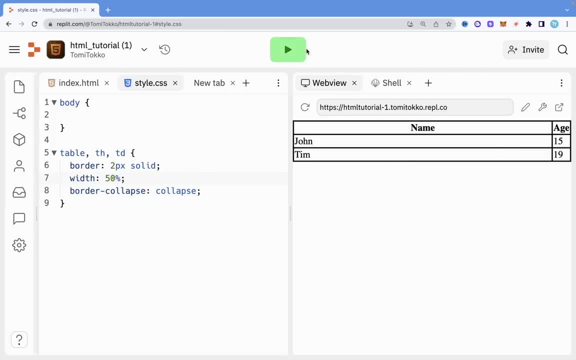 needs to be 50%, So that is basically 50%. So that is good, That is what we want. And now we can talk more about the. you know actual size of this particular table. For example, I can say I want th. let's say like: I just want only this table to have a width of so. 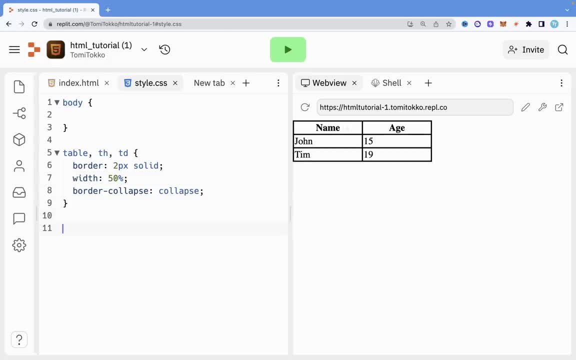 what I can do now is I can come down, and So what I can do now is I can come down and say ch will have a height of, let me say, 50 pixels. If I run this, you're going to see that the height of th is now more like brother. so I can, you know, specify all of these by? 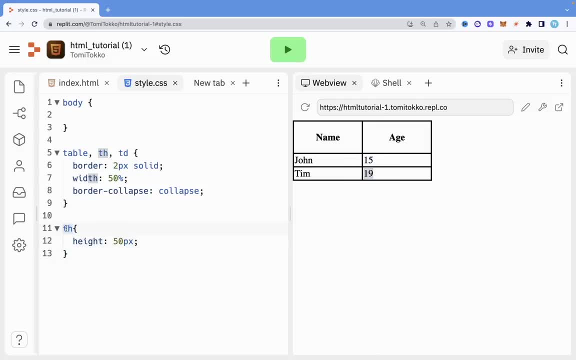 just uniquely using that as a selection like th. then I say it and I give it a value of 50px. So it is that easy to do And you know that's straightforward, And the next thing I can do is to actually talk about this still. 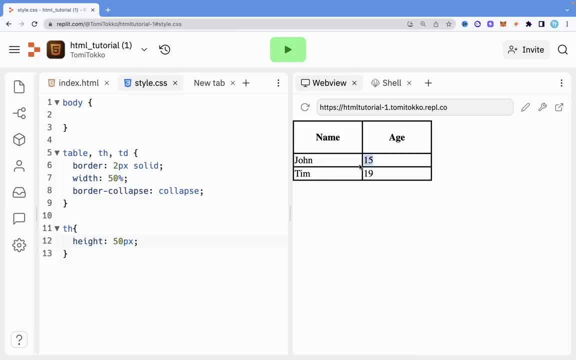 alignment of you know this particular words. I, for example, I want this to be in the center, just the way the editing is. the editing as default is in the center, But for the data I want this to be in center, on the right or wherever. what I just need to do is I need 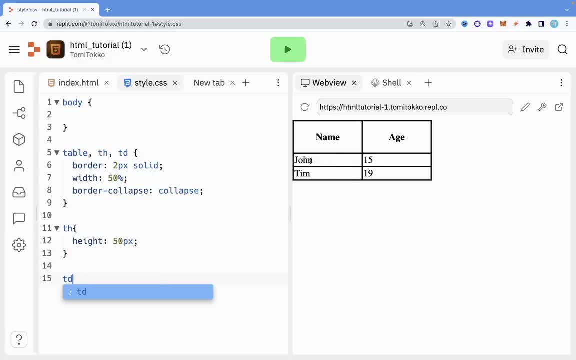 to just say TD, because these are the data right. So I'm going to say TD, I'm going to say text align And if I say right, you're going to see that all the tests aligned to the right side of the particular table. But for it to look good, I'm going to say center, And once I say center, 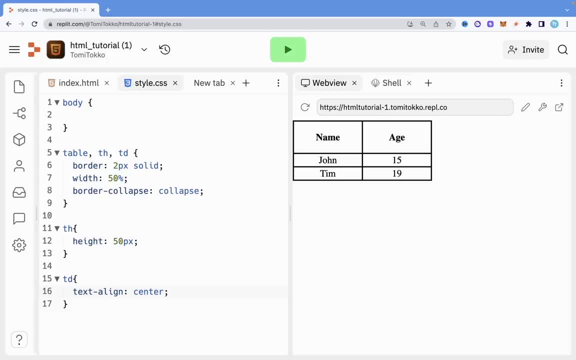 you're going to see that that aligns perfectly. So I can also, you know, change this th to align on the left, so everything can align in the left. the last day I want this to be the left. I can just, you know, copy this particular one and, coming to Th, I'm put that in the 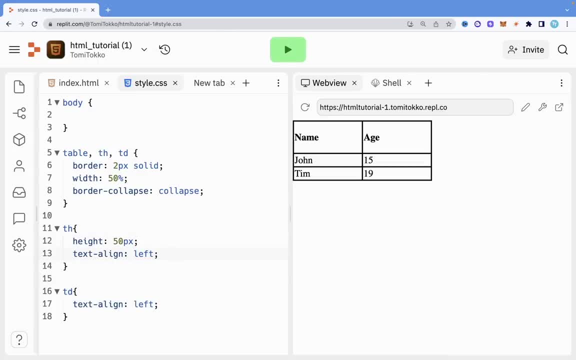 left out that every single thing is in the left. now, that is another way of basically doing that. now, let's say, i want there to be spacing between, like, every one of these like. as you can see, this is quite congested. what i can just do, instead of having like increasing the width, i can add a. 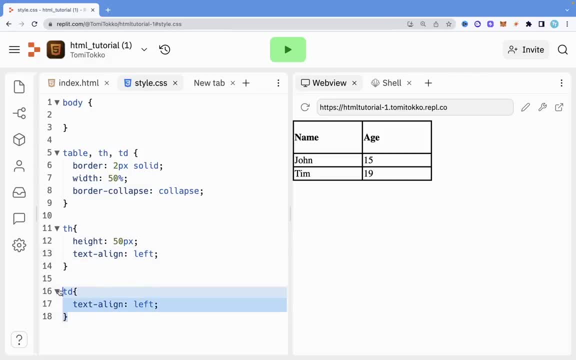 padding to it so i can say i can just get rid of this actually, and i can say th and td should have a padding of, let me say, 10px. i'm gonna get rid of this height now if i run this, and now i'm gonna see that they all have like an equal amount of space. 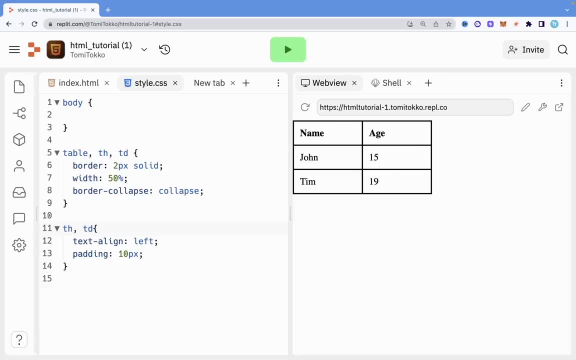 with it. so that's basically what that does right, and that is straightforward, because you know it makes the table actually look very good and that is literally what we want. so what we're gonna do is we're gonna go ahead and see what we have here. what we have is we have a padding of, let me say, 10px. 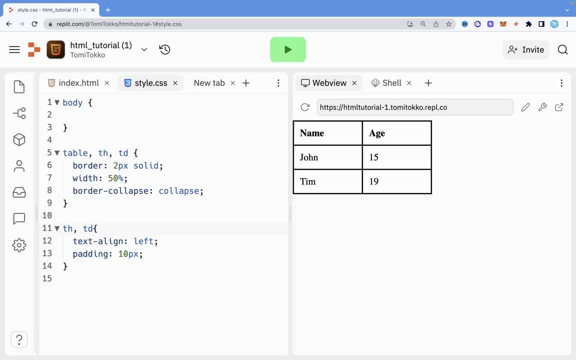 can just do now is to also add some, like you know, something that we can over over. so, for example, if let's say i want to be able to over over this particular line, right, what i need to do is to come here and say table row. and what i mean by over is that when i bring my my mouse on this, 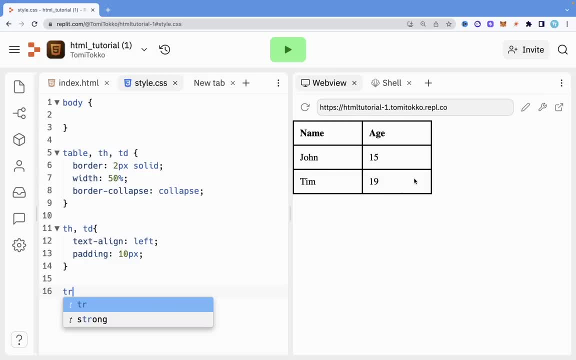 particular part. i want, let's say, it should show a particular color, so it can, or it should highlight that particular row, so it shows that i am over that, so that all of this belongs to table row. so what i'm just going to do is to say tr, which is table row. i'm going to use something different. 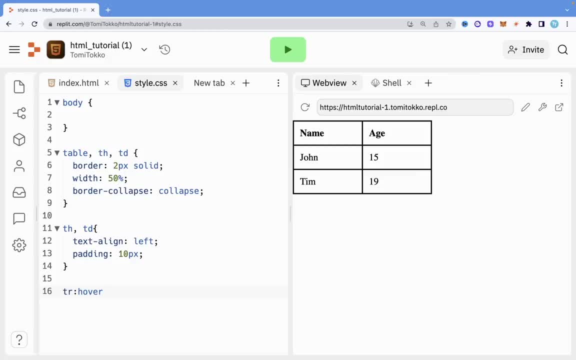 this time i'm going to say column over. now, when i use column over, whatever i do here is only going to happen whenever my mouse is on top of that particular element that has been selected. so what this means now is that if i say i want the background color, 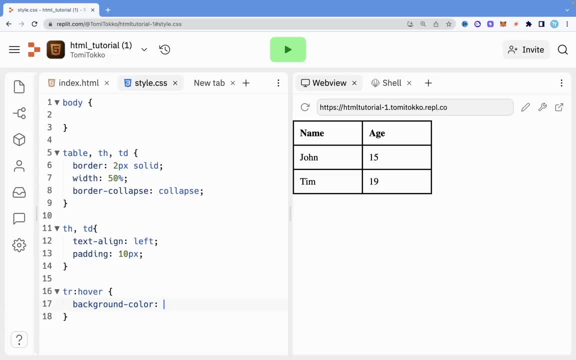 of this tr to be, let's say, blue. now, this is only going to happen. it's only going to be true, only going to happen when my mouse is on it. now, let me run this and show you what that is going to do. so now, when you see that my mouse is on it, you can see that the background color changed to blue. now, this is. 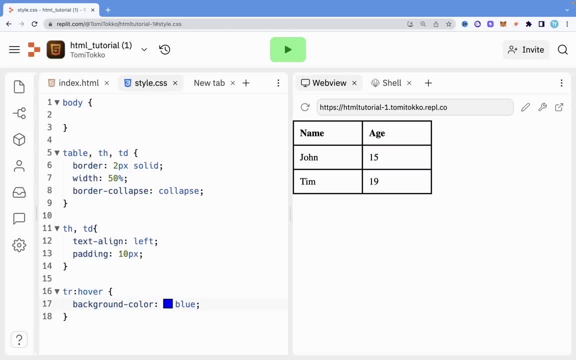 only true when you know my mouse is over it. so that is, you know, a very good one, also because it allows you to easily look at or easily highlight what you want to do on the table. so this is basically the the basic way, or the simple way of designing tables using css. 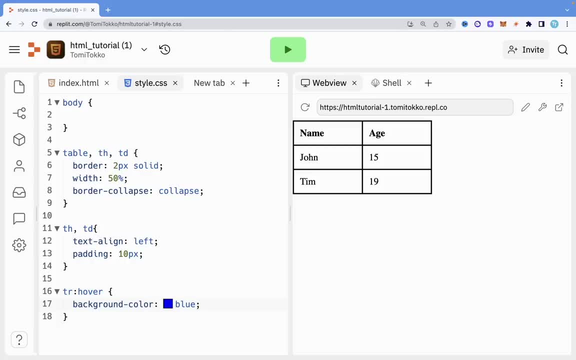 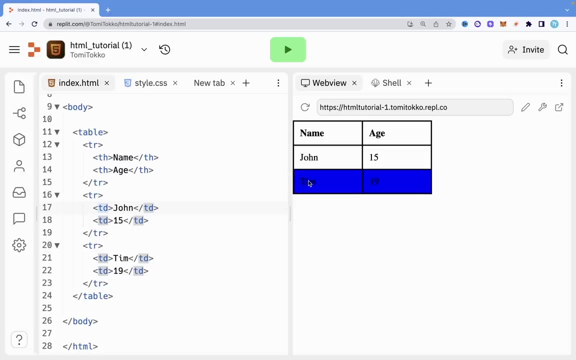 now we're going to be looking at the display property in css. now, what this display property does is that it allows us to, you know, display a particular element, or maybe even hide the element or even remove the element from the web page, but the code is still present. for example, i can get rid of this table and say display shouldn't show. 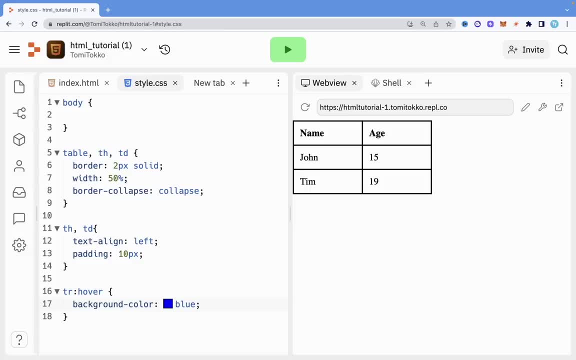 I can hide it or I can do whatever I want to do. And let me show you what I mean. For example, if I come into table right here and I say display should be none, If I run this, you're going to see. 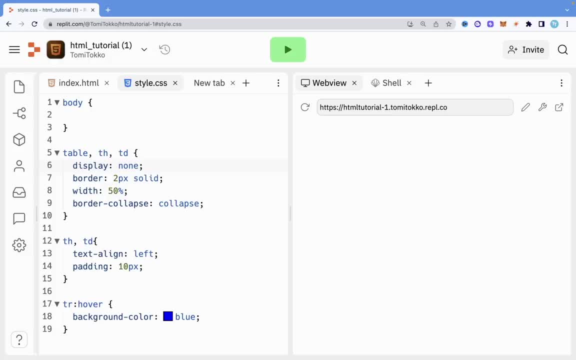 that everything right here is not going to show, no more. And the reason why this doesn't show is just because we've said display should be none. Now there are also many other things I can do, like I can set visibility to be hidden. So if I say visibility, 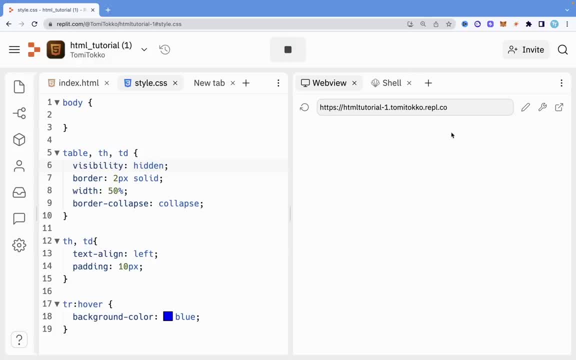 should be hidden Now instead of this. not displaying is also doesn't display, but it is still right there. Now, what I mean by it is still right, there is, if I come in here, unless I have an h1 tag and I say I now, if I run this, you're gonna see that this particular h1 tag starts from here. 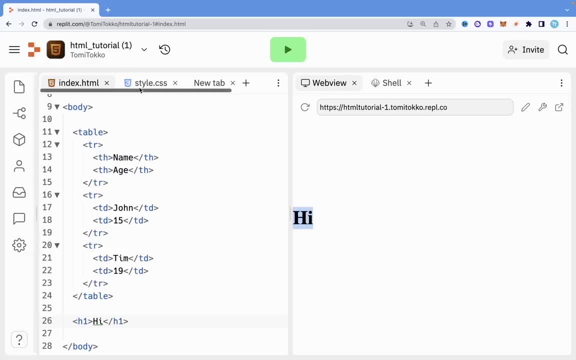 And the reason why the h1 tag starts from here and not here is because we set the visibility of that table to be none. That means it is still present there but is not showing. That is why h1 tag starts from here. But if I said display to be none- display by set it to be none- This basically means remove. 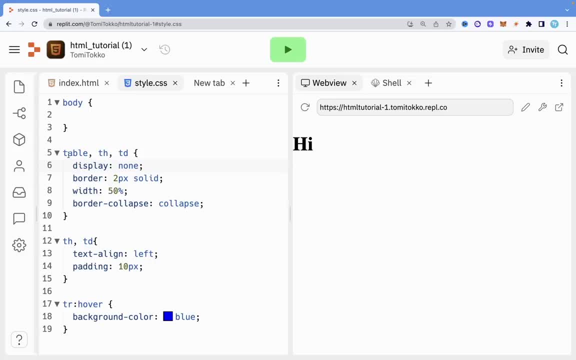 that particular one, from remove that particular table or whatever element from this particular web page. So, as you can now see, I start from the top. So that's the major difference between displaying none and visibility. hidden None allows us to remove that element entirely from the web page. Visibility still lets the element be present in. 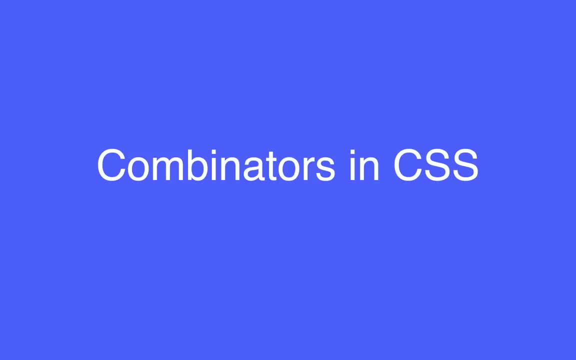 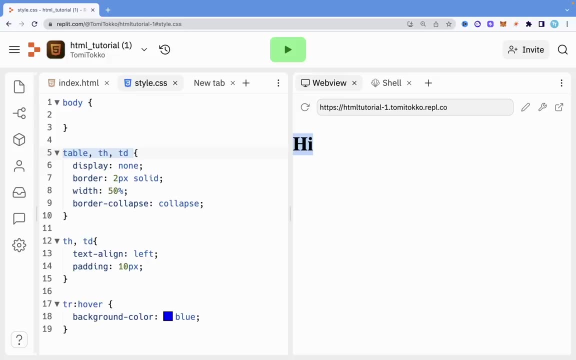 the web page but not show. Now we're going to talk about combinators and CSS. Now, a combinator is something that basically explains, like shows you, the relationship between different selectors. Now there are different combinators and I'm going to explain everything right now. So I want to get rid of all of this. 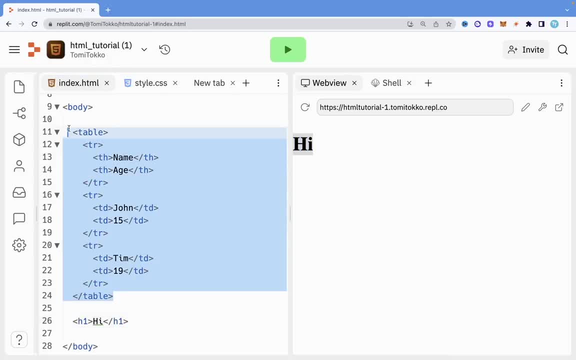 is going to get rid of all of that and also get rid of the old table. Now let's say, for example, we have this h1 tag And it is h1 tag. we now have a- let me just say I- and within this h1 tag, let's say I have another B tag. 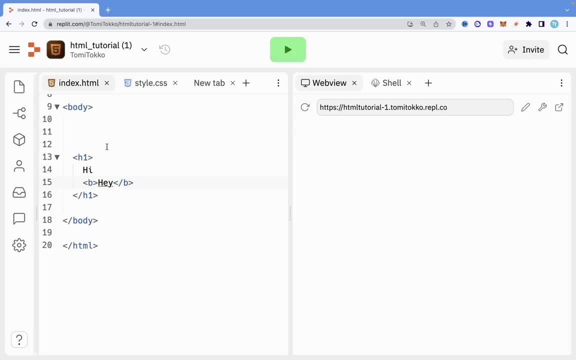 That says a. So this B is inside this h1 tag. Now I can just do is to say I'm going to use something called the descendant selector. So if I now say h1, and I leave a space and say B, what this is going to do is that he's going to select all the B elements inside an h1 tag And whatever. 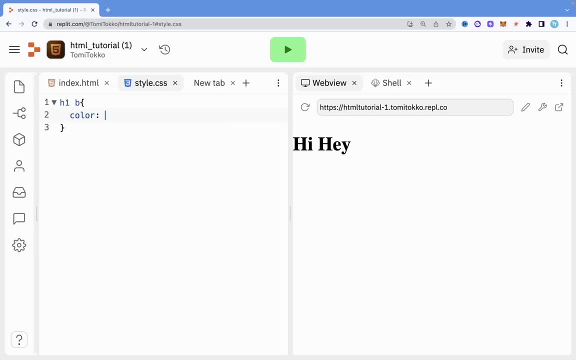 we do here is going to be done to that. If I say colour should be red Now, you're going to see that this a is going to be red now. as you can see, a is red now. what this is is a descendant selector, which means that it selects all the elements that are inside. 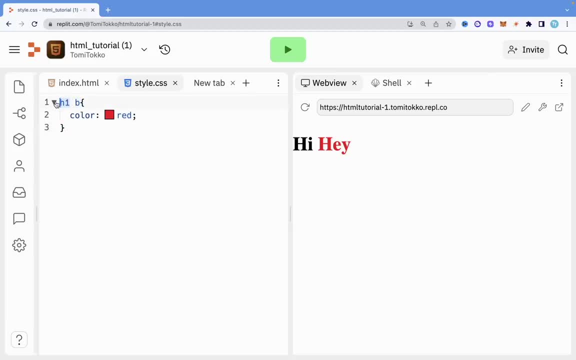 this initial element. so that means select all the b element that inside h1. now if i create another b element- let's say i just create another one, like that- if i run this because that b element is still there, you can see that it says that. and imagine i have a p element, right? 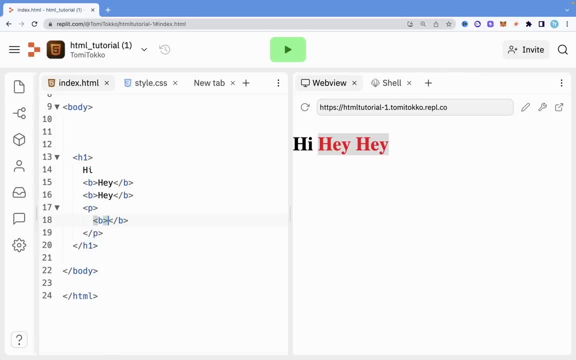 and inside that p element and i have a b element that says what's up, and once i run it, because b element is still under this h1 element- right, it's still a descendant of it, it's still going to affect it and it's going to be red. but now, if we use a child selector, it's going to be different. 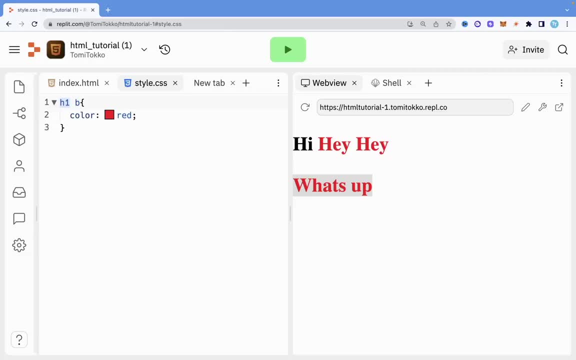 so what we just used now was a descendant selector, but what we want to talk about now is a child selector. now, if i say h1 greater than b, this, this means that it's going to select all the element that is a children or there is a child. 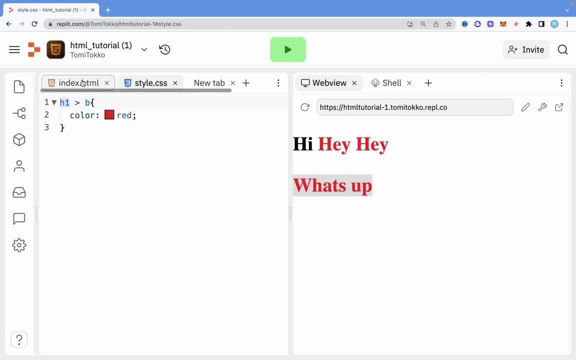 or the b element that is a child of h1. so if i run it, you're going to see one difference and i'm going to explain why. you can now see that this is normal red. this is black now. the reason why is because if i come in here, it's looking for only the b element that are children of h1, even though this b element 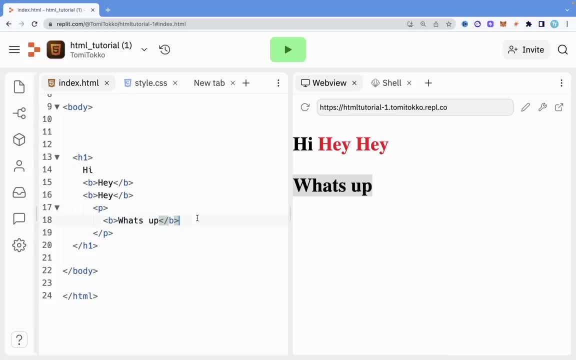 inside this p, and let me just make this like this so you can see it better: even though this b element that is within this p is still under this h1, but because it is not a direct child of this h1, it's not going to be seen. 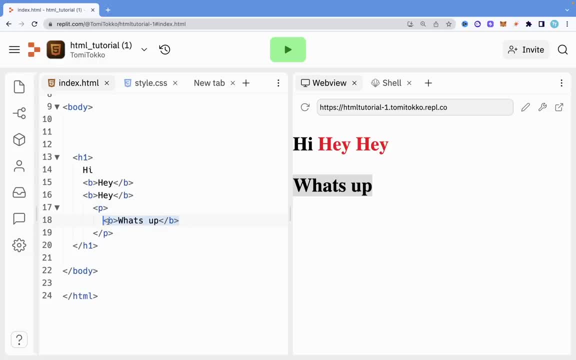 as a child selector. so if i have, let's say i have one b outside this p after a, that b is going to be, that b element is going to be red, as you can see. but because this b is not a child of, h1 is a child, 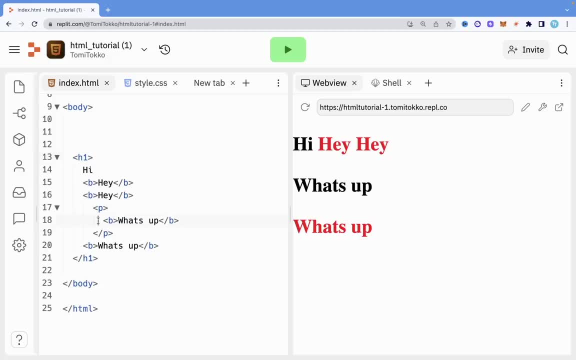 of p, and p is a child of h1. that's why this is still black. now. that's the main difference between a child of h1 and a descendant selector. now the next one is an adjacent sibling selector. now, this just basically selects- if i'm going to use plus to note this, but this selects all the adjacent b. 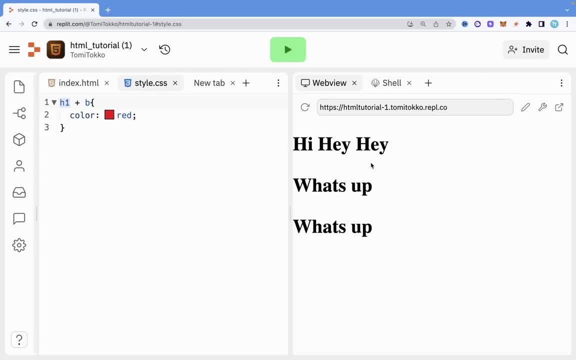 after an h1. if i run this, you're going to see that none of it is red. now the reason is because all of these are children of b, but they are not really out after b. if i come in here now and i paste this, so this is adjacent to h1. it's not a child of it, but it's. 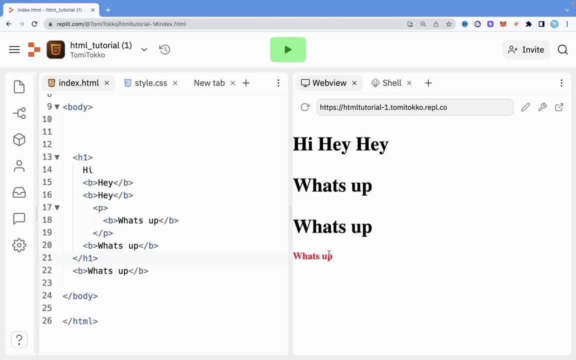 is after h1. once i run it, you're going to see that this one now is actually red. now the next one i'm going to talk about is general sibling selector. so this agency, simply selector, only selects the one that is adjacent to it. so if i come here and paste another b and run, 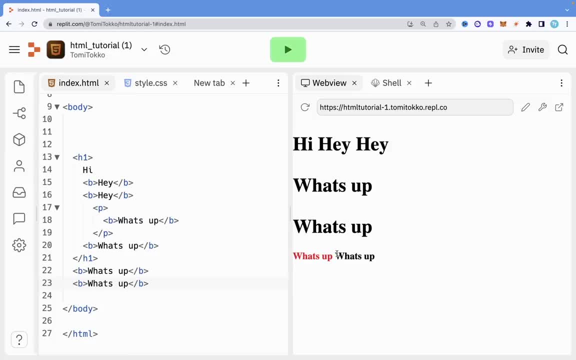 it. you're going to see that what shows on that year is not going to be. as you can see, it is not red. this is because it it only takes the adjacent one to it, and this is the only adjacent one to h1. this one is adjacent to b. it's not adjacent to h1, but if i use the general sibling selector, which is 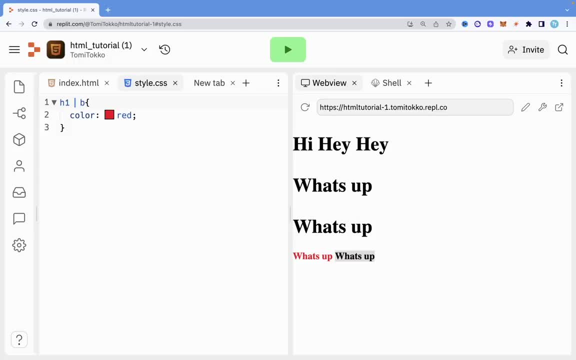 this, you're right here, so we're just gonna get that particular one, the. there's a sign to select the adjacent siblings selector and it is this particular sign right here. so once i use this sign, this shows that any b- that is, you know, the next die like siblings of h1- is going to be red. 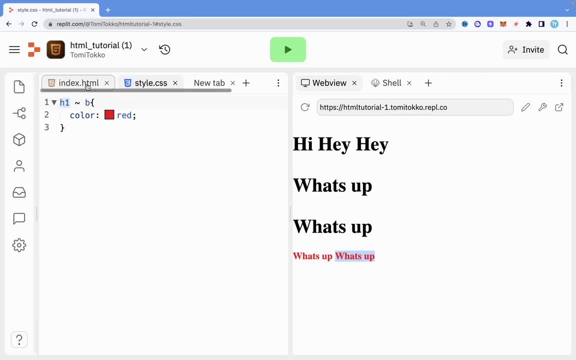 now, once i run it, you're going to see that this second one is also red. now, this is because this second one also come as a sibling to this. it's not just only looking for the one adjacent to it, it's looking for the one that's close to h1. so those are the major four css combinators. 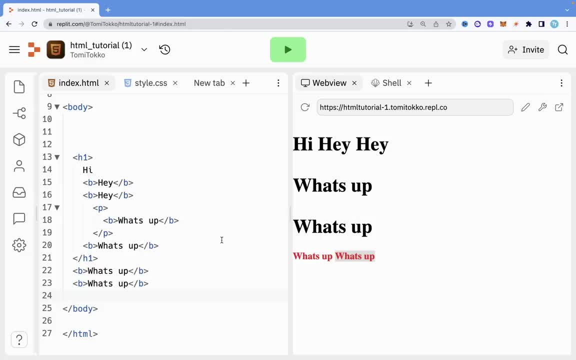 now we are going to look into building drop down menu. so you know normally where you have like an option where you can like over over it, and once you come over it you see something that drops down like a menu. i'm going to show you how you can build that right now, so this is fairly easy. 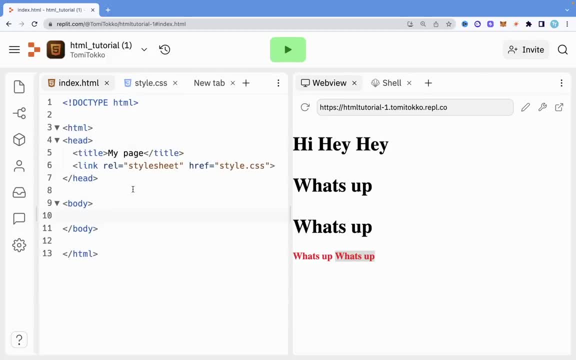 what we just need to do right here in the html body. i'm first of all going to remove everything in the body and what i just want to do is that i want to create a div class. i'm going to create a new div class. we talked about what div class where? i'm going to create this div class. 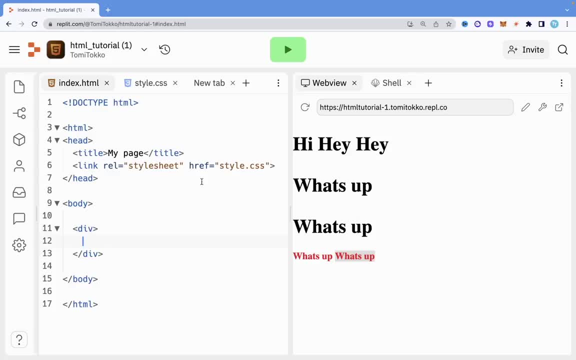 and i'm going to just have it like that and i'm going to give you a class of of drop down menu. so i gave you a class of drop down menu. so this is what i actually want to be dropped down, right, but right here i want there to be like a button that we are going to over over. 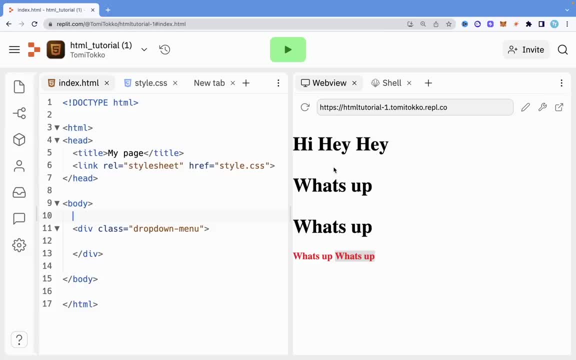 and once we go, our mouse goes on it. we want this drop down menu to show. so here we want to have a button. so there's a button element that just allows us to have a button, basically, and right here we have a button that allows us to have a button, basically, and right here we have a button. 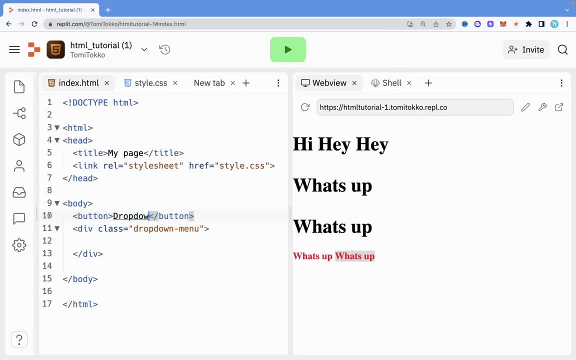 so we're going to select this of button element. here we are going to select the button element component that we want to use. so, right here we want to make sure that we have a button limit. i'm just going to likemodify it sometimesers почему? because usually not every client will. 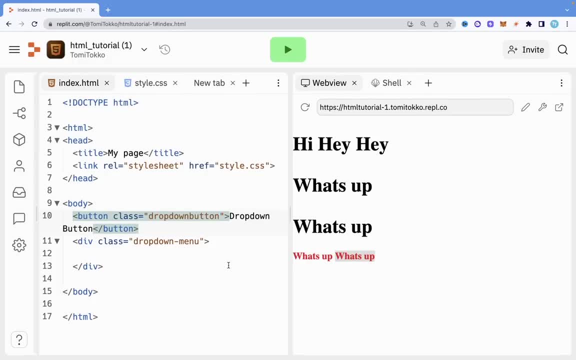 allow us to enable any button, so that's why we have the luxury of doing that right now. um, let's double click aquí to edit this gate. here you can see that we just have a drop down button normally And this div class. we're going to have a basic link, So let's just say a, let's close it And let's say no menu. 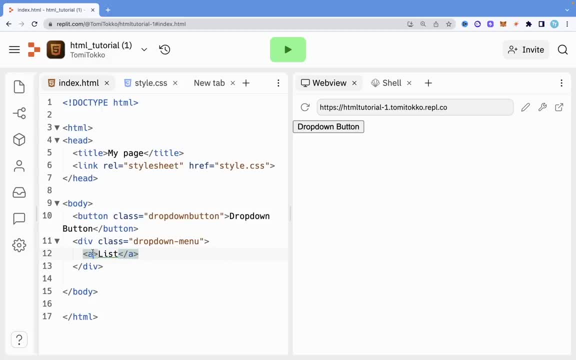 Or we can just say list And then we can say, for now, let's just make it go nowhere. So we can just say link to hashtag. So we have, let's say, four different lists. If I run this, you're going to. 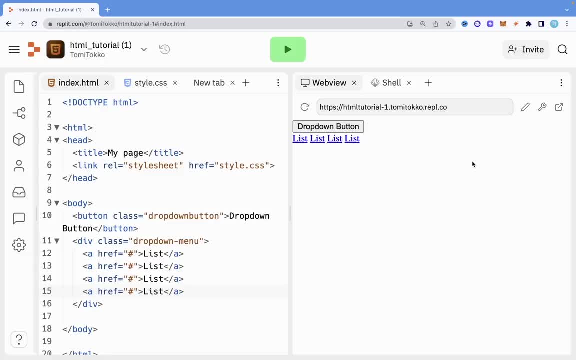 now see that we have that button with four different lists, right. But what I want to do now is I want, first of all, I want this list to not show, and I want to style this button a little bit. Okay, let's take it a step at a time. Let's first tell this button a little bit So what I'm. 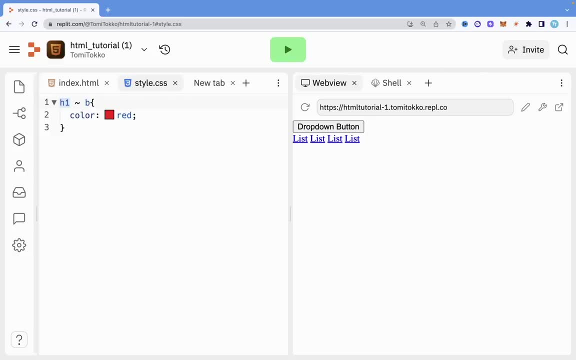 going to do is to come into stylescxs And I'm going to come here and do this. I'm going to get rid of this And this drop down button is. I want to style it. I'm going to take that drop down class And I'm going to say dot, drop down button. 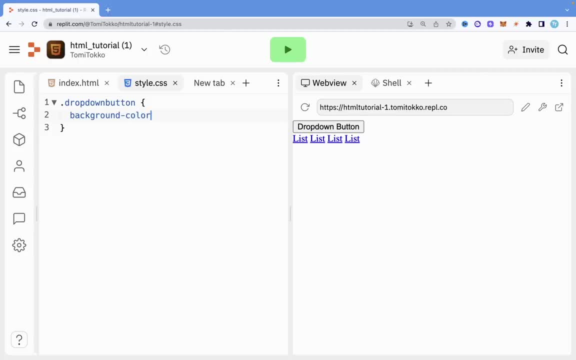 So I want to give you a background color And let me say I give you a background color of blue. Now, if I run this, it should have a background color of blue, which is good, And I want to give the text color. so I want to give the test color white. 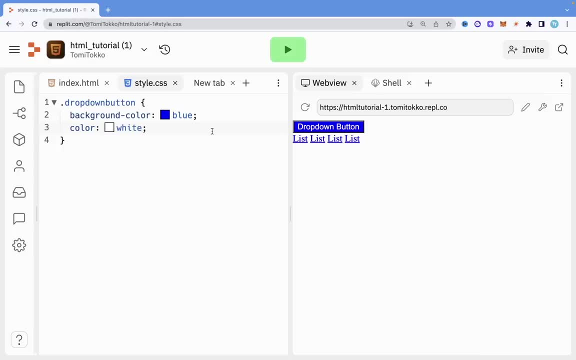 I want the color of the text should be white. So let's see, Good, And what I'm just going to do is to say padding, just so there's going to be a little bit of space And let me give the padding something like 13px. So let's have a colon right here And I'm going to run this. So that is good. 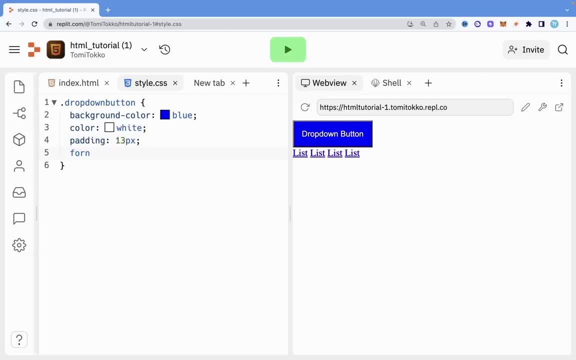 And what I'm now going to do is to say: let me just try to add some font size. I'm going to say 16. pixels. So I just gave that the font size, So now it looks a little bit bigger. And what I can just do now is to say border none. Now the reason why I'm saying border none. 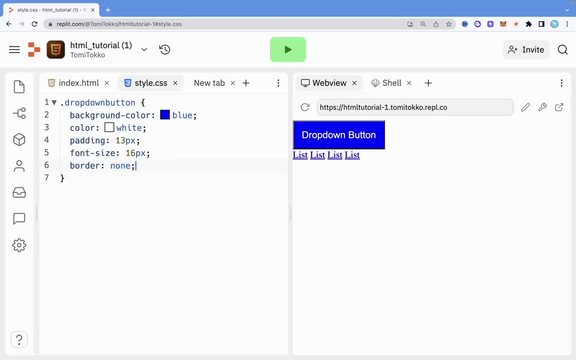 is because, as you can see, on this particular button it has this border that wraps it around, but I want to remove that, So that's why I say border none. If I run this, we shouldn't see any border no more, which is good. And now I want to say cursor. 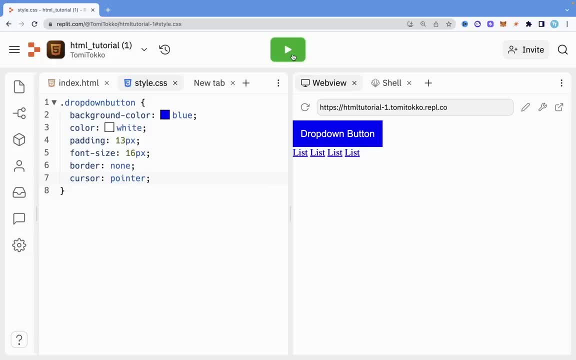 I want the cursor to be pointer, So we're going to run the cursor pointer, right? Good, So that means when we come on this, the cursor is going to change to a pointer, as you can see that, and icon is showing when we come on this. So we've done, we've designed this. 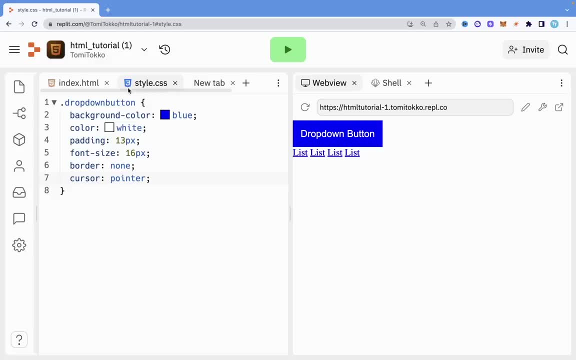 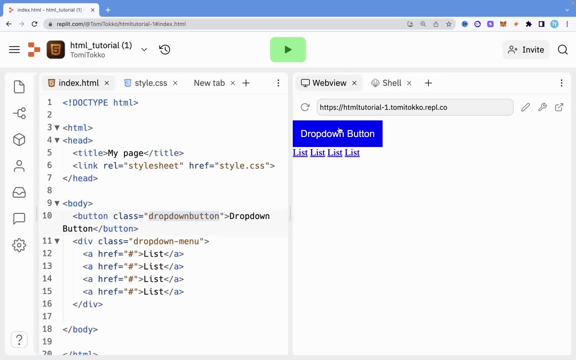 the way we want it to be. The next thing I'm going to do is to actually now come on this list. I wanted to first be a list And then I wanted to not show until my mouse comes over this particular button. Now, let's say, my mouse comes over this button, So I'm going to do this by clicking run. 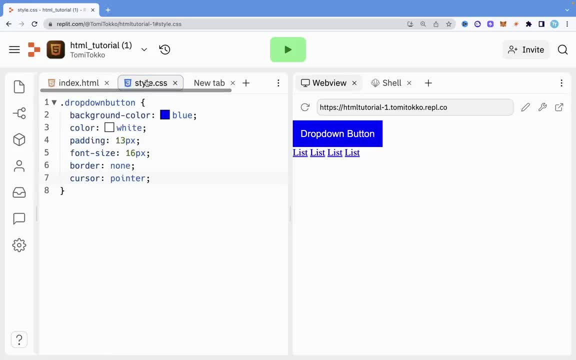 and then I'm going to run this cursor pointer. Now for the cursor pointer. I'm going to go to my go ahead and do that. so what we just need to do is to let me copy this drop down menu class. so, yeah, i'm going to say dot, drop down menu and first of all i'm going to say display. 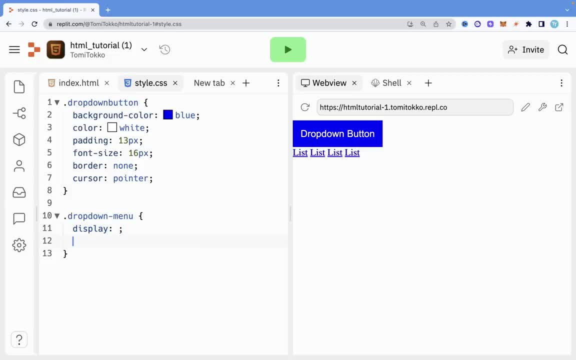 since i don't want to display it, i'm going to say display equals none. but i'm going to leave that blank for now because i want to see the changes i'm making. so let me say: the position is absolute. and once you say position absolutely, we can. then let's run this. first of all, 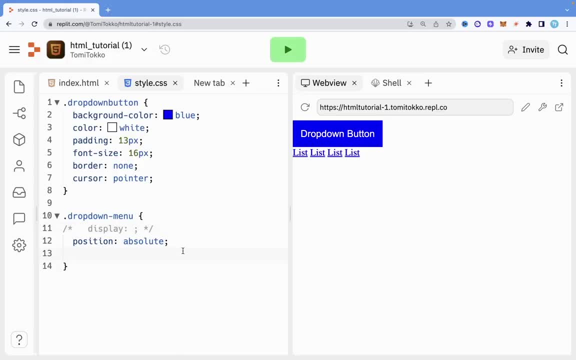 so let's make sure this is this, and then let's say we give it a background color. let's say something like blue, but this time around let's give it light blue. if i run this, you should see that that has a background color of light blue. 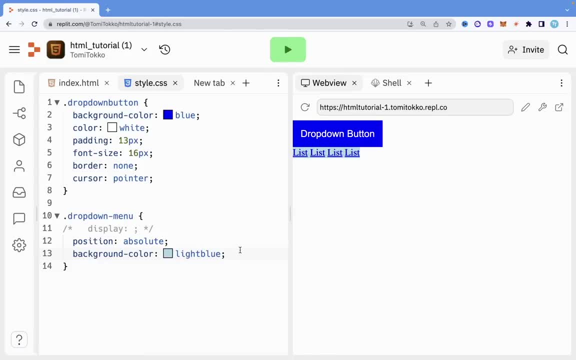 and then let's run this again, and what i also want to give it is a minimum weight. we talked about this. i'm going to say mean width, and when we give it the minimum width, we're going to say something like 150 pixels, and then what we are just going to do is to let's just run this. 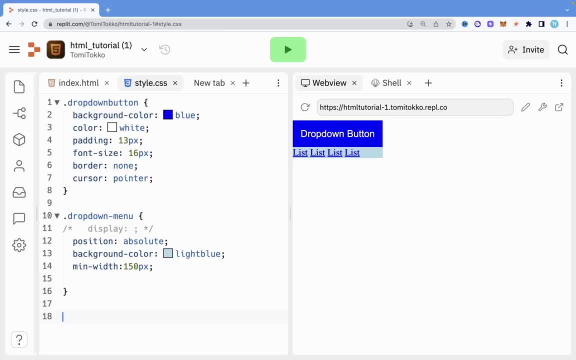 okay, great. so what we can now do now is to say the for the list. under this, we're going to say dropdown menu a. we want to say for the list under this, the a tag. we want the color to be black. i'm going to give you a padding of something like, let's say, 11 pixels and 15px. 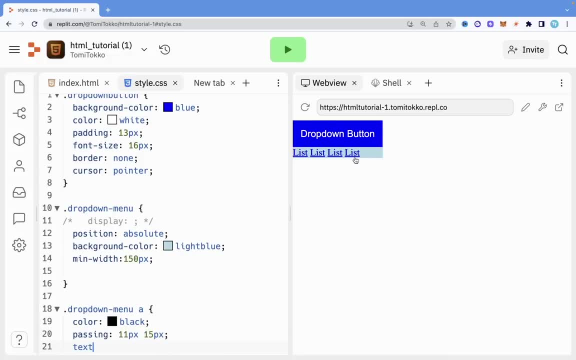 let's give it text decoration of none because it is a link. it's going to have this underlined text decoration, so let's make sure the text decoration is valid because it has telling you know we're going to have this one come to the bottom corner. let's make sure the text decoration is defined in let's- congratulations, because we're such a huge user of text decorations- has a page. LED banner is awakening everything in the title message, in the description. but the next step is we're duplicate them and then, during this process, we want this a bigger one. let's say, once i click on that entry, let's go to 저희가 for remove a vcriptile. we want this. we want to know which ones are obvi. notably these go to tidy code. we now want to TY code. 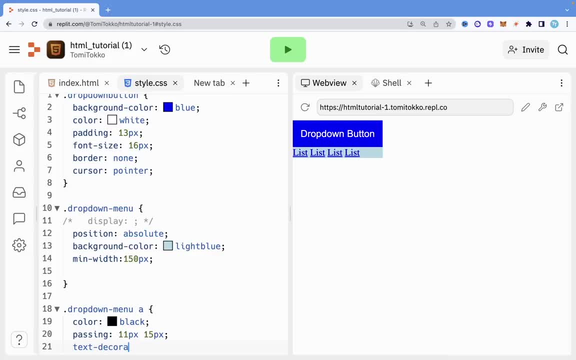 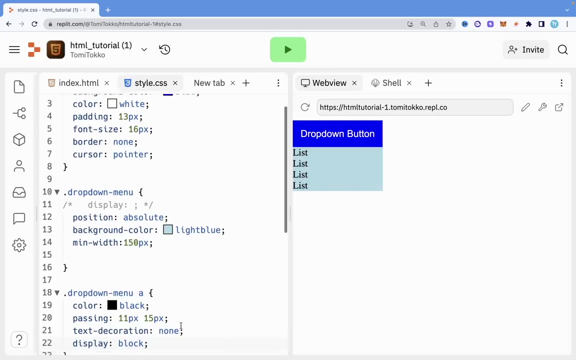 decoration. So let's make sure the text decoration is none. Once we say that, we can say display, So we can give the display value block. Now, if we run this- this should you know, show the changes As you can see. now it's been listed this way, which is what we want, And 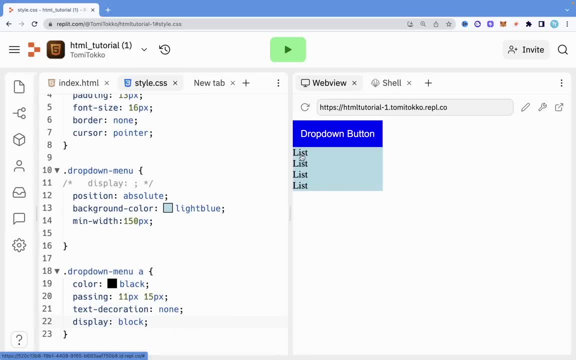 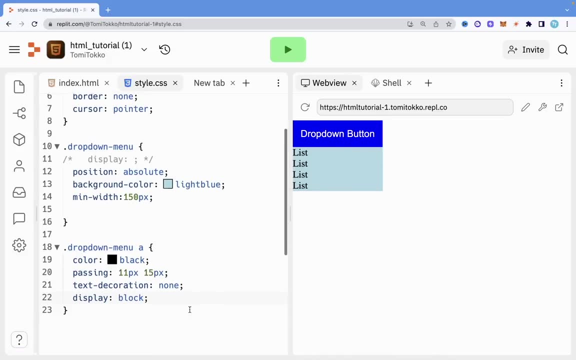 then we give you a text declaration of none. So now it's still a link times, I can still click it and it's going to take me somewhere, as you can see, but it just doesn't show that underline no more, which is what we want. So now we want to have an over. So what we? 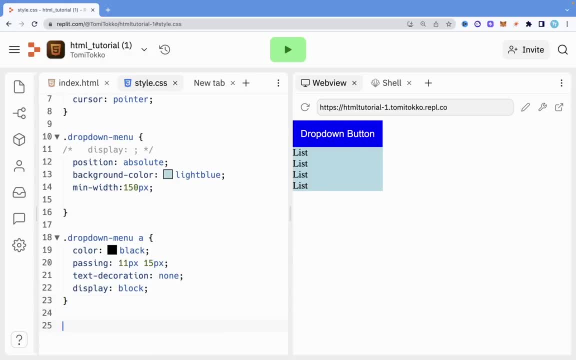 want to do is to say that the drop down content right. we're gonna say a. what we want to do, instead of just saying a directly, we want to say a over. I'm going to do that, So we do this and say over. And then I'm going to give it a background color By giving this: 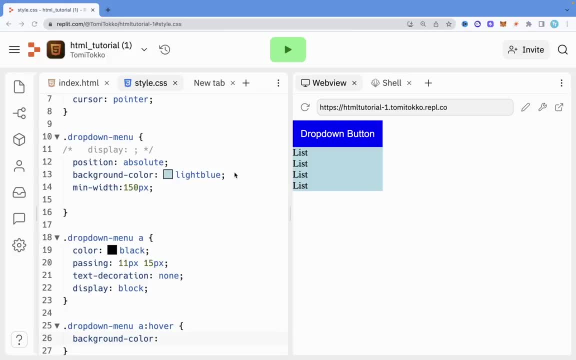 a particular background color when you know we over over every single list on it. So I'm just going to give a background color of you know, let's say white, Let's see how that looks like If I run this and I come over. you can see that when I over over each of 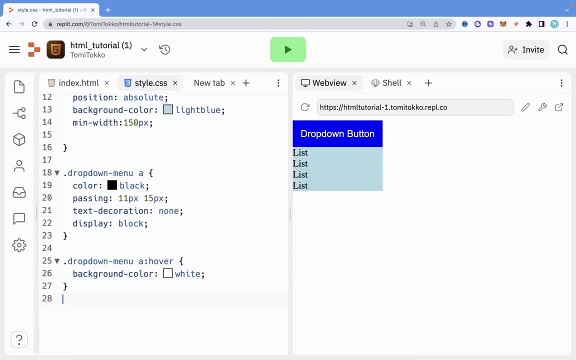 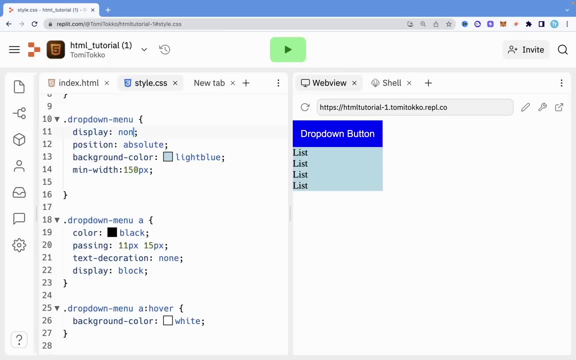 it. now it turns white. So what I'm now going to do is that I want this to only show. so first of all, let me make the display of this. let me remove that comment and make the display of this: none. So now you can see that. Let's wait for it. The list is not showing, no more. 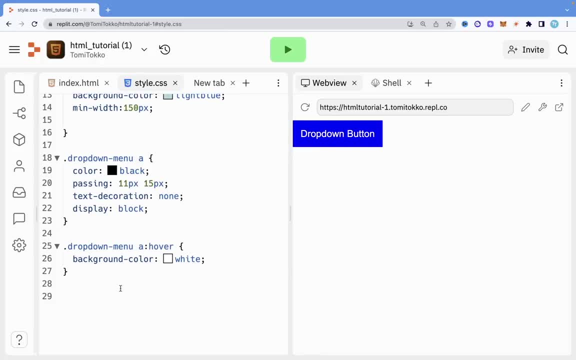 But I want this list to show only when we over on this. So what I'm going to do is to say that this drop down right here, which we already had from the beginning. So what I'm just going to do is to say that drop down. 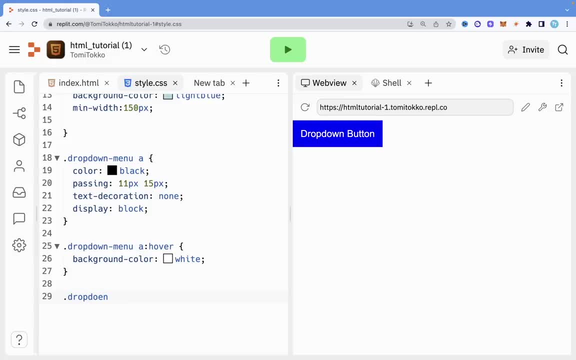 We're going to say colon. So instead of saying this, we're going to say over, And then we're going to say that is drop button. What we want to do now is to just basically: Okay, So thing that we actually need to do is to say the drop down over. we're going to say the drop down. 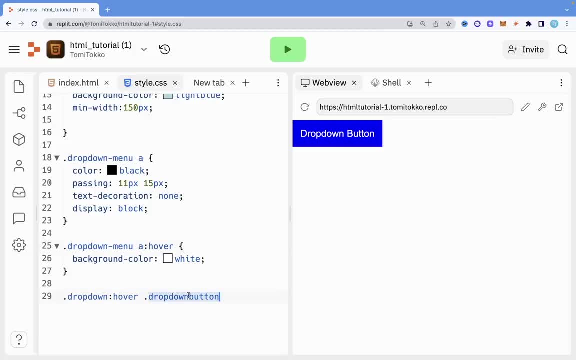 menu, so this whole menu. we want the display to be blocked, right. so we're going to say display block. now, when we run this, what we want is that when we hover over this, this should have a display of block. but this doesn't have a display of block. so the reason why this doesn't have a display of 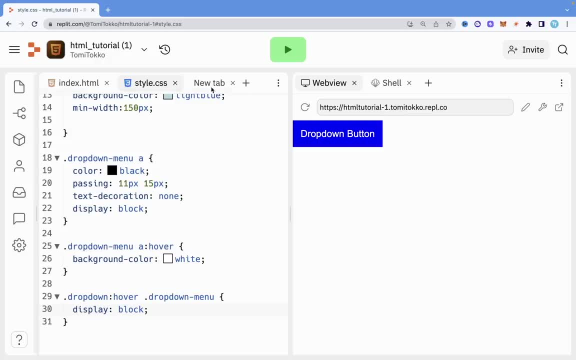 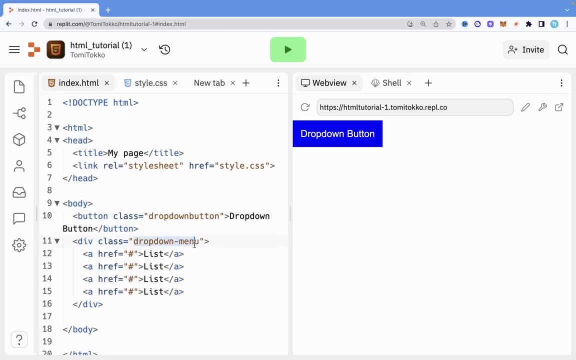 block is simply because when we come in here we want to have this div class to be, so we have to discard as a class of drop down menu we actually want, let's see, we want all of these to be wrapped in a div class. so let's say we cut all of this and say div right, and then we say this is like class. 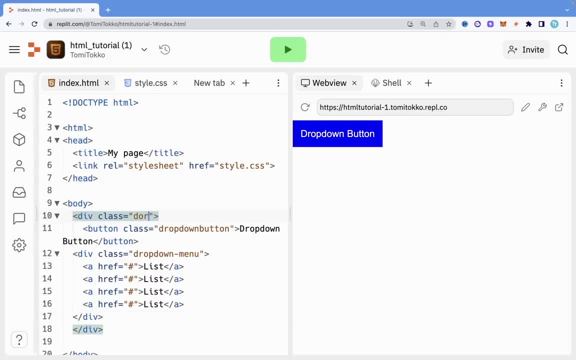 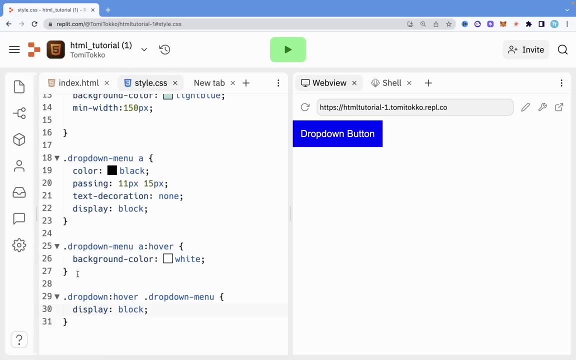 and then we just say equals. you know, let's say drop down. now, since we know we have this drop down here, we can just say, from drop down dot over, that means all of this: uh, colon over, we want to show drop down menu. now let's see what this does. so, as you, 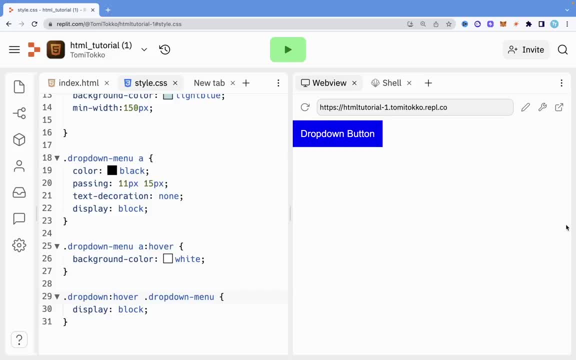 can see now, when we over on this, it basically shows that drop down menu. this is literally what we want to happen now. what we can do, we can just add, you know, a little bit of sauce on it and say the drop down, and when we over on it we now want to even change the color. 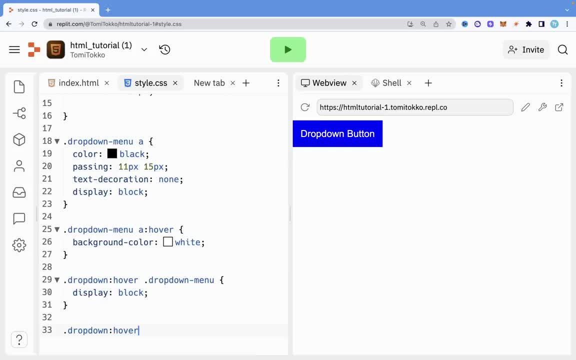 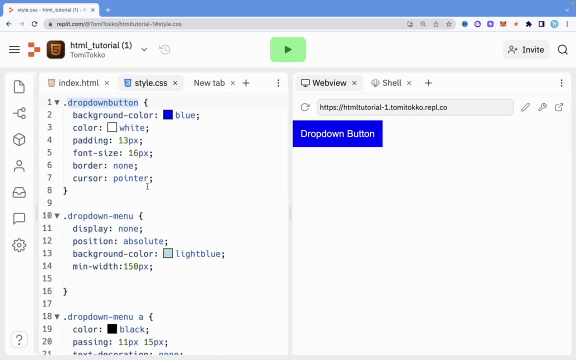 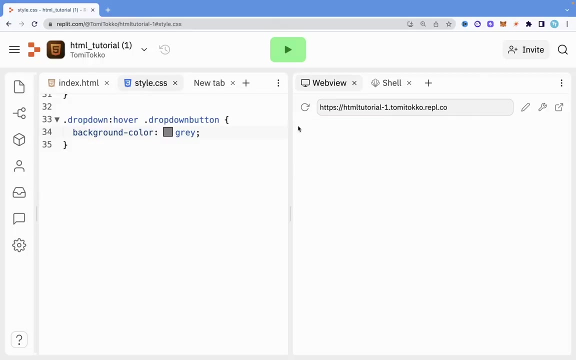 of this drop down button to maybe something lighter, so we can then say dot the button. so the class of the button is drop down button. we're gonna say dot the button. i'm gonna say background color. it'll be something like, let's say gray, let's try it out now. when we run this, you can now see that we have a when i overrun it. 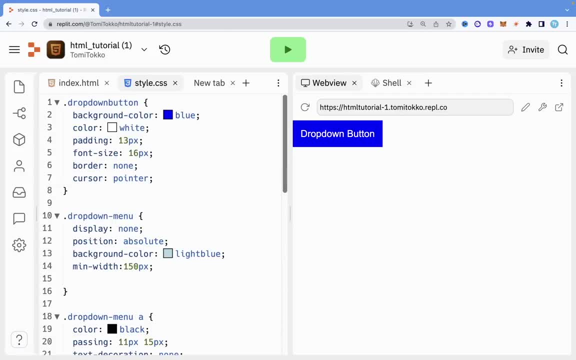 the colors change to gray and we have this basic list right here now. that is literally what we want to happen and that is what has happened. now we can also, you know, as you can see, everything is basically done successfully, but we can just come in here and under this drop down button, 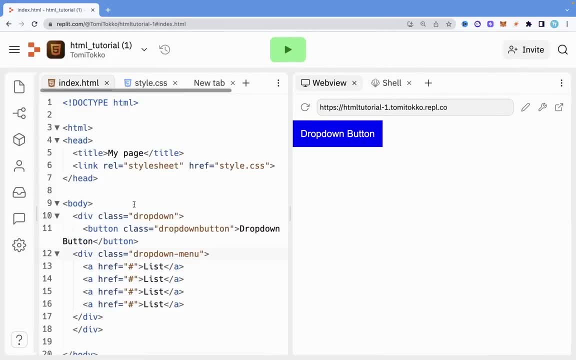 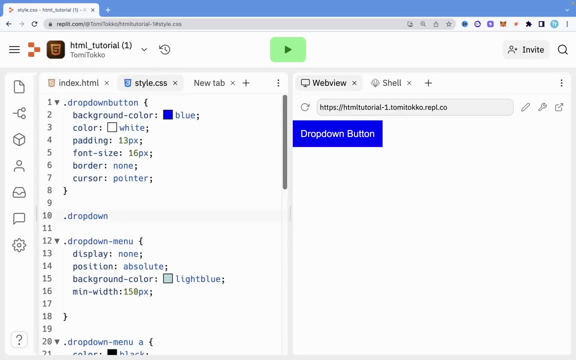 let's say we just want to add some styling to this drop down class. i'm going to come here and just say, dot, drop down. and i'm going to have it. let's say the position should be relative and let's say the display in line. so we talked about this when we were looking into all the different display and 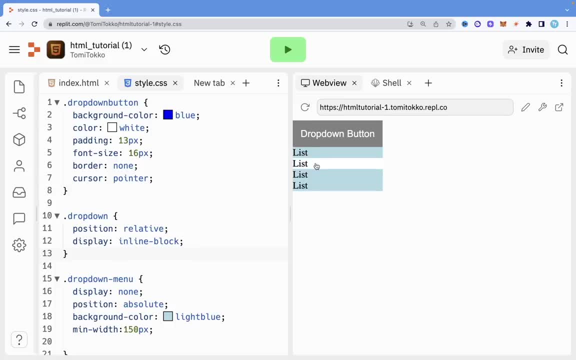 all of that in css. so, as you can see, everything basically works successfully right now. so let's, we can also have this list come into the you know center, if you want. that is, you know, optional, but, as you can see, this is a basic drop down and once we come over this, we can basically look at all of. 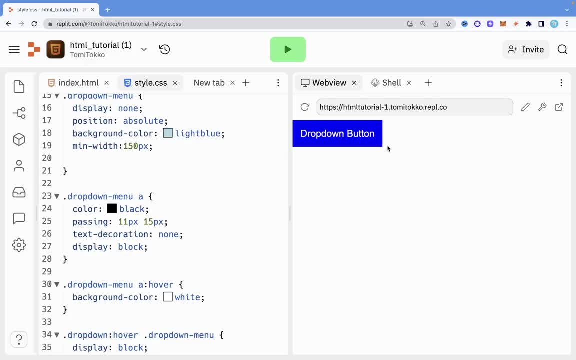 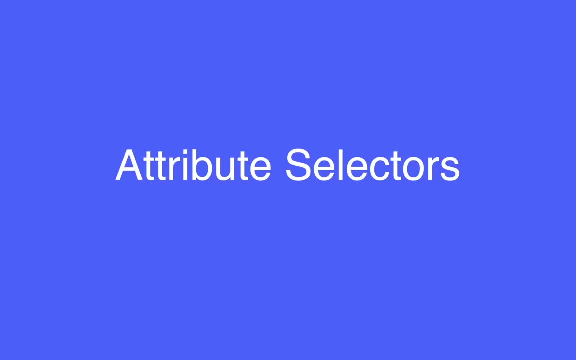 this and we can click on it and it takes us to a particular link. so, as you can see, all of that works successfully. does that to build a simple drop down with css. now let's look into attributes selectors in css. so let's get rid of all of this, and i'm going to go ahead and do that. so let's get. 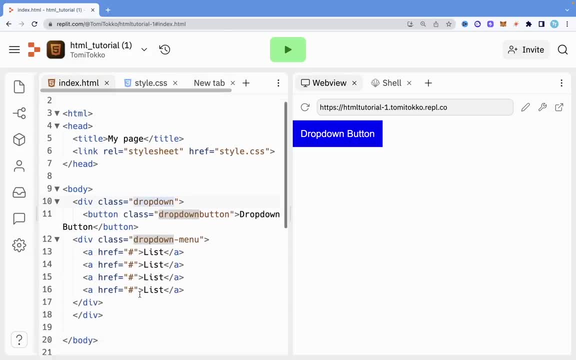 rid of all of this and i'm going to go ahead and do that. so let's get rid of all of this and i'm going to, and i'm also going to get rid of all of this, and let's say i have, let's see, a div class. 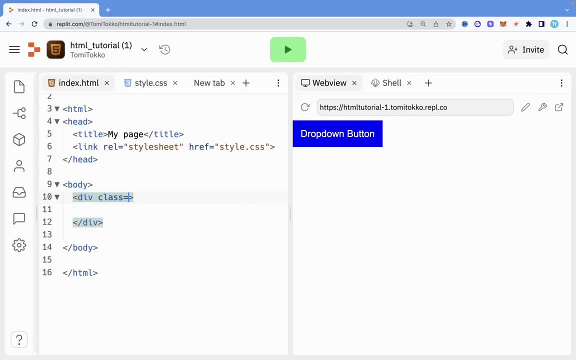 a div element that has a class of, let's say, test, and in here we then have a p that says i. so if i then run this, we just have a basic div class as a p that says i. that's that. so right here, let's say, we want to change something to this old div class, we instead. 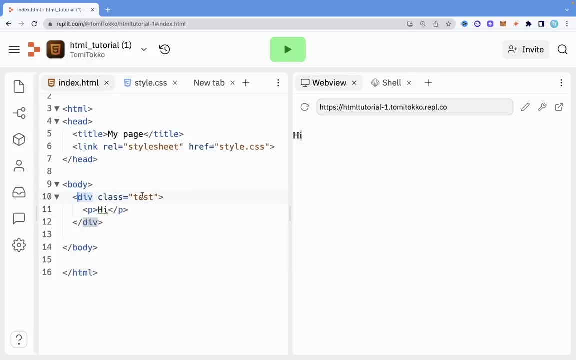 it using its element name. we can select it using its class name. so what we can do is to come in here now and we can just simply say div. so it's going to say any div that has an attribute named class. then we want to change the color to red. so if i run this, you're going to see that the 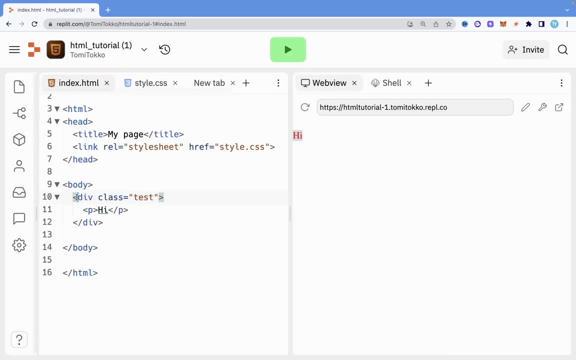 color of this changes to red. now this is because we selected the div that has an attribute of class. so that is a very basic way to actually select an attribute, but an element by an attribute. but let's say that you want to select with the exact value, for example. let's say i want to select 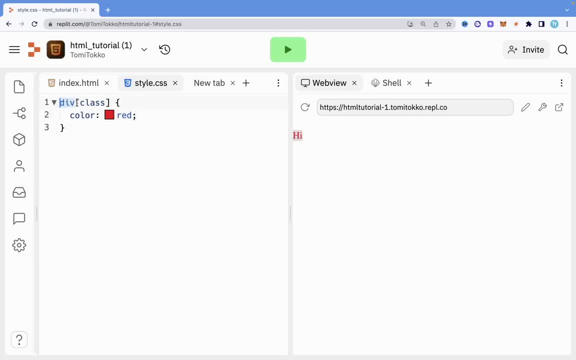 the element that has a div class- not have a div element- and it has an attribute right with a value of test. what i need to do is to say div and then i'm going to say class equals, i'm going to write the value. so this is still going to be i right and it's going to have the 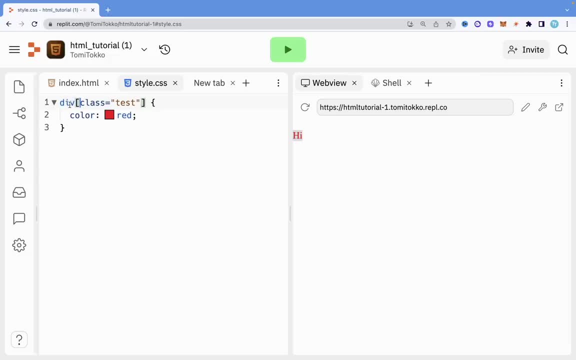 red. this is because it's going to look for a div class with a div element with a class named test. so if you come in here, you're going to see that we have a div element with a class named test. imagine i just remove t and i say test. now this is not going to be red, no more. it's just going to be. 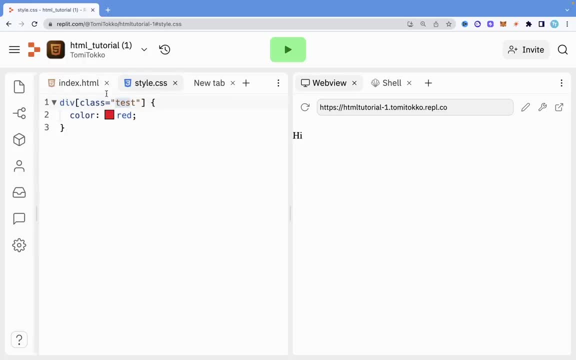 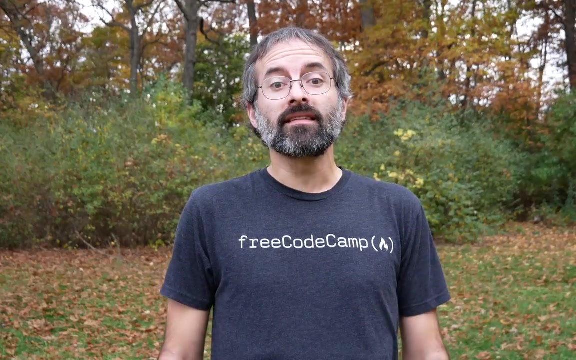 black, because that is not true for this particular condition. so that is a basic way of you know selecting with the value. so that's how to use attribute selector in css. now that you know the basics of html and css, i'm going to teach you how to code in javascript. 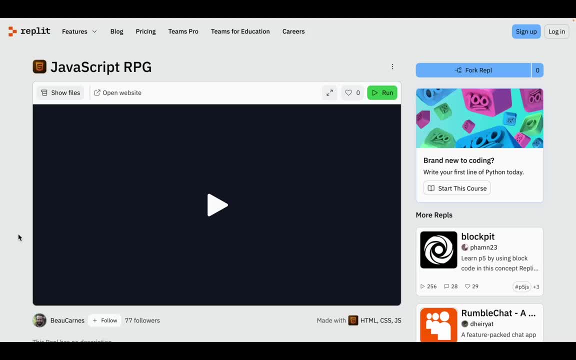 you're about to learn all the basics of javascript programming by coding an rpg game line by line. this way of learning javascript will help you understand better how everything works together. so if you're following along, you're gonna want to know how to code in javascript. so 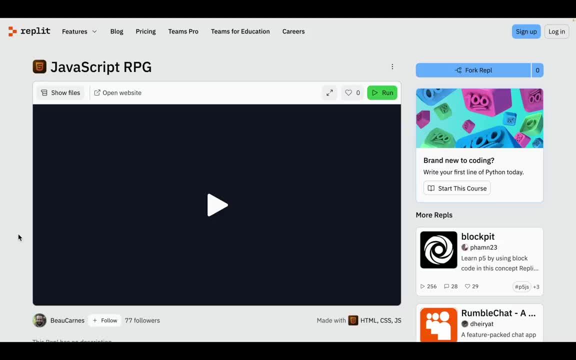 you'll be able to record. you'll be able to code each line right before I do, based on my instructions. There is some starter code, So go to the link in the description and it should open up just like this, And then you can fork the REPL This will give you. 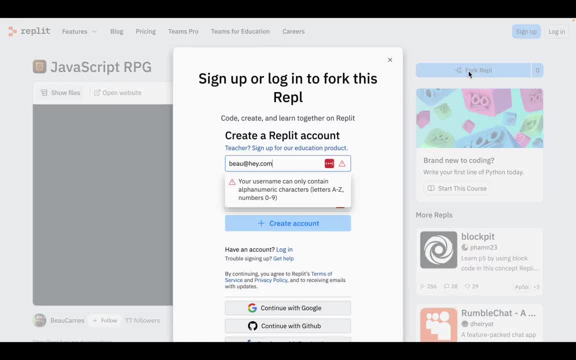 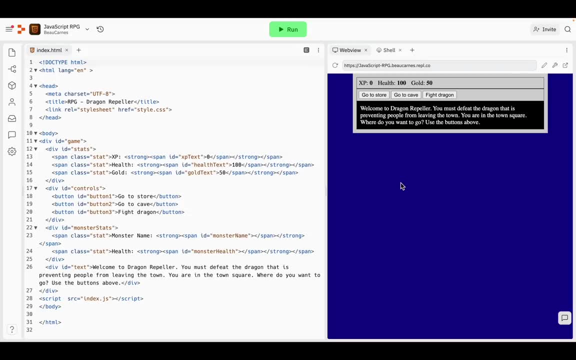 my starter code. So just click fork REPL And then you'll have to sign up or log in if you haven't already. So this is the starter code for the RPG. I've already provided the HTML and CSS And we're now going to create the JavaScript. So let's look what the start. 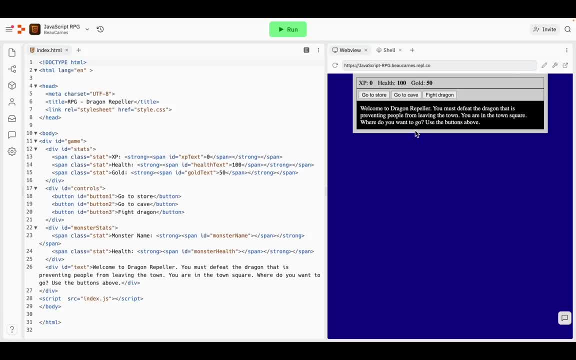 code looks like So when it's loaded in the browser looks like this: So you can see it's a text based RPG and it will give you a description of what's happening right here And then you'll have a few different options in these buttons here And it's going to keep track of your 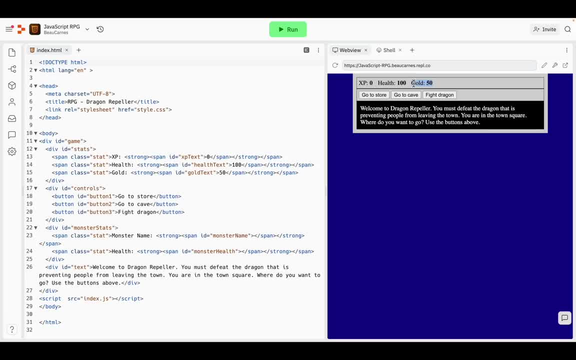 experience point, your health and your code, your gold. Now, right now, none of these buttons do anything. we still have to create that And all. Speaker 4. Speaker 5: this is just hard coded right now So you can see in the HTML. we've already learned about how to. 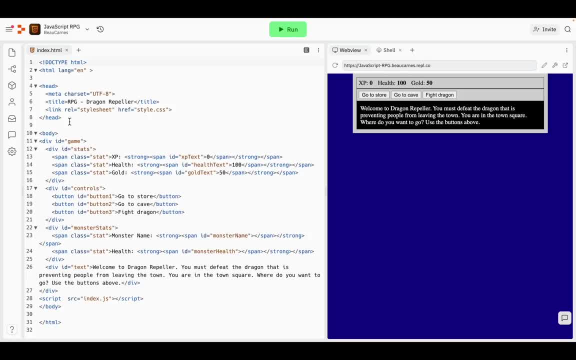 set up an HTML page, So a lot of this should look familiar to you. So you can see, we have a div full of the stats at this. that's this top div. And then we have a div for the controls. Those are these controls here, And then we have this special one called monster stats, And this is not 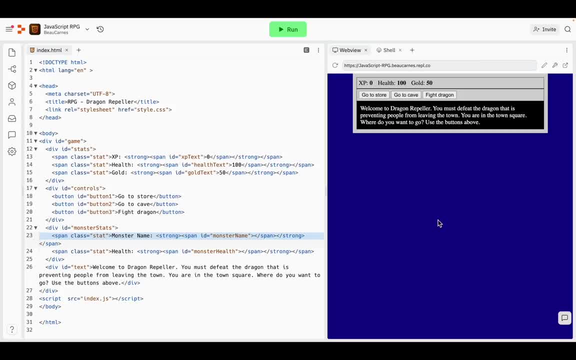 showing up yet because we're using CSS to hide that for now, And we are we're also- we're X- basically hiding this whole section, the whole monster stats section, And because that will only appear if you're fighting a monster, And then we have our main text here And you can see. 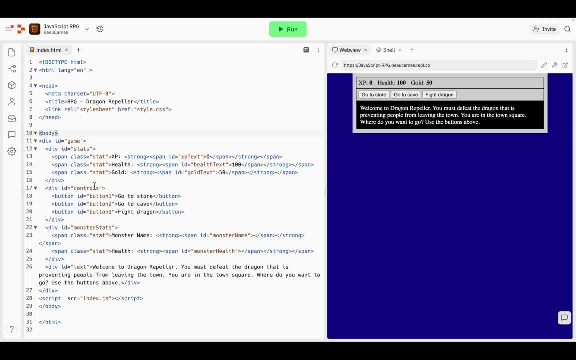 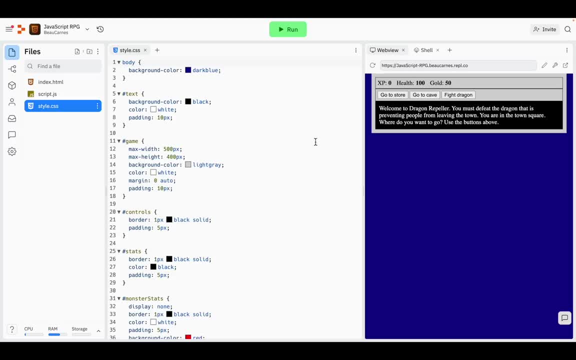 we have all these elements of the page, but nothing is happening yet because we haven't created our JavaScript. But let's look at the CSS really quick. So this is also provided And it's basically just styling the page how you can see it, And one thing to look at is the monster stats. 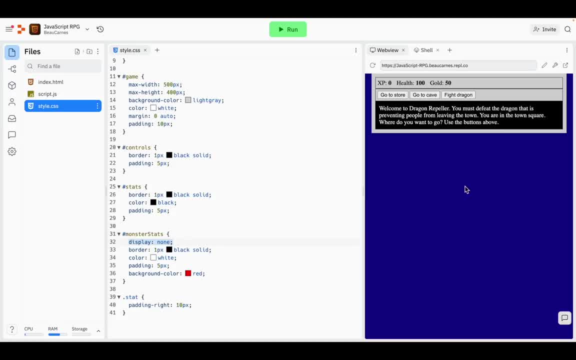 which I already talked about. Currently it's set as display none. it's only going to show the monster stats if you're fighting a monster. but we're not yet fighting a monster. we haven't even implemented that feature of the game yet. So now we'll go over to our JavaScript file. So if you 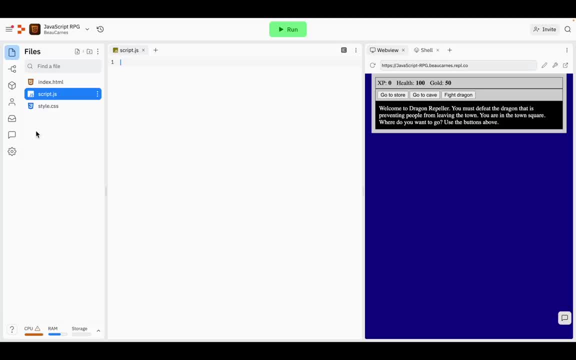 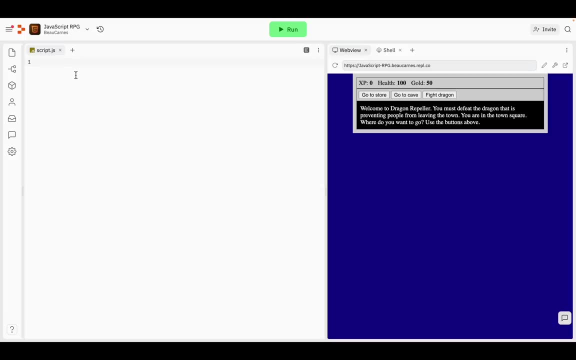 want to just kind of explore the HTML and CSS a little more to understand. you can, but we're now going to code this game from scratch And you are going to code the game step by step based on my instructions. So I'm going to just close this section here. I will zoom in just a. 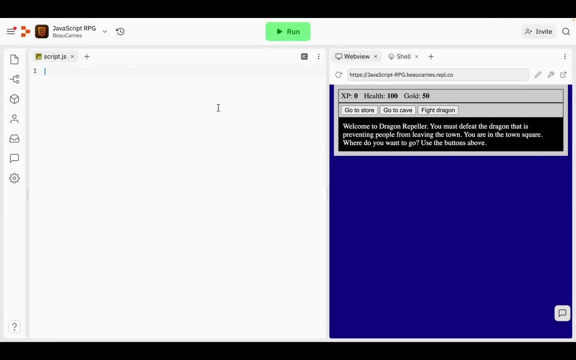 little more so you can see the code a little better. So the first thing I'm gonna have you do is create a variable, But first let me show you how to do that. I'm going to do var, XP equals zero, And we'll zoom in one more time And I can just put a semi colon here. So 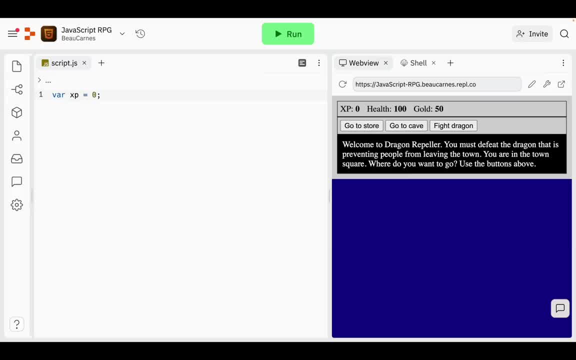 to keep track of the players experience points, we declared a variable called XP and then we've assigned it to the starting value of zero. So I want you to follow this example and create another variable to keep track of health and start it at 100.. So hopefully you're. 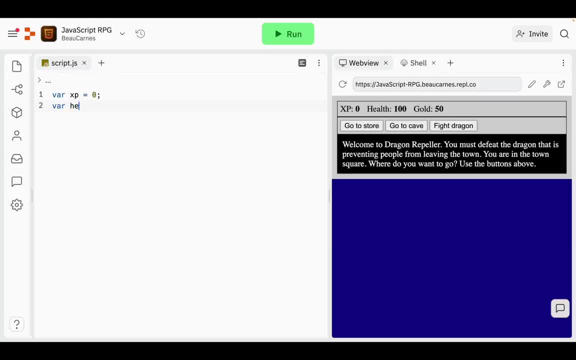 following along. you're trying it before I show you, so now I'm going to show you. var. health equals 100.. And so you can see we follow the same pattern. So this is so. we say it's a variable with var, then we say the variable name, and then we assign it with the equal sign, And then this is the. 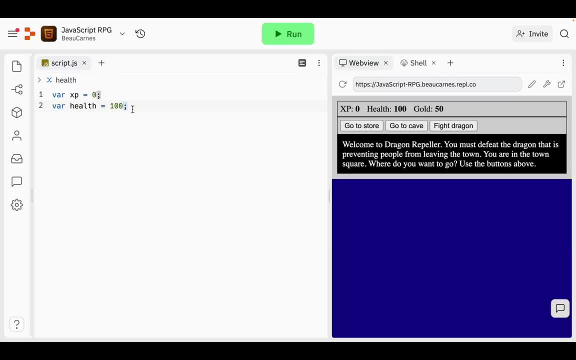 value that we're assigning, And then the semi colon. here in JavaScript, semi colons are optional, So you can use a semi colon to signify that it's at the end of a line, but you don't have to do it. But for now we're going to use semi colons. So now, now that you have, 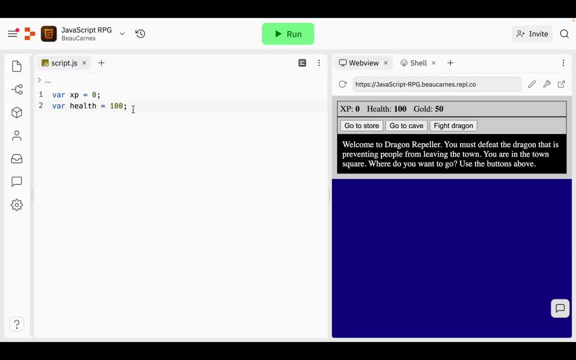 the pattern down, see if you can create another variable called gold and set it to 50.. Okay, now we're going to create another variable And this is going to be called current weapon And we're gonna set to zero. But when a name has two words, 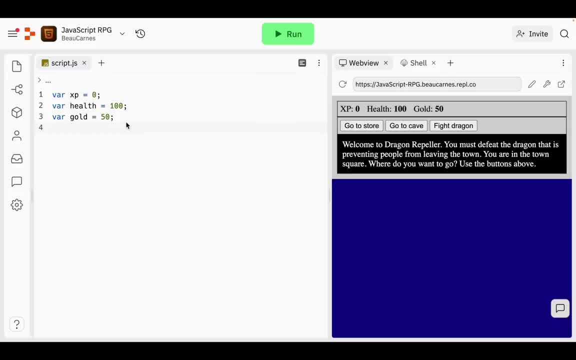 the convention is to use what's called lower camel case, which is how you do, is the first word is all lowercase And then the first letter of every preceding word is uppercase. So we'll do current, So we'll do var. current weapon equals zero. So we've been declaring all our variables. 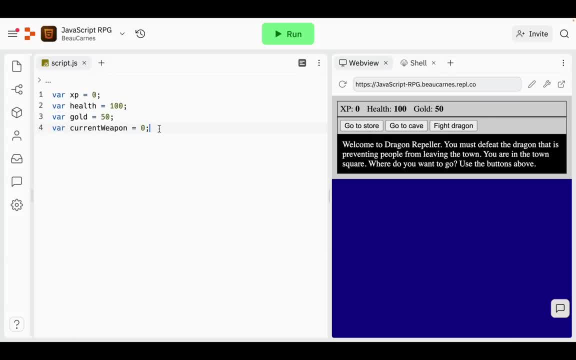 with VAR. However, in modern JavaScript, it's better to use let instead of var. you can- actually there's three ways to to declare a variable. you can use var, let or const. it's better to use let instead of var because it fixes a number of unusual behaviors with var that make it difficult to 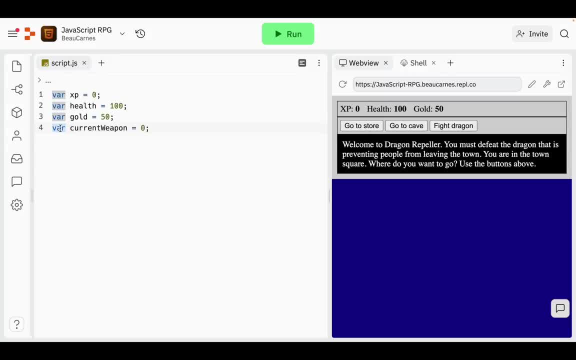 reason about. So let's change all the bars to let. And one quick way to do that in Replit is I can highlight the first var and either do command or Ctrl D to highlight the next, and every time I press Command or Ctrl D it highlights the next instance of our. and now I'm actually using multiple 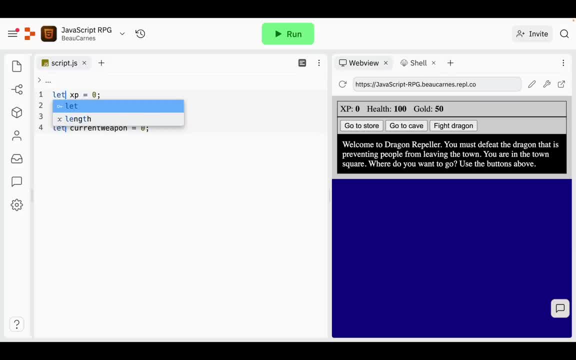 cursors And I can just type in all at once, So I change them all to let. now let's declare variable without a name, All right. so now let's go ahead and type in a variable without a name. And now let's. 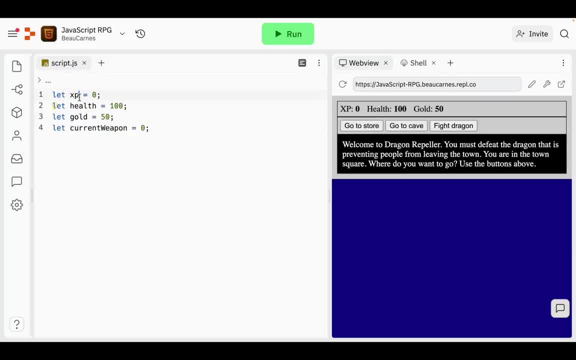 initializing it. So in every one of these examples we've initialized the variable, that's this part where we set it to equal something. But you can create a if you just don't put the equal- a number, equal value- you can declare it without initializing it. 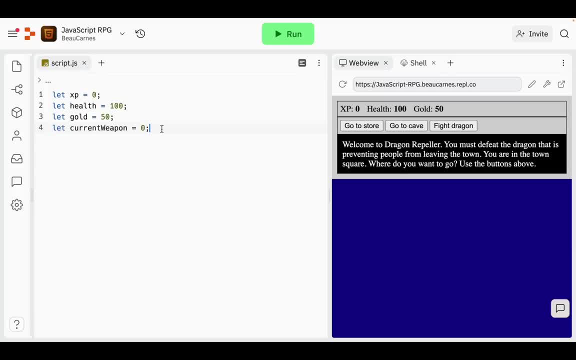 So, using the let keyword, let's declare a variable called fighting but not set equal to anything. So it's just like this: let fighting. Now we'll do the same thing with variables for monster health and inventory. It's common to just create all your variables up front at toward the beginning of your program. 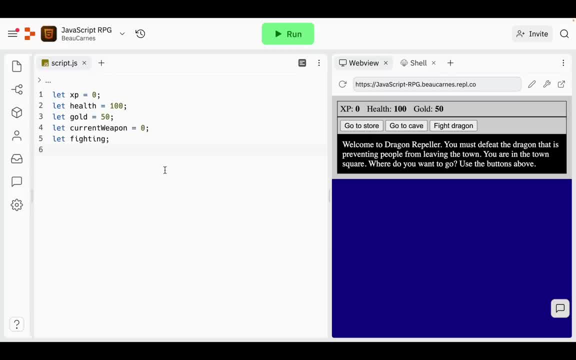 Before you start using them. you want to have them declared before you use them later in your program. So we'll do let monster health and let inventory. Now let's set the variable inventory to equal a string stick. Strings are a group of characters surrounded by quotation. 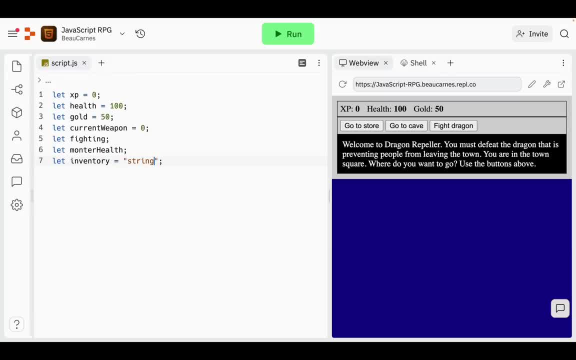 marks. So we'll do equal string Or equal stick And we use double quotation marks. But you can also use single quotation marks as long as the quotation marks are the same. Another thing: you can also use back ticks, but you just have to make sure the at the beginning and the end are both the. 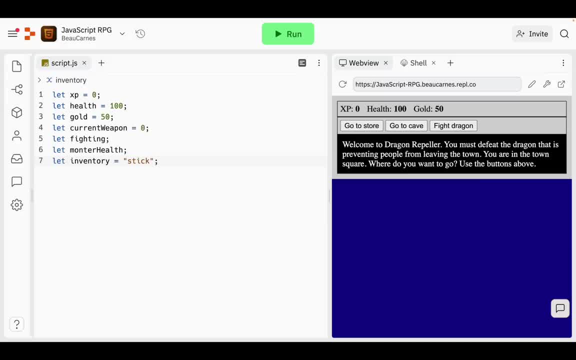 same. For now we'll just use double quotation marks. Now, right now the inventory is just a single thing, a stick, but the inventory can store multiple items. So we're going to change the value of inventory: inventory to be an array with the item stick, dagger and sword, And array is basically just. 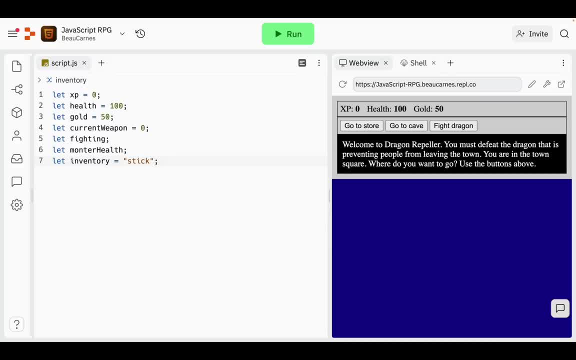 a, a list of different values. you can store multiple values in an array And you create array by putting brackets around the list of values. So it's just gonna be like this. So the first item we're going to put the bracket here, stick, and then we will have 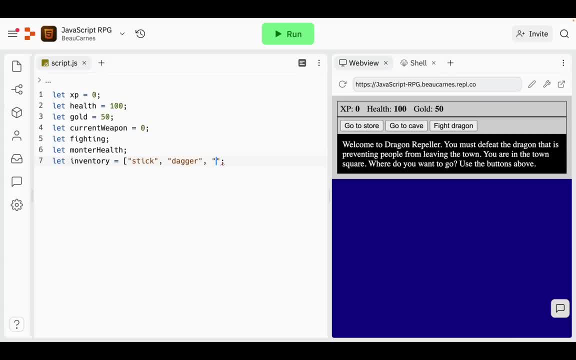 dagger and sword And then we do an in bracket there. So now we've created an array of three strings. Now, putting three items in this list was just an example. So for now let's just start the player with just the stick. So we're going to keep this as an array, but we only want 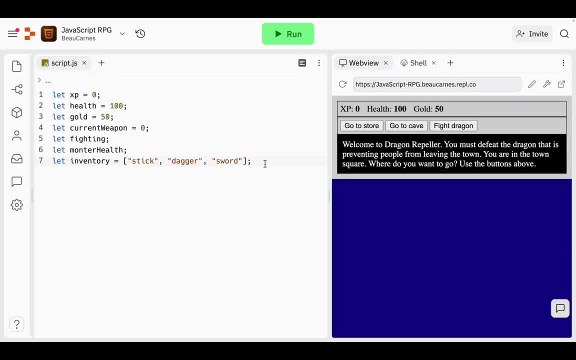 one item. So we're going to delete, dagger and sword those items And then later that will give the player an opportunity to add more items to the inventory. But it has to start out as an array if we want to add elements to the array. In order to update HTML elements on a web page on an HTML page. 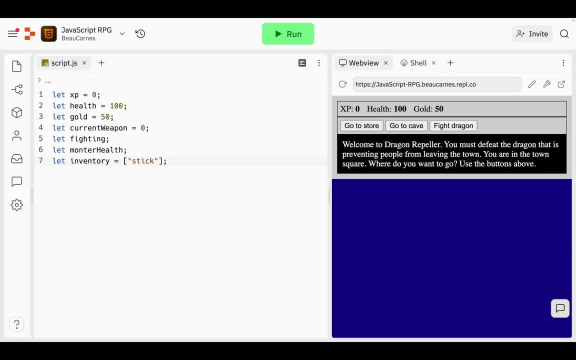 you need to get references to them in your JavaScript code. So here's an example. This is not the one we're using. I'm just giving you this as an example, where we can. this will get a reference to the HTML element with an ID of L, because this is the 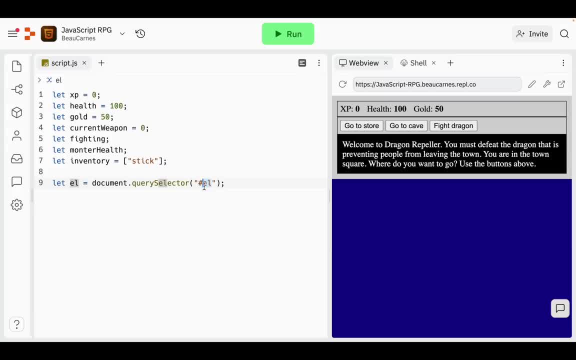 CSS, CSS selector for ID and it's going to have the ID of E, L And we're going to store that, that HTML element, in a variable called L. What I want you to do is update this to get a reference to the HTML, the HTML element with the ID of button one, and assign. 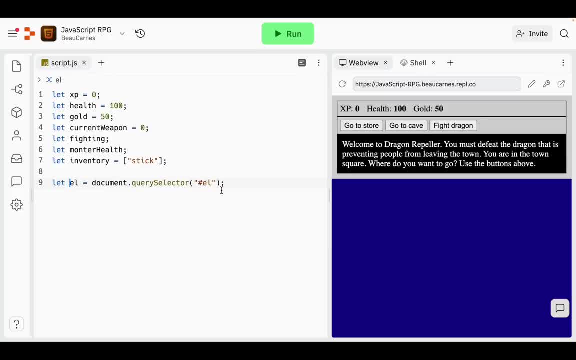 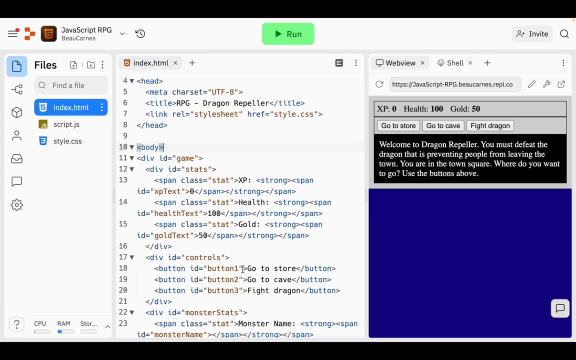 it to a variable with the name button one. So basically we're just going to do button one and button one. let's just look over our HTML really quick So you can see where that is. if we go to the HTML and we can see here button ID of button one, that's this one where 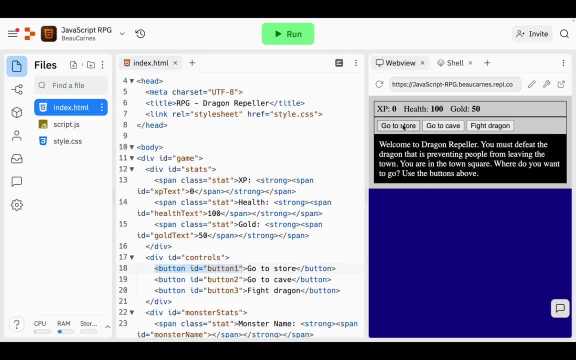 it says go to store. So now we're getting access to this element And we can do things to it, like we can change the text in the element or basically do whatever we want using JavaScript, once we have a reference to that element. So we'll go back to our JavaScript. 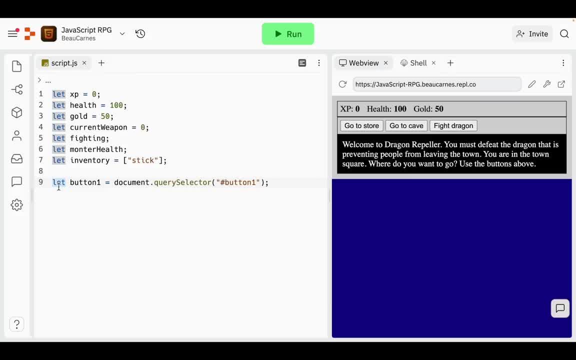 And now what we're going to do is change this let to const. So I already told you earlier that you can create a variable with var, let or const, So var allows the most changing, basically it's. so you can basically do anything you. 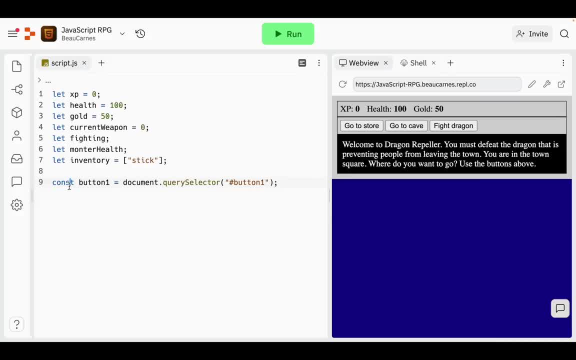 want with a var later, but you may. but that could open yourself up to bugs And const. it means that is the least amount of changing. Once you declare a variable as a const, you cannot update it. So we do. we are going to want to update the XP, the health, the gold, But now once 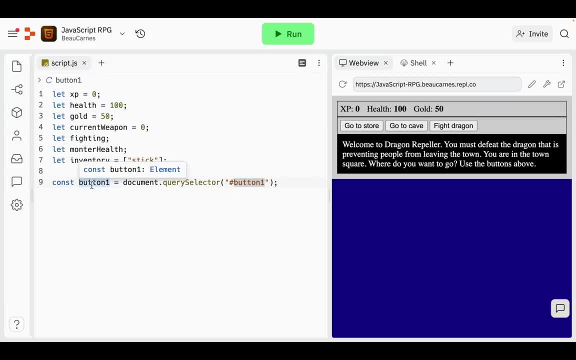 we get access to this button. we're never going to want to update this variable. we're not going to assign button one to button two. it's always going to be button one. So that's why we can use const. You want to use const anytime you're creating a variable. that should. 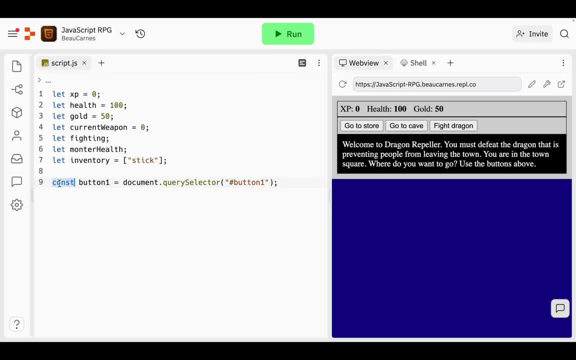 never change. if the value is never going to change, you declare the variable with const because it's a constant. So now we want to. we want to get access to a bunch of other elements on the website. we're going to basically get access to elements with all of these different. 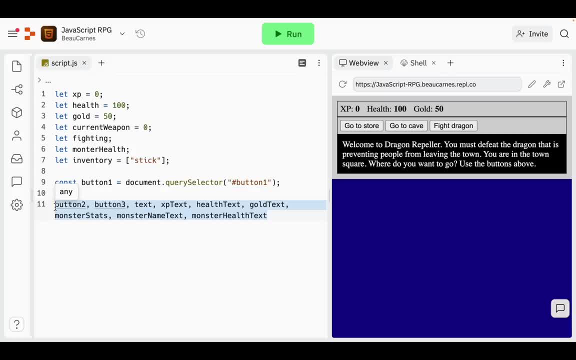 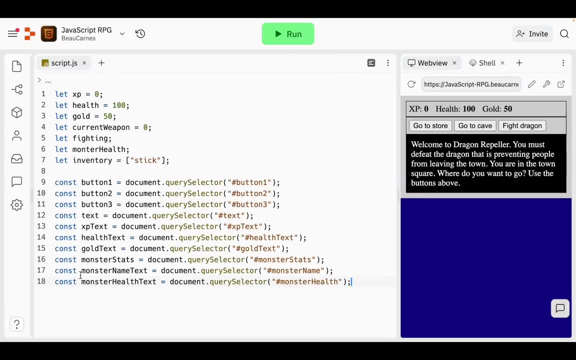 IDs. I'm just going to paste it in here, But you can give it a try yourself if you want first. Okay, so we got these all pasted in. So basically, we have access to all the different elements on our website that we want to update using JavaScript. So now, instead of updating, 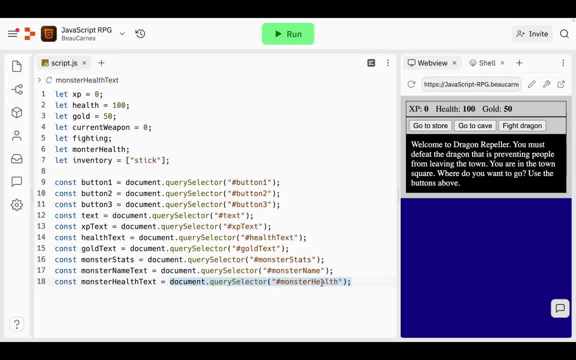 instead of typing this whole thing, and every time document query selector and then the ID, we can just refer to the variable. Okay, now we're going to make a comment to describe what the next few lines of code will do. comments can be written with either two forward slashes: 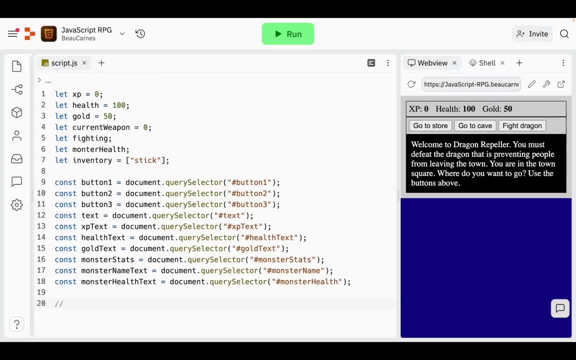 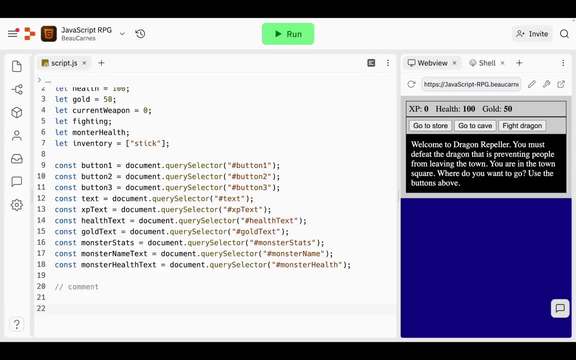 or with a multi line sequence. So if you're going to make comments on one line, it can just be two forward slashes And you can do comment. Or if you want to make a multi line comment, you can use slash star at the beginning and star slash at the end, And then you can. 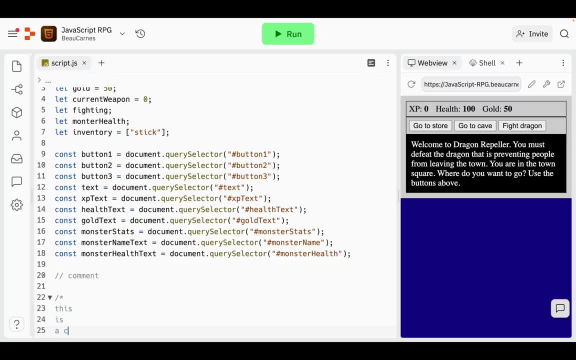 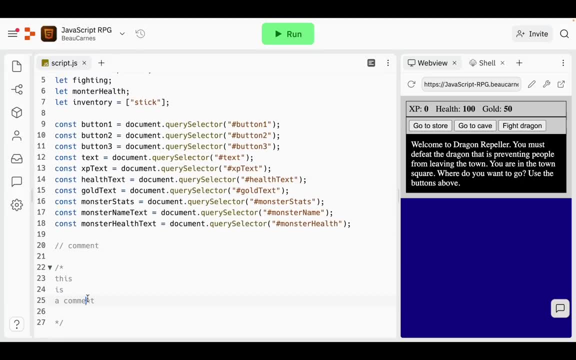 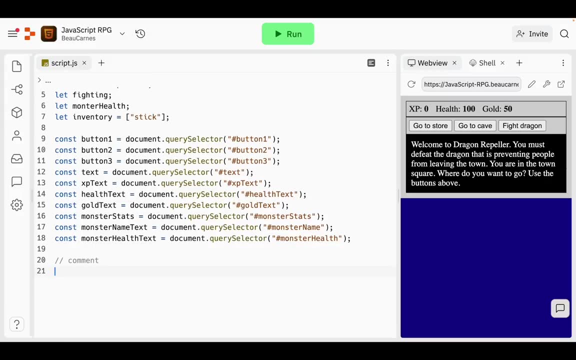 say this is a comment And then you can see that the comment. the code editor automatically makes comments gray And because this is a multi line comment, you can see it's all gray here. So basically we just want a single comment that's going to say initialize buttons. 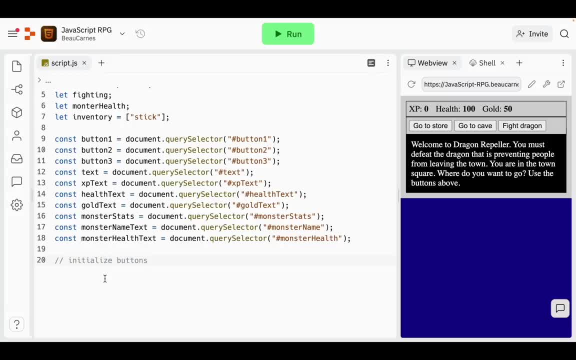 Okay, so now this indicates what the next part of code will do. So let's designate what the first button in the HTML does by setting the on click property of button one- And we're going to set that property to the function name: go to store. So here's an example of how you would do it for a. 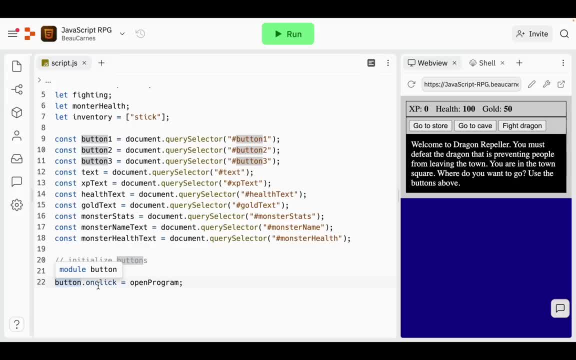 different button. So this is just a generic button And if you want to make the button open a pro, call the function open program. you could do it like this, But we're trying to make it so button one, we'll call the. 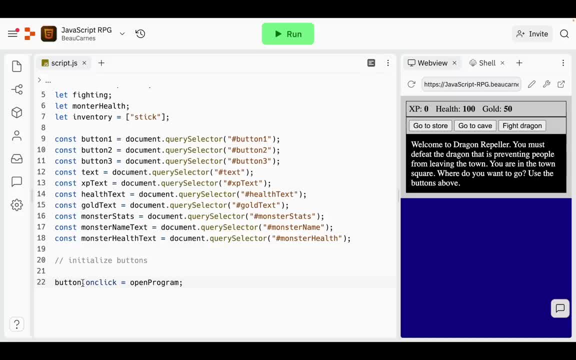 go store function, which is a function we'll create later. So basically it's gonna be button one and just go store, And so we can see that the button one already says go to store. So now when we click the button one, it's going to call this function which is going to make our game go. 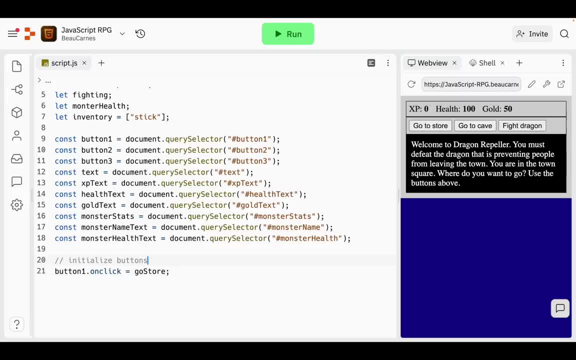 to the store in the game. Now we're just going to follow the same example to set the on click property of button two and button three to be go cave and fight dragon. So I can just actually copy this line, paste it in here. So this will be button two, button three and there'll be go cave. 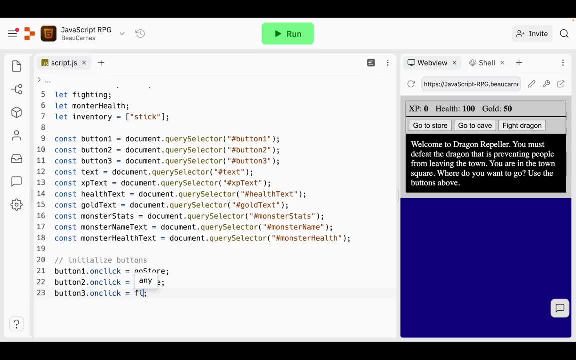 and fight dragon. Now we're going to create a function, So we already made it, so these functions will be called when you click the buttons, But let's now create these functions that are called now. functions are just a group of a section of code that you can run over and over again every time you call that function. So it's a way. 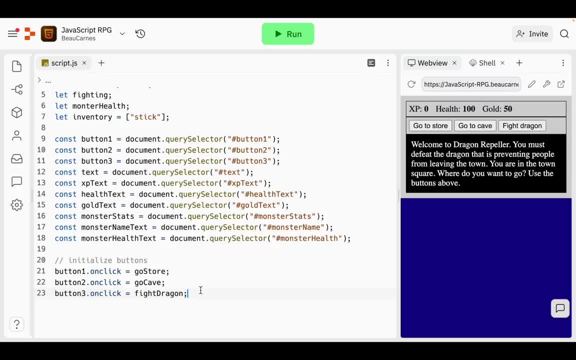 to repeat, easily repeat code. So every time that function is called it just runs all those lines of code in that function. So let me show you how you would just create a generic function. So see, you always start with the word the keyword function And 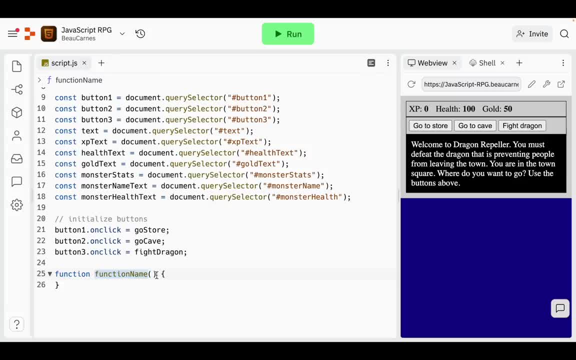 then you do a space and then you put the function name, which can be anything, And you're always going to have two brackets or two parentheses, and then these curly bread brackets, And inside the curly brackets, are where you put the code that's going to run when you call the function. 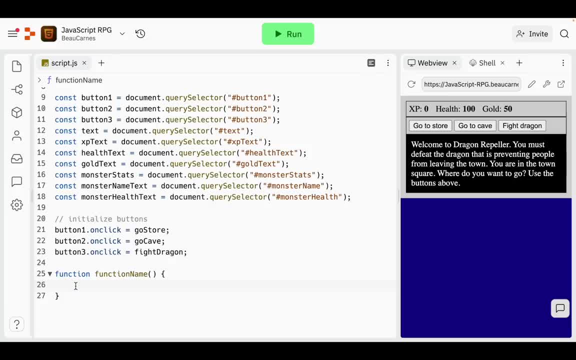 So right now, instead of creating the function called function name, we're going to create a function called go store. So that's pretty simple: Just do go store. That's what it's called now. Okay, now let's make this function do something. We're just going to basically do some example code really quick, But 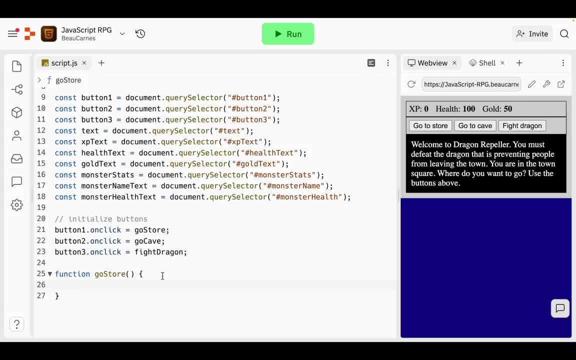 we're going to make the ghost store function output the message going to store to the web console. So basically we do console dot log And then in parentheses we put the string going to store, just like this console dot log. So it's going to log it to the web console going to store. And 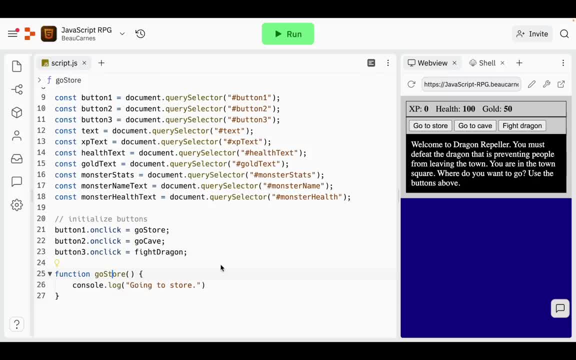 that's it. Now we have something that this function will do, And now we've actually done enough to test our program out. So what now? when we click go to store, it's going to put going to store in the console. Now, where's the console? It's not this, this isn't the 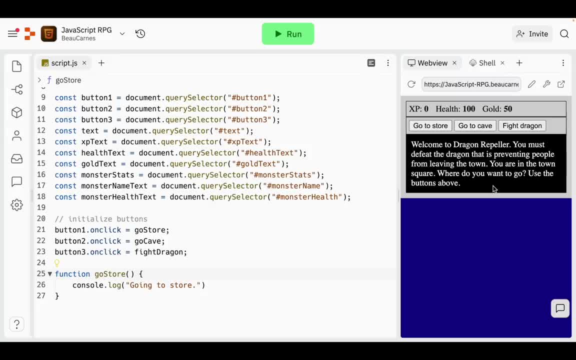 console. this is part of the website, So to get to the console you can do it either from your browser's dev tools or right in Replit. we can click this, this thing, this, this wrench here, toggle developer tools, And now down here we have our console. So click the Run button And 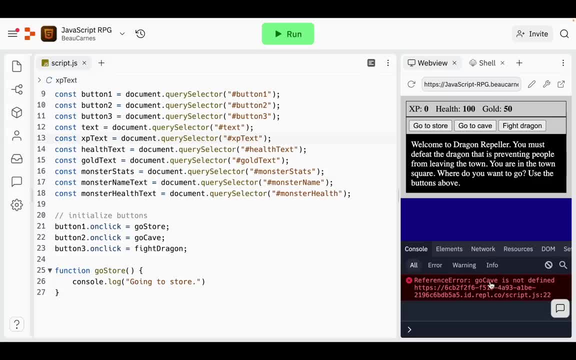 now we do get the. this go cave is not defined because we haven't created yet, But we still should. still should work. I'll click go to store And it says going to store right in the console. So let's create a go for. 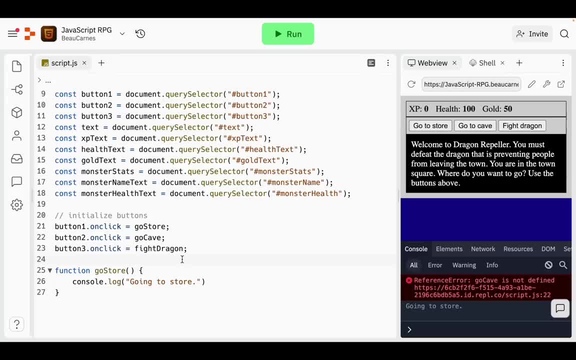 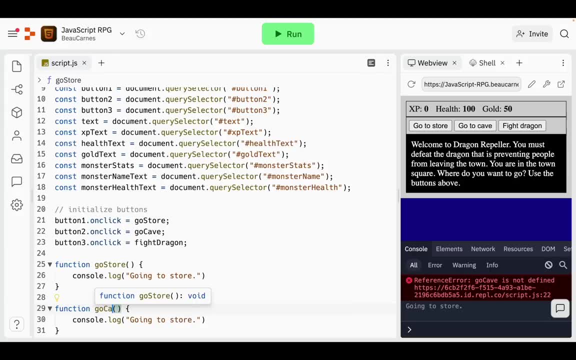 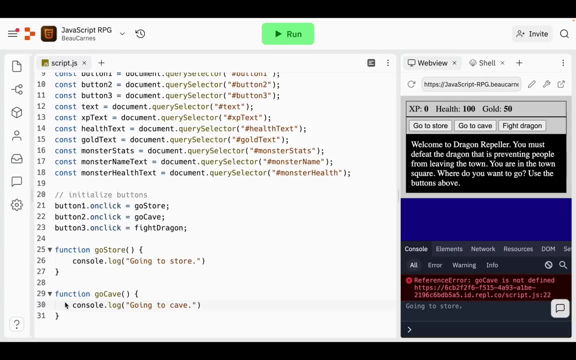 cave function. that will console, that will log to the console going to cave. So I can just copy this and just paste and put go cave going to cave. And then we'll just create a fight dragon function that will say fighting dragon. So we'll just print, paste in another one here And this: 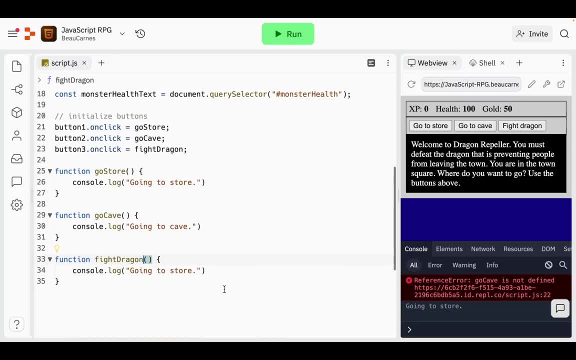 will be called fight dragon And it'll say fighting dragon. And now we should be able to run this And we don't get an error down here, because all the functions are defined. So go to store, go to cave and fight dragon. we can see in the console. 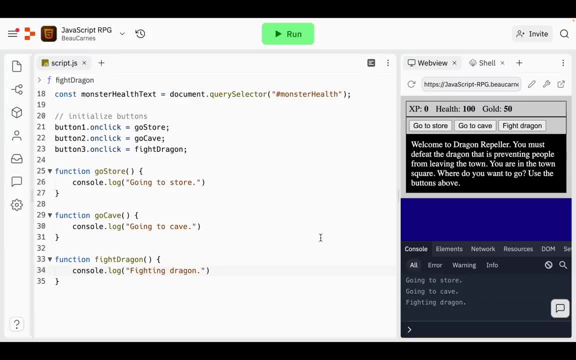 those are appearing. Okay, well, let's do some refactoring. refactoring is when you change code to improve code or make it better that you've already created. So we're going to change the go to store function. This was just kind of to demo it. 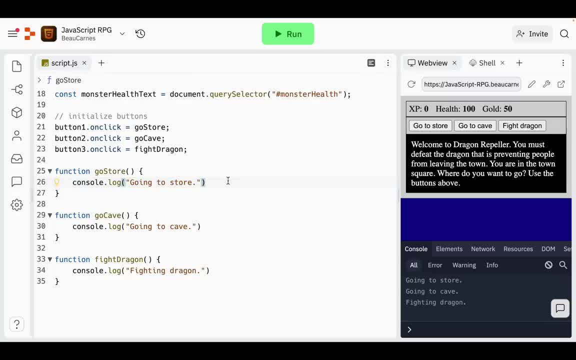 we're not actually going to console, going to store, And we're not going to log that to the console, Because when people are playing the game they won't actually be seeing the console. So when we, when a player clicks the go to store button, the buttons in text in the game should change. 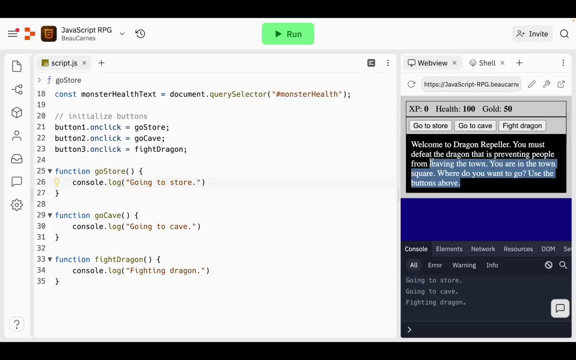 So what's in these buttons to change and what's in this text up here? it should tell you what's happening at the store right down here. So we're going to remove the console dot log. we're going to remove the console dot log and we're going to remove the console dot log. And now, when you're 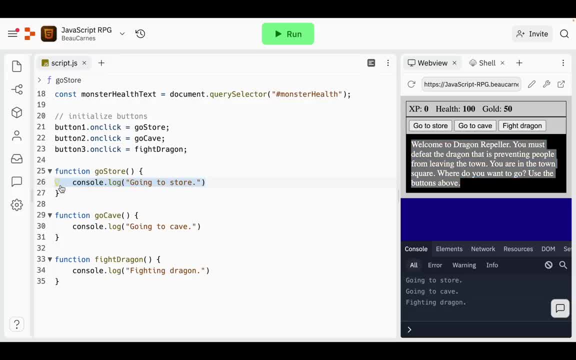 this, And we're going to add a new line of code inside the function that updates the text of button one. So it says I 10 health for 10 gold. So I'm going to delete that. And then let me just show a quick example. We're not going to use this one, But this is how you would update the text of: 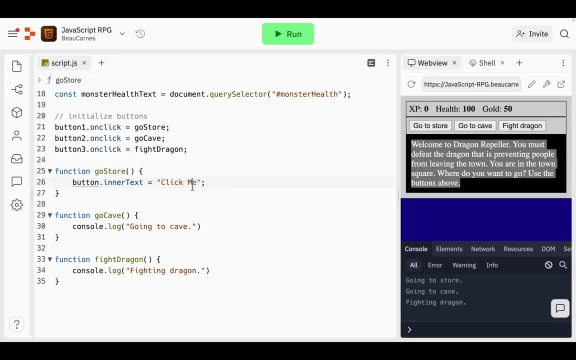 a button, button dot, enter text and then set what it equals. And we're going to make the button one say I tingle by 10 health for 10 gold. So we just change this to button one And then we just change the text in here. the inner text is now going to be by 10 health, And then we'll just put in. 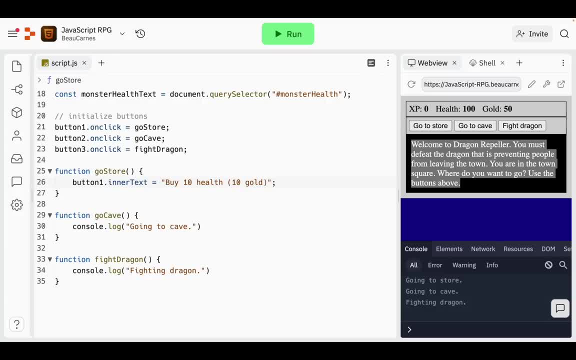 parentheses: 10 gold. Now we also want the text of button two to say: I weapon 30 gold and the text of button three to say: go to town square. So basically, you're going to go back to where you began, So I can just copy this: 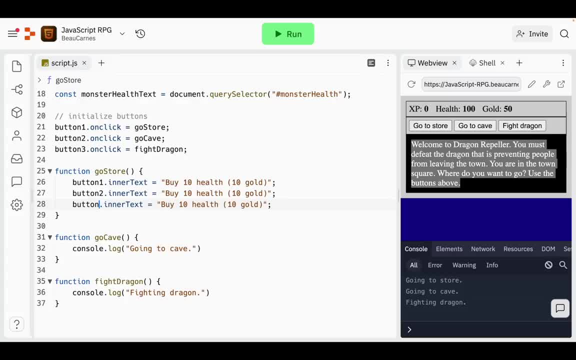 And then we'll do button two, button three, And then this will say: by weapon for 30 gold and go to town square. So now that the text on these buttons have changed, the on click properties on the buttons should change. So 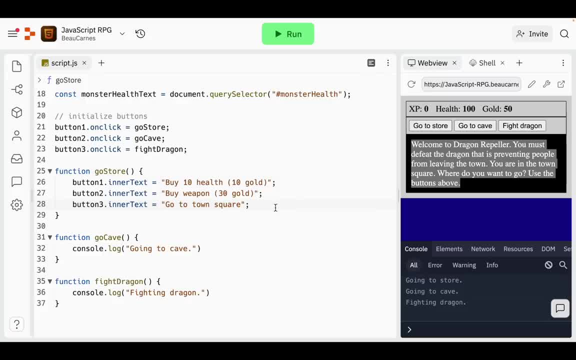 inside the go store function we'll update the on click property of all three buttons. the new function should be by health, by weapon and go town And you should already know enough right now to be able to do that all on your own. But basically I can just copy the initializing. 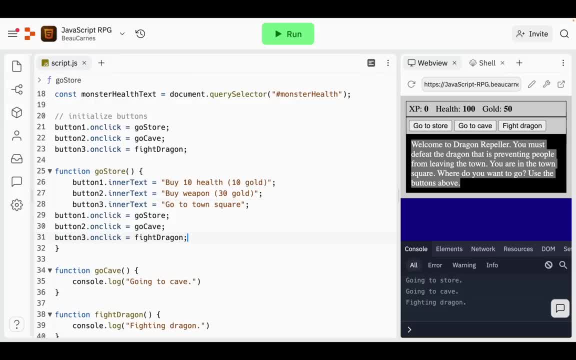 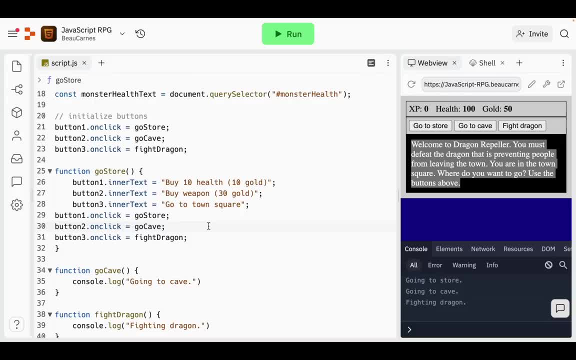 to be the same amount Now. indenting is actually going to be the same amount Now. indenting is actually optional in JavaScript is just to make sure that your code is more readable, But it's still good to do. any time something's in a block of code and these curly braces, you want to indent it the same. 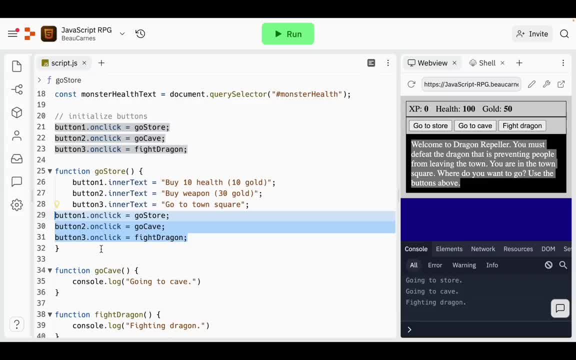 amount, even though it doesn't actually impact how your code's working. So I'm going to highlight everything And now I can just press tab and we'll indent everything at once. So the button one is now going to say by health, button two, or is that going to go to not say 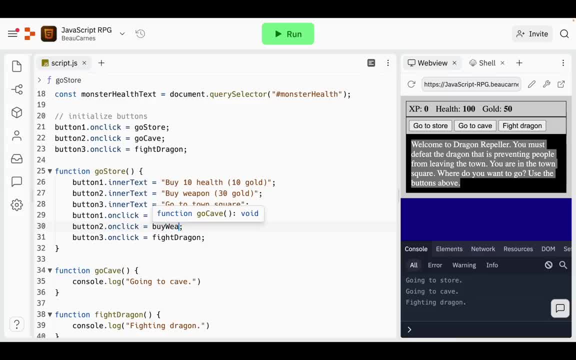 by weapon. This is the function that's gonna be called and then go down. Now we're changing the inner text of the buttons, But we also want to change the inner text of this section here. That's the property, This is the has the idea of text, And we want to say: 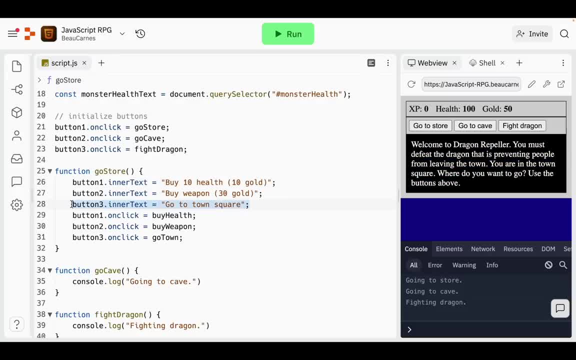 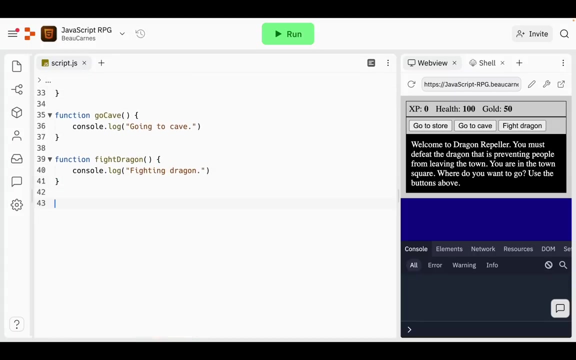 you enter the store. So I'm just going to copy this again And just say text: you enter the store And now let's create three new empty functions called by health, by weapon and go town. So we're going to create a function. you have to use the keyword function. 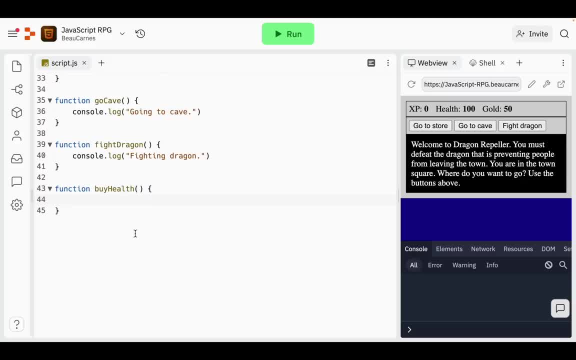 by health parentheses, and that's just gonna be an empty function. And then we'll do another one, and another one. so by weapon and go town, And at this point we can test it out. So I, if I click, Go Store. 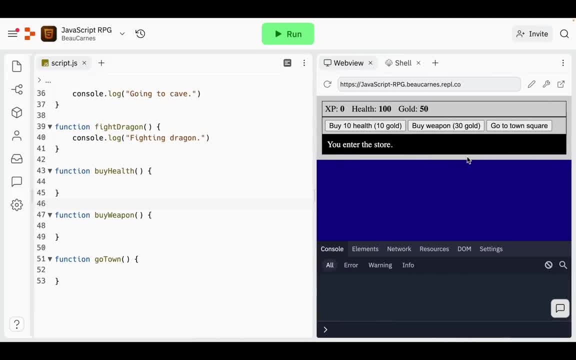 I'm going to just move this here so you can. the button still stay in a row here, So you enter the store And unfortunately can't go back to the town yet. But we were able to enter the. but we were able to enter the store. If I refresh this, I can try it again. Go store. 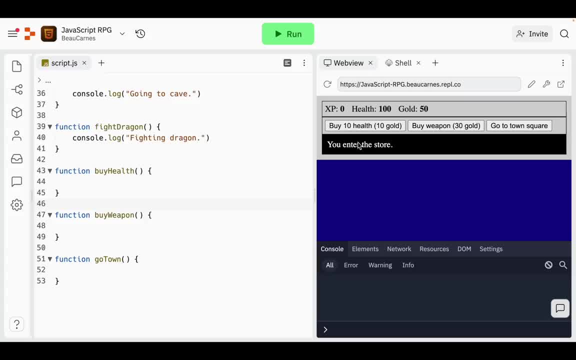 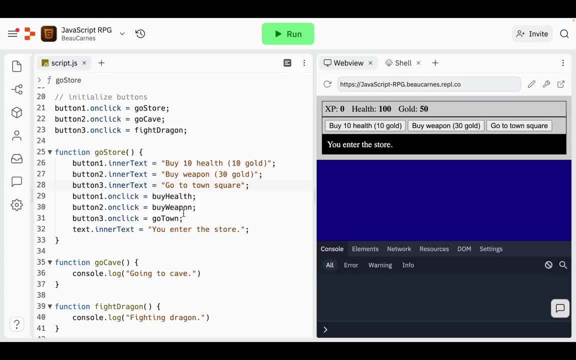 you enter the store. Okay, so every time you click a button, it's basically going to do all this thing: is going to update the button one, update button to update button three and then change the functions for the buttons And it's going to put some new text here. 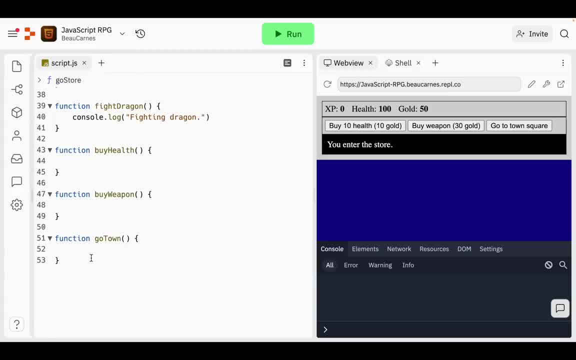 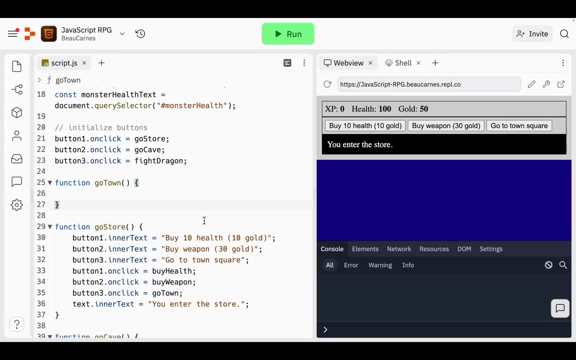 So we're going to move this go town function to be the first function And then we're just going to copy all this and put it in that function. So I'm going to just do Command X or Ctrl X to cut it, And then we'll put it right here, Command or Ctrl V, And this time I'll do: 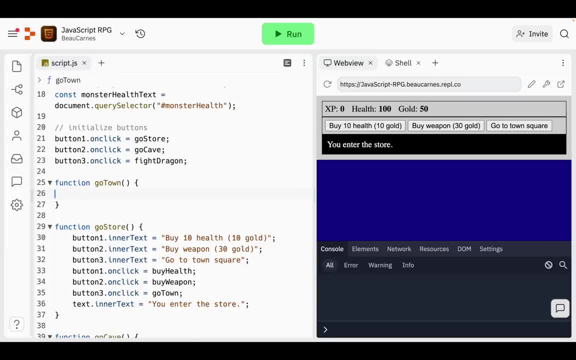 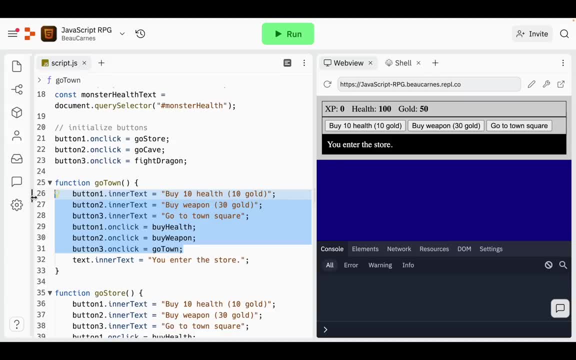 Ctrl or Command C, And then I'm just going to paste it. And basically, when you go to the town, we want all this to be what we started off with. all the text we started off with is what's in the town, And then we're going to paste it, And then we're going to paste it, And then we're going. 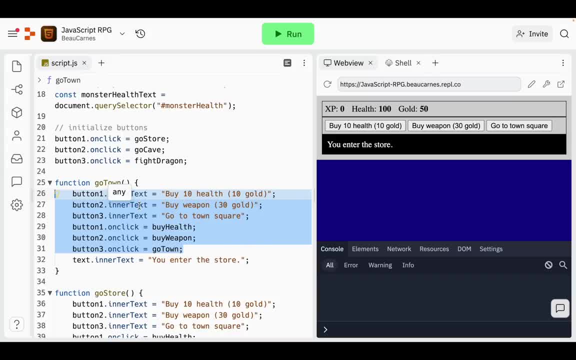 to paste it, And all the click, the on clicks we started off with was what we want the town to have. So I'm just going to just paste an update, the updated code with: go to store, go to cave, fight dragon, And you can see. these three are the same as these three, But instead of the text being 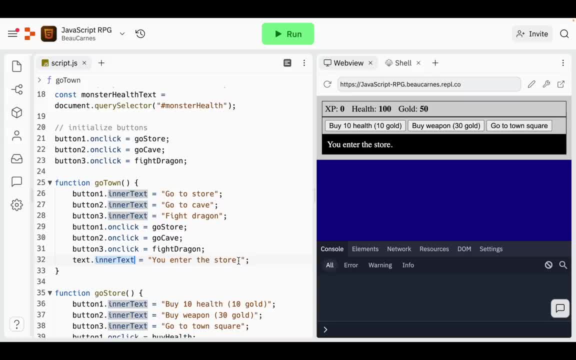 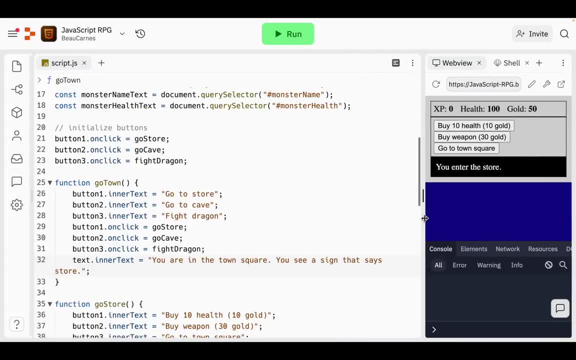 you enter the store. now we're gonna say: you are in the town square. you see a sign that says store. You see a sign that says store. Well, this should be actually in quotation marks, because it's what it says. So let's put quotation marks around the word store. So now we can see based on what: the color. 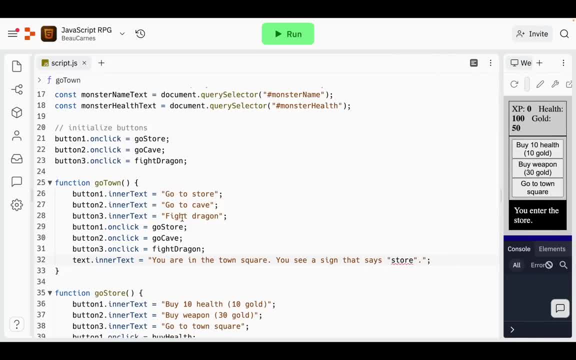 of the this, that something's wrong. So usually strings are this brownish color, but it's switching the black and we have the squiggly lines, because you can't put quotation marks inside a string. Well, actually you can't. I'm gonna show you how. if we put a backslash before each one, 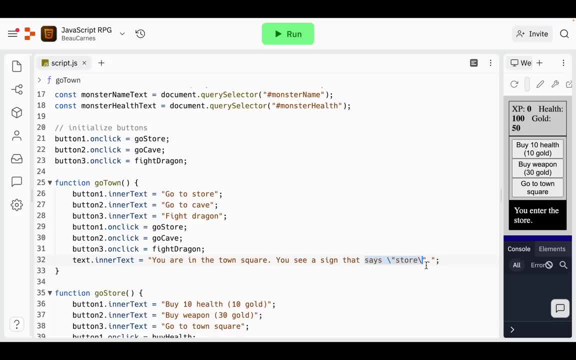 you can see now it all is the right color. So putting this backslash, this is called escaping And it's signifying that the next character after that slash is not supposed to be. it's not supposed to be the end of the string, it's supposed to be literally rendered. So there's. 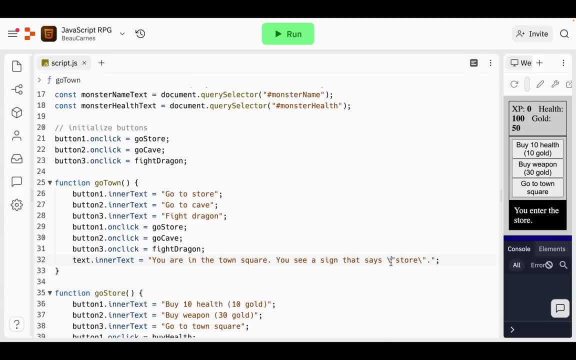 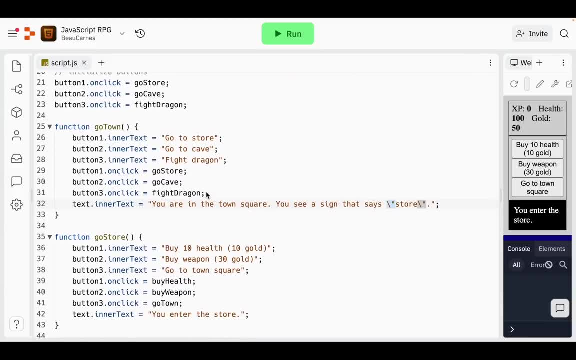 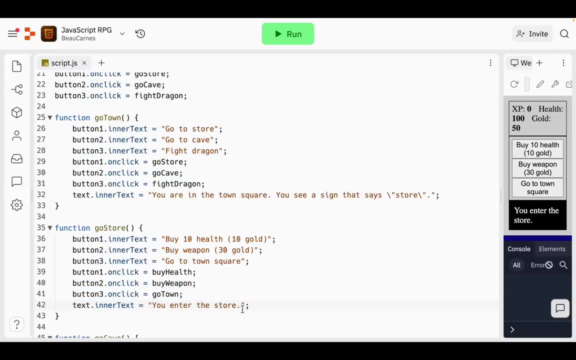 quite a few different special characters that you can use, that you can put in with escaping the character, like that. So you may have noticed that there's some repetition in our code. So if we look at this, all this code looks very similar to all this code. And when you have 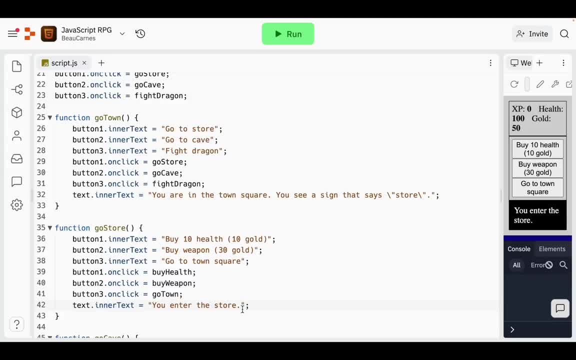 repetition in code. it's a sign that you need a new function. So above the go town function, let's add another function. we'll create an empty function called update. This time the function should take a parameter named location, So data. 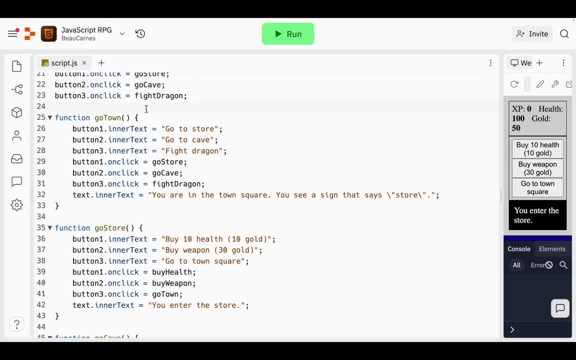 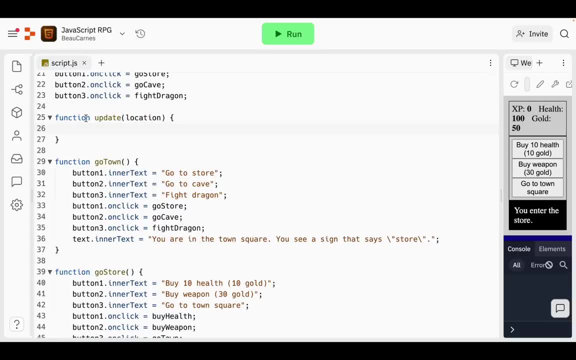 can be passed into the function when it's called. a parameter is a variable that you just put in the parentheses. So let me show you what that looks like. So we have the function called update And this is the parameter we can now pass in. when we call the function, we can pass in the location. So 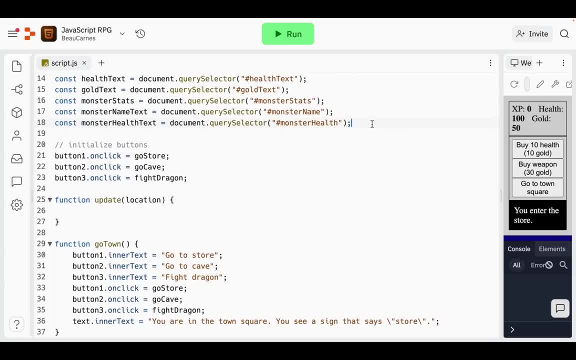 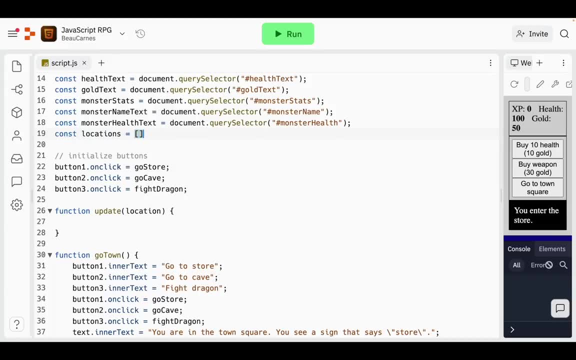 let's create a new const here called locations, And we're going to set it equal to an empty array. This will be used to store all the data for the locations in the game. Now, arrays can store any data type, including objects. Objects are similar to arrays, except that, instead of using indexes, 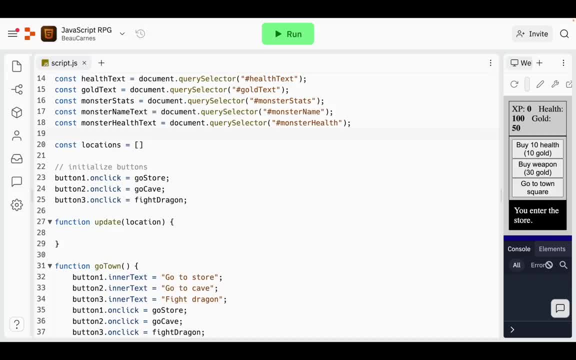 to access and modify their data. you access the data and objects through what are called properties. So inside the locations array we'll add an empty object using curly braces. So basically we just put these two curly braces And here we're going to add an empty object And we're going to 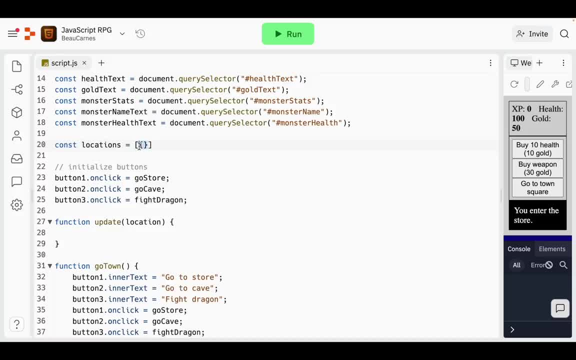 add an object here. So now inside the array, and there's one item which is this empty object, and the object is going to consist of key value pairs. So let me just give you another example of an object. So here is an, an array that has an object that curly braces and there's one key. 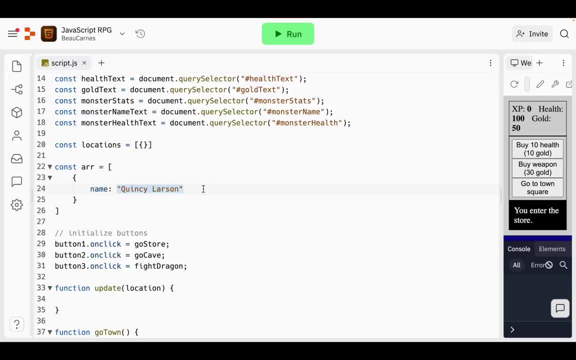 value pair. the name is the key, the value is Quincy Larson, So we're not going to use this. this is just an example. So here now we're going to create a property called name, or the property is also another name for a key, So the property. 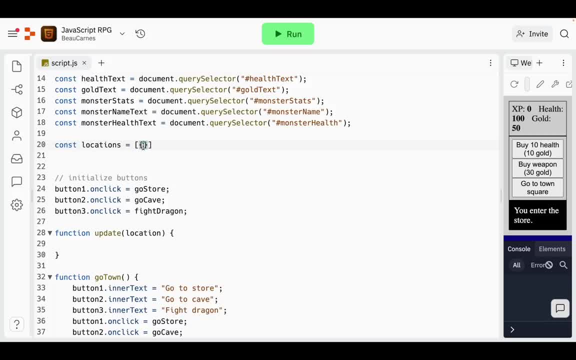 name called name with the value of town square. So we'll just put these on to new lines, like in the other example we saw, And then I will do name town square. So now after the name property we're going to put a comma And then on the next line we're going to add a property named button. 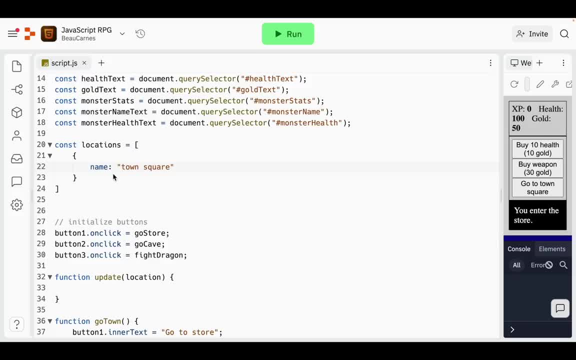 text, And then we're going to add a property named button text, And then we're going to add a property that has a value of an empty array, But since button text is two words instead of name, is this one where we're going to need to put quotation marks around it. So I hope you're following along. 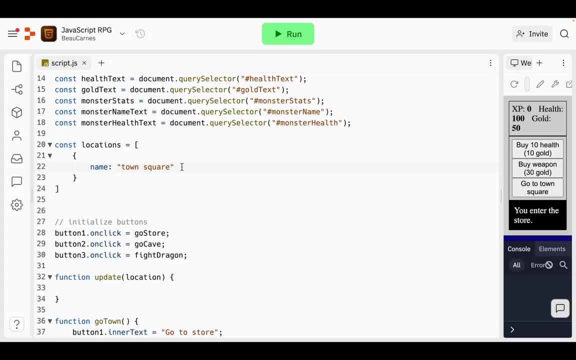 and you've tried this. So, as just as a reminder, you should be trying everything right before I show you And that will help you learn this on your own. So we're going to do button text And then we're going to just set that to an empty array. Oh, and, like I said, we do need a comma. 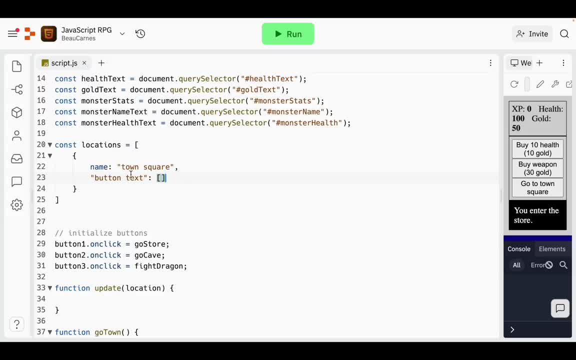 here. So each element in the object, each, each key value pair and the object is separated by a comma. So we have two, two elements in this object. Okay, so now this button text inside this array, we're going to make it a, a list of three strings. we're gonna do me three elements inside the array And it's. 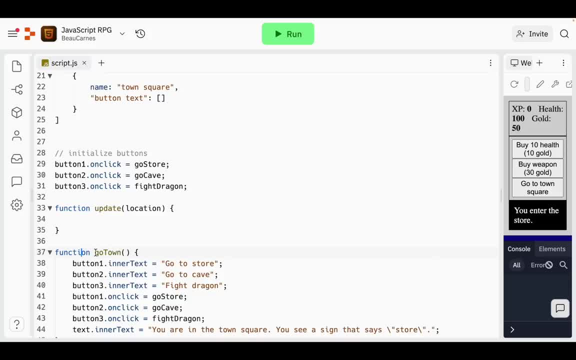 going to be the button text that we see in the go town function: go to store, go to cave and fight dragon. So I'll just actually paste that in there, just like that. And now we're going to add another property in the object with the name button functions, And the value should be an array. 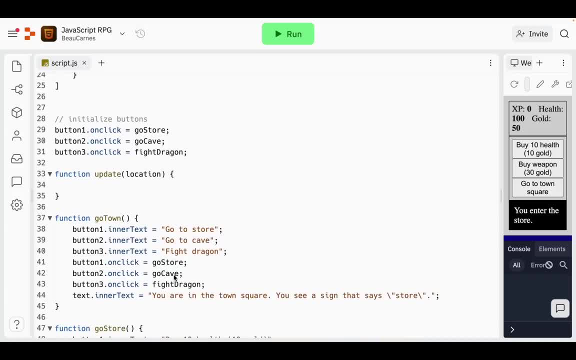 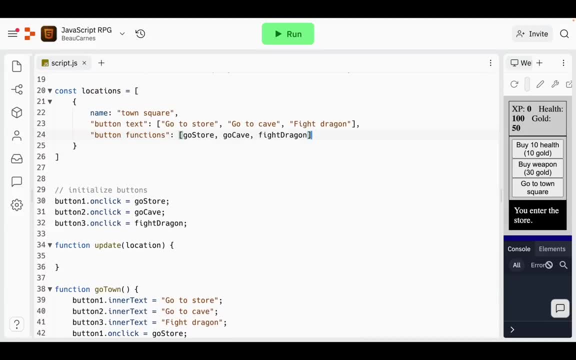 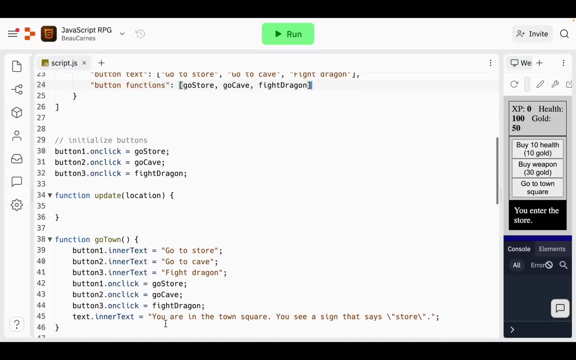 containing the three on click functions, the ghost or go cave, fight dragon. And you see these aren't strings, so they will not be strings in the array either. So it should look just like that. Now we'll just add one final property called text, And it will be the text from here you are in the town. 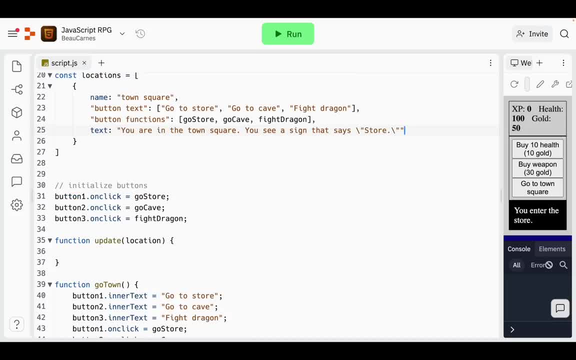 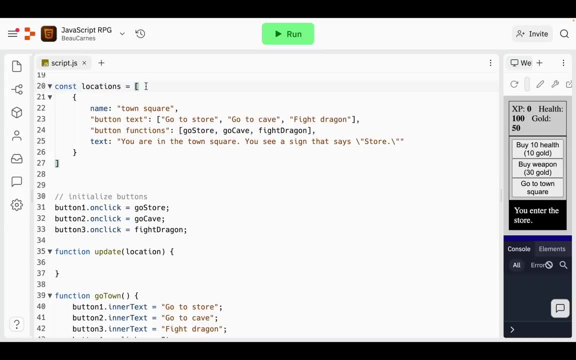 you see a sign that says store, Just like that. The locations array currently has one element which is an object within the array And after the objects, final curly brace, we'll add a comma And on the next line, within the array: 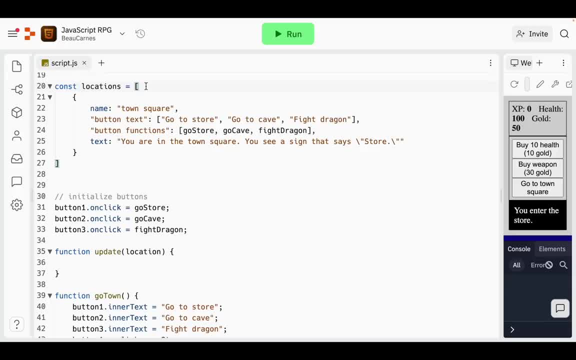 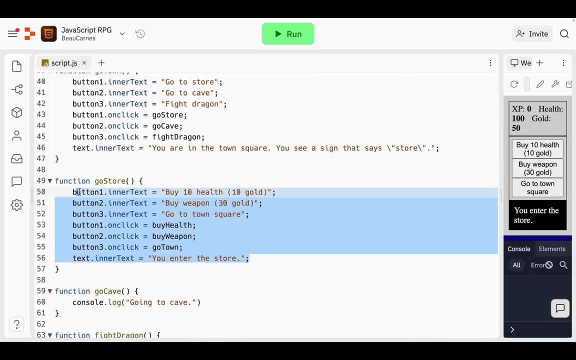 we'll add another object with all the same properties as the first object, will keep the property names the same on the second object but change all the property values to the information from the ghost store function And we'll set the property name to store. 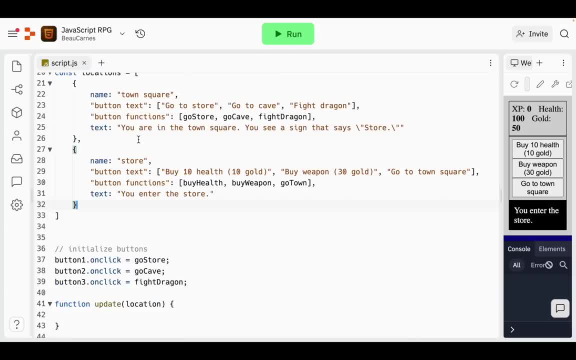 So let's go up here And I'll just paste it in to make it a little quicker here. So now we have an element in this array, that's an object containing all the information from the ghost store function. Now we can consolidate the code inside the Goten and ghost store functions. 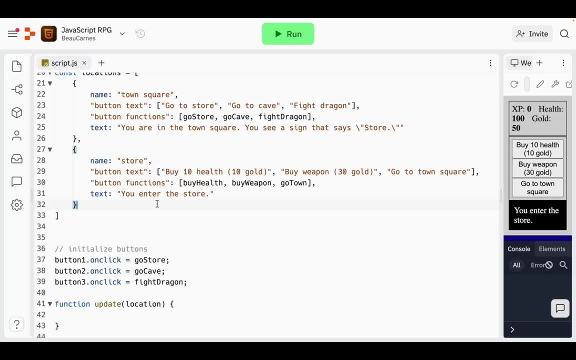 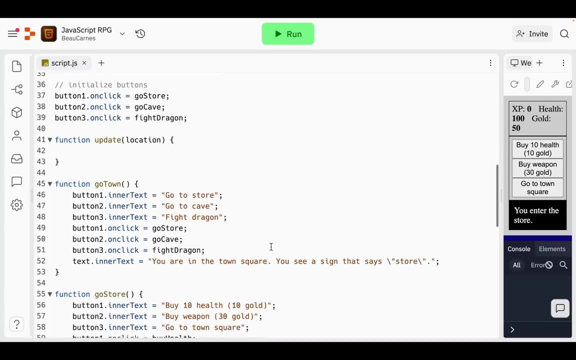 So we'll copy the code inside the go town function and paste it in the update function. then we'll delete all the code inside the go town and ghost store function. So we're gonna come down here. So here's where we're going to copy that and put it right in. 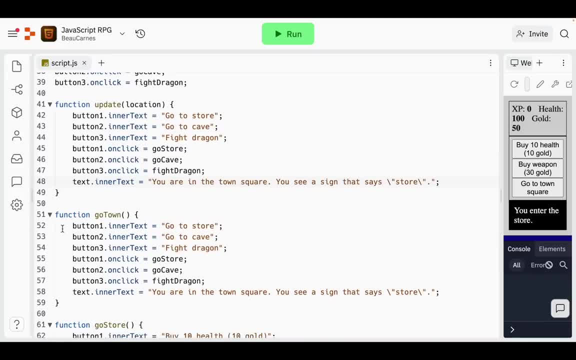 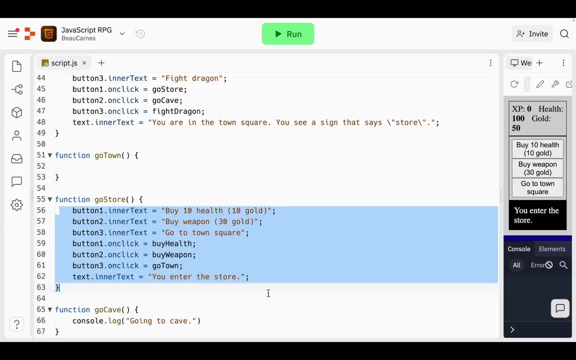 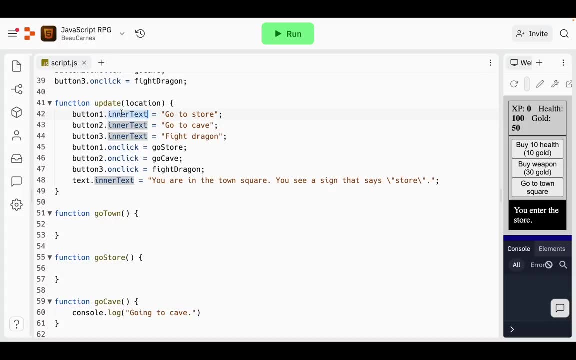 the update function. And then we don't need this code here now. And then we don't need this code. Okay, so instead of assigning the inner text and the on click, like we're doing now, the update function will now use data from the location that's passed into it First. data needs: 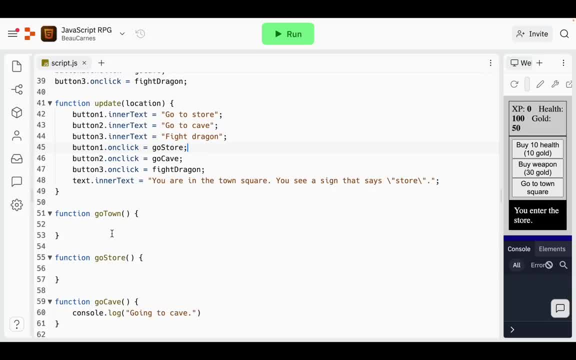 to be passed into the update function. So inside the go town function we'll call the update function. So to call a function you just put the name and then parentheses after it. So we now have called the update function. So when you call the go town function it will now call the update. 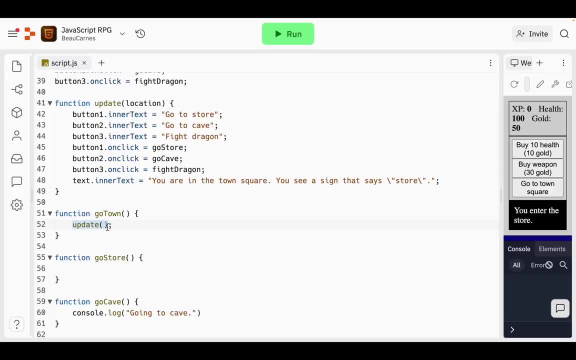 function And we're not just going to call the function. when we call the function, we need to pass in an argument. See: it accepts a location. when we call the function, we can pass in a location. So here we're going. 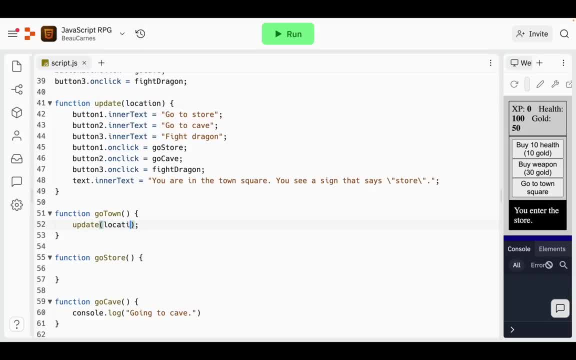 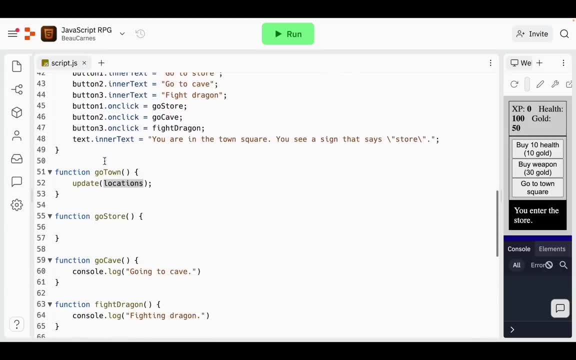 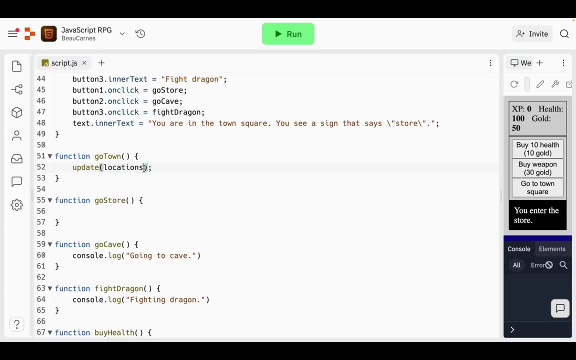 to pass in the locations array Just like that. And so this is the locations array right up here. So the locations array actually contains two locations: the town square in the store. Currently the entire array with both locations is being passed into the update function, But we just want to pass in the first element of the locations. 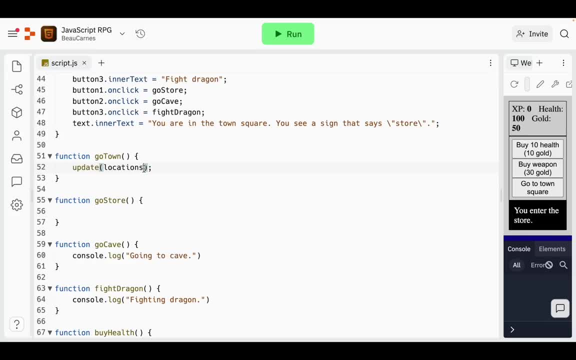 array. So we can do that by putting brackets at the end and putting a zero, just like this. So this is going to pass in the first element in the array, because in programming counting starts as at zero. So zero is the first element, one is the second element, two is the third element. 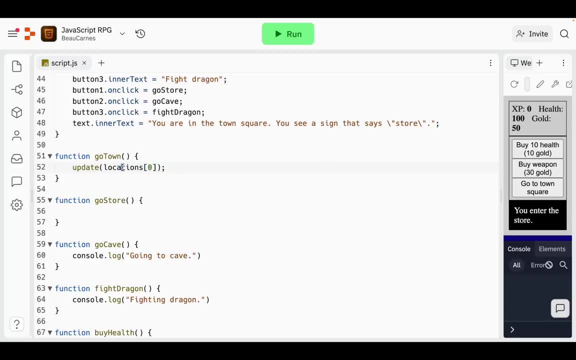 and so on. So when you put the name of an array and then use these brackets and then put a number in those brackets, that's how you specify a single element in the array. So now that the go town function calls the update function, with the first 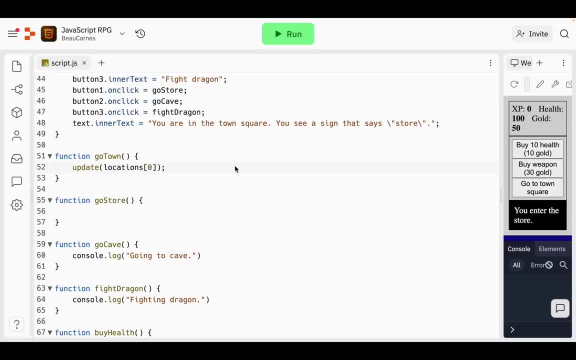 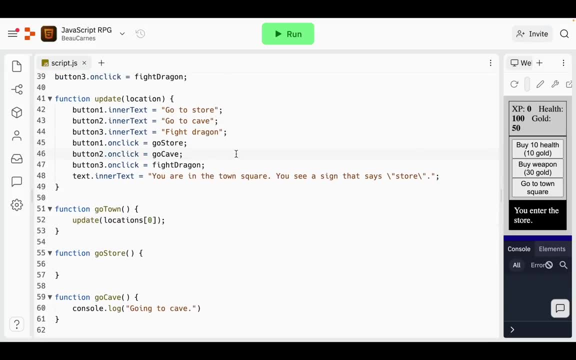 element of the locations array. it's time to use that location information to update the inner text. and on click properties Inside the update function, let's change the button one dot inner text, this one right here, to equal the- the button text, the the location button text. So we can do it. 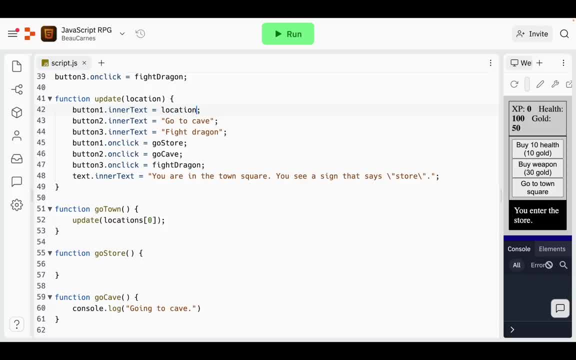 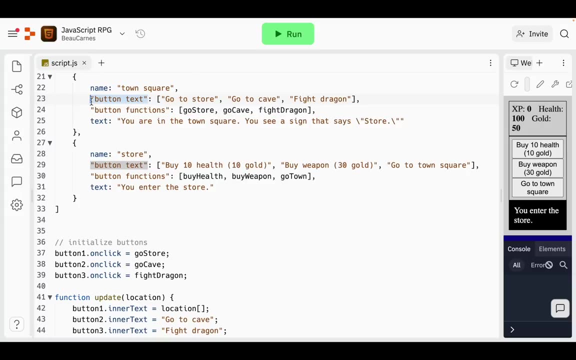 like this: we'll get the, we'll use location, that's what was passed in. And then we'll use brackets, just like before, But to specify a specific part of the of the object. we're going to do just like this: see how we have button text: we want that button text, So that's what we're going to put in. 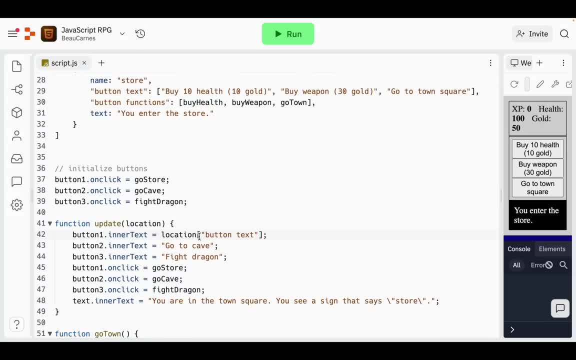 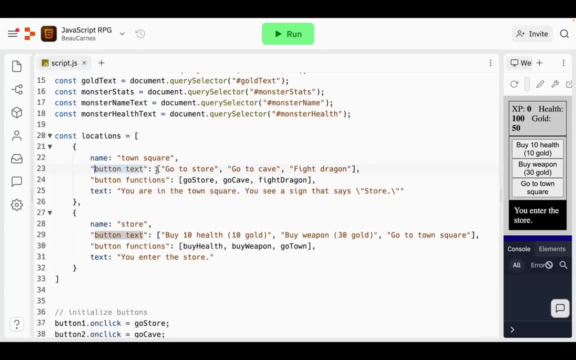 But I just copy that. I'm going to paste it in here. So the location with brackets- button text: that's how we access a specific element in an object, And you can see. this just happens to be an array And we already know how to access a certain element in an array, which is the same. 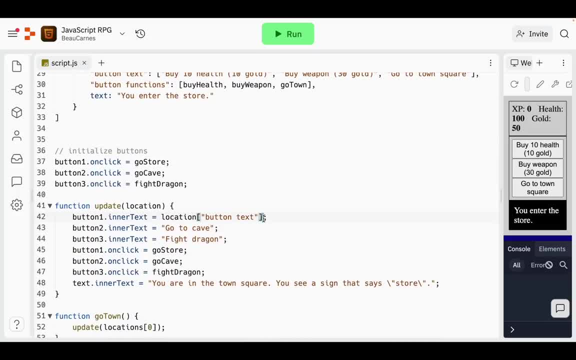 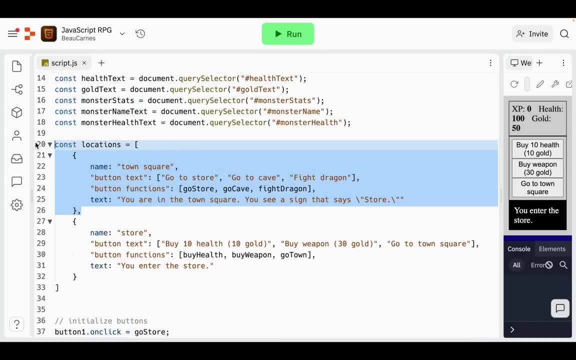 way we use brackets again and we put the index number, in this case index zero, So the location gets us this whole thing. And then we put the bracket button text, that gets us this, and then we put bracket zero, that gets us this. So we've now access to go to store. So now let's update this. these next two. 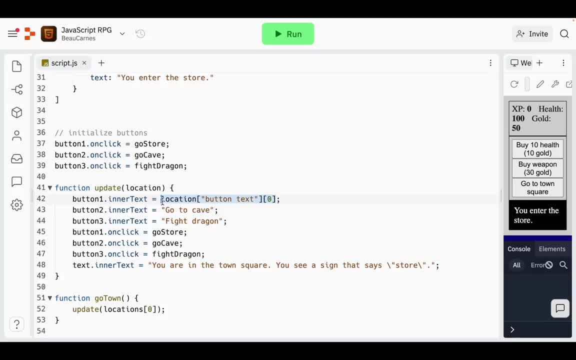 items using this same pattern. So I'll just paste these in And then we can just do: element index one, element index two. so the first, second and third element. Now we can just use the same pattern for the on click of the buttons. So I'm just going to paste this in, But instead of button. 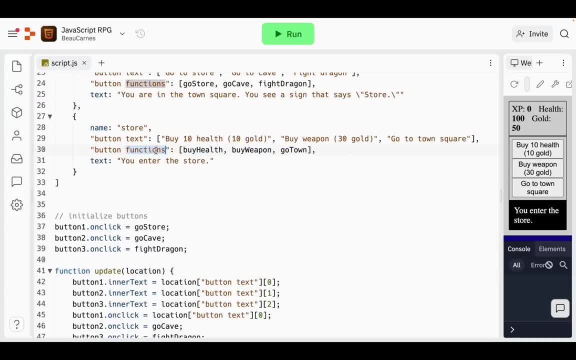 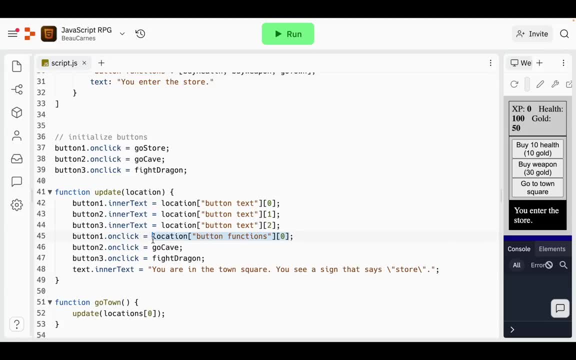 text. it's going to be button functions, So I'll just copy the word functions, button functions. and it's still going to be zero again, because the first item here. so let's update the go cave fight dragon 012.. And then, finally, we'll update the text: dot- inner text. 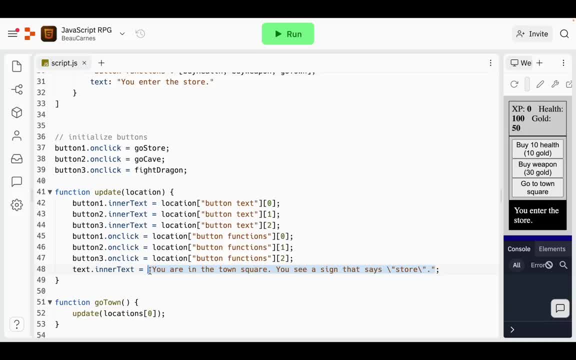 to also get from locations. Now there's there's two ways we can do this. We've been using bracket location, which is just like this location Text, so we could use this notation, but we can also use dot notation. So to use dot notation, there's just two ways to do. 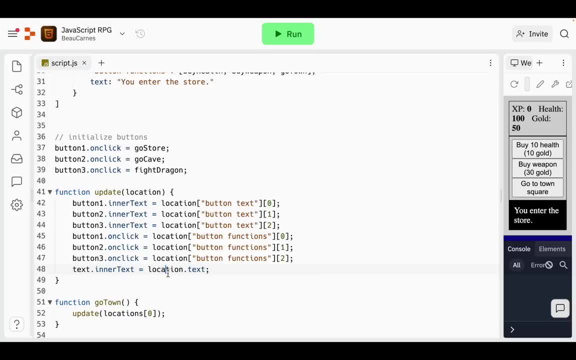 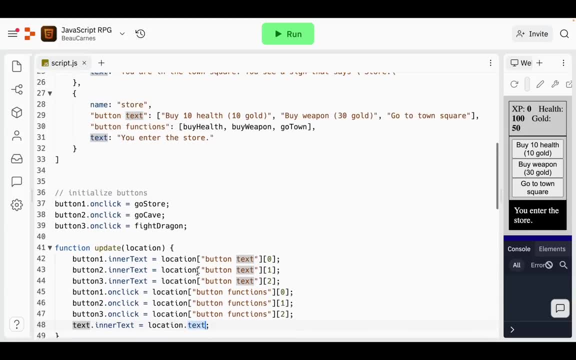 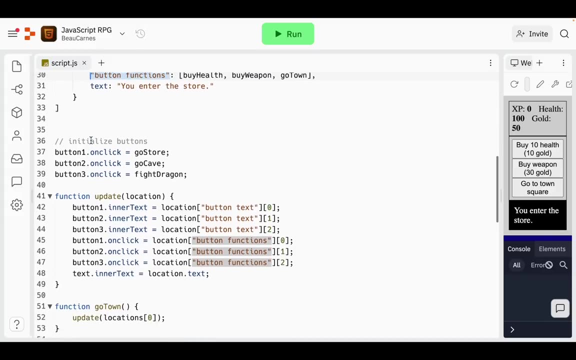 it. We'll do dot text, So we can do location dot and then you just put the word here. Now this only works if it's a single word, like this: When your key is two words, like button functions, you have to use bracket notation, But for the text we can just use the dot notation. 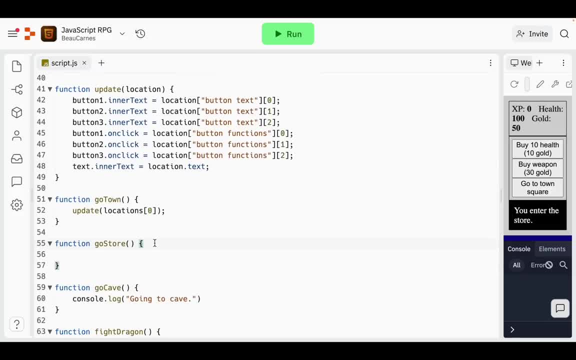 Okay, now we'll just update the ghost or function, And so the code should look basically the same as the go town function, except the number zero, So should be changed to one. So let's just do that really quick, And then it will be time to test our 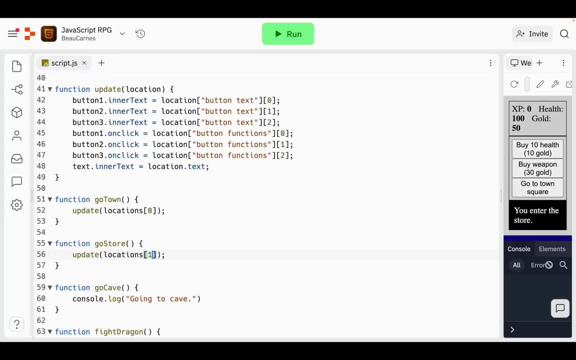 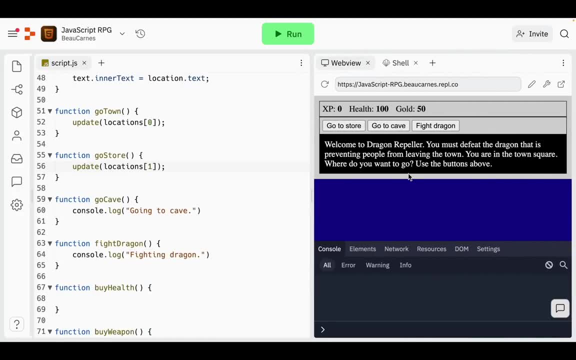 game. So up to locations one And now click Run And we should be able to move between the store. Oh, good, See, it has the information for the buttons. We have you enter the store. I can go back to the tone square. you are. 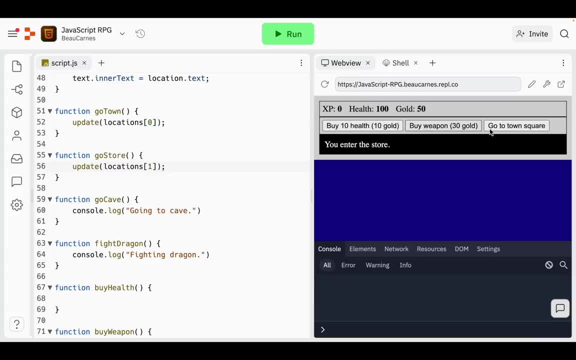 now in the telling town square you see a sign that says store. So now we can move between the town square and the store. If we press these other buttons, nothing happens. We haven't done that quite yet, But this game is starting to work Now. 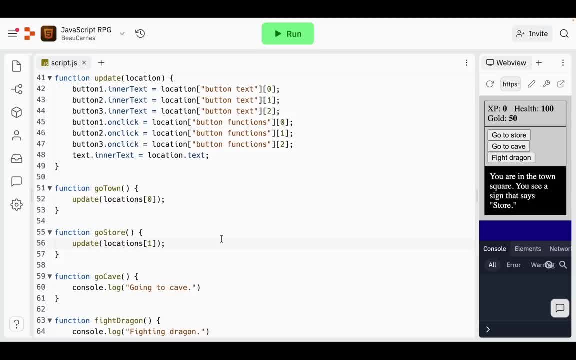 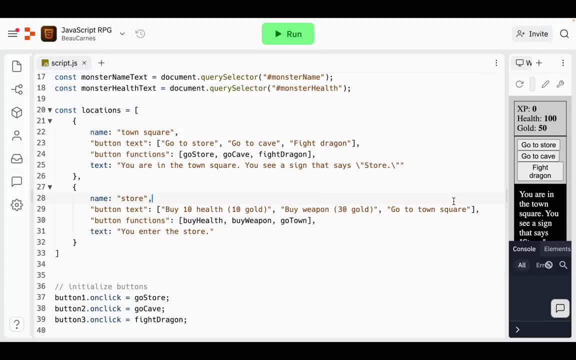 I'm just going to shrink this a little bit And we're going to add a third object in the locations array. It's gonna have the same properties as the other two objects. the name will be cave, And then the button text is going to be: fight slime, fight thing beast and go to town square, And then the 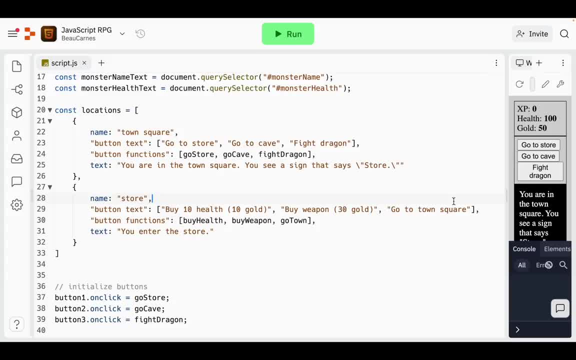 button functions. we're going to have some new functions: fight slime, fight beast and go town. And then the text is just going to be: you enter the cave, you see some monsters. So maybe you tried that on your own. I'm just going to paste it in here. See, we have the cave with new button. 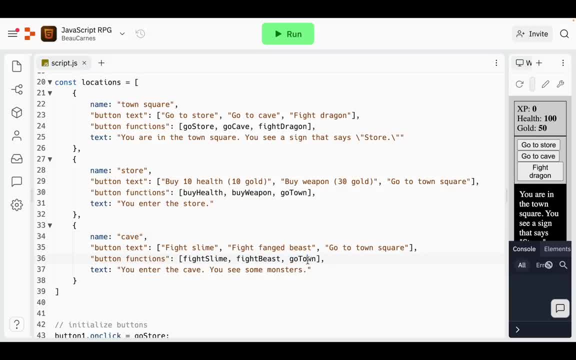 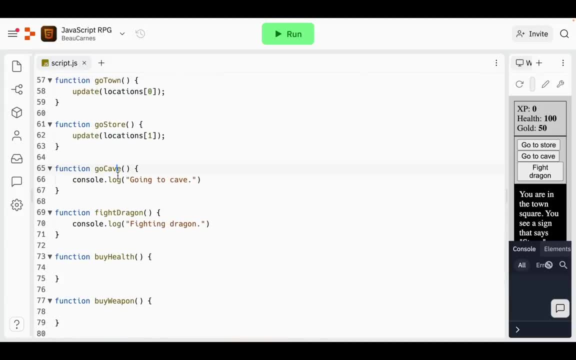 text here And then new button functions- a few of these we still have to create- And you enter the cave. you see some monsters. So now we'll just update the go cave function with using our calling or update function And let's create some more empty functions. here was for the fight slime and fight beast, So fight. 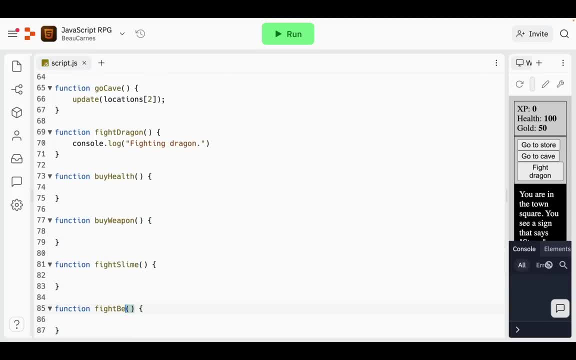 slime. So now that the store and cave locations are complete, we'll code the actions at those locations. So first we'll do the by health function. So inside the by health function says gold to equal gold minus 10.. So it's just like this: gold equals gold minus 10.. And you can see. 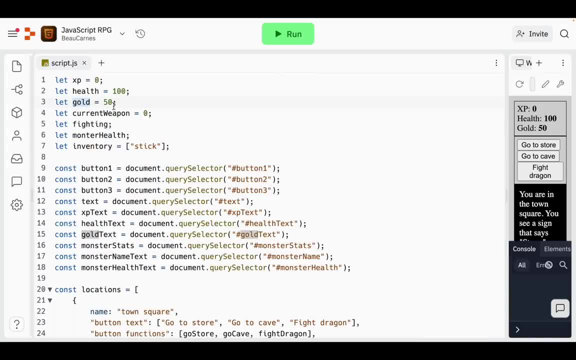 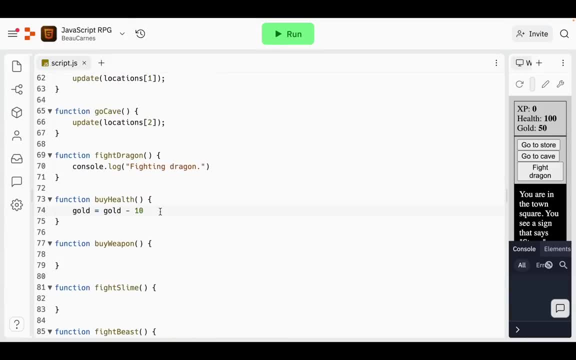 we're getting the gold from our variable that. we've already said. we start with 50 gold, But when you buy health we're going to subtract 10 from the gold, And for subtracting 10 from the gold we need to give some health. So let's add 10 to the health. So that's pretty straightforward. 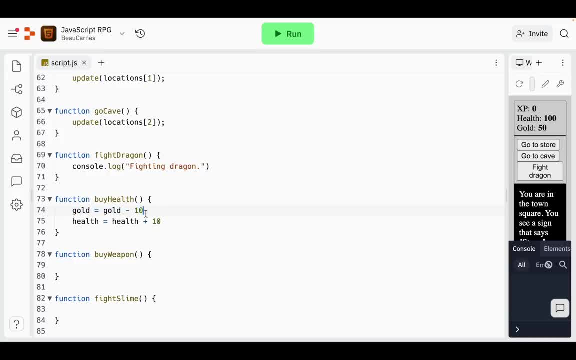 But let me tell you about a quicker way. you can do something like this. So there's a shorthand way to add or subtract from a variable called compound assignment. The long way to add it is like this. But there's a short way where you can do gold plus mine or we can do gold. 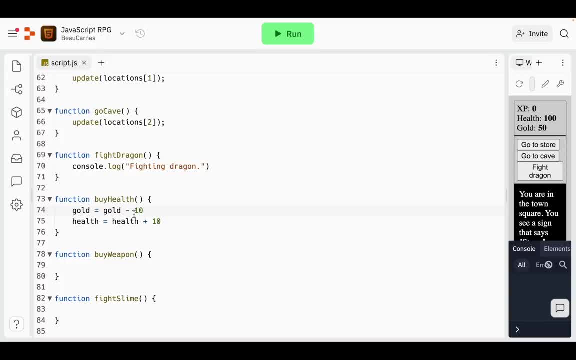 minus equals 10.. So let me show you, if we just do minus equals 10, that's just the shorthand of subtracting 10 from whatever that value is and assigning the new value to the value. So this basically does the same thing as before. So let's change this to also use the compound assignment. 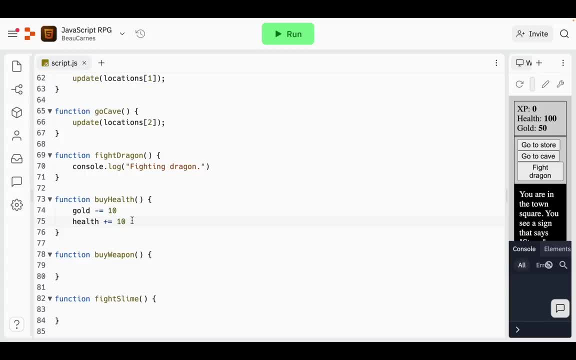 So it's just going to be: health plus equals 10.. So the line that I changed this from does the same thing as the line that I changed it to. Okay, so now we're going to go ahead and add a new value. Now that the golden health value variables have been updated, we need to update the values. 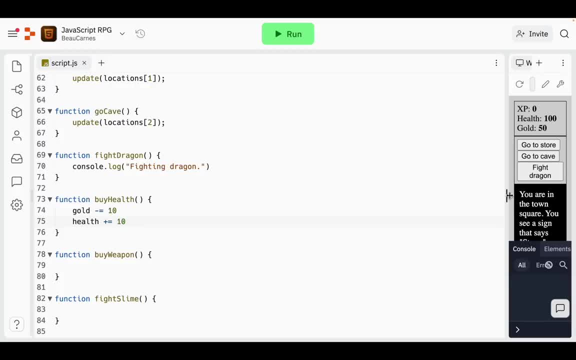 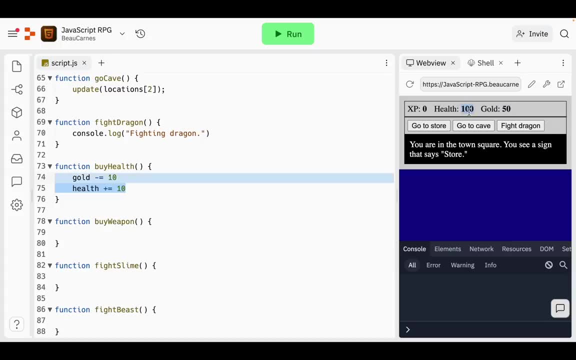 displayed on the screen. So if we look at what's being displayed here, we have health 100, gold 50. Well, we've changed the variables, but it didn't actually change anything on the screen. So how can we do that? Well, we can use the. we can set the inner text to gold. So for the gold tax, that. 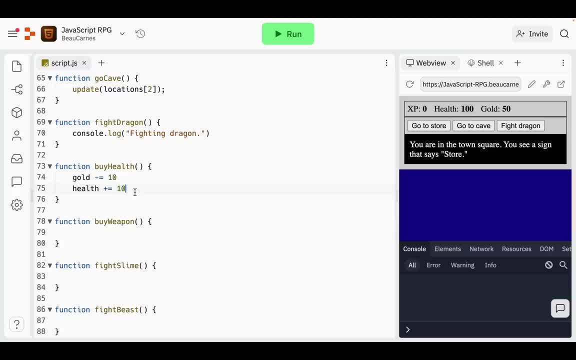 inner tax. let's set to gold, And we'll use the same thing for health tax. So so gold tax, inner tax equals gold, health tax, inner tax equals health, So we can update the text on the screen. So what if the player doesn't have enough gold to buy health? Well, let's put a code in this. 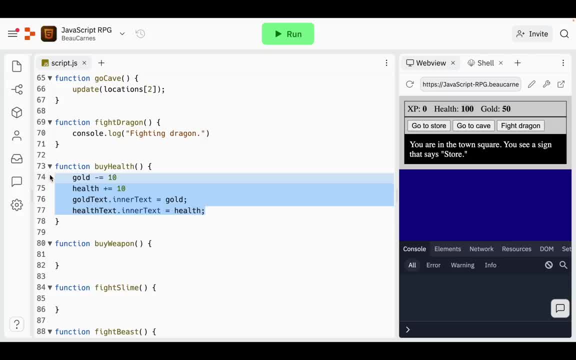 by health function. we're going to put all this code inside an if statement, So let me just show you how to do that. So I am going to add an extra line here And it's going to say if, and we want to say if condition- we'll update that later- And then I'm going to put curly. 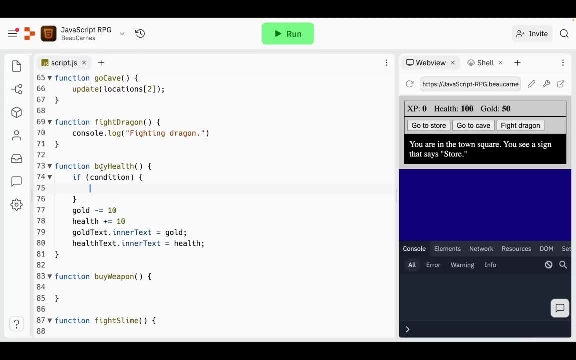 braces, just like we have the curl. it's kind of looks similar to a function where we have something in parentheses and then we have the curly braces. I'm going to copy this, or I'm going to cut it And then I'm going to put it here. let me get the tabs correct. Okay, so this is an if statement, So 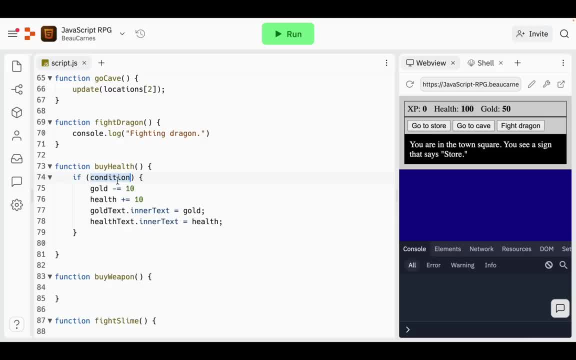 if something is true- we haven't specified what we want to be true, though, But if something is true, then we do all these things right here. If this is not true, then all this code will be skipped. This is called a conditional, So it's code that you only want to run in a certain circumstance. In 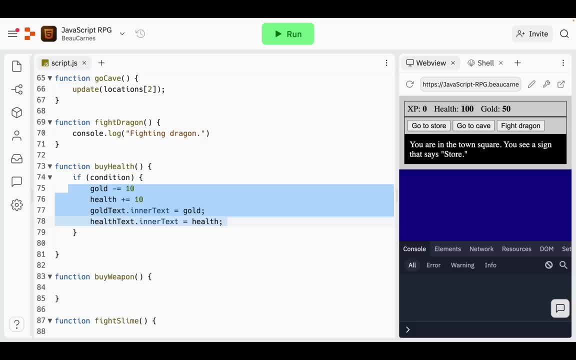 this case, the circumstance is we want to check if the amount of gold the player has is greater than or equal to 10.. So we just have to do: gold is greater than or equal to 10.. So if this is true, if the variable 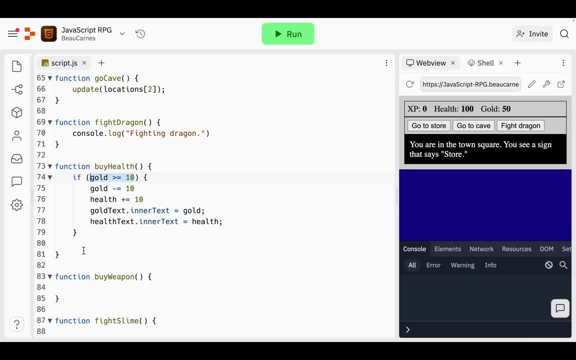 is equal to, greater than or equal to 10, then we can buy health. If not, all this will be skipped and we cannot buy health. And you can also do: instead of just greater than, it can just be, instead of greater than or equal to, it could be greater than, it could be less than, and so there's a 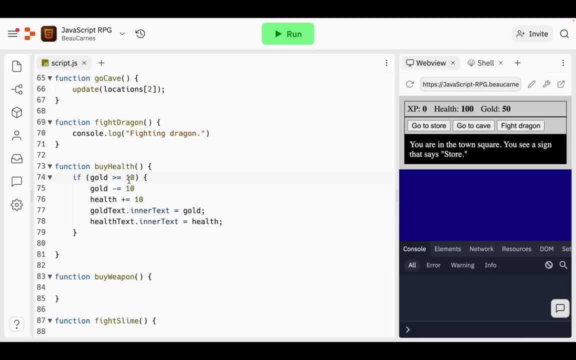 few different conditional operators that you can use, but we're just using greater than or equal to. So if you want code to run, only if this is false, then we can put an L statement, So an L statement just like this else, And then we put curly braces, So any code in these curly braces will run. if this 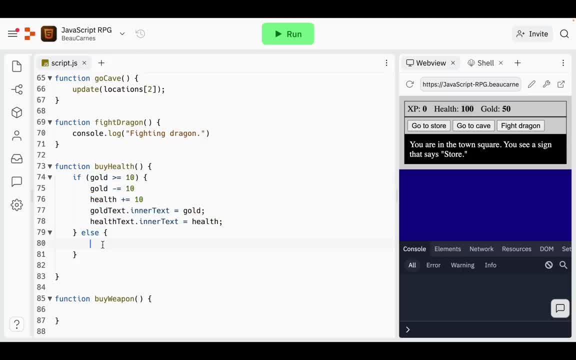 is false. If it's true, we run this code. If it's false, we run this code. So if the player doesn't have enough money to buy health, will inform the player. will set the text that inner text to: you do not have enough gold to buy health, Just like that. Okay. so before we write the code for the 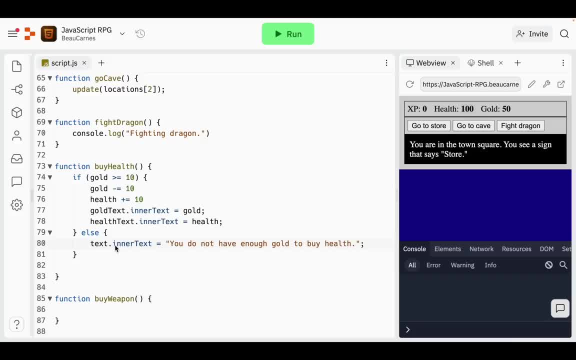 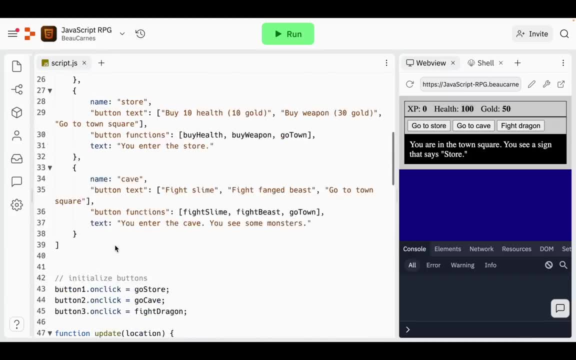 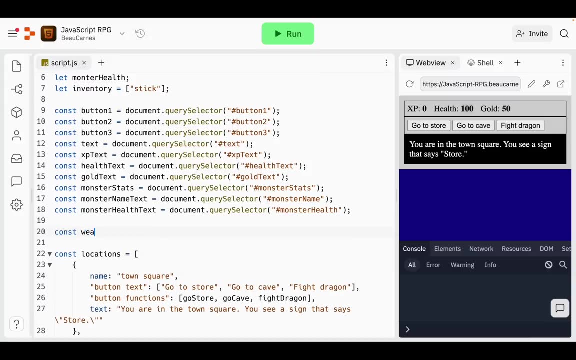 buy weapon function. we'll use const to create a weapons variable right above the locations array and set it to an empty array. So then I go up here, we got the locations array And then I'm going to do const, weapons equals empty array, Just like in the locations array. all the elements in 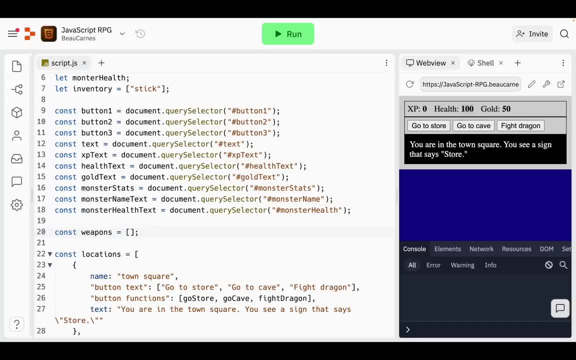 the weapons array will be objects. So we'll add four objects to the weapons array, each with two properties. The properties are name and power. So the first would be the should be the name stick with power set to five, then dagger with power set to 30.. 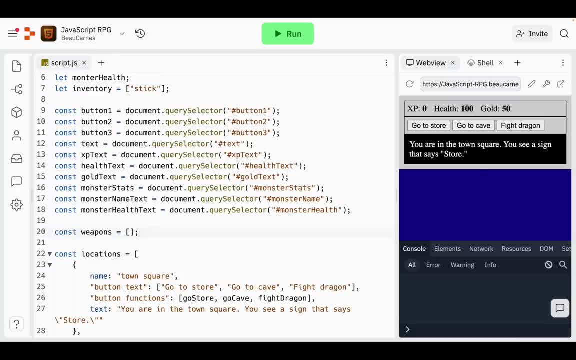 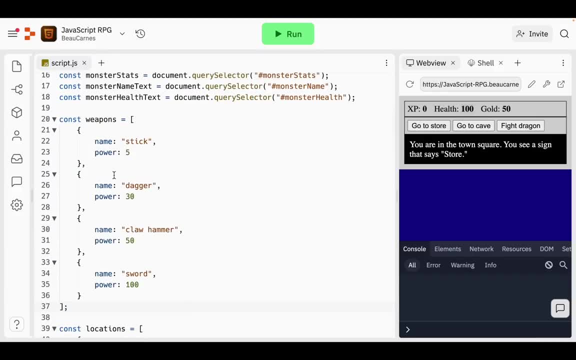 Claw hammer with power of 50.. And finally, sword with power of 100.. So if you do all that, it will look like this. So we can see we have all the different weapons And just so you know, these don't all have. 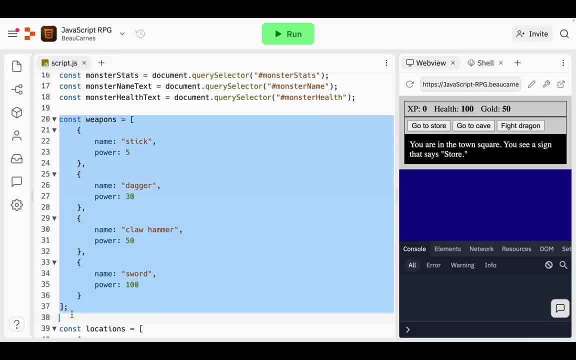 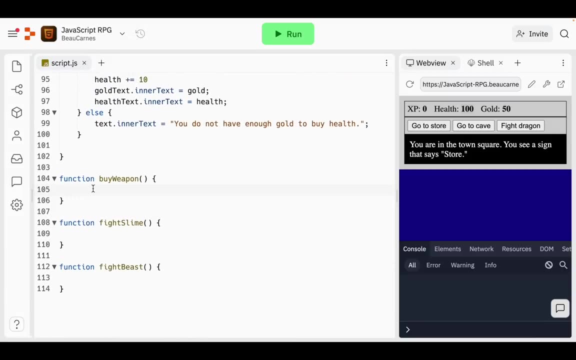 to be on different lines. This whole thing could actually just be one line of code, But spacing things out this way just makes it more easily readable for humans. So let's go back down to the buy weapons Function And we'll we want to check if gold is greater than or equal to 30.. 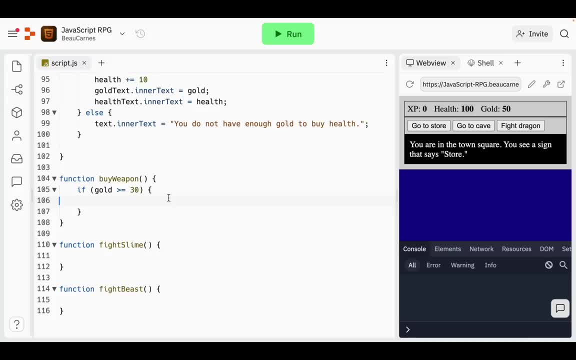 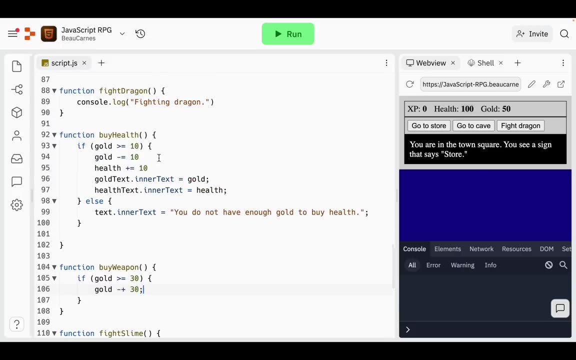 So just like that, and we're going to put some code in this if statement, if that's true, the first thing is we're going to set goal to equal 30 less than its current value. So bold minus equal 30. And you can see. every once in a while I forget the semi colons, And it is there. 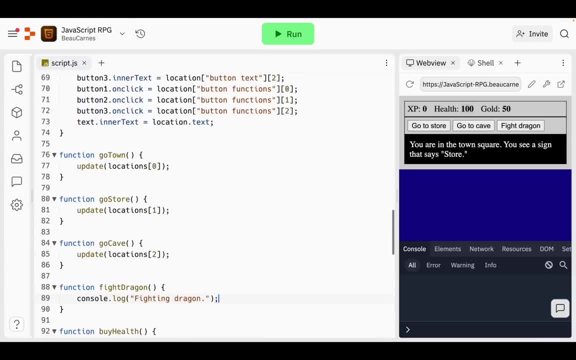 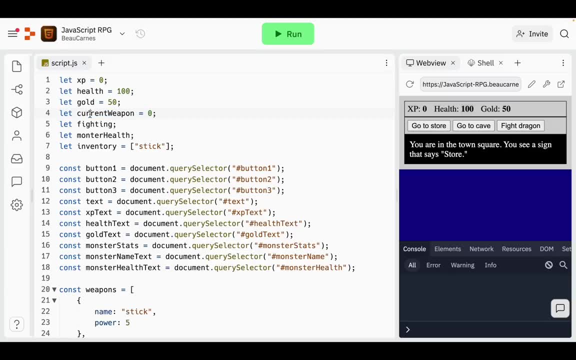 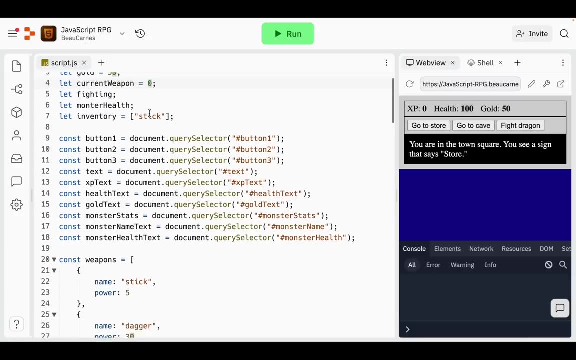 they are optional. It's just usually people just use, always use semi colons or never use semi colons. So if we go back up to the top, we can see that the value of current weapon is going to correspond to an index in the weapons array. you start with the weapon at index zero, that's stick. 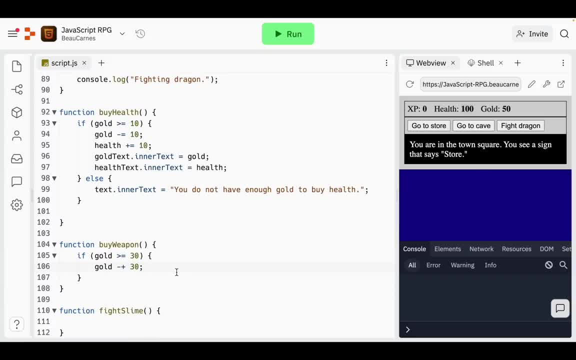 So let's go back down to I weapon And the player starts with a stick. But in the bi weapons function we want to add one to current weapon, since the user is buying the next weapon in the weapons ray. So we just do current weapon. 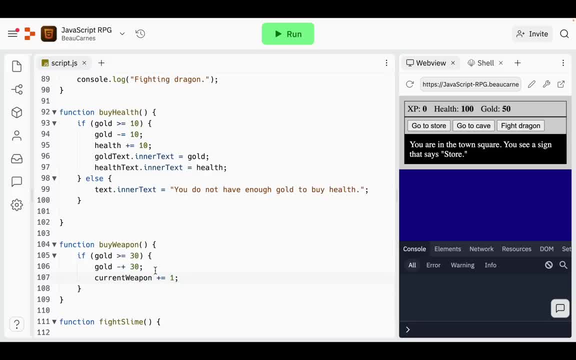 plus equals one. Oh, and I this was supposed to be an equal sign that. you probably heard me say it and you probably noticed. but yeah, minus equal 30. So just how there was a shortcut mood with it. First we did gold equal 30. And then we added one to current weapon, And then we added one to 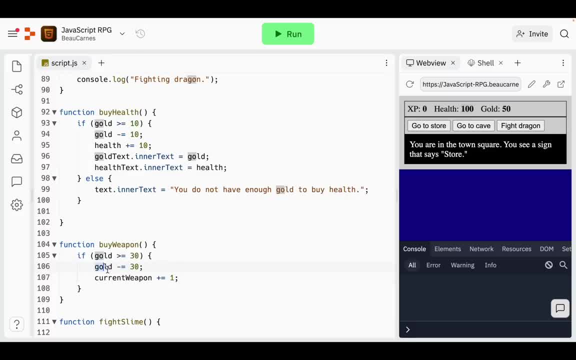 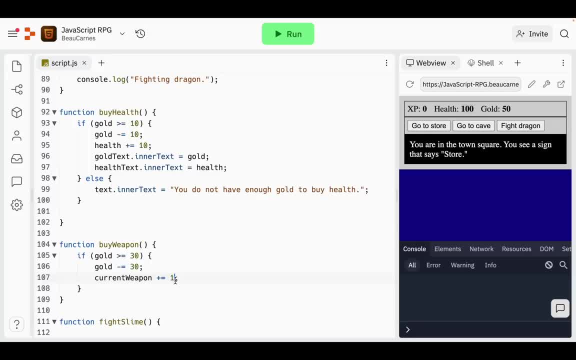 so add one or subtract one. there's a shortcut just for doing that. So whenever you want to do current weapon plus equals one or current weapon equals current weapon plus one, here's the shortcut, just current weapon plus plus. So doing plus plus just adds one to the. 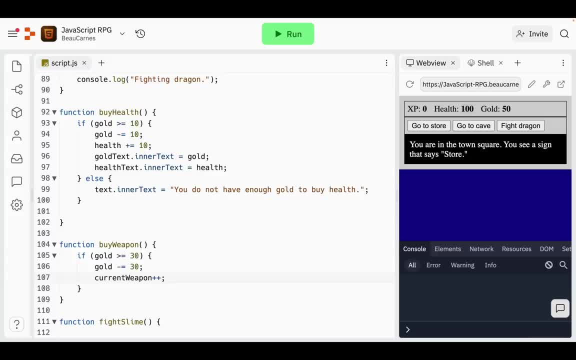 current weapon And now we'll update the inner text. property of gold text and text text is going to equal. you now have a new weapon, So it should just look like this: Now let's tell the player what weapon they bought. So, in between the two lines that we just wrote and between these two, 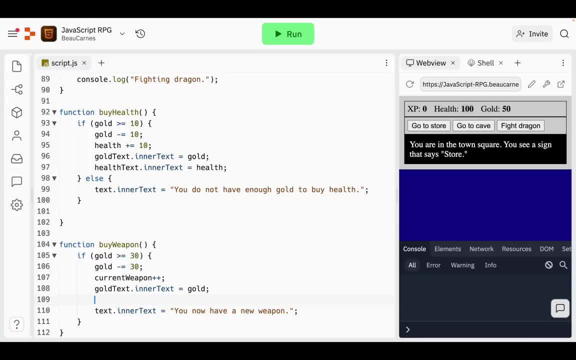 we're going to add a new line. we're going to use let to initialize a new variable called new weapon and set new weapon to equal weapons. So new let, new weapon, equals weapons. So right now we're just making it equal the entire array. But now we're going. 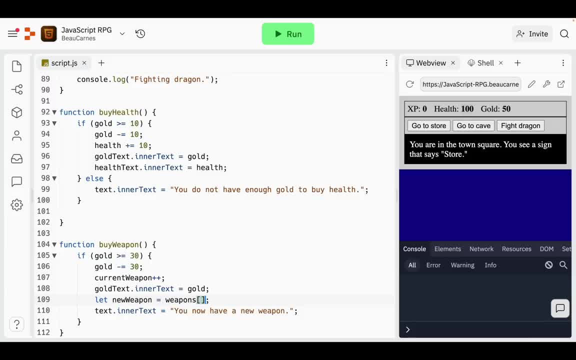 to add brackets so we can get to an individual weapon And we're going to set it to the current weapon. So instead of just putting a number here, we can put a variable And this is going to be the index of a certain weapon in the weapon array: weapons array. 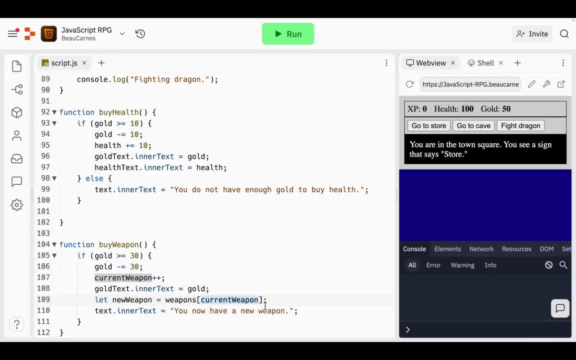 But we don't want just the entire weapon, we just want the name. So we can use dot notation and do dot name. And now let's see how we can insert variables into a string. we can do that with the concatenation operator, which is actually just a plus symbol. So we're going to update this string. 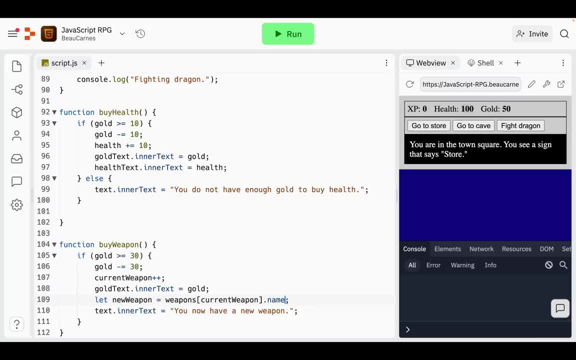 to, at the end of a string, add a plus and then put the new weapon. So we want this to say: you now have a and then put the new weapon. So basically it's going to be like this: you now have a and then I will do plus. 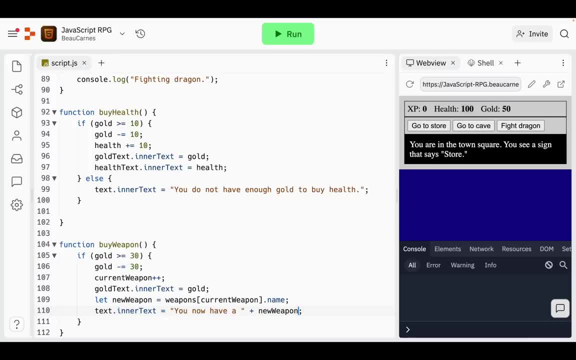 new weapon. So this is outside of the string And we have to make sure we put the space here. So it's going to put in a space a new weapon. we also want to period at the end, So we're going to have 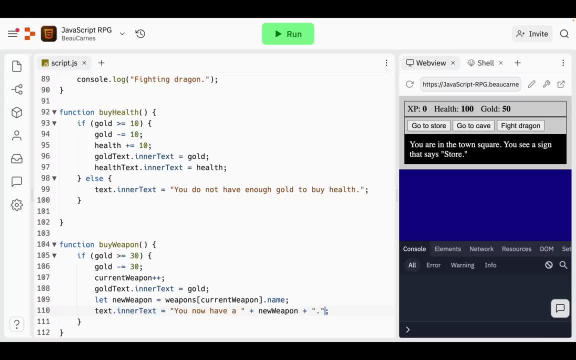 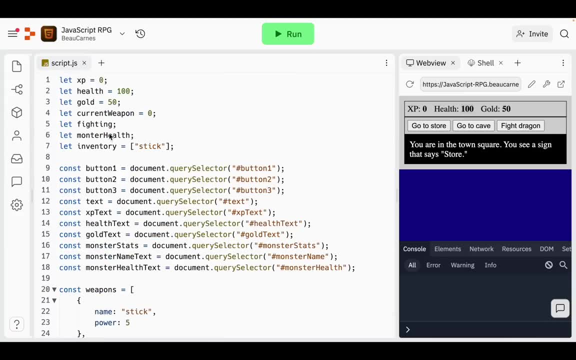 to concatenate a period period. at the end you now have it and then it's going to show the new weapon. So way back at the beginning we made this variable variable called inventory And the inventory it starts off with just a stick. So what we want to do is add a add the new weapon on to the end of the inventory. 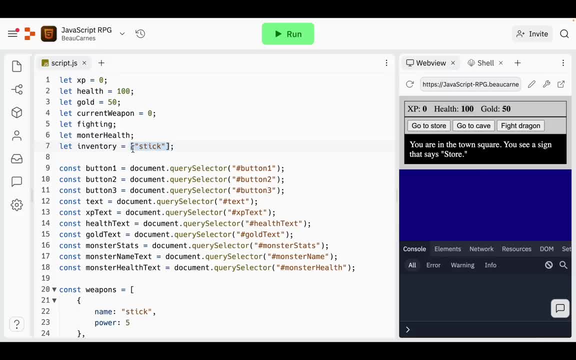 because you still keep the inventory. what you already have will still keep the stick. But if you buy a new weapon now, you should have the next weapon in your inventory And you can do that by using dot push. So we just do inventory, dot push And then we put the new weapon in. 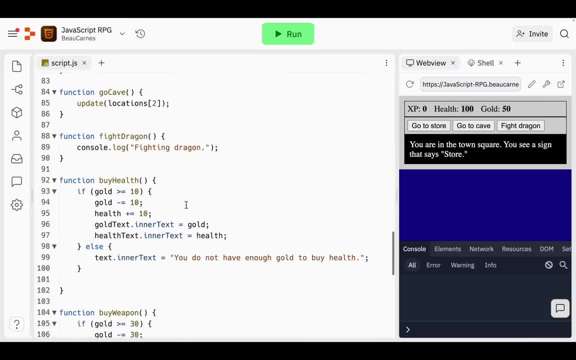 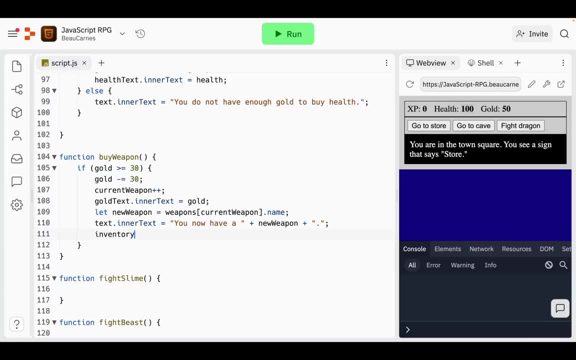 parentheses. it's just like this: we'll go back down here And then we will. where is it? inventory dot push new weapon. So we've added that to the inventory. So so far, anytime that inner text was updated, the old text was completely erased. But this time 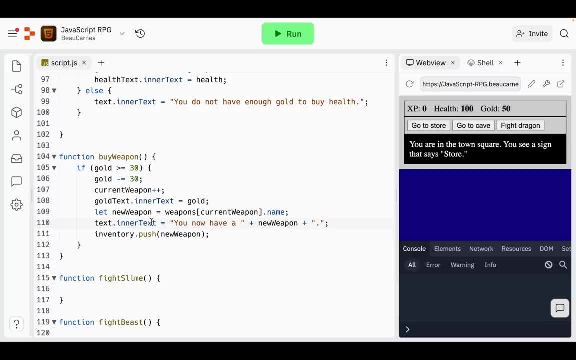 let's use the plus equal operator instead of the equal operator So we can add text to the the end of text dot, inner text, And we're going to add the text. So we're going to still, we're going to have this text, But then the next line, we are going to add a string in your inventory you have. 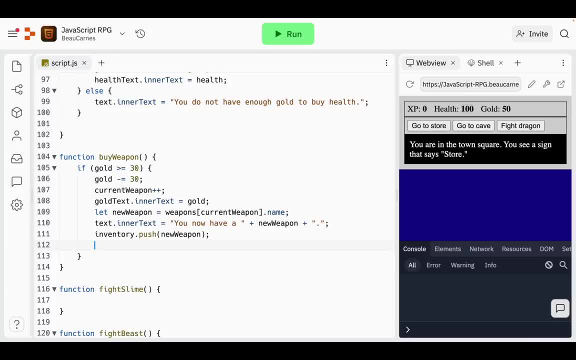 And we are going to put what we have in our inventory. So it's basically going to look like this text, that inner text plus equals, and then we're going to have a space because we want to have space after this period, And in your inventory you have, and then I can just put: 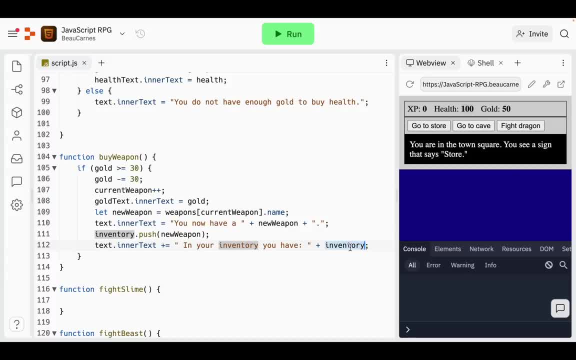 inventory. Now, this is an array, And whenever you print out an array, it's just going to put every element in the array, separated with a comma. Okay, now we just want an L statement And else, if it's just going to say, we're going to update the inner text to say you do not have enough gold. 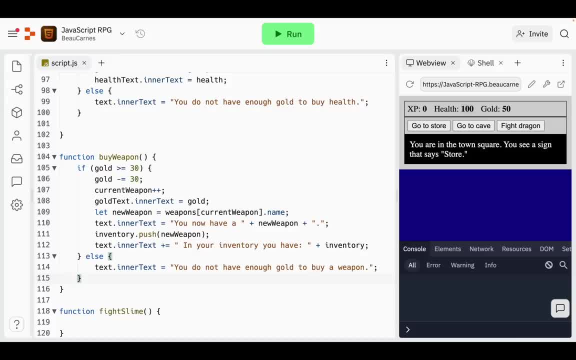 to buy a weapon. just like that, Once a player has the best weapon, they can't buy another one. So let's wrap all this code in the bi weapon function inside another if statement. So basically it will be a net will have an if statement inside another if statement. This: 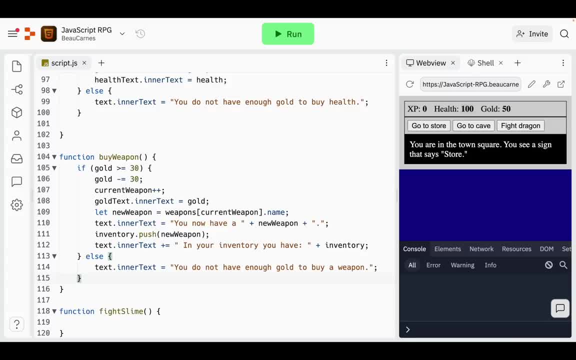 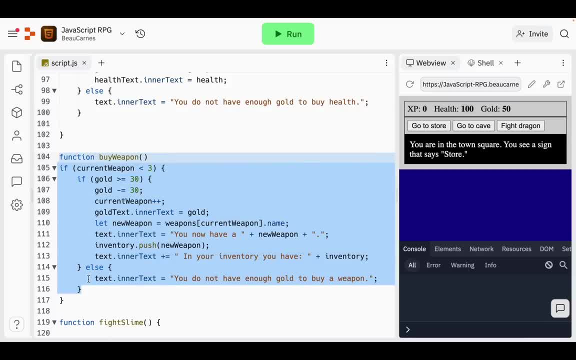 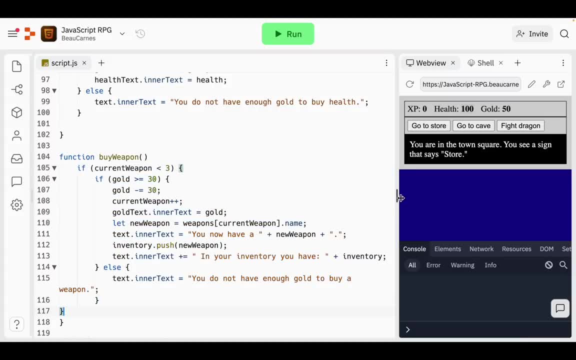 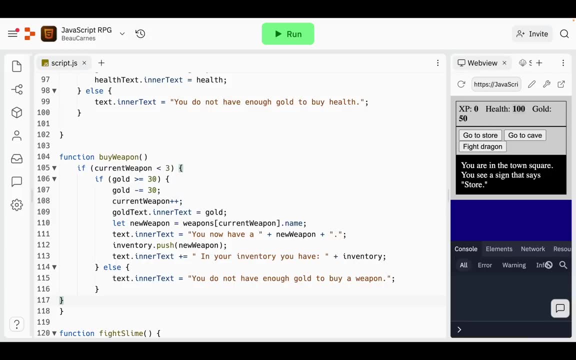 statement here. Now let me tab everything over And then put another curly brace here. I move this over. Now we can see everything. Okay. so if- Oh wait, this has to be lined up right there. Okay, so if current weapon is less than three. 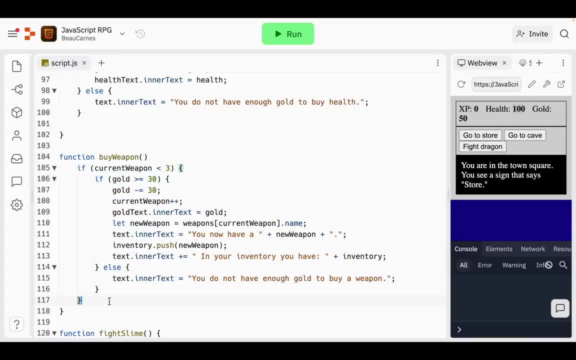 then we'll do all that. So at some point in the future you may want to add more weapons. So instead of checking if current weapon is less than three like this, let's check if current weapon is less than the length of the weapons array. So we just have to put the name of the 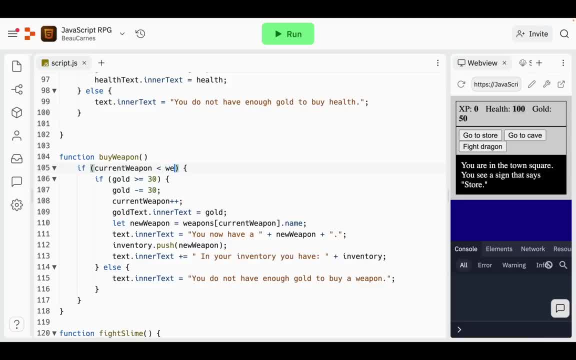 array dot length. So, just like this: weapons dot length. Well, not quite. this is not quite what we need to do, because we've now introduced an error. the current weapon variable is the array index. array indexing starts at zero, So the index of the last element in the array is one less than. 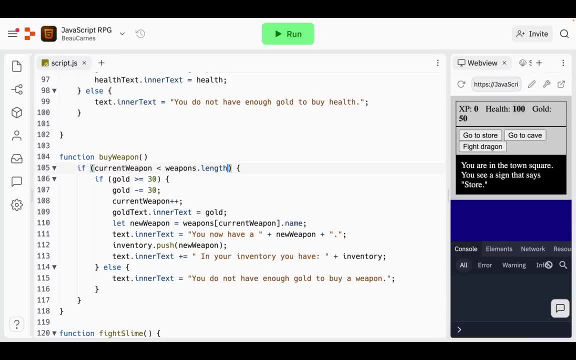 the length of the array. So in this if statement let's change weaponslink to weaponslink minus one, And if the user can't buy a weapon, we'll update the inner tax to say: you already have the most powerful weapon. So here we go, Else. 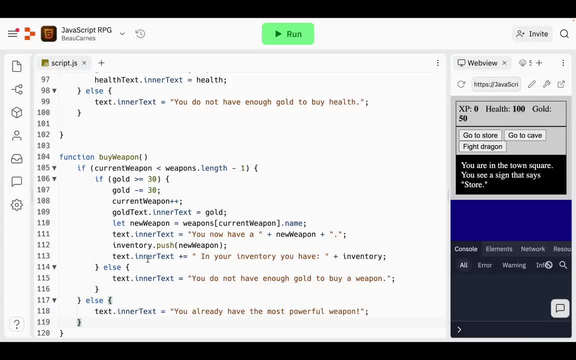 intertext: sex and intertext. you already have the most powerful weapon, And once a player has the most powerful weapon, we'll give them the ability to sell their older weapons back. So in the else statement we'll set button two, dot intertext to equal cell weapon for 15 gold And we'll set 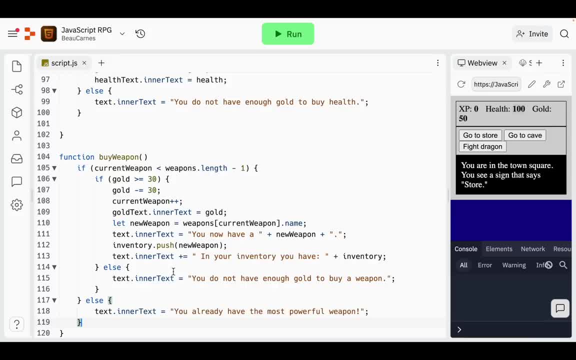 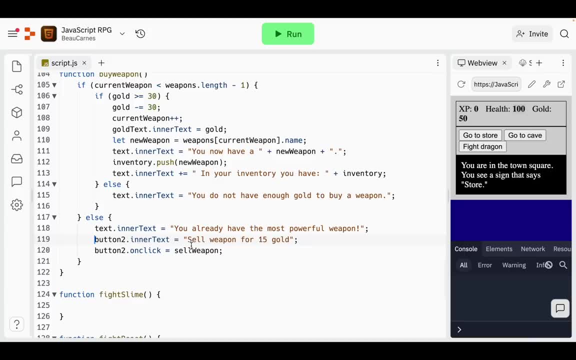 button two dot on click to the function name cell weapon. So just like that, so you already have the most powerful weapon and then the button is going to change And then you can. if you click it it will do cell weapon. So after the buy weapon function, let's create an empty function. 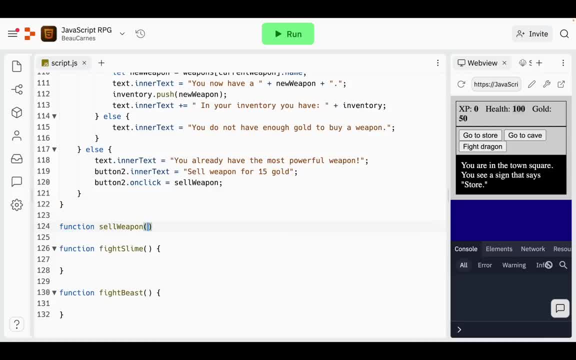 called cell weapon. So, first of all, pay players should not be able to sell their only weapon. So inside the cell weapon function we'll add an if statement with a condition that checks if the length of the inventory array is greater than one. Okay, and then inside this statement, 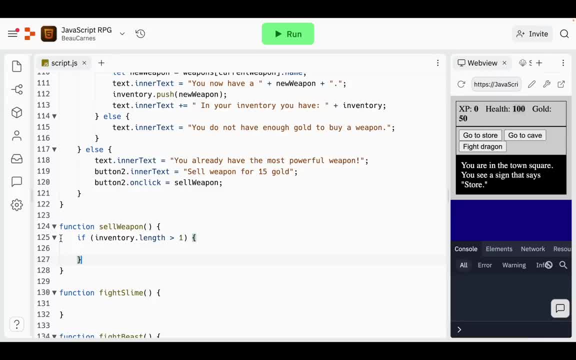 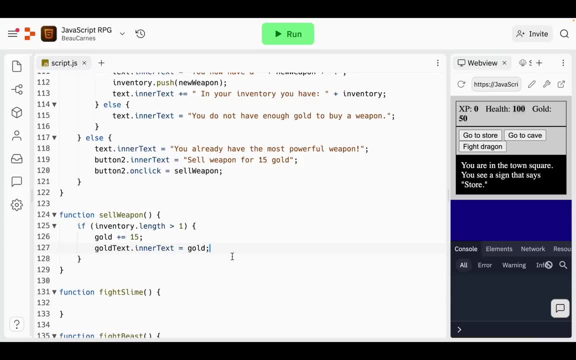 we'll set goal to equal 15. more than its current value and update gold dot inner text to the new value. Okay, now let's set use the let keyword to create a variable named current weapon, but we won't set it to anything. 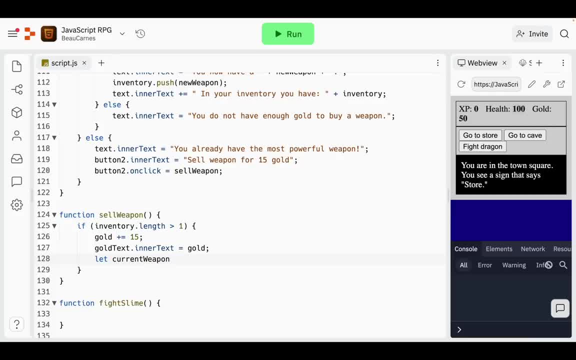 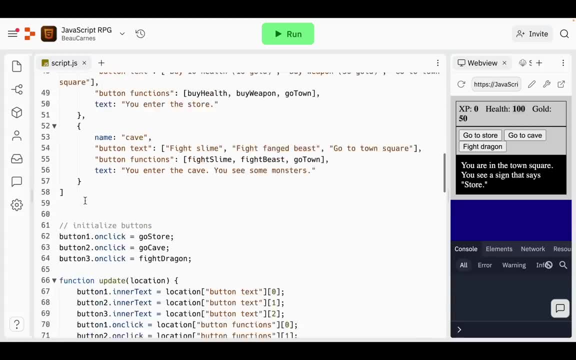 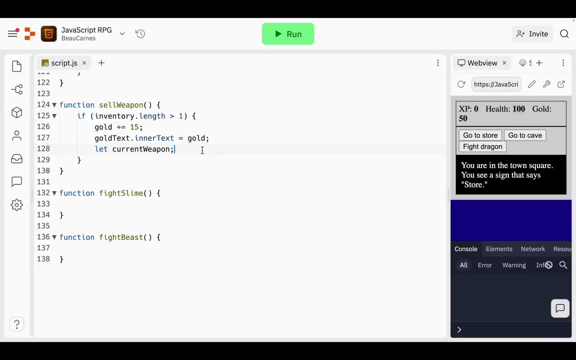 yet And if you notice, if you remember, we already have a current weapon appear. we've already have a current weapon that we've used And this and another function we've used in the by weapon function. But since we've created, since the let keyword is used instead of var, this new. 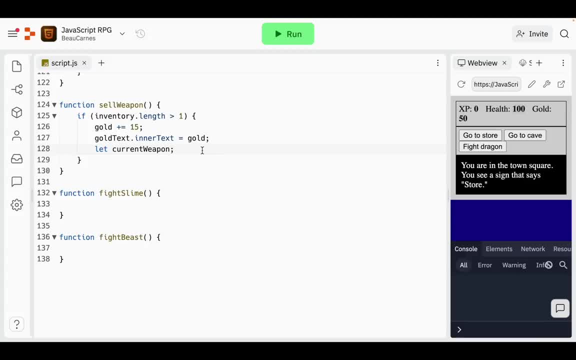 version of current weapon is scoped only to this if statement. So at the close of the if statement, once the if statement is over, then the old version of current weapon will be used again. So this will can't come out of the if statement because we use let. if we use var, then it would. 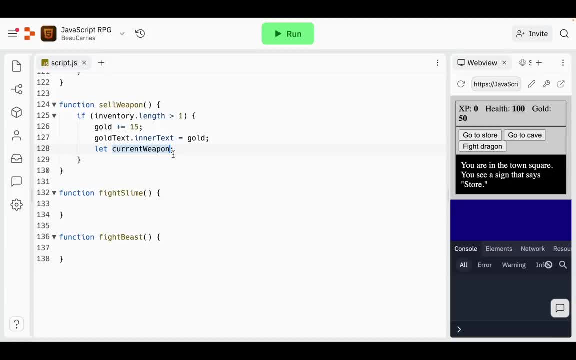 be able to be used outside of if statement. we're going to remove the first element from the inventory array and put it into this current weapon variable. we're going to use the dot shift method. So it's going to be like this: equals equals, inventory Dot shift. Okay, just like that. So shift is. 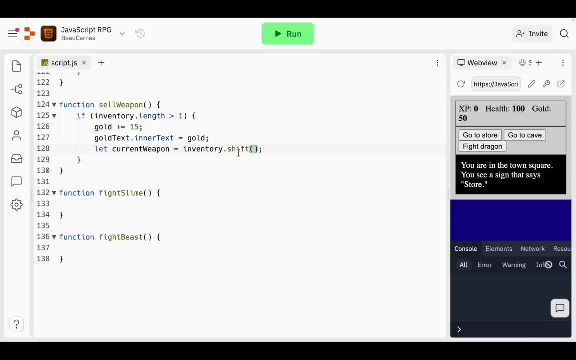 now removing the first element from the array and returning it into this variable, And now we'll just set the inner text to: you sold a and then put the current weapon. So it's just gonna look like this: you sold a plus current weapon, plus period. Now we can use the plus equal operator. 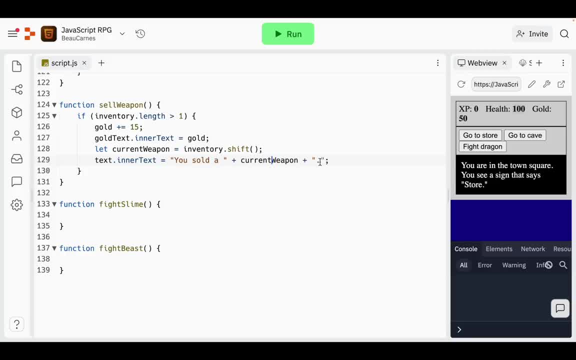 to add to the inner text and add the string in your inventory you have and then add the inventory variable at the end of the string, Just like that. So now let's add code so that if the length of the inventory is not more than one, 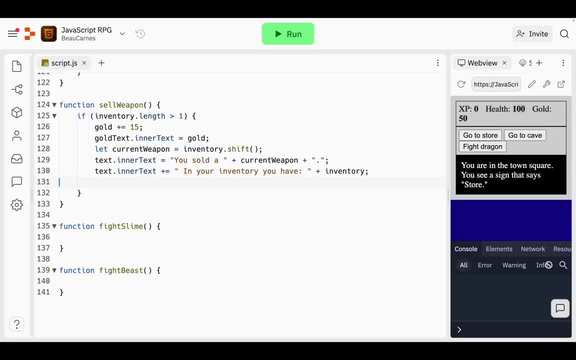 a text message appears. it says: don't sell your only weapon. So we can just do that with an else. So now we'll start working on fighting monsters. Let's organize the code by moving the fight dragon function to the bottom of the code, near the other fight functions. So I'll just go to fight dragon. 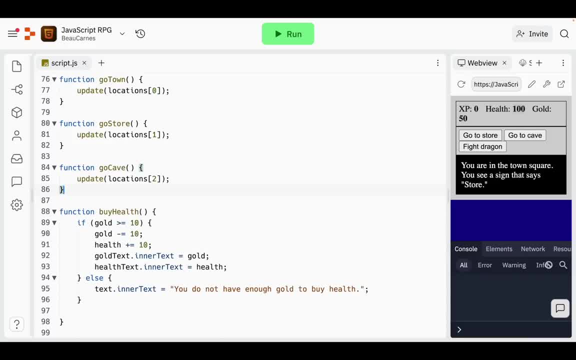 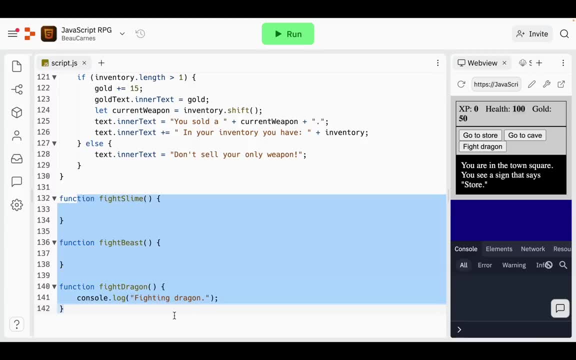 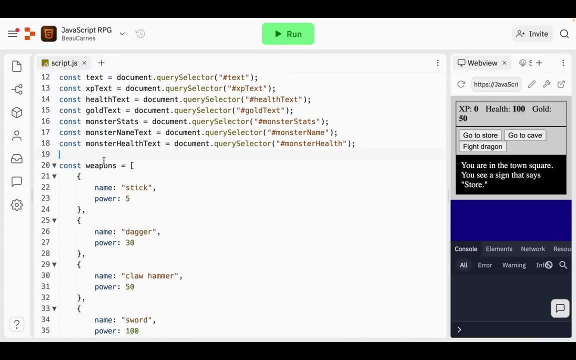 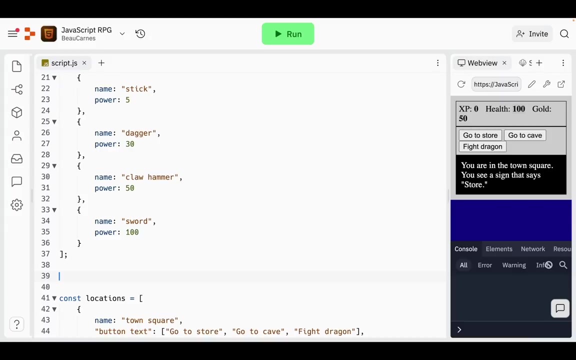 cut it and they'll just put it here. So now we have all the the monster fighting functions all together. Now below, where the weapons variable is declared. so we have the weapons. here we're going to create another array called monsters, And in the monsters we are going to set the 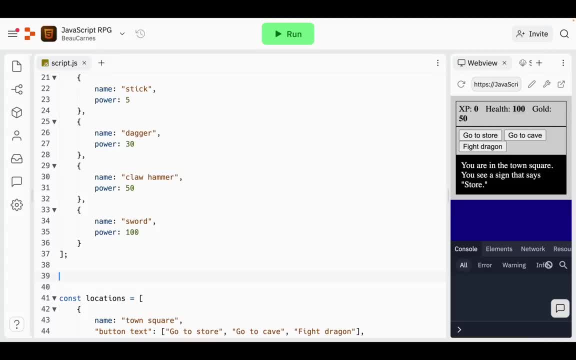 monsters, with three different monsters, And then we're going to do all the monsters. So we have monsters that each have a name, a level into health. This time I'll just show you, Okay. so see, we have the monster slime at level two- health 15,. the fang beast level eight- health 60,. 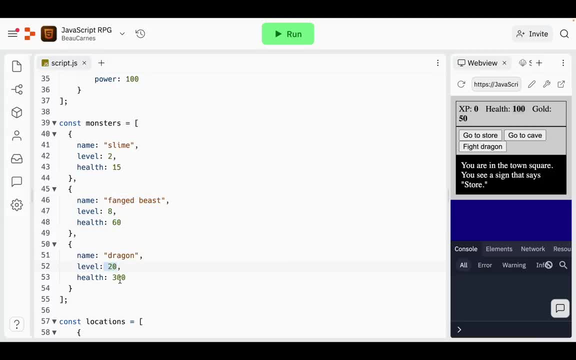 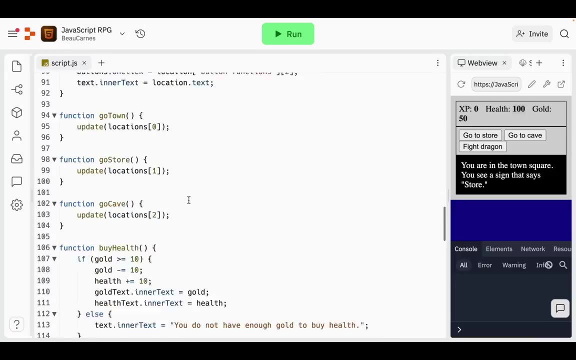 and the dragon level 20, and health 300.. And fighting each type of monster will be very similar. So all three fighting functions will call function named go fight. So at the end of the code let's add an empty function named go fight. Here I can just copy this function And this will be. 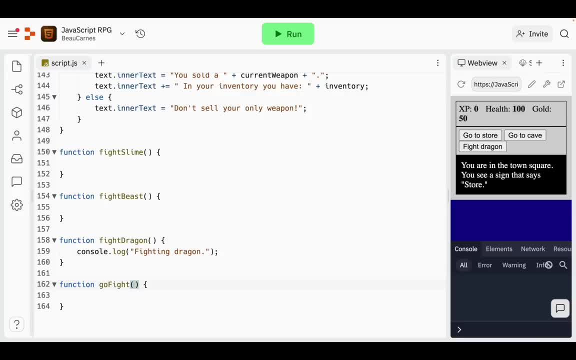 called go fight. So inside the fight slime function we'll set fighting to equal zero, which is the index of the slime in the monsters array, And then we'll call the go fight function. And so, just like this, fighting equals zero, go fight. And then we'll do the same for fight. 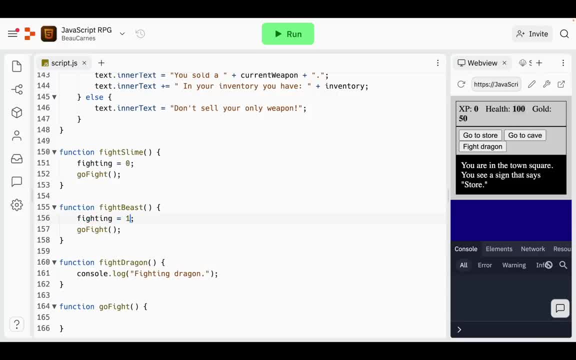 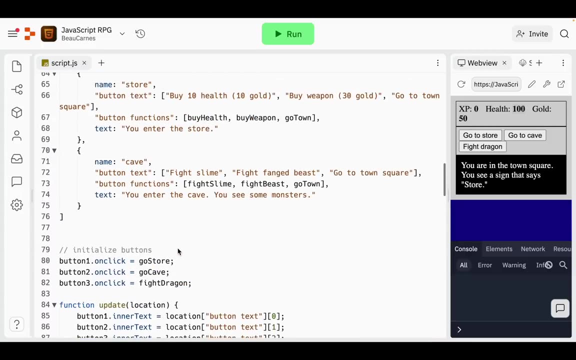 beasts and fight dragons. So this is going to be one, And then we're gonna. we don't need the console that log, and this is going to be two, So 012.. And now we need a new location in the locations array And it's going to have the same properties as other objects in the array. 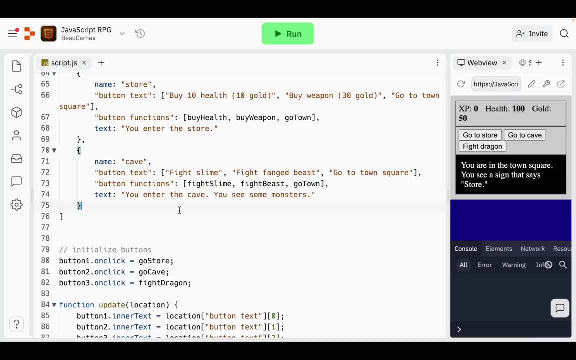 We'll set name to fight. the button text is attack, dodge and run, And the button functions are attack, dodge and go town, And we'll set the text. so you are fighting a monster, So just like that, And now we have an attack and a dodge. we need two more functions. Let's, so, let's, create those. 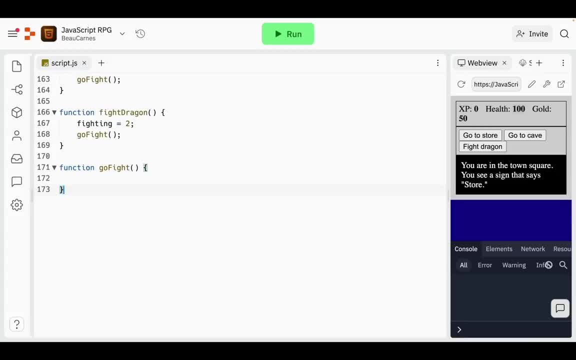 functions at the very end here. So we have attack and dodge. So in the go fight function let's update and pass in the location of the fighting location. So just like that, Next in the go kite fight function, we'll set monster health to equal the health of. 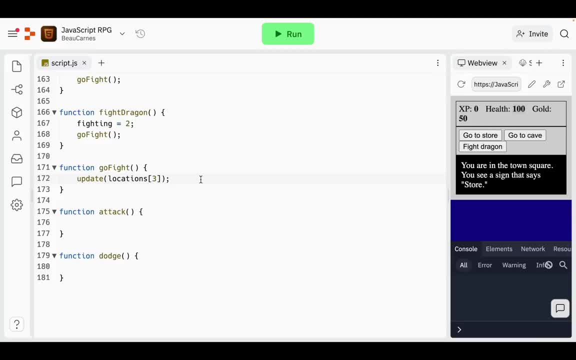 the current monster. You can try to figure that out first, or you can just wait for me to show you how to do it. So monster health equals monsters. So that'll be from the list of monsters, And then we have the index of what monster wolf we're fighting like, say, it was two, And then we're going to get 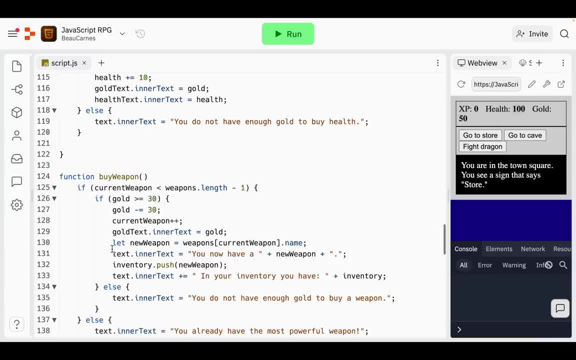 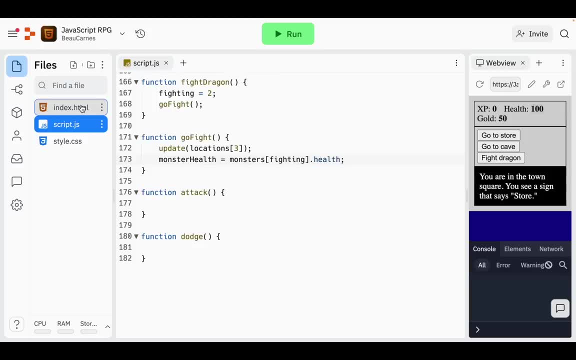 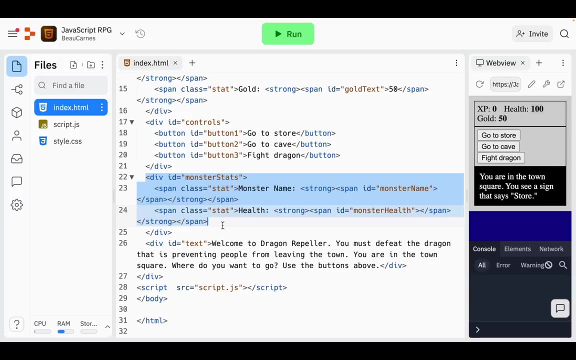 the health. So it's using the combination of bracket and dot notation. Okay, let's go look back at the HTML really quick. If you remember from when we talked about this, the HTML earlier, we have this monster stats, And the monster stats has a style of display. 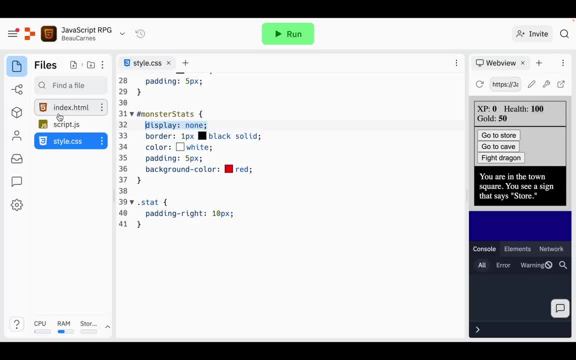 none. So it's hidden, it's not showing up. But when we're fighting a monster, we want the monster stats to show up. So we're going to display the monster stats. HTML- HTML element by updating its CSS display property to equal block. So you just basically do the element that style, that display. 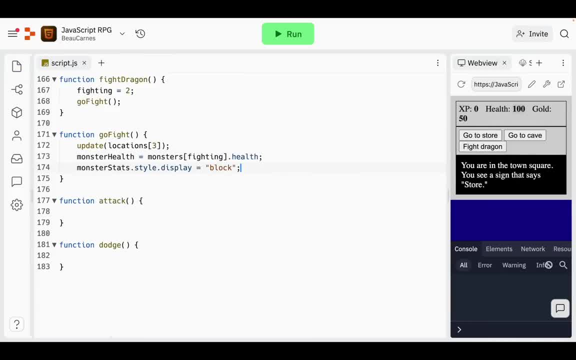 equal block. So it should just look like this: See monster stats HTML element. So it should just look like this: See monster stats HTML element. So it should just look like this: See monster stats. that style, that display, And this is if, if we use an element, that style. this is how we can. 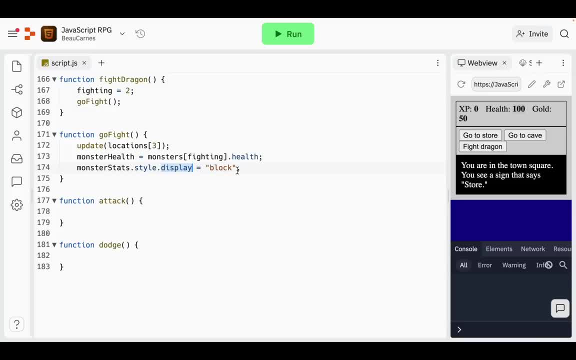 update CSS styles through JavaScript. Now let's set the inner text property, the MO, of the monster name text equal the name of the mouse for fighting, and the internet's inner text property of the monster health text to equal the monster health. so it should look just like this: So the name. 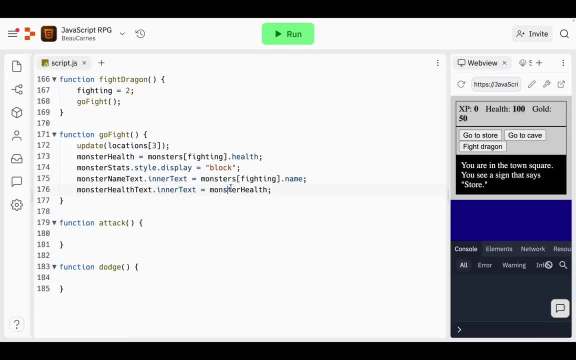 text is: monsters, the monster that we're fighting, the name property and then the monster health. we already got that from up here, So we'll build out the attack function. Now for the first line in the attack function. let's update the text message to say: the monster attacks, but use the 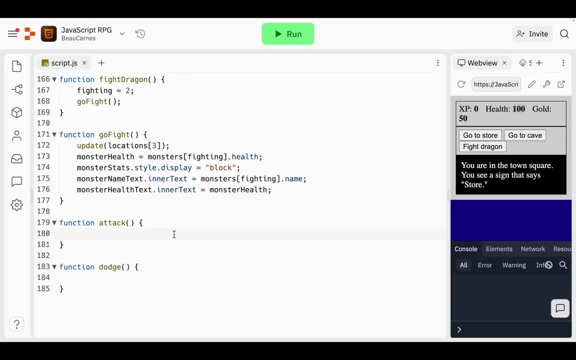 actual monster name of what the monster of which monster is attacking. So it's just gonna be like this: the monster- that's how we get the name- attacks. Okay, now we'll use the plus equal operator to append more text to text. that inner text we'll add the text. you attack it with your. 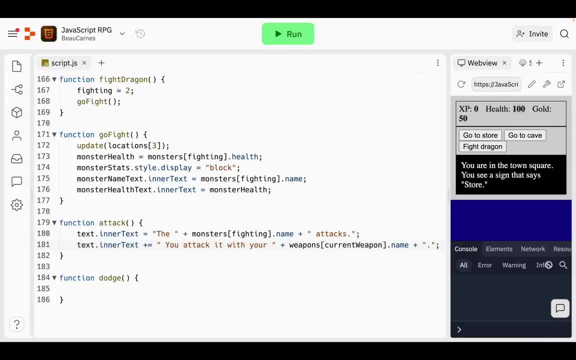 and then we'll say the weapon name. So that's going to be just like this: we have the plus equals, we have the space here, So have a space out of this period. you attack it with your and then we use string concatenation to get the, the weapon name here Now. now let's set the health equal. 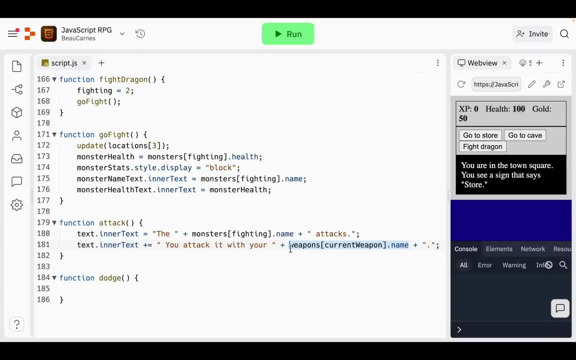 health minus, And then we're going to add the string concatenation to get the weapon name here, And then we'll add the monster health equal monster level And you can get the monsters level very similar to this, but instead of name it's just going to be level. 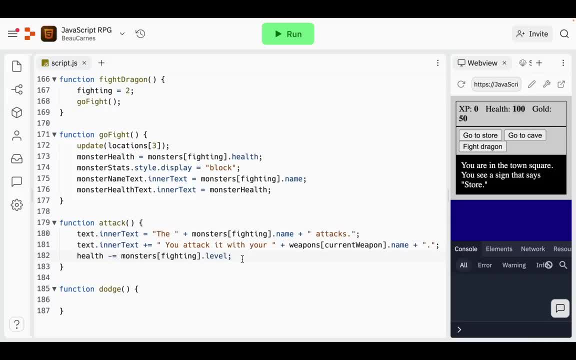 So, just like that, now we'll set the monster health to monster health minus the power of the current weapon. Okay, so when you attack, you get damage, the monster gets damaged, And then at the end of the line we'll add a random number. 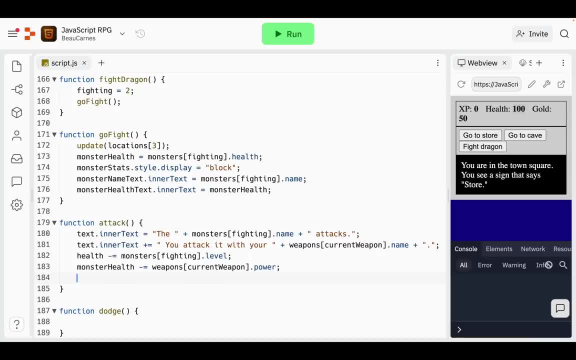 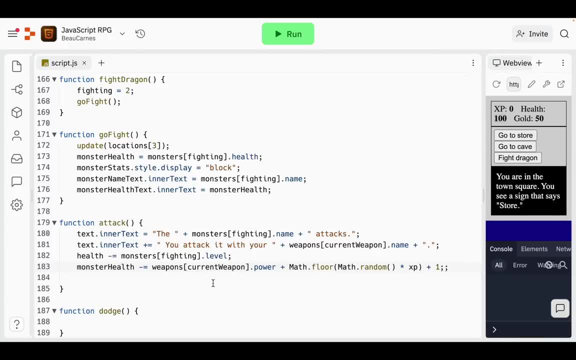 between one in the value of XP. that's the experience. So let me show you. I'll just paste that in here So you can see what that looks like. So we're subtracting from the monster health, the power of the weapon plus just some random amount based on the experience. So 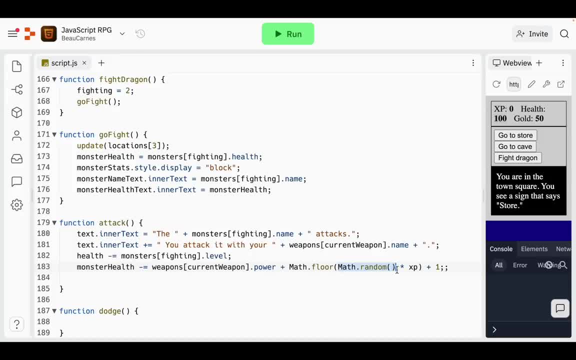 math dot random is going to create a random number between zero and one And then it will multiply it by the experience points And then math dot floor will round down, round down to the nearest whole number. So get this all rounded down to the nearest whole number. 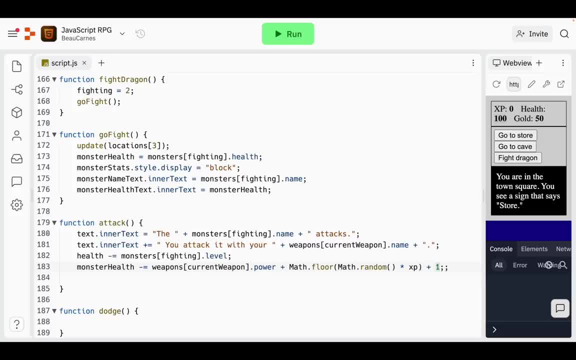 and then add one. So basically that's the formula for getting a random number between one and the value of XP, And we'll just update the inner text of the health and monster health And then we'll check if health is less than or equal to zero. 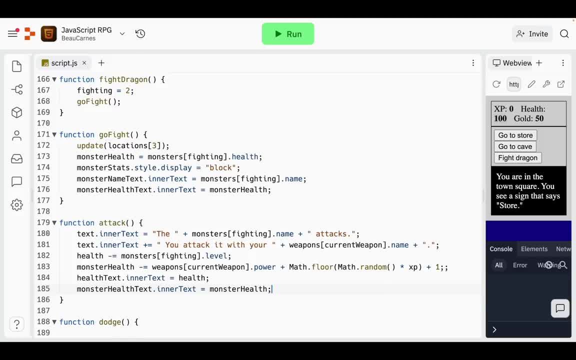 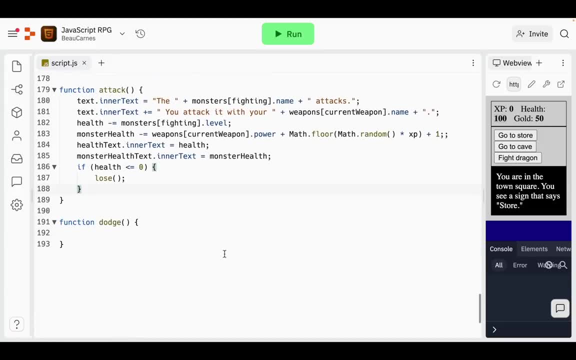 If it is, we'll call the lose function. So then remember, see if you can try to figure out this stuff before I show you. but that's just like this: if health is less than or equal to zero lose. So we've talked about if and else statements, and else statement can be conditional. 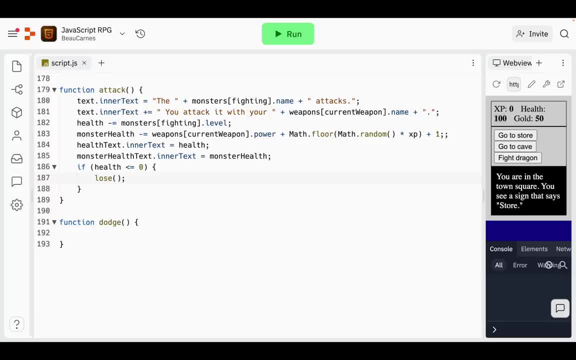 with an else if statement. So at the end of the if statement let's add an else if statement to check if monster health is less than or equal to zero, And if it is, we'll call the defeat monster function. So that just looks like this. So 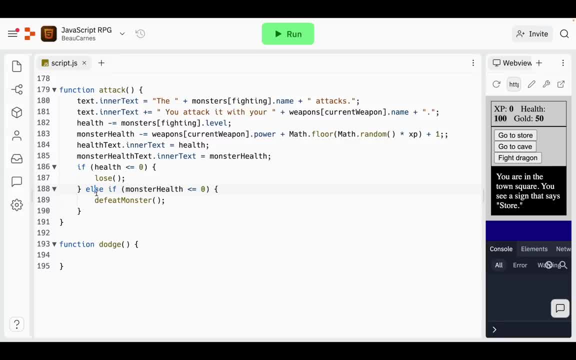 normally is else, and then we have a curly brace here, But now doing else, if, and we can put another if statement and then defeat monster. So if this else, then we'll do do another if statement. we'll only go to this if statement if this one is not true. So if we haven't lost and we'll. 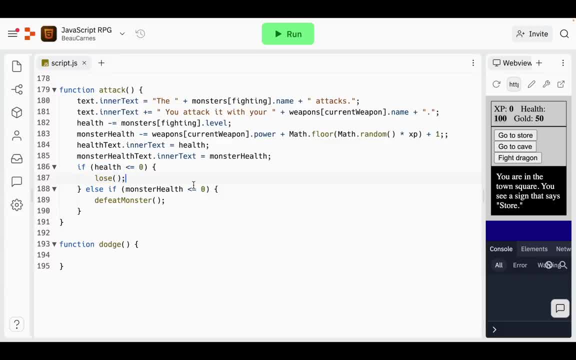 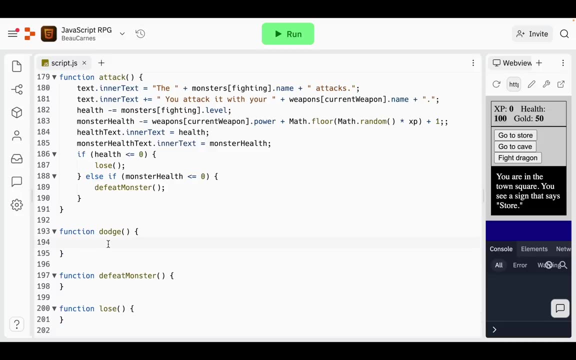 check if the monster has lost. if the monster's health is low, we'll call it defeat monster. So we'll just have to add those two empty functions for defeat monster and lose. Okay, there we go, And inside the dodge function let's set text. that enter text to you. 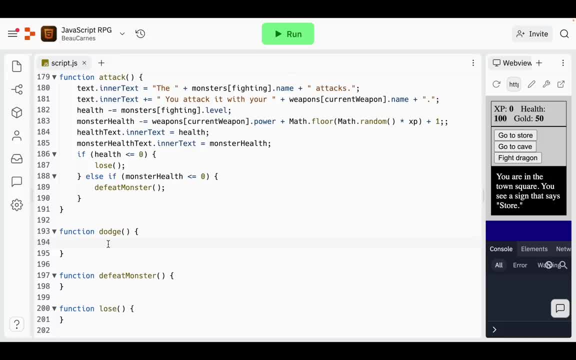 dodge the attack from and then put the monster's name. So, just like that, you dodge attack from and then monsters, that we get the monster who are fighting, the name and then the period, And then we can update the defeat monsters function. So inside this defeat monsters function. we're going to set gold to equal the monster's level. 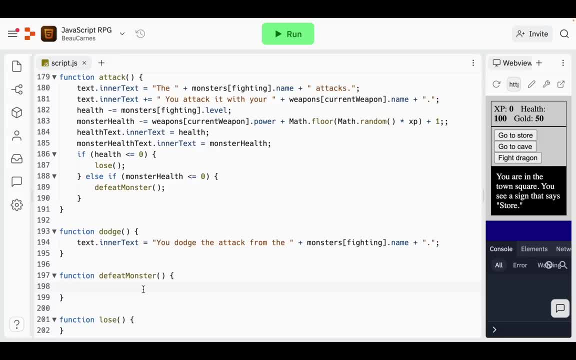 times 6.7.. But then we went around that all down to the nearest whole number. So, just like this, gold plus equals, And so we're going to add this, this new amount of gold which is going to be the level times 6.7.. And then round down to the nearest whole number. Then we'll set XP to equal. 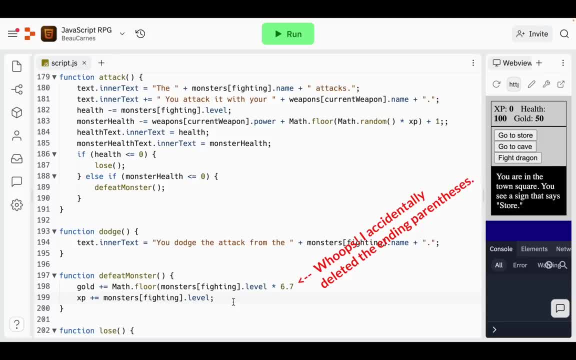 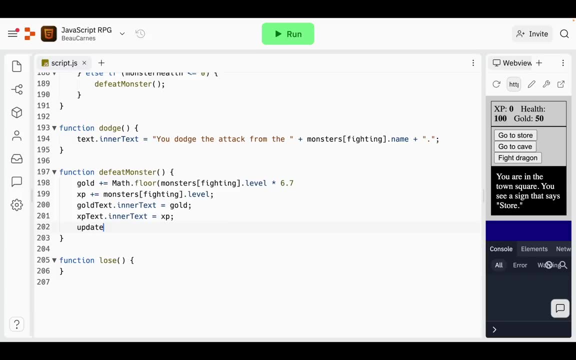 plus the monsters level, And now we just have to update the inner text on the screen And, finally, we'll finish this function by calling the update function and pass in locations for. so update locations for. so that's obviously a brand new location that we're going to have to add to the 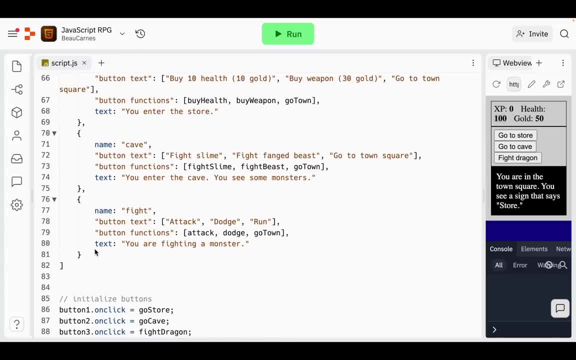 folder And then we'll add: add a new location. So just like that, we don't have to change it. We're going to do an initial changes here in the top right hand corner And what we're going to do is we're going to add an object and then we're going to add a new location, because that's. 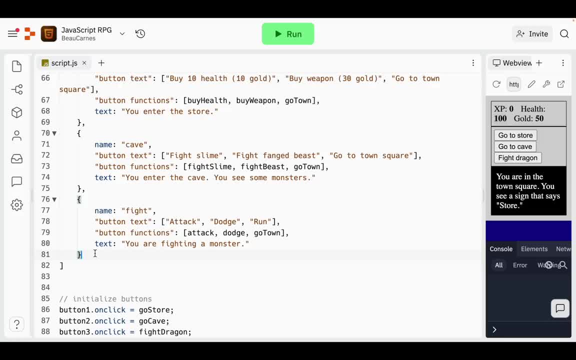 actually the fifth location index for, and so we're going to add a new location. what we're going to have? the same properties as all the other objects. the name is Kill Monster. the button text is go to town square. go to town square and go town square, because there's only one thing you can. 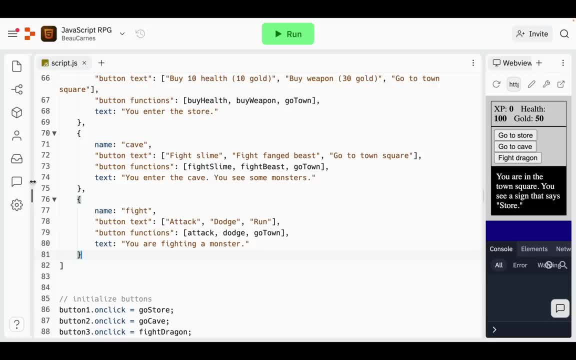 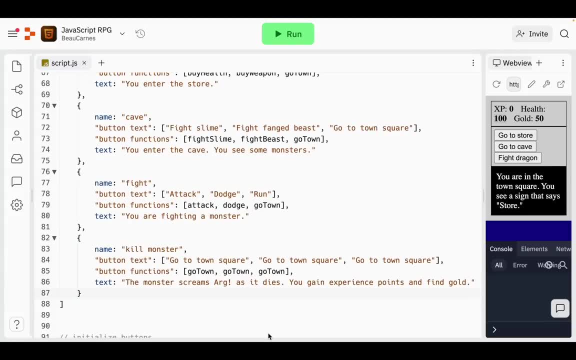 do after you kill a monster, And then the button functions go down, go down, go down And the text. So we have all that updated for what happens after you kill a monster. Now, where says the monster? screams are here. If you're saying something, there should be quotes around it, So let's add. 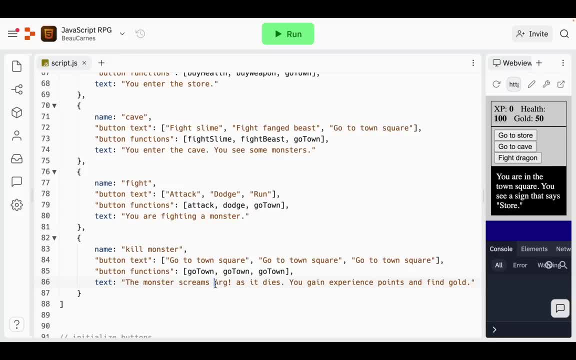 quotes around that. we already learned about escaping quotes. But there's another way you can include quote marks is if the outer quotes are a different type than the inner quotes. So if we want to have the inner quotes be double quotes, we can make the outer quotes single. 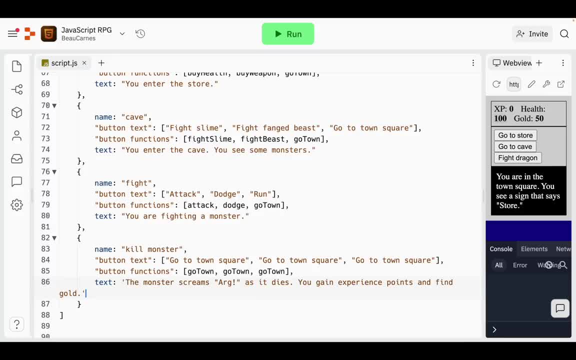 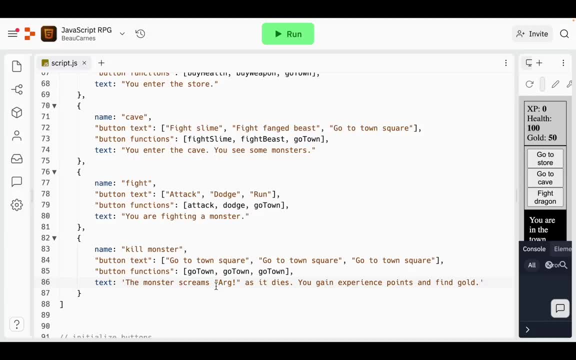 quotes. So let's do that. So now you can see the color all looks correct. So we're using the single quotes at the beginning and the end, So we can use the double quotes in the middle And that now these will appear and we don't have to escape them. they'll actually appear. this text will 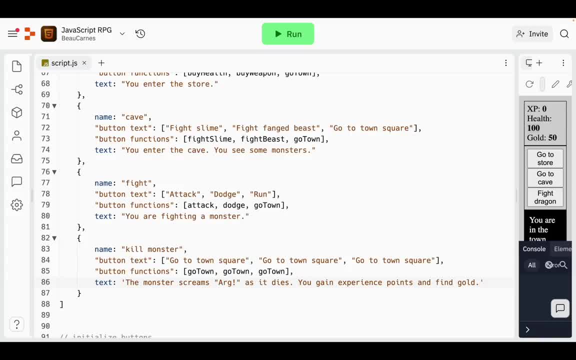 appear as with the quotation marks, And let's just add another location for when you lose name. lose button text is just all three says replay. question mark button functions are just restart And it's just going to say you die. So it's gonna look just like that. So there's only three options that can happen: The. 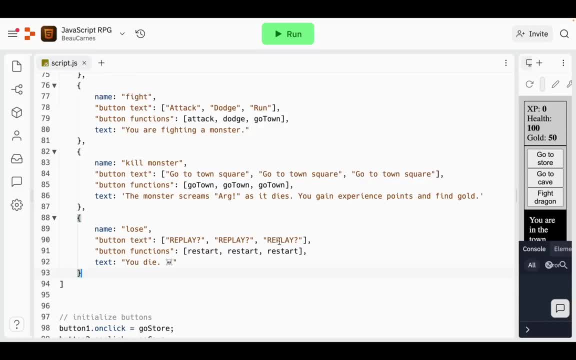 buttons all say the same thing And the button functions are all the same. So after a monster is defeated, the monster stat box should no longer display. So on the first line of the update function let's add that the monster stats style display is none. So every time you do that 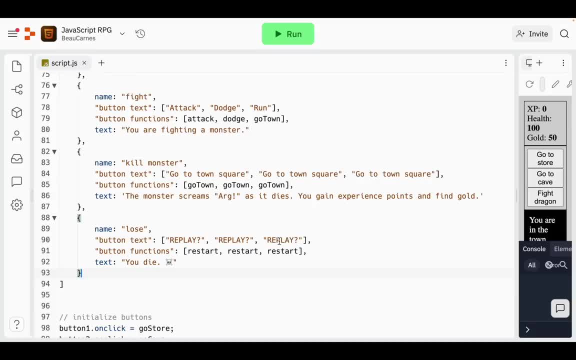 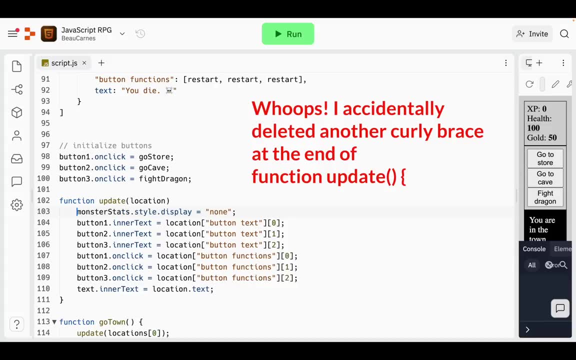 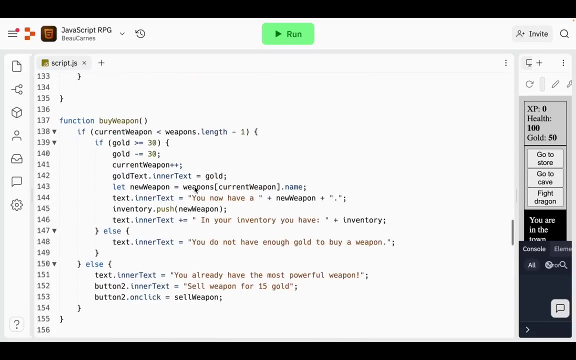 it updates, it's just gonna make sure that the display box goes away. the monster stats box goes away. So this is here And I'll just put in there. So whenever you go to a new location, the monster stats will no longer show up. Okay, now let's go use the loop that we have to lose. 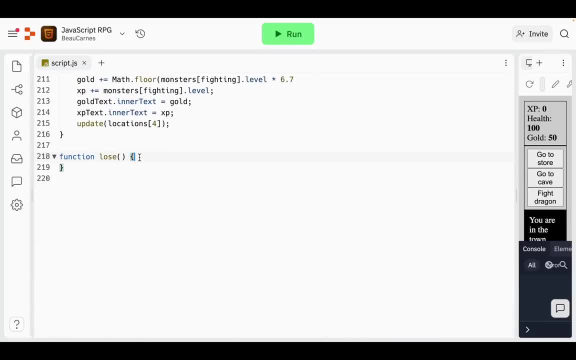 function at the bottom. So let's make it go to the correct location. Update locations Five. And now at the end we're going to make a restart function. So after you lose, you may want to restart, and we just want to set all the initial variables back to their initial. 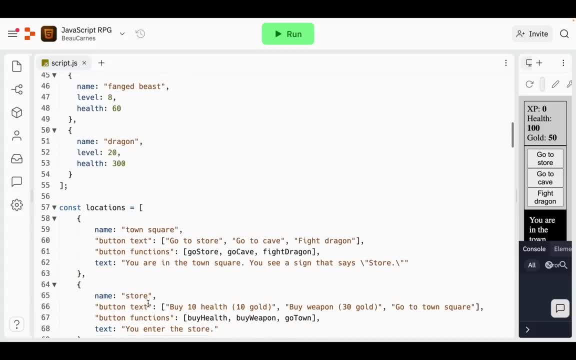 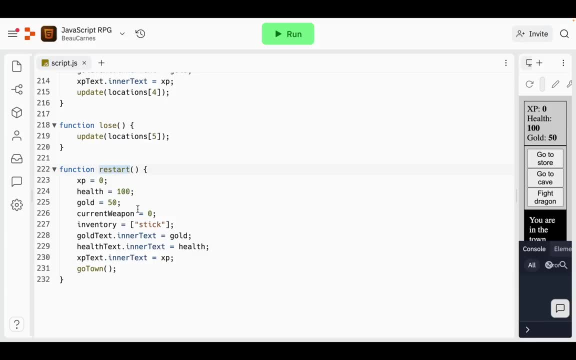 settings. And then we want to go to the town, So let's go all the way back to the bottom and create that function. So then we got restart and see we're seeing all the variables back to how they were at the very beginning. we're making sure the inner text of all these things on the screen. 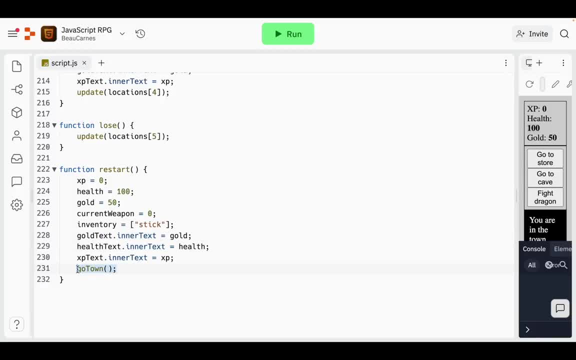 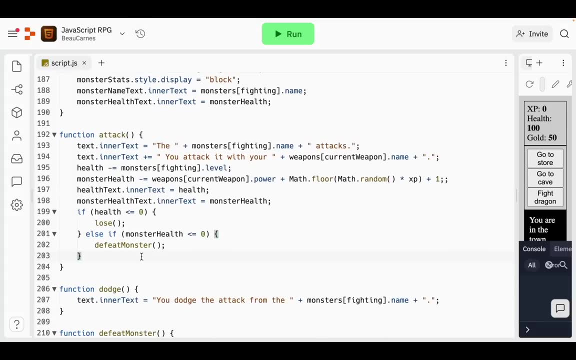 are the correct values, and then we go to town. Okay, now let's make an update to the attack function. Inside the attack function, we're going to update the contents of the else if statement. This is, which is this statement right here. So we're going to update the contents here. 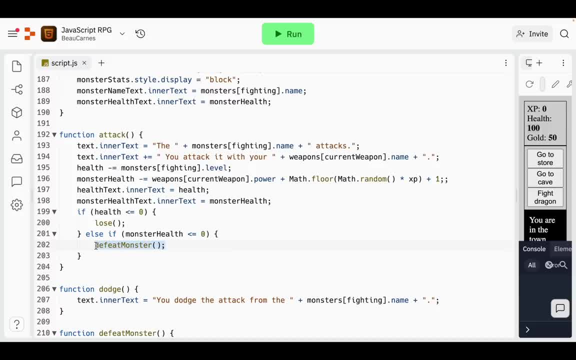 instead of calling the defeat month, instead of calling the defeat monster function right away, we'll create an if statement with an L statement. If the player is fighting the dragon, which is if fighting equals two, then we'll call the win game function. 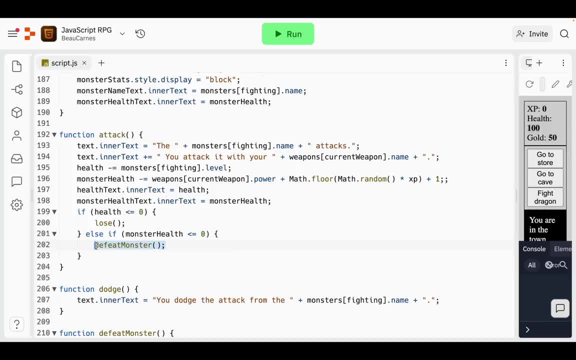 else we'll call the defeat monster function. So let me show you what that looks like. And we're going to talk about something new, which is this opera. So if fighting equals to win, game else defeat monster. So here you never just want to use a single equal sign, because a single equal 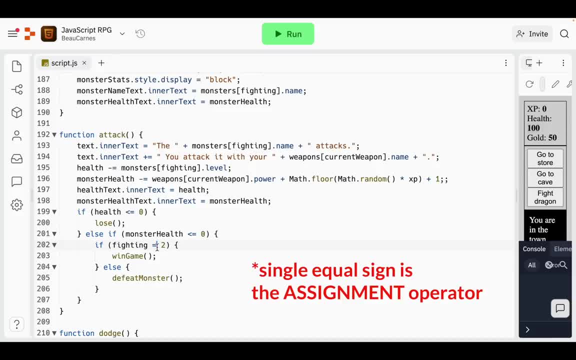 sign is an equal sign, And if you're going to use an equal sign, you're going to have to use an equality operator. you either want to use the double equal sign or the triple equal sign. If you want to compare two things, if you want to see if one thing equals another thing, 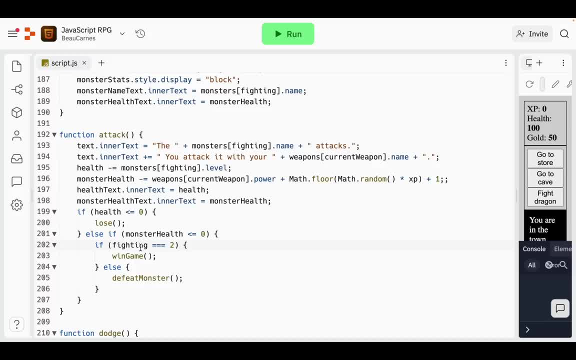 as far as comparing, you're going to use double or triple equal sign. So double equal sign, that double equal operator will compare for equality after doing any necessary type conversions and the triple equal operator will not do the conversions. So two values have. 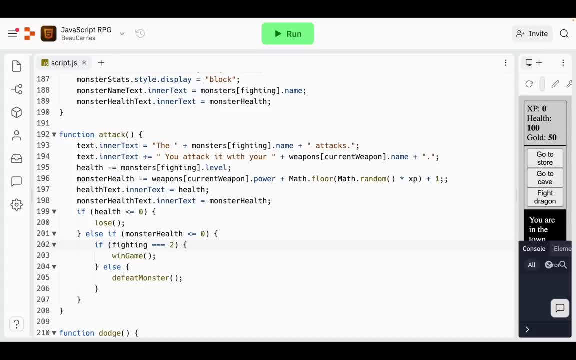 to be the exact same type. So it's often safer to use the triple equal sign, because it's not going to do any conversions to test the equality. And this is the perfect time to talk about the ternary operator, or sometimes called the conditional operator. It's basically: 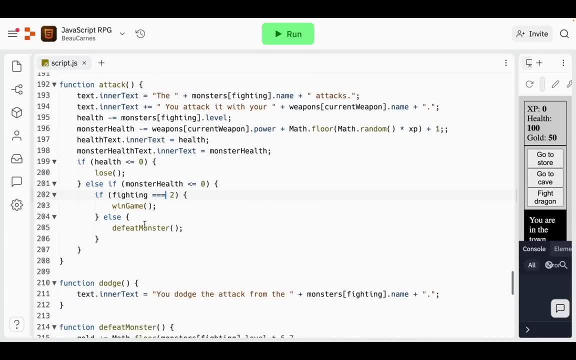 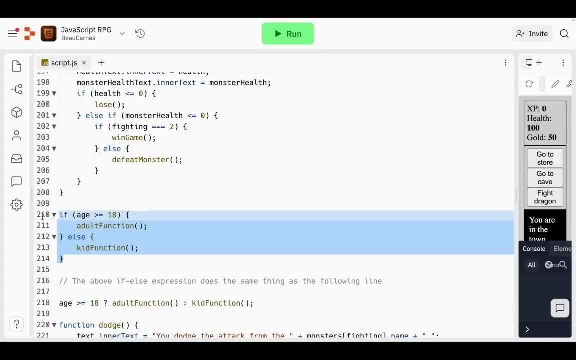 can be used to do a one line, if else expression. I'm just going to show you this: paste in some example code which we're going to delete. So the example. here's the example code. So if, if age is greater than or equal to 18, adult function, else kid function. we can simplify this. 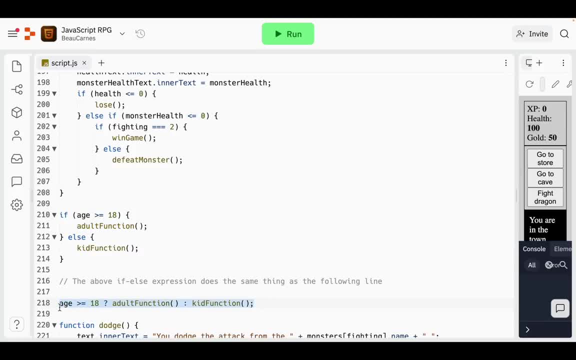 using the ternary operator. So basically, you put the what's in the if statement right here, and then we have a question mark And this would be the if true, and you will put a colon and this is else. So this is going to be the if true, this is the else. So the key things that we see here are: 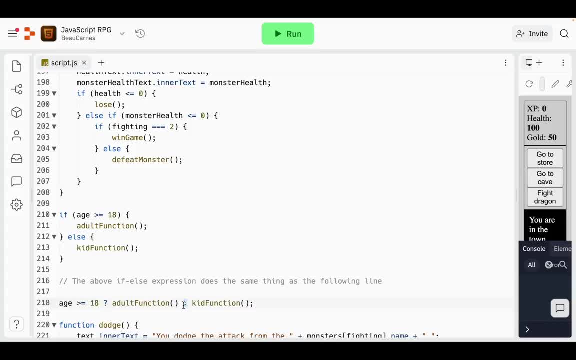 the question mark and the colon. So basically it's a one line if else statement when you only need it. they're very helpful if you only need to do one thing in the if, in one thing and else, which is exactly what we. 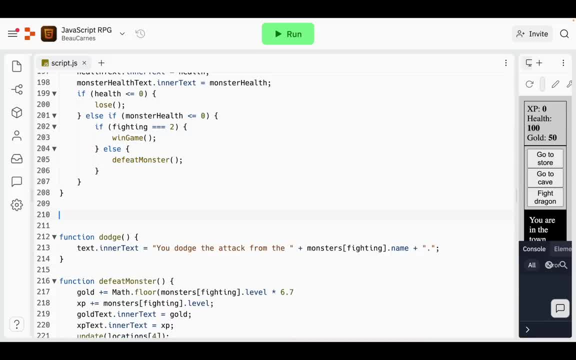 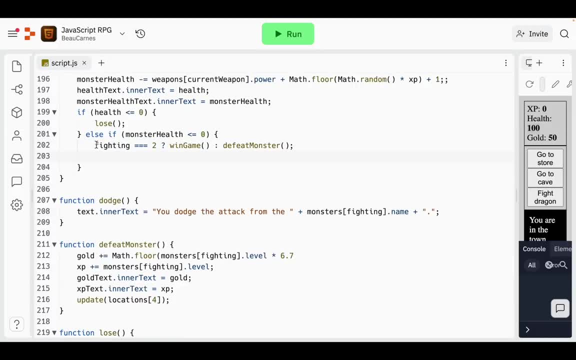 have up here. So I'm going to delete this And we're going to update this code to use a ternary statement, So it's just going to look like this. So, basically, it simplifies things quite a bit. If fighting equals equals. 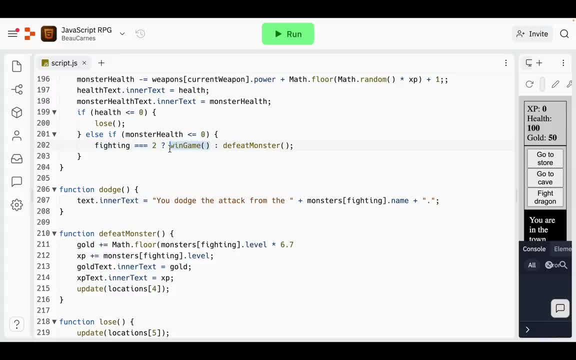 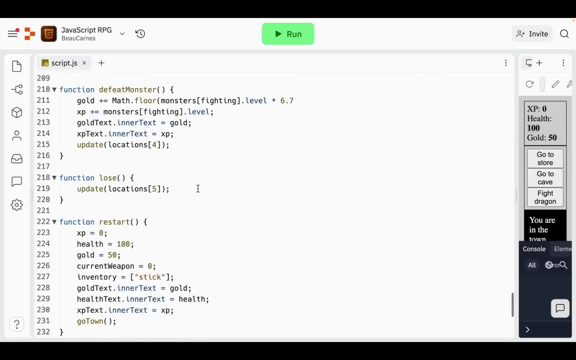 equals two. then if it's true, when game- if it's false, defeat monster. Okay, after the lose function we're going to create a new function called when game and inside that function we'll call the update function and pass in location six. So you can see. 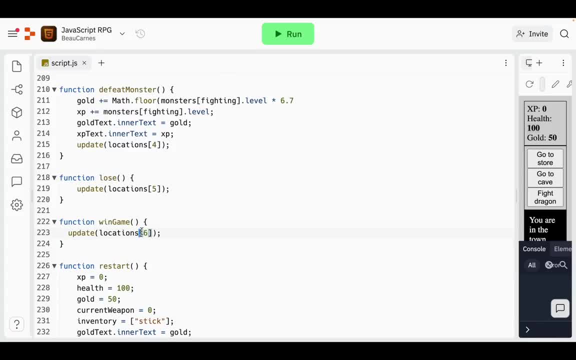 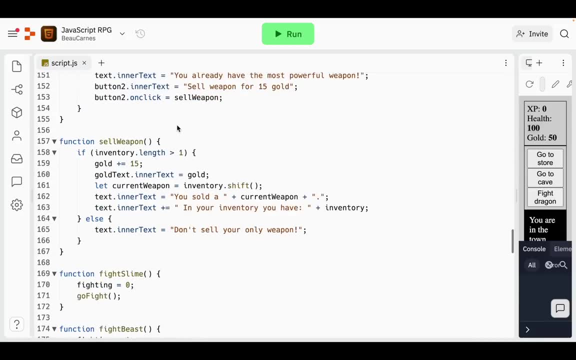 it's going to look very similar to the lose function. we're just calling location six And that's a new location. So let's create a new location. Everything should basically be the same as the lose location, except the names. when we win And instead of saying you die. 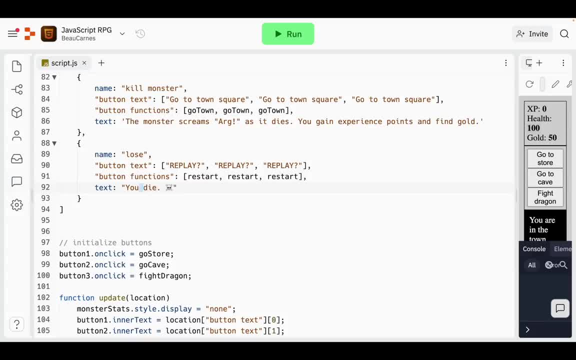 it will say: you feed, defeat the drag and you win the game. Just like that. the replay and restart are going to be the same. Now the game could be complete. Now we're going to add a few extra features, But let's test it out. So I'm going to click run up. 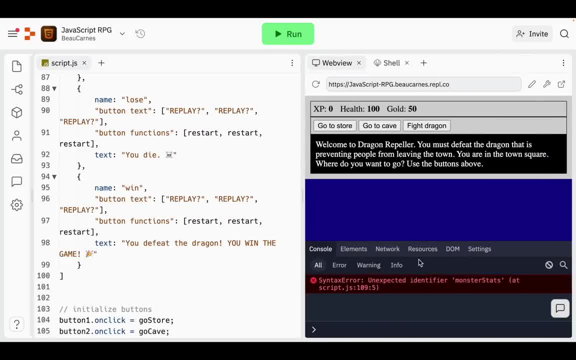 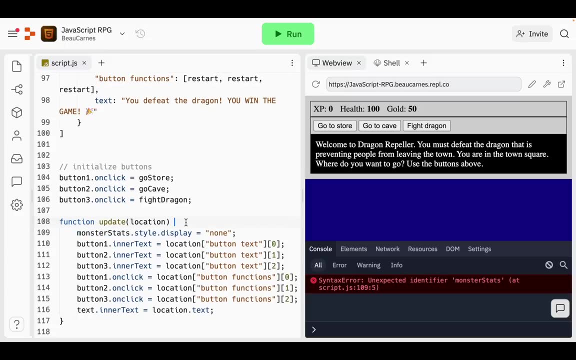 here And we'll be able to see if we made any mistakes already. So, monster stats, unexpected identifier. So let's go to line 109.. And it looks like it's because we forgot this curly brace, or I forgot it. Hopefully you got it right, Because I'm probably put a little note at the time. 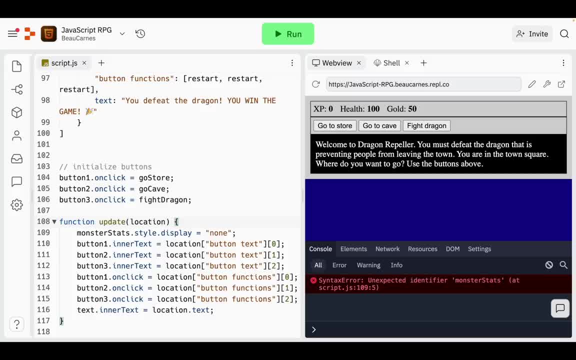 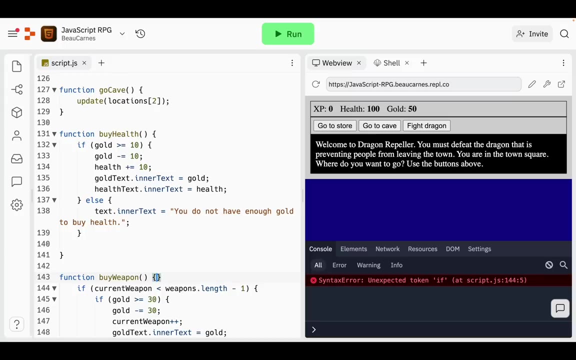 saying that I made a mistake there. So this is why it's sometimes helpful to test out your code more frequently, So you don't have a air a while back. So let's try it again. So click Run, And then we have another error here. So let's check that- 144.. And again it's just a missing curly. 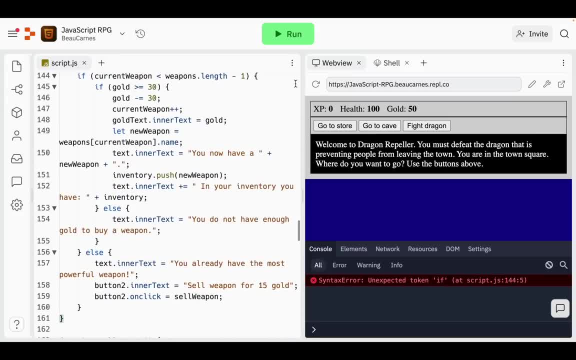 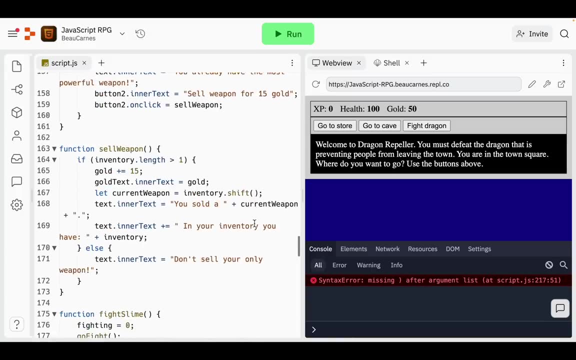 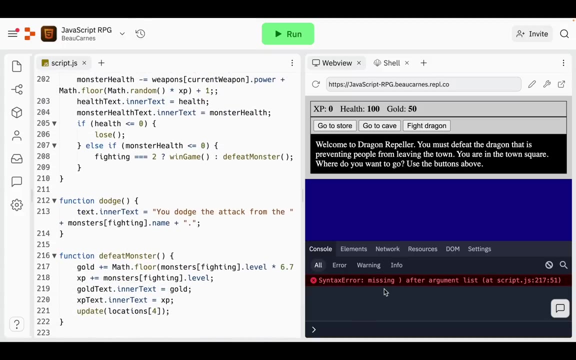 brace And hopefully we don't get any more of those missing curly braces. Okay, And then we have a missing semicolon, So at 217.. One thing this helps you realize is that finding errors can actually be easy. just by looking at the console and the errors you get right in there. 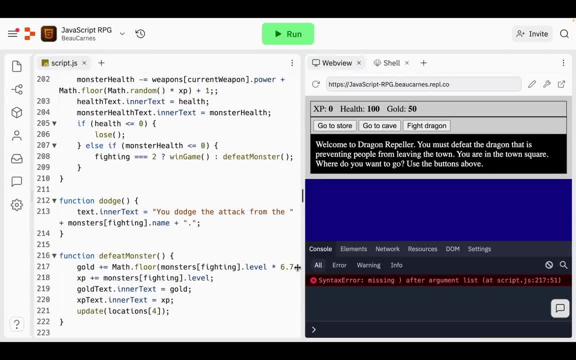 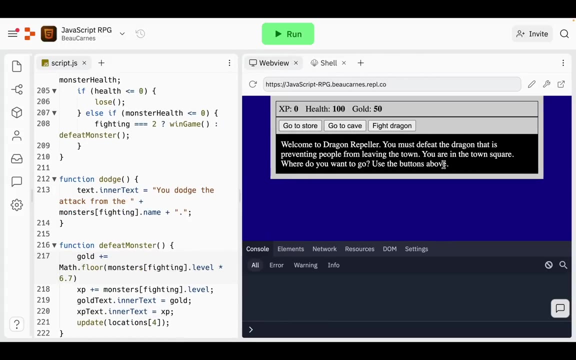 So it looks like we just need to have a semicolon here. Okay, And no more errors. I fixed my mistakes that hopefully you already had fixed in your code. Okay, so let's test out the rest of this application here. So, welcome to dragon repeller. So we have all this information here. 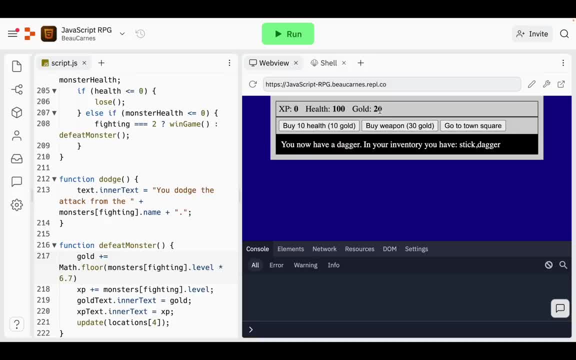 go to store, Let's see if we can buy a weapon. Yep, my gold went down And now I have an extra thing in my inventory: I can buy some health, And my gold went down, my health went up. Let's. 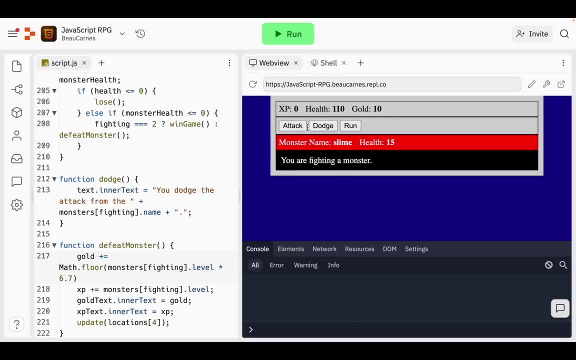 go down to town square. go to the cave. I'll fight the slime. Name: slime health 15.. You are fighting a monster I am going to attack And my health went down. My experience went up And it tells right here what happened. So go to town square. I'm gonna go to the cave again. fight the. 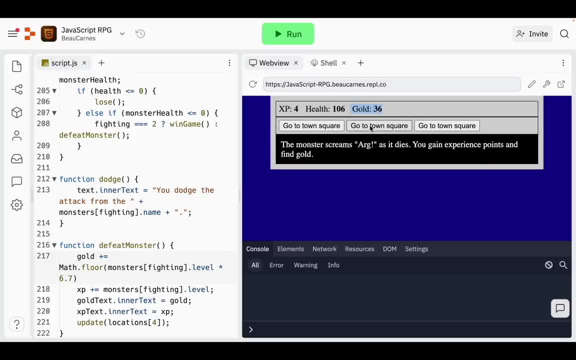 slime attack. And now I have more gold So I can go to the store and buy a better weapon. Now I have a claw hammer, So I'm going to go to the cave And now I can fight the thing beast and attack that a few times. 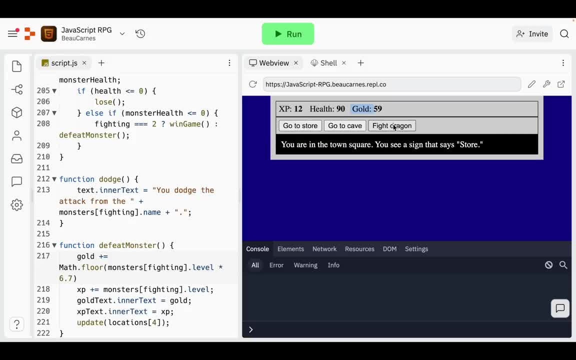 I defeated it. Now, let's just- I'm not going to check every single thing here, But let's check what happens if I fight the dragon and die Attack. Okay, my health is going down quickly. I don't have the most powerful weapon, yet You die. See, my health went down. So if I replace 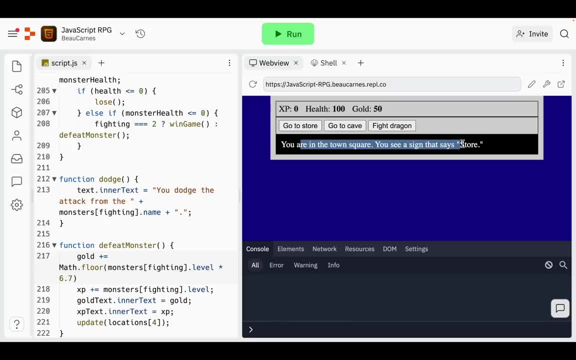 play. yep, it starts back over. You are on the town square. you see a sign that says store. Great, everything seems to be working so far. Okay, let's do a few things to make the game even more interesting. First of all, I'm going to close the console here. we don't need that. 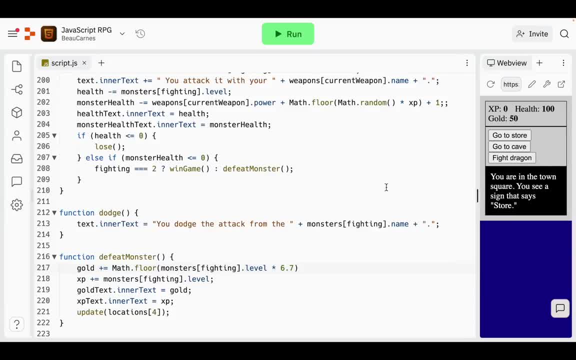 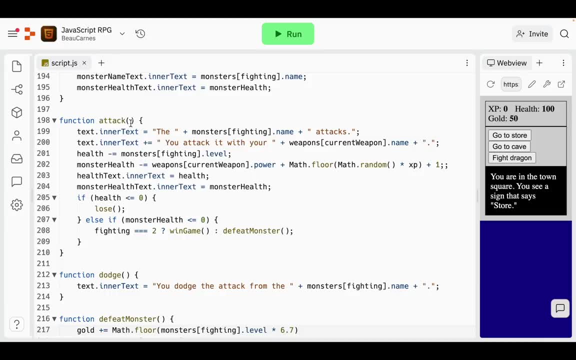 anymore. We're gonna bring this over. And now let's go to the attack function. So in the attack function, we're going to change this line right here to something that's going to be a little more complicated, basically. So instead of just subtracting the level of the monster we are, 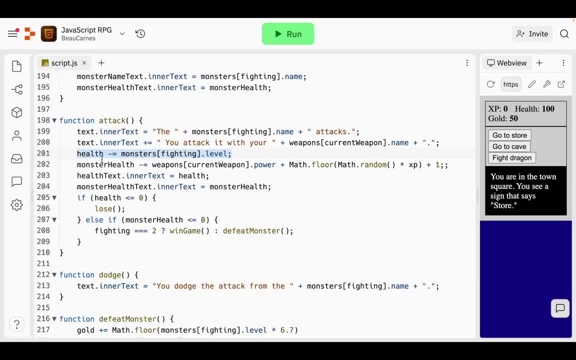 going to get an attack value based on the level of the monster. So I'm going to put in a. I'm going to call a function here actually. So get monster attack value. And then I'm going to pass into the function the level of the monster. So we're. 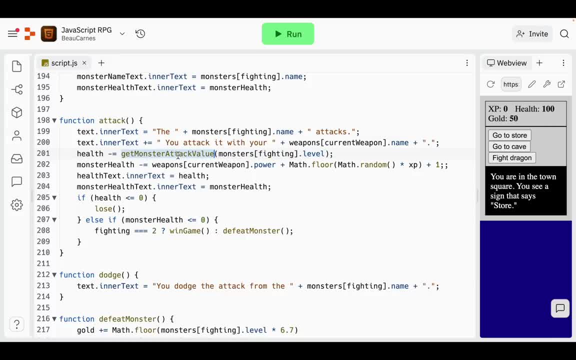 passing in the level of the monster to this function And this whole function is going to return a number that's going to be subtracted from the health. So let's create that function. So we're going to call that function to me right here. it's going to take a level, So get monster attack value. 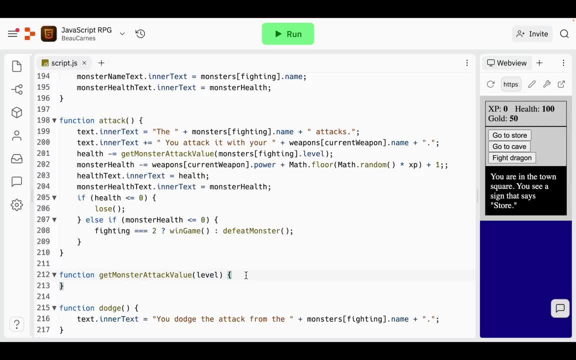 it takes in a level. So we're going to call that function. it's gonna be right here. it's going to level here And now. the attack of the monster will be based on the monsters level and the players XP. So in this function we'll use let to create a variable called hit and we'll set it to. 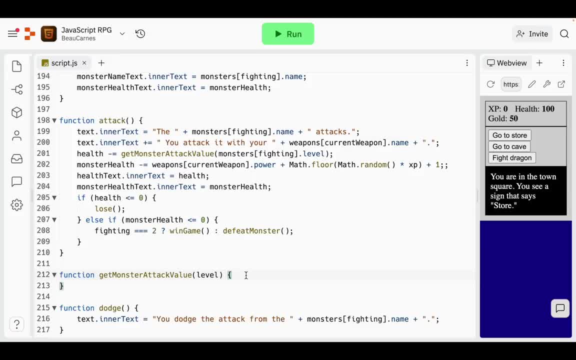 equal to an equation. Let me just show you, instead of explaining it to you first, So you can experiment with different equations to figure out what the attack value is going to be. But in our case we're doing. we're first we're multiplying the level, the monster times five, And then we're. 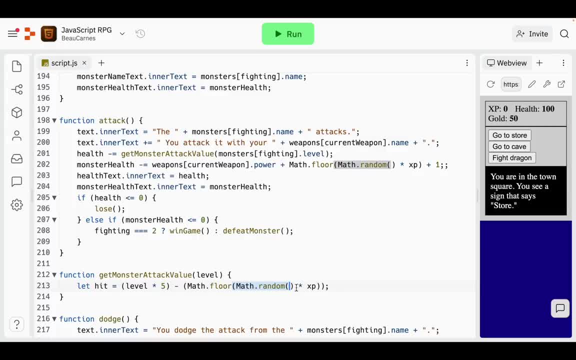 subtracting. Well, we're getting a random number times XP And then we are rounding it down. So let's do a console that log. we're going to log the value of this of hit to the console to use in debugging. This is something we talked about in the previous video. we talked about it in. 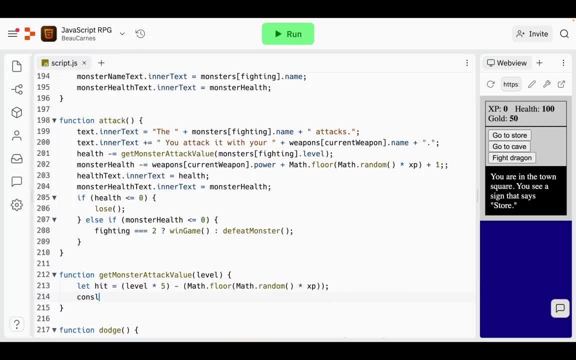 at the beginning console dot log. so do console dot log and then pass in hit. And now we're going to do something we haven't done before in a function is to return a value. we already talked about how we're going to get the return value to pass into health, But we haven't created a 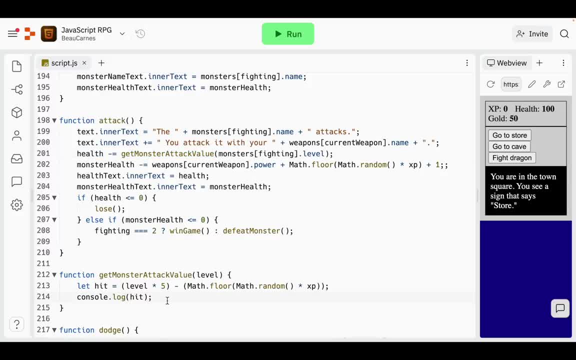 function with the return value yet. So we're going to return, we're just going to use the return keyword And then put hit. So just like this, return, hit, Okay. so now, when we call this function, it's going to return a value that we can then use in this health equation up here. Okay, 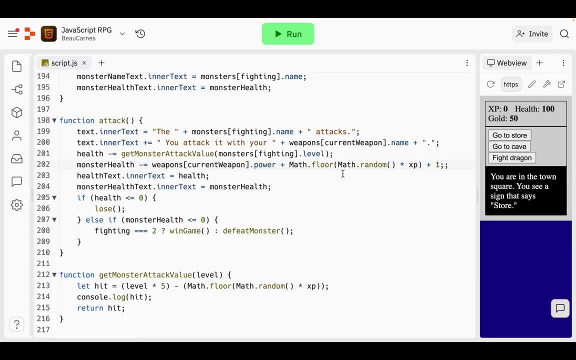 now we want to make it so a player can potentially miss when they go to attack. they can miss. So first of all, there's an extra semi colon here. So extra semi colons basically don't do anything. they're not, they're not going to make your, your code fail or anything. So 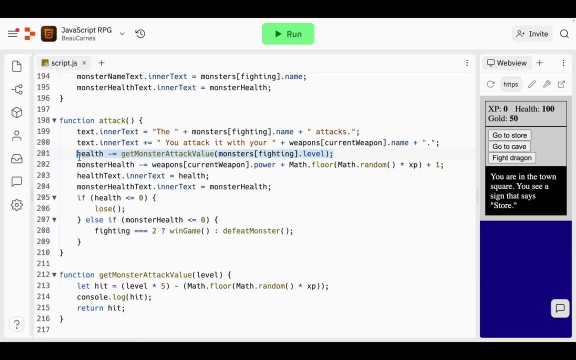 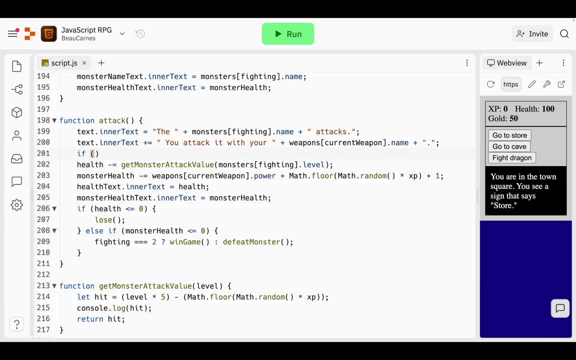 we want to put this whole line in an if statement. So if, and then the condition of the if statement is going to: we're actually going to call a function to get the result to see if this is true or false. So we're going to say: if is monster, hit is monster. 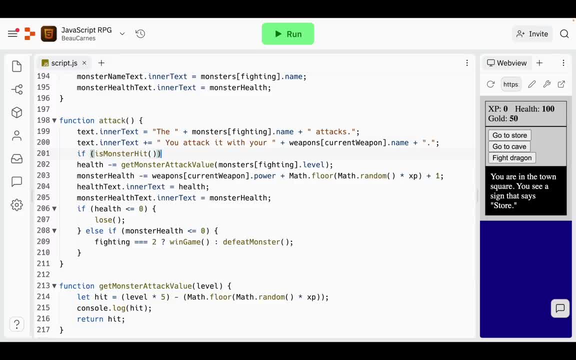 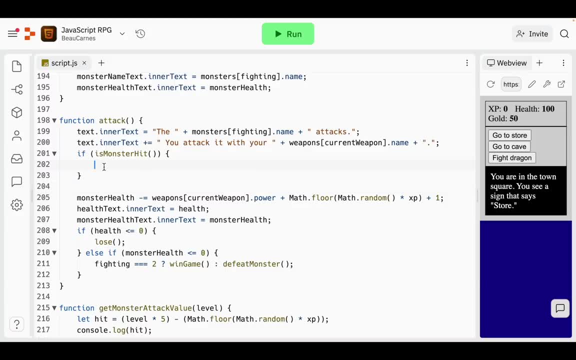 Hit And we're going to check if the monsters hit And if so then we are going to subtract from the health And if the monster is not hit we'll have an else And we'll use the plus equal operator to add the text you miss on to the end of text. dot enter text. So it's. 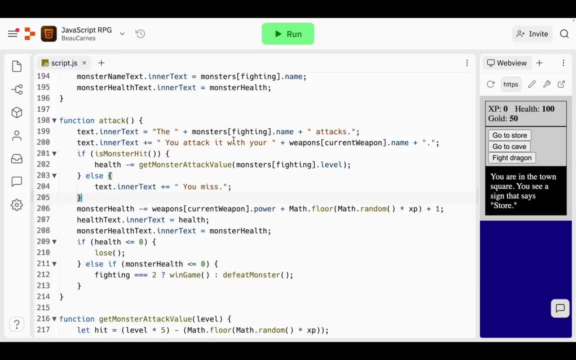 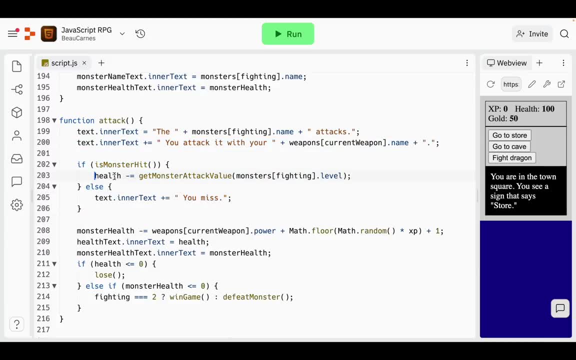 just going to look like that, So maybe I can even put some lines on here. So we're going to see what happens. So if the monsters hit, we'll subtract this attack value. If not, you miss, Obviously. we now have to create the is monster hit function. we're going to 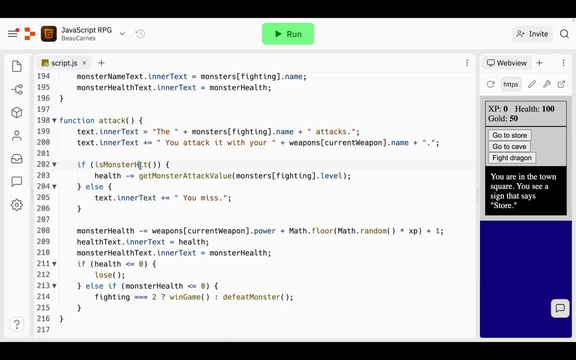 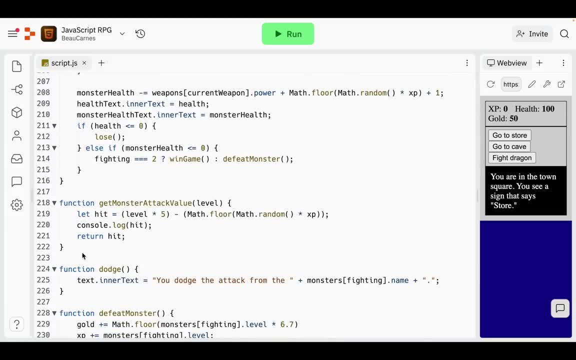 use the math dot random function to make it so. 20% of the time it's a myth and 80% of the time it's a hit. So after the get monster attack value, I'll make another function, other function, And this is how we're going to do. that is monster hit. we're going to 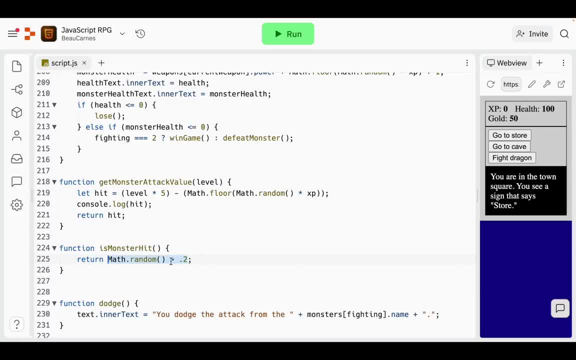 return. and then we're going to do a conditional. anytime you have a conditional like more than less, than more than equal to, or like the double equal sign, the triple equal sign, it's always going to return a true or false. So math dot random. if you remember, I said it gives a. 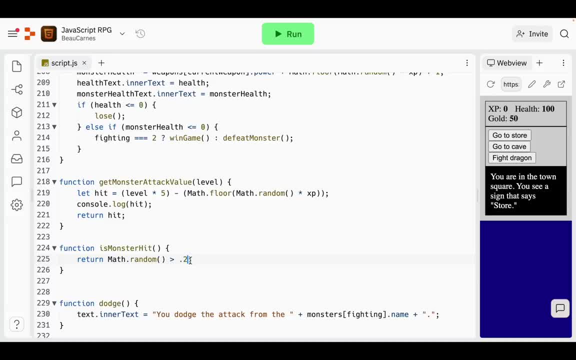 number between zero and one. So so point two, that's basically 20% of time it's going to be point two or less, And then 80% of times can be above that. So it's going to return when math, that if math that random is greater than point two, that's 8% of the time it's going. 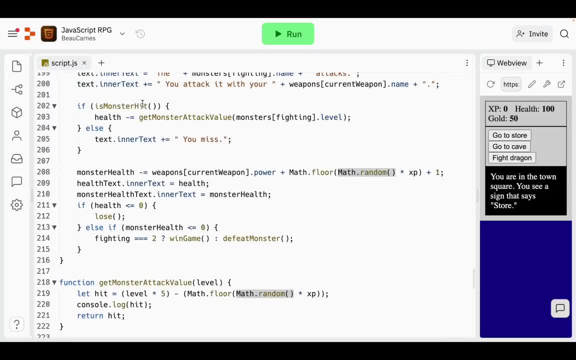 to turn true, otherwise false. So 2180% of the time there's going to be a hit. Now we want to. actually, the player should hit if either math that random is greater than point two or if the player's health is less than 20.. So basically, it's always a hit if 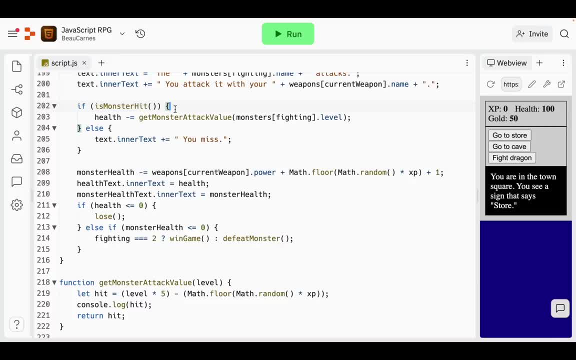 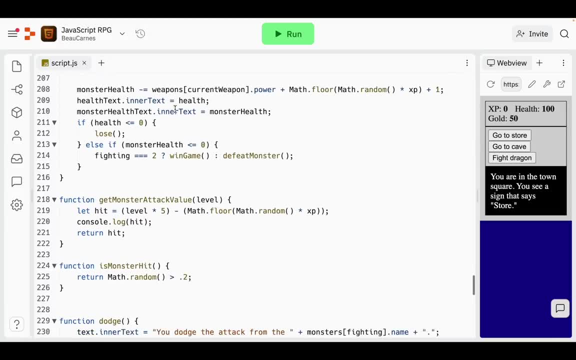 the player's health is less than 20.. So let's look at this. Let's look at how you can use an or in an if statement. So you can check for two conditions in an if statement. So we actually want to return true under two conditions If math. 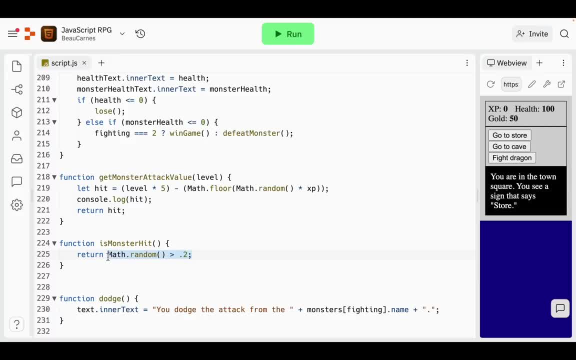 that random is greater than point two, or if the player's health is less than 20.. So if the player has low health there's always going to be a hit. So at the end of the return statement we're going to add the logical. 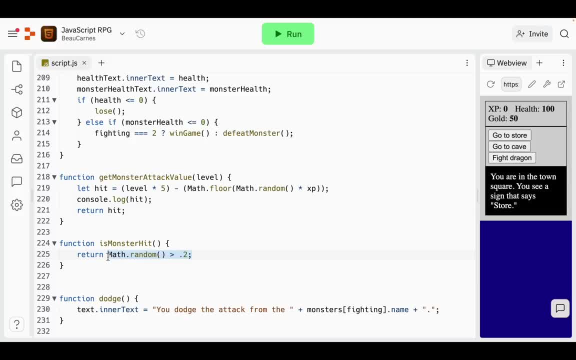 Or operator, which is just two straight lines, and then we can check if health is less than 20.. So let me show you what I mean. So this is the two straight lines, this is the or operator. So we're checking for this or this. So if either one of these is true, then it's. 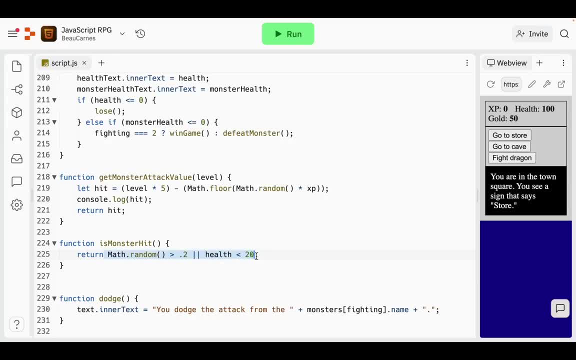 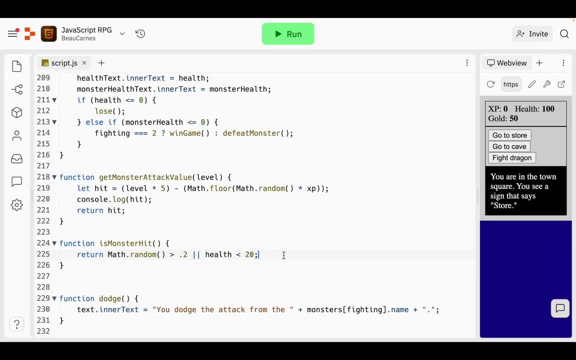 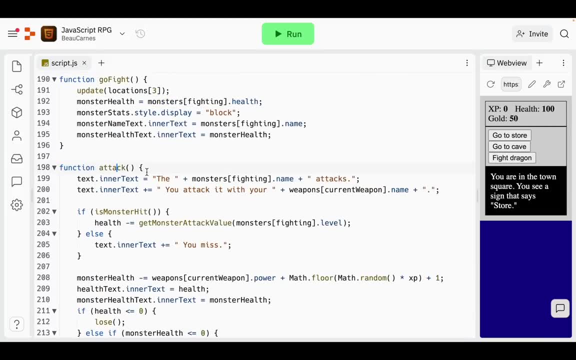 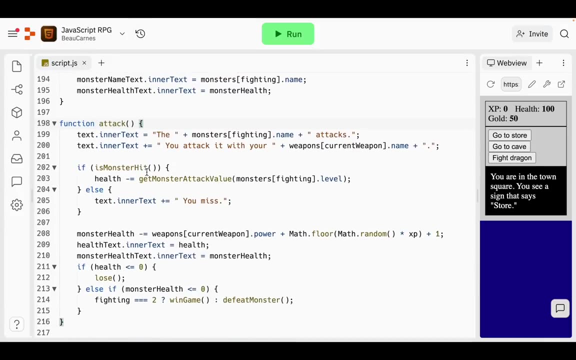 is false, then returns false, but we're going to go back to the or the or operator. Okay, now let's add another thing. So for the attack, we're going to make it so on every attack there's a small chance that the player's weapon breaks. So at the end of the attack function. 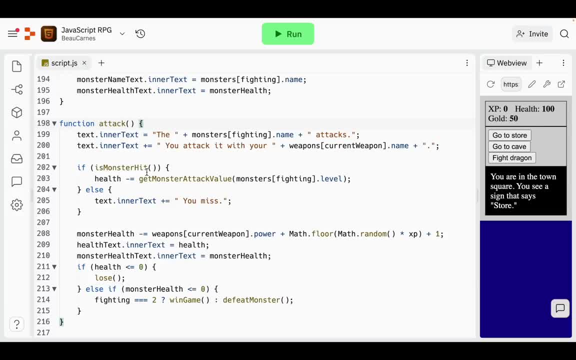 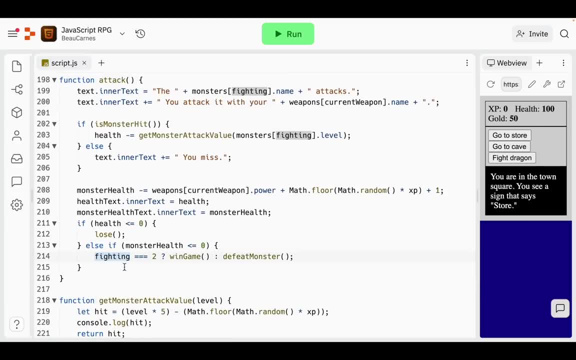 we're going to add an if expression with the condition math that random is greater than or equal to point one. So let's go here. Okay, now we'll use the plus equal operator to add your, and then it's going to say the: 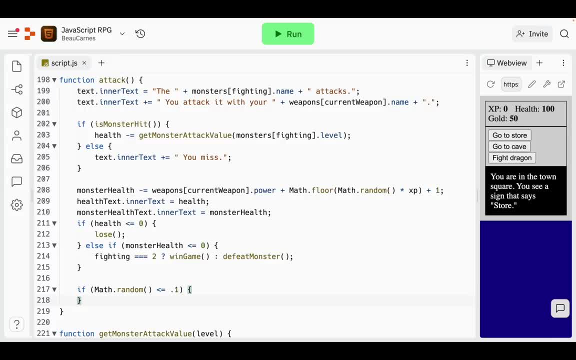 first item in inventory array. your weapon breaks And it's going to add that to the end of internet text And we can use inventory dot hop to both remove the last element from the array and return the element. Let me show you what I mean, So right in here. 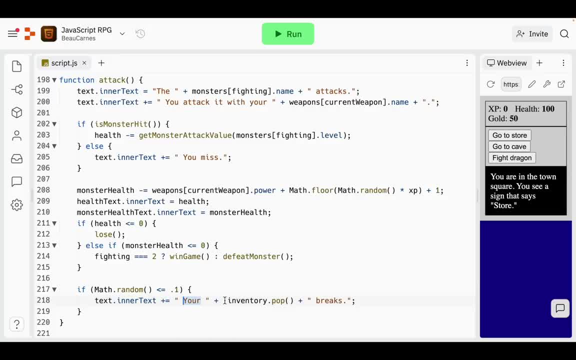 text. enter text plus equals your and, or using a string concatenation with the plus your. And now we do inventory dot pop. this is both going to remove an item, remove the final item in the array and return it. So it appears in the string here breaks, So it's not going. 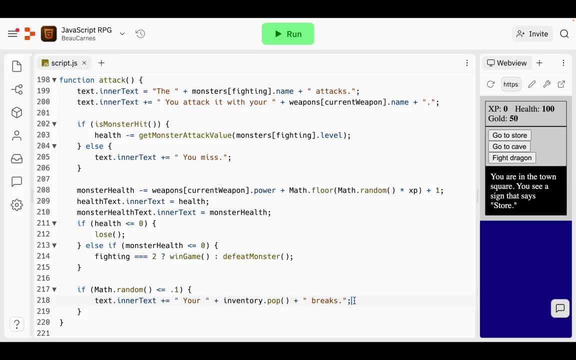 to be in the inventory anymore And we get to see what the item is. And now we can next decrement the value of current weapon. So we'll just do that with current weapon minus minus. But we never want the player's only weapon to break. So So well, let's use the logical and operator which I was. 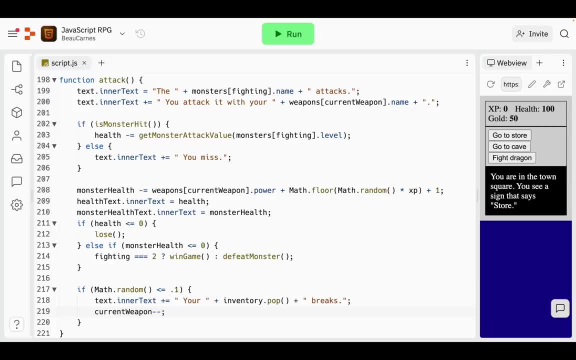 talking about earlier, to add a second condition to the if expression we just wrote: if a player's weapon, a player's weapon, should only be able to break if inventory, that length does not equal one, So you can do. does not equal with an, with an exclamation point before the double equal sign. So 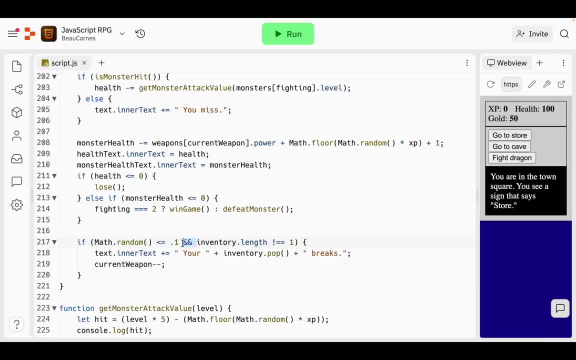 so let's see that. So we're using the and ampersand ampersand for and, and then this is the does not equal. so there's two conditions. both conditions have to be true math, that random is to be less than or. 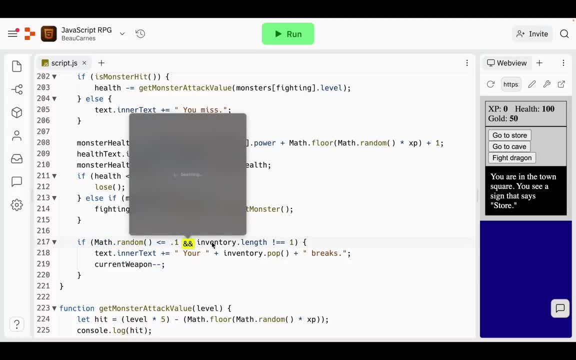 equal to point one, And also the inventory. that length should not equal one. So for not equal you can either: this is the not equal, that's equivalent to three equal signs. And this is the equal, that's equivalent to two equal signs. It's for the most part you should use the one that's. 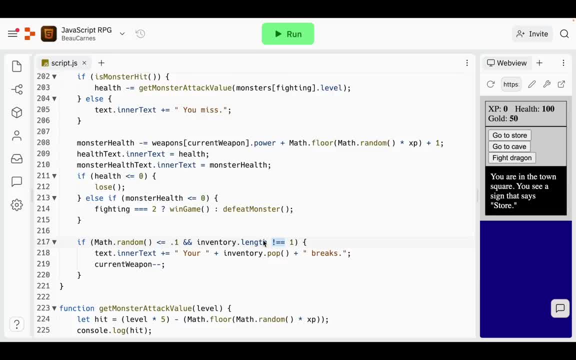 equivalent to the three equal signs. So we're checking for both, though it can't just be one or the other. both have to be true for the inventory item to break. Let's do a quick test and see if we can get our, our inventory, our item to break. So if I just go to K, I'm just going to. 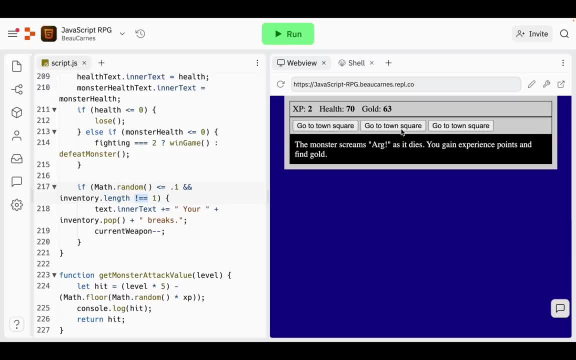 keep fighting the slime Until we hopefully. well, actually we have to buy. first we have to buy, go to the store- I forgot where to buy the weapon- And then we can see if we can get it, that the break. So go to the cave It. we may have to do it quite a few times to get the break, Your dagger. 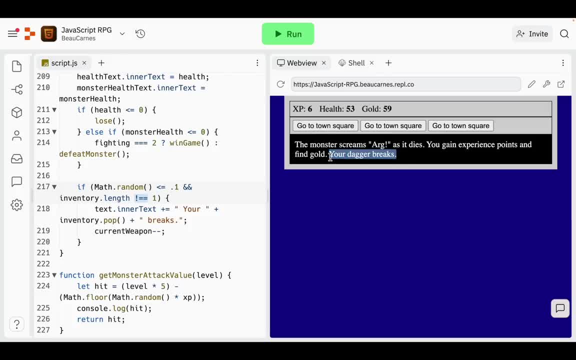 breaks. it happened Well. so what? we kind of got lucky where I guess unlucky to get to break. So so our dagger breaks, and now we only have a knife Or a stick or whatever the first one was. So so that's actually working correctly, So everything's. 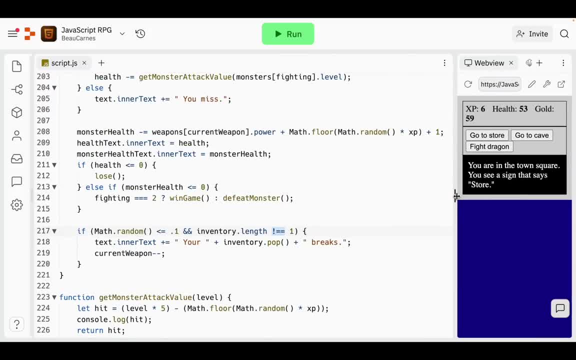 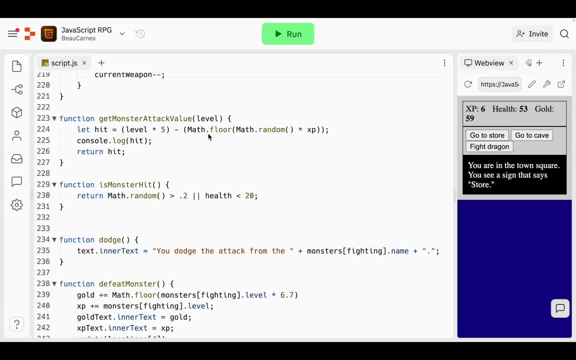 working basically how we want. There's just one more thing to do, which is to add a mini game- Easter egg, basically a hidden feature of the game, And really this is just a reason to be able to teach you one last part of JavaScript. So at the end we'll add another function called Easter egg. 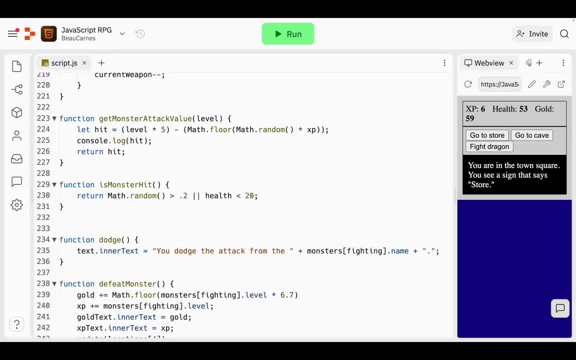 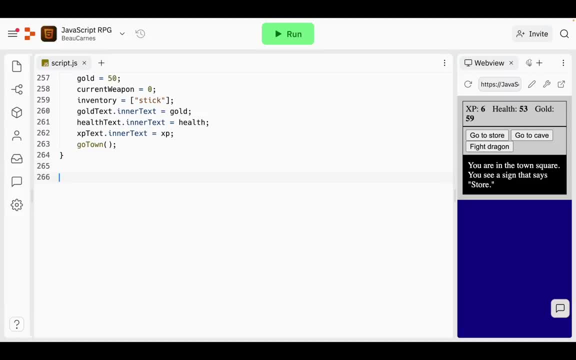 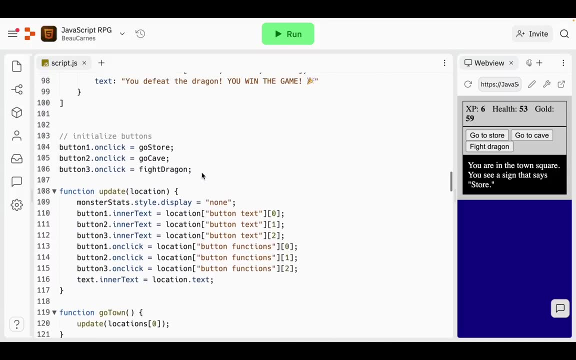 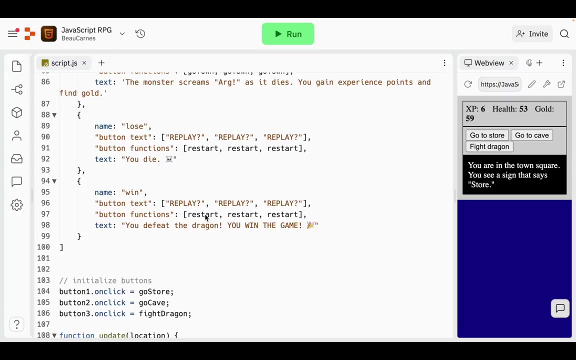 and it's going to call the update function and passes in locations seven. So we'll add that the very end, Easter egg, location seven, And then we're going to have to add the new location for the Easter egg. it's going to have a name of Easter egg And the button text is going to be to eight or go to town. 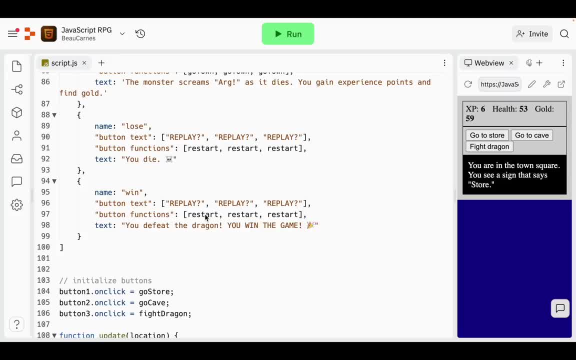 square And the functions are gonna be picked to pick eight or go to town. And then the text is going to be: you find a secret game, pick a number above 10. numbers will be randomly chosen between zero and 10.. If the number you choose matches one of the random numbers, you win. 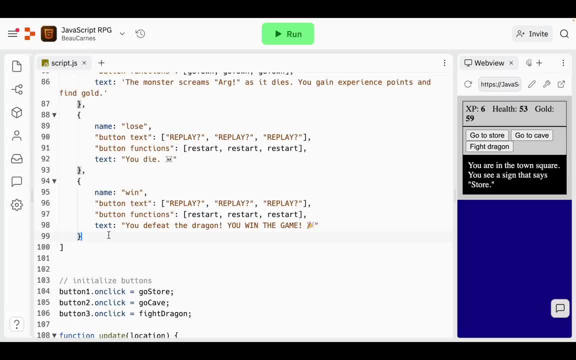 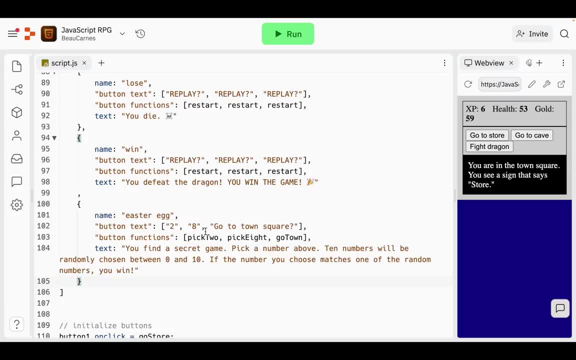 So we'll just add that and you can see that text here. basically, you can only choose two or eight for for the numbers, So now we just have to add the code that's going to randomly choose these numbers between zero and 10.. But why? we can do that. anyway, we can change it a little bit bigger. here you can change the text, here we can change it to whatever you want it to be. So that's what it does. So now we just search for It works fine. I can also edit it. It really works fine. So we're going to go back and try to boot this. 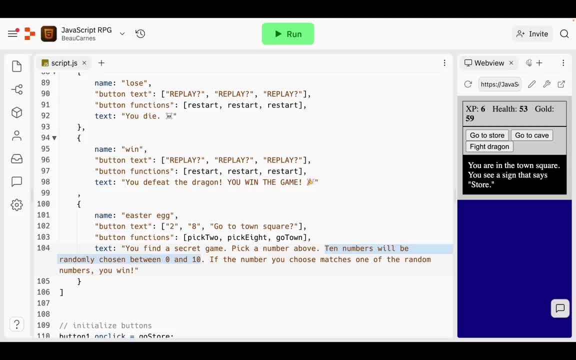 So we're gonna do just some editing stuff now and, kisses, Remember to type any sticker on this statement. first, let's create the, the pick two and pick eight functions, And each function is going to call the pick function, which we sought to create, and pass either a two or an eight into the pick. 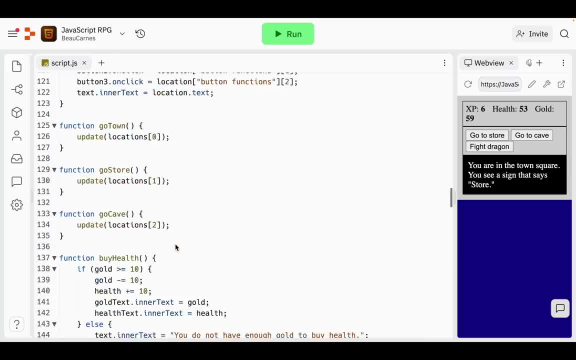 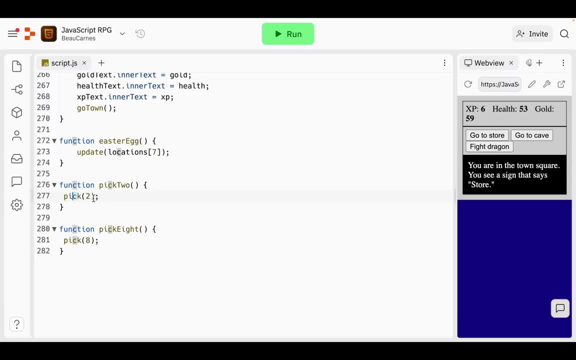 function depending on the function name. So let's go down and add those functions- pick two was going to pick two, or pick a is going to pick eight, And then the final thing is to create the pick function. So let's create that function. So function pick and obviously it's going to need. 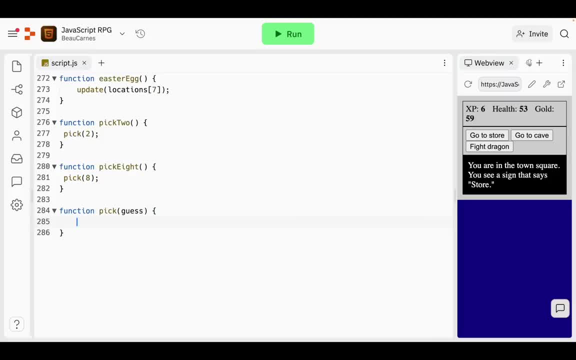 a guess. And then what's going to happen in this function? Well, first let's create a new variable called numbers, and it's going to be an empty array, So let numbers and it's going to equal this empty array, And we're going to push numbers onto this array using a while. 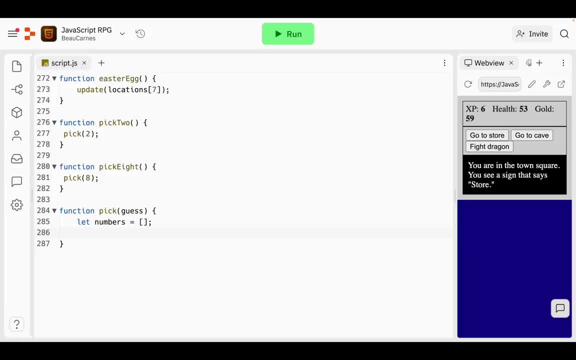 loop. So we're going to talk about two different types of loops in this section. The first is a while loop and a while loop. we'll keep doing something while a condition is true. So a while loop, it start. it starts off looking kind of like an if statement. So we're going to do while and. 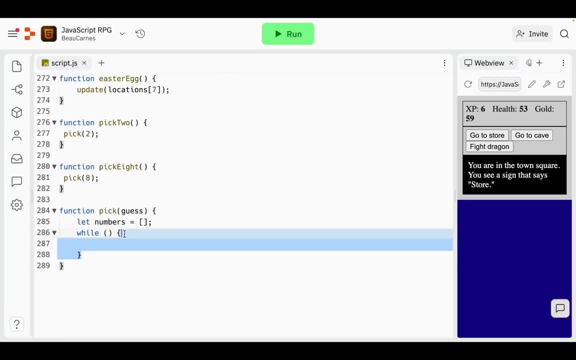 there's gonna be a condition. we'll fill that in a second And there's gonna be some code in between these curly braces. So the condition we want to put in is: while numbers dot length is less than 10.. So numbers- dot length is less than 10.. So it's gonna. it's the right now the length is zero. 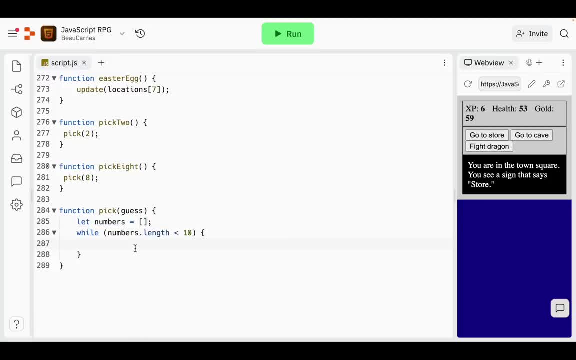 So while it's less than 10, that's going to do something. So we want to push an item onto this array, So we'll do numbers dot push, So numbers dot push, And then we're going to put what item we want to put on, And here we're going to create a random number between one and 11.. 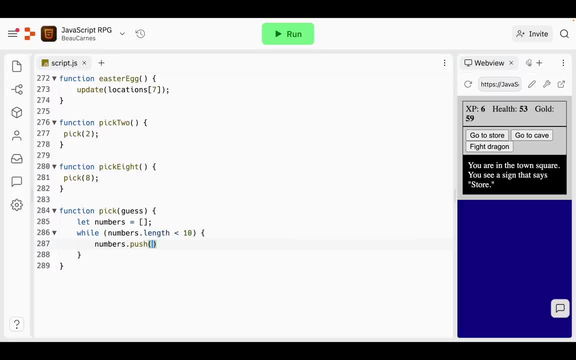 Or one and 10.. So to create a number, lan number, there's a, basically a formula. we've already kind of discussed, we've already discussed the formula. But we're going to do math, dot random, to get a random number between zero and one and we multiply it by 11.. So now, if we just round this, 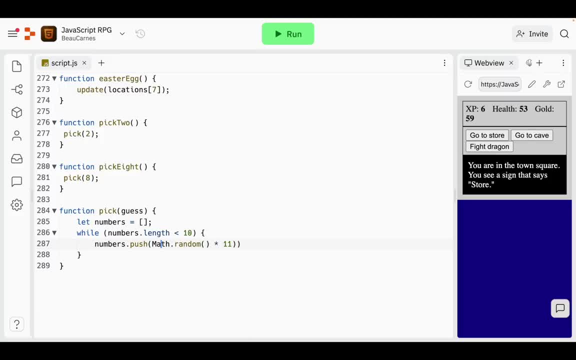 down because it's going to. it's going to have a decimal, so we'll do math: dot floor. This will give us a random number between one intended to put onto the numbers list. So there's definitely different ways we could have created this list, But I wanted to demonstrate how to use a while loop. So while this condition, 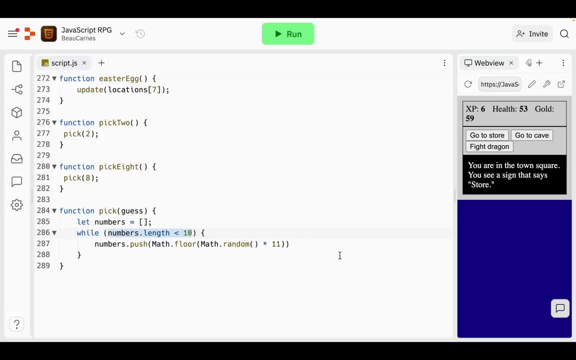 is true while there's less than 10 numbers, we will run this code And then, after this code pushes the 10th number onto the list, the 10th random number, it will go back to the condition again and it won't be true anymore. So we'll pop out of the while loop and go to the next line of 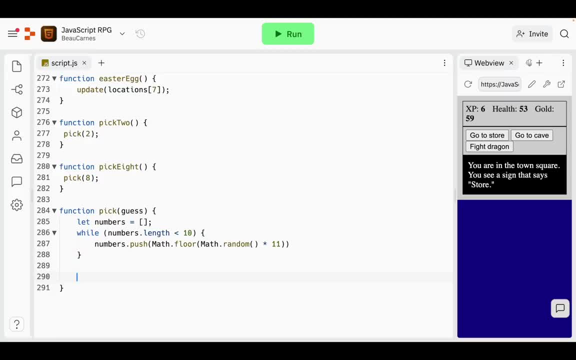 code And the next line of code is: we are going to display using the text that enter text. we're going to set to equal you picked and then put what they picked. Here are the random numbers. One thing I just added to the end of this is an escape character. So with this x, slash in. 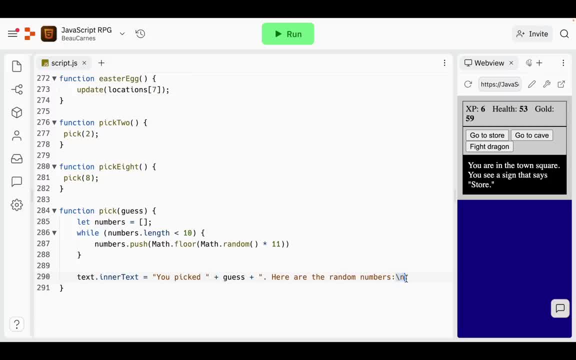 that's the. that's the how you say new line. So if you want to add a new line right in the string, you can use the, the escape character, the backslash in, and we'll. we'll add a new line to the into the string. 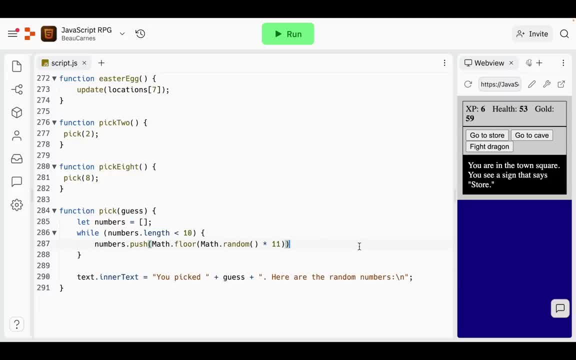 And let me just add a few semicolons here. Okay, now we're going to talk about a new type of loop called a for loop. Again, it's going to be set up just like the while loop at first, So we're. 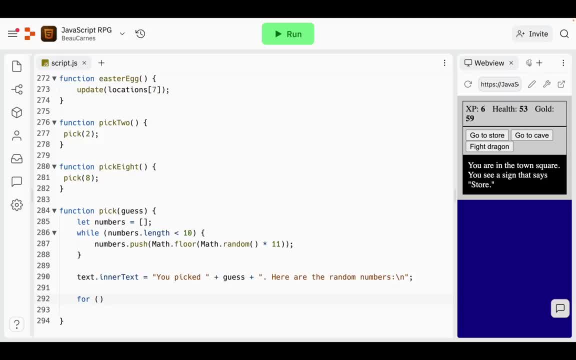 going to have the, for that's the key word. there's going to be parentheses, and then we're going to have the brackets or the curly braces. So we're going to run this code in here based on what's in these parentheses. So there's going to be three items in these parentheses, each separate with. 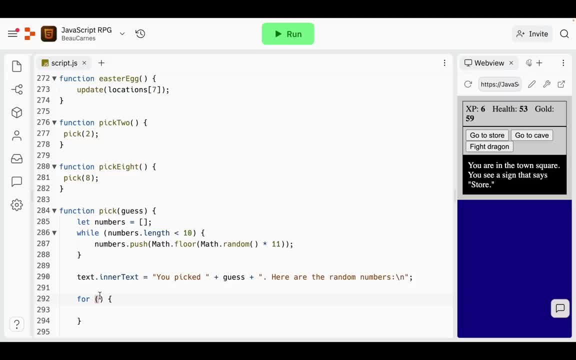 a semicolon. So first we're going to initialize a variable. So first we're going to initialize a variable, then we're going to put the condition that we're looking for for the variable to have before we, before we're done with the for loop, And then we are going to be able to change the. 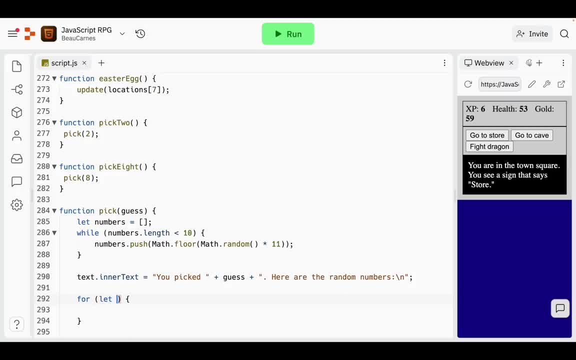 variable. We're going to have a variable for the for loop And then we're going to be able to change. So let me show you what I mean We'll do. let i equal zero semicolon. i less than 10, semicolon. 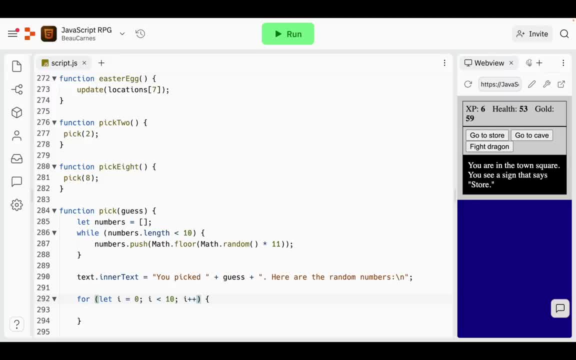 i plus, plus, So let's go over this. So first, when this, when we go into this for loop, we're creating a new variable just for the for loop. So as we use let, it's only going to apply in this block of code And we are going to loop until i is less than 10.. So once i is, i is less. 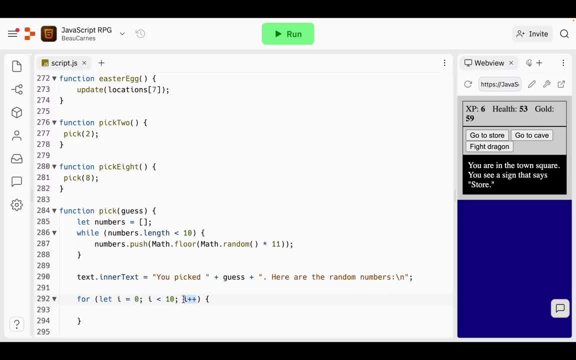 than 10, we'll be out of the loop, And this is something that's going to run at the end of each iteration of the loop. I plus plus. that just means i equals i plus one. So I start at zero and then every at the end of each iteration of the loop is going to go up one, And once I is. 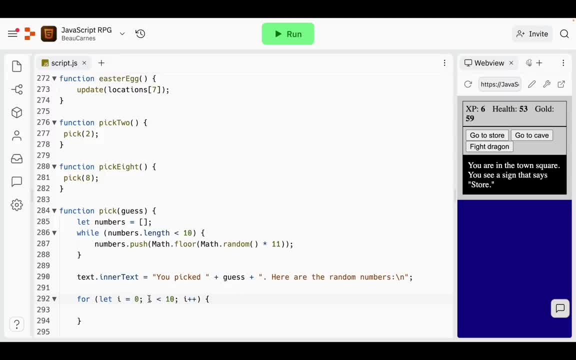 and it's actually basically it's. it's a while while lie why i is less than 10, it's going to keep looping. So while i is less than 10, it's going to keep looping, And once I is no longer less than 10, the loop will be over. we are just going to use this loop to add a, to add all the. 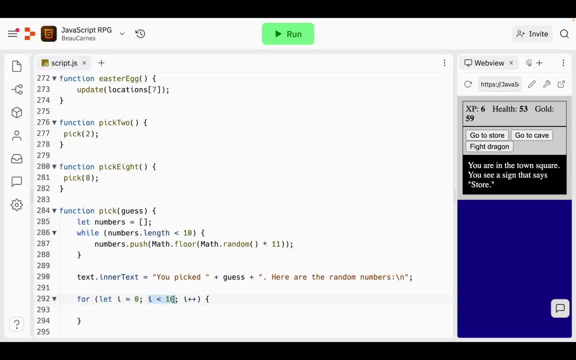 numbers from our list And it will put a new line character after each number on the list. So just like that. So do plus equal numbers And so when we do numbers, I so first it's going to be So I is going to be updated each time we go through this loop. So the first time we go through, 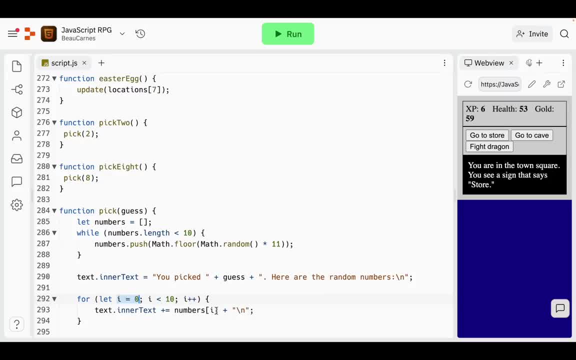 the loop, I is going to equal zero, So this is going to be the number. This is number here at index zero, which is the first index. Now it's going to go through the next index And for this number, And then I will be updated And then it'll be index one, index two, index three. 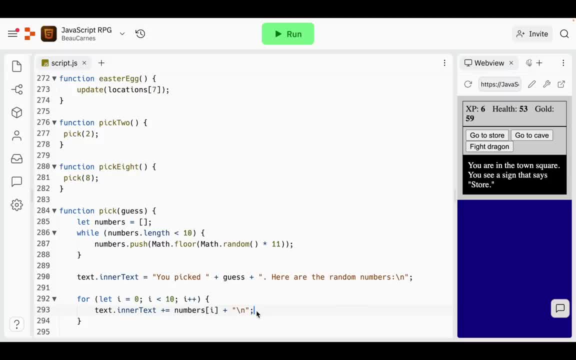 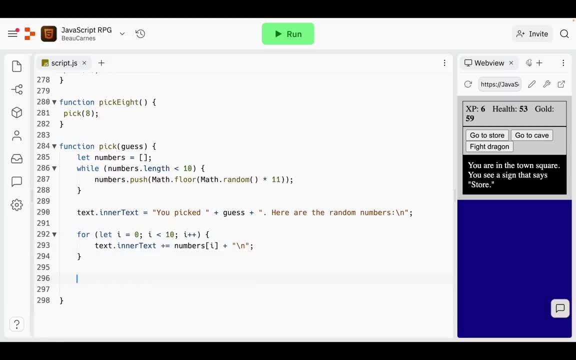 until the loop is over with, And after each number we will put a new line. Okay, so now we have our final section. we're going to put an if else statement. we want to figure out if the number that was picked is in this list. Well, there, there's a kind of a fancy way we can do. 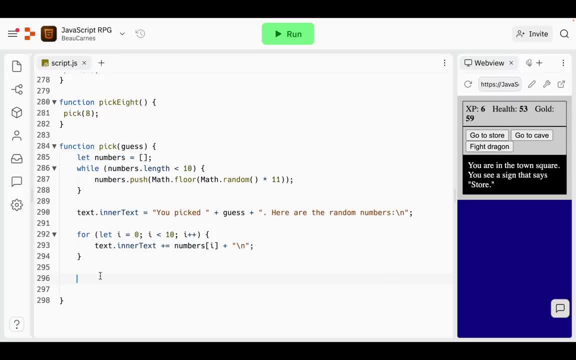 that. So first let's create the if statement. So, if so, we're going to put the condition here, we're going to find the index of the guest number, So we can do numbers dot, index of and we can pass in the guests. So in this case it's going to either be two or eight. 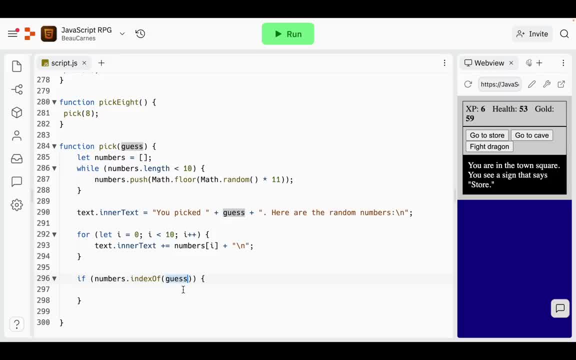 but we can use this function for any, for a guess of any type of number. So we're trying to find the index of it, of it, we're looking for that number in the numbers array And we're trying to find the index. So the you know the index starts with 01234.. So which part? 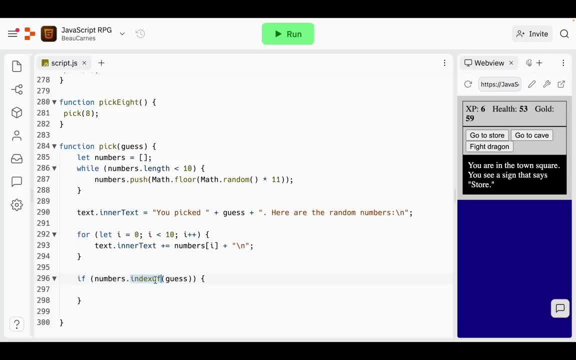 of the array. which order in the array is that number? but if the number? so this is always going to return a number. but if the number, if- is not in the array, if it cannot find the index of that guess, it's going to return negative one. So we can use that. So if the index of guests does not, 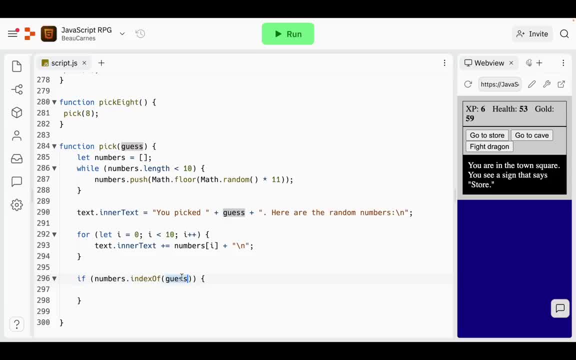 equal negative one. that means it's in the list, that means you guessed a correct number. So we're going to do the does not equal and then put negative one. So in that case we are going to set inner text to write: you win 20 gold, we're going to add 20 gold and we're going to update. 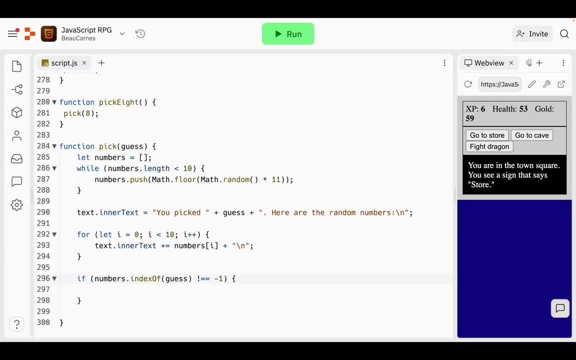 the inner text. So we're going to add 20 gold. we're going to add 20 gold and we're going to add the text of the gold. Just like that, plus equal right, you 120 gold. we're going to add to. 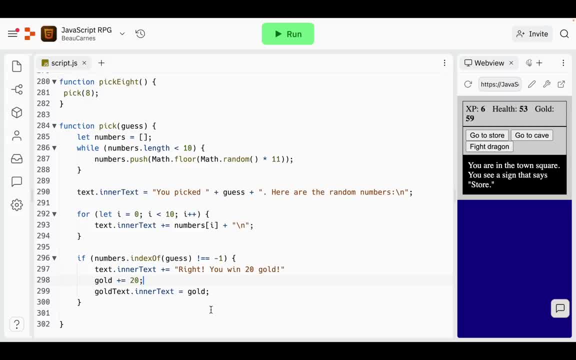 the gold and then update the inner text of the gold, Else it's going to say wrong, you lose 10 health. we're gonna subtract 10 health And we are going to set the inner text of the health So it's. 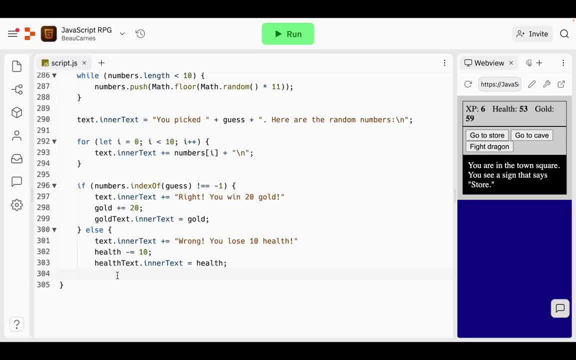 going to look just like that. Let's put the other curly brace here, And anytime you subtract health, we have to check if the player has lost. So that's what we'll do now: See if you can figure out what code you should. 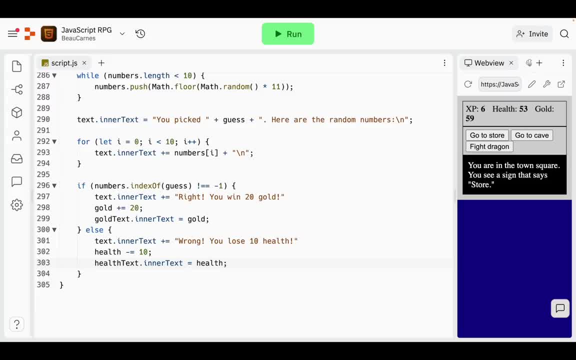 add to if the player has died. That's gonna be just like this: If health is less than or equal to, zero, lose. Okay, we are done. The only other thing we need to do is make it so you can get into this. 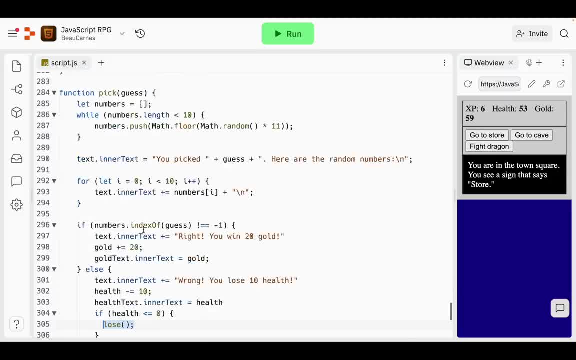 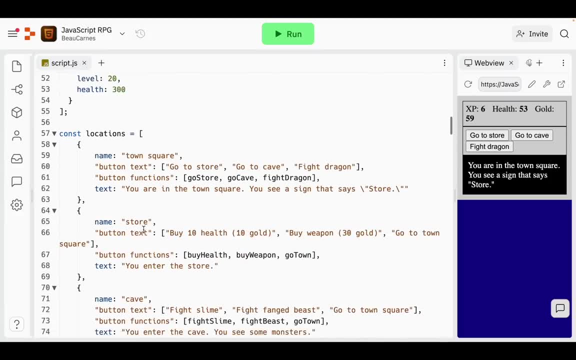 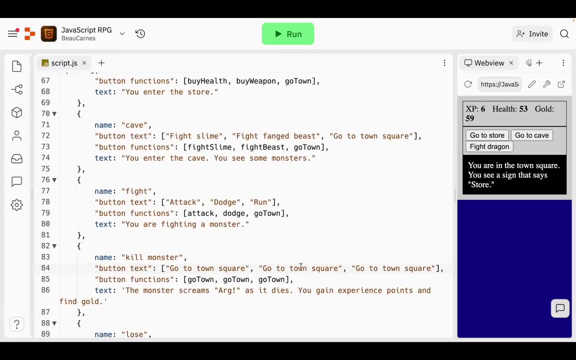 Easter egg. So how we're going to make it so you can get into the Easter egg is we're going to go back up to the locations And during the kill monster, once you've killed the monster, it's gonna say: go to town square, go down square, go to town square. But we're not going to use the same. 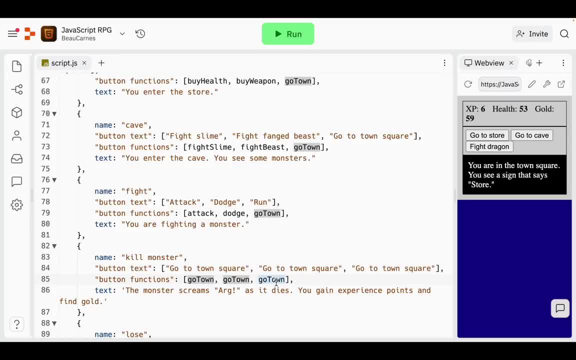 functions for each of these. the final function we're going to do Easter egg. So even though it says go to town square, it's going to say go to town square, go to town square, go to town square. if you know the Easter egg, you're going to go to the Easter egg function, Okay. so now there's 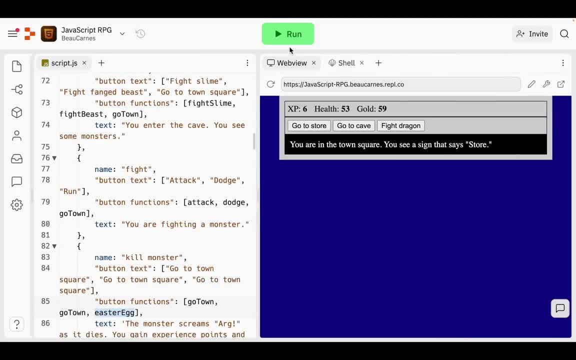 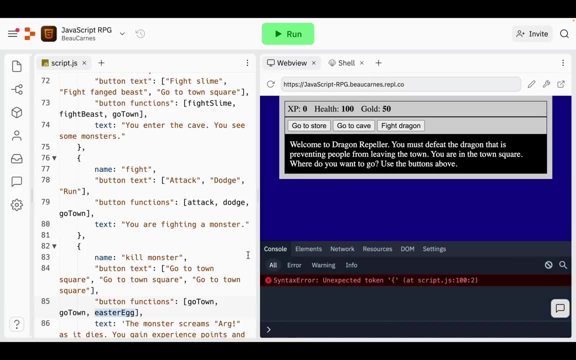 nothing else to add. So let's just try out the Easter egg. I'm gonna go to run And we know that if we go to the cave, we know. Okay, now let's just check out. Oh yeah, we got obviously there's. 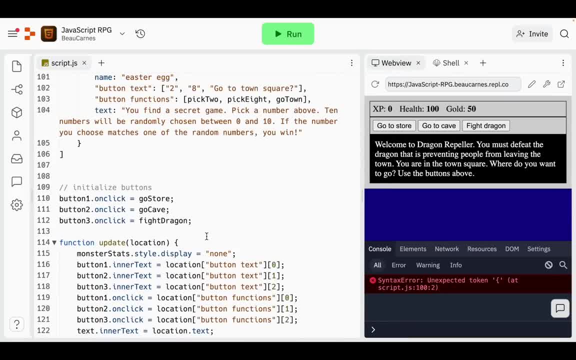 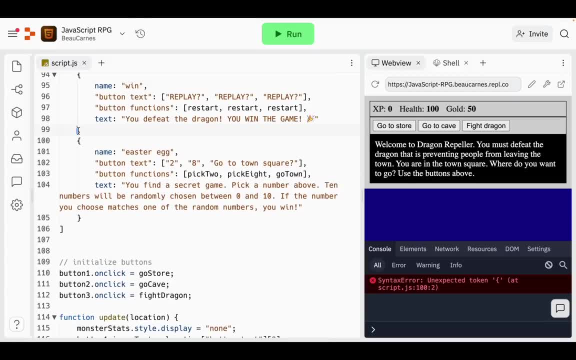 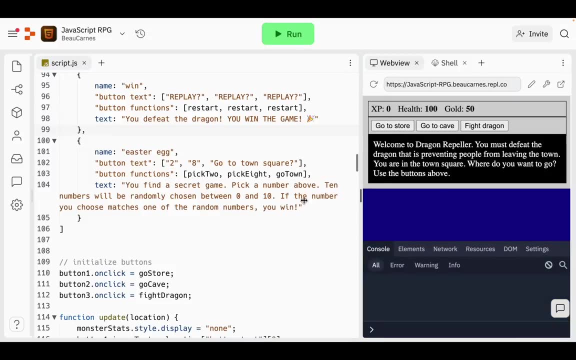 some sort of error we have to fix here. So let's go to line 100.. And oh, when we add- when I add- Easter egg, I somehow deleted that curly brace. Okay, so now I'm going to. first I'll just go to the store by weapon, Now I'm gonna go to the cave fight the. 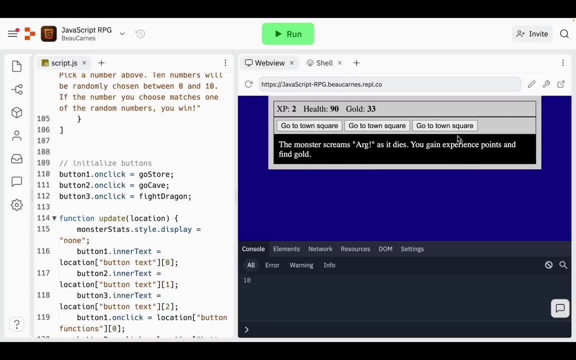 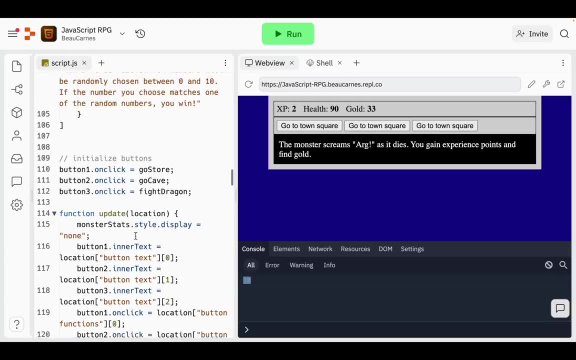 slime attack. Okay, now I'm going to click the third: go to town square. Oh yeah, And while we're doing that, you can see in the console it's putting the 10 here, Because, if you remember, we did do that in the last video, we did that in the last video, we did that in the last video. 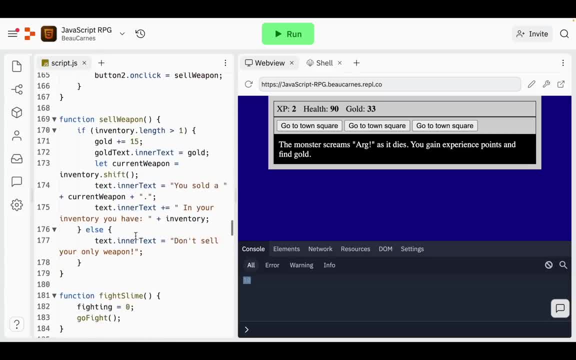 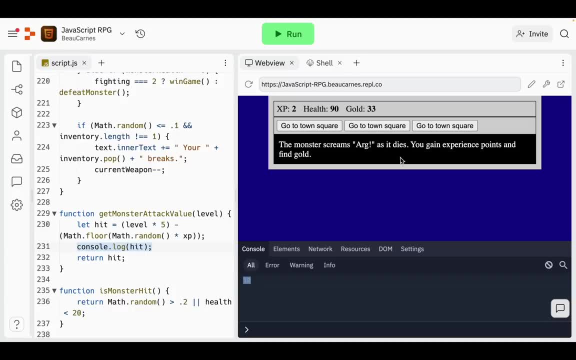 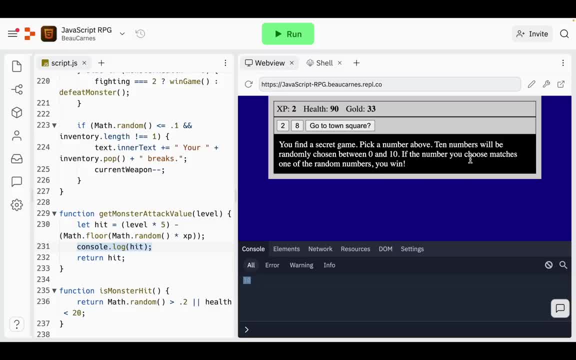 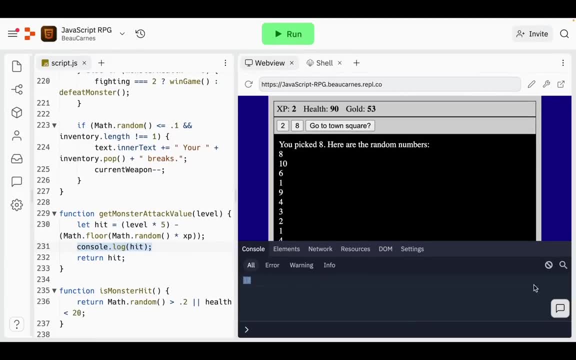 above 10.. Our numbers: we randomly chosen between zero and 10.. And then, if you choose them, if the number you choose matches one of the random numbers, you win. So I can click eight. you picked eight here, the random numbers. Let me just turn off this console. right? you win 20 gold because 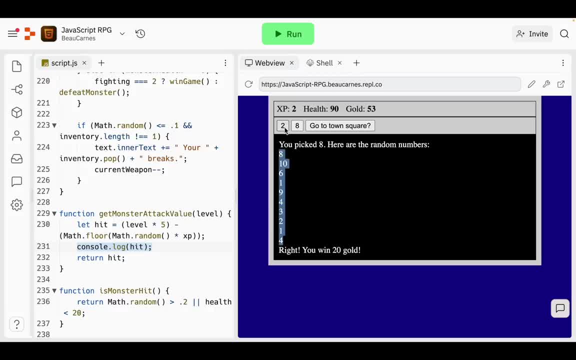 eight was in there, And then if I choose the wrong, because I can play again, so you pick two. right, I got right that time, right again. oh man, I'm on a roll here. Wrong, you lose 10 health. 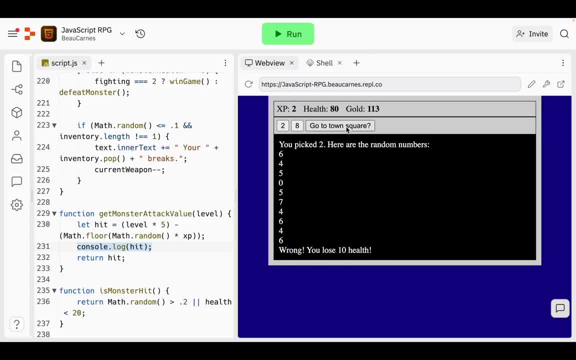 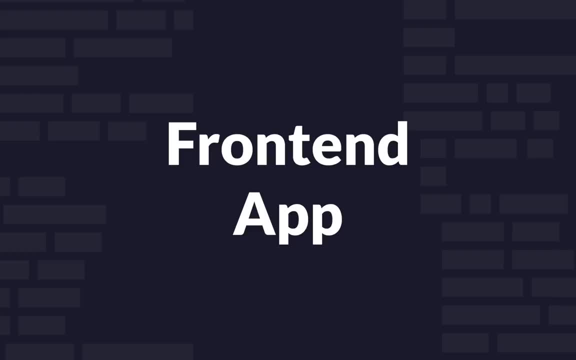 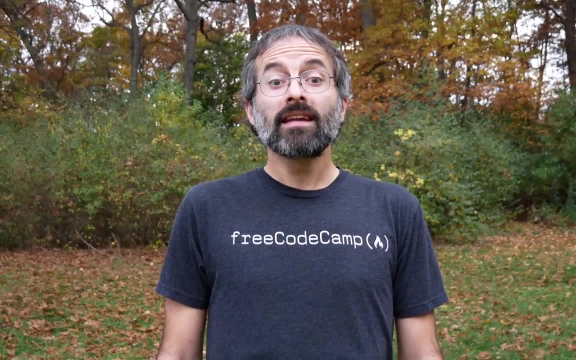 So I tried too many times. So now I can go to town square. The game is complete. Now that you know the basics of JavaScript, Tomi will take over again for this next section. He's going to teach you how to create a front end web app with HTML, CSS and JavaScript. 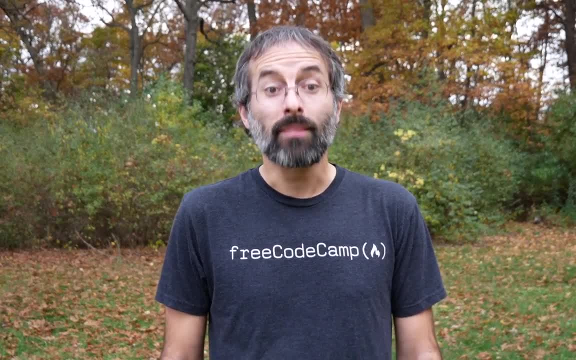 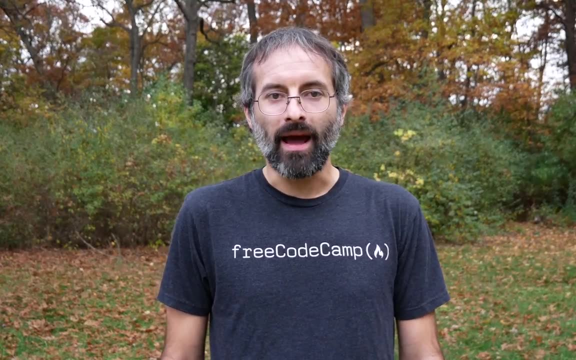 Afterwards, I'll teach you how to create a back end web API using NodeJS, Express and MongoDB. Then I'll teach you how to connect Tomi's front end web app to the back end web API. In this section of this course, we're going to be building this web application. 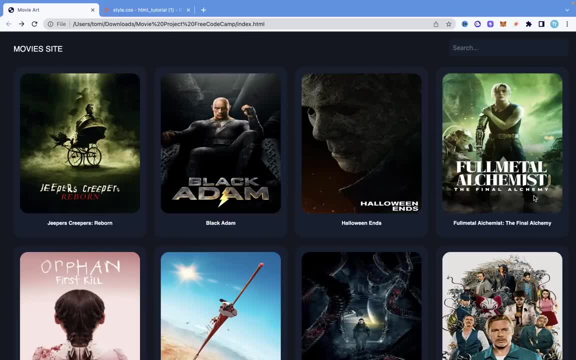 that you see right here. So it's going to be a very basic app And what is going to do is that you're going to be able to just allow a user to search for any movies and it's going to show a result of those movies, For 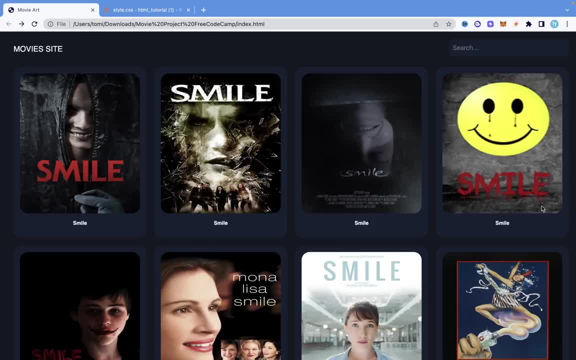 example, if I search for smile, you're going to see that I have results of the movie smile. So I'm going to show you how to build this from scratch. So we're going to design the HTML, the CSS. then, once we're done with that, we're going to use JavaScript to fetch this. 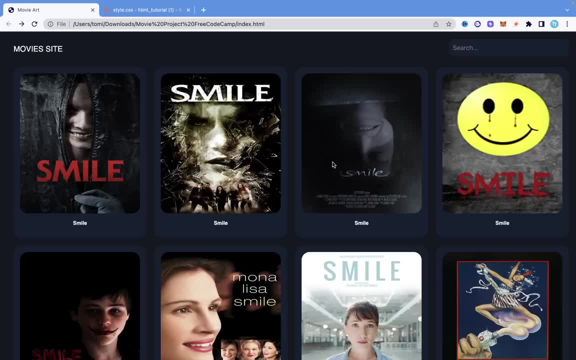 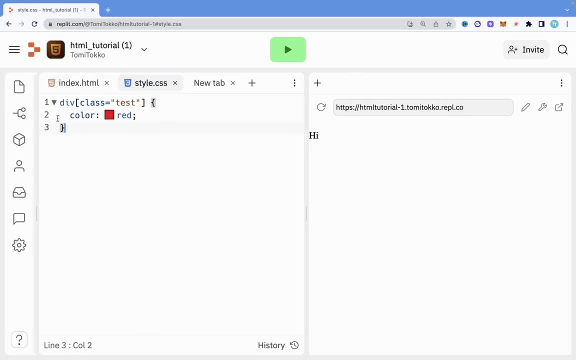 data from an API, So let's get straight into it. So I'm just going to close this tab And we're going to come back to replicate And let's just start with our index. So I'm going to close this And what I'm actually 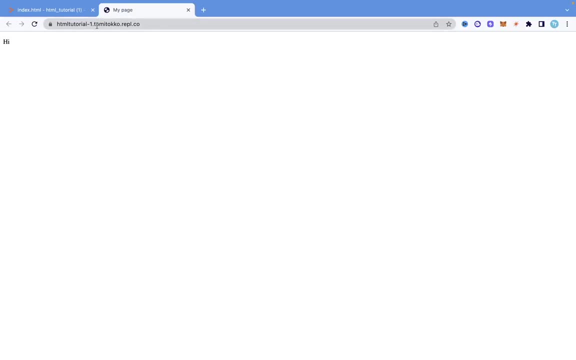 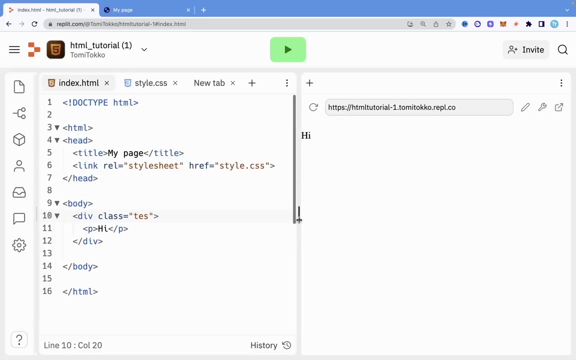 going to do is I'm going to open this on another tab so that we can just see how the application looks live, rather than having it like in a small frame. So that is also what you can do with replicate. So now I'm going to close that And we have all our you know code enough. 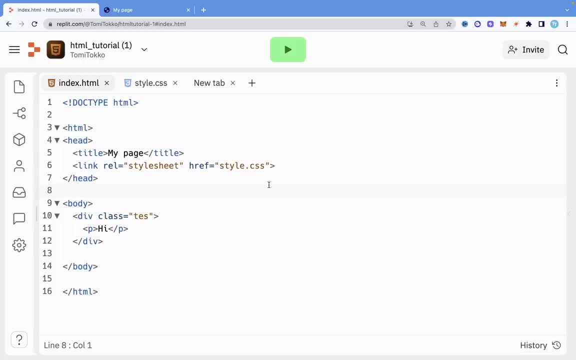 with enough screen for us to use. So what we're going to do: first of all, I'm going to actually just have all the, the HTML, you know, diff element, everything I'm going to use. then I'm going to start styling everything that we code in here And after styling it, 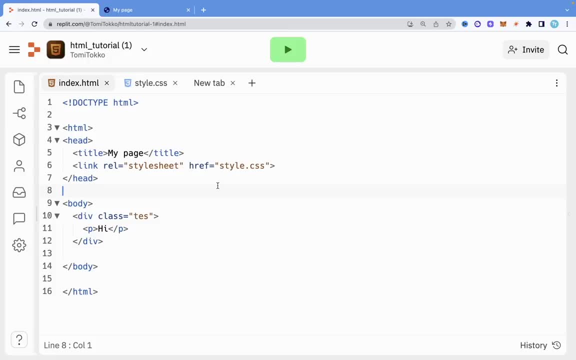 then I'm going to use JavaScript to you to fetch some data from an API. So I'm going to show you how to do all of this. If you don't know what these are, don't worry, I'm going to walk you through it. So the first thing I want to do is to actually just get 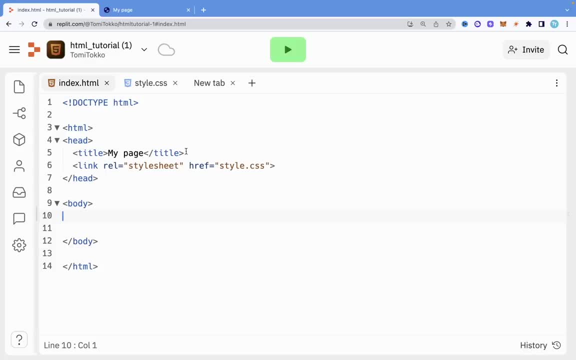 rid of all of this And right here, I'm just going to leave this title blank. So I'm going to give it the name I'm going to use, versus destruction And, trust me, I'm going to delete every text that we are going to use. Like we said, it stopped and stopped eliciting. 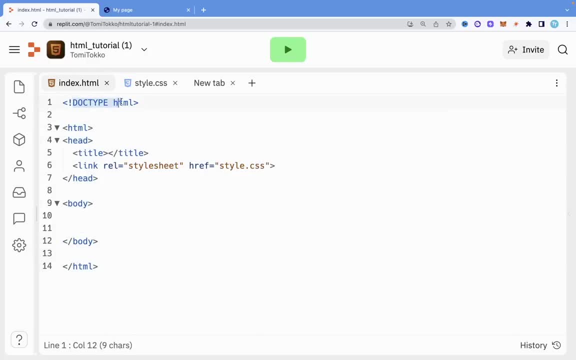 every text on it And, as you can see, you can see some of the notes in the class. however, you can see more details about what you must do. So that kind of mental evacuation competitor, For example in functional mode, like to smoking. 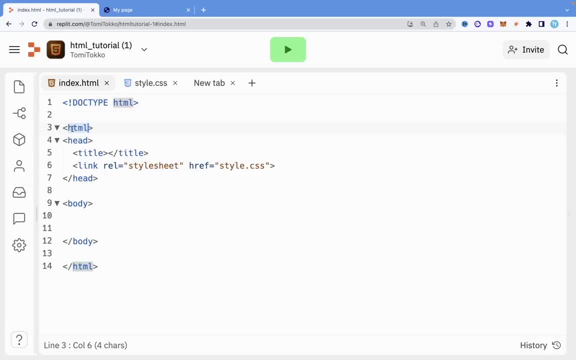 So we can actually see everything, So you can see that we don't have anything except like one box at the top. Okay, all this documentation, for example, as I said, I'm going toband them on image. So now we have seen. for example, I've already have the busk, The same. 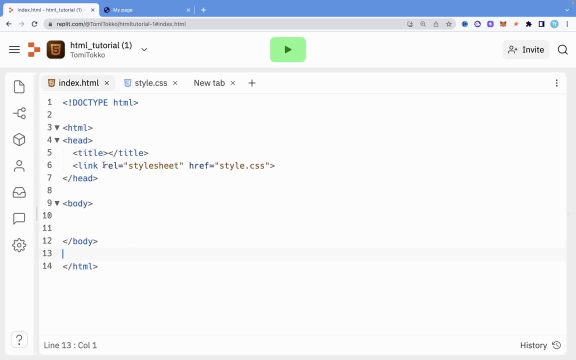 thing here Once again. we have here now we have a rules, properties and it can be edit the text. So the way there's a link in here right here. Then, after the edit, in the head we have the title and then the css that we're going to be using, which is this stylecss. 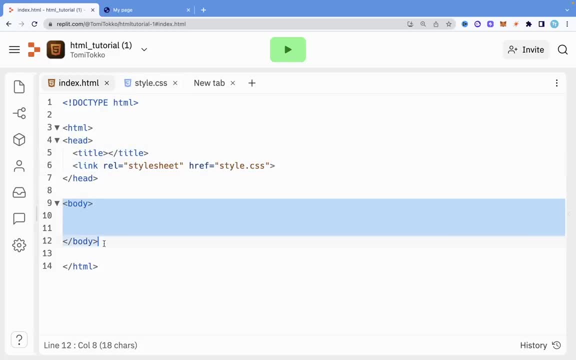 we have it linked right here, and then this body is where most of the visible stuff, or basically all of the visible stuff of the web page, is going to be. so let's get straight into this. so what i want to do now is i want to change this title to movie. 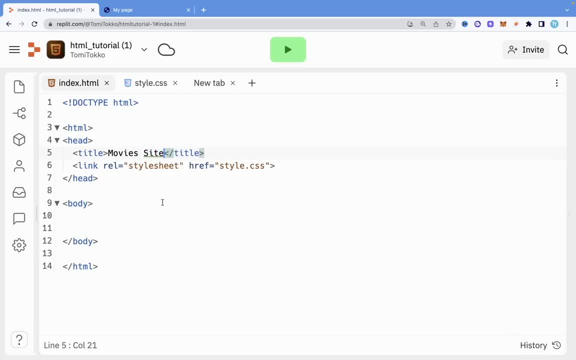 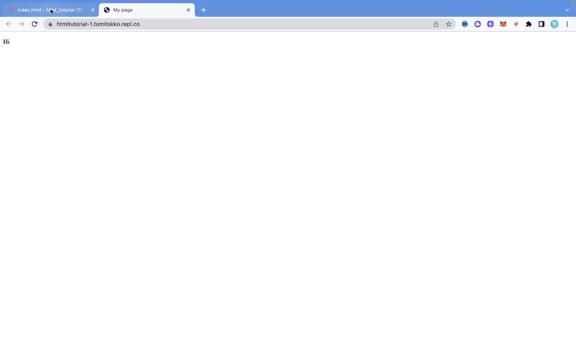 site. so once i change that to movie site, let's just come straight, and the first thing i want to create is like a very basic navbar right here. so, as you saw in the demo i showed you, there was a navbar that just shows movies and at this right corner there was like a search bar where a user 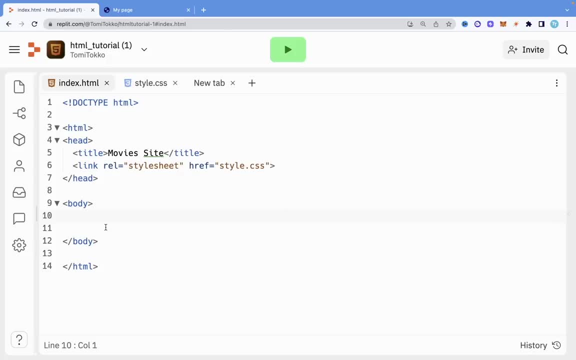 could search for something. so let's start with that. so the first thing i want to do, i'm going to create a new div element and that development i want to give it, let's say, a class of top nav. so i'm just going to give all of them different attributes, so i 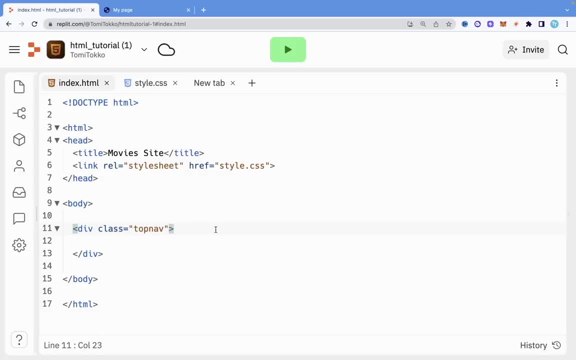 can just give them different attributes. so i can just give them different attributes, so i can use the attributes to actually style them later in the css. so now that i have that, the next thing i want to do is to just, let's say, have an, a tag, and this will just say movies site. so this movie site. 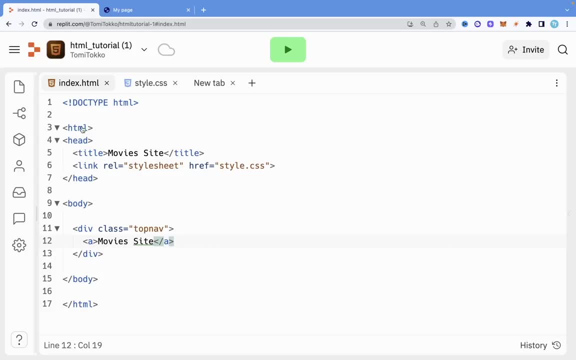 now is you know what is going to be shown right here, and let me say i'm going to give this a class also so we can style it. so let me just say this is active, and i'm going to say this is active and i'm going to say 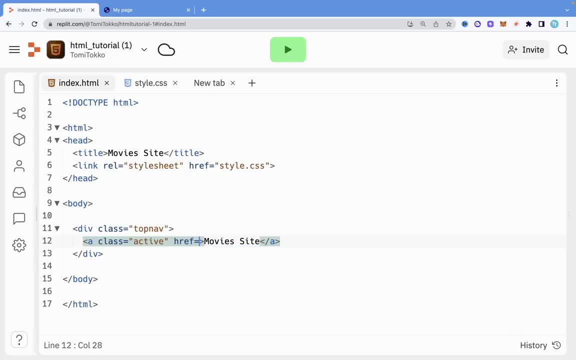 it should link to. we don't actually want it to link to anywhere, so i'm just going to give it this value hashtag, so it doesn't really go anywhere. so that is what we need to do for the movies heading. now. the next thing i want to do is to actually create another div tag in here, and i'm 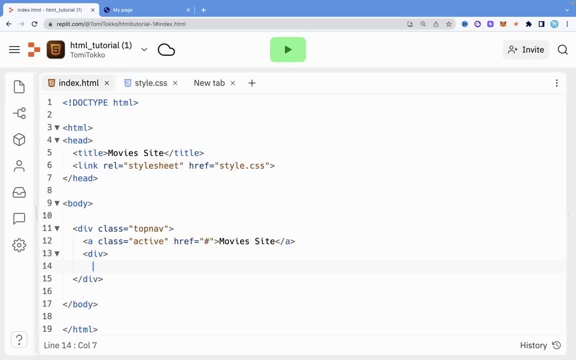 going to give this gift tag a class also, so this should also close. i'm going to close that div tag. so now that i've closed the gift tag, we just need to make sure everything is right and structured. so this is the div that is ending here. that's the a tie and this is a div tag. 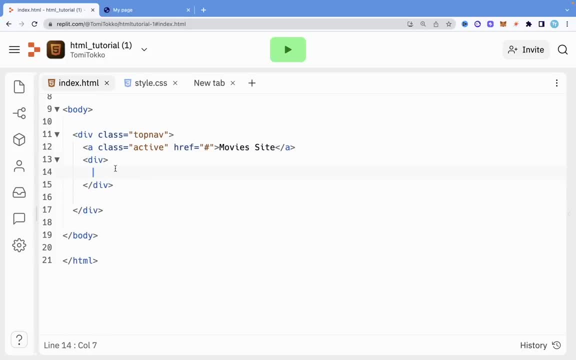 so in here, what i want to have is basically a form. so i'm going to have a simple form right here. i'm just going to say form. you're going to create that form for us. let me just bring this here now, before we have this form, let me give this div his own class so we can style every single thing if we. 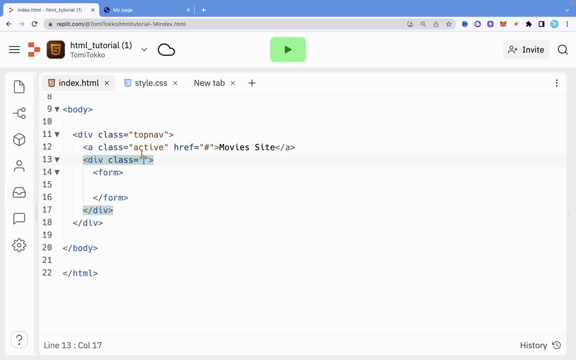 want to, and let me say this, because this form is going to contain this search bar, so let me- and this search bar is going to be part of this div class, so let me say it's like a search container, right? and then this form: i want to give it, let's say, a role. 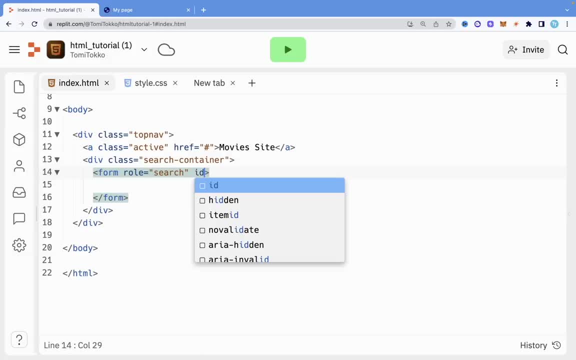 of search and i'm going to give it his own id now. i'm going to use this id later in the javascript also, so i need to name it: form now. it's just going to have one input and the input is going to close that input and the type. 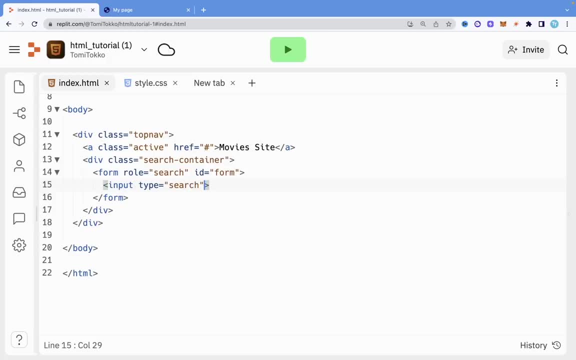 is going to be search. there's actually a type that is search, and when i say id, let me just give it, let's see, let's say query, and we can give it a name of just q and let's give it a placeholder and let's just say search. now, this is what we've done till this point. let's actually. 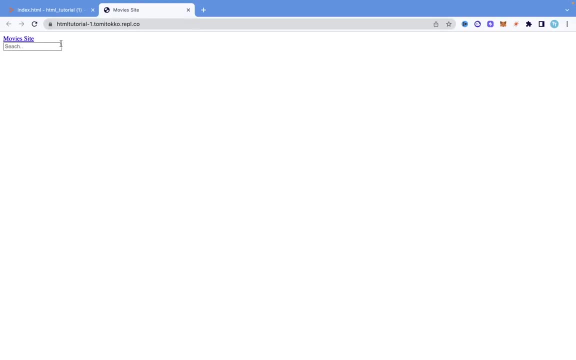 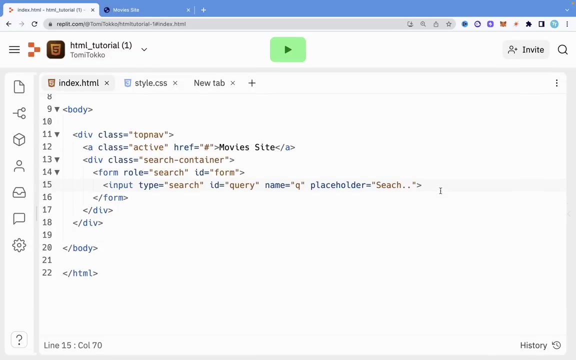 come here and see what that gives us. so if we refresh this, you can see that we just have this basic movie site and this search bar. now let's come back in here and what i can just do is let me change this to search. what i'm going to do now is after this div tag or this div class. 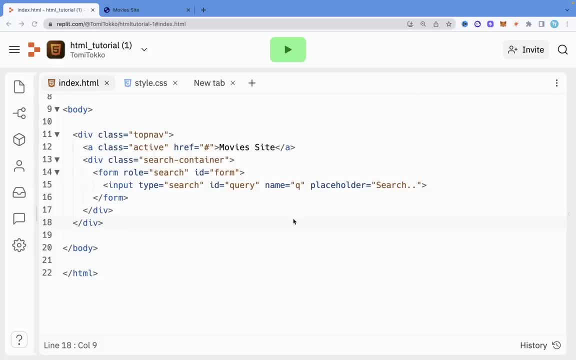 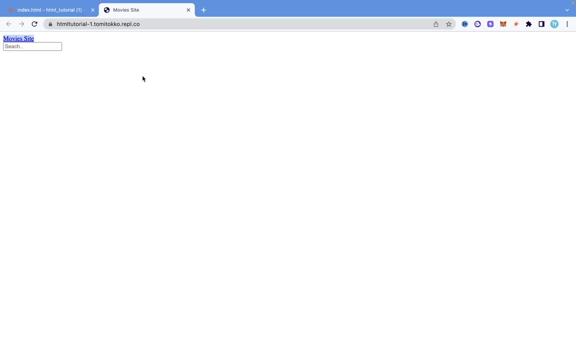 i just want to have another, you know, div element that is going to take care of the whole film. so you know, when we search movies in that site, when we search movies and we saw some like cards here that shows the image of the movie and the title. that's what i want to do right now, so i'm going 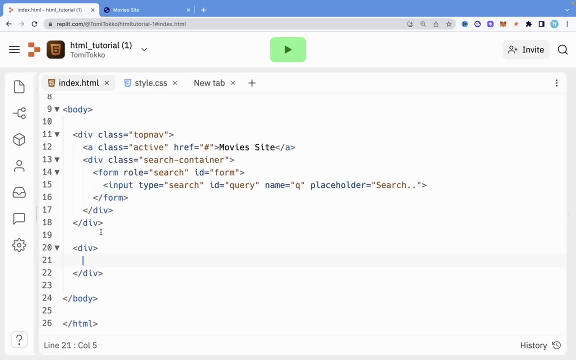 to have one div and i'm going to have this, have a class of row. it's going to be row and i'm going to, and i'm actually going to have another div in there. so now this is going to take care of the column class, so we're going to say class. 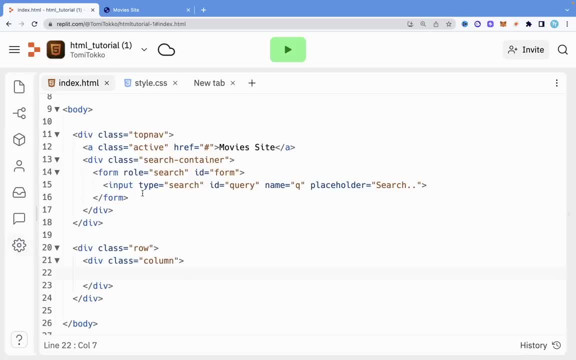 equals column. so just the way we have rows, because you know that we're going to have a row and we're going to have different columns, so we need to have that specified in the div type. and then let's create one more div tag and this one is going to have a class. 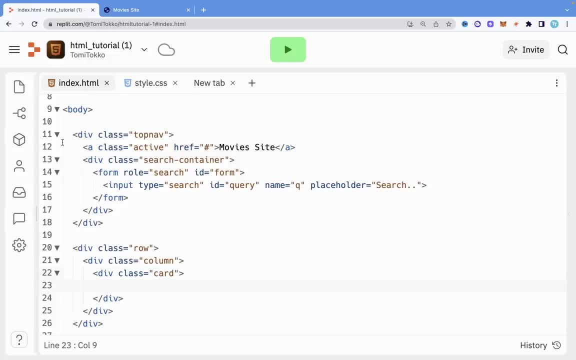 of card, because this is going to be the one that contains the actual, you know- details of that particular movie. so i want to have an image in here, and that image is, let's say, going to have a source. so for now, let's leave the source as hashtag. 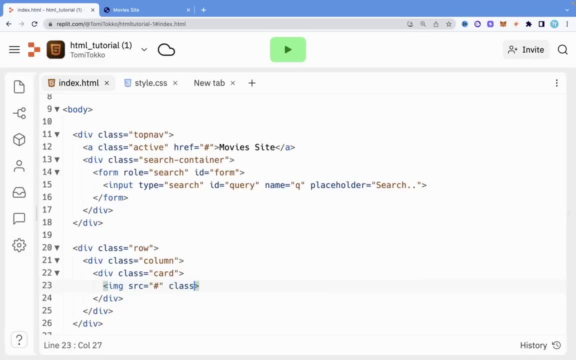 let's say, that's hashtag, but i want to have a class and i want to name this class thumbnail. so that's what i'm going to do to that, and what i want to do is i want to put this in an element named center. so once i say center, i'm going to put that in there. i'm going to show you why i did this. 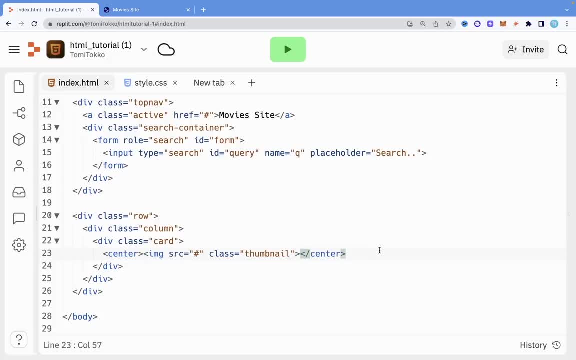 later, when we are styling it. now, we're also going to have: um, let's see, let's use an h3 tag to take care of the title of the image of the movie. so let's say movie title, right, and that is basically what we need for this part. so let's have 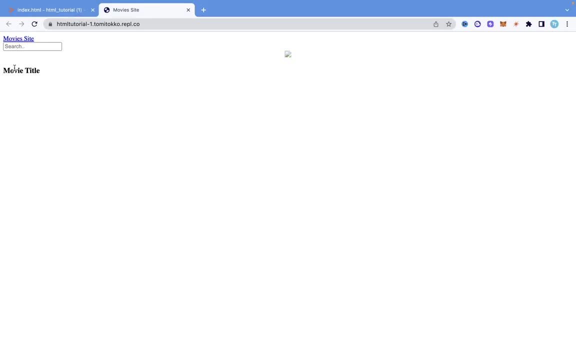 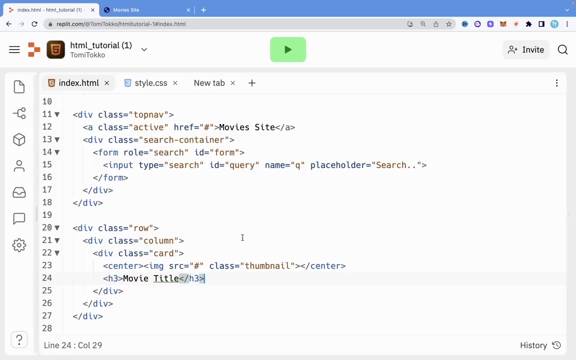 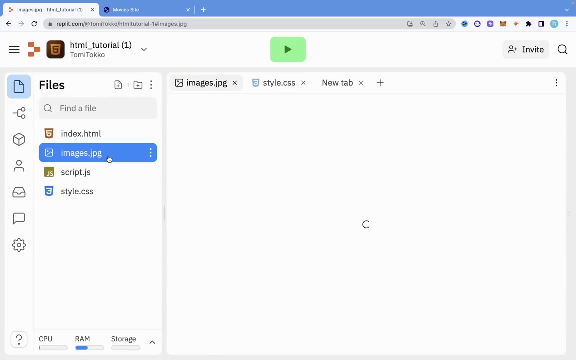 if i save this and you just come here and hit refresh, let's see. so this is the image, this is movie title. everything is all over the place for now, but don't worry about that, let's actually give you like an image. so if i open this up, i put this imagejpg there and if i click on it it just shows. 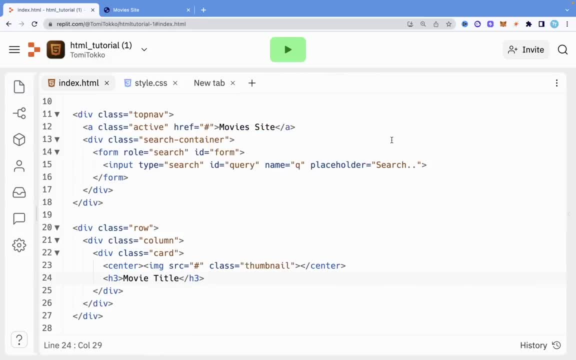 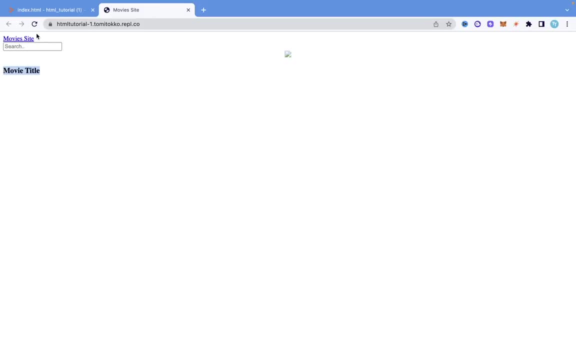 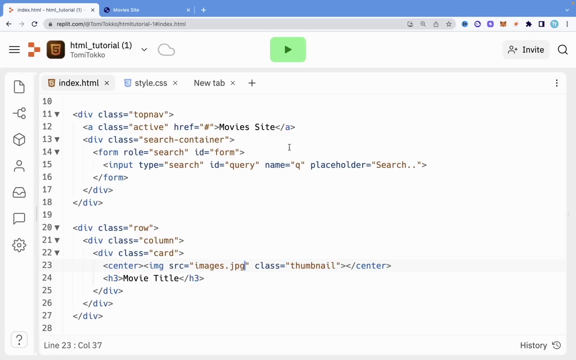 this wakanda forever image. so what i'm going to do is in here. let me just say images jpeg if i come down and hit refresh, so that should show basically right there. so we're going to style this later, but let's keep going. so what we cannot do now, since we have all of this, let's actually have a padding. 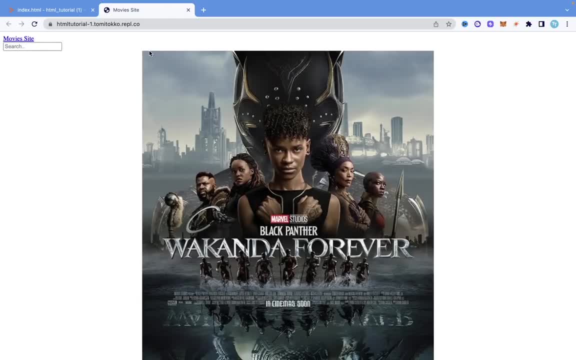 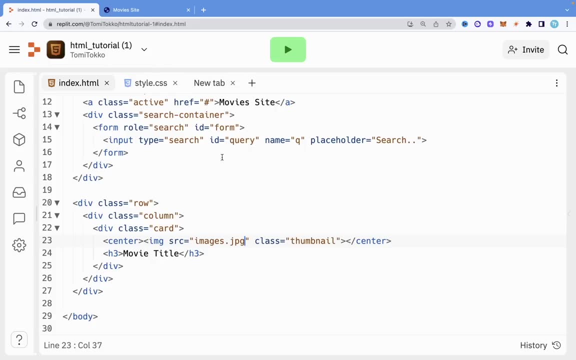 because, as you can see, just after that navbar there is like the. the movie card is right after it, so we'll have some spacing beside it, so we can just have like, let's see, we can start this in the css, but let's take care of it right now and we can say div right, and then 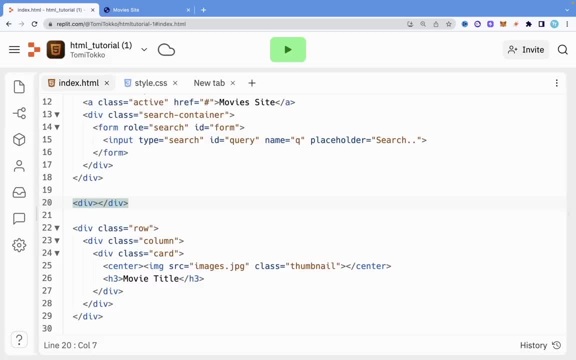 do is to say style, let's say padding. let's see, let's say left and give it 16 px, just so it has padding from the left and automatically- i'm going to explain something right now. so this basically has a padding on the left. so what we're going to do now is to 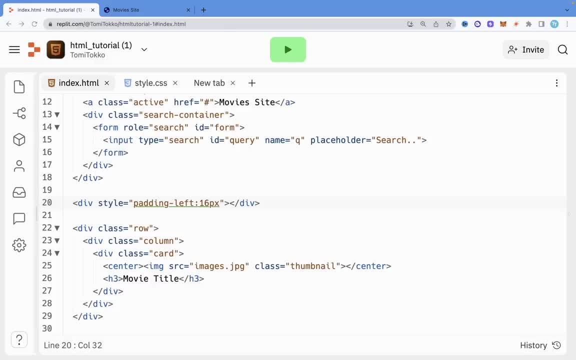 make sure everything is correlated. so we have that having a padding on the left, but we also wanted to have, like, some spacing on the top of it. so what we can just do, let's actually get rid of this, and this is just going to give you some padding on the left for you to. 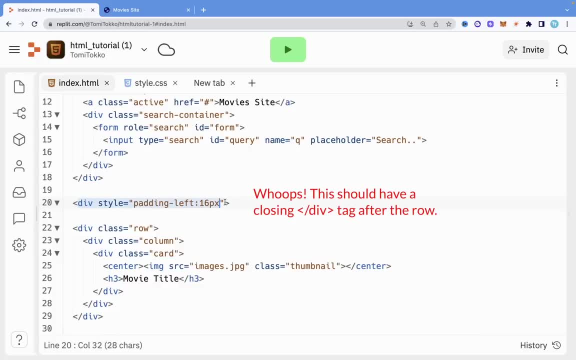 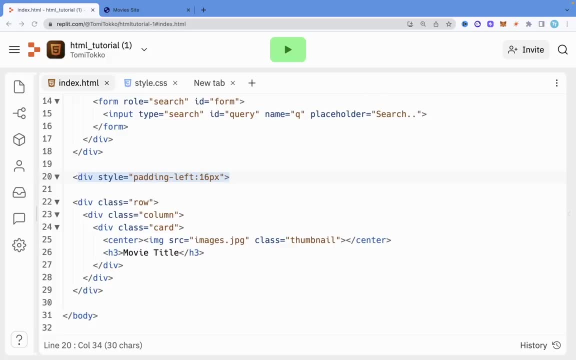 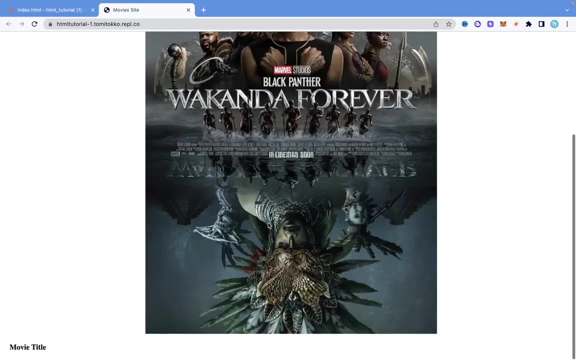 have some spacing on top of it. that is automatic because we already have one div like one div tag here. so once i save that, that should be fine right now and let's see. let's see what we're going to do. so we have the div tag that we've done to this point. okay, cool, so this, that doesn't take. 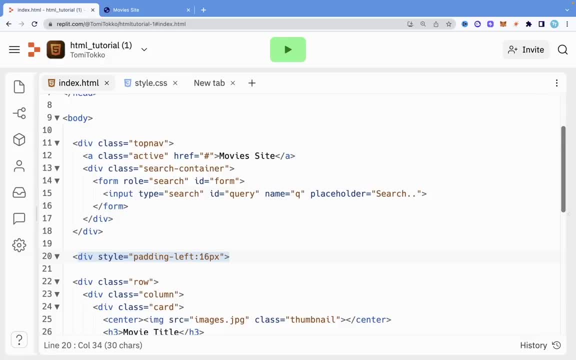 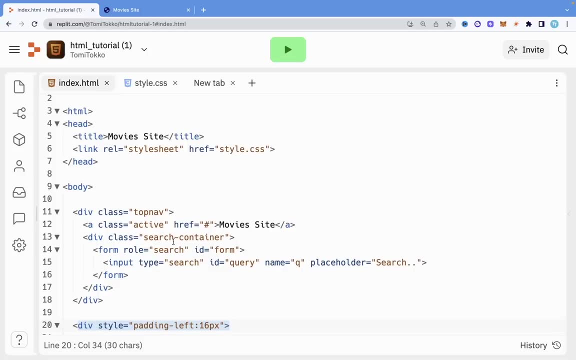 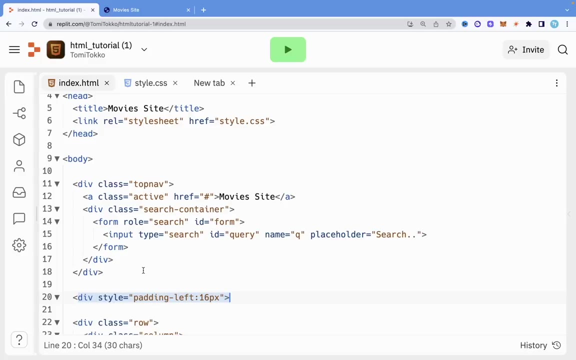 care of the spacing here, but we're going to take care of that in the css. but let's, let's just move forward with. you know the styling, so let's go through what we just did right here. so we created a div class for the top nav, that's for the navbar. we add all the details of the navbar in there. 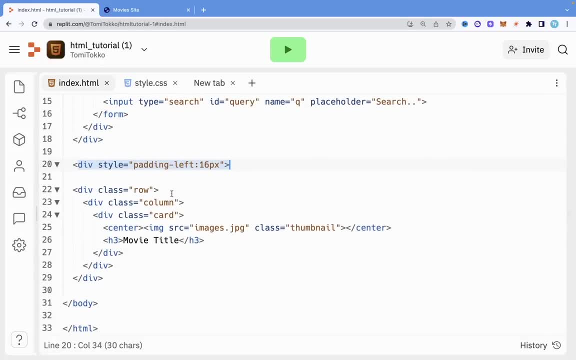 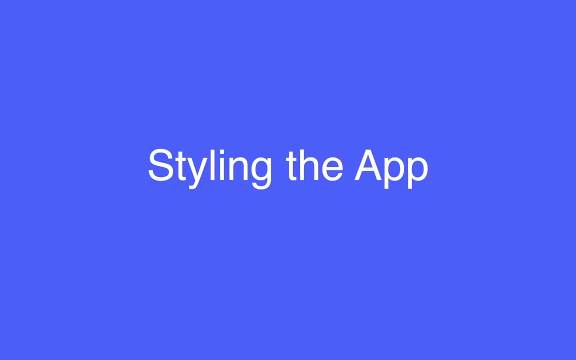 and then we just added this div tag for some spacing, and right here we have the row, we have the card and in the card we have the image and the h3 tie. so we have all of this done. now the next thing we want to do is to actually go into the css and start styling all of this. so right now we're. 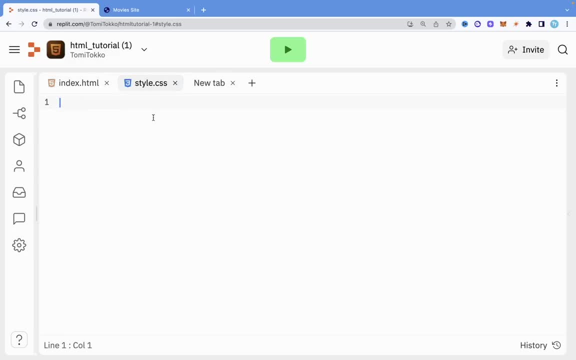 going to come into the stylescss file and let's just get straight into it. so first i'm going to use this asterisk selector and i'm going to say: the whole element in this should have a box sizing of border box. yeah, let's give it that. so, as you know, the asterisk selector basically affects all the 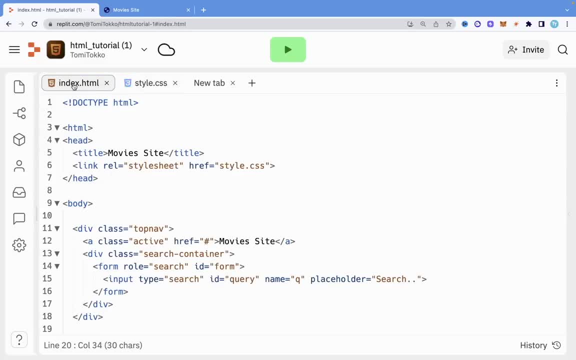 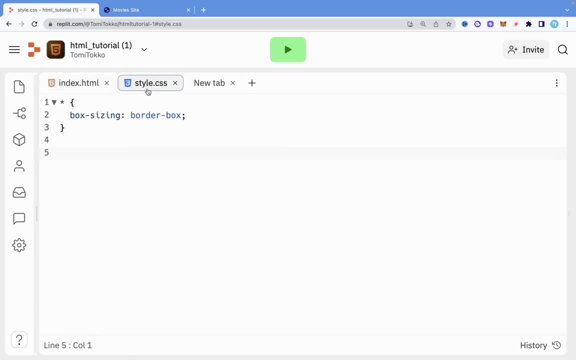 whole element in the html file. before we even get here, we must make sure that this stylecss is connected to this html. if not, it's not going to affect it. so since we know that we've linked it right here using this link element, we can go ahead and start. you know coding right. 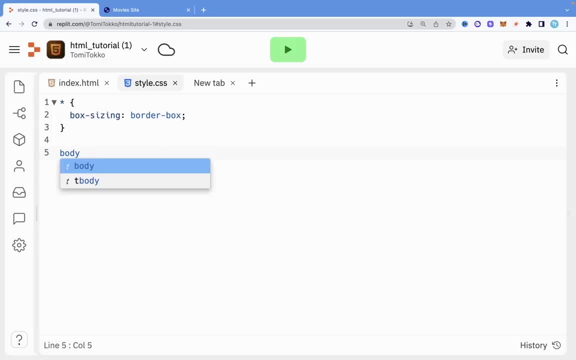 here. so let's see, let's say we want to have the body to have a background color. i'm going to give it this background color. so i'm going to show you the color code. it's hashtag 131 720. yeah, it should look like that. then we're gonna do that and let's give it a font: family. 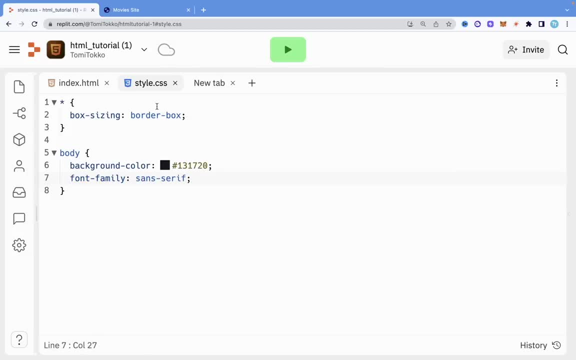 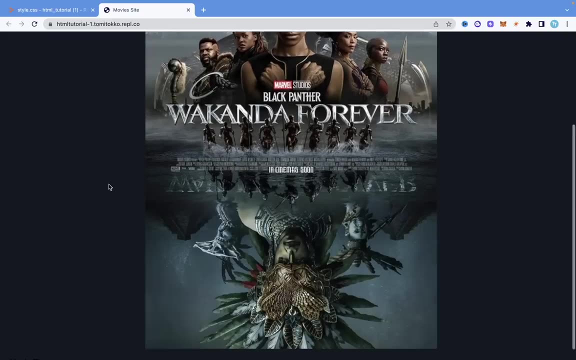 and, let's say, sans serif. now let's save this and let's just see. we come here and interface. good, so you can see. now that is looking like what i showed you in the video beginning. so we have the background color and this is. we're going to take care of this later. 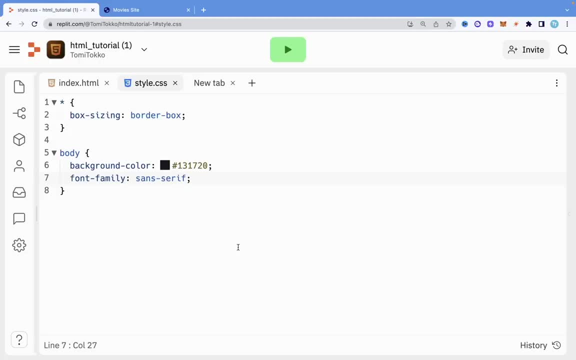 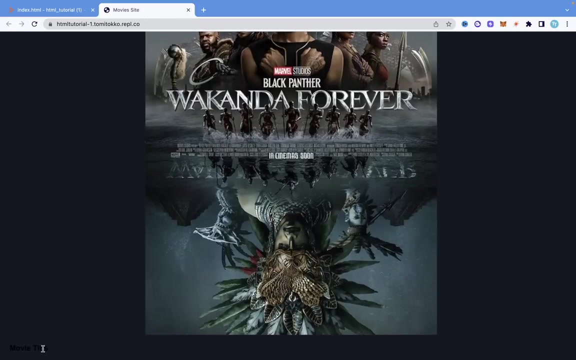 but let's just keep going. so when using replete, you actually don't need to save the file before you come here and hit refresh automatically. it's like saves it for you. that's also why i like replete. so since we've taken care of the body, let's just see. so we can see that right here, this is a black. 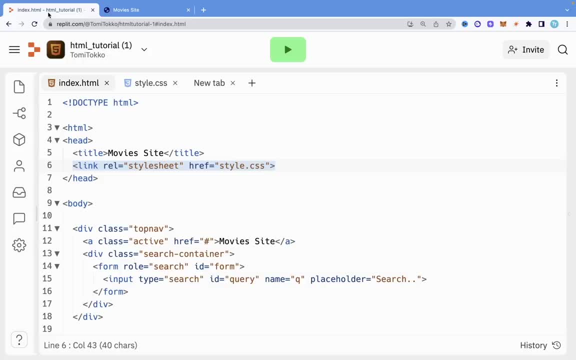 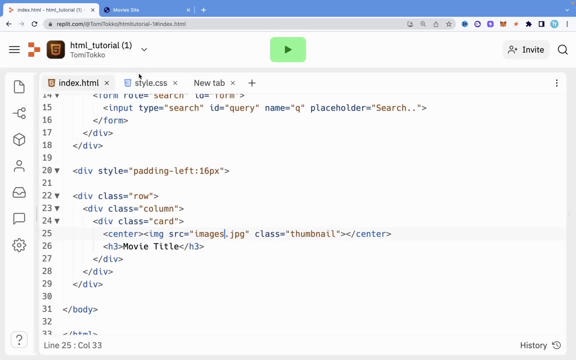 but i want it to be white so it actually shows because of the background color. and that is in. uh, let's see, it's an h3 tag. so we're going to come in here into our stylecss and we're going to say, for h3 tag, you select that. 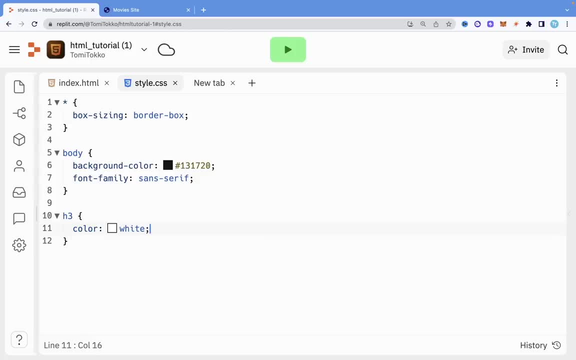 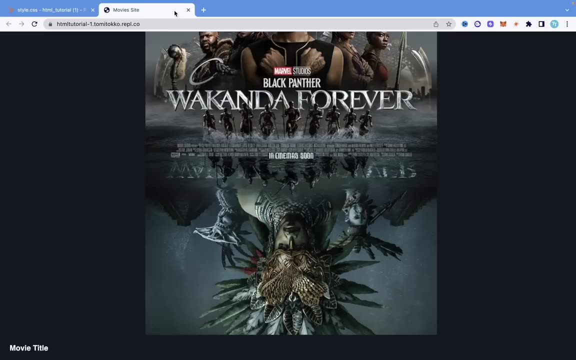 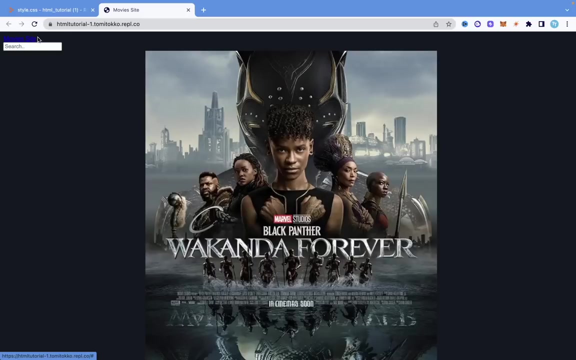 i want to give it a color of white. so now, if i hit refresh, we should see that that is white. good, and what we're going to do now is to just add some proper styling to this nav bar that we have right here. we want this to be here. we want this movie site to actually look good. 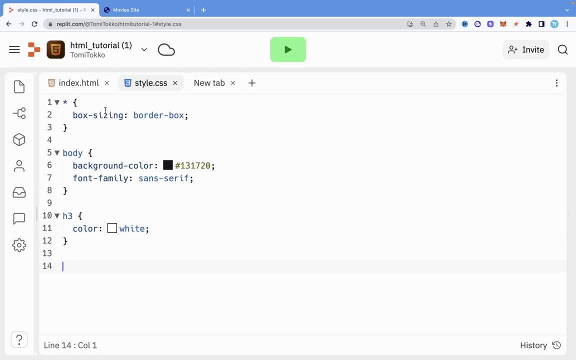 let's do that. so we're going to say: let's see the class we used for that top nav, so let's just copy that. so now we're going to say dot top nav, let's give it an overflow and let's say that should be hidden. 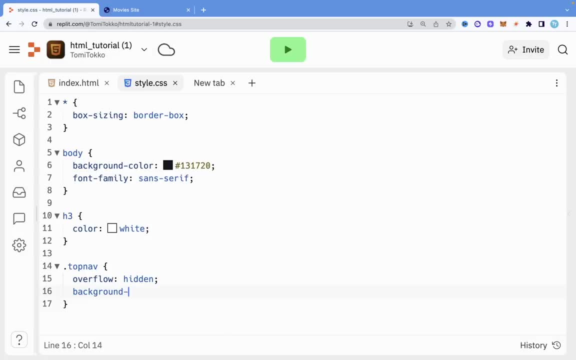 and we're gonna give that a background color. let's give it the same background color as the normal background color of the body. so we're gonna say one, three, one, seven, twenty, and we want to have a color at the top of the body. so we're going to say 131720 and we want to have a 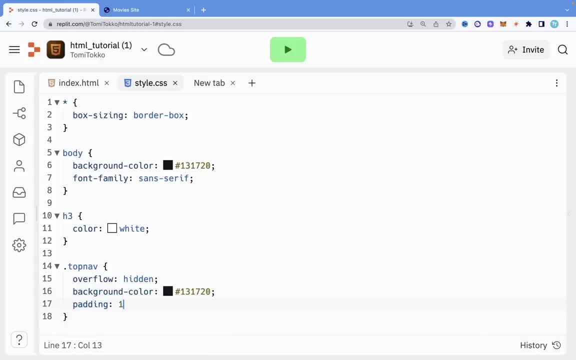 padding of 10px. it's going to have a padding on the top, on the bottom, on the left and the right of 10px. remember earlier in this course i thought about you know this padding when you have just one in css, when you say padding and you have just one value, it uses that value for the left right. 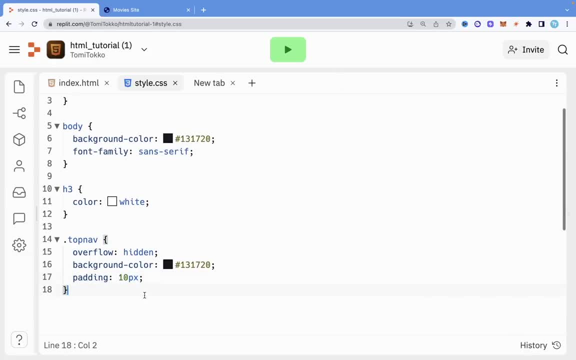 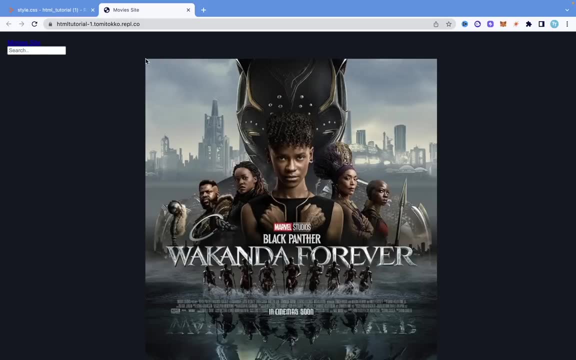 top and bottom. so now let's come here and let's see what that has done. so you can see that there is some padding up here and you can see that the space that we talked about earlier is. you know, it's not as close as it was before. if we have a padding of like 30, this, this is going to come. 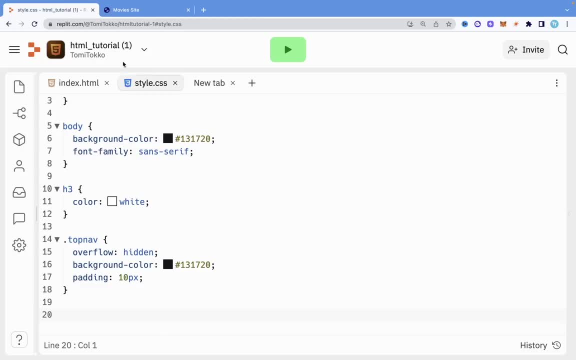 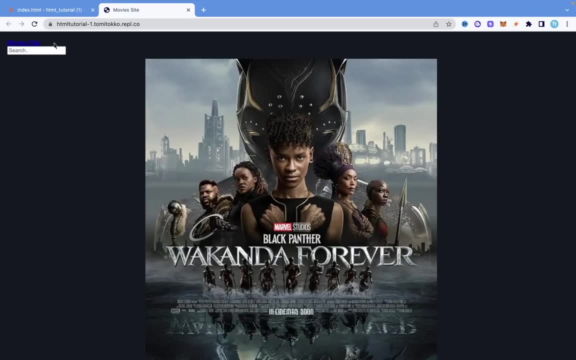 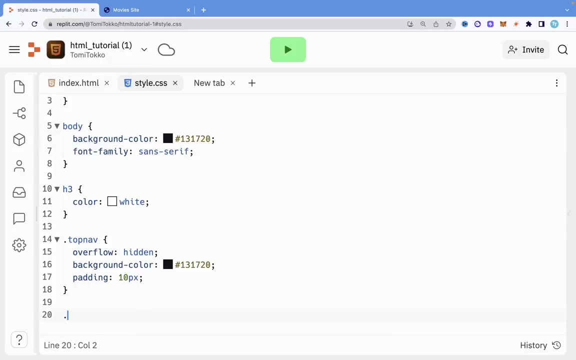 down a lot, but let's just keep going. so now what i'm going to do: let's see, we have in here, we have okay cool. so let's style this movie site. so this movie site is in an, a tag. that's what we're going to do right now. so we're going to say for the top nav. 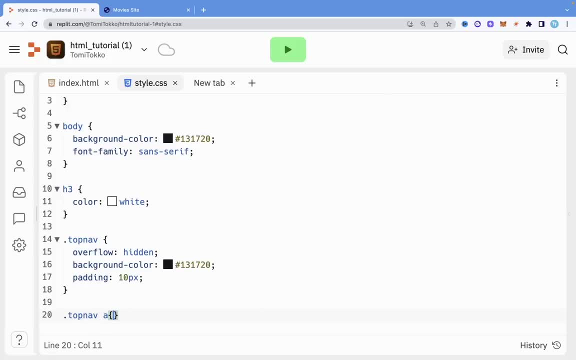 you want to select the a tag in there, the a element, and we're going to say, let's see, let's float it to left. we're going to say left, and then let's have a display of block and let's give that a color also of white. 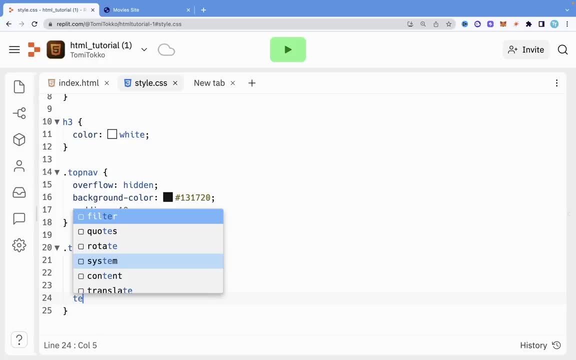 and we want to give it. let's align the text to the center, so we're going to give it a color also of white, and we want to give it. let's align the text to the center, so we're going to give it a color also of white. 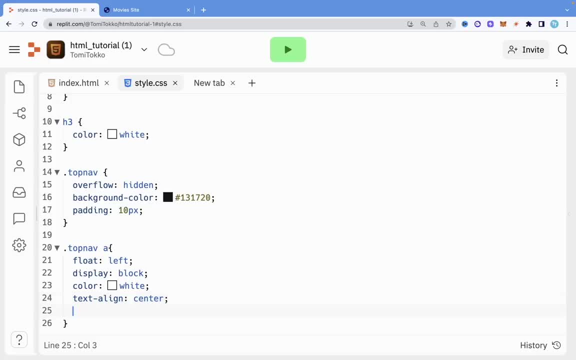 can say test, align center, and let's give you a padding of 14 px and 16 px, so this is going to split it evenly between both top, right and both left, both top and bottom and left and right. so let's also have a text decoration of none, because it is. 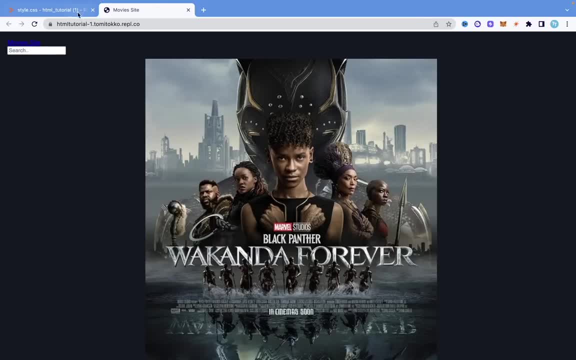 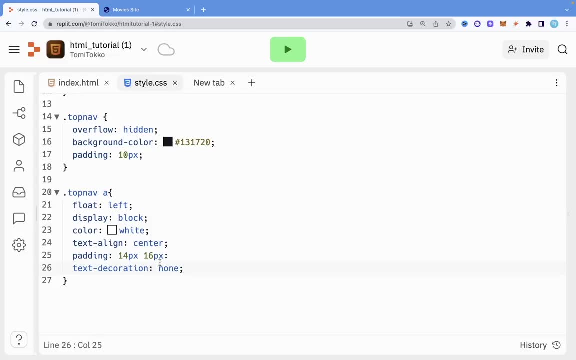 a link, right, it's an, a tag. it's going to have this underline on it. so when we say text decoration none, then that should take care of that. we are not going to have, it's not going to look like a link, basically, and let's give you a font size. so, instead of using let's, instead of using px, 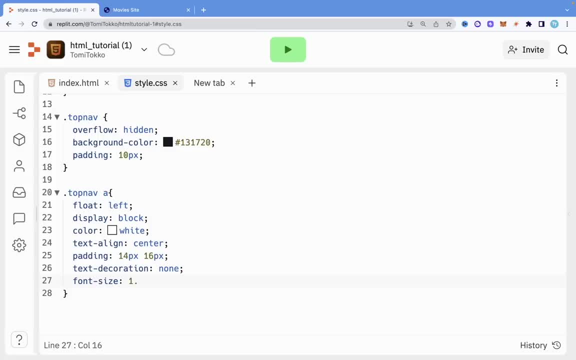 let's just use rem. so i can say one point: let's see two rem and let's make it uppercase. this is the title, the text transform and we can say uppercase. i think that's enough styling for this, and let's see how it looks like. so let's go ahead, and let's go ahead, and let's go ahead and let's. 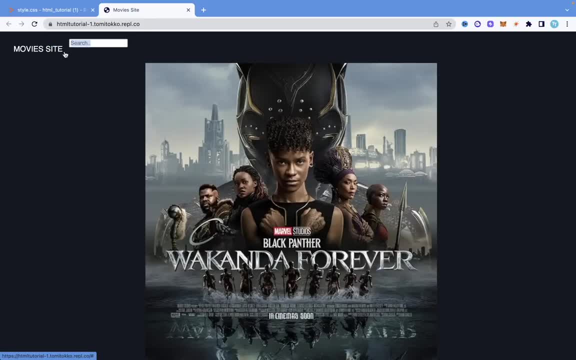 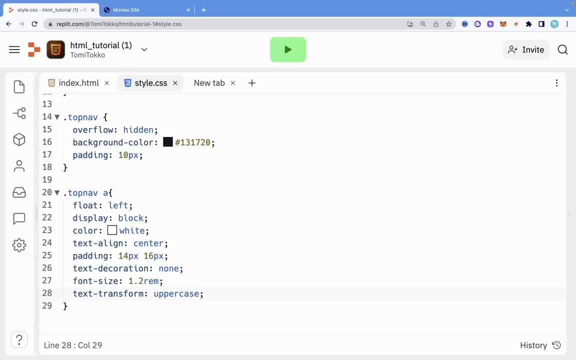 see what that does. so, as you can see, now it changes all of that. it doesn't look like a link. everything is uppercase, test declaration is done, good, so now the next thing that we want to do is to take care of this particular search. it's not looking good, so let's see what that is. so 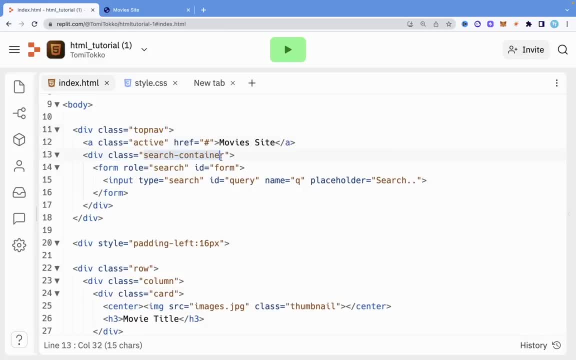 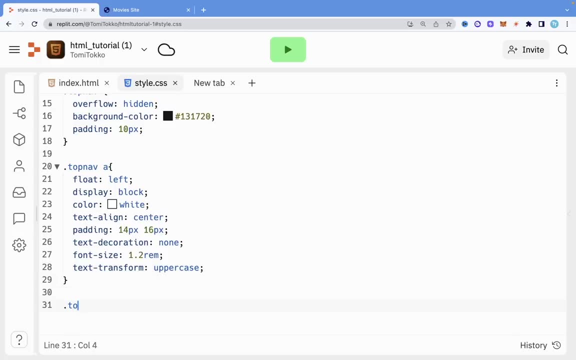 it's under the top node also and it's called search container. right there's in this div class of search container. so what we're going to do is to say dot top nav. since we're using the class and not the actual element, we're going to say dot. 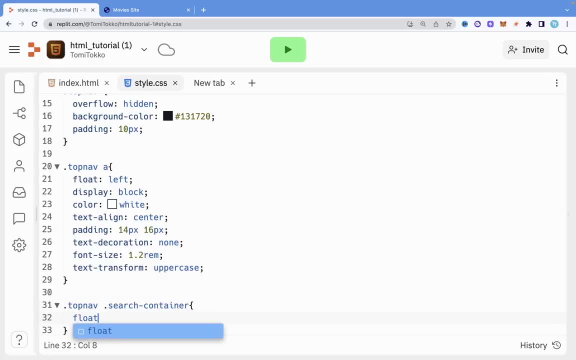 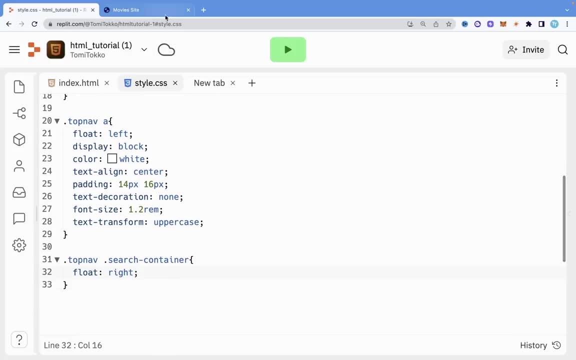 search container and let's float. let's float it to the right. so let's save that. let's hit refresh. you can now see that that is on the right. that is good. now the next thing we want to do is to take care of. let's see, let's come in here. 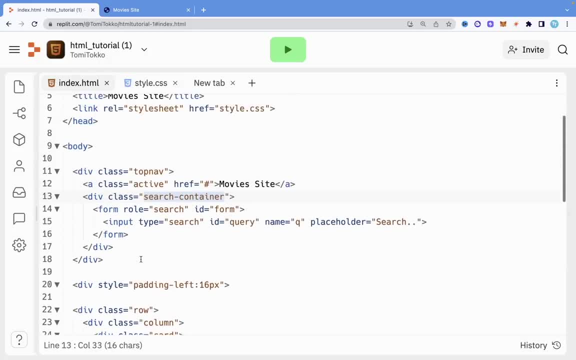 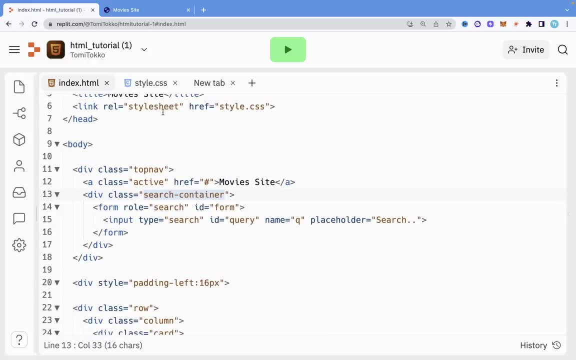 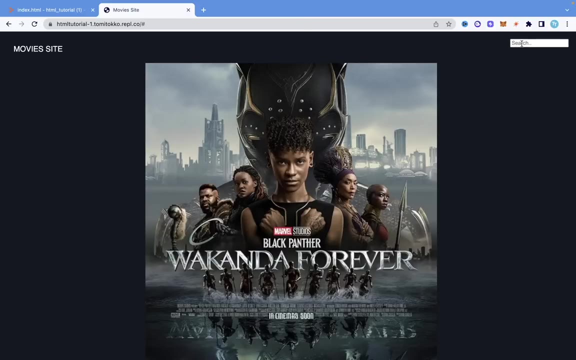 okay, so we're already taking care of that particular search bar and let's just take care of this whole form in general. so what we can do, since we took care of this particular- you know- input, but we want to add more design to this form because it's not looking good right now. 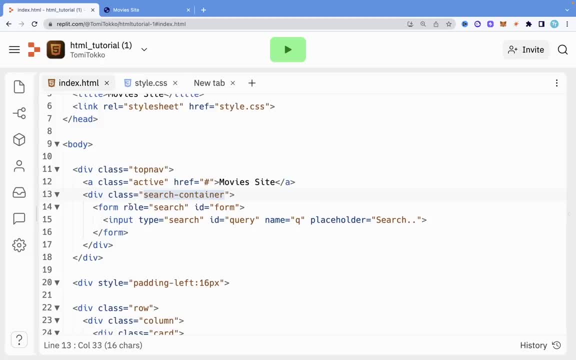 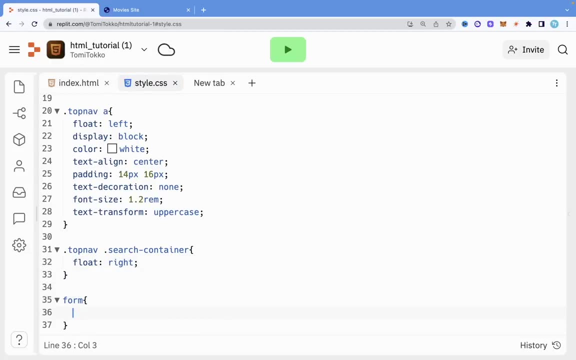 so we're going to do that. so what we're just going to do, since this is already a form tag, we can just come in here and say form, i want the form to have a background color, so i want it to be different from the normal background color, so it's noticeable. let's say 151. 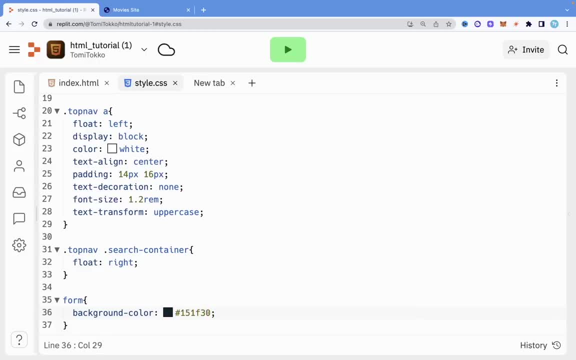 f30. yeah, that's how it looks like, and then we should have, let's see, a width of 300 px and let's also have an height of 43 px and let's get a border radius, so it's actually, you know, circular at the edges, something like this. 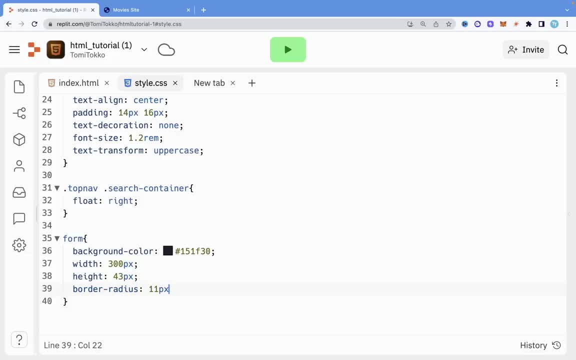 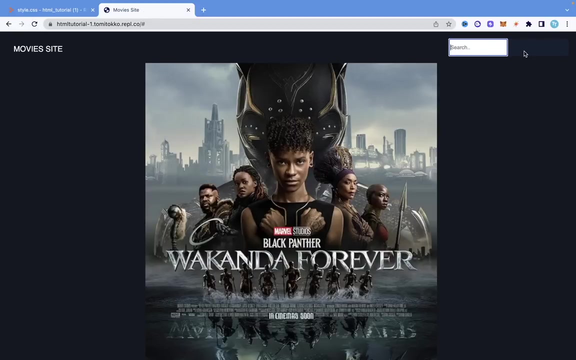 border radius, let's see, let's say, 11 px. and display: let's make this display flex now, just so that looks better. and let's align the items to the center. let's come here and see what that makes. good, so this is what we want to see. okay, so this is how that looks. what i want to do now is to you. 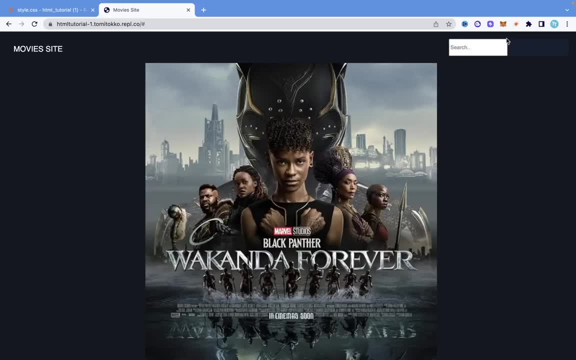 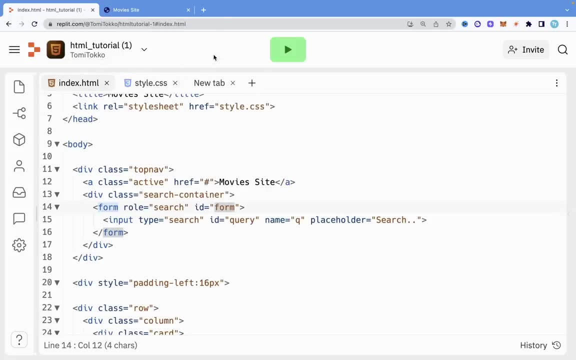 know, give it more styling because i want this. you can see that it still has like an edge, but this has a border radius. i want it to look. you know better. so i'm going to actually style the input, because this is the old form. but this input now is what i want to style, so it has an input tag. 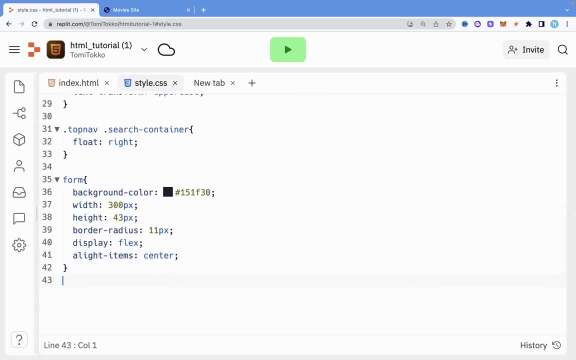 let me just copy that and in here i'm going to say input, input. let's say all should be unset. i'm going to give you a font of, let's say 15 px, and let's give it system ui. let's give it a different color. let's just say normal fff and height. now let's wrap. 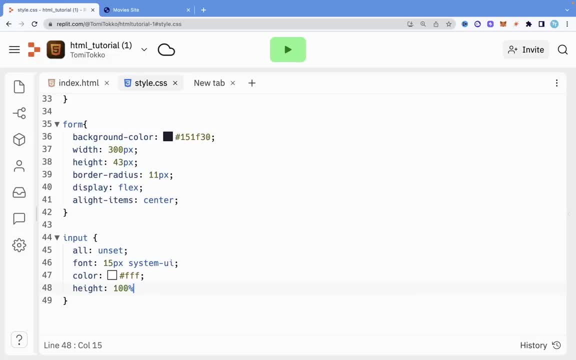 it around everything that the whole. you know ice, that it can take, so 100 of that, and the width it also be 100 percent of that. let's make sure that we have our semicolon and let's give you a padding so the spacing around it. let's give it six pieces and then we can say 9px. let's see that. 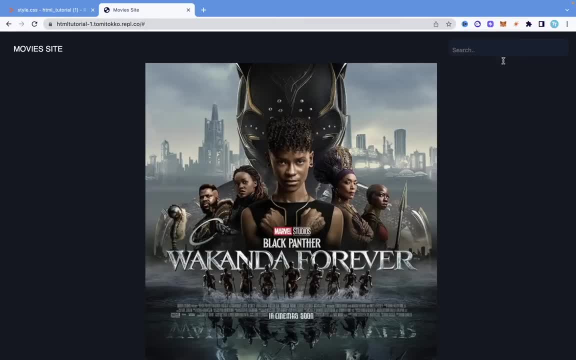 should look good, good. so, as you can see, this looks a lot better. now let's keep going and let's see what we can do. so now that we have that done, i think the next thing we should just talk about is this image: it's not looking good right now, so let's just go ahead and move on to the next thing. 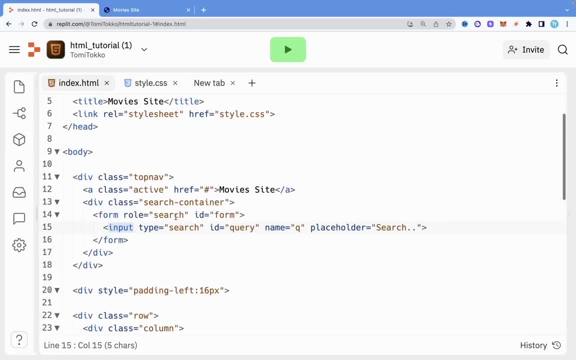 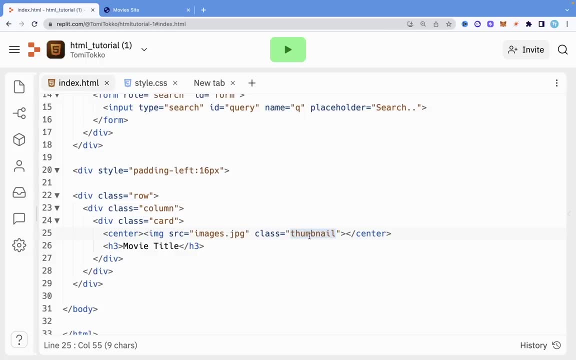 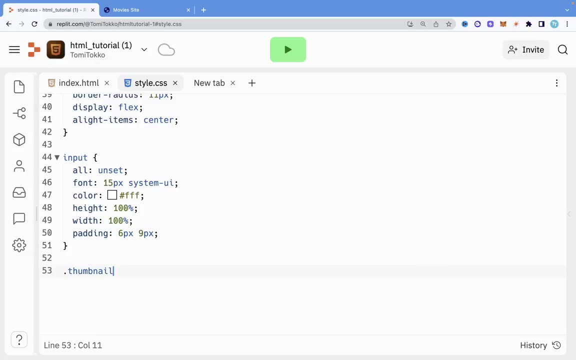 now. So let's see what we use to identify that image by. come in here So we give you a class of thumbnail. in a copy that thumbnail, I'm going to call me to cloudcss And I'm just going to say: this is a class I'm going to use dot. let me give you a height when I 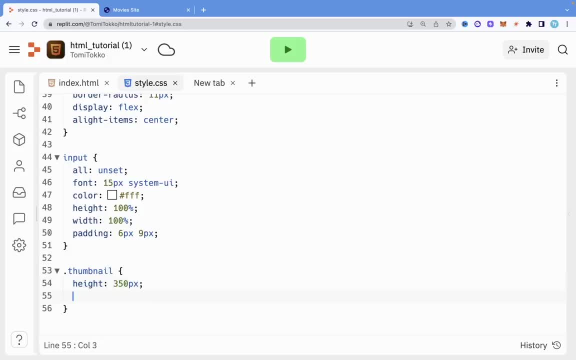 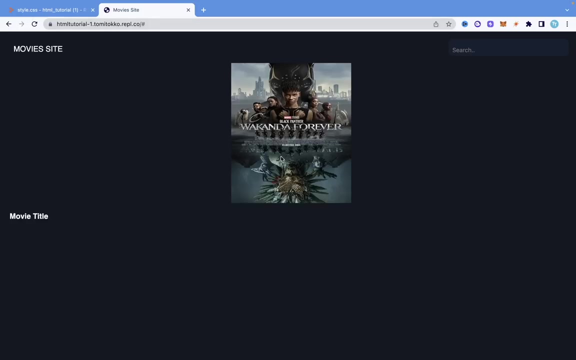 say I should be 350. And I'm going to give it a width, And I say that with it be, let's say 300. And let's give you a border radius, So it's not just like showing like this, as you can see, the border radius of less than 19.. Let's see how that looks like. So, as you, 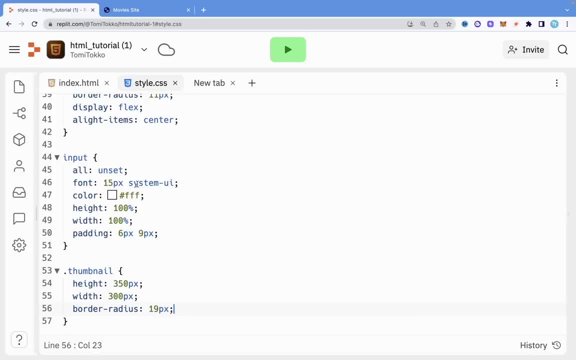 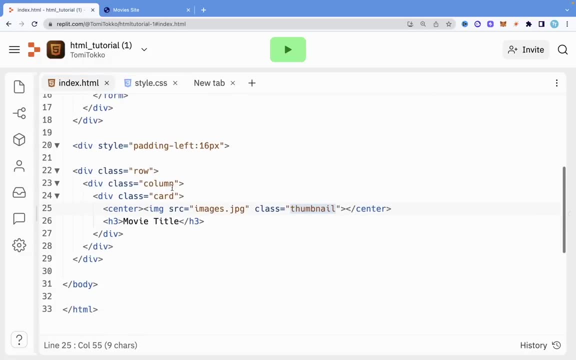 can see that is smaller. Okay, that's good. That's what we want to see. Now. the next thing that I want to talk about is: let me come in here and see. So what we can do now is to start this div tag that I 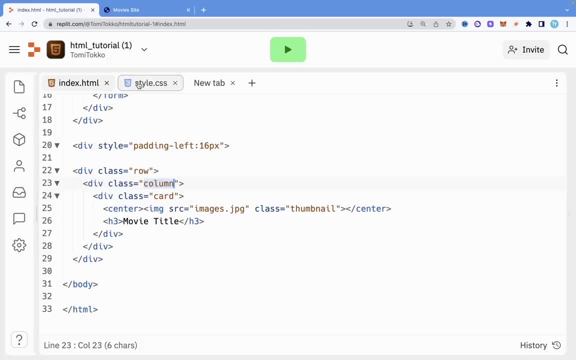 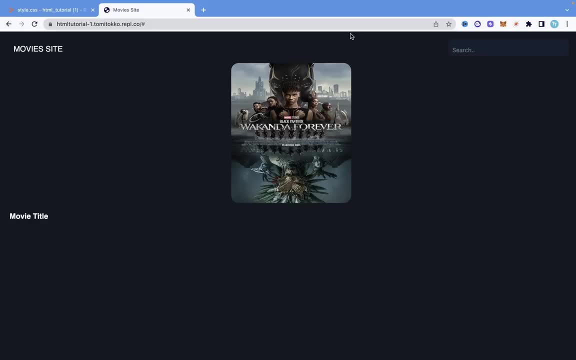 as this colon class. what I'm just going to do is to copy that colon class. I'm going to come in here and I'm going to say dot, colon. And let's look at what is wrong with this now. As you can see, it's in the right, but we want it to float to the left. So what we? 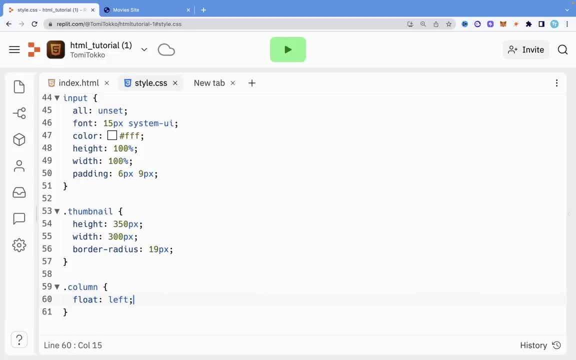 can do is to say: float left And let's say with: let's give it a width of 25%, 25.. Let's give it a padding, So it's going to have some spacing around it. It's a 10px And let's. 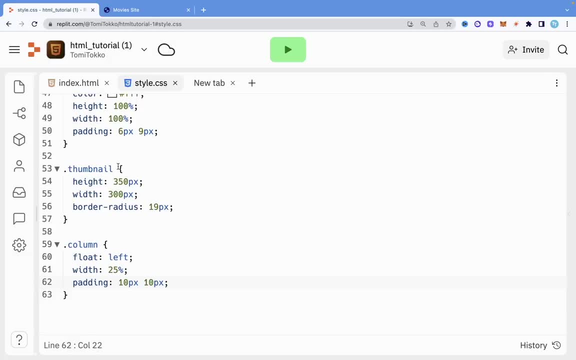 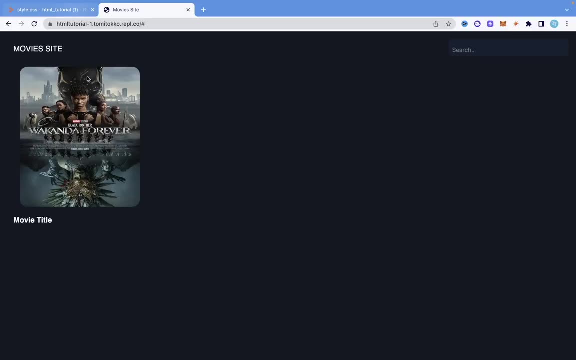 just say 10px also. So that, should you know, give it a little bit of styling as it refresh and let's see Good, So that this is how it looks like. But now, what do we want to do? We want this to be in a card. If we come in here, you're going to see that we have this. 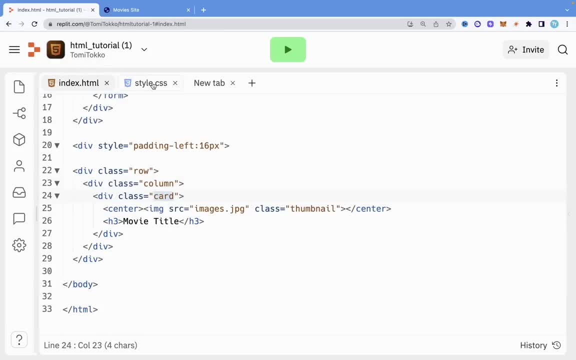 card class, that is, that belongs to a div element. I'm going to style this card So I'm going to say: dot card. What I want to do now is to say: let me give the card its own, a border radius, So it's going to have like a border on its own. I'm going to give 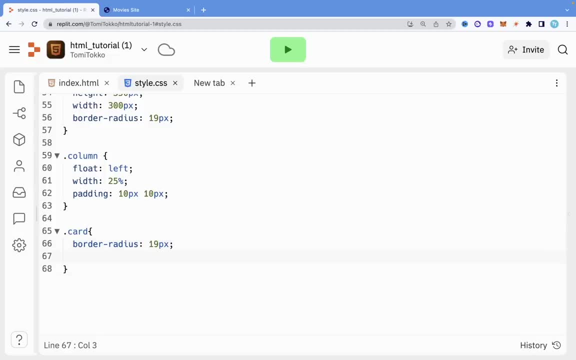 you a border radius of like 19px And I'm going to give you a padding also, So you're going to see the spacing around the card, So you're going to see what is on top of the card. basically, let's say 15px And let's align it to the center. 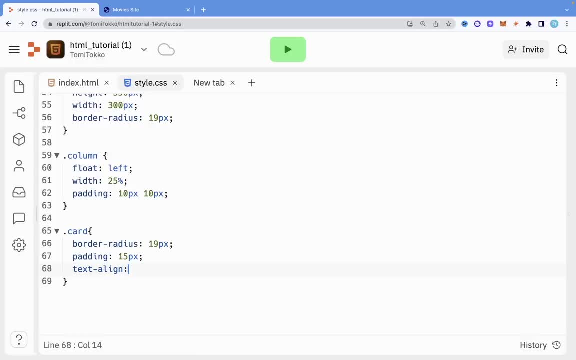 So anything that is with it should be. any text within it should be in the center And let's give it his own background color And let's say hashtag 151, F 30. Just the one we used before. So now I think this should be good with the styling. Let's see the result. 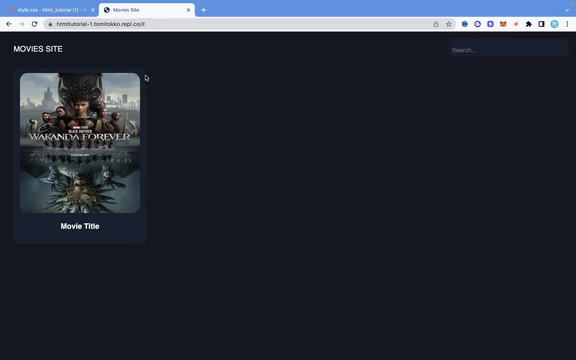 and see if we need to add anything. So let me hit refresh: Good, So you can see now that this is the card. right, It has its own border radius. This is the card that we want to add. So let's say hashtag 151, F 30. Just the one we used before. So now I think this should. 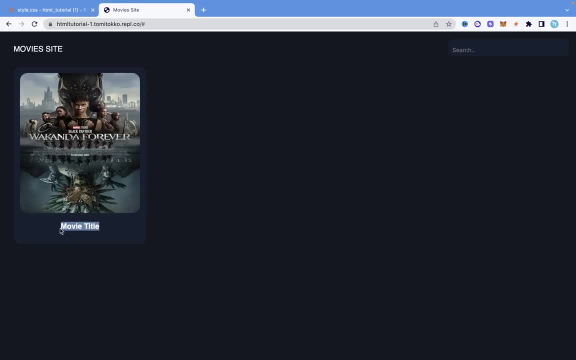 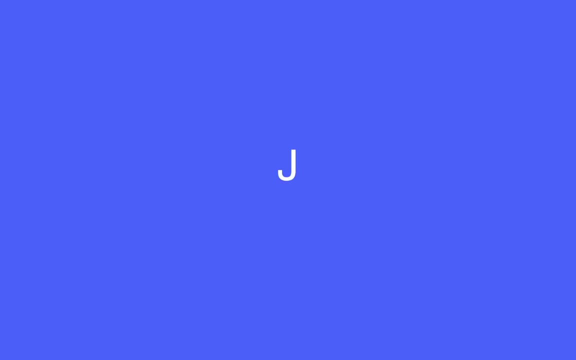 be good with the styling. Let's see the result and see if we need to add anything. So let me hit refresh. Good, So the image it has his own border radius and the text within that card is centered to the middle. So this is actually what we want to do. 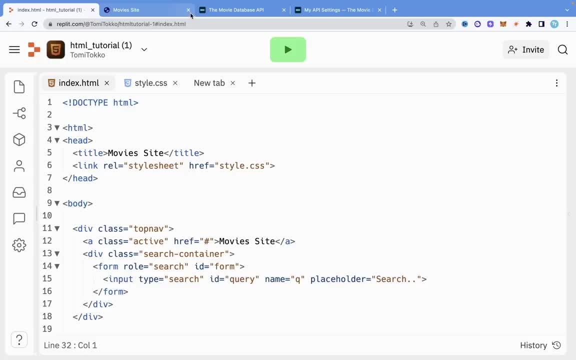 Now that we've done all the styling that we need, what I want us to do, all we're going to do now, is to just add our- you know- JavaScript to it, So we're going to be getting some results from an API. Let me just open the page again. 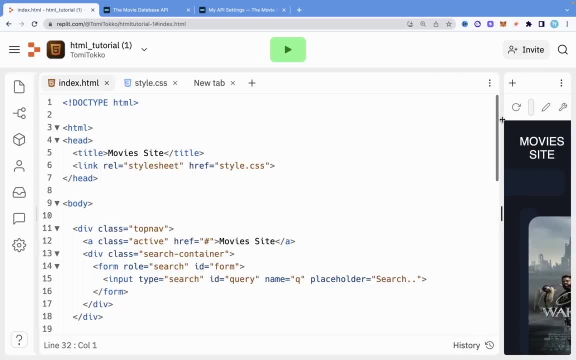 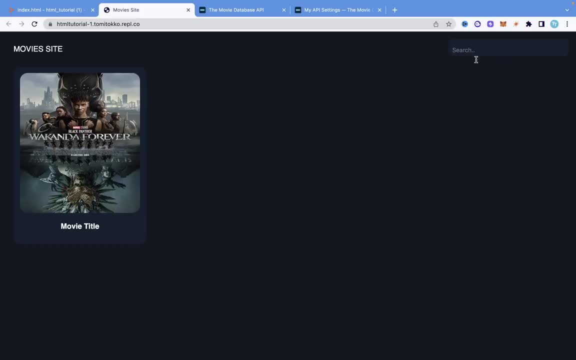 And so just drag this, able to open that. so right now I want us to do is that once we set these, let's say we say something like smile, which is a movie, if you bring out the results of that movie for us, which you know, the image and then the 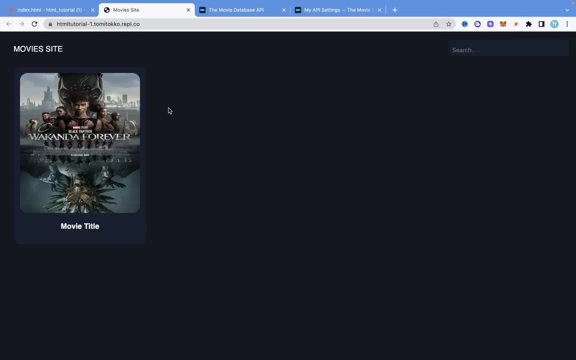 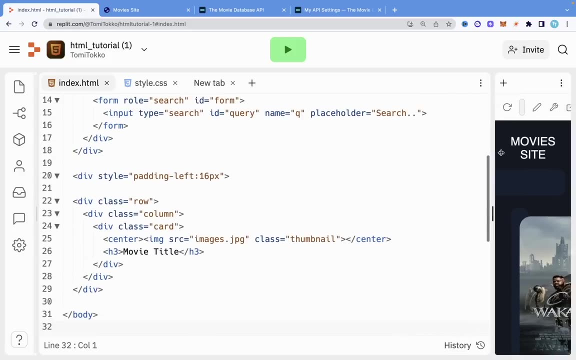 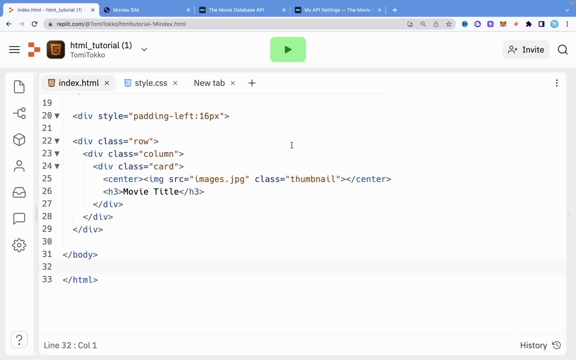 title. so for now this is just a static, you know data, because right now is just the data that we put right here in our HTML. but we want- let's just close this real quick- but we want this data to be like dynamic, like whenever we set something, that is what you show there. so what we're gonna do to or we're gonna- 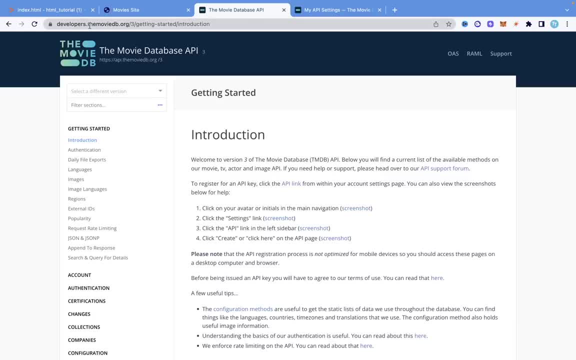 use to do. this is an API, so we're gonna use this movie DB API. so or you just need to do- you don't need to read all of this- you just need to make sure that you have an API key from this movie DB API to move forward now for each of these. 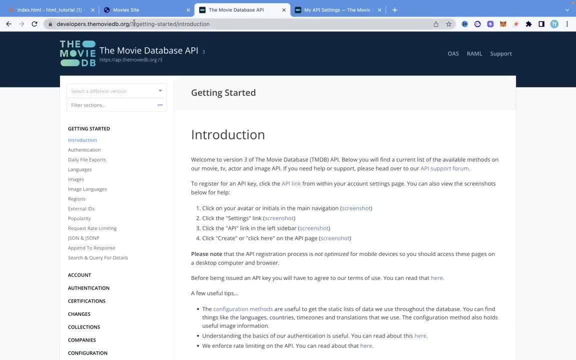 API key you need to click, you need to come to this page, right here, right, and then you need to click on this api link. so once you click on this api link, it's going to take you to where you're going to create an account and login. once you do that, make sure that you click on this api link and then it's. 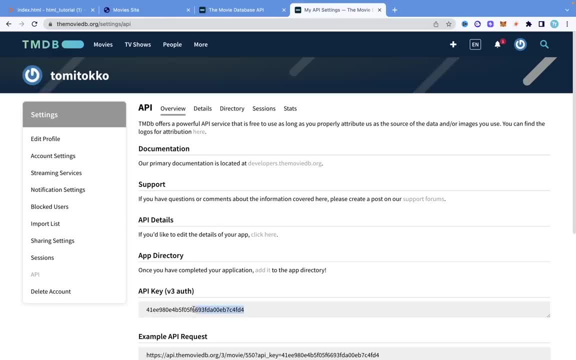 going to take you to where you can create an api key. so i have created my api key and this is the api key i have right here. you need this api key to move forward in this tutorial, so once you know that you have this done, we can move forward. so the first thing that i actually want to do before i go: 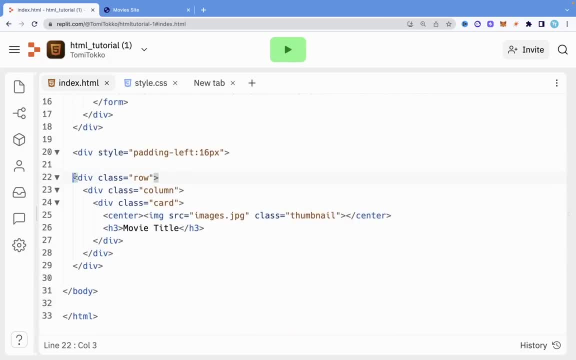 into my javascript. is that right here? i want to make all of this, all this old div, be inside like a section. so i'm going to have a section element and i'm going to put all of that in there. now, this is just so that i can group all of this into one section, and when i'm using the javascript, you're. 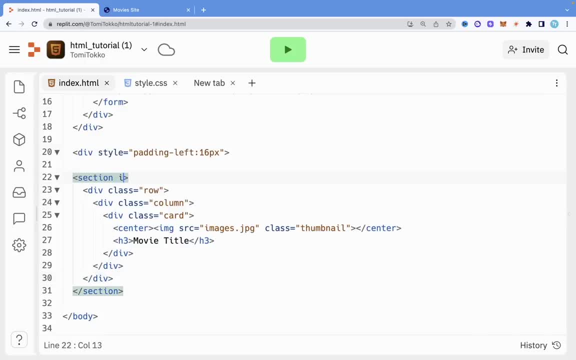 going to understand later when we are coding it in javascript. so i want to give it an id of- let's say, the id should be section- and i actually want to get rid of all of this. so for now, i'm going to comment it out now. this might look weird for now, but i'm going to explain why i'm doing this if we come back in. 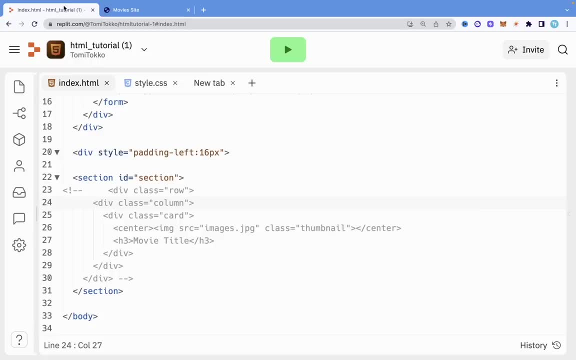 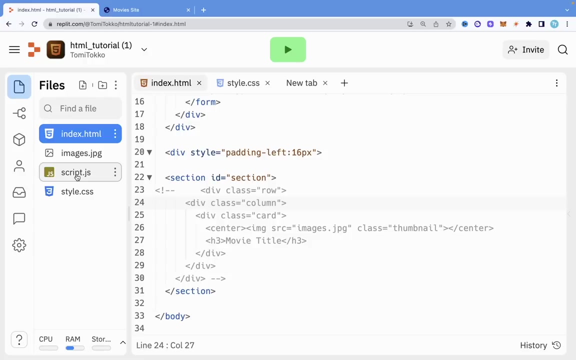 here and hit refresh. we're not going to see any data for now, but what i'm going to do is that i'm going to use javascript to dynamically automatically create all of these tags right here. i'm going to show you in a bit. so if i open this up, you're going to see that we have this scriptjs, so i'm 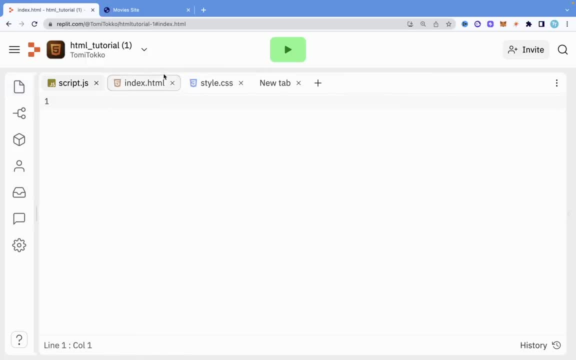 just going to drag that scriptjs right here because we need that now. but before we can even use this scriptjs, we need to link it with our HTML. so to connect your HTML file to this scriptjs file, you're going to have to use the script element and it's going to have a source, so you're going to give it a source. 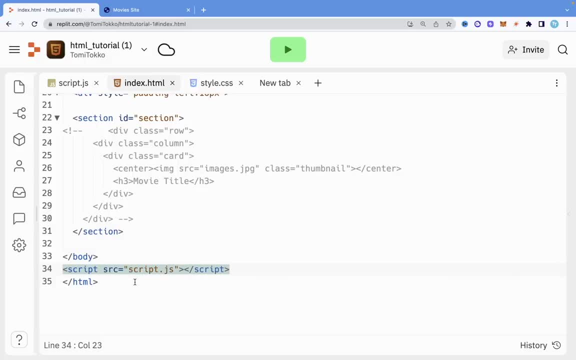 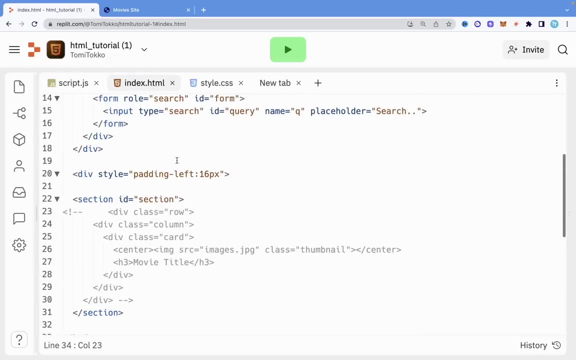 and the source should just be scriptjs. so that is that. and now, when any javascript we put here will be this, it will have an effect on this right here. so i'm going to walk you through everything that we're going to do right now. the first thing we're going to do is to create like six different constants, or 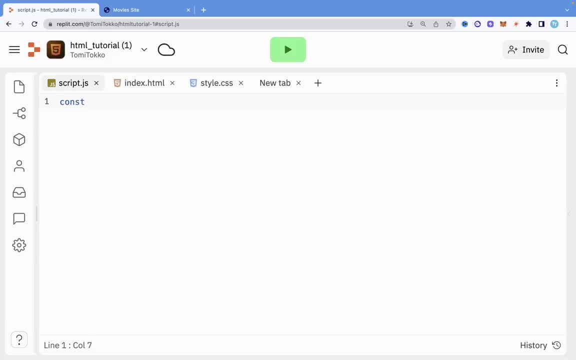 variables. so I'm gonna have const, I'm gonna say API link and for now I'm gonna leave this blank. I'm gonna come back to this and I'm gonna have another constant and I'm gonna say IMG path. so this is the image path that is gonna show that. 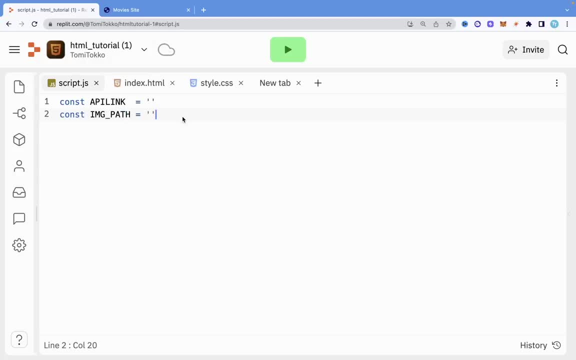 is gonna, you know, specify the paths or the link to the image of every movie, and I'm gonna have another constant and let's say, search API. now, these are the API. you know, remember, I say we are using that API, right? so this is specifying the link of where we can access the API from, and this is specifying, you know, how are. 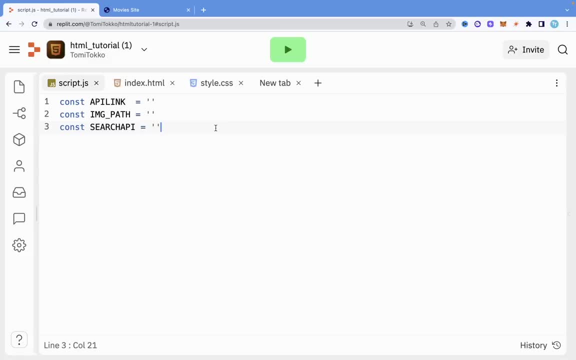 we actually gonna search for something and get some response from that API. so now that I have all of that, what I'm gonna do is to give you some values. so, right here on API link, I'm gonna paste in this code this link. actually, you can see that I have a link here and I'm gonna paste in this code this link. 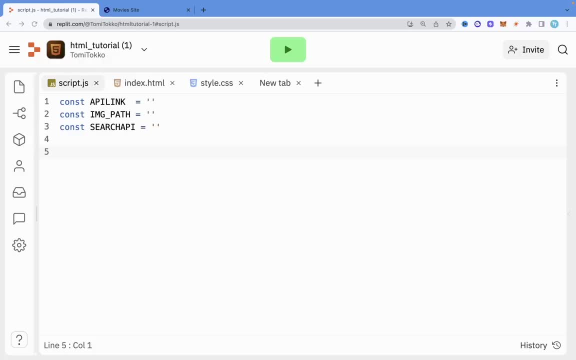 actually, and what you just need to do is to type out what I pasted and I'm going to explain it for you. so, right here, I'm gonna paste this in here. so, as you can see, this is like the link to that, the movie DB that I 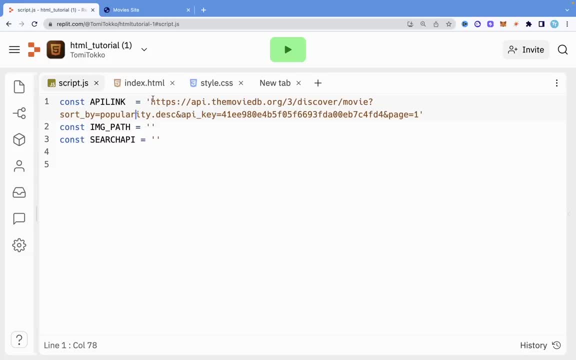 talked about, but we're accessing it through his API, so just write everything out the way it is, right here with the page and every single thing. the only thing you need to change is your API key. remember when I showed you how to create an API key from there? make sure that. 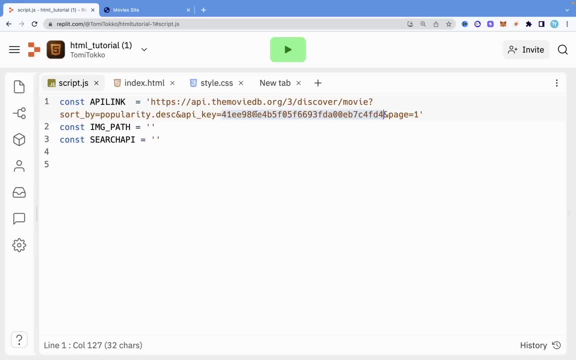 this key right here is your API key. so this is my API key, but make sure you change it to yours. and for the image part, I'm also going to paste in an image link and I'm going to show you what this is. so this image part is actually the. 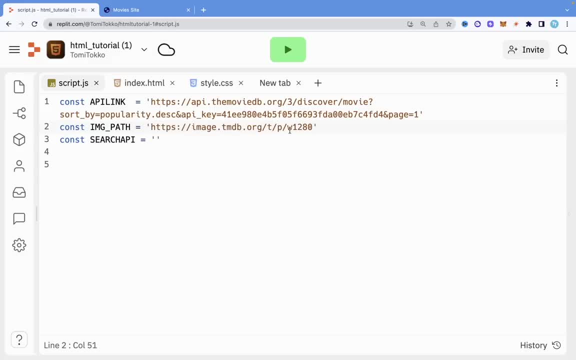 root parts to every single image of the movies. so that is what this is. and then for the search API, I'm also gonna paste in the query. so what this does is that if I paste this, it uses that the movie DB right to search for a movie, and you must change this to your API key. 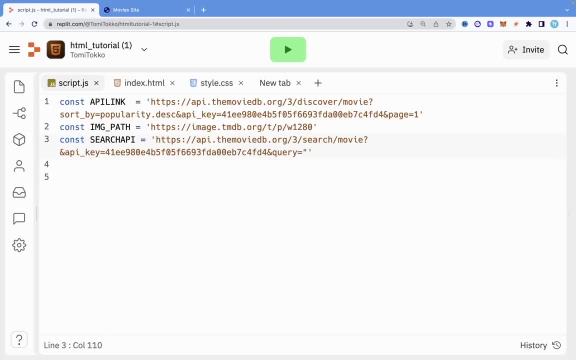 also. that's the only thing you need to change, and this query, we are going to add our own query to it. so what I mean by that is that the query that we use is what we're going to add, like, let's say, for example, if a user searches for, like you know, Black Adam or something else, that is what. 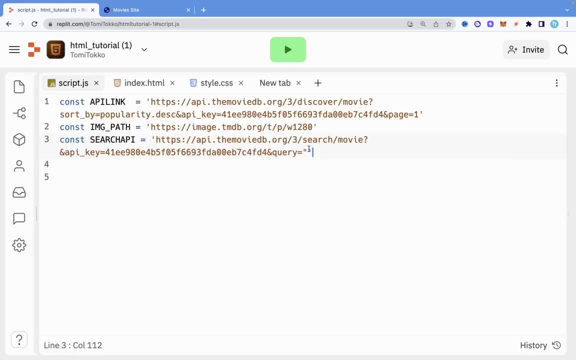 is going to be put in this query right here. so that is what you need to know. so let's get rid of this. let's make this double quote right. so now that we know that we have all of that, since this is JavaScript you must add, you should add- a semicolon at the end of this. and now the next. 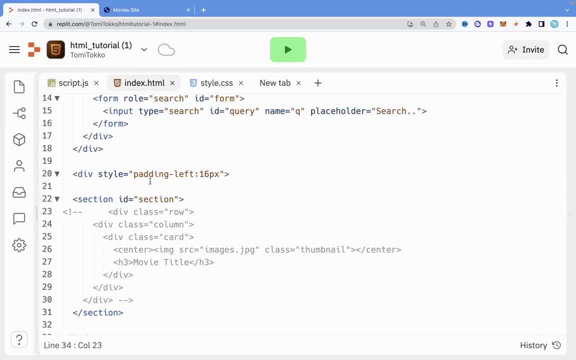 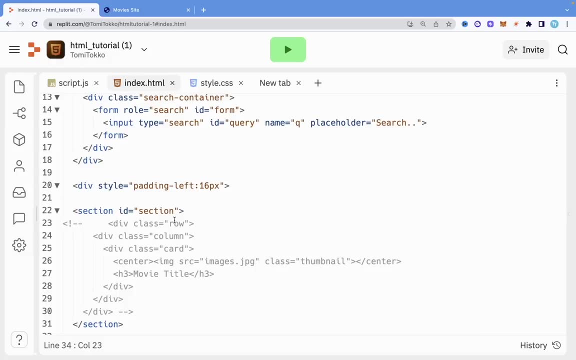 thing I'm going to do is to actually get some elements in this HTML file, so I want to get this whole section. so what? let me walk you through what I'm going to do to actually make this work. so what I'm going to do is that I'm going to, when a user searches for something and click enter. 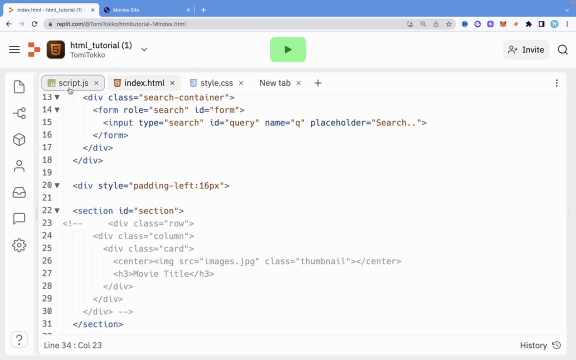 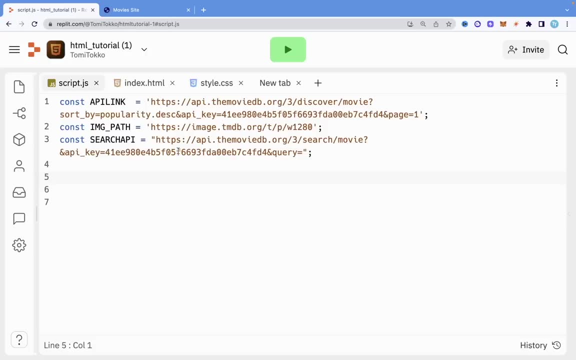 we're going to have a function that gets the result of what the user search, then sends that query to this API and the API is going to send up some response. so let's say, the user searches for like Barbie, right, it's going to send us, let's say, 10 or 20 different responses, with the image and. 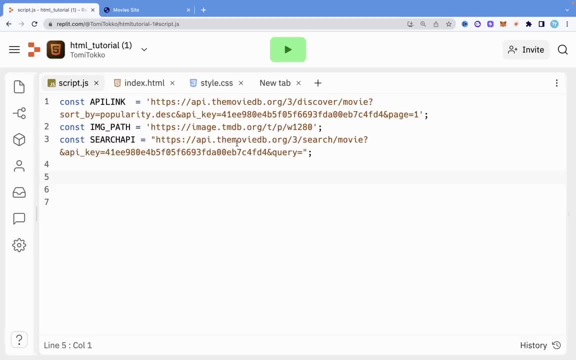 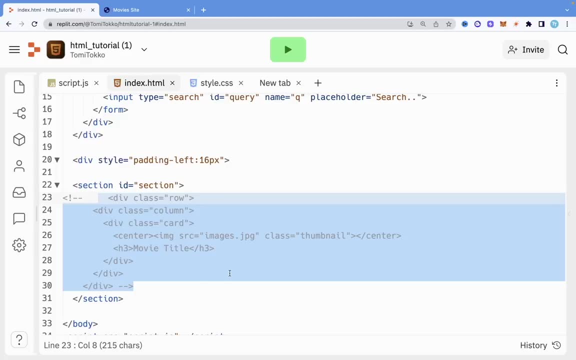 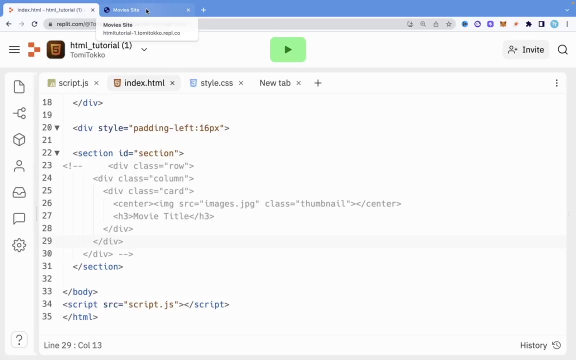 the name. so when I get those image and the name, I'm then going to create a div, this, all of this div tag right containing the data of that particular image and name. right here you can see that we just have one div tag, but what I want is that, depending on how many 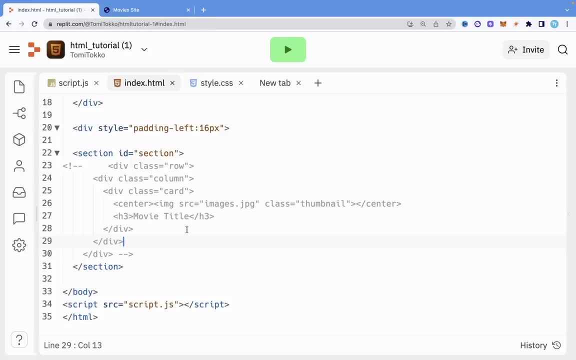 results right that we get. that is the amount of div tag I want to have. so that's why we're going to have to create this div tag from JavaScript. so there's a way JavaScript can create an element for us and it's basically going to create all of this. I'm actually going to delete all of this later, but 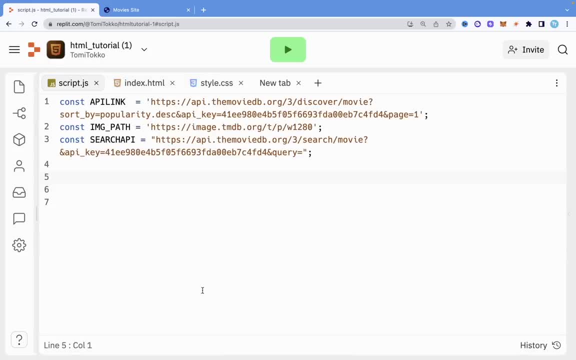 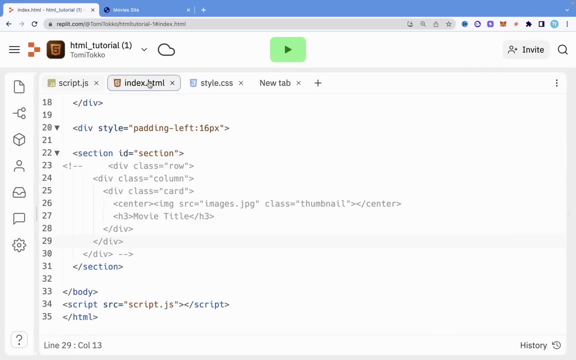 for now. I'm going to use it to reference when we are creating all this tag in JavaScript. so let's move forward and let me explain. so what we need to do now is to get this. we're going to get this section right and then we're going to. we have to get the form which: 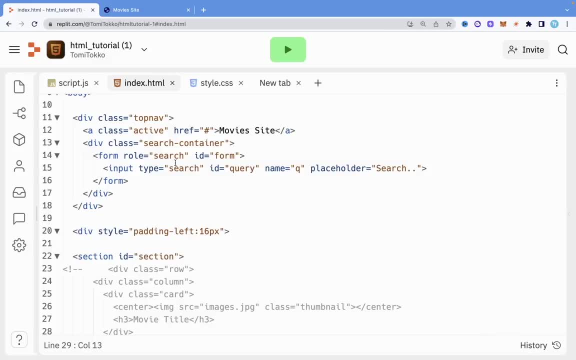 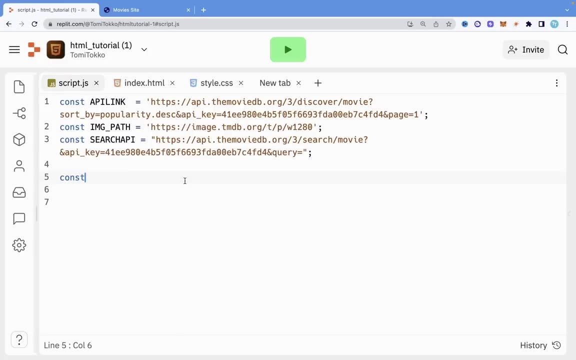 is this form right here so we can actually get the from the form we can get the. you know the query that the user search for. so what I'm going to do now we need this section. so I'm going to say let me name it main. I'm going to say: equals to document dot get element by ID. I'm going to name it section. 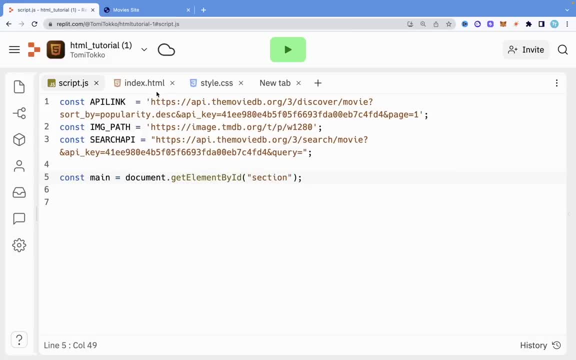 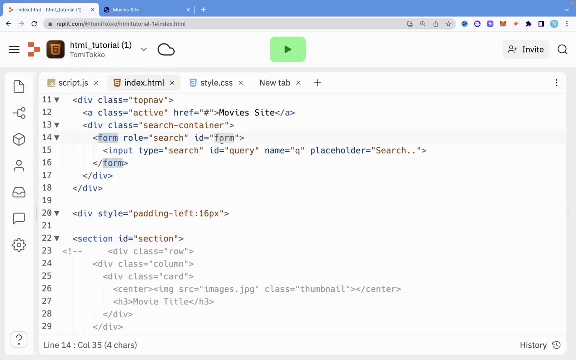 so we're getting the elements by the ID and the ID is section right. we're going to do the same thing for the form and search. so we're going to say form search, so we want to get this whole form right, and by getting it by the ID, we need to use the ID of form and then for the search, since we 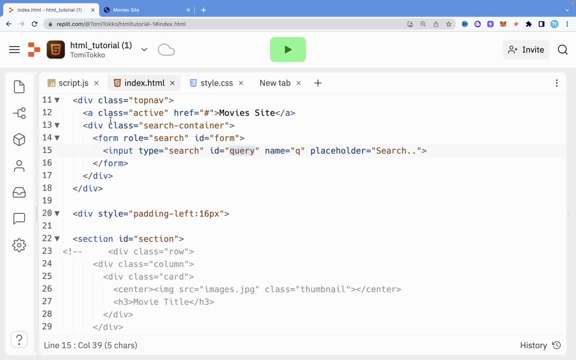 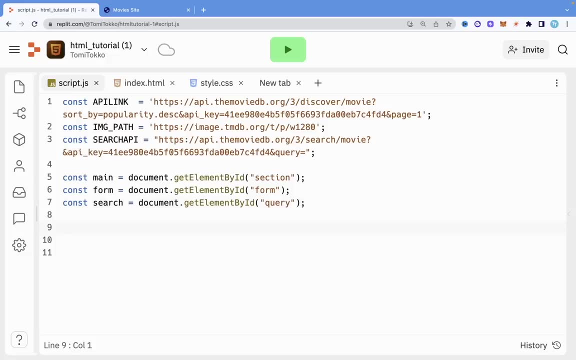 want to get the actual query, we're going to use the ID of this input and we're going to say query. so once we have that done, the next thing I want to do now we're going to have to create a function named return movies. so let's just say let's see, let's say function and we're going to say return. 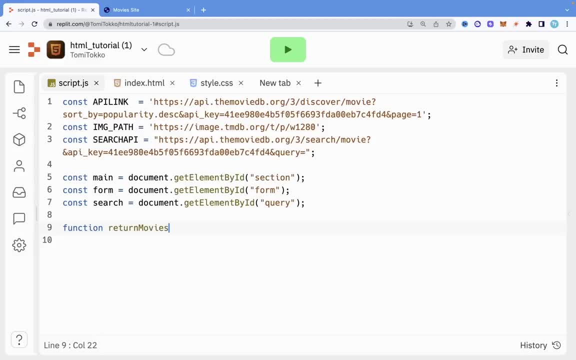 movies and we're going to give it a URL to outside here. when you have this and what we're just going to say is we're going to use the fetch, so we're going to fetch from the URL. so then I'm going to say res equals, greater than resjson, because I'm going 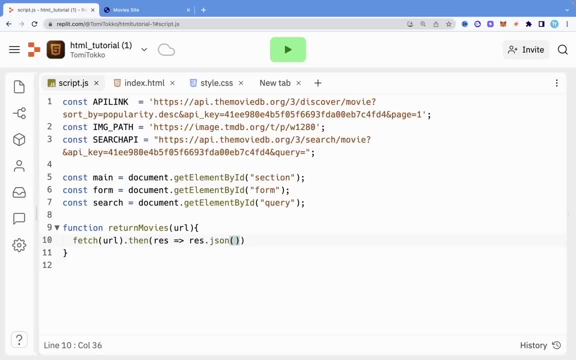 to get a JSON response. then we're also going to say that's then function. and here we're going to say data, right and right. here we're going to open under curly braces and let's just say console, let's print out the data in the console so we can just say data, the results. we can use this to debug later. 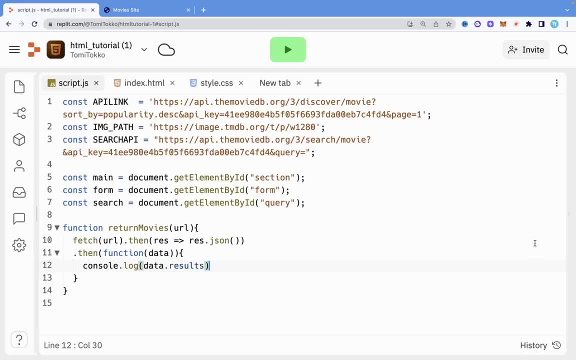 let's just have that right there and now. what we can just basically do is to say data results. so I'm going to come down in here and I'm going to say, right here, we actually need to have a semicolon to show that. that ends there. I'm going to say the data, that we get the results. 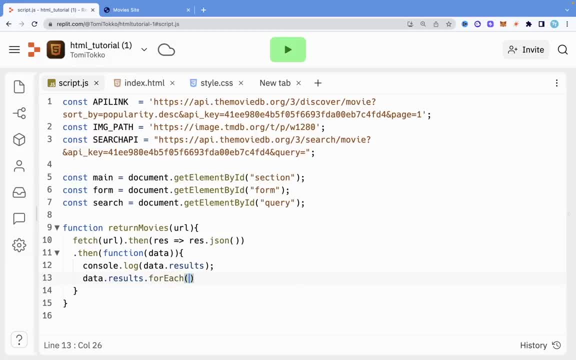 dot for each. so we're basically looping through all the elements in the result. so for each element I'm going to say: let me have it here, element. and then what we want to do is to say I'm going to create some constants now. so I'm going to show you all of this, why I create all. 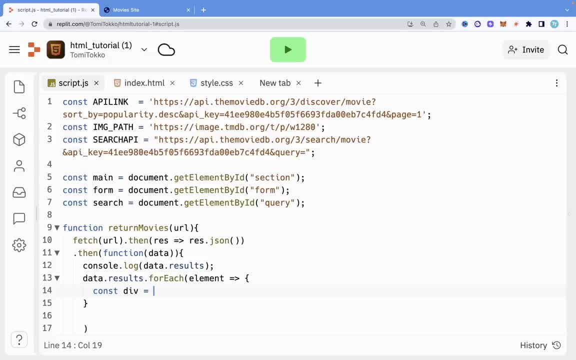 this constant. but for now let me just say: div equals to document dot, create element. so I'm creating a new div tag right in this, my HTML. so, as you can see, when we say create element is creating a new div element and we're storing that in this constant name: div. so for now, let's. 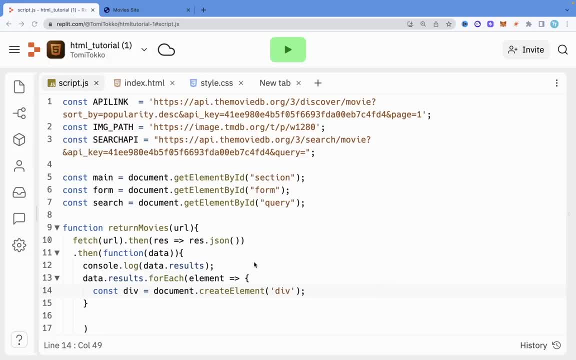 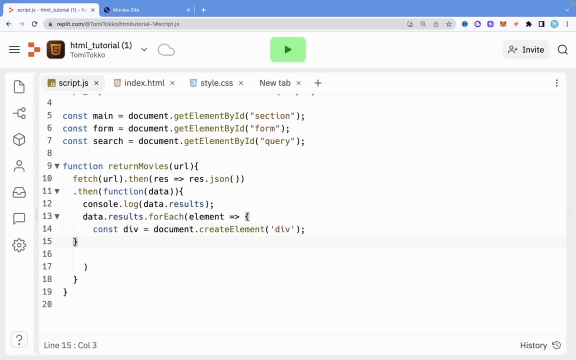 just, you know, go through all of this and what I want to do. I'm going to show you why we use all of this later, but for now, let's make this here. I'm gonna do this and what I need to do is to add this here, just to have. 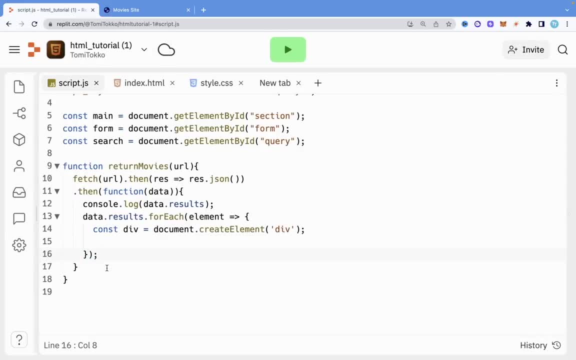 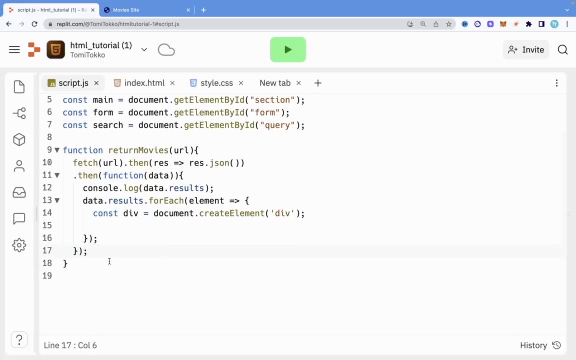 perfect and right here we need to have the closing bracket and we put that there. so this is everything in this particular function for now which is working. so what I want to do is, up here, I actually want to call these return movies, so up here I'm going to paste that function. so I want to, you know, call that function up here and 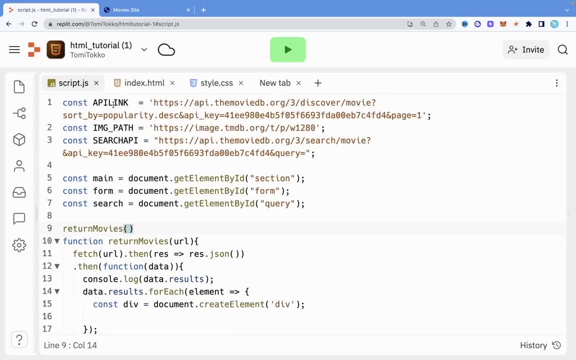 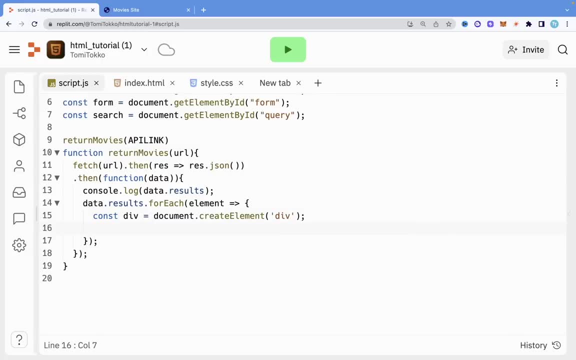 the URL that I'm going to give. it is this API link right here. so that's the link that you know we want it to fetch from. so now I'm going to explain everything I'm going to do now briefly. so what I want to do is I want to create, you know. 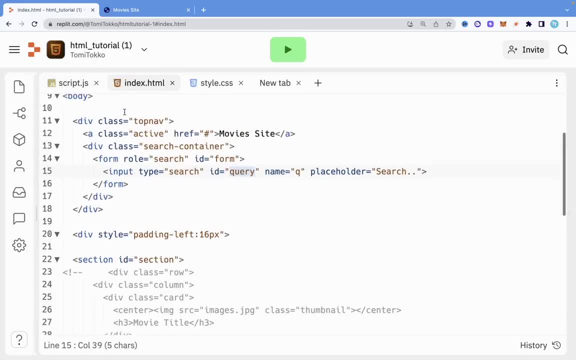 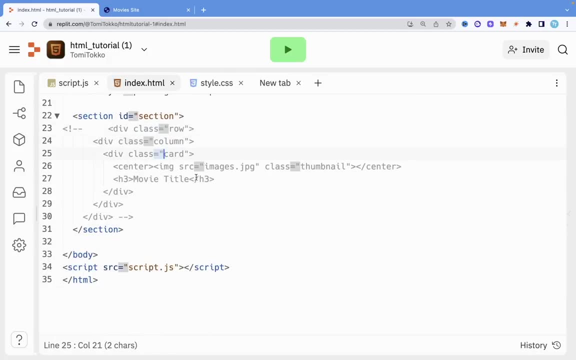 a div tag for all of this. so I'm going to create a div tag for the row. I'm going to create a div, a div element for the colon, for the class. yeah, I'm also even going to create like an image element. I'm going to create this center element, this h3. I'm going to create everything and once I create, 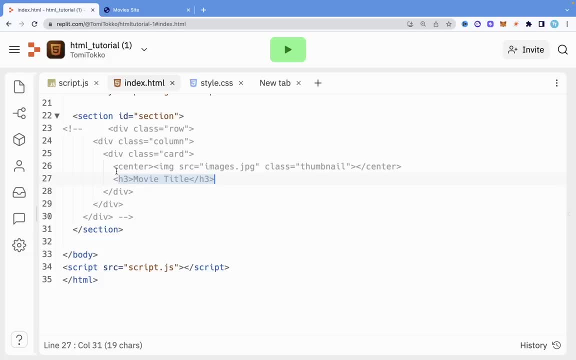 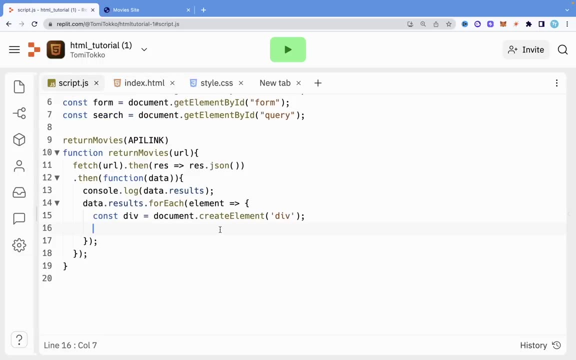 everything. I'm going to show you how I'm going to put this image in the center. I'm going to put this center in this div that has a class of card. so I'm going to show you how we can do that. so what I'm going to do right here- I have div right, what I'm going to do is to say div card, because that's the. 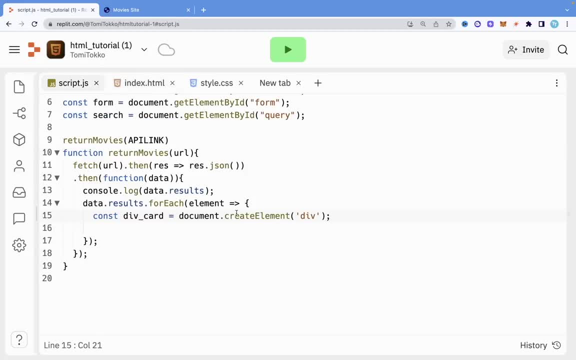 first one: I want to create right here the first div div card and I'm going to say document or create element, div. so you're just creating a div card element. and the next thing I want to do- let me just actually copy this- I want to create the div row. 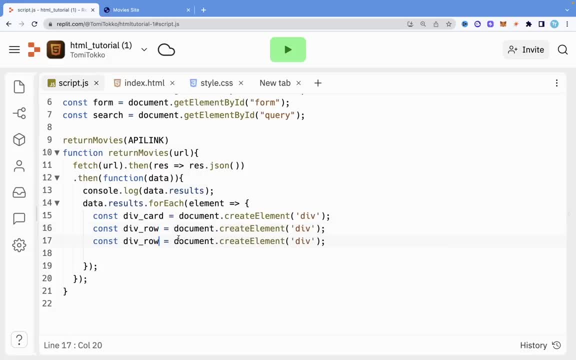 which is also create element div, and I'm going to create the div colon. and the next thing I want to create is for the image. so I'm going to create an image element, so I'm going to create img and I'm going to create the title. so the title right here, which is an h3. 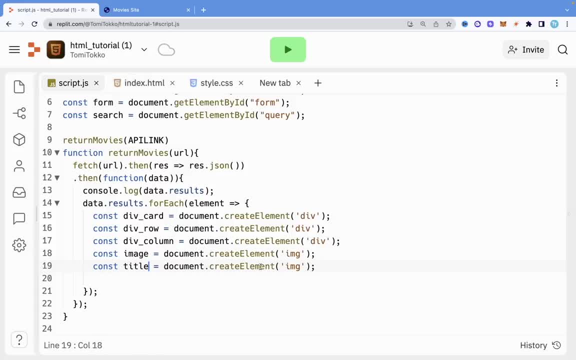 so we have to say title and we're going to create an h3 element and I'm going to create. the last one I'm going to create is: let's see, I think I need to create: yeah, this center run right here now. we're creating every single element. 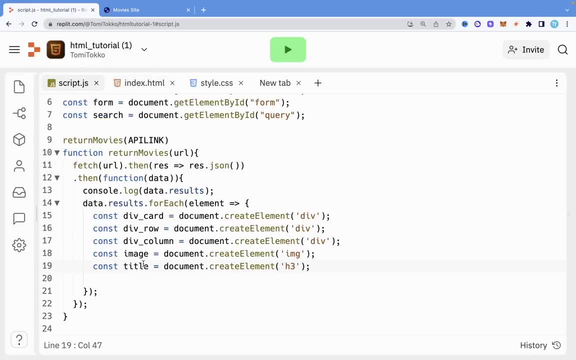 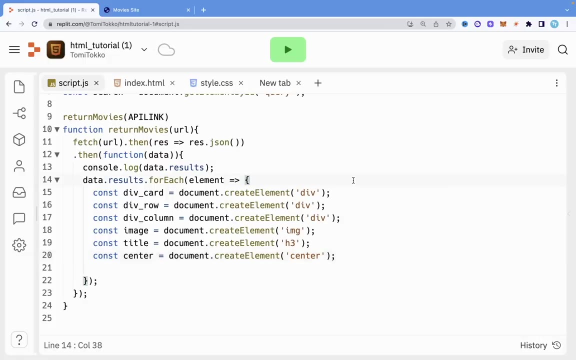 just so. it doesn't, you know, affect the styling. so I'm gonna say, right here, I'm just gonna say center a, create element Center. right now. that should work. now that I've created all this element, what I am going to do is that I am now going to start inputting. 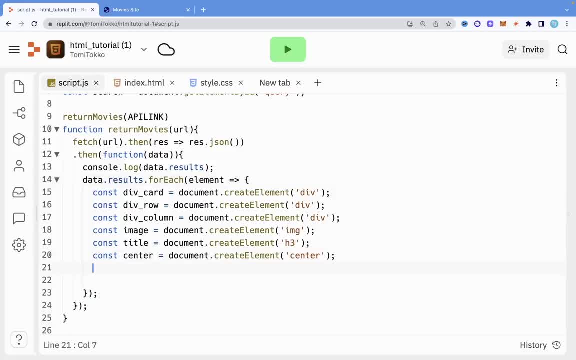 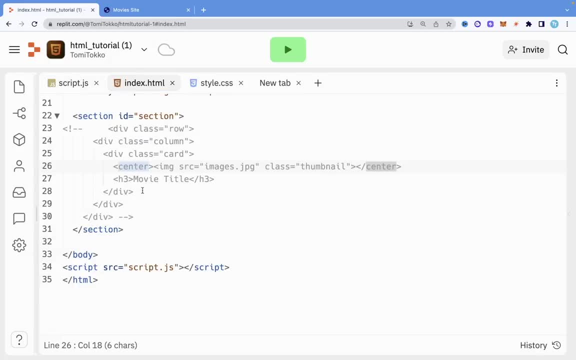 them into each other. so first of all, before I even input anything, what I'm going to do is to say this title. since I know that this title right here is basically showing the movie title right, and I know that this image that I created right here is meant to show the image of that movie, then what I can now do is to say title. 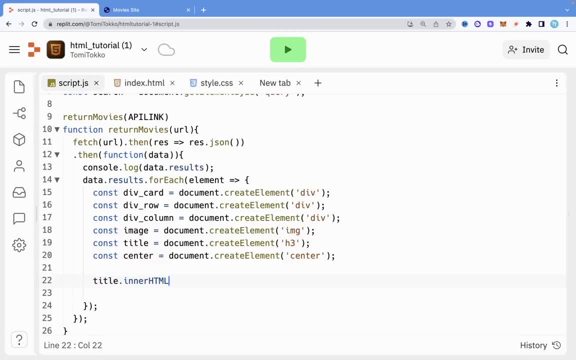 dot inner HTML. so, using inner HTML, I'm gonna say so we're gonna have to use this particular code. the code is the one that we use when we are, you know, giving it a value. in here, this code, So in there, I'm going to use the dollar sign And I'm going to say element. 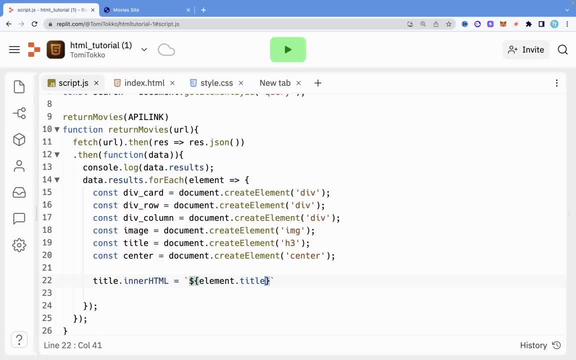 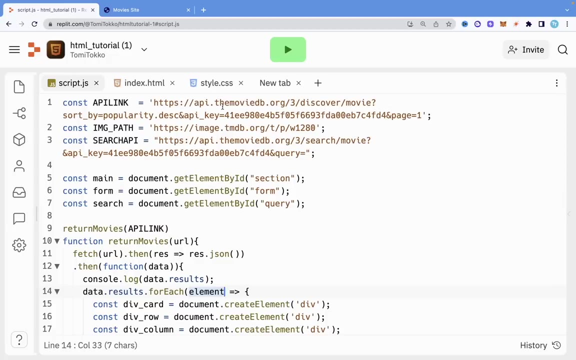 dot title. So this element that we, you know right here, you know we're looping through every single result and I give you this element, So I think, element dot title, And whenever we get a response from this particular API, it saves, it, returns the movie name as title. 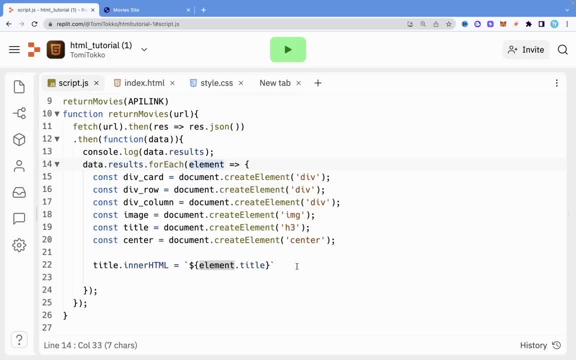 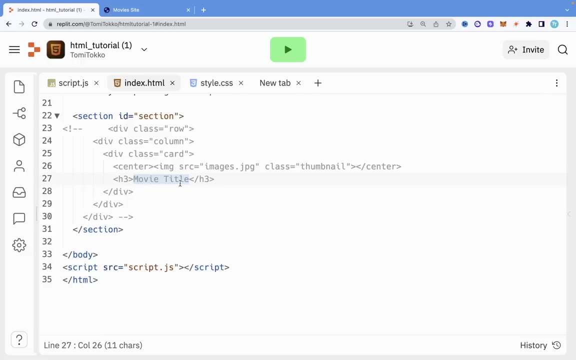 right. So that's why we're using elements dot title, And the next thing that we're going to do is to say image dot, so this image Now we don't. when we say in our HTML, he basically says this value, So we're saying this value should be. you know the title of the, of the. 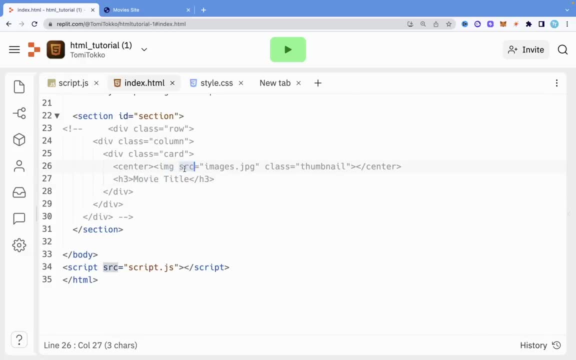 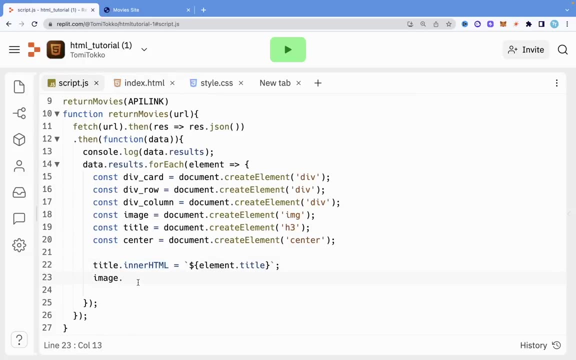 movie. But for this image, we're not giving it a value. what we want to set is the attribute, which is SRC. we want to give the attributes of value. So we're going to say image dot- src. right, I'm going to say equals, to now remember this image part that we created. 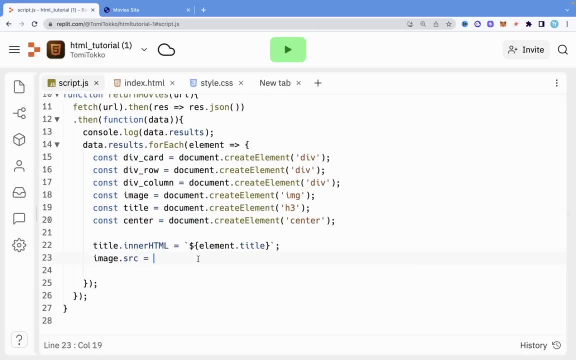 this shows the patch to that image. So I'm going to say image, but plus, now I'm going to say element dot poster. But now what this does is that you know, remember we did element dot title. I said that because it returns the movie name as title And for poster part it returns. 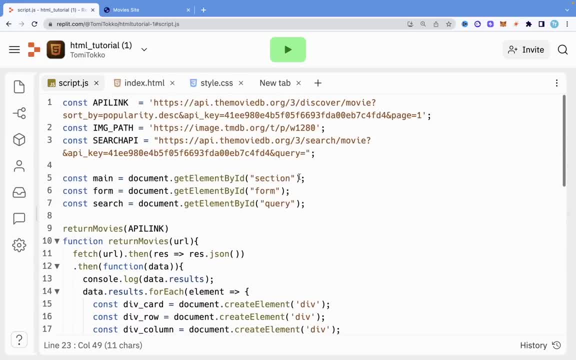 the link to that image as poster part. But we need to add that particular link or that particular one that it returns to this. So imagine it returns. let's say it returns something like you know, six days is slash wherever. imagine does the post up to the URL. we're. 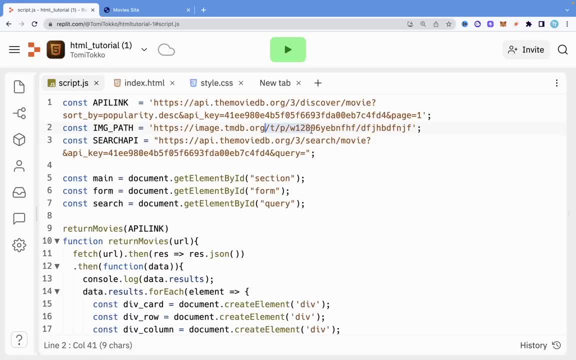 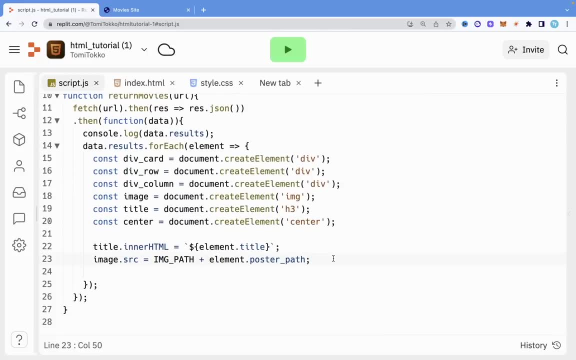 adding it to this route URL. That is why we do so. I'm just going to get rid of that. That is why we do image part, dot element, dot. poster part. So now that we know that we have that, we basically already have what we need, which is the movie name and the image of the movie. So what I 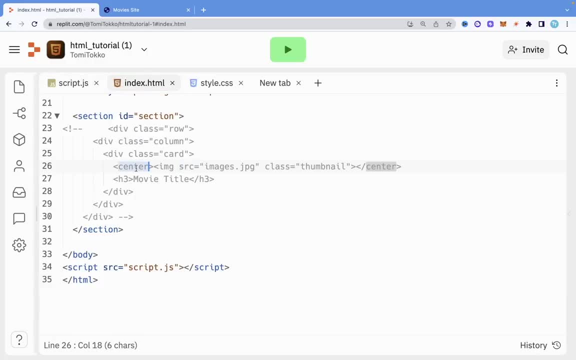 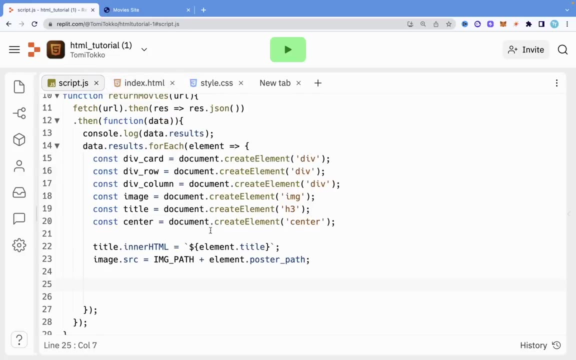 want to do now is I'm going to say this center that we created. I want to add this image tag on that: the center, since it is under the center right here. To do this, I'm going to say center that we created- dot append child. 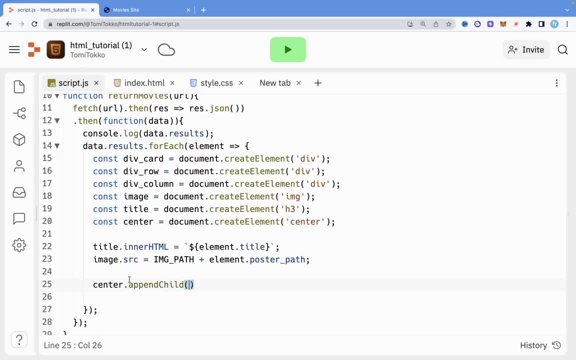 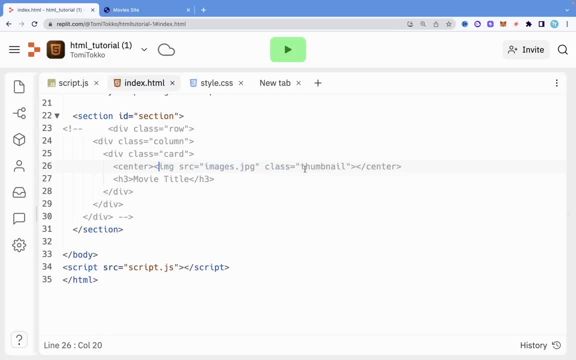 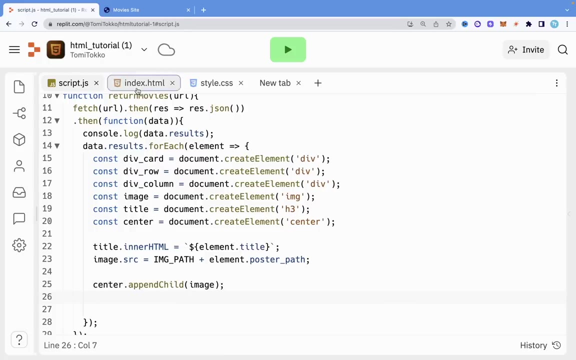 Now, when we say append child, it allows us to add an element on there, another element To sustenance: append image as a child of center. that is true here, because image is actually a child of center. So once I do that, the next thing I want to append by keynote seizure: 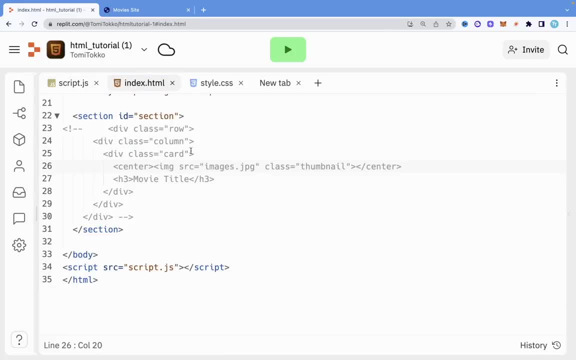 is, I want to append this center now to this card And now we'll append this A3 also to discard. So I'm going to append the center element and the title element. So now, before I'm going to add a selected note on from here to the one I inserted, Let's make sure all 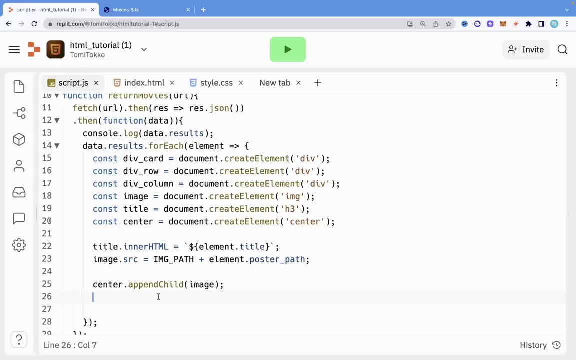 element and the title element. So now I'm going to say: div card right here, dot, append child, And the child I want to append is the center That should be under that. I'm going to do the same thing, But this time around I also want to append its title. Now the next. 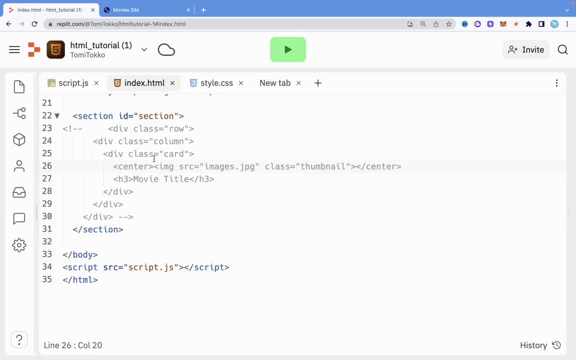 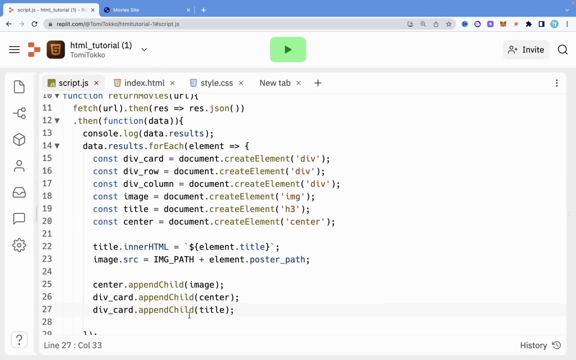 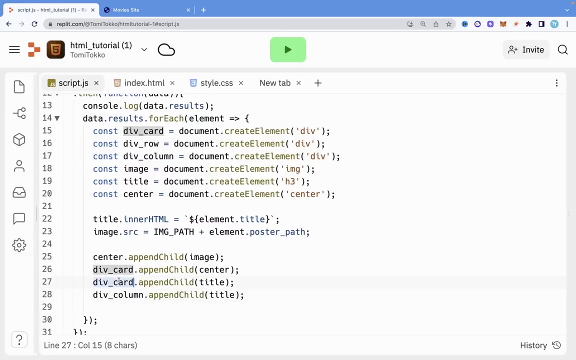 thing I want to append is now this old card div. I want to append it to this colon div And after that I want to append this colon div to this row div. So I'm just going to do that. So I'm going to say div colon. I want to append div card as a child. And now 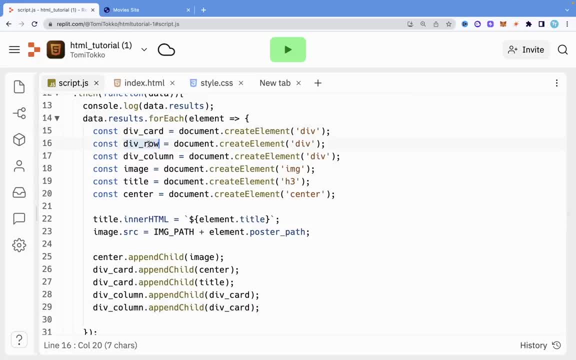 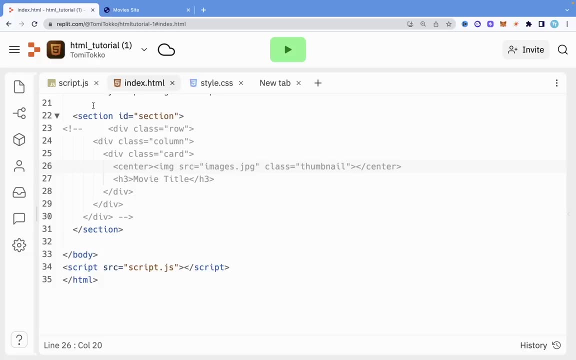 I'm going to do for the last one and I'm going to say div row. I want to append div column as a child. So now, as you can see, we say we first have div row, which is what we have here, And on that we have colon, on that we have card. you can see on that div. 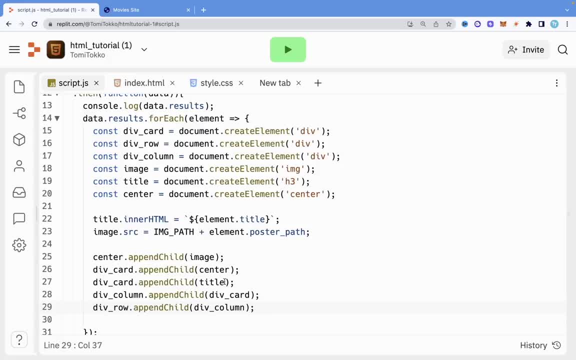 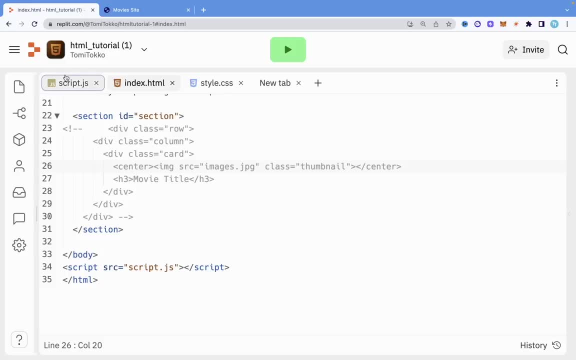 row. we have colon. on that colon we have card. on that card we have title and center. Look, on that card we have title, right and center, And on that center we have the image. As you can see right here, on that center we have the image. But now all of these I 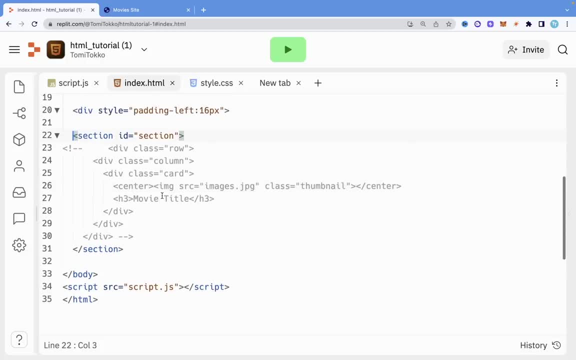 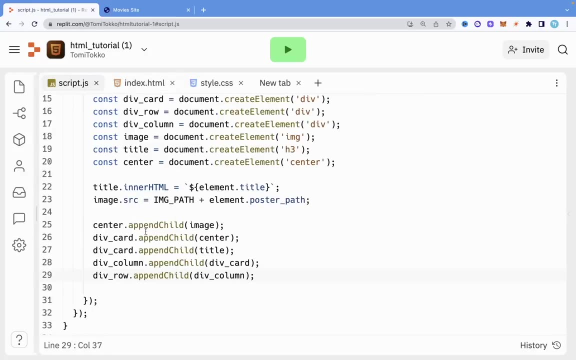 want to add it to this section, this section right here, Because if I just say add, right, is is just going to add it like anyway, once or right now. basically, what I've done is I created this div and I said we should append all of. 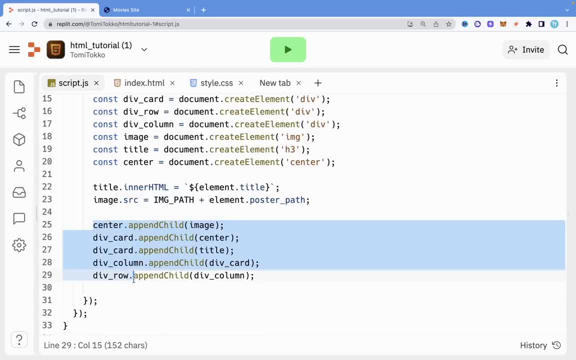 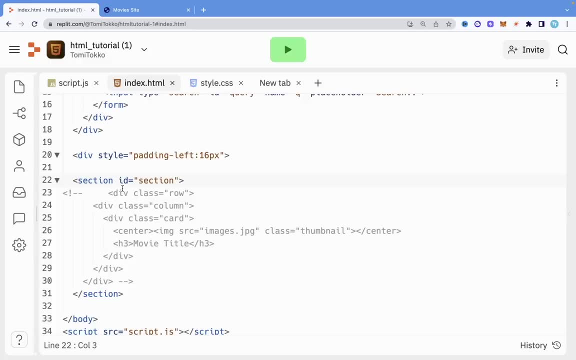 this, But I've not told you where all of these should actually go. So if I say this div row right should go into this section- that is already in here- then what is going to do is: I'm going to take all of this and put it in this section. So I'm just going to do is. 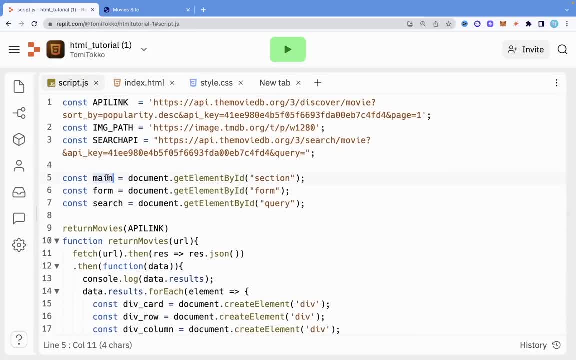 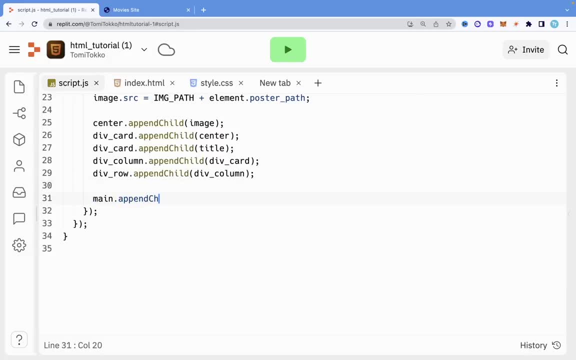 to say think we already got the section Using main, So this main right here. I'm just going to say main dot, append child And once I append div row as a child, that means all of this goes on. that is the div row is. 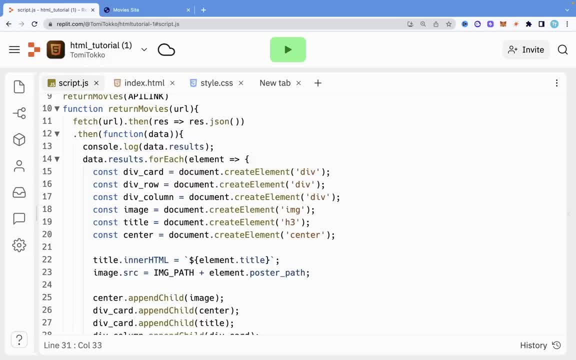 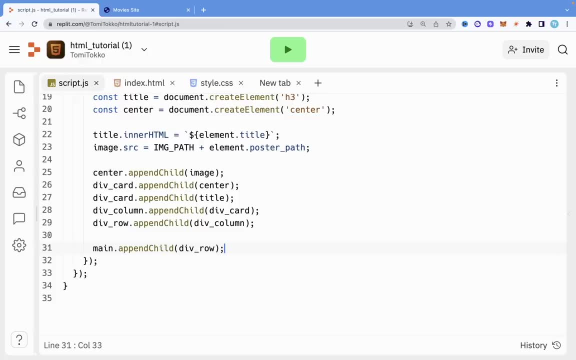 not a child, And that is basically what we want. So all of this should be good And, yeah, I think all of this should be working. The next thing that we want to do is to actually create an event listener. So this event listener. 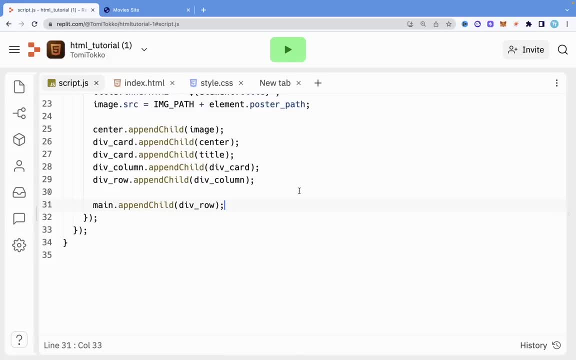 is going to be like for the form, so that when the form is submitted, you know, we know when you submit and I'll get the value of that form, And then you know we call these return movies right here. the way I can just do is to say: 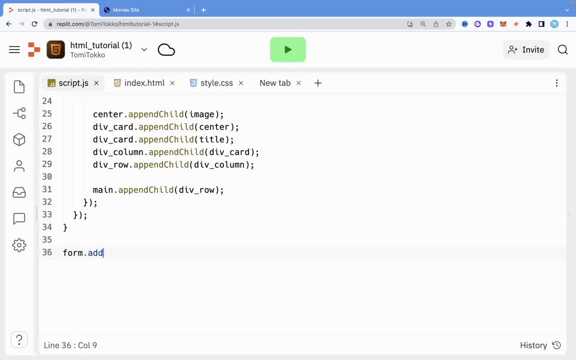 form dot. add event event listener. So I want to listen on submit. So submit is the one for the form S relationship is submitted right, Say E. And then what we can just do is to say let's remove all of. 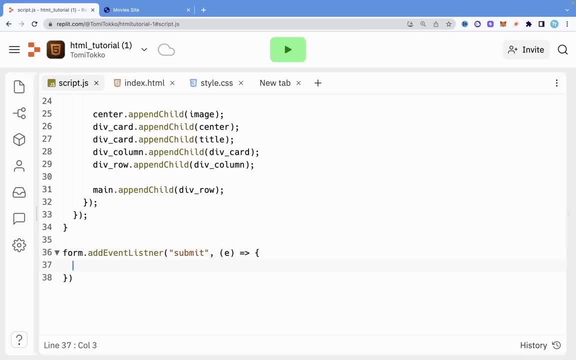 this And just add this and say he does prevent default. So right, here we're going to stop that. And then we're going to say: main dot inner HTML equals blank. Now the reason why we're saying main dot inner HTML equals blank is because when someone searches for like 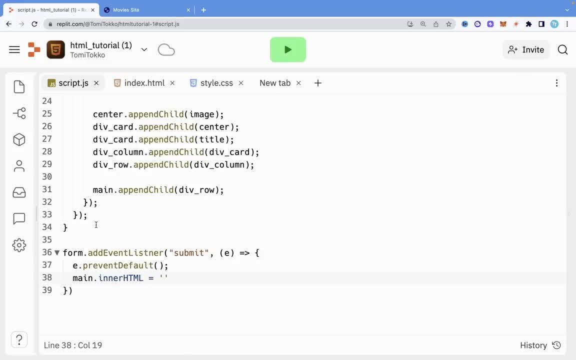 a new query, a new movie. we want to remove all the other movies that were there and replace it with the new movie that is searched for. So this allows us to remove all the movies that were initially there And now we want to replace it. So let's first say: let's get. 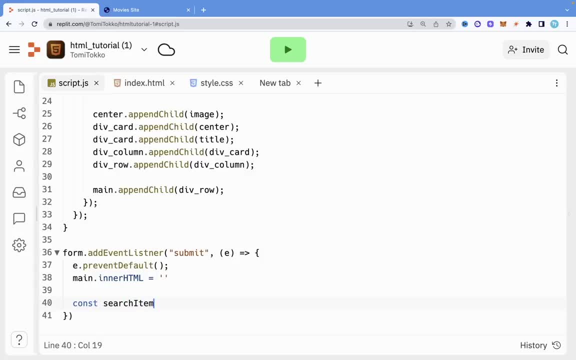 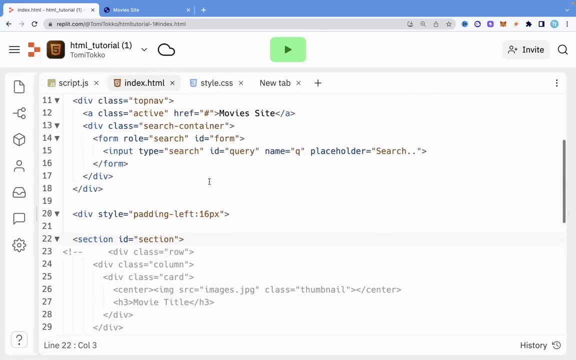 the search item Just to search the value, right? So this is the actual value that user input And this search, remember, is what we got from here, which is the query of this particular, if you come here, of this input. So now that we are getting the value of that search, then 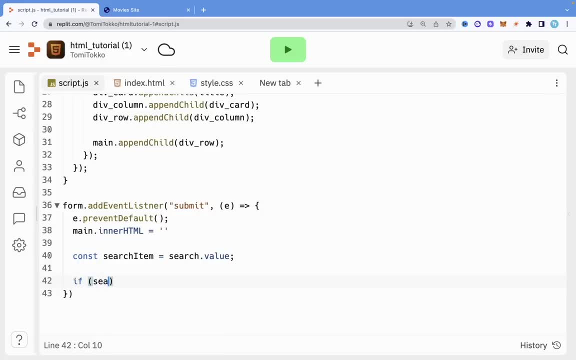 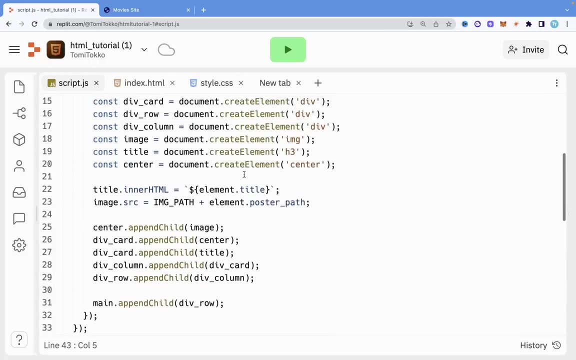 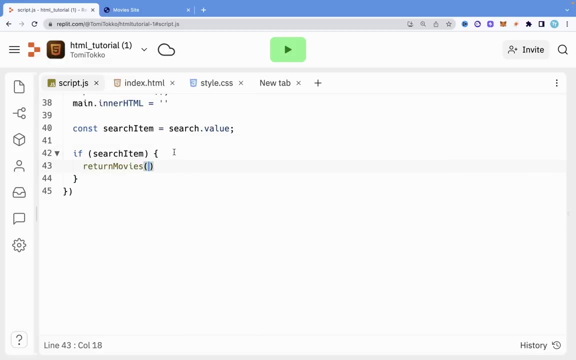 we cannot use stated condition and say if there's actually a search item, like if we actually get a search item, then we want to say we want to call this return movies And we're going to call return movies even it, the search. 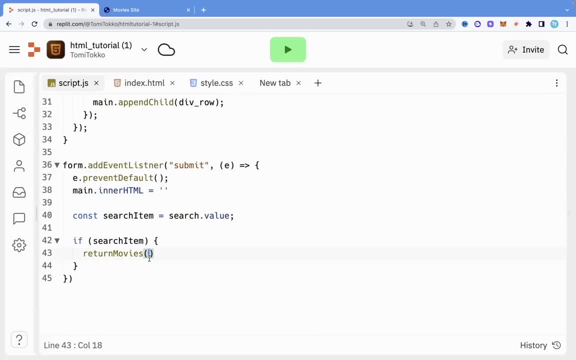 API, plus the search item, Plus this search item that we are passing in here, And after that we just want to clear up that particular input. So search, the value equals clip. What this is doing is that whenever I say someone searches and hits enter, we just want to show the result and clear up what was in there. 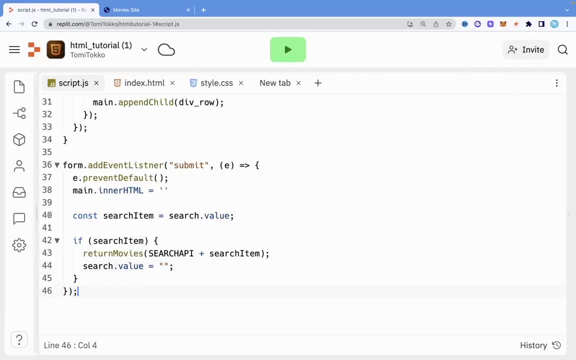 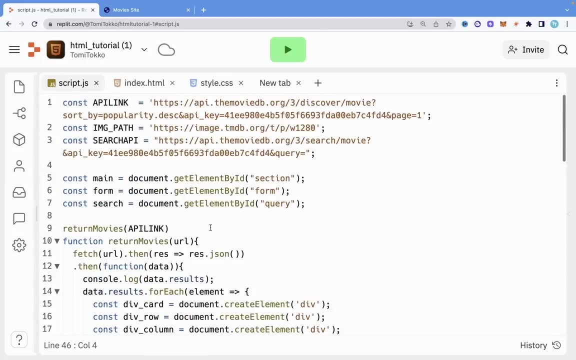 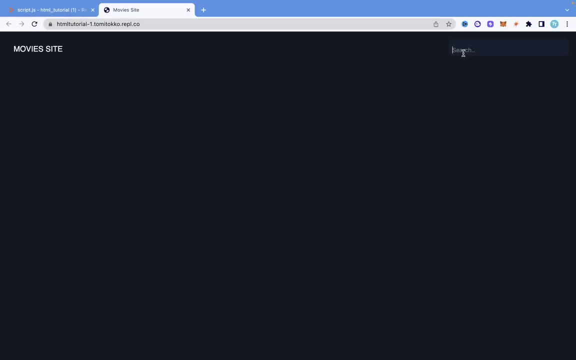 you can add that. you don't need to add that. it's not that important. so we put the semicolon to end that. so, as you can see, all of this should be working now. let's test here and see what we've done till this point. if i hit refresh now, you can see that nothing shows. let me search, let's. 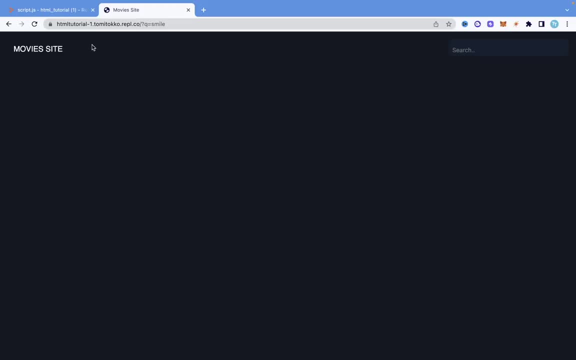 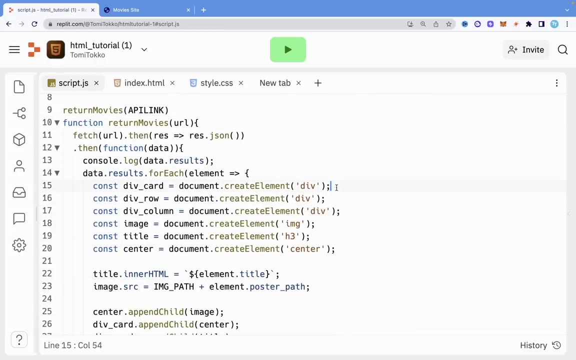 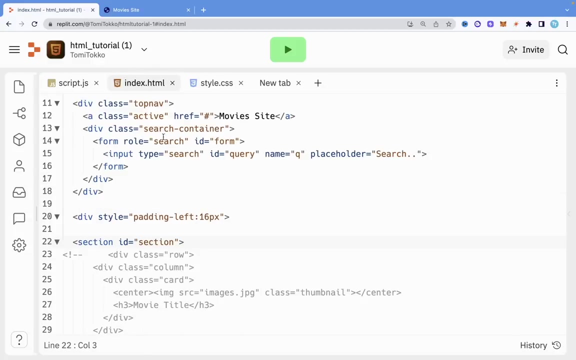 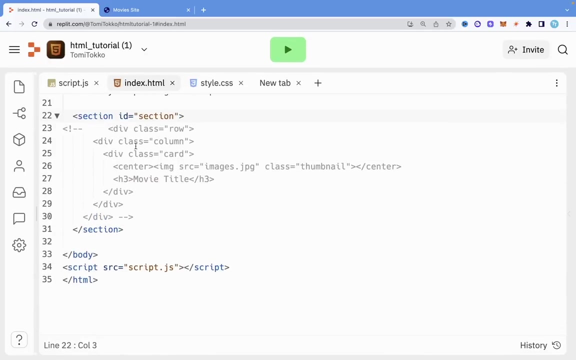 just smile and hit enter: cool, nothing shows. still now, what we need to do is: right here we need to add, let's say, the particular attribute. so what i'm going to do is because in here you can see that this div card. where's the div card if we come here you can see that, for example, 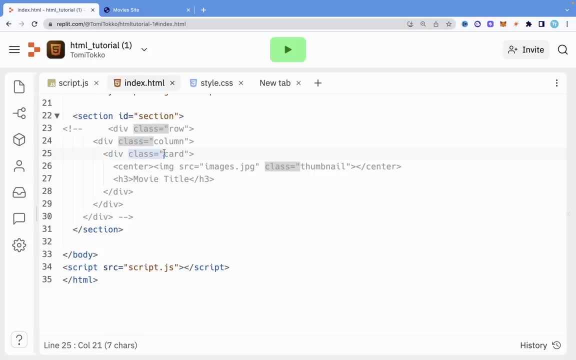 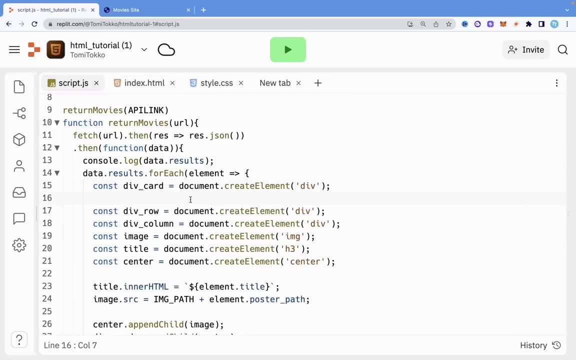 a card. this div has a card. you can see that, for example, a card this div has a card has a class of card. so we actually need to set all these attributes for it. so this div card, we already know that it has a class of card, so we can now say div card. 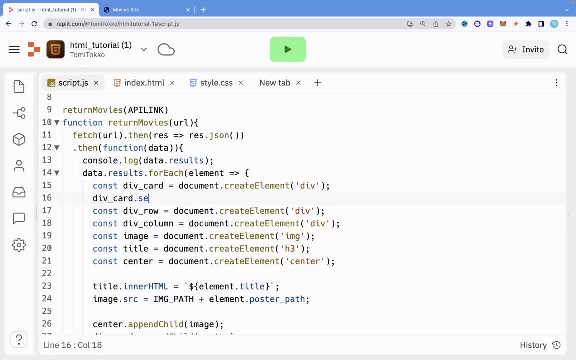 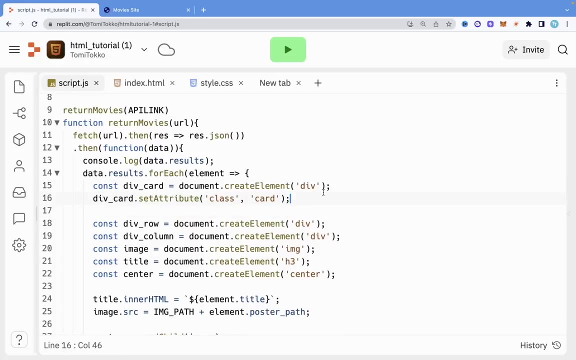 we need to set this attribute when we are creating it out here, say, dot, set attribute. i'm gonna say class, i'm gonna say card. so this is what we need. am i gonna keep doing that for basically all of this, all of them, because all of them has one or two attributes. so we're gonna say: 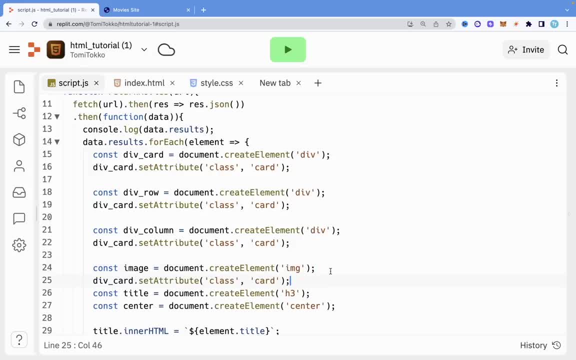 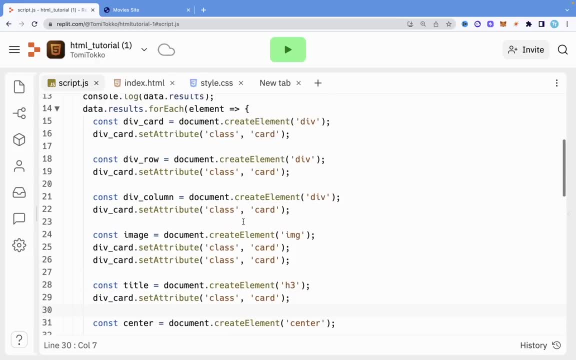 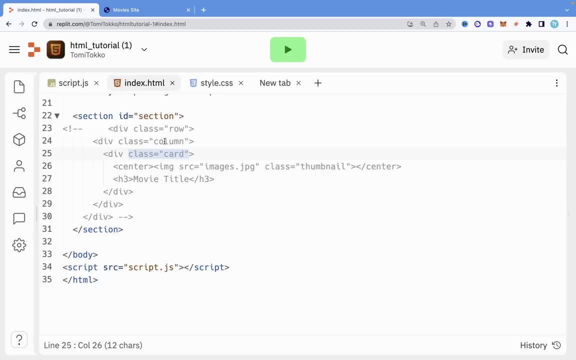 colon and i think the image has two attributes and the title: yes, it has an attribute. also, this center doesn't have an attribute. so now let's check what attribute for row and colon. so row basically has a class of row and colon has a class of colon. so we just let's copy colon. 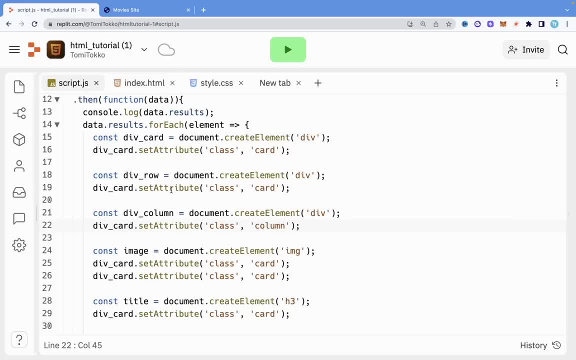 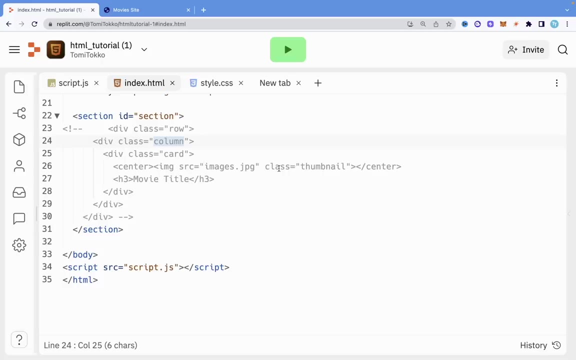 so set a class of colon. and for row and colon, we're going to say row and colon. for row, set a class of row. so div card as a class of card, div row as a class of row and div colon as a class of colon. and for the image we have two different attributes and the attributes we have 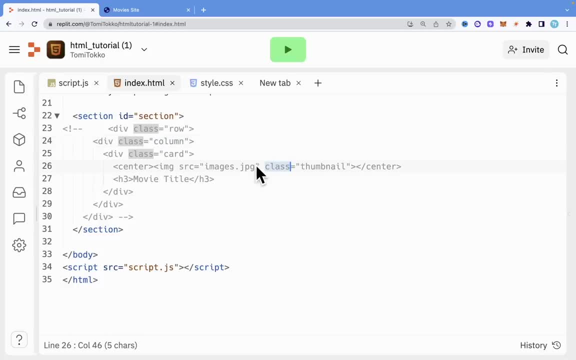 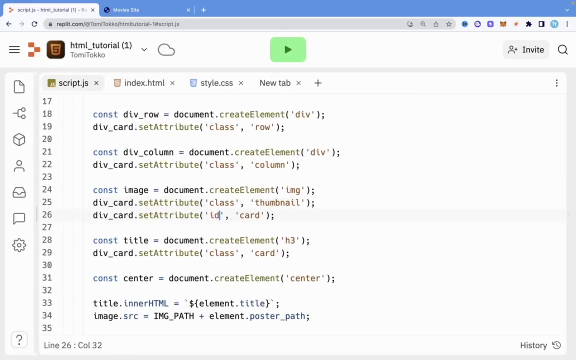 this class. so we need this class and we actually need an id for this image also. so let's see: for image, copy the class. let's say thumbnail. we need an id for this image and let's give it an id of. let's see, let's say image. 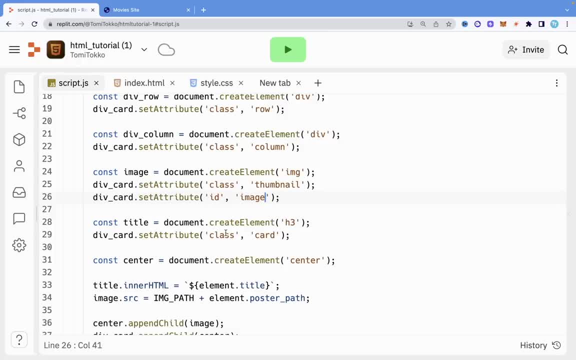 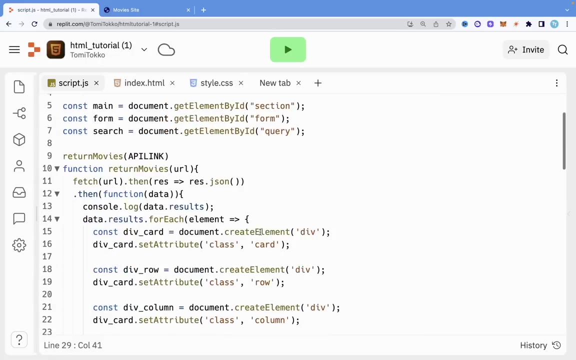 let me give it an id of image for the title. the title just has a id come in here, so we didn't create an id here, but let's give it an id of title now. the reason why i'm giving all of this, this id, is because we we need to get the values of all of this right. so 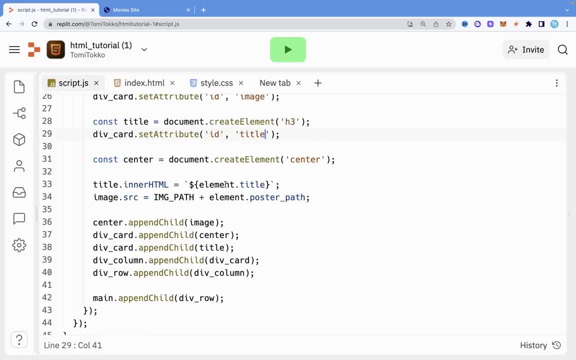 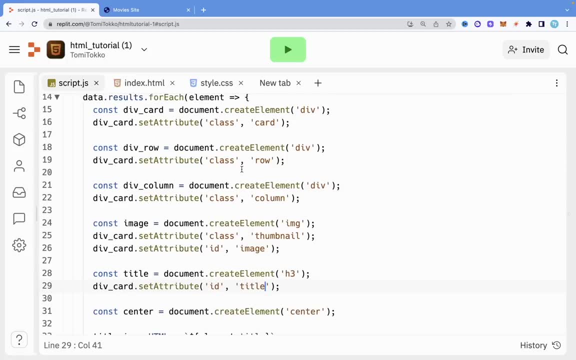 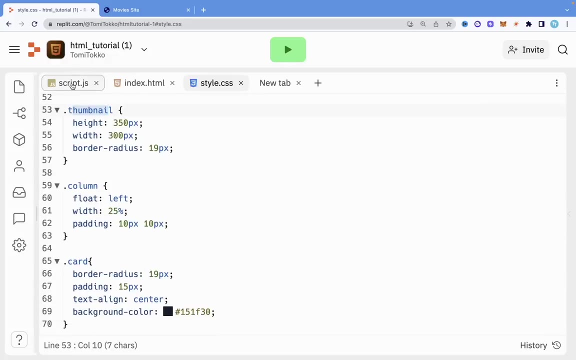 let's see. so we already have title, we have element title, we have image. so we're already giving it these values. and the reason why we're giving it all this id and you know classes and all these attributes is basically because in our css, when we're styling it, we, you know, use the attributes to style them. so 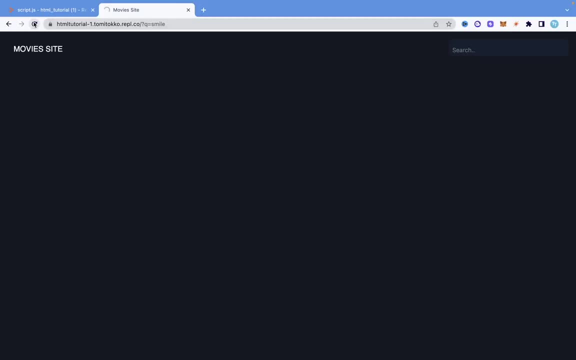 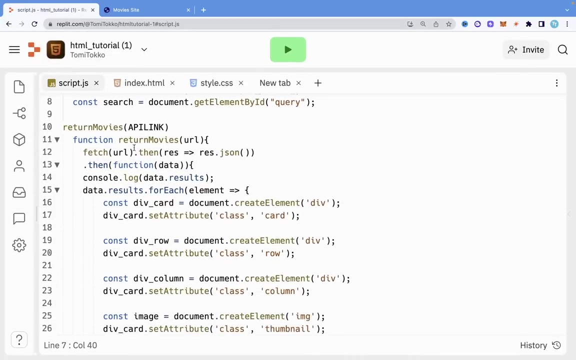 now that we have all of this done, let's see if there's any changes. so if we let's say, as you can see, no result is showing, there's probably some errors in here. so let's see what that is. um, we scroll down to this function. let's see. okay, right here we have two different two. 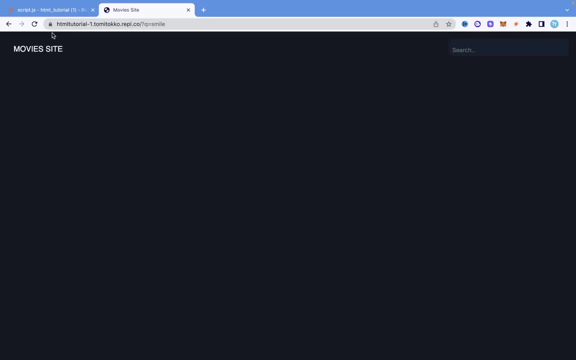 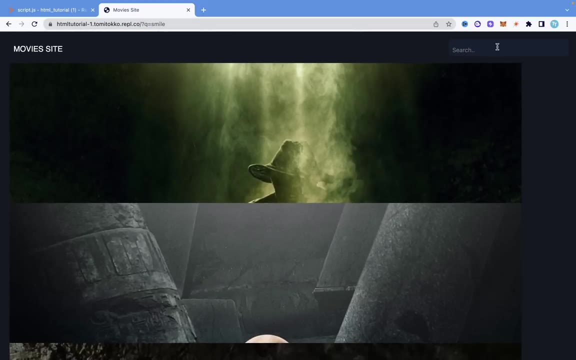 brackets. that should just be one. let's see if that make any difference. does it refresh? oh good, so as you can see, we have some. you know results showing right, so let me see. if i search as a smile, that doesn't change the result. so there is still some errors and this is not the styling that we. 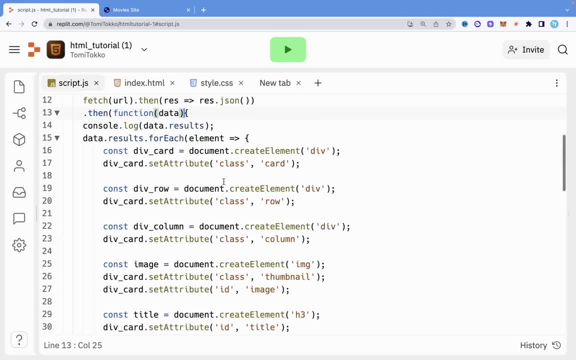 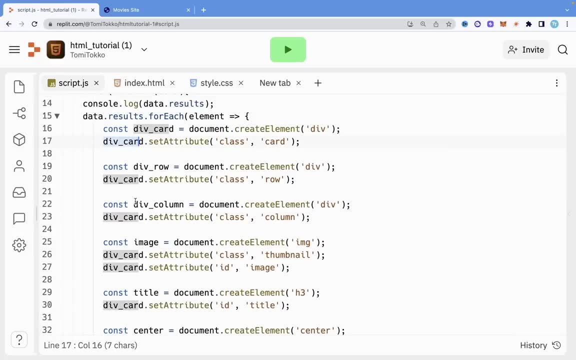 want, so let's go down and try to fix it. so, first of all, for the styling: okay, so you see where we're setting attributes, for here we're setting the attribute for div card right here we should be setting the attribute for div row right here, which is setting the attribute for div colon. 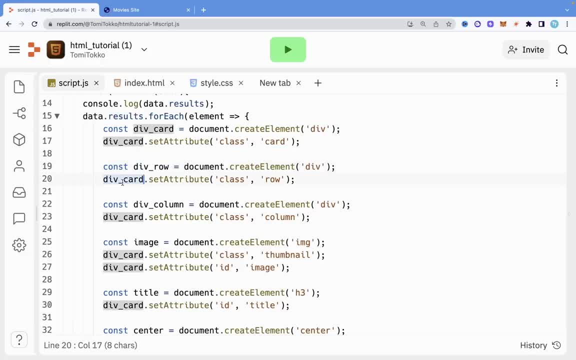 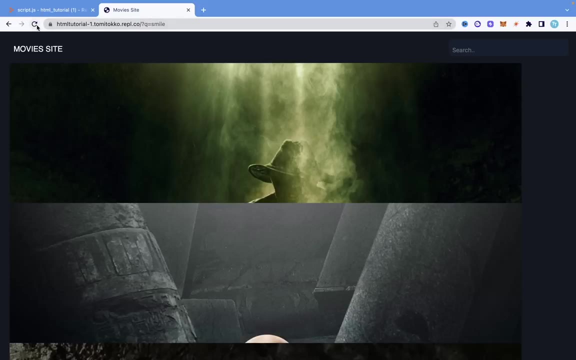 but we are setting all the attributes for div card. so that's where the error is coming from. if we just try to fix that image, the set attribute and then the set attribute and then title and that. so now, if we come back in here and let's just try to refresh this page, 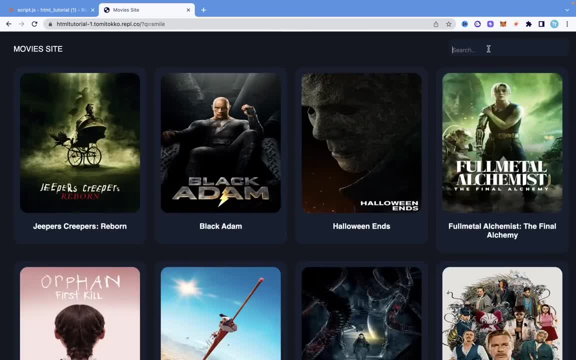 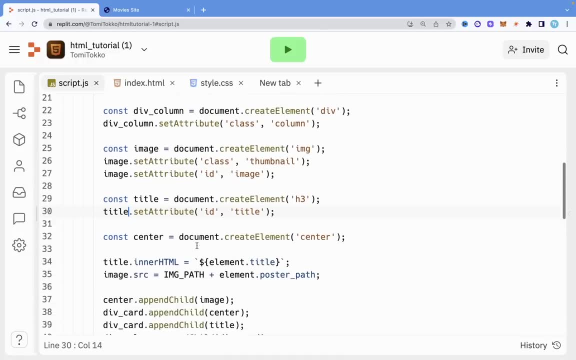 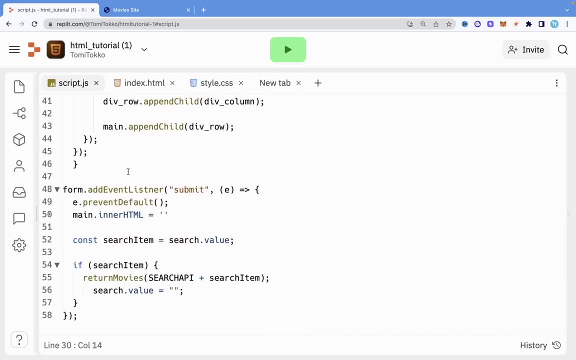 great. so, as you can see, the results are showing. so if i search for smile, let's see, the result doesn't change. that means there's an error somewhere. the error can't be here, because this, this is not where you know that happens. let's see formtxt. 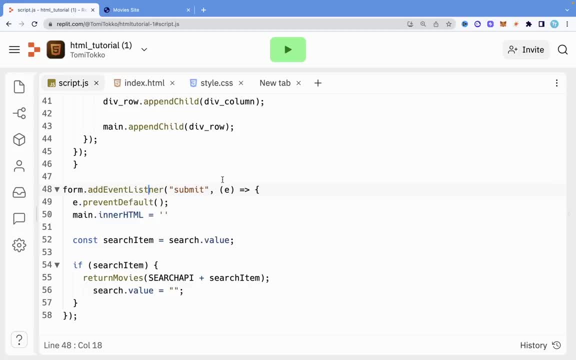 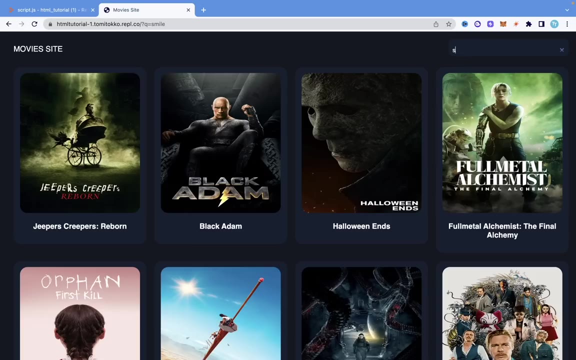 add event. okay, so there is a error in the spelling of listener. so there should be e before n and right here we should have a semicolon. so after all these, our app should be working perfectly. if i come in here now, let me hit refresh, let me search for smile. 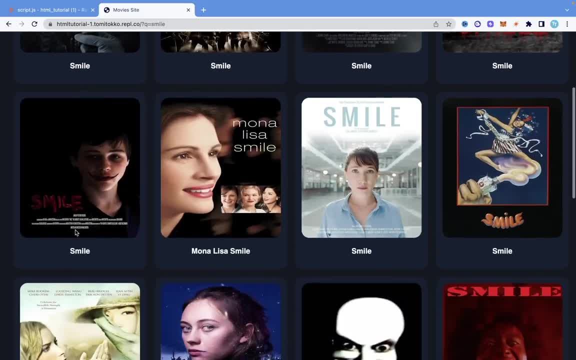 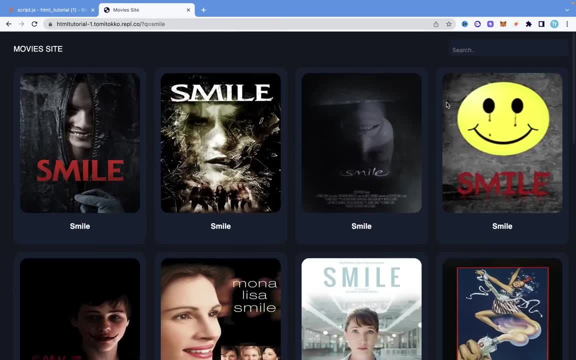 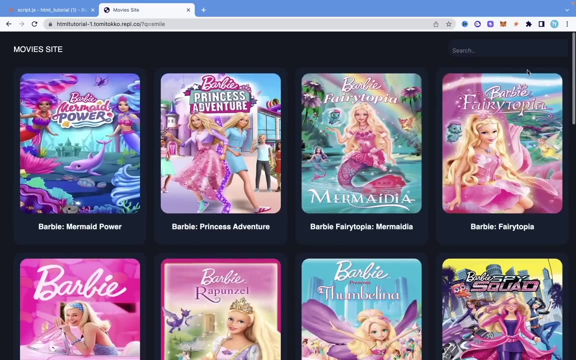 great. so, as you can see, now we have results on smile. we can scroll down to see different results. as you can see, everything is basically working perfectly- gives us a bunch of results on the movie smile. let's say, i search barbie, right, it gives us lots of results on the movie barbie. so that is working. 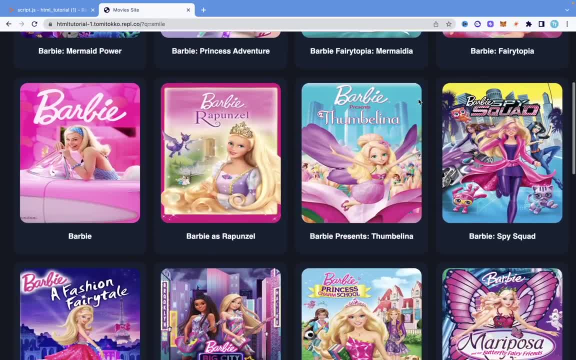 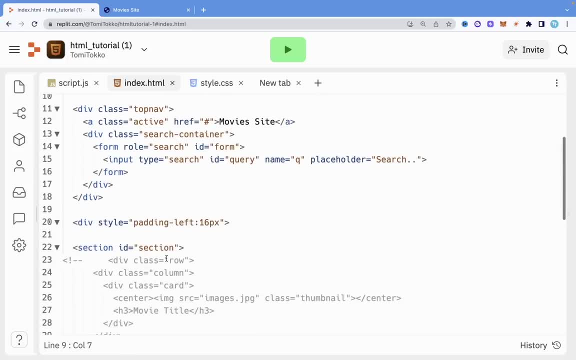 very well, and this is, you know, the basic app that we've built. so let me go through everything that we did. the first thing we did was to style the, you know, create all the elements we need in the html. then we came into the css and styled it, and then we came into javascript and showed you how to you. 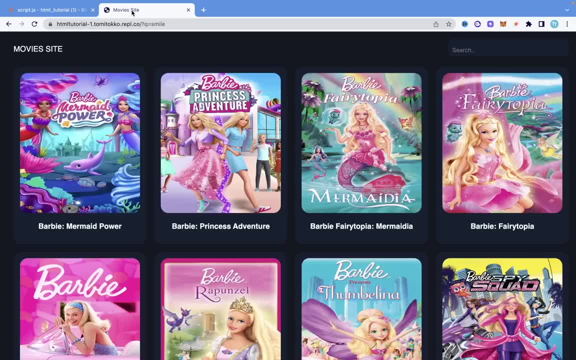 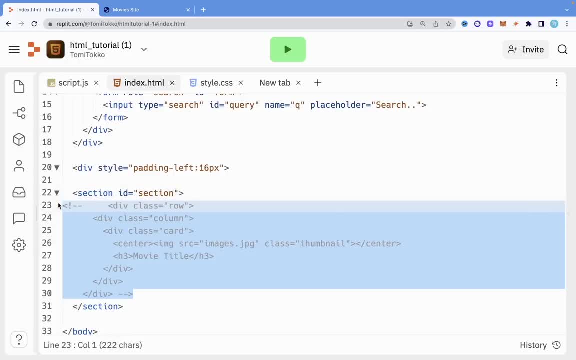 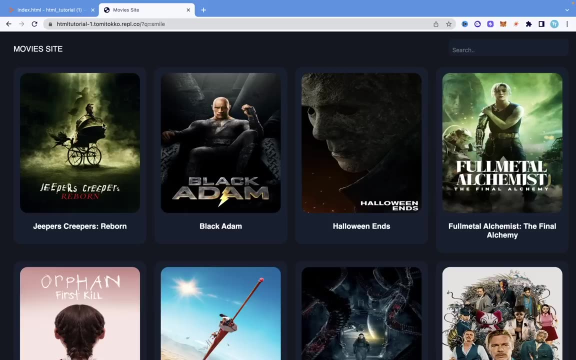 know, get results from the api and use that and show those results on this page so, as you can see, that is working perfectly and right now we can even get rid of this particular you know row if we want. so if i come in here and let's see, i hit refresh, everything is still showing, and let 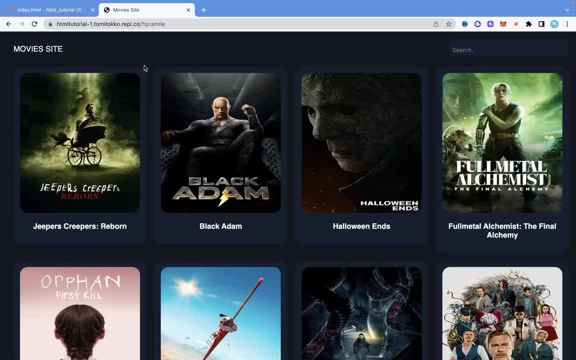 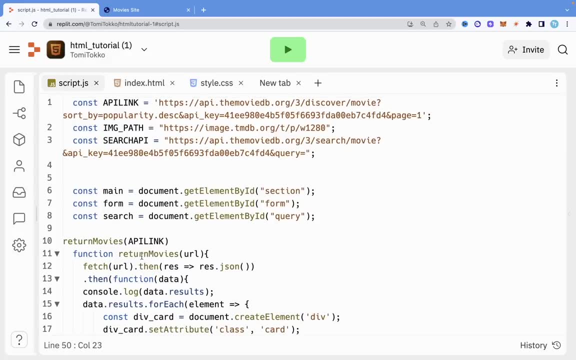 me explain why we, even without searching, we just have some results. so right here where i run. so i'm just gonna go back in here, right here where i run these return movies url and i just use the api link. so what this is doing is that it's just getting all the 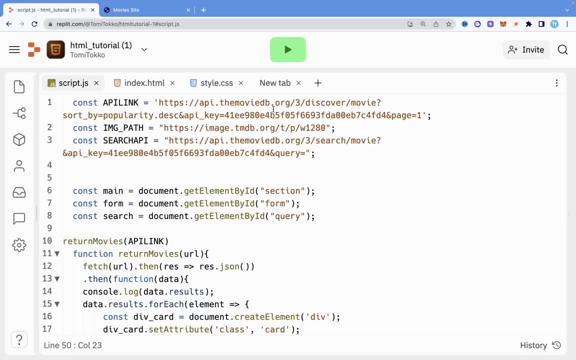 images, i mean, sorry, all the movies on the normal page of this, the movie db website. so, without searching for anything, without filtering, filtering any such, it's just giving you, like, the latest movies on this site. so that's why we see we have some results showing here. but then when you search, 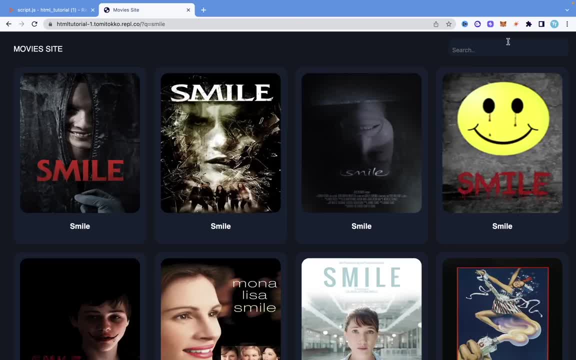 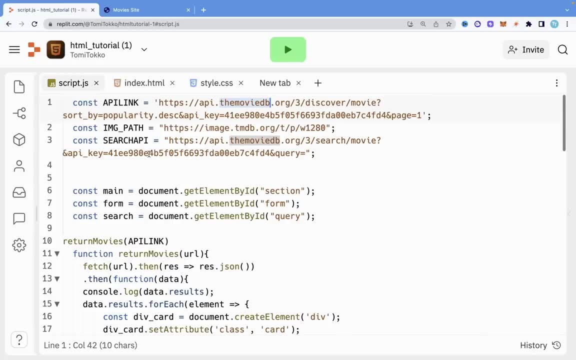 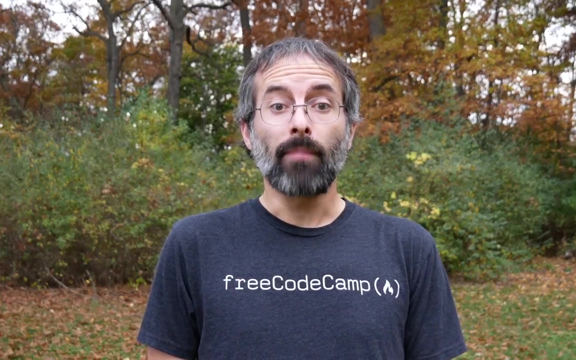 like i said, smile. it then shows some results about what we search. so that is working perfectly and everything is running. so i hope you understood everything that we've done in this tutorial up to date. i'm about to show you how to create a back-end api that can be used to create movie. 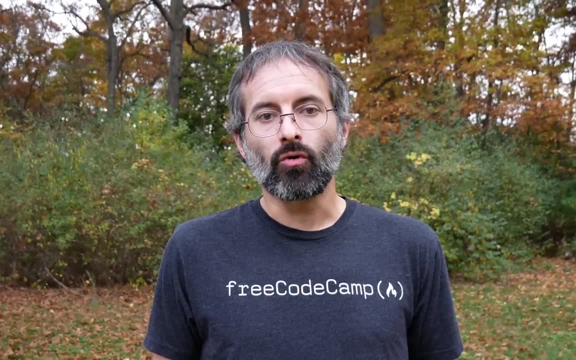 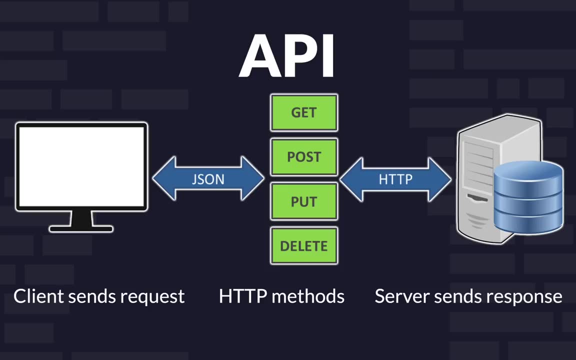 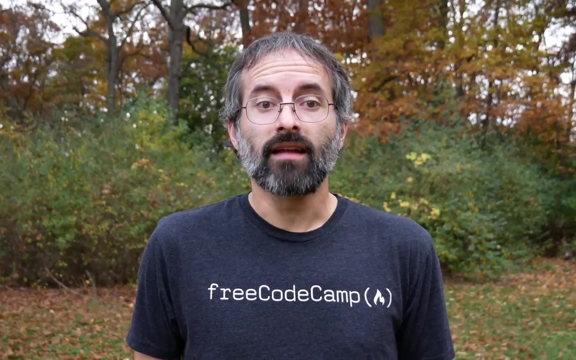 reviews. an api is a way for two or more computer programs to communicate with each other. in our case, we'll use url endpoints that can be used to interact with the database. this is more advanced than the beginning javascript project, but don't worry if you don't understand everything at first. 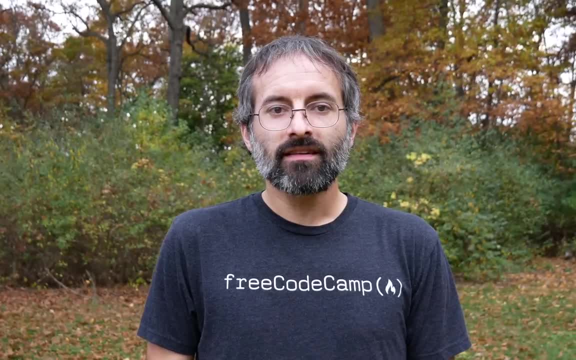 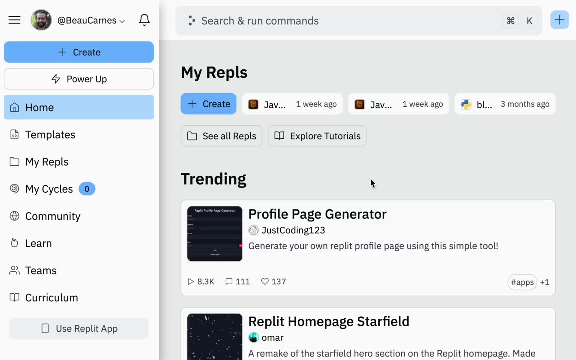 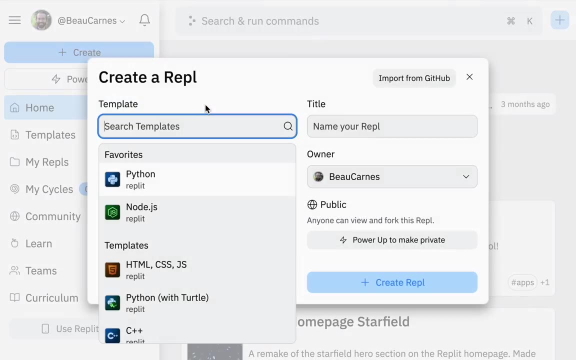 i recommend following along on your own and you'll eventually see how everything's comes together. so let's create the back end api that will use to create, read, update and delete movie reviews. i'm on replicom and i'm going to create a new replant. 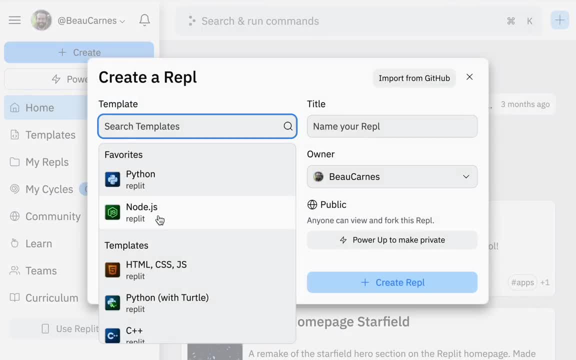 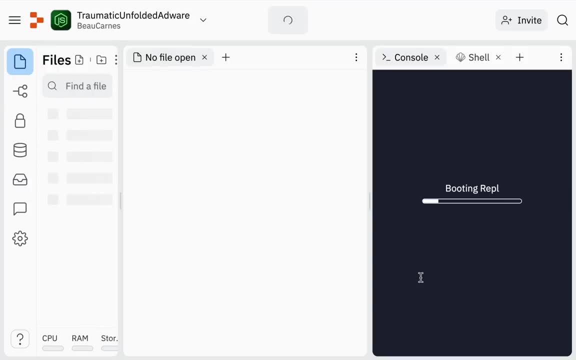 and we're going to create a nodejs replant to write javascript for the backend. so i'll just do create rebel, and now i'll just. I could have created the name when I was creating it, but I can also update the name here, So we. 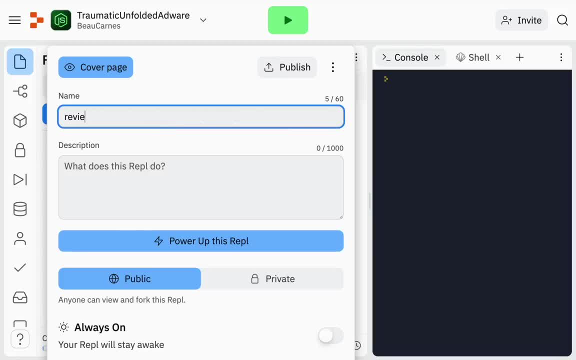 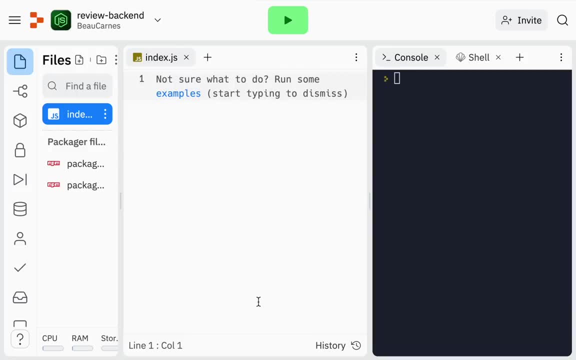 have the default name, but I can just type in review Backend. Okay, That's a good name. So one good thing about replet is that we don't really have to do npm install anything, because when you run your code, anything that you've imported, it will automatically install for you. 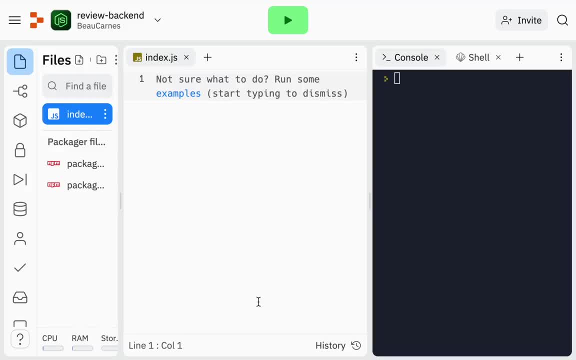 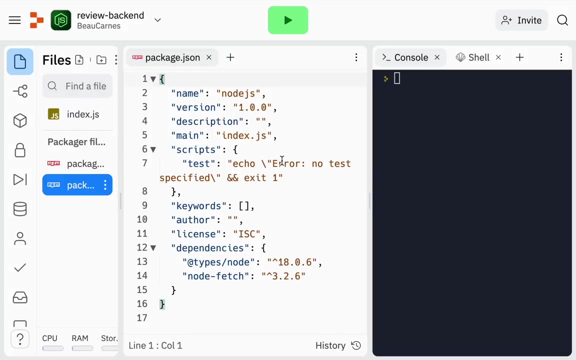 But one thing we're going to do, we're actually going to be using import statements from ES six And with node js that's not. that's not done by default. So we have to go into our package that JSON. Now, if you, if you're doing this locally, you could do the same thing Once. 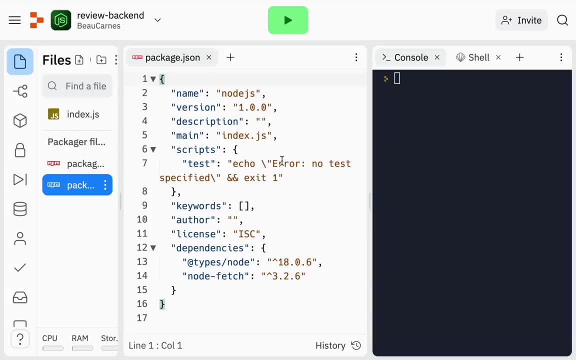 you initialize your, your project with npm init, it will create a package that JSON- but we're doing it automatically- is created on replet. So what I'm going to do is you, right after main, I'm going to add type input module. This will allow us to use import. 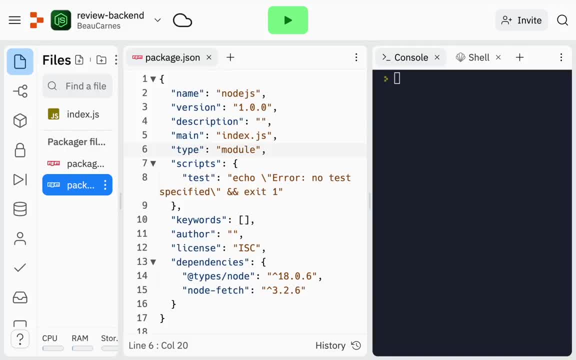 statements, which I will be talking about more later- And I like how there's two others two spaces here. everything's indented twice. Well, let's make that the default is currently not the default, So I'm going to go to indent size and go to two. Okay, now I am going to open my indexj. 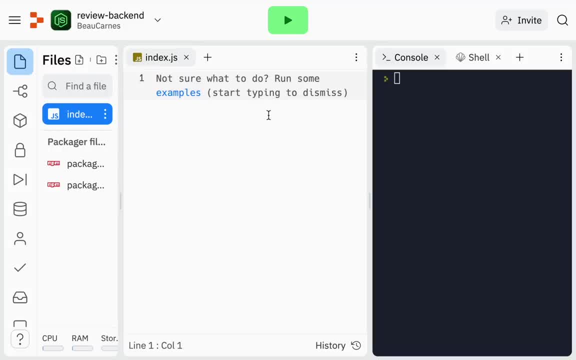 And we're going to create the back end server. we're going to separate our main server code from the code that is accessing the database, And all the routes will be in separate files. Now, we could do this all in one file, especially since we're doing a pretty basic app, But when you create a 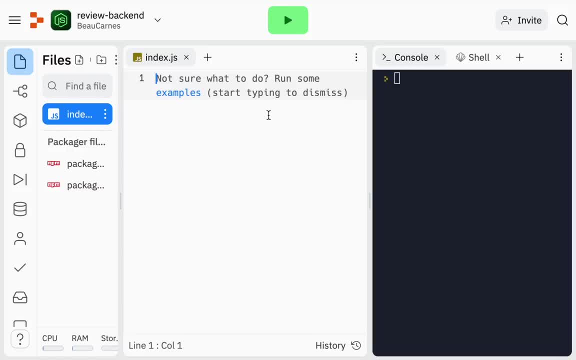 much larger application. you really want to have separation of concerns between your different files, So we're going to use some best practices for how to do that. So we're going to use this standard background file here. So we're going to create a backup link and then, if we want to do, an入f, or or we're going to use a boot, we're going to use a backup link in the backup link that we have in control, But first of all you're going to want to do a backup link to this And 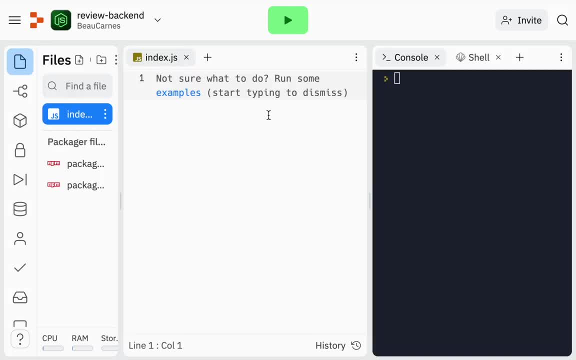 we're going to have the backup link And now we're going to want to only use a backup link: practices for how to separate different parts of your code And that will allow you to see how you can access code from one file in another file, And eventually we will be using indexjs. But 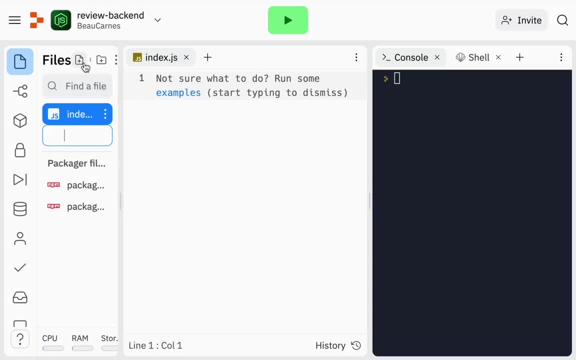 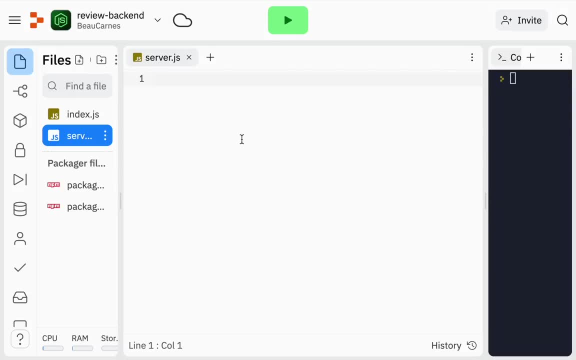 actually we're going to first create a another file called serverjs, So click new file, serverjs- And I am going to make this a little smaller because we're gonna be focusing on the code for now- And in this server file we're going to create an Express server. attach the cores and. 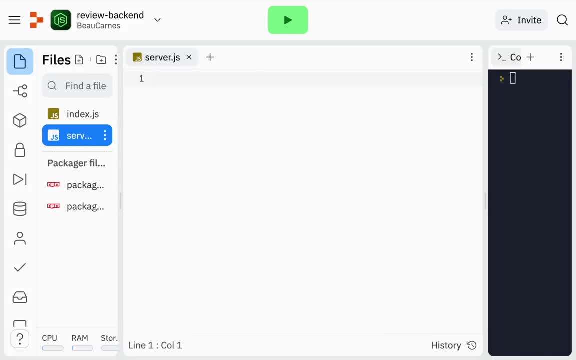 Express, that JSON middleware, since we'll be sending and receiving JSON and make the server listen on port 5000.. So let me explain a few of those things before I start typing some code here. But we're going to be using Express, which is a lot of fast and lightweight web framework for no. 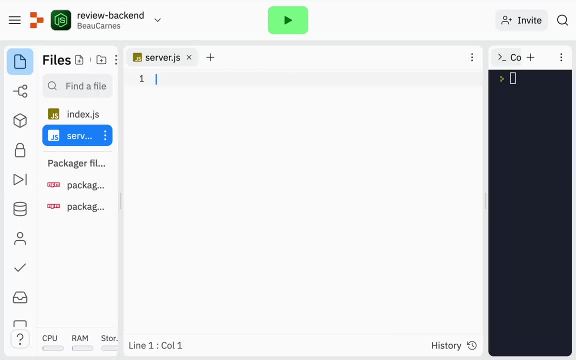 JS And it makes it easier to make HTTP endpoints that we can use for our web server. And then we're also going to be using cores, And then we're also going to be using core. So we're going to be using cores, And then we're also going to be using cores, And then we're also going to be using cores. 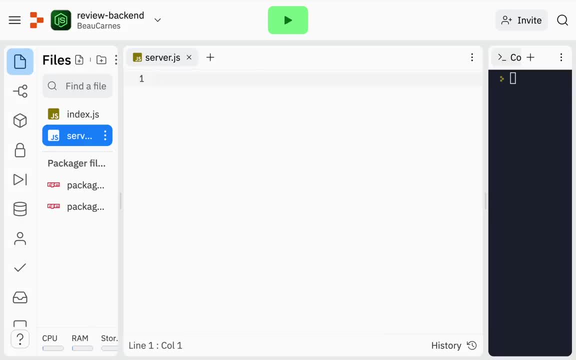 That's the cross origin resource sharing, which allows Ajax request to skip the same origin policy and access resources from remote hosts. Basically, it will prevent some errors when we're trying to access our database from a different host as our server, And the course package provides an Express middleware that can be used to enable cores. 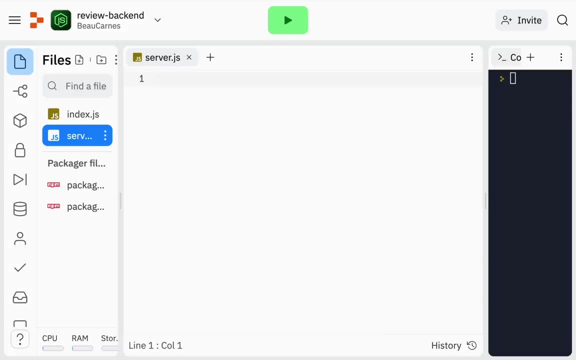 with different options. Now, if a lot of this that doesn't make sense, don't worry about it. just fall along And a lot of things will start to make sense as we go. So I said we're going to be using Express, So I'll do import Express from Express. So normally, if you're doing this locally, 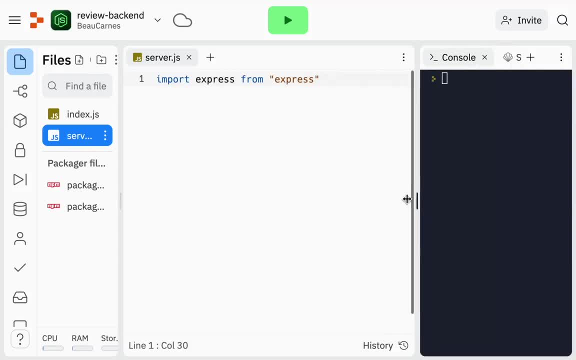 you would have to do npm, you would have to go. well, let me just show you how you do that locally. we in replica, we have a shell And I can clear that, And I could do npm, install Express, And that's how you would do it locally And I could do it on replica. 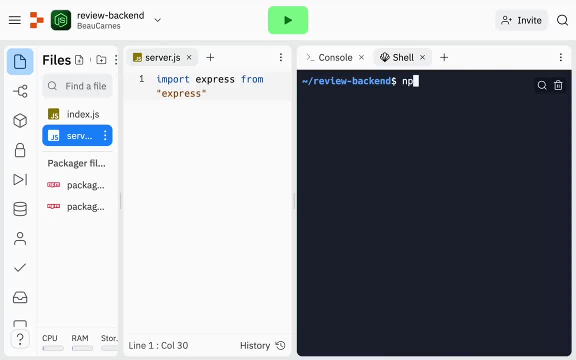 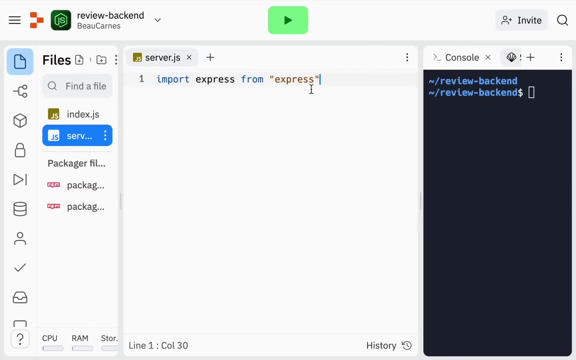 also. but it's going to automatically install Express when we press this play button to run our program, So we don't need to install manually. So what? so it's going to be looking for the Express that's been installed and it's going to install into our node modules directory. 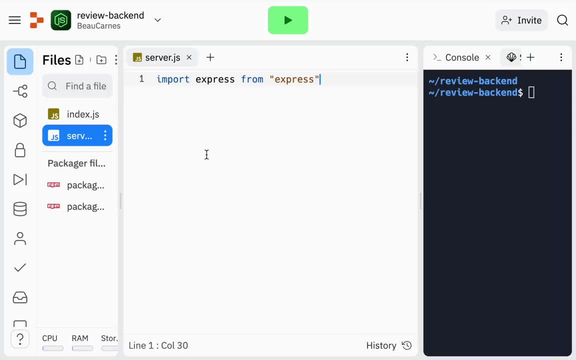 That's one great thing. But JavaScript is there, there's tons of extra frameworks and there's tons of frameworks and code that has already been written And you can just import that code And then you, David, don't have to write things from scratch, And it makes it. it makes it much easier to write programs. 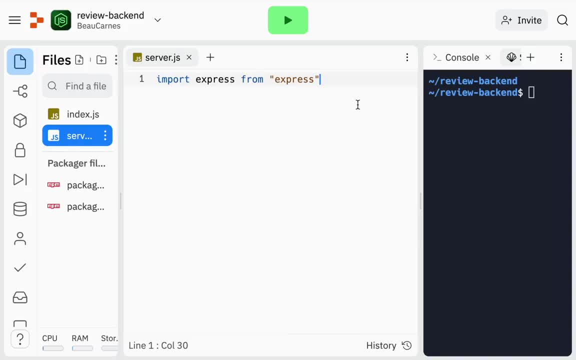 in JavaScript to use code that someone else has already written. So Express is just one of those popular JavaScript packages or a set of JavaScript code that we can use to make creating our JavaScript program a lot easier. And then we're also going to import cores, like I said, and we'll 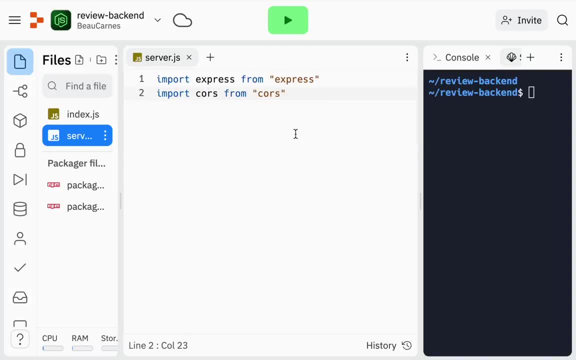 do from cores, And this is something else that will be installed automatically into our node modules directory when we run a program. Like I said, that helps with the cross origin resource sharing. If you've done other web development, you'll probably be familiar with that, And if 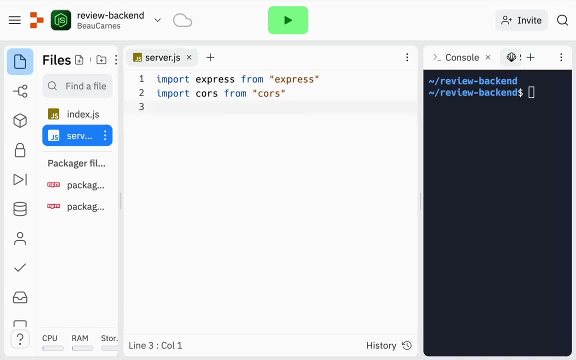 you haven't. you're going to get familiar with it soon And we're also going to now import a file that we are going to create. So these first two things we're not creating. it'll just be imported. But now we're going to import a file that we're going to create, So we're going to import the file. 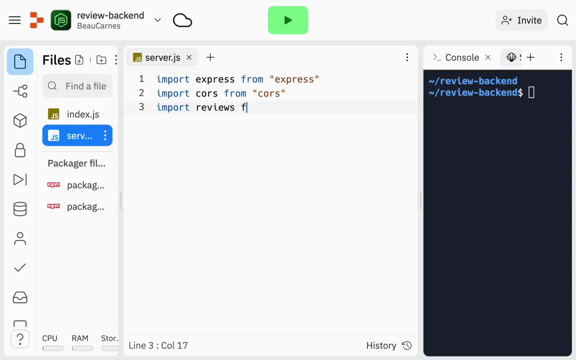 reviews From. Well, that's not the name of the file. That's the name of what we're going to export from this file, And the file URL is just API slash reviews dot route dot j s. So we are going to have our URL routes. 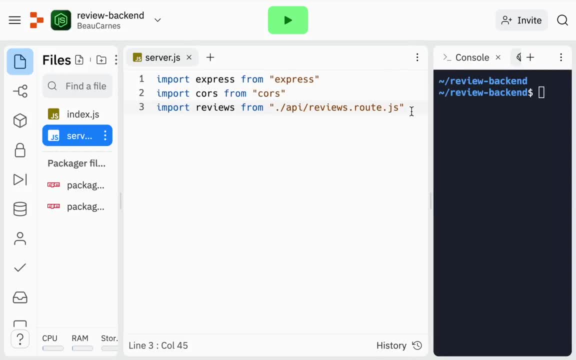 separate from our main server file, And now we have to get access to Express app, const app. that's a variable that we're just going to load Express into And this is what we'll be using to create our code, And then we're going to import our code. And then we're going to import our code. 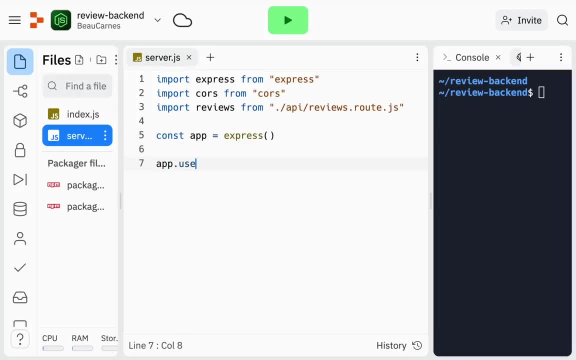 our web server. Now we can do app dot use. Now this is how we can use middleware. middleware are just different, basically programs that Express is going to use to change how things work. So we're going to first do cores that we've already imported And then we're going to app dot use. 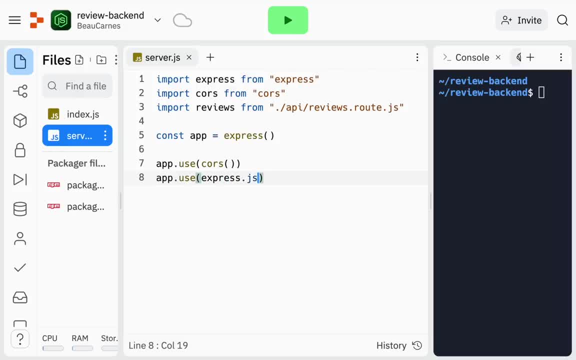 Express dot JSON, So what this one is. this will allow our server to accept JSON in the body of a request. So if somebody sends a get request or post request to our server, it'll be able to read JSON. So requests are when you go. 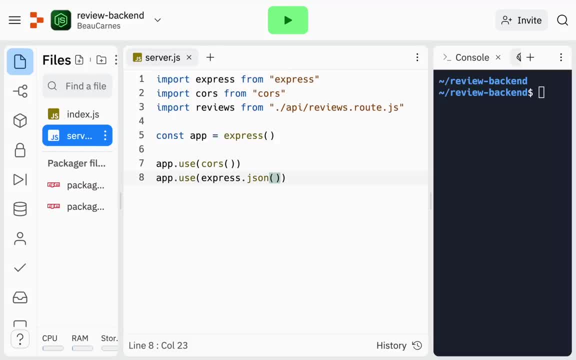 to a website that there's a get request to get the information from the website, or you can do a post request to send information to the reg, to the URL, And now we'll be able to send and receive JSON because we're using this middleware. just add some extra features to our. 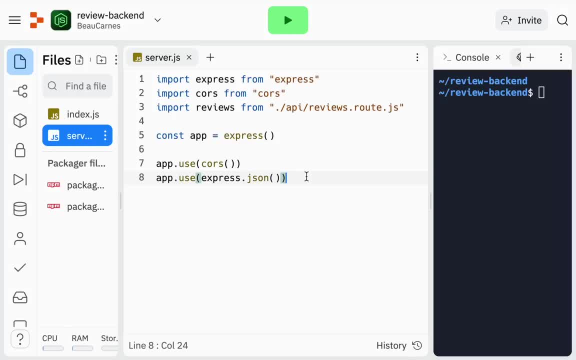 our web server that we're creating. Okay, now let's specify some of the initial routes. So the initial routes are basically the URL that you access to get to send and receive information. So we'll do app, dot use And then we'll pass in the basically the URL, And so it's going to be. 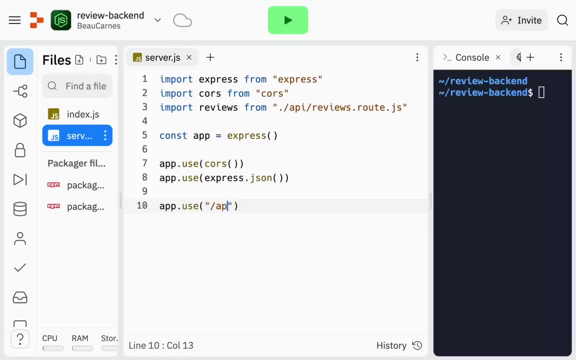 that we have a root URL and then it's going to be slash API, slash v one, slash review: choose. Now. this is just that we can use any URL here, But this is best practice When we are creating an API. it's often you often want to specify that it's an API And then often it's. 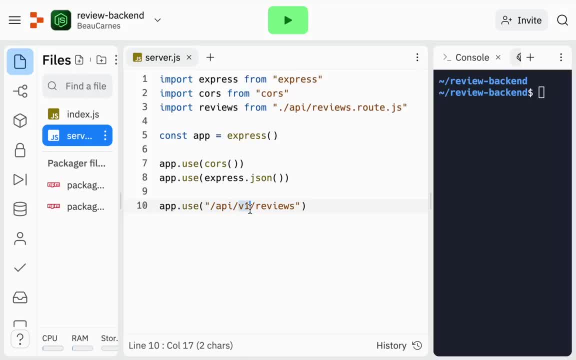 good to have versions of the API, just in case, in the future, you create a new version. Now, this is just like a demo app, So we know there's never going to be a version two, but it's good to start learning the best practices now And we for this URL. we are going to use the routes from the. 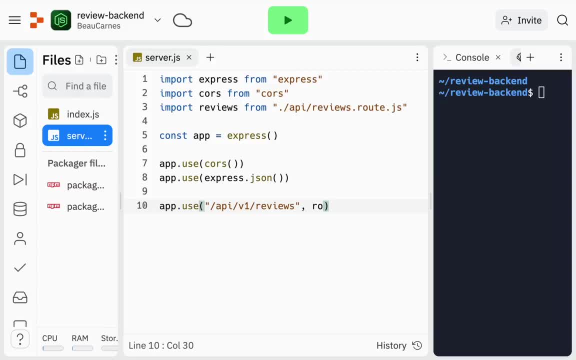 file. So I'm just going to put a comma here And then I'll put reviews. Okay, so now we're going to use the routes that we set to create later, But this is showing that for this URL we're using that route. Okay, now we're going to create just the backup route If someone goes to a URL. that's. 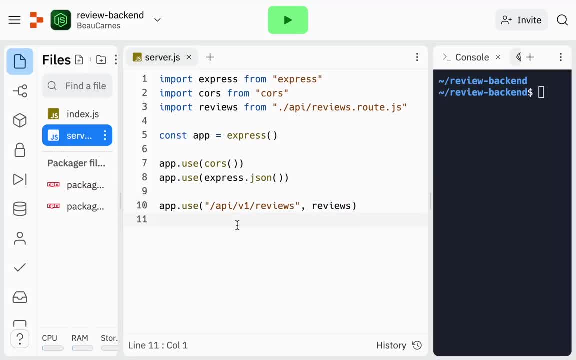 not included in what we create. in that route file. we'll do app dot use And then if I put asterisk, that's just means anything else, And now, instead of loading it from a different file, we'll just put it right here And we're. 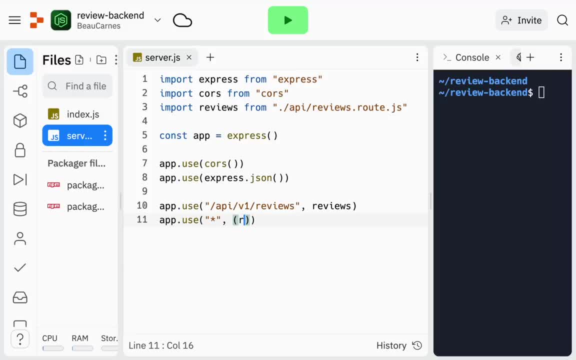 putting a little little function right in the line here. So I'll put our IQ RS. So that's the request and result And this is something that's just part of Express, with the information that it's requesting here And for the RS. that's the response, not result. the response is going to be: 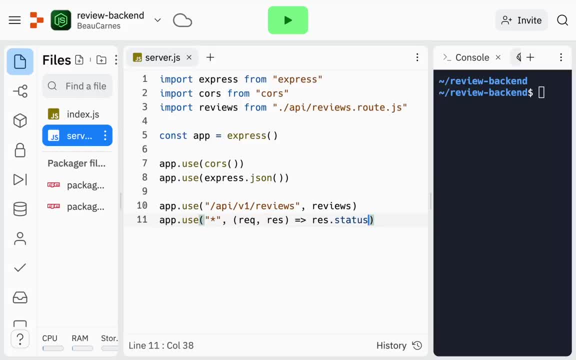 RS dot status And it will send the 404, the 404 code and then it's going to send some JSON and I'll say: error not found. Now we'll eventually see this this appear in a web browser when we go to a specific URL that's not included here. 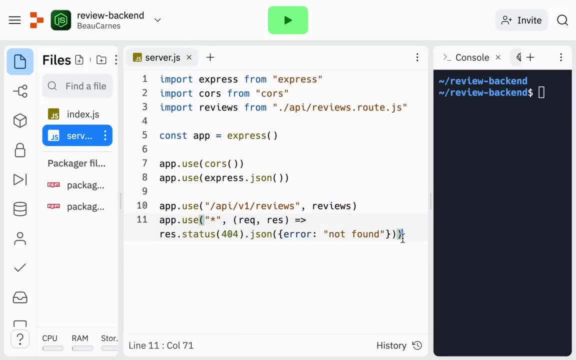 And finally, we talked about how we are going to be connecting different files together. Well, next speaker, teetle masaya truly got msweio with us, So now for sure, thank you for watching Up� 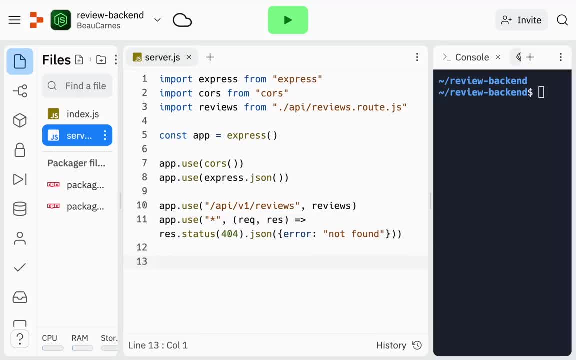 are going to export our app as a module, just like this export default app. So that app is this app that we created here, that we added all these things to, And this will allow us to import app in the file that accesses the database, which will be the file will run to get the server running. So 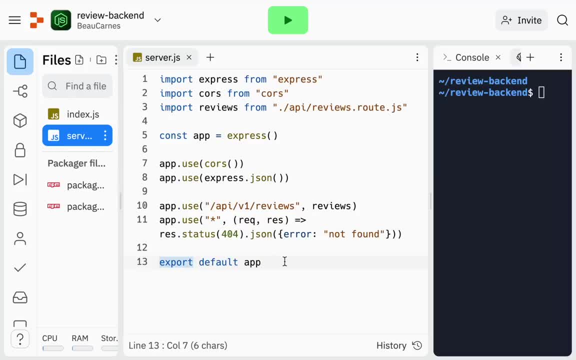 when you want to use code between files, you're usually going to have an export statement at the end to export the file, something from that file to you to import into a different file. So we want to separate our main server code from the database code. So here's our main server code. 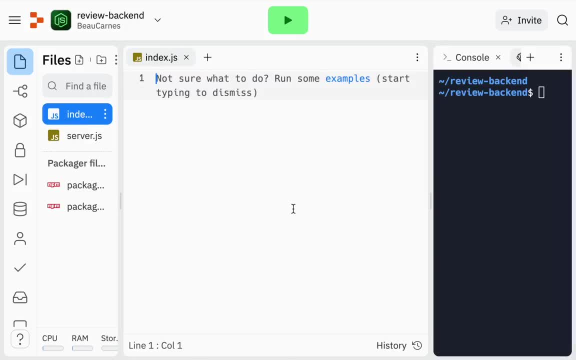 So let's go back to the index dot j s. this is where we're going to start making the database code. But for the to start working with database, we need a database. Now there is a way to use databases included in replete. it has a. where is it here, the database here? But this is this. 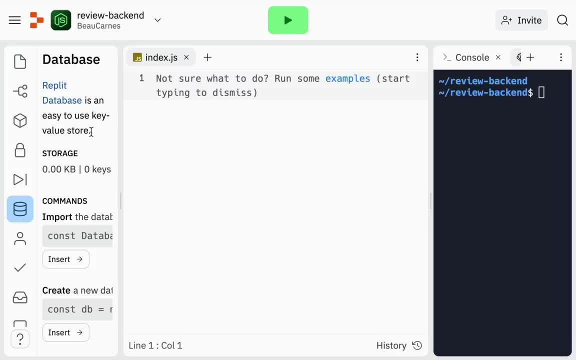 is a pretty simplified database which probably would be okay for our purposes, But it's not going to really work in a production environment. So I'm going to show you how to set up MongoDB As our database. we're actually going to use a different website, the MongoDB Atlas website. 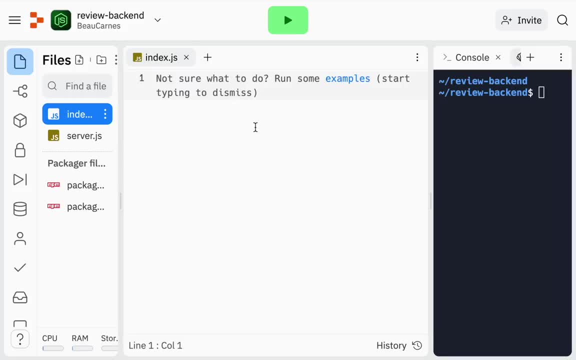 to set up our database. Now you can run MongoDB locally And we could even set up to run MongoDB right in our our shell here, But we're going to be using the online version of MongoDB, where it just stores everything in the cloud. it actually simplifies things. 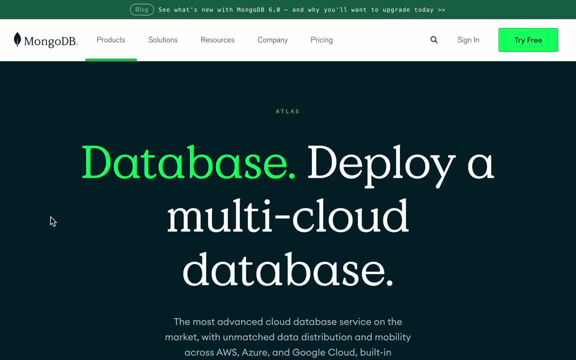 and they have a free plan that we can use. Okay, so now I'm over on the MongoDB Atlas website And you can either create an account or sign in. I'm just going to click Sign In here Now. you may have to figure out some things when you're creating your account for the first time. 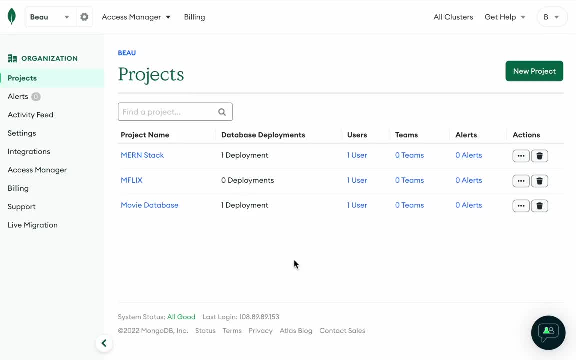 it's not going to go to this website, But you can use that to set up your database. So let's go to this right away. But at some point, either during the account creation process or after the account creation projects process, you'll be in your projects page and you'll go to new project. 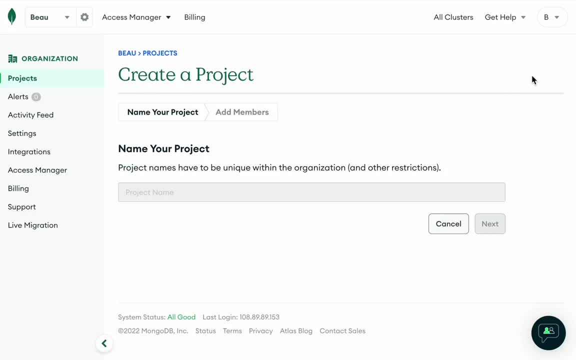 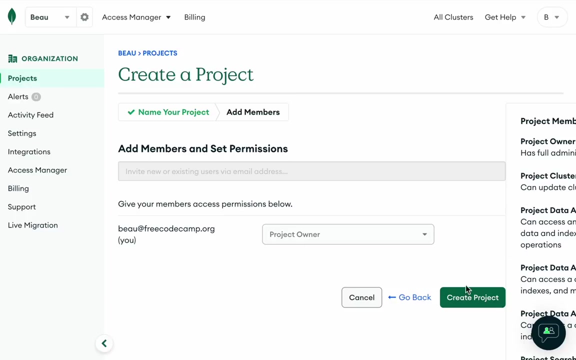 it may go directly into the create a project page when you're creating a new account, So we'll just name the project. I'm going to call this movie reviews. Okay next, And then we can just go through. we'll just use the default project owner. 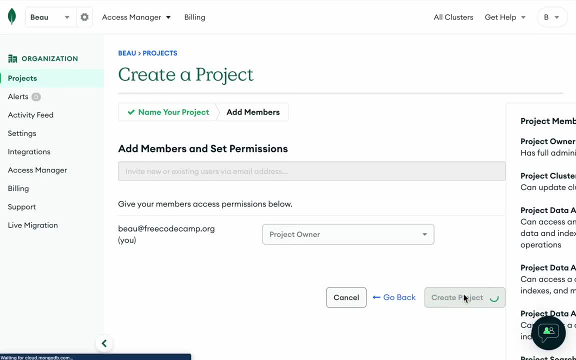 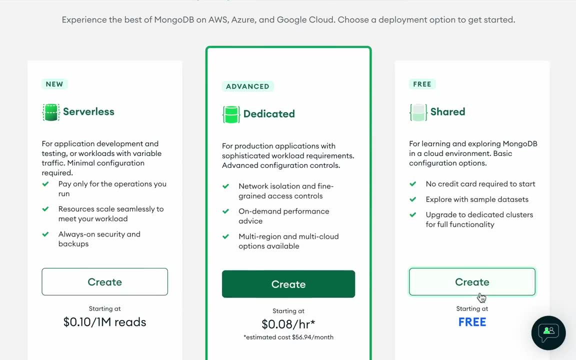 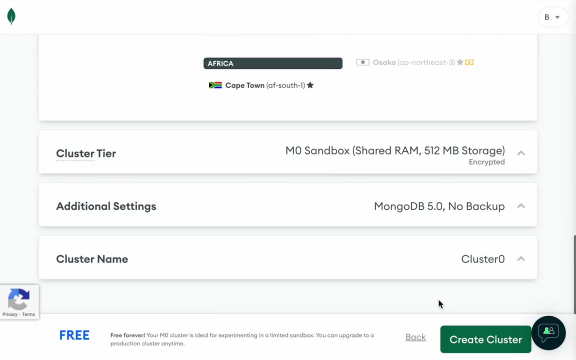 which is me. Okay, now I'm going to build a database. Now we have a few different options. I'm going to go with the free option, which will definitely be good enough for our purposes. If you want to specify any of these things here, I'm just going to leave this all default and click create. 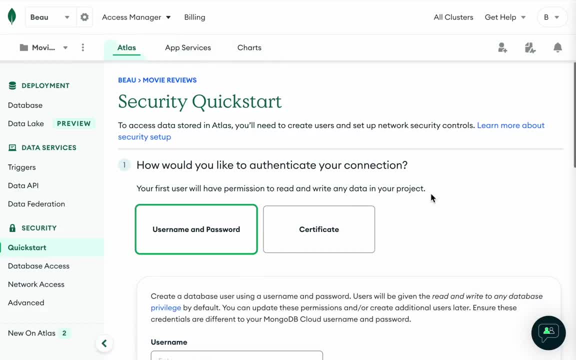 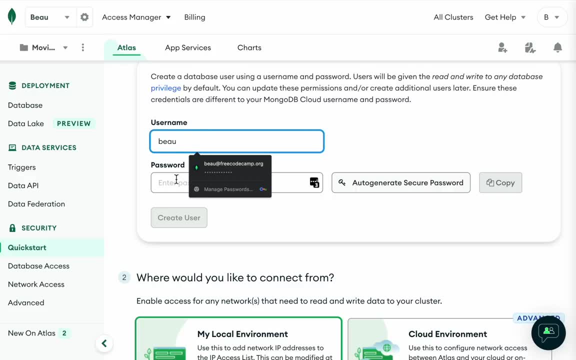 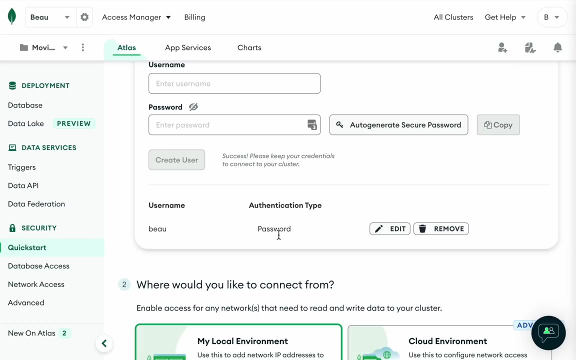 cluster. So this will create a free database here And now I can create a username and password. So I will create a username and password here And then just click Create user. Okay, so the username and password, just you know, this is just for this database. the username you put here is completely. 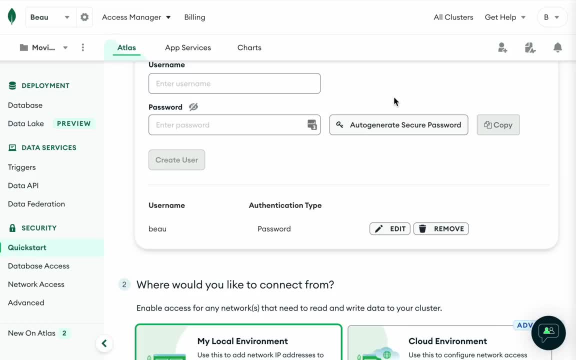 separate from your MongoDB username. It's separate from your replete username. you can basically use anything here. it's only for the specific database we're creating right now, And then we have to do a couple of things here. First of all, we're going to do a couple of things here. First of all. 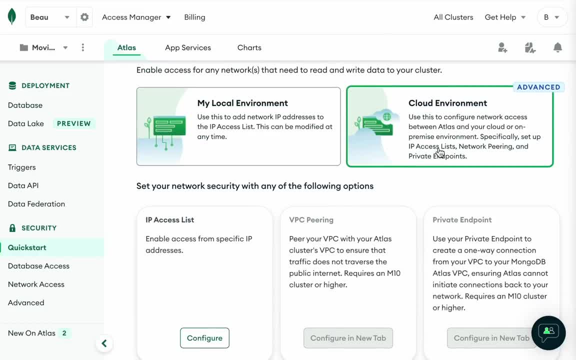 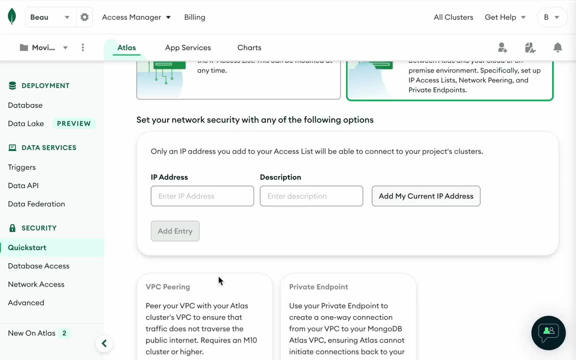 we're going to do a couple of things here. First of all, we're going to do a couple of things here. Well, I'm gonna do cloud environment, because we're connecting from replete, which is a cloud environment, And then we have to configure enable access from specific IP addresses. Now, 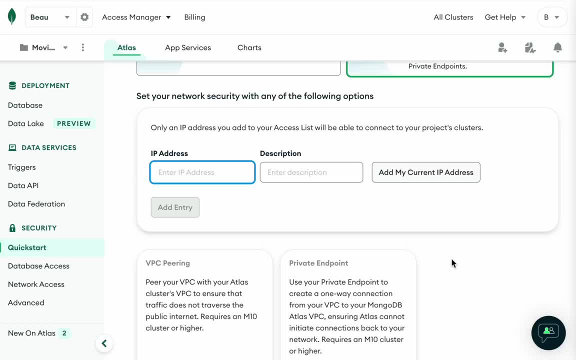 since replete uses, it doesn't always have the same IP address, it could be variable. we have to make it accessible from any IP address. To do that, we'll just do 0.0.0.0, slash zero And. 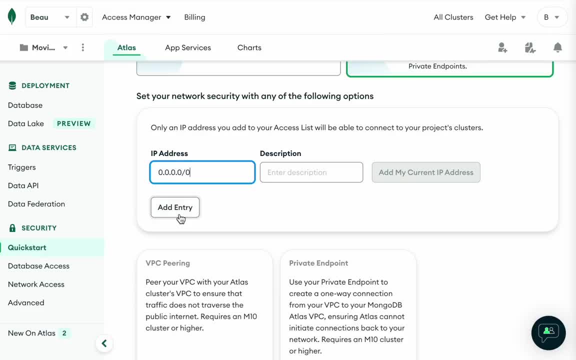 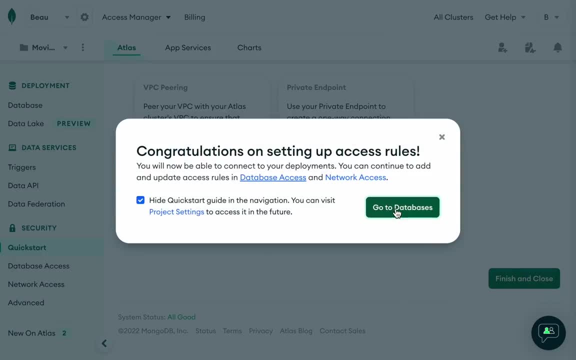 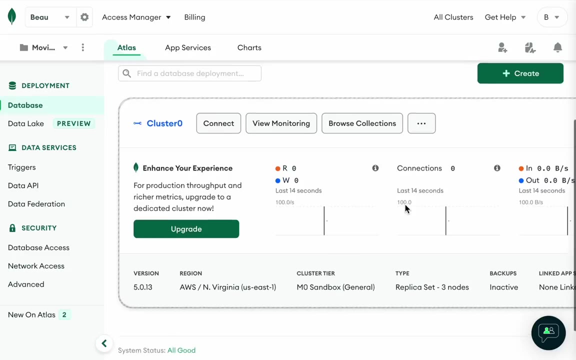 now we'll be able to access from any IP address And I'll just click Add entry there And then we'll keep going down and then finish and close And now we can say: go to database. I am gonna, yeah, I'll click, keep that click. So now it's creating our database, which is going to 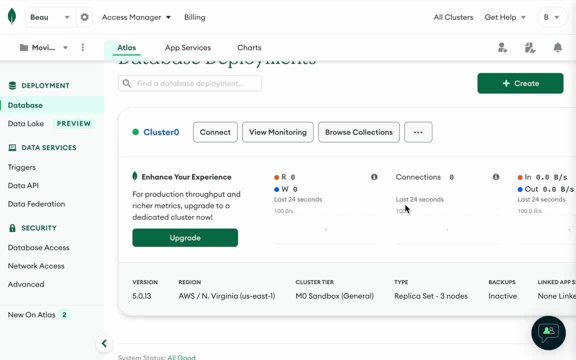 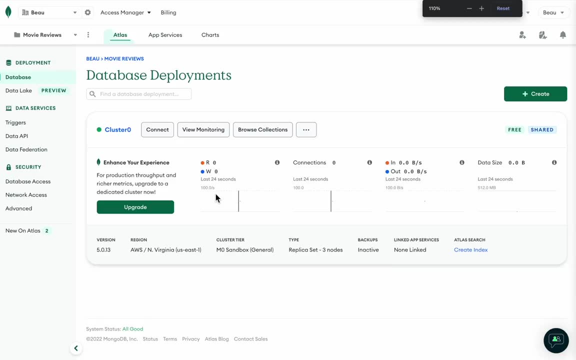 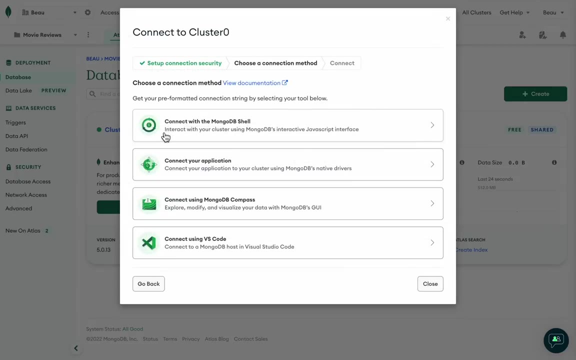 take a few minutes to create here While this is creating- oh, I guess it just already created, it, did not take a few minutes by zoom out here, So you can kind of see what this all this is what the page is more likely to look like to you. So if I go to connect, this is what we're going to. 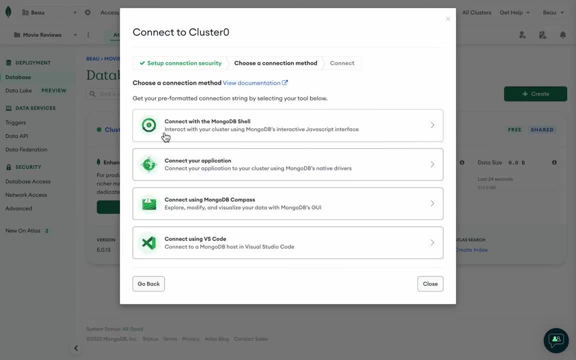 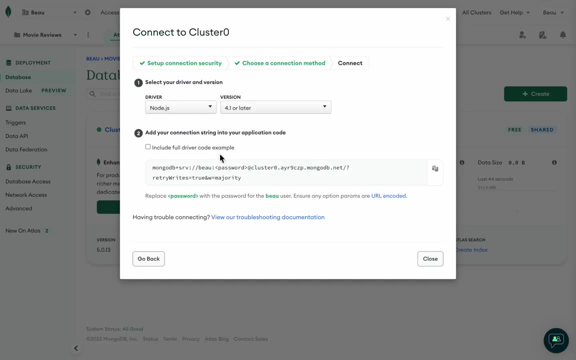 we're going to get some information here to connect to our database from replete. So I'm gonna go to connect your application here And then I'm going to make sure I'm on the node js. it's the default here And we have this connection string. Now we're going to need this later. 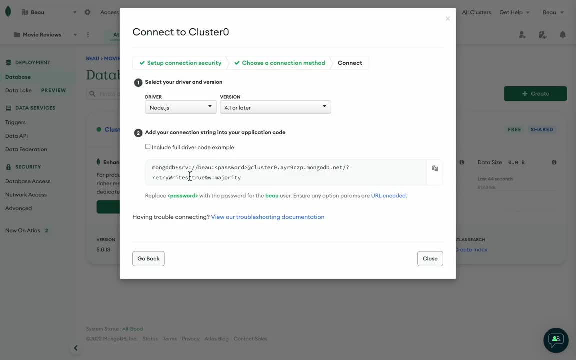 I'm just going to click the copy button to connect. I'm copying this connection string which is we're going to put into a certain spot on replete so they can connect to our database. So let me just go back over to replete, So before we start typing into anything into our indexjs. 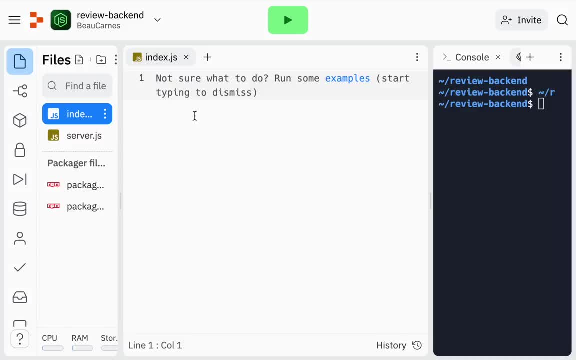 let's create some environment variables, Because, if you remember, we just created a password and you never want to store a password right in your JavaScript file. you want to store in an environment variables. environment variables are things that are not often like, are not saved. 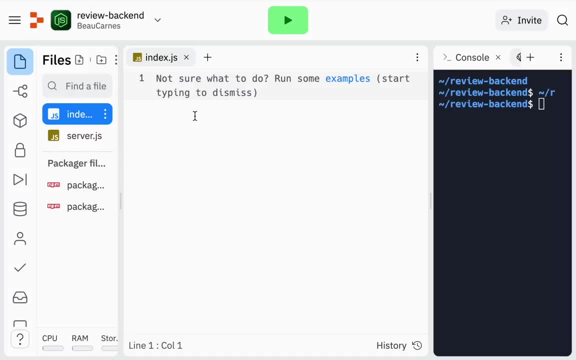 they're harder to access. We need any special information like passwords or anything that could change regularly. you may want to put in an environment variable instead of right in your code, And also with environment variables, if you're going to ever put things on the GitHub. 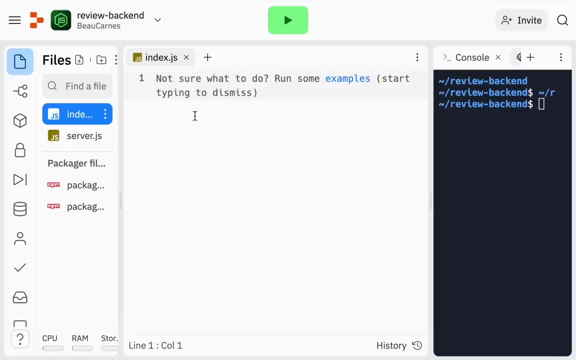 you never want to upload passwords or anything on the GitHub, So you want to store that into an environment variable. that's only stored in the environment, And then you can still access that, what that variable is, from your program. But you don't actually have to have the hard coded. 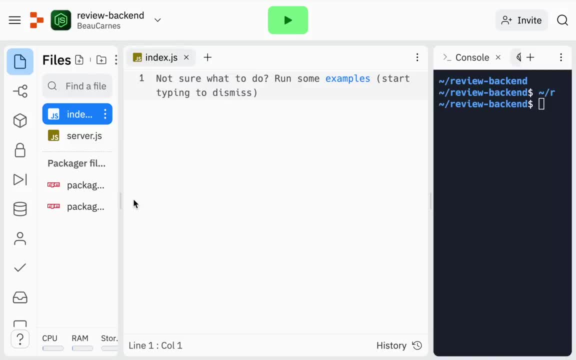 password right in your program. So in replete there's, you know, there's you know. there's a special way to deal with environment variables. it will be a little slightly different if you're working on a local machine. But if you're just doing it locally you can just kind of look up. 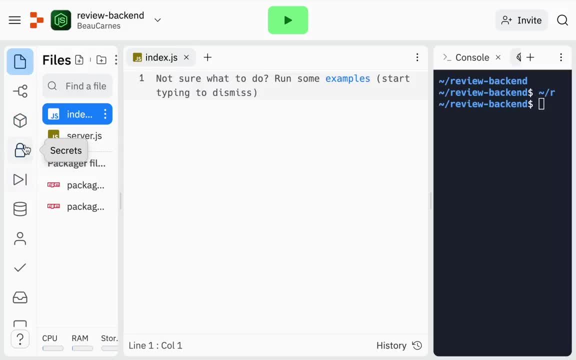 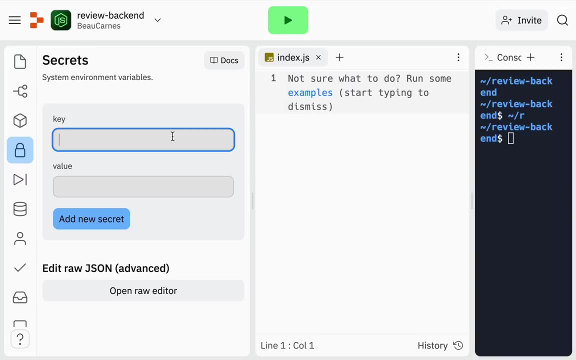 how you would deal with environment variables locally. But on replete, we're going to go to secrets And let me bring this out here. So we're going to create a key. So the key is like the variable name and then the value will be the: the value, the value of the variable. So we're going 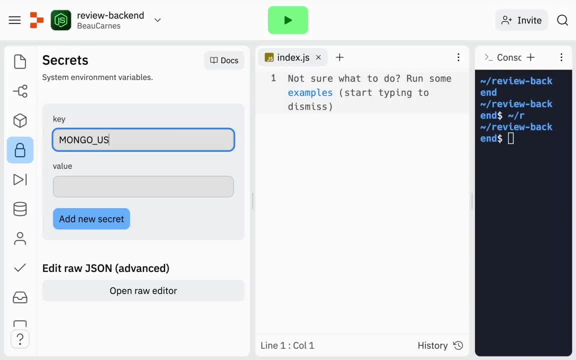 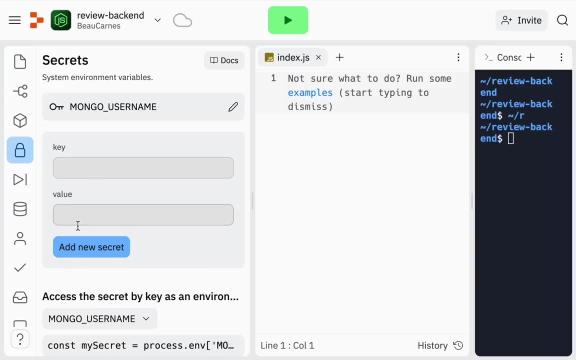 to create a one called Mongo user name, And then we're going to create a one called Mongo user name And then I will put bow. So this was just the username I created for our database. add new secret. Now let's do Mongo password. Okay, you have to promise not to tell anybody. 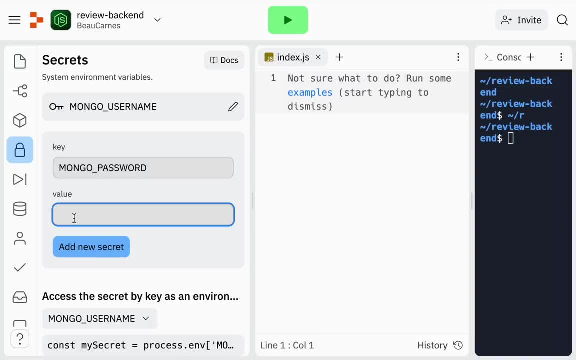 what this password is. This is just between me and you. It's a complete secret. You cannot share this password with anybody. But I use free code camp. Okay, so I'll add new secret And now we, we can now access these in our code. But I'll just close that for now And then I'm going to 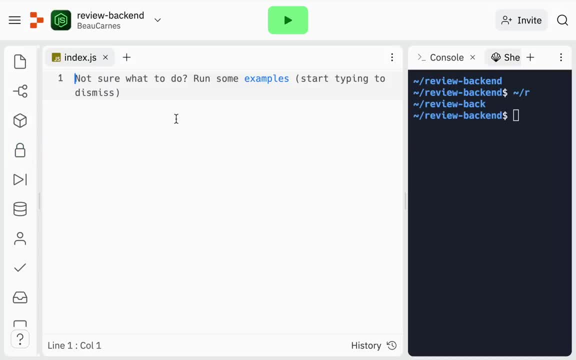 create a new password And then I'm going to create a new password And then I'll add new secret And let's start creating this file. So first. so in this file we're going to connect to the database and start the server. So first we'll do import app from see. 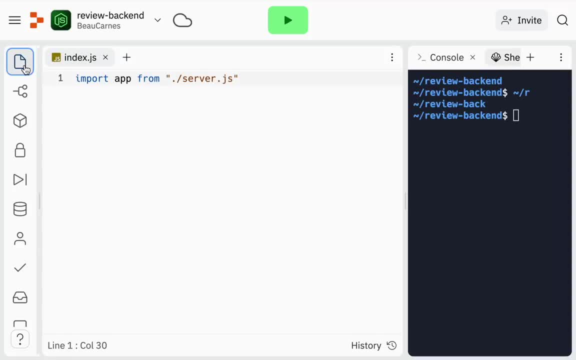 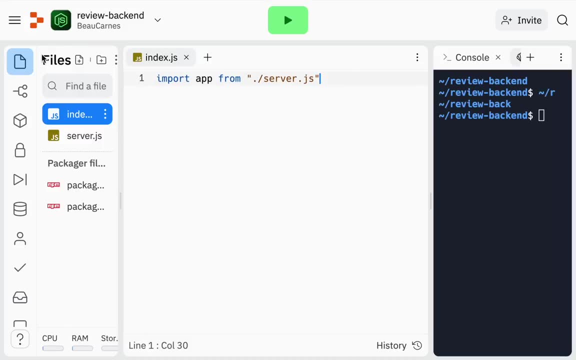 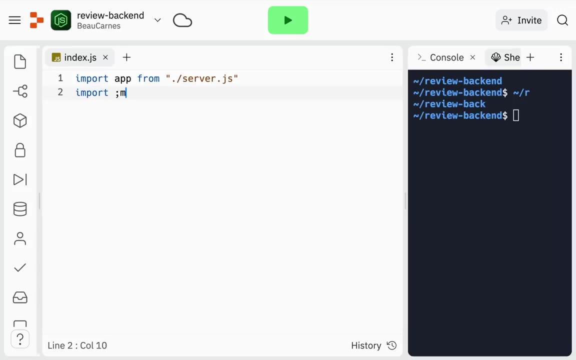 serverjs. That was just the other file. we created serverjs And we exported the app down here And now we're importing it. So now we can use that code in this file And we can have separation of concerns between what we're trying to do here. So now we'll do import among. 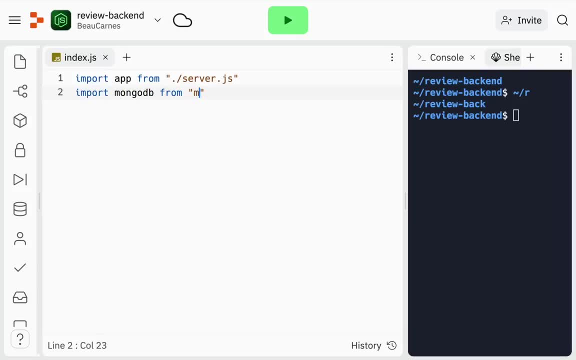 MongoDB from Mongo MongoDB. Now, this is just a JavaScript library that, when we run, our code will automatically be imported And then we can use these special functions that were created, that the people who create MongoDB also create this JavaScript library to make it easier to interact with our MongoDB database from JavaScript. And now we're going to. 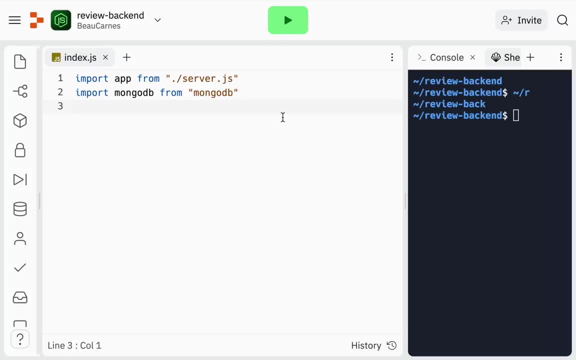 import another thing and some from a file that we we still have to create. So this is going to be called reviews da Oh now, and it's going to be called for. it's going to be from that slash da o, slash reviews da ojs Now da o. here that stands for data access object. This is basically a common 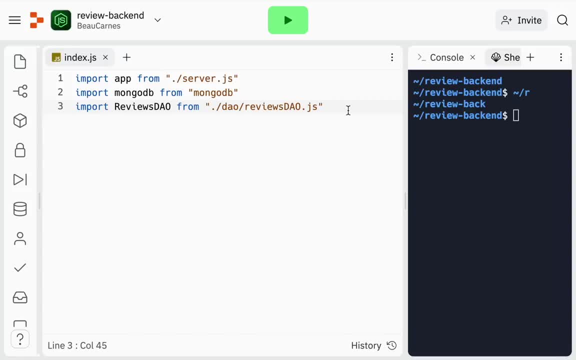 pattern for writing programs that work with databases. So the data access object pattern separates a data resources client interface from its data access mechanisms. it adapts a specific data resources access API to a generic client interface, And so we're following that pattern in how we set up this. 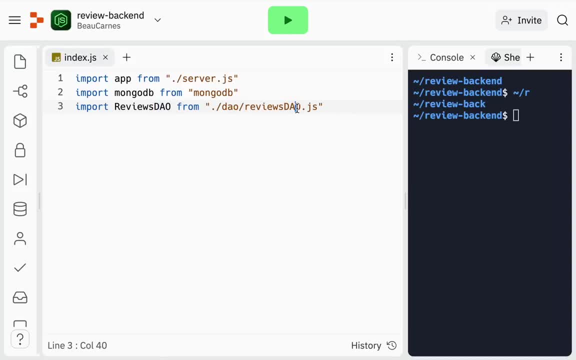 this program, And that's why it's called da o here. Okay, we've imported everything we need to import. Now we'll create some variables. we're first going to create a Mongo client. This is something that comes right from MongoDB, the MongoDB JavaScript library that was created by MongoDB to make it easier to 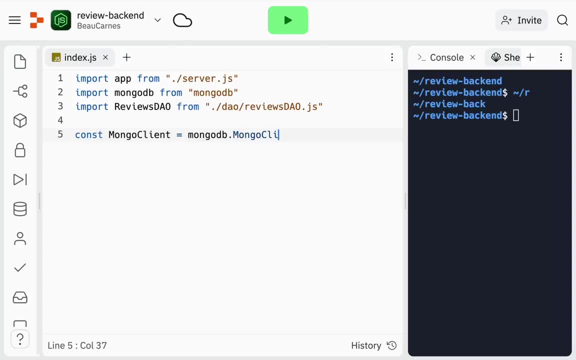 work with our database. So MongoDB dot dot. Mongo client. So I've created a variable called Mongo client that we get from this, And now you'll see how we'll be able to use that to connect to our database. Now let's get access to our username and password. 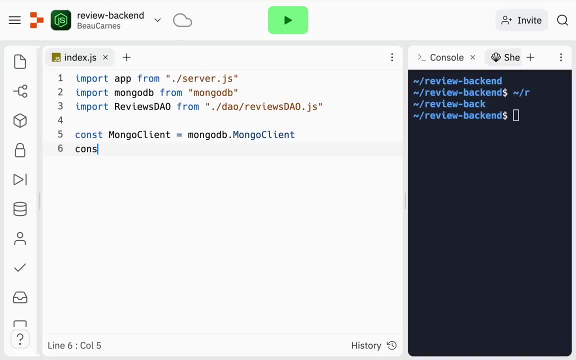 We've stored in environment variables. So we'll do a const Mongo username equals And then we will do. this is how we get an environment variable process dot e and v. Now this is actually basically what you would do to access an environment variable in a local machine. to. 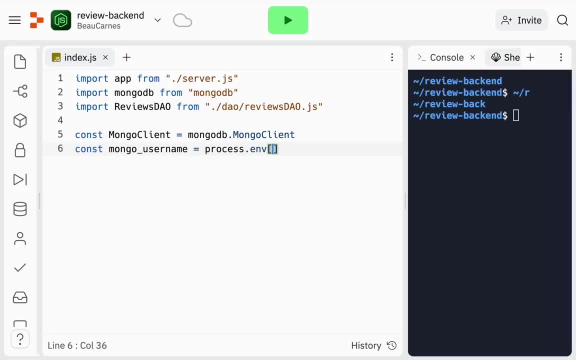 process dot e and v, And then we will do Mongo underscore username. So remember that was the name of our or one. Now I'm just going to copy this line And then we'll do mongo password And then Mongo password. 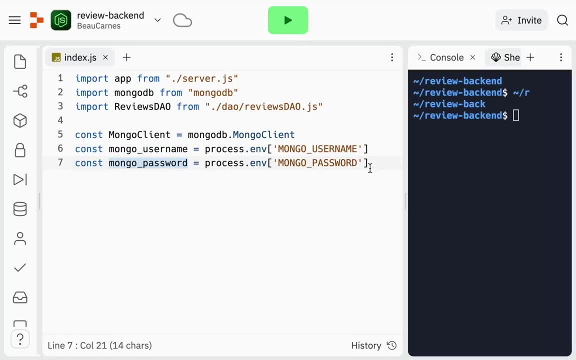 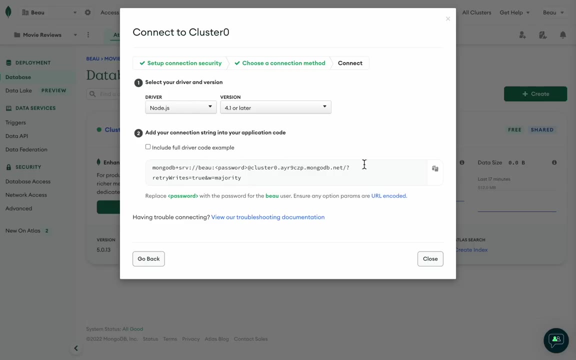 So now we have access to both of our environment variables in the in these JavaScript variables. Okay, now, this is the, the last one. that's just important const, And this is the UI. Now, that's a what we got here on the MongoDB website, where we copy this right here. This is the, the. the URI is: 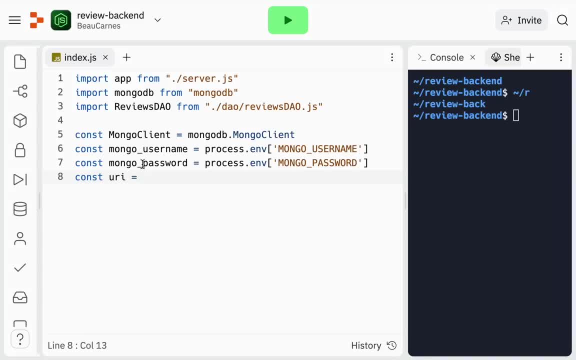 the connection string. So I'm gonna go back over here And I'm going to put it in a string I'm going to use. I could put the string. I could use double quotes or single quotes. I'm going to use the backtick And using a backtick allows us to do something special. allows us to access JavaScript. 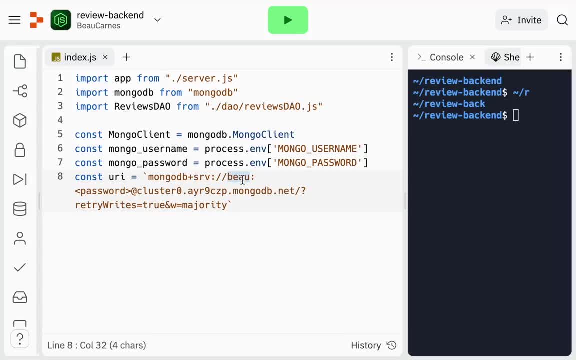 variables from inside the string. So we have the username hard quoted right in the string here, But I'm not going to use that variable here, So X, I'll just. I'm going to copy that variable. And now I'm going to do dollar sign and then curly braces, And now I can just put that variable here. 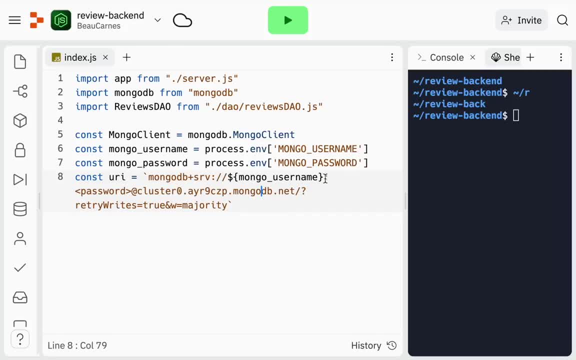 Now you can see, since this is a different color, it's black. That's how we know that this isn't part of the string. we're actually just inserting that variable into the string And we can do the same thing with the password. So where it has the angle brackets with the word password. 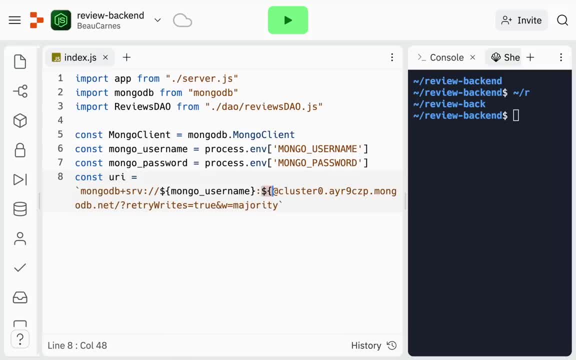 I'll do curly break brackets like that. I'm going to copy this and then just paste it right in there. So now we were putting our username and password right in the string And that will allow us to connect to our database. Okay, well, actually we're making one more variable, which is: 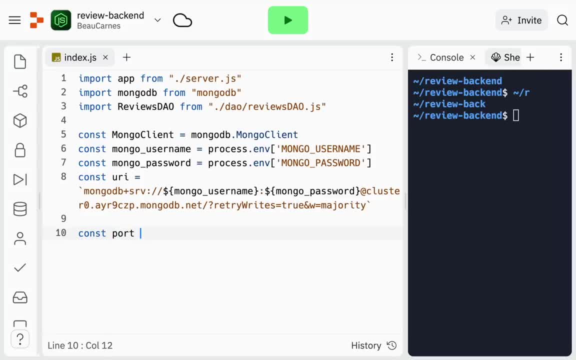 the port. we were basically running our server on a specific port, And the port that we're going to be running on is going to be 8000.. So you can. the port number isn't super important, There's just different ones that are common to use for different things. Okay, now we are going to connect to our database. 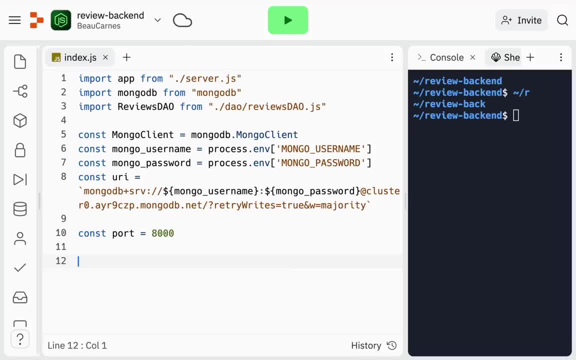 So we'll do a Mongo client- I meant to do Mongo client dot connect, And this is just something that comes with the MongoDB JavaScript library, And I will do a parentheses And we'll start by passing in the URI And now we're going to pass in some options Now 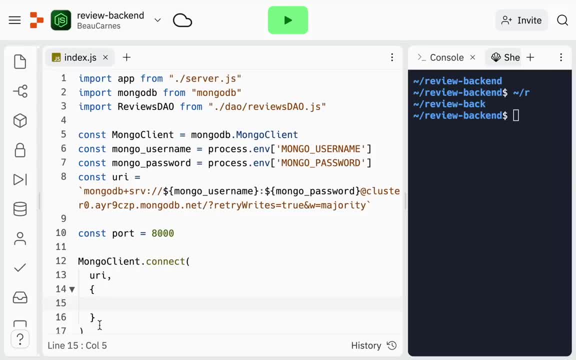 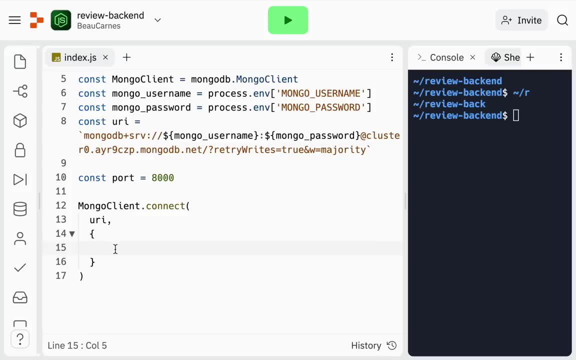 these options are going to be a JavaScript object. that's why the curly braces here, which is going to be a set of key value pairs, And these are just options that the Mongo client is built in to be able to accept. we'll do a max pool size. 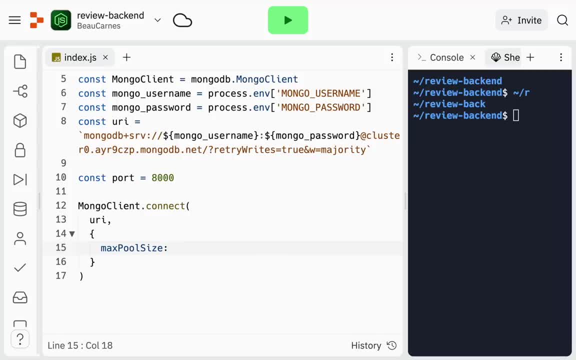 which is the amount of people that can be connected to at one time. we'll set it at 50.. And then we'll do a w time out, dot ms, And we'll set that to 2500.. That's, that's 2500 milliseconds. 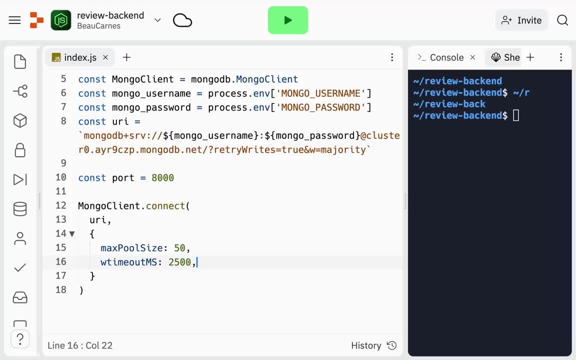 or 25 seconds. That's how long a connection can be trying to connect before it time times out, And the final thing we'll do is use new URL parser and set that to true. Now that's added because the MongoDB Node JS driver rewrote the tool that it uses to parse. 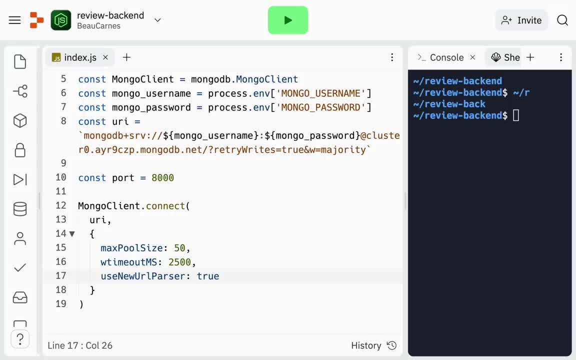 MongoDB connection strings And it put the new parser behind a flag, So you basically always have to set that to true, And so that will end the connection. So we've connected by passing in the URI and then the options, But after we connect we want to do a. 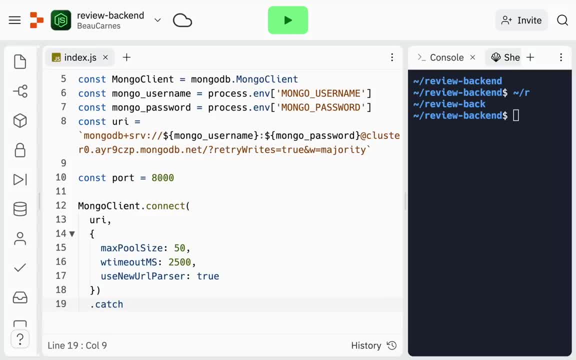 dot keV So this will catch any errors that happened when you're connecting. So whenever you're going to access an external resource like this database, you want to deal with errors. So we're gonna do a dot catch to catch any errors that could happen. but they may not happen And I'm going to put in 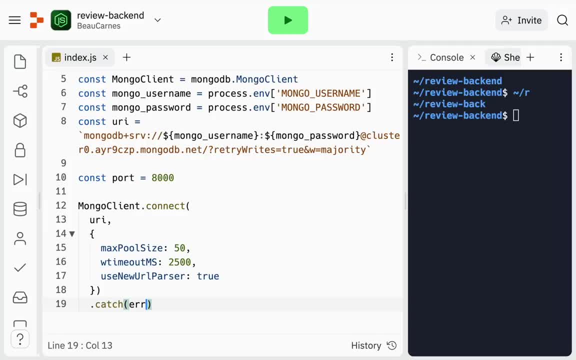 an error arrow function. This is a special type of JavaScript function that that makes it easier. that just simplifies what a function looks like And you can put it all in one line and you don't have to name the function. So this is the ERR, is what we're passing into the function, And then I 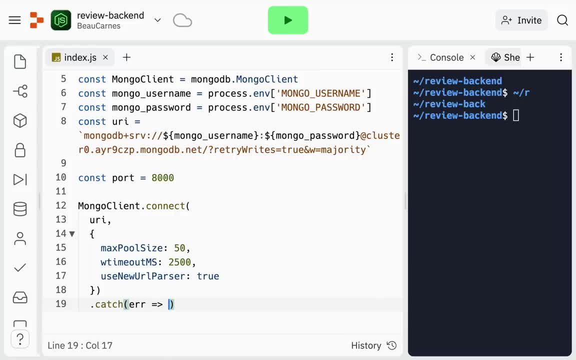 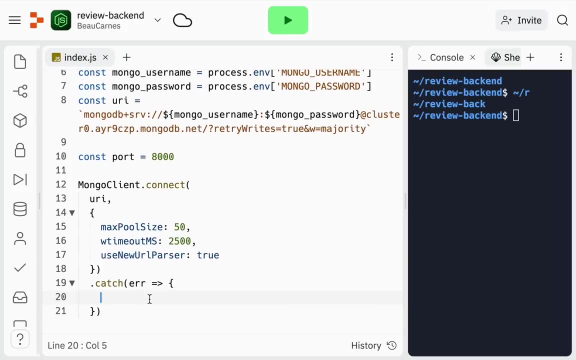 put an arrow, just like that, with the equal sign and angle bracket, And this is the body of the function and these curly braces. So what we'll do if there's an error, we will console dot error. Now, console dot error is similar to console dot. 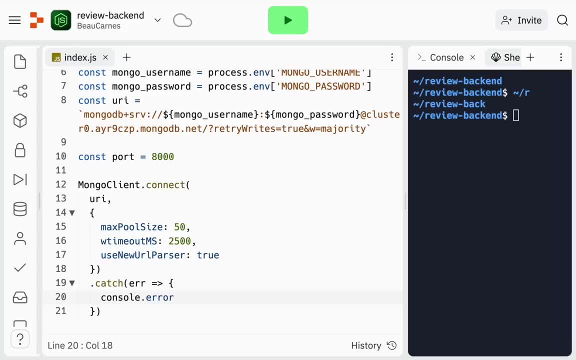 error. Now console dot error is similar to console dot error. Now, console dot error is similar to log, but it just communicates that it's an error. it will appear right, it will be, a message will appear in a console And it just. it's just like a special type of console dot log And we'll log. 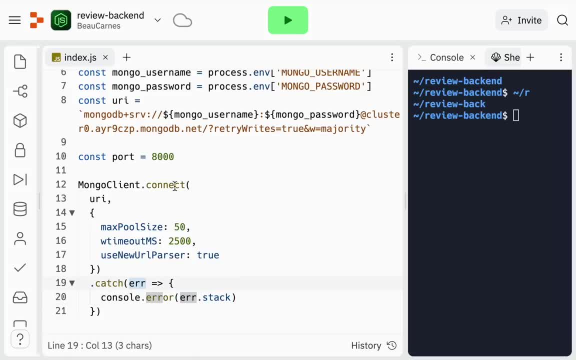 air dot stack, So the air that comes from connection. if there is an error, we'll just log the error stack And then we will also do process that exit one that just means we're going to end. this is just like a fancy way of ending the program. we're exiting the process. 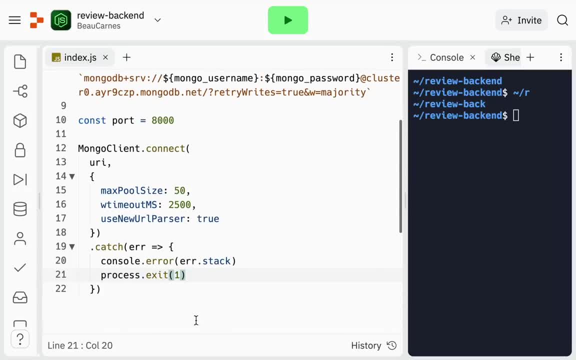 of the process would be that the program that we're running, So after we is, when there's no error, then we can go to the next part, which is a then statement. So first we're going to connect, then we're going to do something. well, we're going to pass in a function into here, So it's. 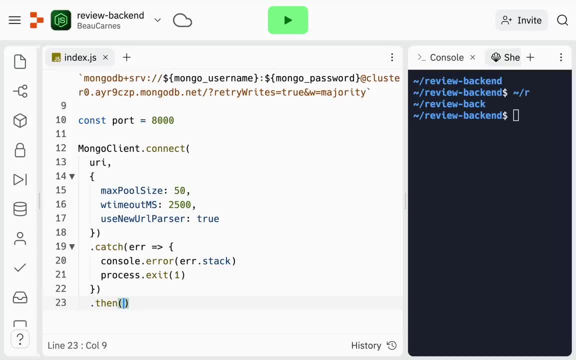 going to give me an an error function and it's going to be a special type of function And it is a sync function. And a sync function is just a function that can run asynchronously or it can run at the same time as other things, So you don't have to wait for one thing to end before. 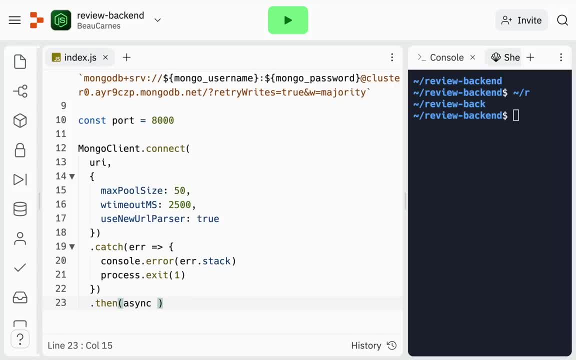 something else happens, Or you can use an async to make sure you wait for something and before something else happens, which is what we're using it for. So we are going to get the client. So the client is what comes from what we're connecting to the. 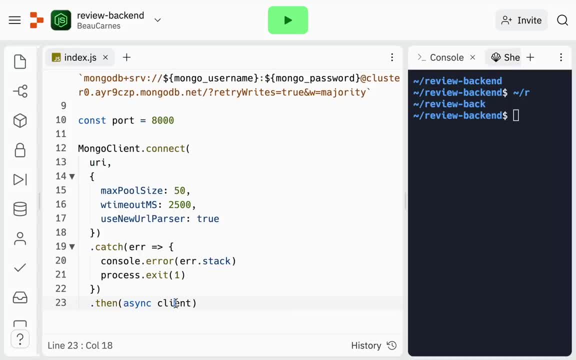 data. So we're going to get the client. So the client is what comes from what we're connecting to the database And it's going to return a client. So then it's the. this client variable is coming from the connection to the database And we're making this into an arrow function. Okay, we're. 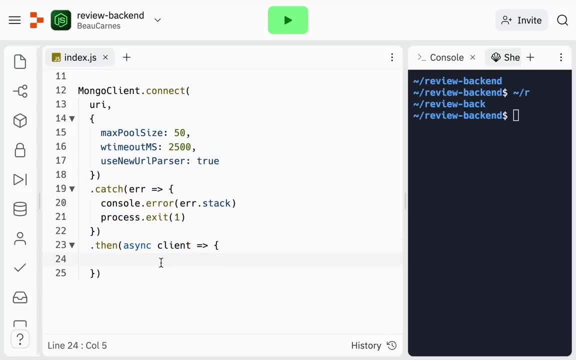 not going to actually use the client just yet. First we're just going to start the web server So we can just just kind of test everything out. So I'm gonna do app dot listen. So we got right here. the app came from our server up here, And app dot listen is how you start the server. So we are. 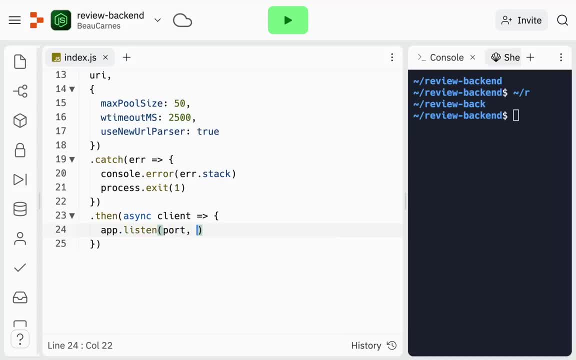 going to listen on a specific port number And so we pass. there's two. basically, this is a function here And we're passing in two pieces of information: the port and then an A. we're passing in a function and we're going to use an arrow function. So if you use parentheses here, 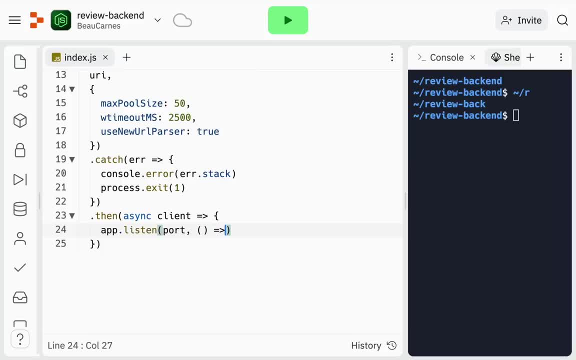 that means we're not passing any, any data into the arrow function. So we're passing in a function and nothing to this arrow function. And inside the body of the arrow function we are going to just log some information. console dot log And we will just log listening. 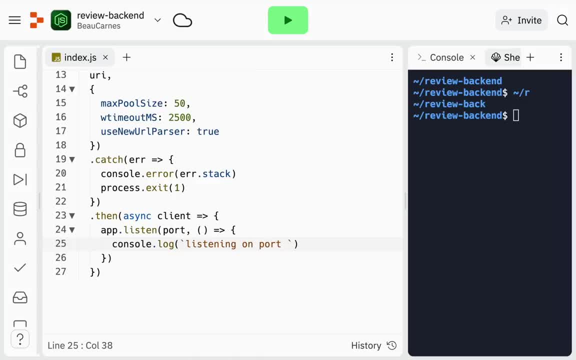 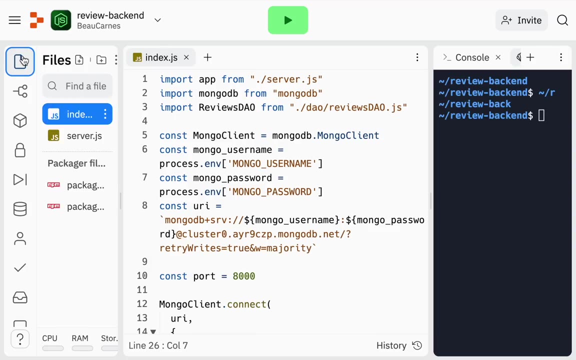 on port and then just the port number: port. Okay, it's actually almost time to test out our server, But we also need to get a route. So, if you remember, back over on our other file, our serverjs- we have this reviews route, So we need to create a route. 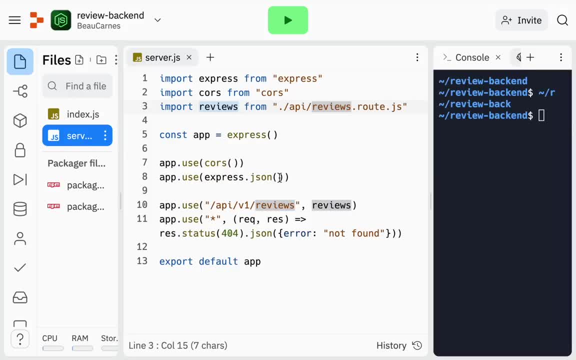 before we can test out the server. Now, let's make it. we're gonna make it as simple as possible to test out and then we'll make it a little more complicated. So I'm going to create a new directory Now. you don't have to, but it helps to keep your code organized, And this directory is: 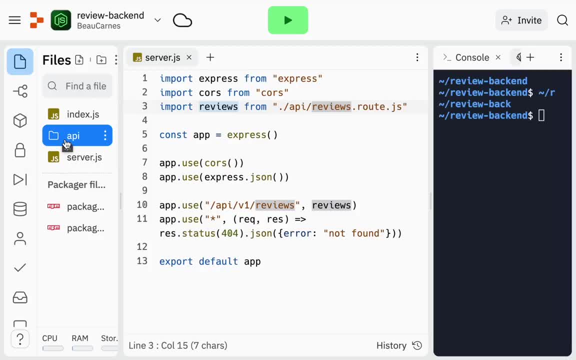 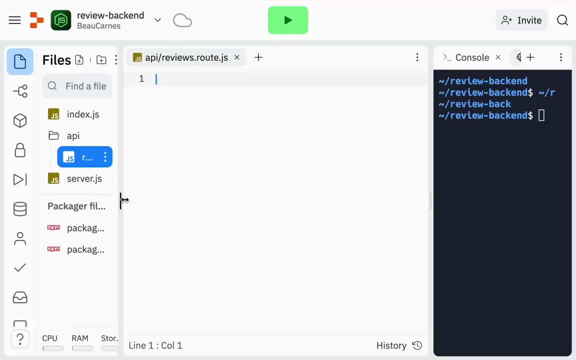 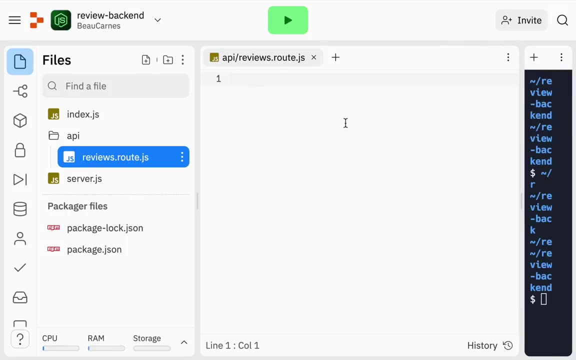 called API. So all the all the code for API will be in this directory. First we will create the review dot routejs So I can. so reviews that routejs. Let me make this over a little bit here And so. 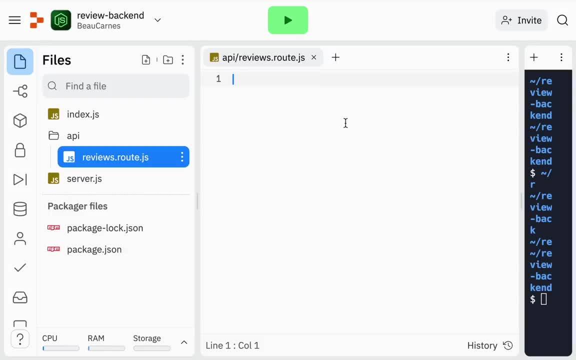 to create our route. we'll first import Express from Express, then we will create our router, const router. So this will, when people go to our URL, this will route the request, two different, different parts of our application, So Express dot router. 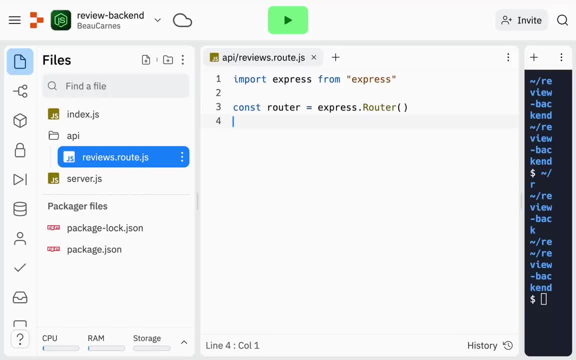 it's just part of the Express that helps us make our our web server And now we'll do router that route And then we can pass in. so slash just means that the base, the base route, and we'll do that, get. And then you always need, when you're creating a route, you always have a the request. 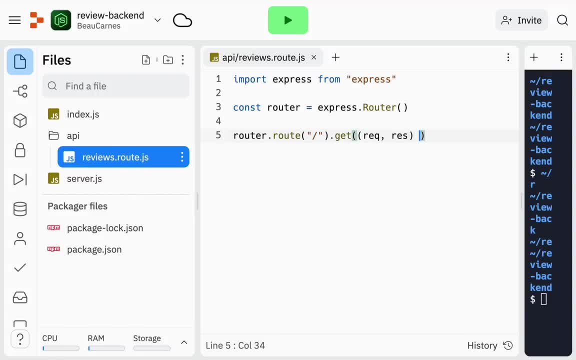 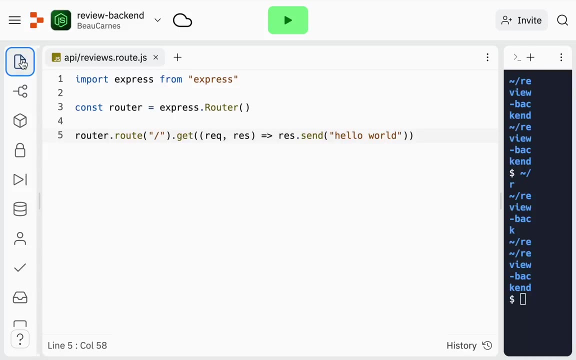 and the result- And this is going to be a little arrow function here- And the result that send. we're going to send this result to whoever is requesting that route And it's just gonna say: Hello world, Let me close that So it can be all in one line there, And then I will just do. 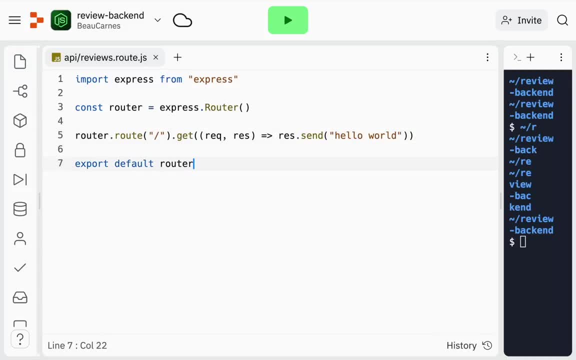 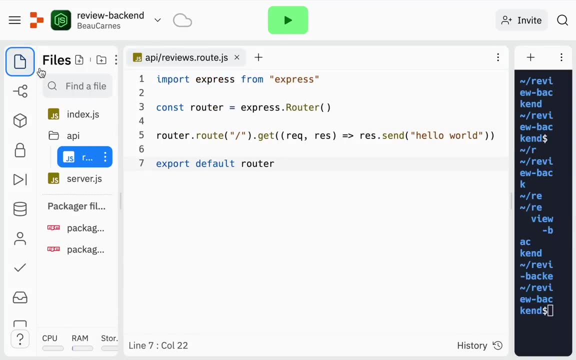 export default router. So it can be. we import the route in our other file. Okay, I think it's time to test out. Let's try this. So when we press run, it's going to run index indexjs where it's. 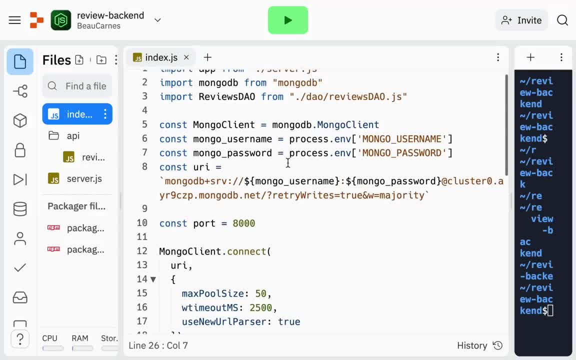 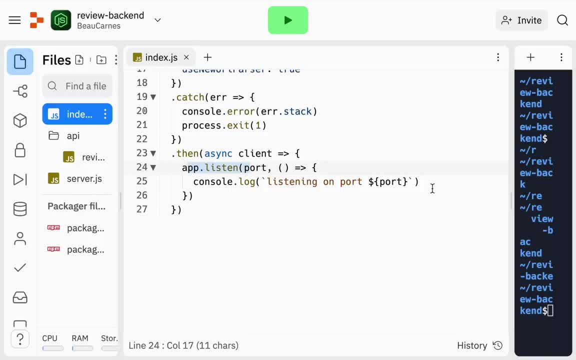 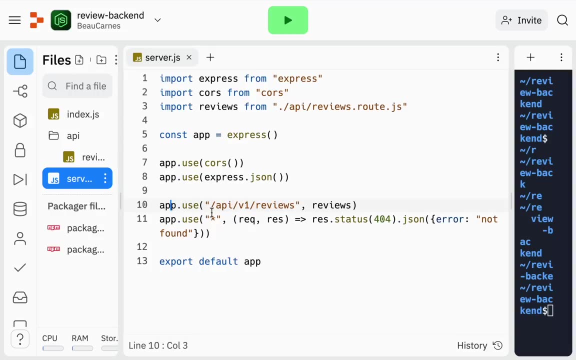 going to get access to our database, But we're not actually going to do anything to our database quite yet. But when we do app that- listen here- after connecting to our database, it's going to run this. it's going to run our app. when we have, we're using this route, And so this is our kind of 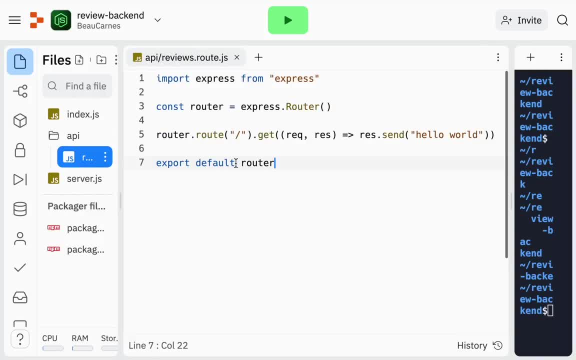 our base URL, which I'm going to copy right there, And then it's going to put this at the end of our base, our base route, And then, if you go to that URL, it's going to do Hello world. So let's test that. 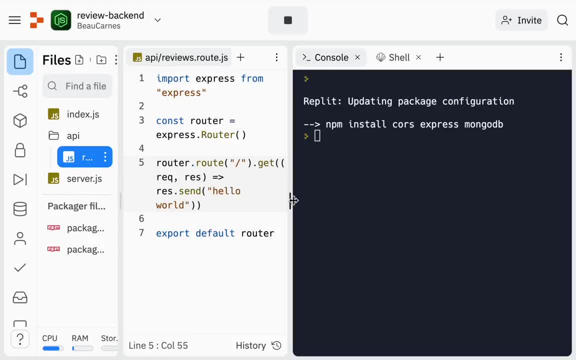 out Now I just press Run And so the first time you run it's going to have to install everything. So it's doing npm: install cores Express, MongoDB, MongoDB- See, we imported all of these libraries- cores Express and MongoDB- And because- see. 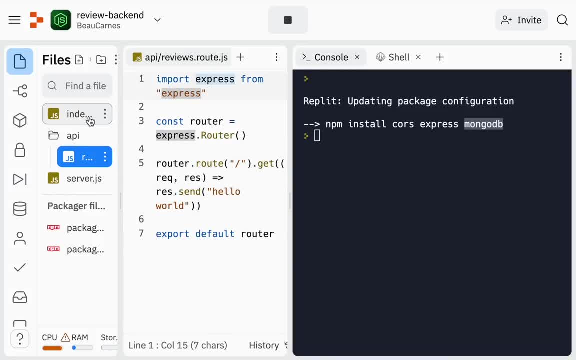 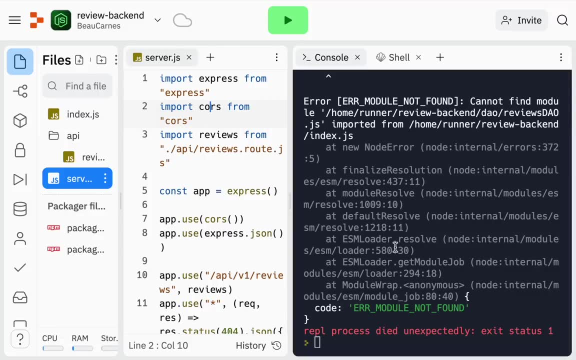 so we're basically just waiting for it to finish. But you can see we import Express here, we import cores And let's see we already have an error. it cannot find a module And because what this is one. we haven't actually finished creating the reviews, dao reviews down. So if 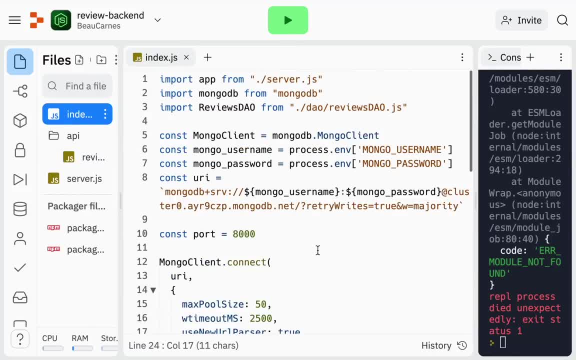 we go back over to our indexjs, Let's, let's just we're not using it yet, So let me just comment that out With you. know, the two slashes will comment or what I just did. you can do command or control and then press slash will automatically make into a comment. 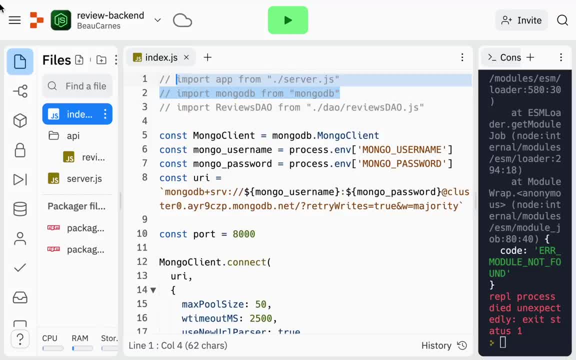 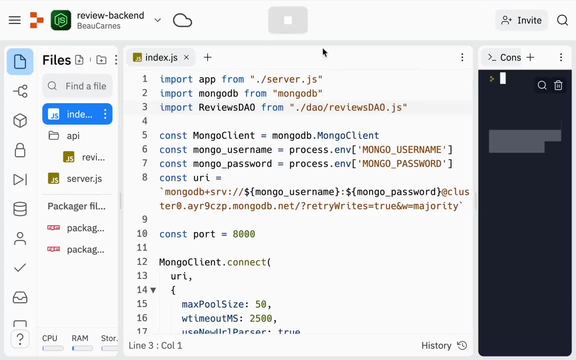 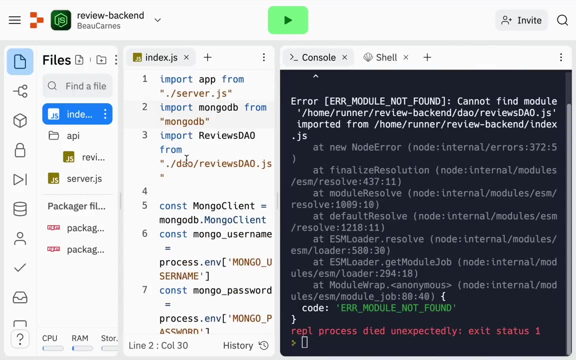 you can actually do that for multiple. So if I highlight everything, do command or control slash, and then I can kind of turn off it and on a comment, So we're not creating that yet. So let's try running this again And then here. Oh, I somehow didn't end up with that still being. 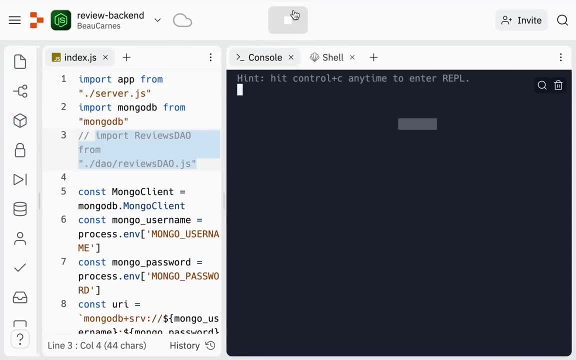 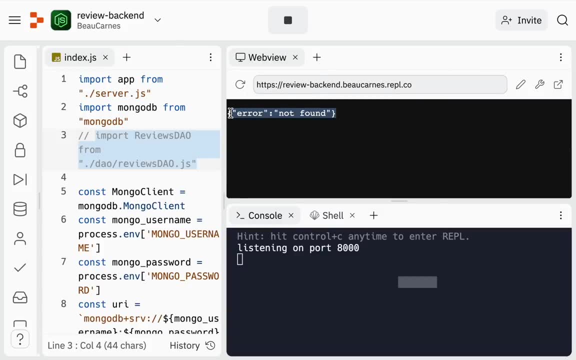 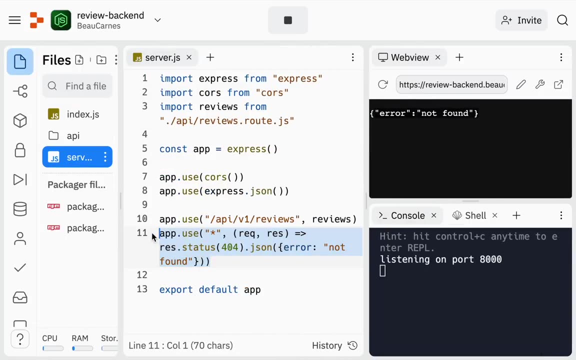 a comment, So comment that out. Now run it. Okay, so it's opening up our web view: error not found. Well, that's coming directly from our server here. If you go to a URL that hasn't been specified, it's going to say error not found. Now let's see what happens if we go to a URL that. 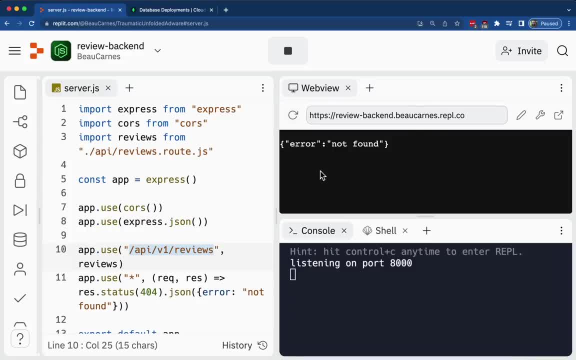 is specified. Another thing I want to show you is that you don't have to use this little webview right here. So this web view x, it only lets you go to the root URL. But since I'm going to copy this now, I'm just going to go open this up in a new tab And you can see it's saying error, not. 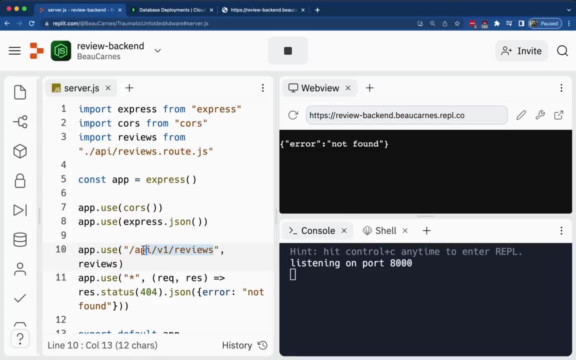 found, just like before. But now I'm going to get this to add to the end here And I'm going to add that to the end of the URL And I'm going to click on that. Now I can see right here it said: 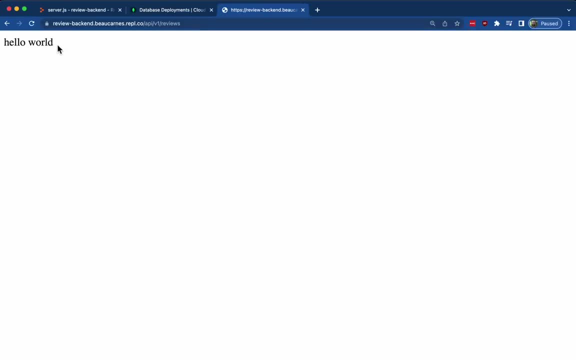 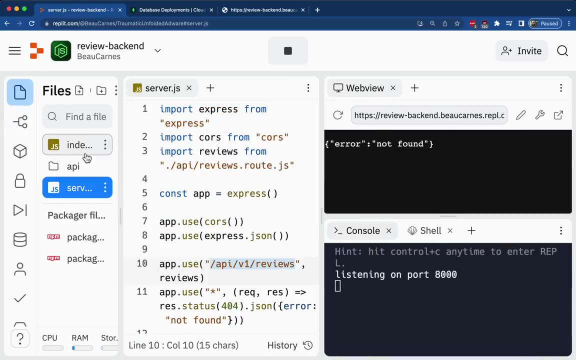 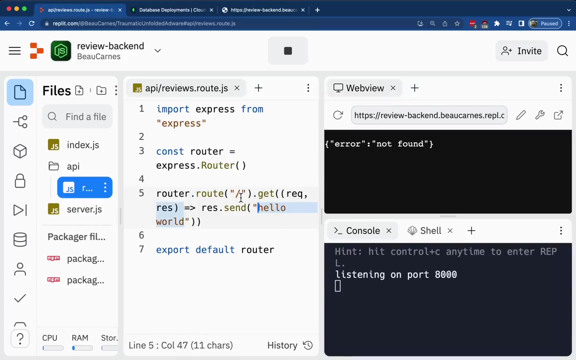 And it says Hello world. So when we go to the URL, it says Hello world And it's coming right from our route, the route that we create here. it's sending Hello world. when we go to the, we go to the root URL and then there's a slash at the end And it works. So whenever you go to a 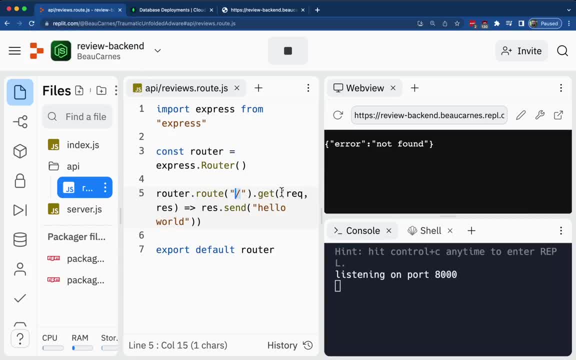 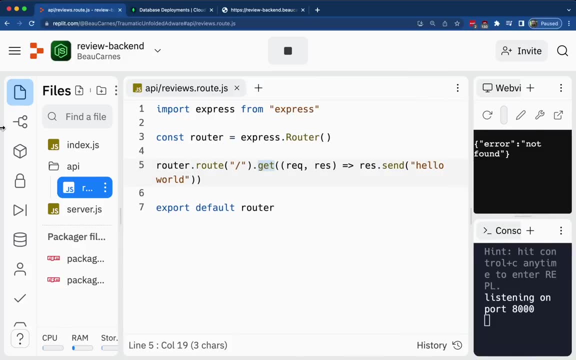 URL on a. in a web browser, it's almost always doing a get request, But, as you may know, there's other types of requests, like post put and delete requests, which we will be using as we continue here. Okay, so let's update this. So this is just a sample to see how you can go to a specific route. 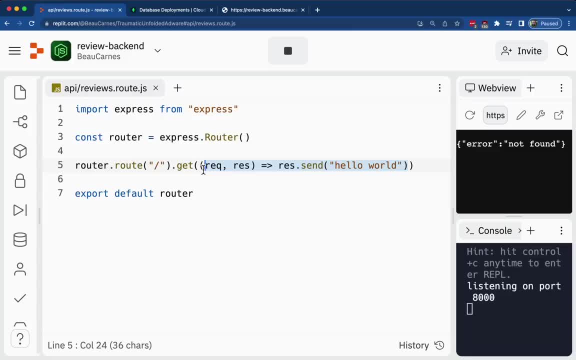 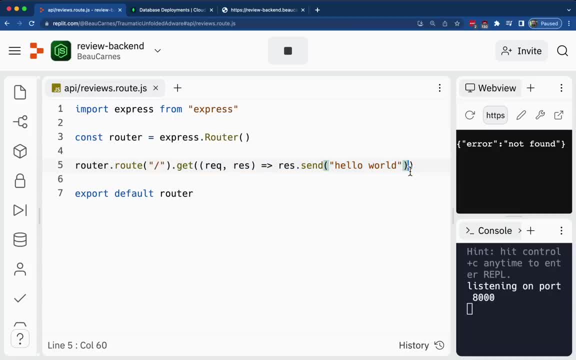 going to put what's returned in or what happens when you go to that route and a different file. So right now, what happens when you go to that get request route? it shows right here, but we're going to try to separate that out. So we have our route file and then we're going to have a control. 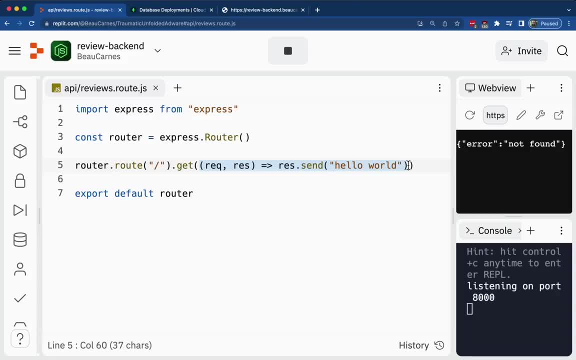 that our controller file and we're going to access our controller file to tell what we're going to do when we go to the different routes. So I'm going to import another file here. So import reviews control from and we'll do reviews controllerjs. Okay, so we slept. so we have to create that file. But 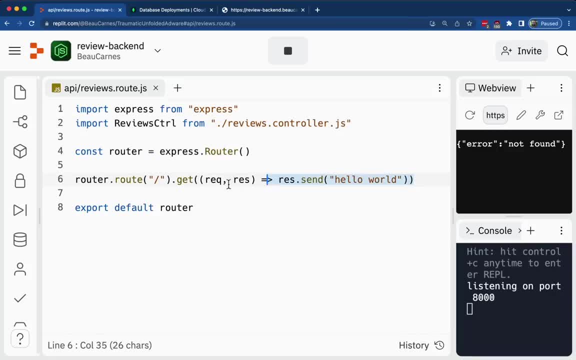 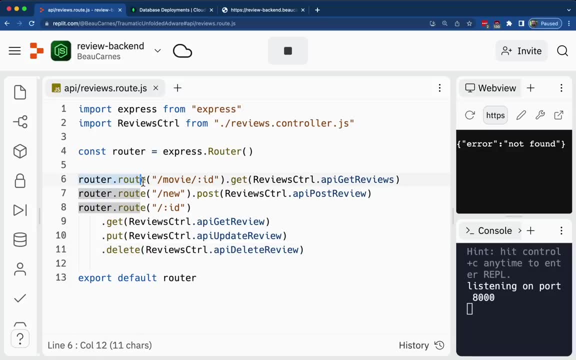 before we create the file, let's, let's use it in this file. So this time I'm just going to paste in some code here and we'll talk about it. So this: now we have a different type of route. So before we just had the slash as the route, but now we have slash move. And now we have slash move. 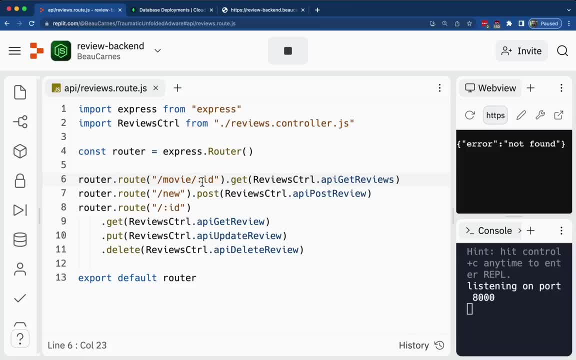 slash ID, but it has a colon here. So if you have a colon in your route here, that means this could be anything here And this becomes a variable called ID. So now we can do movie and then put the movie ID like like 5678, or something like that And then in our, in our review controller. 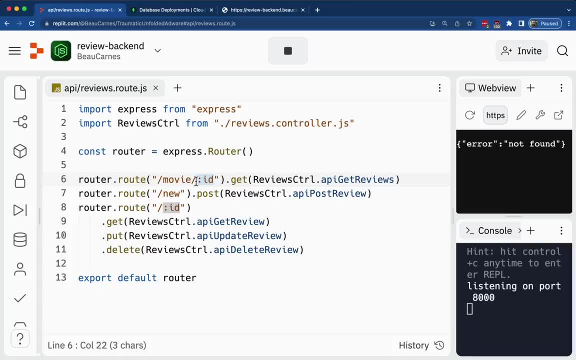 we can get access to whatever ID was put into the URL to do something With that ID. So this is our, this is a get request where we're trying to get information And see we can see where all these were using the review. we're calling functions in the reviews. 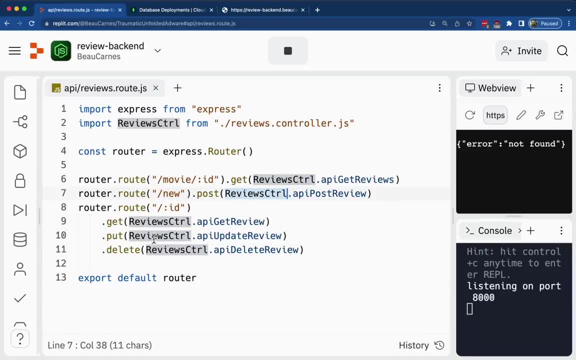 controller. we're going to create all these functions to say what happens when we go to that route. So this is the API get reviews function, where it's going to return all the reviews that are attached to a specific movie, And then here route slash new is when we want. 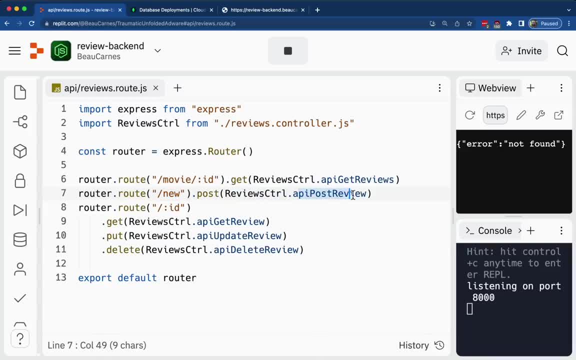 to create a new review. So review controller dot. API dot. API- post review. we're going to be using a- see, it's a post request here, And post requests are usually used when you're creating something new- And then that we use a different format here, where now all these routes are these: 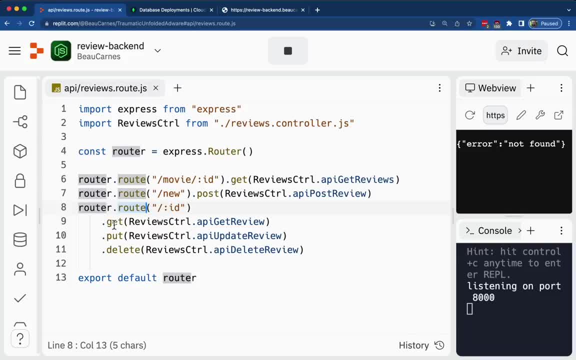 are all different HTTP request keywords for the same route, So it's slash ID. So here is the movie ID, But here it's the, the review ID. it's a different type of ID and we can get access to the ID And if it's a get request, we'll call this function. if it's a put request. 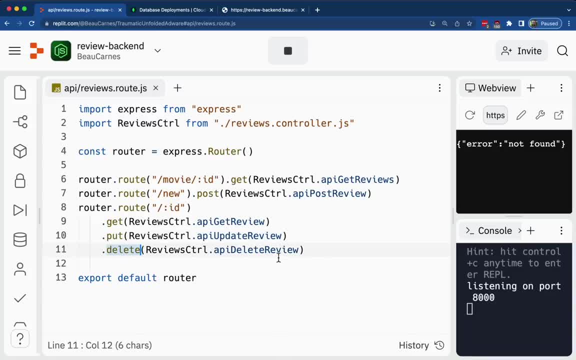 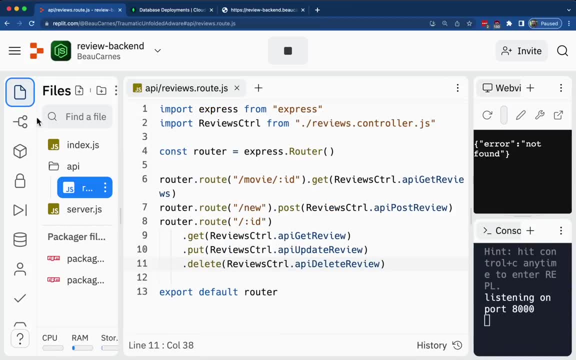 we'll call this function. If it's a delete request, we'll call this function. So let's create our reviews dot controller. So I'm gonna go over here and we'll do reviews dot controller, do dot j s And you can kind of see what that looks like here. Now, close that we're in our reviews. 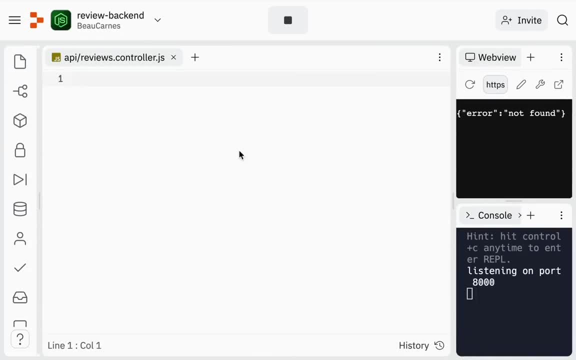 controller. Okay, this time I'm just going to paste in some code to make it a lot faster. then we'll review it. Now it's gonna look pretty complicated, We it's more complicated than our last JavaScript project, But just stay with me And I'll explain how it all works. So let's go. 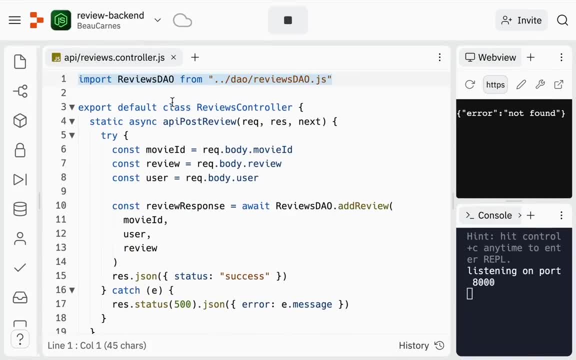 back to the top. So first we are going to import our reviews down Now. this is is is what we're going to use to actually access the database, to actually make changes to the database, And we'll be creating that next. So basically, this file is all about getting information from the, from, from 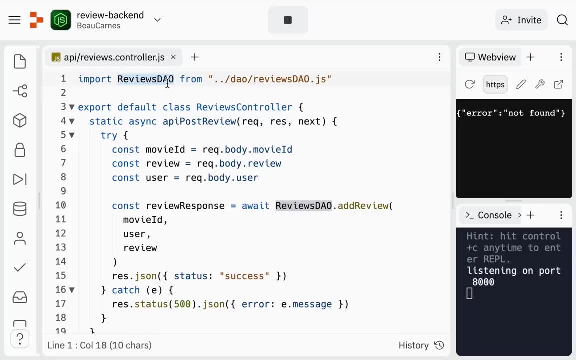 the that was sent to the to the route and sending it to the reviews down. So it will. we're all the controllers- just getting information from the route and then doing something with that information. And what it's doing with that information is sending it to the reviews down, which will actually access the database, and then 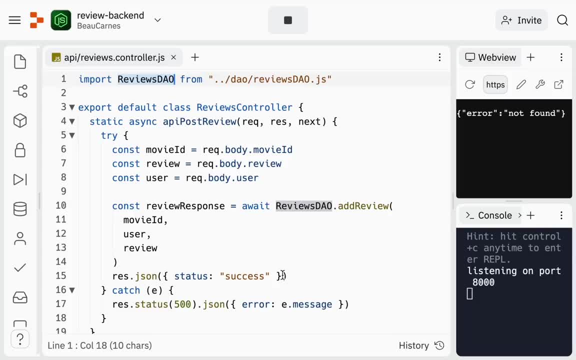 it's going to get information back from, from the database. So let's, let's look what we're doing here. So we are going to. first, we're going to be exporting default class reviews controller, So this just means we've had had exports. 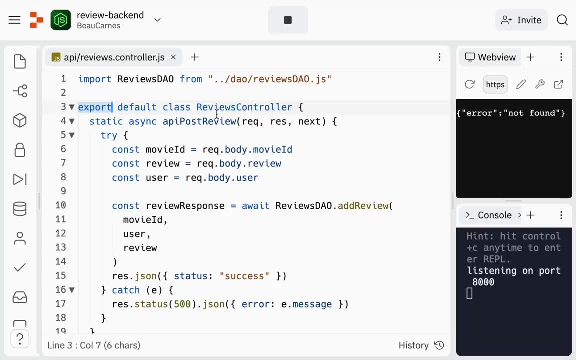 on all of our files so far. So, since we're exporting the reviews controller, that means we can import it in other places, And this time we are creating a class. So a class is something is. a class is used in JavaScript to have multiple functions, So we're going to create a few. 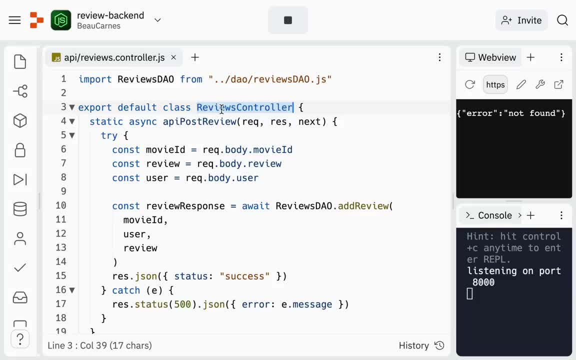 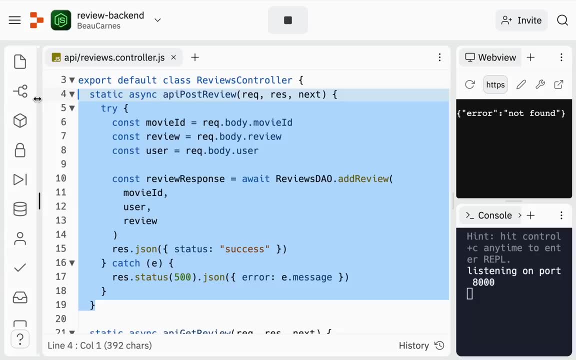 different functions in our review controller that we can then call in our in our routes file. So here's the first function. here It's a static function because you can call it directly from the reviews controller. If it wasn't static, we would have to. 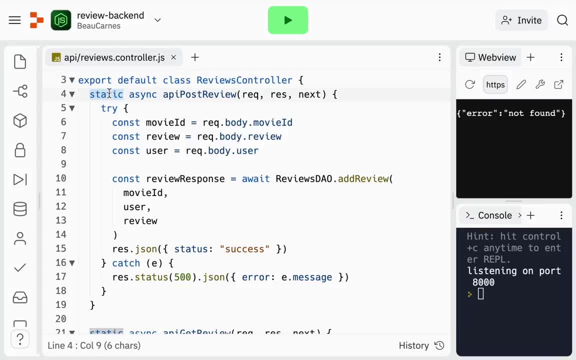 create an instance of a reviews controller, which we're not going to talk about it right now in this section, But since it's static, we don't have to create an instance Now. since it's a sink, we can then use a weight- a weight to wait for things to come back to the review controller. 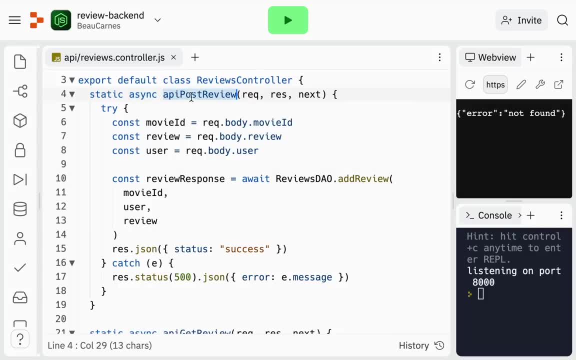 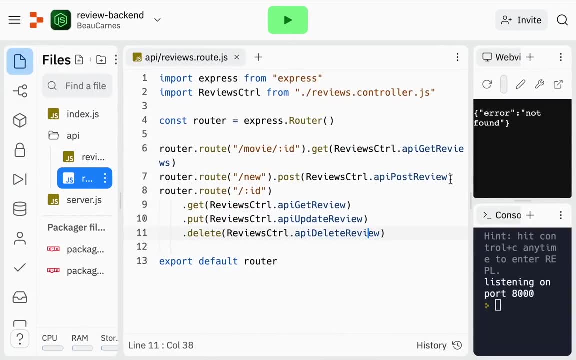 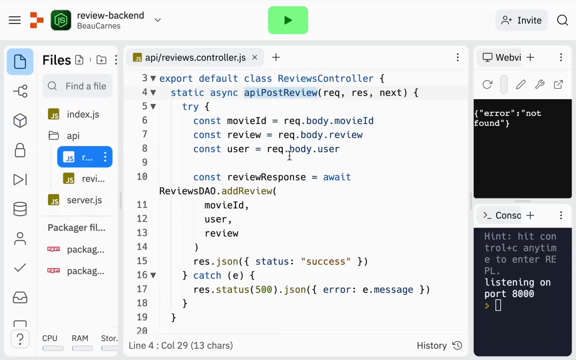 Theか Finn's m bugs to be posted as. so if in those cases, let's say we were and hungry and accomplished something in this case And we can go back and close the worried things to happen, And so the name of it is API post review. So if we go back over to our our routes file, we can see 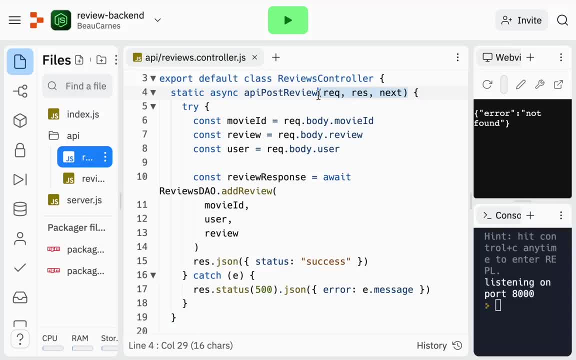 it says one right here: reviews controller API post review. So we're creating that right here. That's what we're creating. So this information is actually just coming right from Express in the request. the request is going to have a body, So a body of the request that's going to. 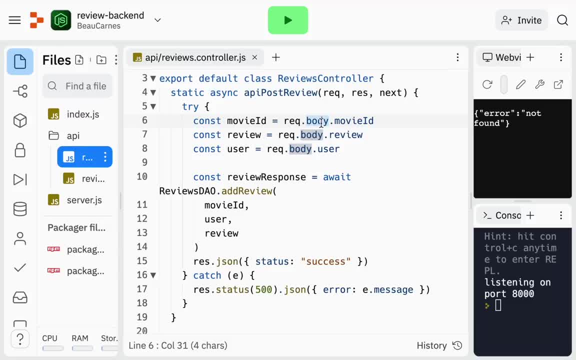 be some JSON that's that's submitted with the URL request, HTTP request, and it's going to have some information. it's going to have the movie ID that we're connecting the review to. it's going to have the review, the actual text of the review and the user. So the user that's creating 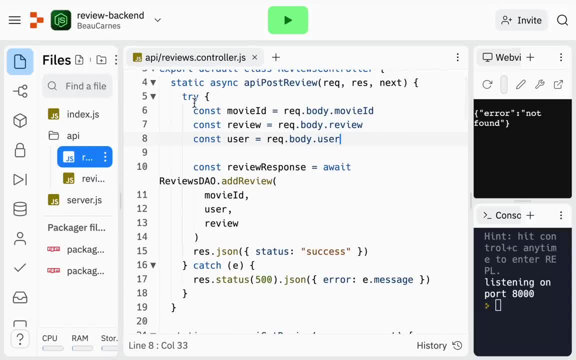 the review. So- and right now we can see that we're doing a try catch, So we're going to try to do all these things. And it's going to try to do all these things And if there's an error, it will catch the error and it will respond. So right now we're just trying all these things And 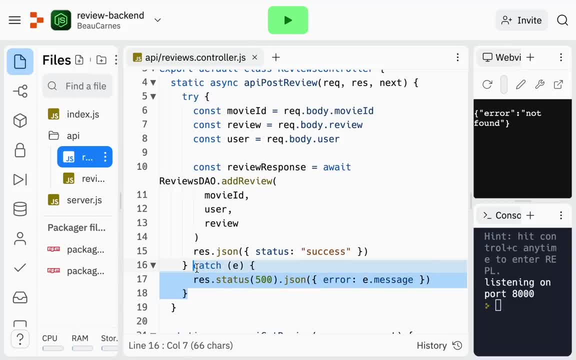 if it's there's no error, then it never does. the never catches the error. So first we get access to these variables- the movie ID, the review and the user- And now this is where we add the review. So we're creating a variable. 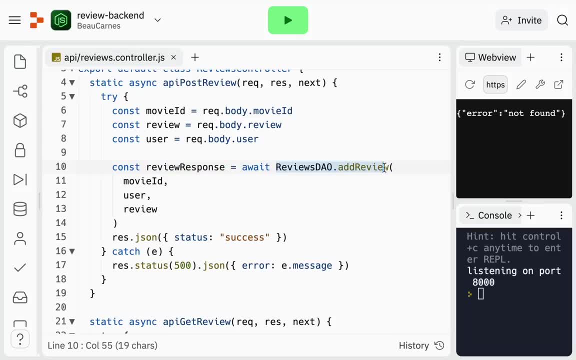 review response. we're awaiting the result of this, which we we have to create this. So the reviews dow dot, add review. we're throwing in all the different information And then we are responding to res dot JSON. Remember, before we respond with Hello World, Now we're responding with a JSON that says static success And if we 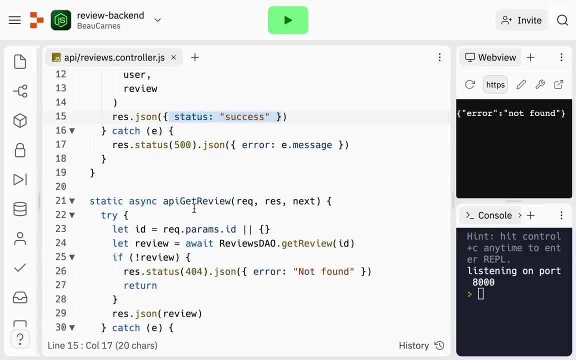 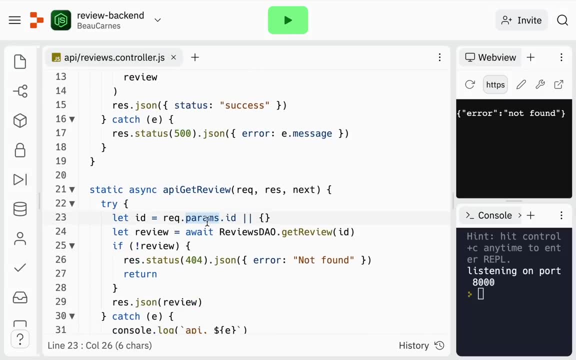 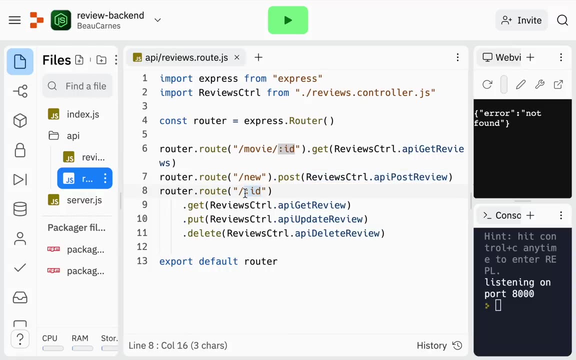 go down. a lot of these things are pretty similar, So there are some things different. So now, here was all that wrecked up body. Now we're doing wrecked up params. If you do wrecked up params, then let's go back to the route file. That's where we get this right here. This is a param, So a body. 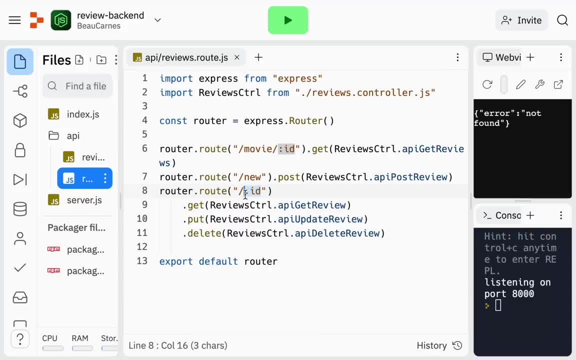 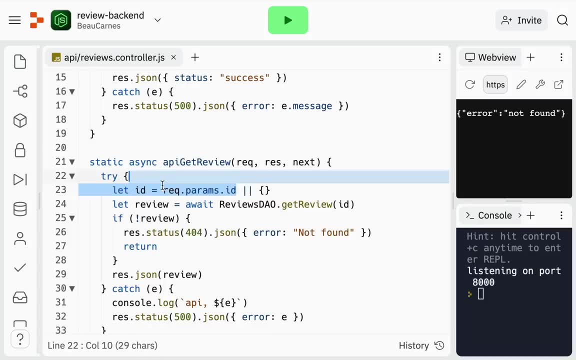 is actually some JSON that you include, But the params you can get it right from the, the URL. there's just different ways of getting information, So we got it's. either we're gonna either get the ID or it's just going to be an empty object And 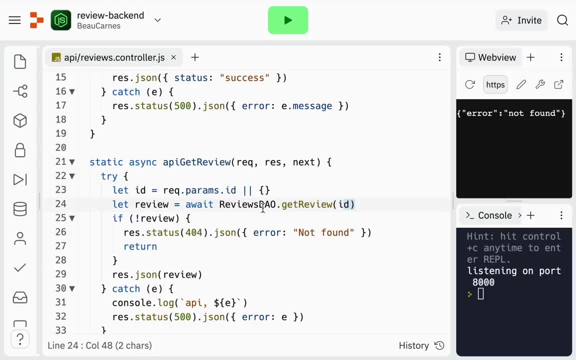 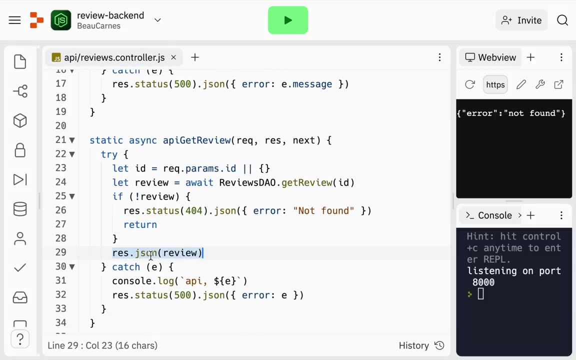 then we are going to get the review. we're passing in the ID that we want the review And if there is no review then we respond with not found and then we just return from the function. But if we haven't returned from the function then we'll respond with the review. we'll give back JSON of. 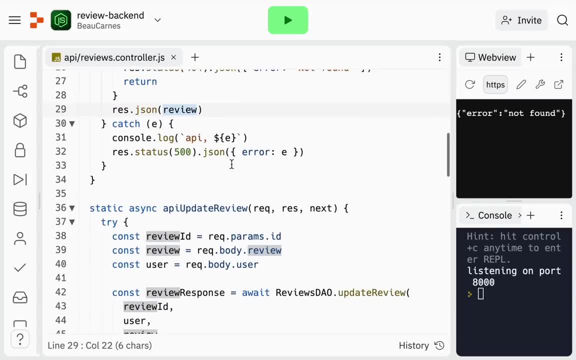 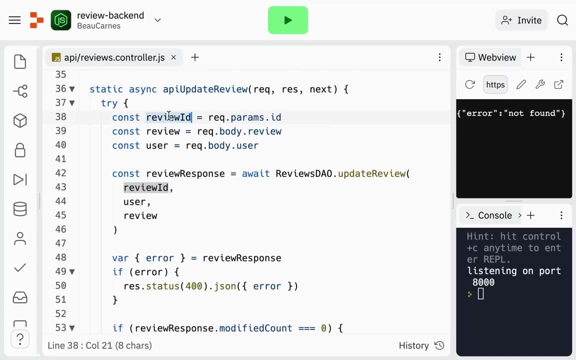 the review that we're trying to get based on the ID, And then you can see that it would also log an error. And then here to update the review. Well, first we have to get access to the review ID. This is from wrecked up params, But the actual review and the user are from the body. Now 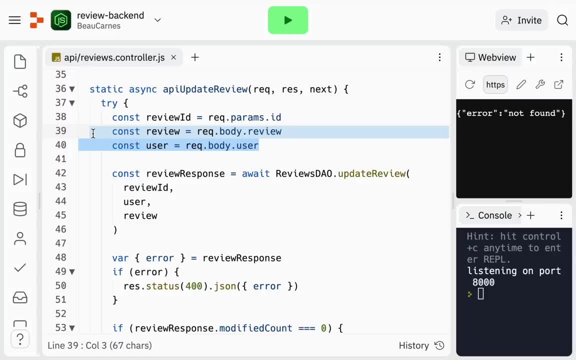 when we test this out, you'll see exactly how this works, how you can give data with the parameter and how you can give data in body, in the body, when we're when we're testing this out later. So then we're going to update the review. revamp used out, update review. this is a function we still have to. 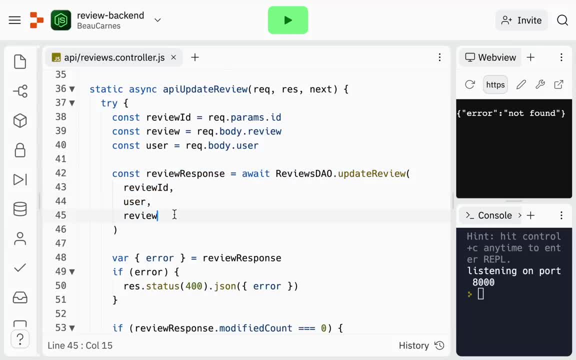 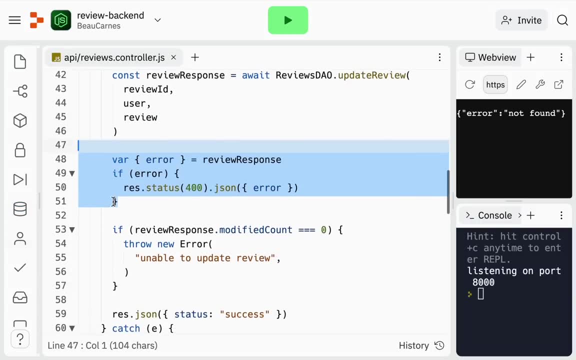 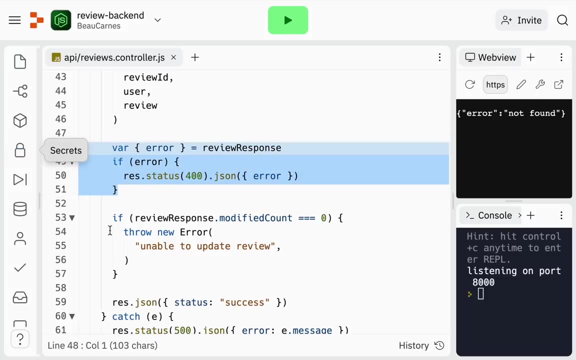 create. we pass in the information, the review ID of the user and the review, And then if there could be an error or there could be, basically these are just two ways there could be an error. So this is one way there could be an error. This is another way it can be an error. basically, 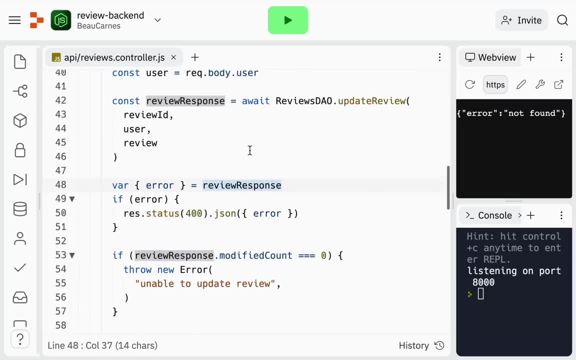 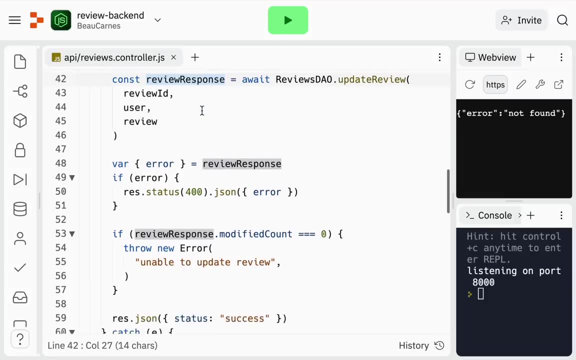 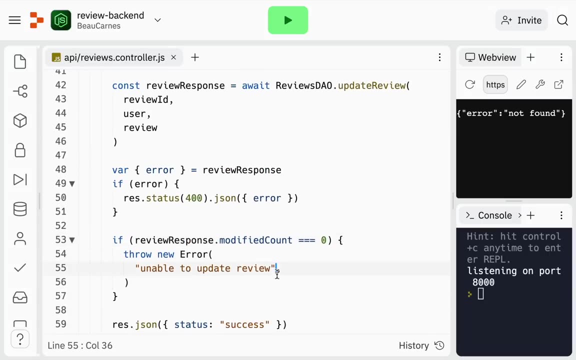 if nothing was modified. so there's going to be response here That's coming directly from MongoDB. there's gonna be a response from MongoDB And if the modified count equals zero, that means nothing was changed, And then we'll just we'll create an error, throw new error. this is creating a new error unable to 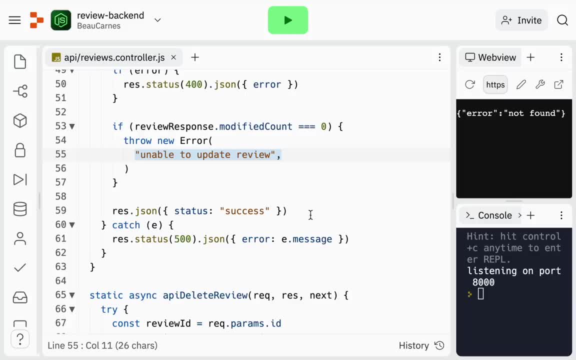 update, review. So if there's not an error, then we come down here where we do the, we respond with the JSON success And if there was, if we did throw an error, if this error happened, then that error is going to get to this catch block here which is going to just respond saying what the error is. 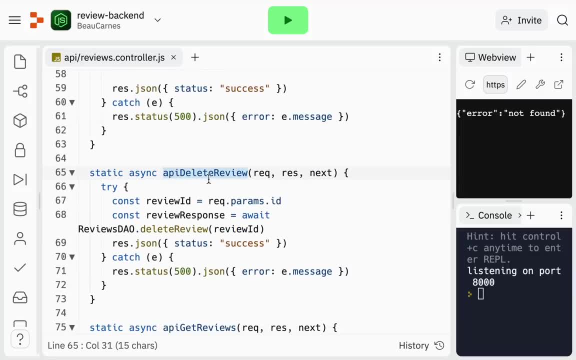 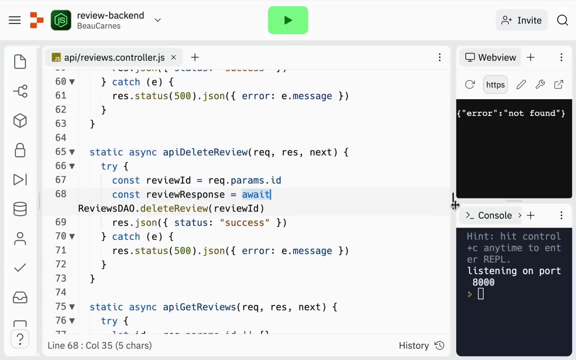 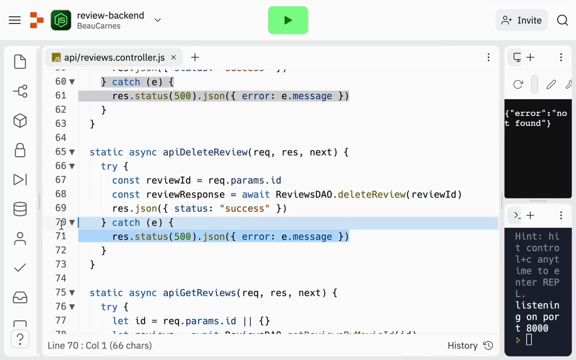 okay, then the next few are pretty similar: delete review. Here we only need an ID. we're getting the ID parameter And then we are awaiting calling reviews down that delete review. we're passing in the ID and it's either going to be successful or there's going to be an error. 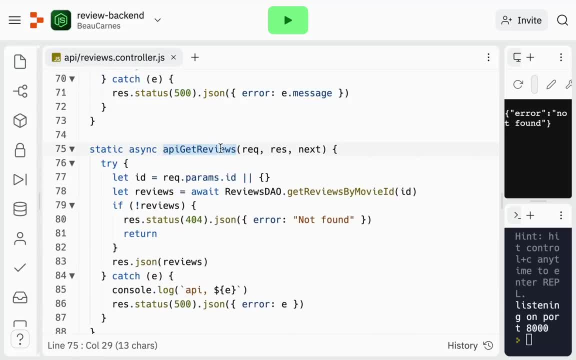 And then the final one get reviews. So this is slightly different, because we're getting a list of all reviews And then we're going to pass in an error, And then we're going to pass in an error, And so the ID here is not the review ID, but is the movie ID, And this we're going to be calling. 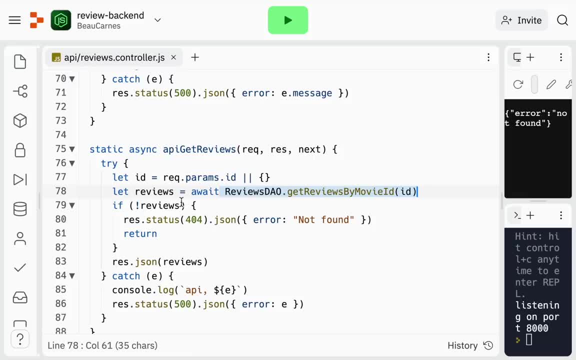 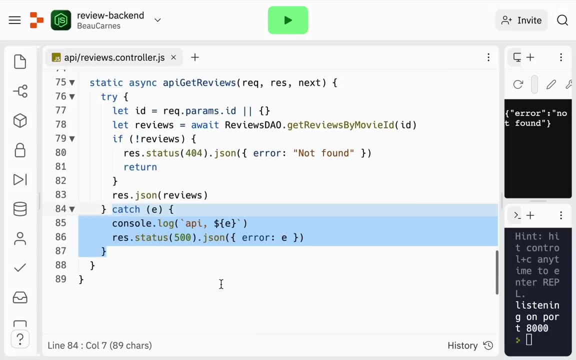 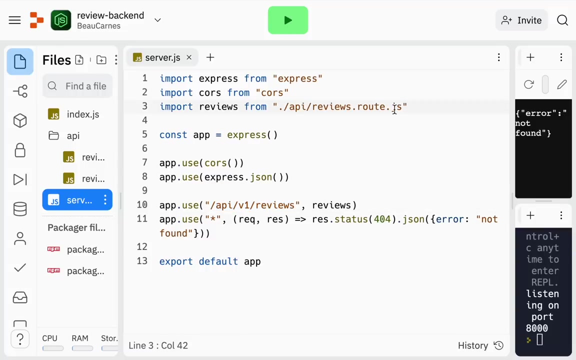 the reviews dot get movies ID, And if there's no reviews, then we'll say not found, or else we're going to respond with the reviews. So or there could be another error that will then log here. Okay, so now let's create our final file Now. we already referenced the file here And since, since we 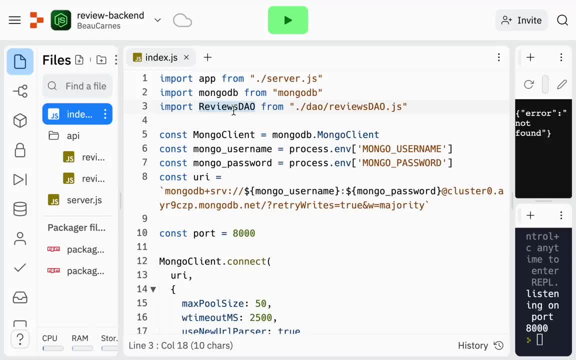 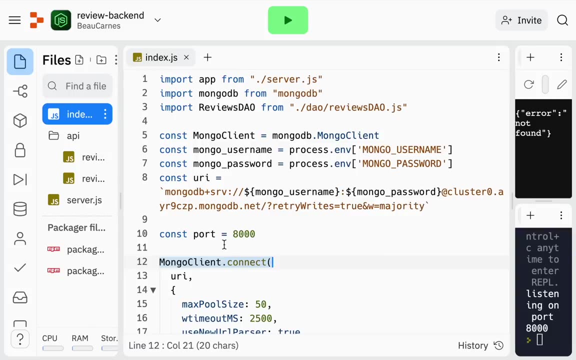 referenced it, let's let's use the file before, So we put in here but we haven't actually used it in our indexjs. So basically, the reviews Dow is where we're actually interacting with the database, But we connect to the database an indexjs, So we have to somehow send the database. 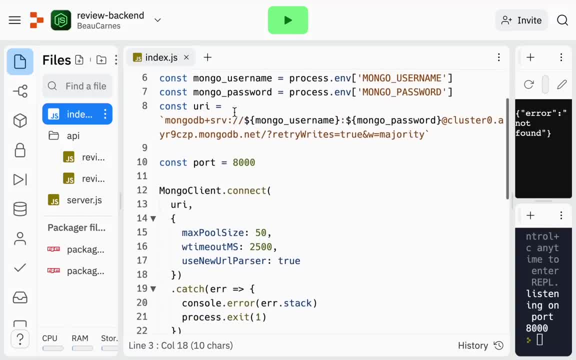 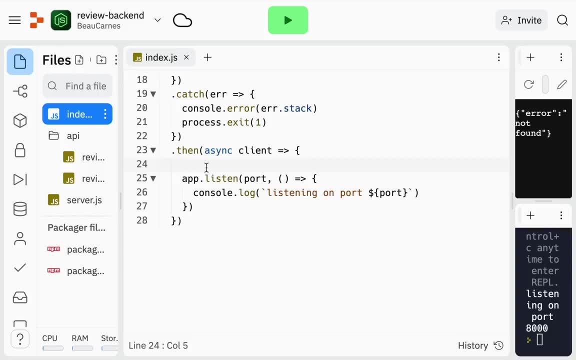 connection to the reviews down, which we'll do down here. So, right before we start listening, we're going to basically connect this together. So await reviews. Dow dot, inject DB. Now this is a function we have to create that we'll see just a second. So we're going to inject the client. 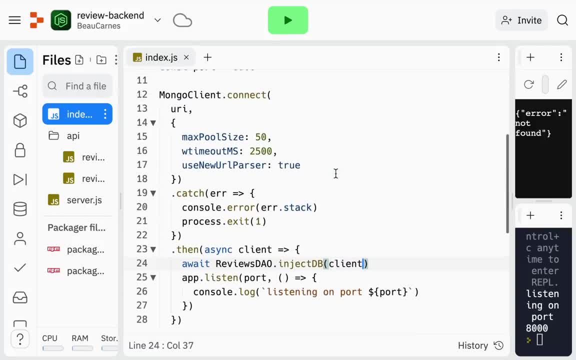 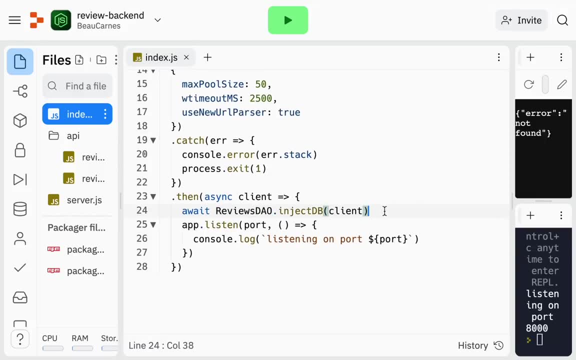 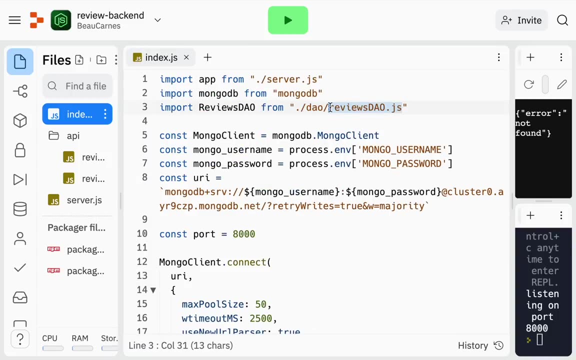 Basically, this is just a way to send our database connection to the reviews down. that was within we can use to access the database. So let's actually create that Now. we can see that slash, now slash reviews datajs. So I'm going to 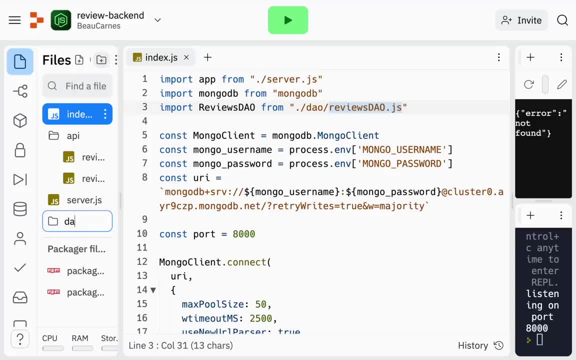 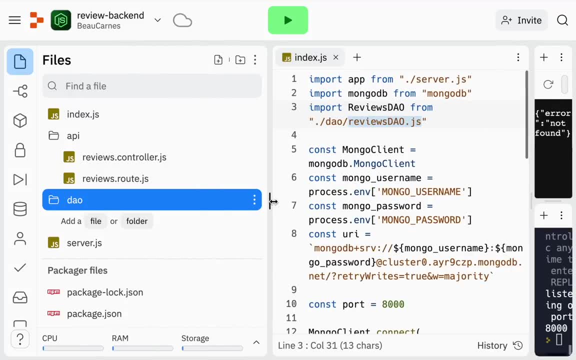 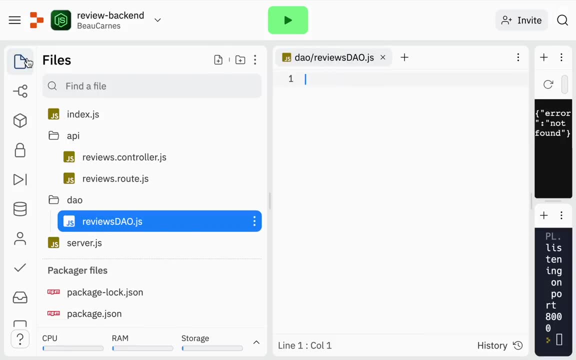 create that. now. I will create a new folder called da Oh, and then I will create a new file called you can see, I just paste that in there. Oh there, There it goes. reviews dow dot j s. Okay, we're now going to see how to actually connect to the database. we actually haven't yet. 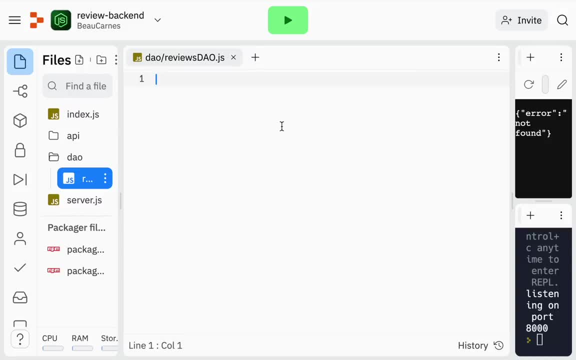 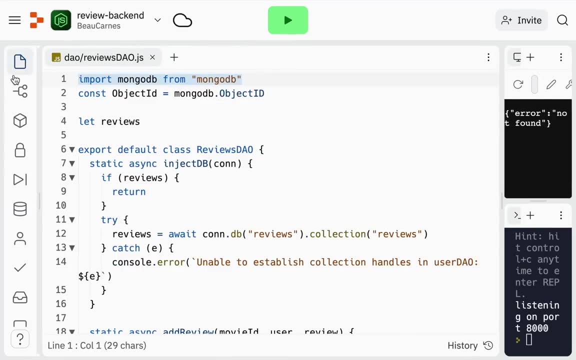 connected to MongoDB yet, And this is where it all happens. So again, I'm going to paste in some code And then we're going to talk about it. Well, first we're going to import MongoDB. That's important because we are using the MongoDB JavaScript. 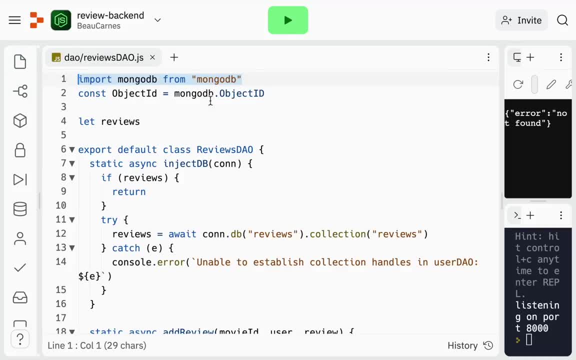 library to access MongoDB. Now from MongoDB we're going to get access to object ID. Basically we're going to be sending and receiving text and integers from our back end to our database, But our database can't for when we're actually searching for a record in our database. 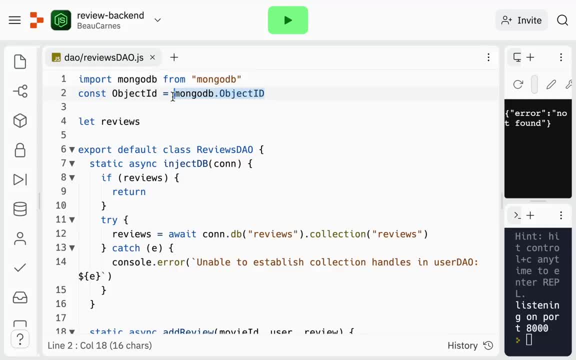 by ID. we can't just search by a integer or a string. we have to actually search by a specific data type called object ID, Which is different than a string or integer. So we're going to convert our, our string or integer into an object ID when we send the ID to the database, so the database will be able to. 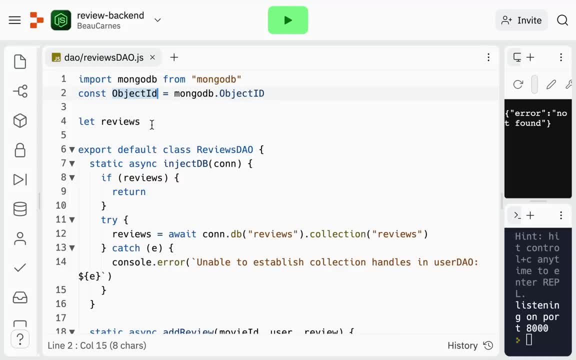 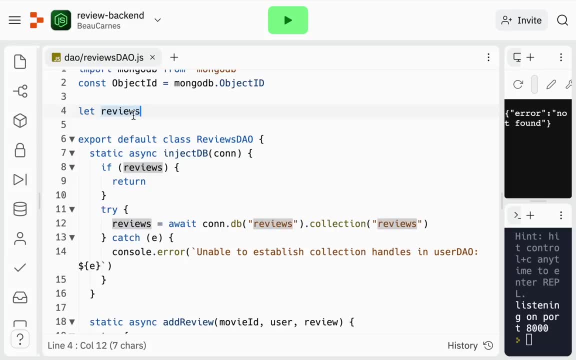 correctly. look up a record Now. you'll see how that works in just a minute here. So first we're going to create reviews. that says let reviews. that means we're creating a variable called reviews. that we haven't put into where we've created the variable but we have not assigned the variable to. 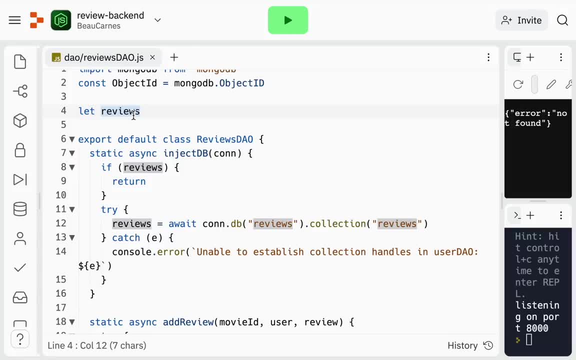 anything, But this is where we're going to assign our, basically our, connection to the database. So remember we call the index inject DB function. Well, first of all, we can see that we're exporting this class reviews down, So we can do reviews down dot inject DB because it's a static. 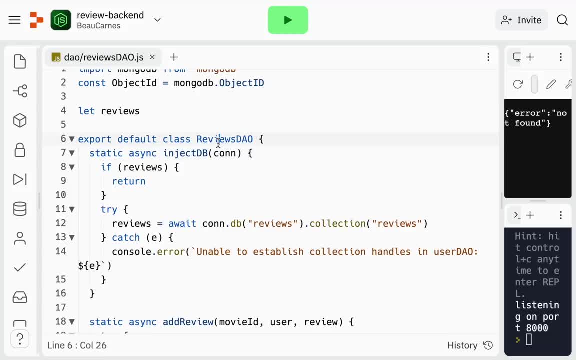 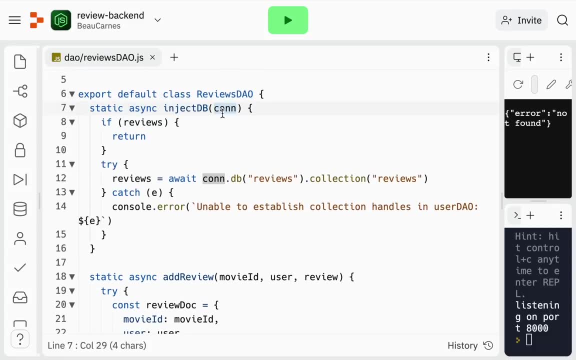 that means we don't have to instantiate the class before we call the function. So we are getting a connection. that's the connection that that we got in the other file, And if there's already, it says if reviews return. that means if there's already a database connection. 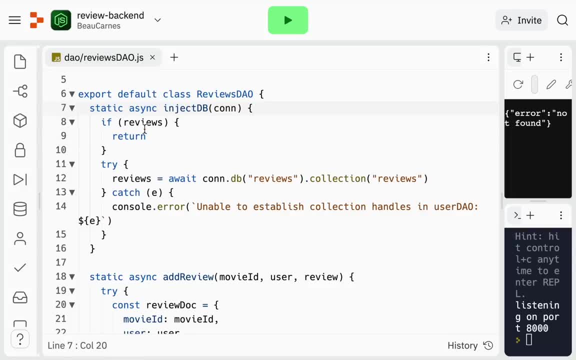 don't inject, don't, don't do anything, But if there's not the database connection, we're going to try this. So there's a try catch block. So first we're gonna try this. if there's an error, we do what's next. So this is specifically right from the, the MongoDB a. 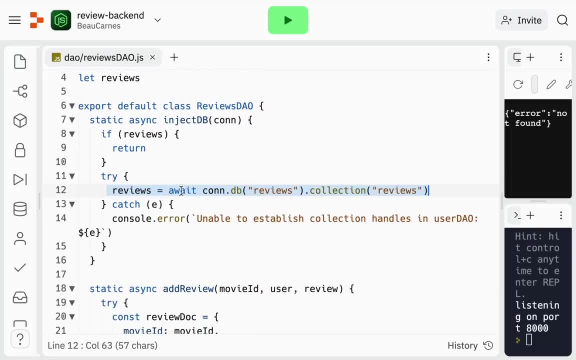 JavaScript library. So we're going to wait for the database connection. So the here's the connection that we got from the other file And then we're going to first get the DB, the database called reviews, and then we're going to get the collection called reviews, Now MongoDB database. 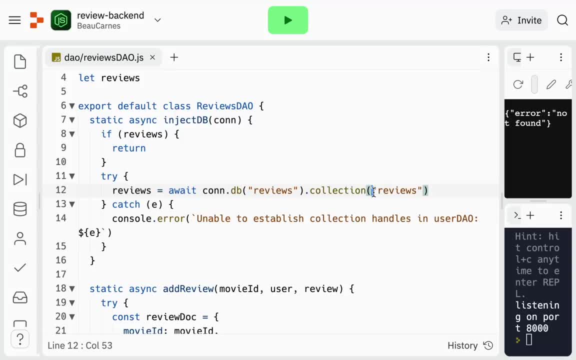 has like that on the top level, you have your database and you can have multiple collections in the database. Now, it's not. you can. we could name these anything we want, But since all this is just reviews, I just named the database reviews and the collection reviews. 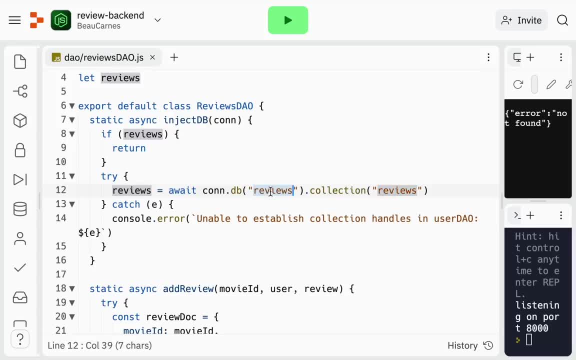 but you can just change this to be anything you want, So you may have, like this could be movies, And then you could have multiple collections. there could be a reviews collection, you could have the movie information collection, you could have the. 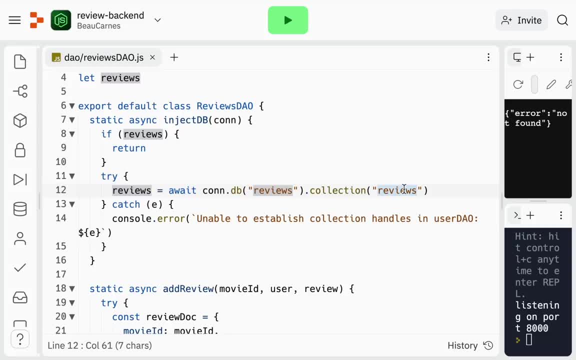 I don't know- movie posters collection, So you can have a bunch of collections And a collection is basically what you would think of as a database. So it's like a bunch of smaller databases within the overarching database. You'll see what I mean later, once we actually see what this looks like. 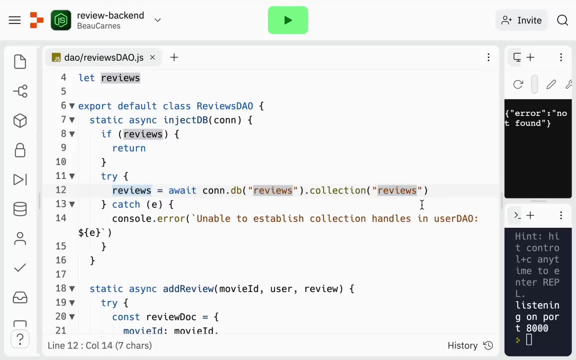 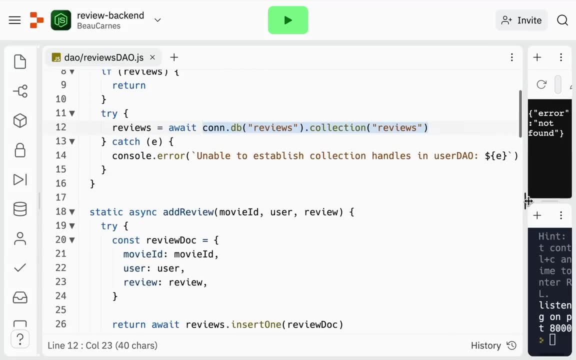 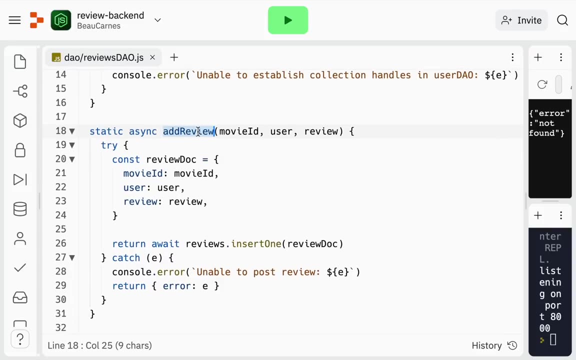 MongoDB Atlas. So basically, we're getting access to our database. Okay, so now the rest of the functions here are all doing something with the database, So we can add, review, And so all these fun, all these functions are functions that we already called. 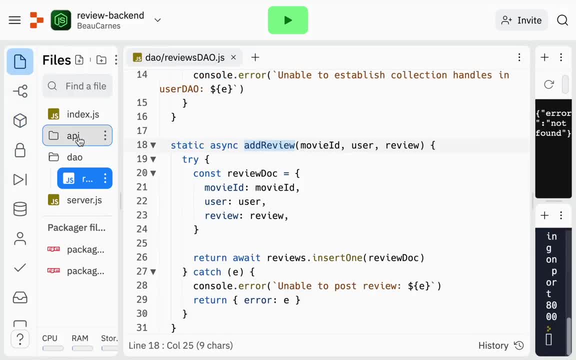 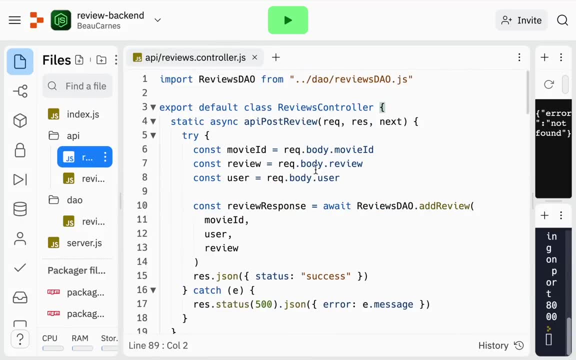 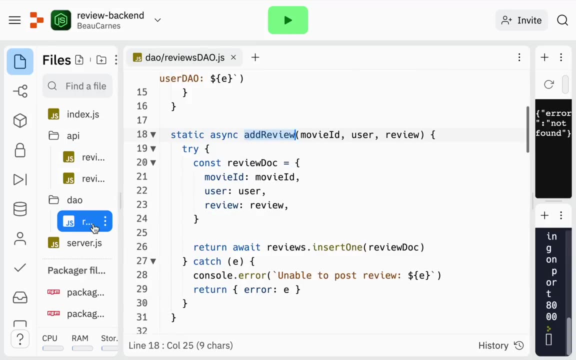 in our other file. So if we just go back over there really quick- So for instance we have our ad review, we're just passed in the movie ID, a user and the review. So we go back here. we are now going to receive the movie ID, user and review. So first, 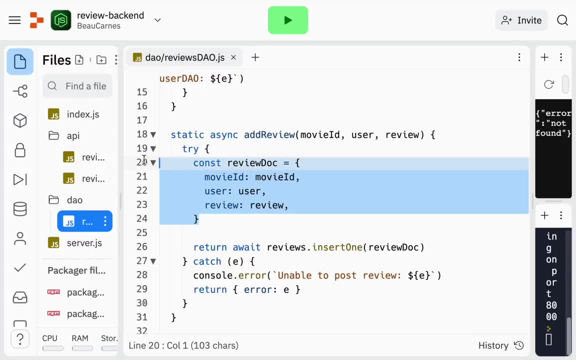 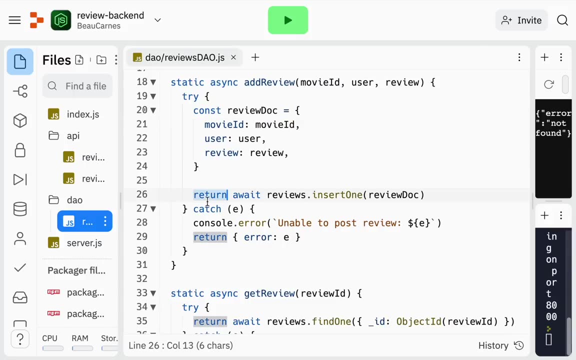 we're going to create our document. this is basically our database entry, And it's going to be a JavaScript object with the movie ID. So these are the key value, key value, key value. Now, we are now going to return from this function. what happens when we? 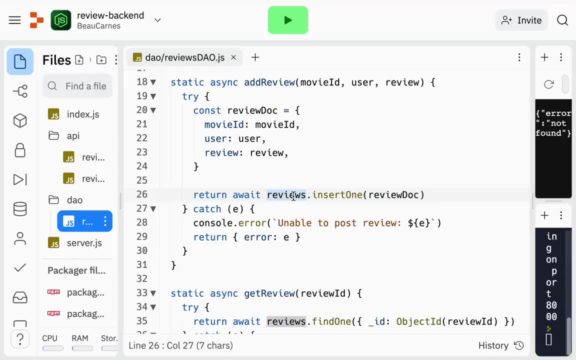 await this to happen. So reviews, that's our database insert one. insert one is a MongoDB command And it's how you insert a document into the database And we're inserting review doc. So that's pretty simple And then we can catch. if there's an error we'll see unable to post. 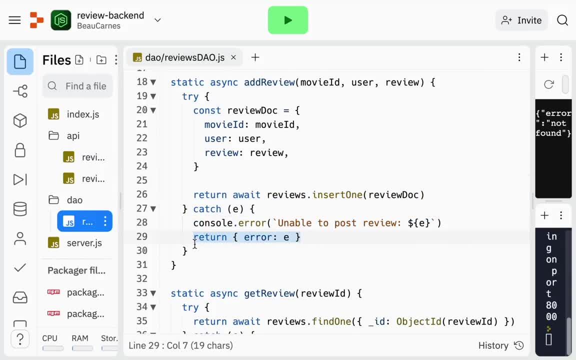 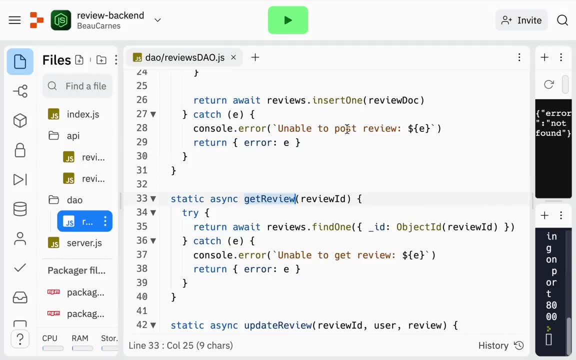 post review: a list error and that's going to return the error. Okay, now to get a review instead of inserting one. we're going to find one, And if you're going to find a document in a MongoDB database, you have to find it. you have to say what you're going to be searching for, the document. 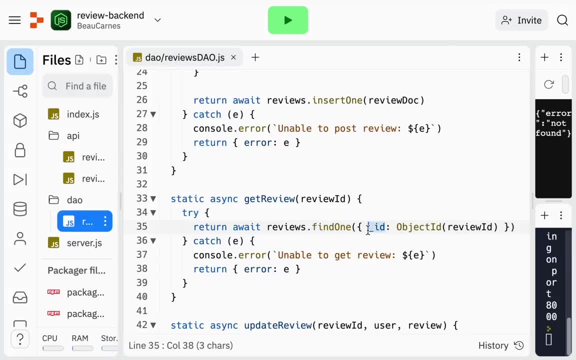 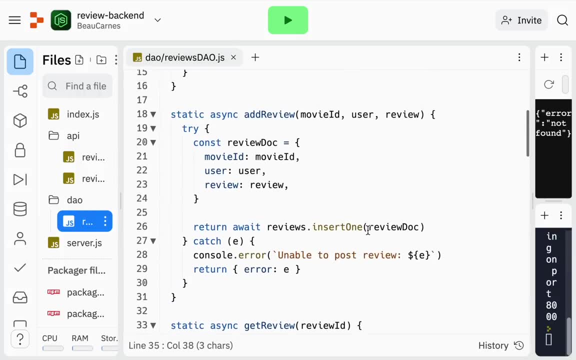 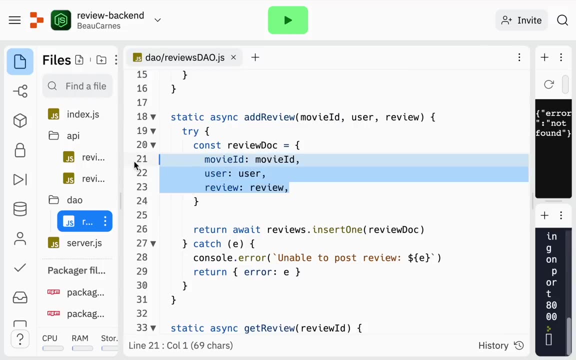 by. it's very common to search by the ID. By default there's a single. every ID is different. So and these IDs are created automatically. So when we, when we created our document, the movie ID is not the ID. the ID was created automatically when we create the document. So if 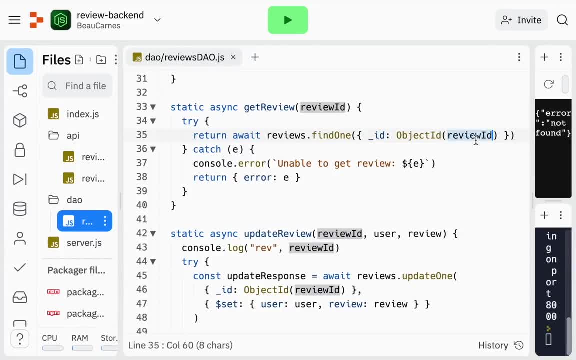 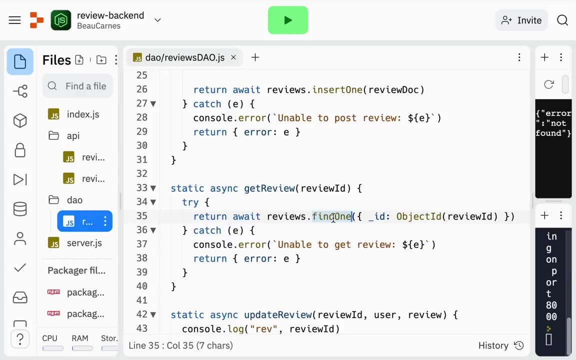 we know the ID. we can now search by the ID. Now review ID. this is coming in as a, as a, basically a. it's probably coming in as a string, But we're using object ID. that's from here to convert it, to convert the string to an object ID that we can then use with the fine we can find. 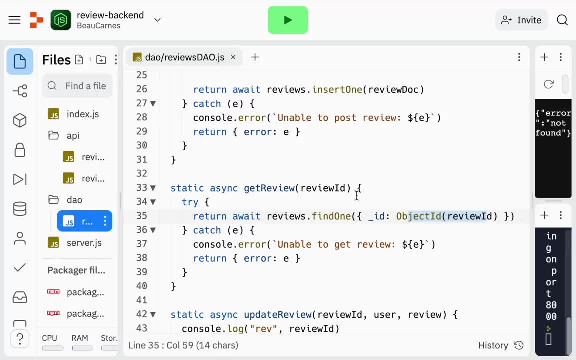 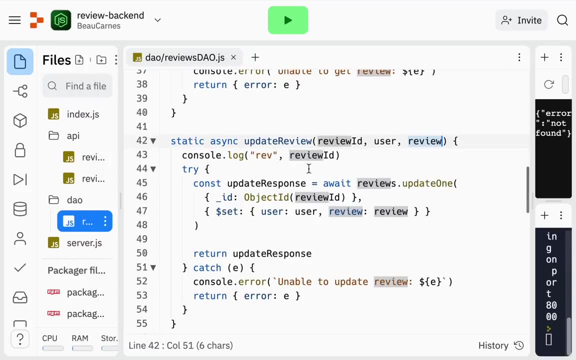 the ID that has the object ID of the ID that we passed in and if there's an error we catch the error And then same with update review. we pass in the review ID, the user and the review and we don't need this console, that log. this is a test out thing I was doing earlier. 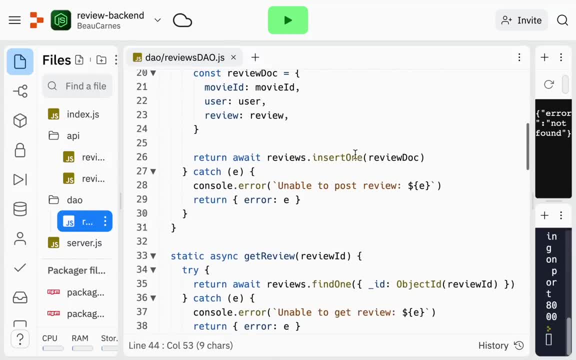 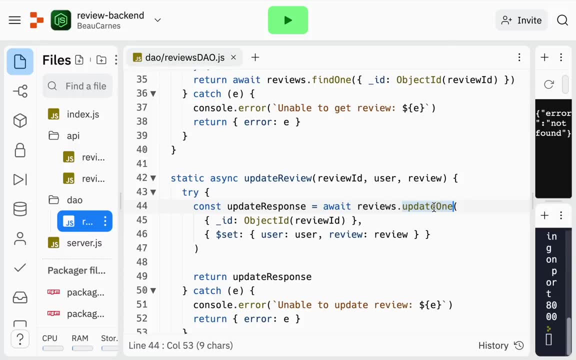 So now we can update one. so so we basically have insert one, find one, update one, And when you're updating one, it's like a combination of a find and basically create the putting the information. So so we're passing in two things. So when you're updating one, it's like collecting the servi, the. 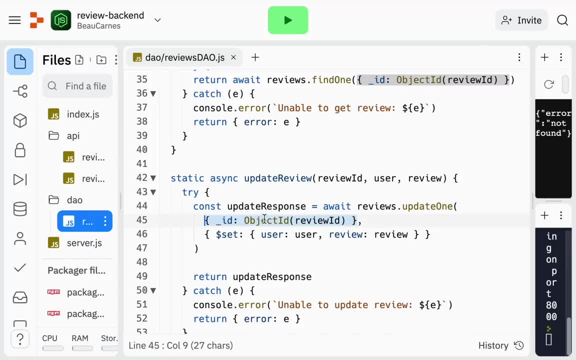 link. then what we do is we do a training order And then we do our analytics report. So you'll see the. So first is the object which get says what we're searching for. So we're we're finding, we're trying to find the document with that review ID. that's the one we're going to update And this: 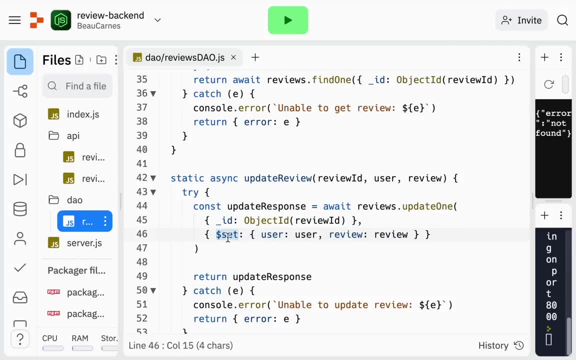 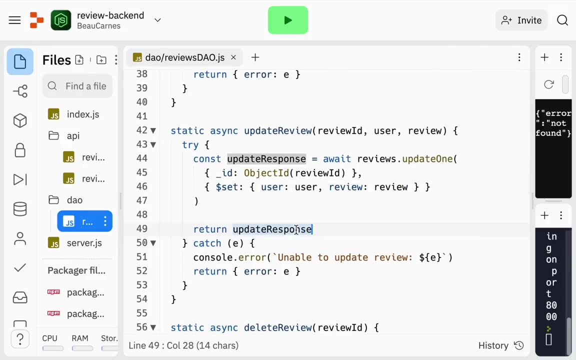 is how we're going to update it. we are going to set, So you're gonna have to- this is just something specific to MongoDB. you're gonna have to set a user to be the user and set the review to be the review, And then we can return the the response that we get, And then we have the air. 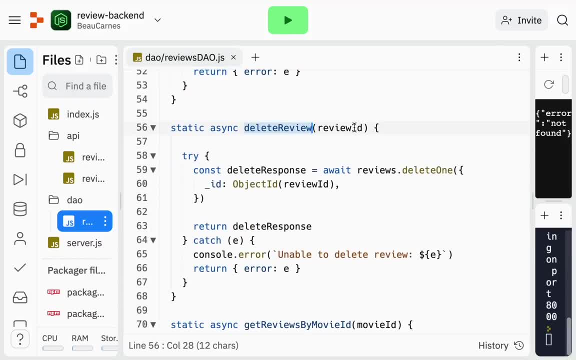 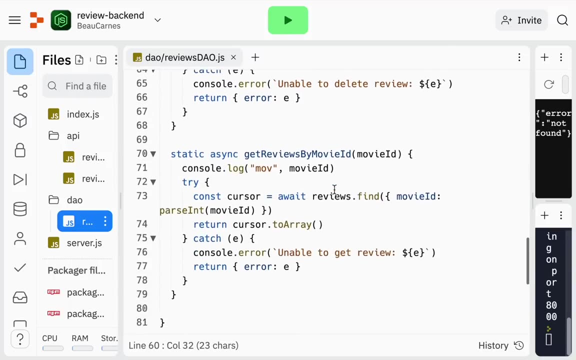 and then finally delete review. So this is just getting an ID, delete one, And this is: we're searching by the object ID to the review ID to find what we're going to delete And then finally get movies by ID. So this time we're at. 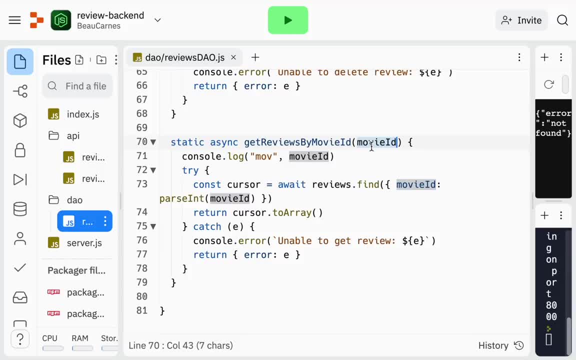 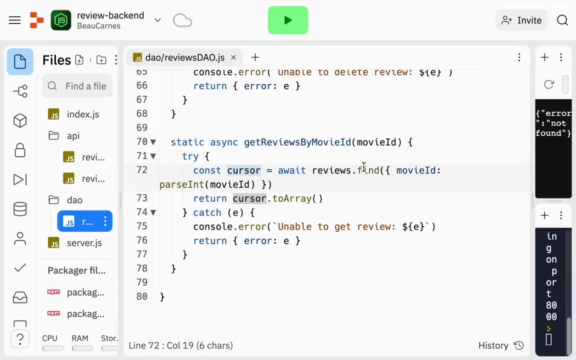 we have a movie ID. this isn't an object ID, this is basically just an integer that we're passing in And where, again, we don't need this console dot log. So we're going to get a cursor. So this is what, basically: when you find multiple items, it's going to return a cursor and we're 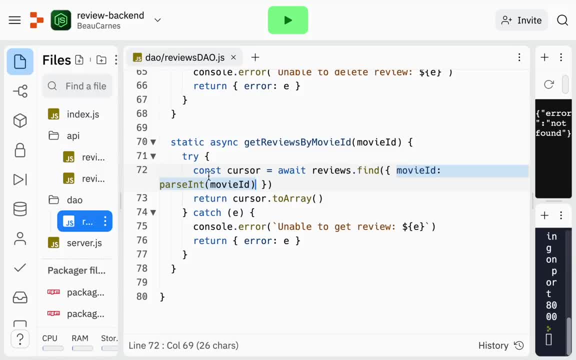 finding every item that has the ID And you can see we are having this part, we're passing in the ID to this poder And then, lastly, here we have- right here- I just cut this pick here, So I'm just going to do this- that he has a couple er sweet, but it's a little bit frustrating. So 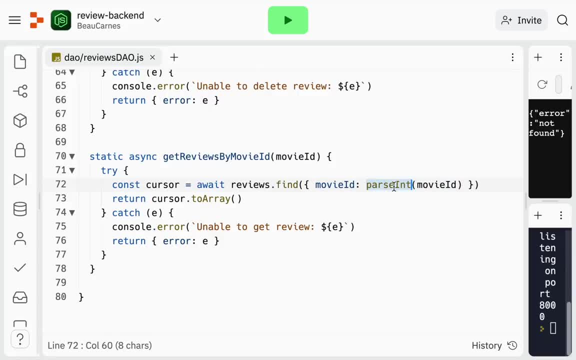 int function. So it's going to be a string but parse int. this is from JavaScript. parse int is a function from JavaScript to convert a string to an integer which we're then going to pass in to our find command of MongoDB. And we need a cursor which is basically just a list of all the 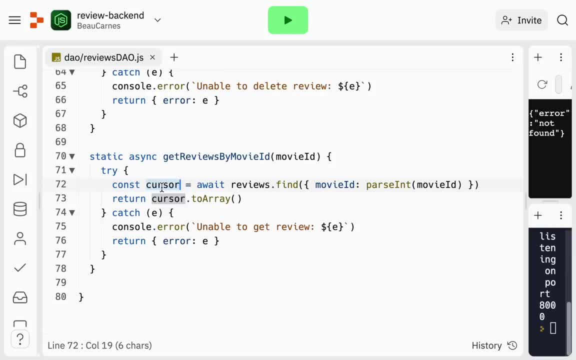 documents, but it's not, then it's not in the format that we want, So we have to convert it to an array. we're going to return cursor dot two array and then it's going to catch an error. Okay, let's try. 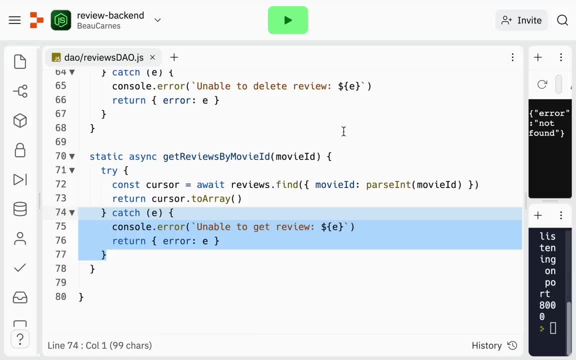 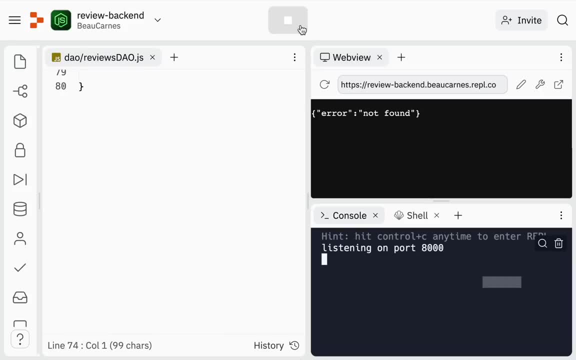 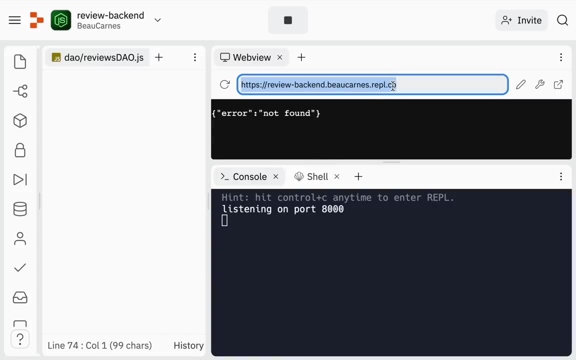 this out. So I am going to bring here. let's just press play here, See if we have any errors. No errors so far. So what I'm going to do is go in to so with this here, basically with a web browser. 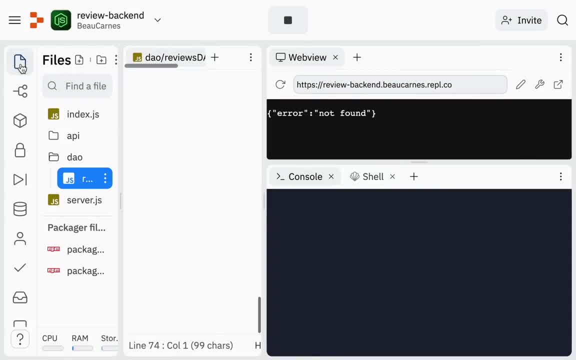 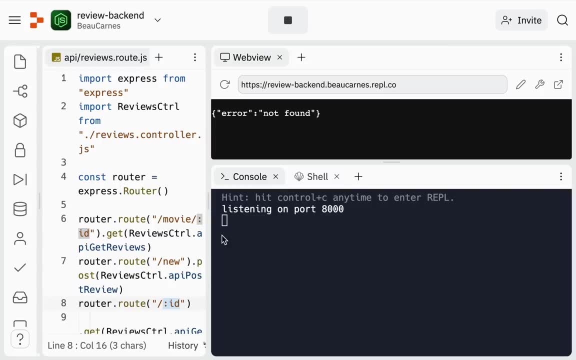 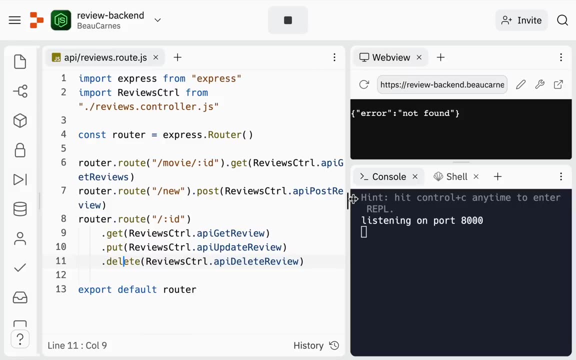 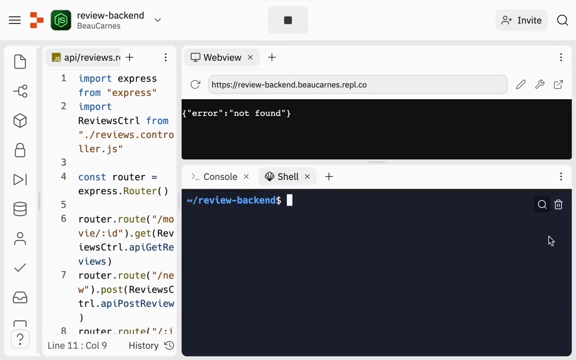 you can only do, get requests. But if you remember, on a route we have a bunch of other types of requests. We have the post request, put requests, delete requests. you need something special to be able to do those types of requests, So we're going to use a common command called curl. Now a lot. 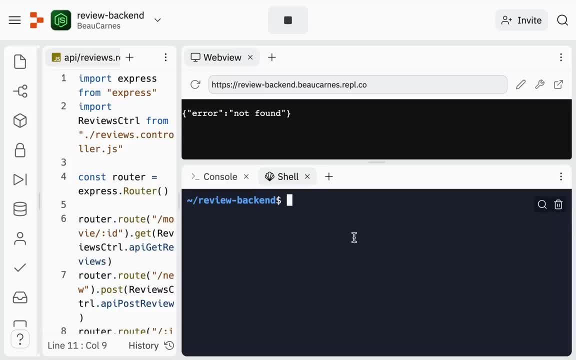 of computers come with curl built in, and replica does also, So we can go to the shell, And we can now run some kernel commands, So the first thing we're going to try to do is to create a review. Before, though, let's go back to MongoDB Atlas. 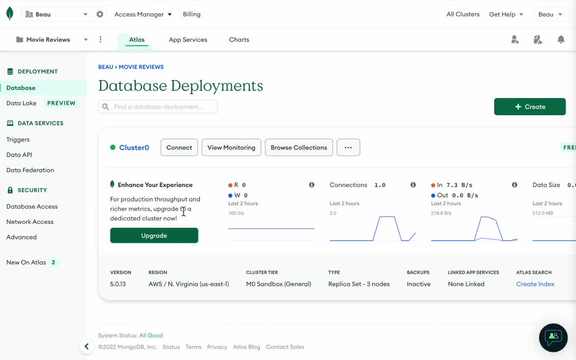 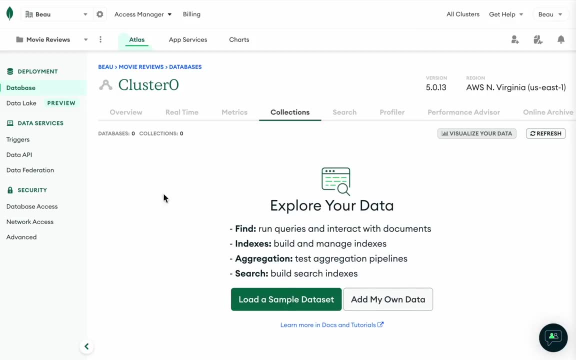 Before we create a review, I'm going to go to browse collection. So we're going to browse all the documents in our database So we can see that for databases we have zero databases, zero collections. So we don't have any information, we don't have any records in our database. But 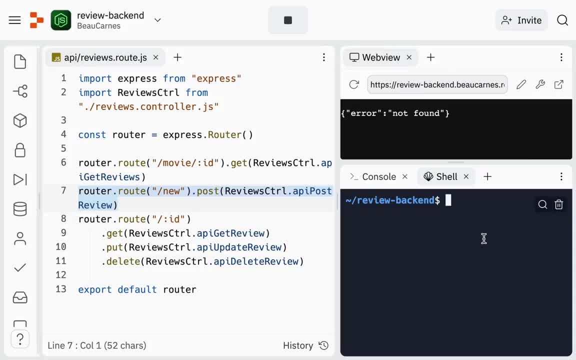 we're about to change that, So I'm gonna go back over here And in my console I'm going to paste in a curl command. Now there's a few different ways we could test this API. We cannot really do with a web browser very easily, because web browsers are mainly dealing with get requests. 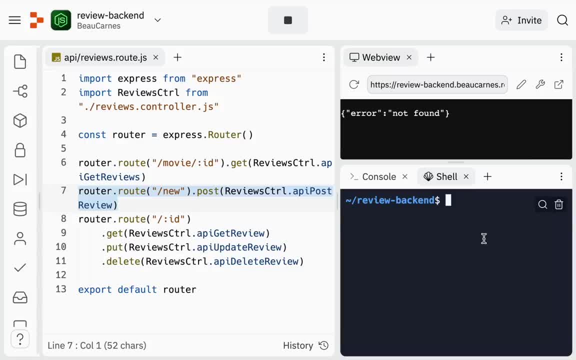 But if you there's some programs such as postman or API or something like that, we're going to go ahead and create a review And we're going to. I think it's called insomnia. you can use to do it more of an in a graphical way, But most 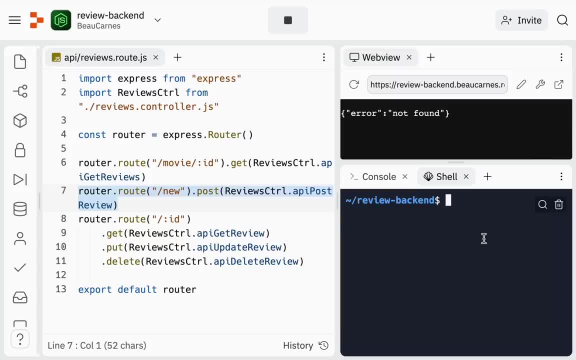 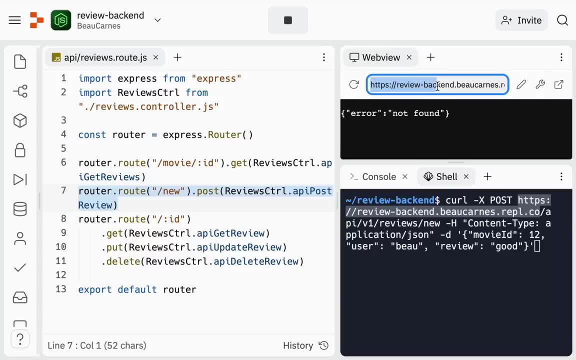 the URL here, So this URL is just coming from up here. And then we have the, the slash API, slash v1, slash reviews- that's our, our key, our base URL. and then slash new- that's right here, our slash new, right here, And we're doing a post request. And now we are going to set the headers. 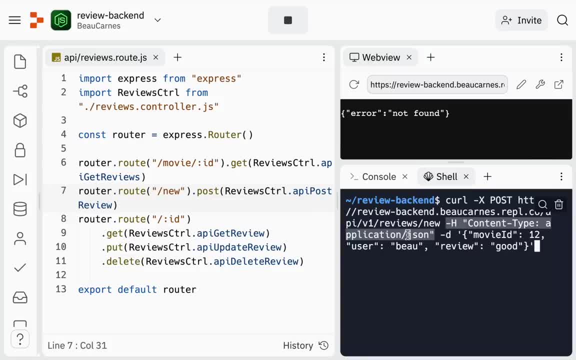 of their quest. So we're going to set the headers. the content type is going to be applicationless- JSON. And now we're going to set the body of the request. So for the body, we need to set the movie ID, we need to set the user. 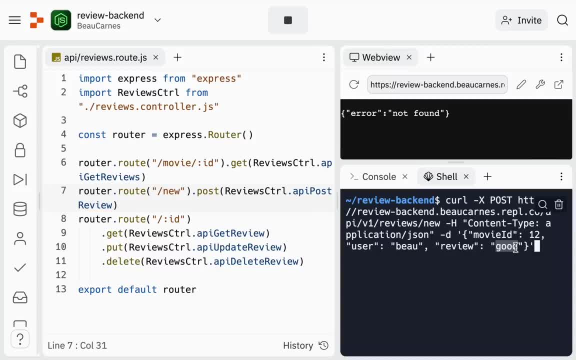 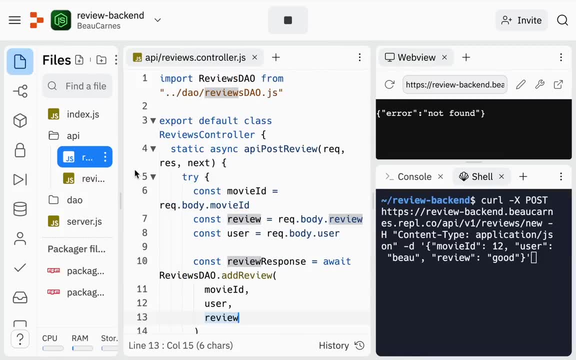 and we need to set the review. So the user is me bow and the reviews is good And the movie ID is just an integer here So you can go back. we can actually go into the file where we use that information In the post review. we're getting the movie ID, the review and the user. 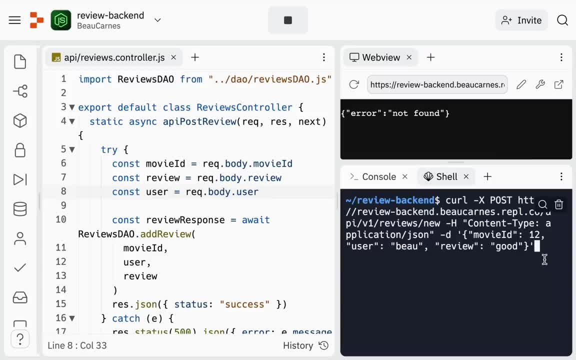 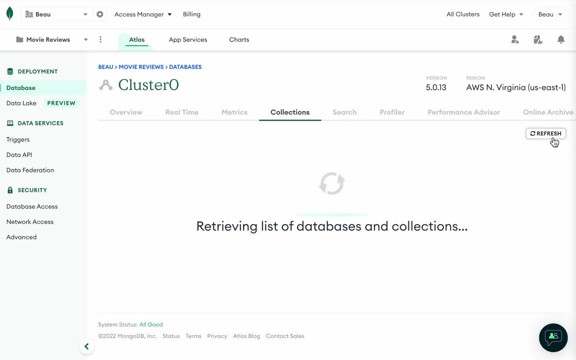 and then we're going to create a movie. So I'm just going to press enter And then we're going to return. It says success. Okay, there's a few different ways we can test that it actually works. But one way is to go right back over here, And now I'm going to click Refresh. You can see. 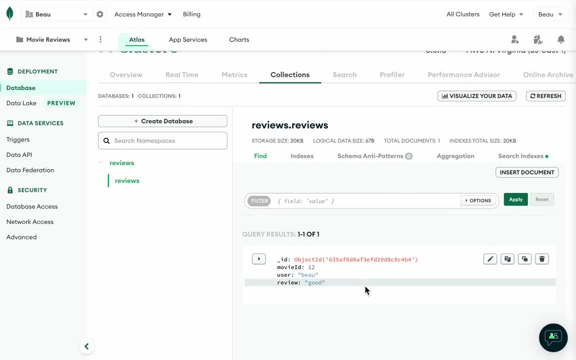 we is now showing the information in our database And we have the movie ID, 12 user, bow and review- good, And we have it created an object ID. So it automatically creates an object ID. Like I said, every ID is different. Well, I'm going to, actually we're going to actually use the object ID, But first, 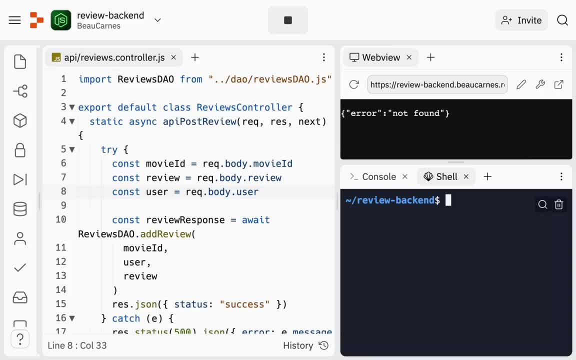 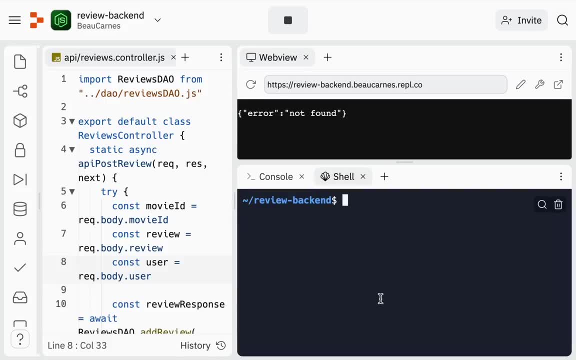 let's go back over here. So let me just clear this again, And we'll make it so you can see more of the console. So let's see if we can get that document that we just created. Oh, let's create a few more documents And then we'll try to get them. So I'm going to do a curl, we'll do same. 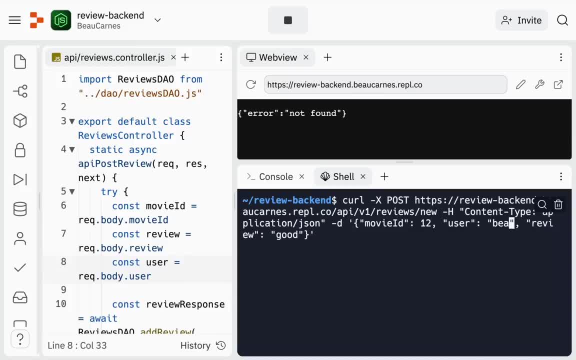 movie ID. we'll do movie ID 12, user, bow and review, And then we'll go back over here And we'll do movie ID 12.. We'll do for the user. we'll do Quincy for the review. Quincy did not like that. 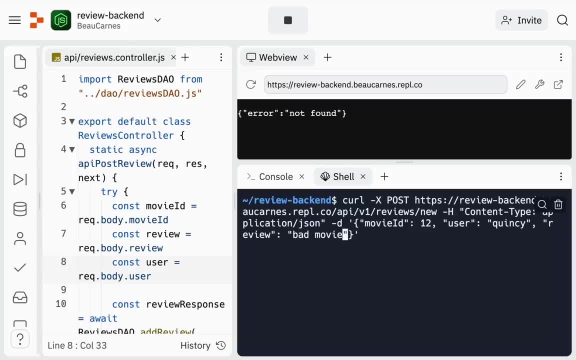 movie, bad movie. That was his review. Okay, let's add one more, And this time we'll do a different movie ID. we'll do movie ID 13. Read- I don't know how this change review: Wait name. 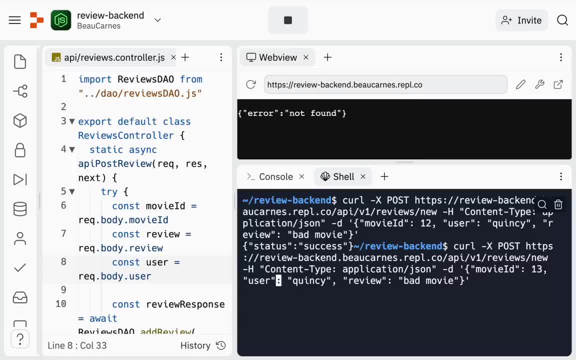 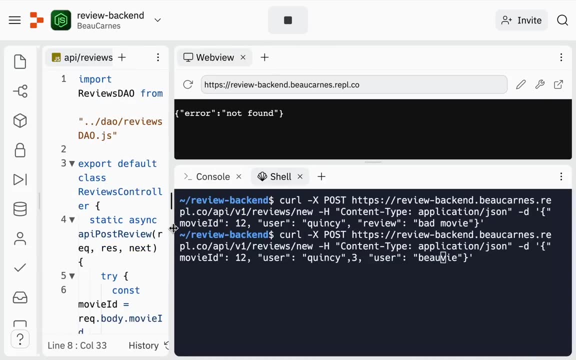 no user. So movie ID 13. User. this time we'll go back to bow. Sometimes the replica console does some weird things When you kind of move it back and forth to update. Let's see movie ID 12. User Quincy: Oh yeah, see, this number kind of got in there. 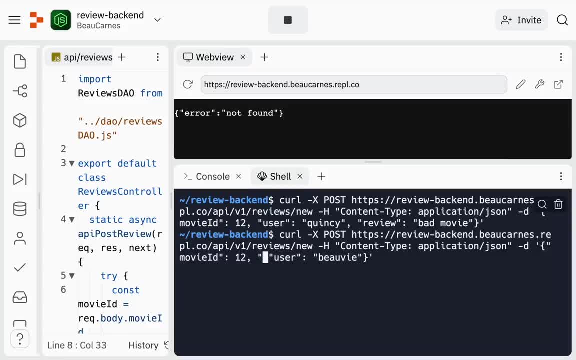 I'm gonna give it a valid date. Okay, I just have to stop that one. I got to anxious. stand up and wait. Okay, that's the user bow And review And We'll be awesome. Okay, let me just see if I've 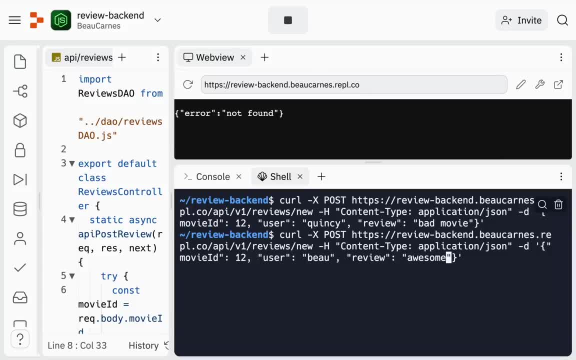 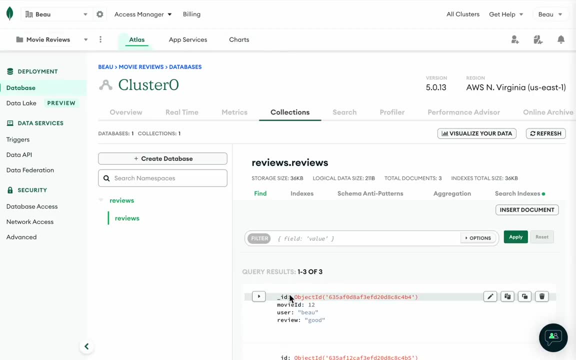 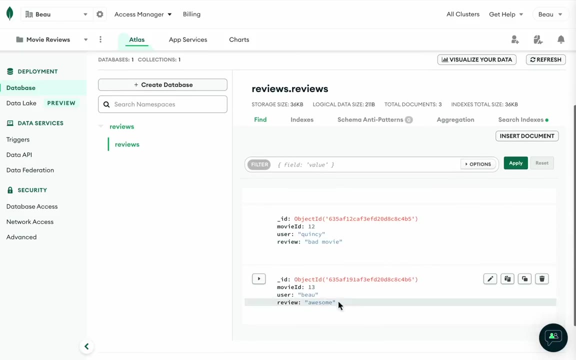 how everything was changing here. I think that's what we want, Oh, except I wanted a different movie ID, Okay, Okay, now let's just check back in here what they look like. So I'm refreshing in here. And we got the first one movie, the movie 12, movie 12, bone Quincy. and then we have another. 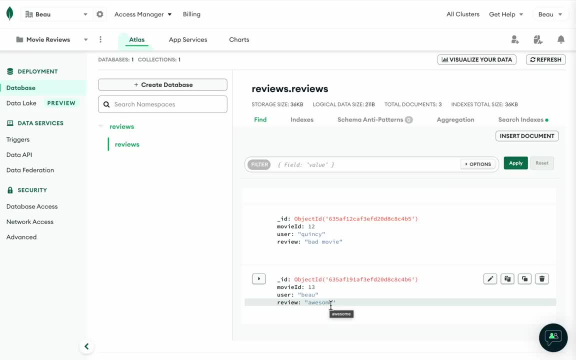 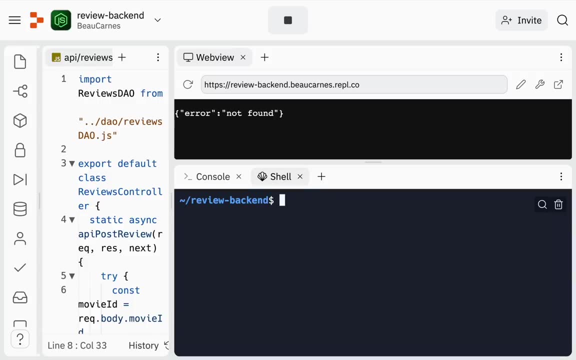 one movie: 13.. Awesome, Okay. now what I'm going to do is go back over here, And now I'm going to make a get request. So let me clear that, And we'll do curl x, get And I'll show you how we can. 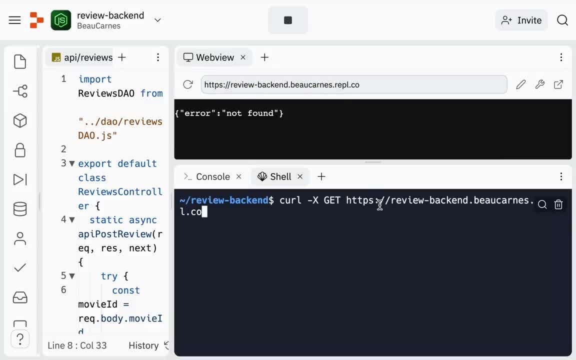 actually just make this instead of just pasting all, and I'm going to copy that, And then I'm going to put slash- was it slash API? slash v one, slash reviews. And this is just going to be a get request, But I'm going to put: 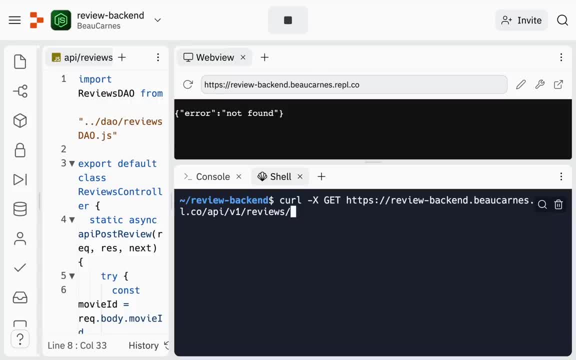 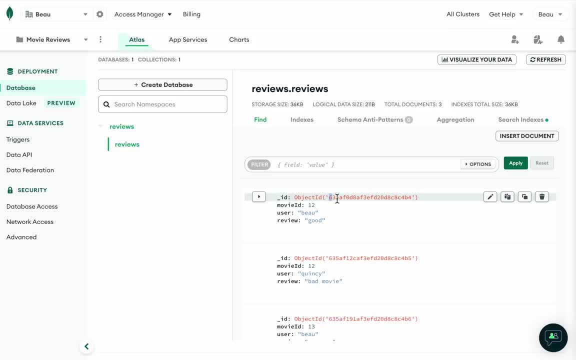 the object ID of the review at the end of this. So I'm going to go back over here, I'm going to copy this idea And let's see if I can get access to this specific URL. So I'm just going to copy. 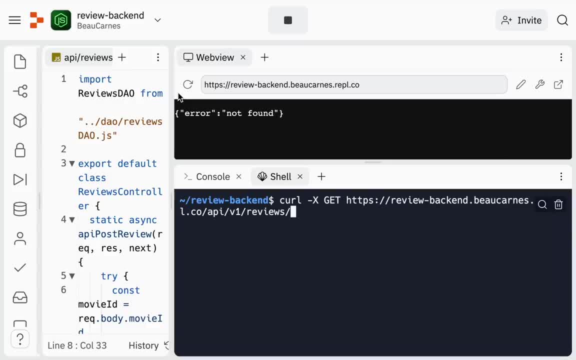 that string and put that in there and return. Okay, we got it. Look, movie ID 12: user bow and the review is good. Okay, now let's see if we can get the reviews for all the reviews for movie 12.. So I'm going to clear that And I'm just going to. this is gonna be a get. 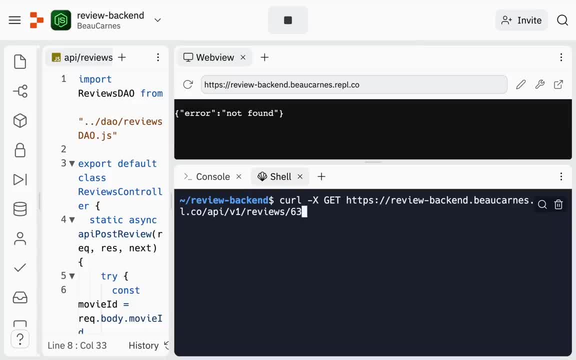 request, But if remember how you do that, we're going to review slash movie, slash 12.. And now we've returned two reviews. So we have user bow review- good. user Quincy review- bad movie. So we just returned all the reviews for movie 12, which was 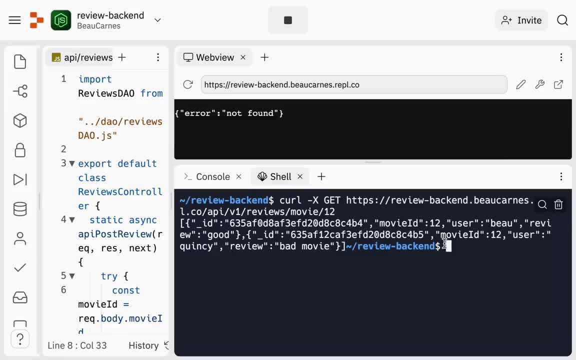 two different reviews. Okay, now let's see how we can change a review. So, to change the review, I'm going to do curl x, put and then I'm going to put the URL I'm actually going to. I'm going to copy most of this, But we have to put the ID so I can get the ID from right here. 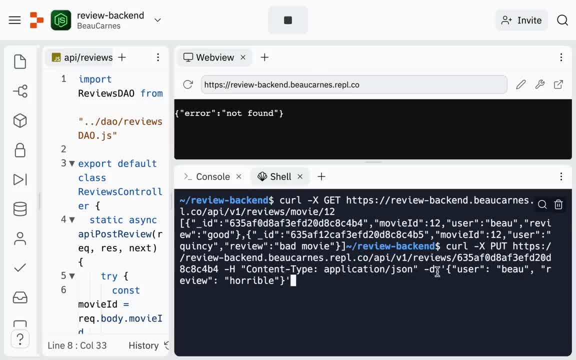 And now I'm going to create this header And I'm going to set the user to bow, which already was like could change the username, But I'm going to leave it the same. And then now the review is going to be horrible. So it used to be good, Now it's gonna be horrible. Okay, now I'm going to go. 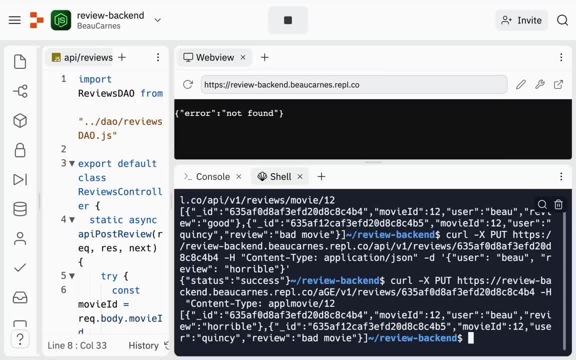 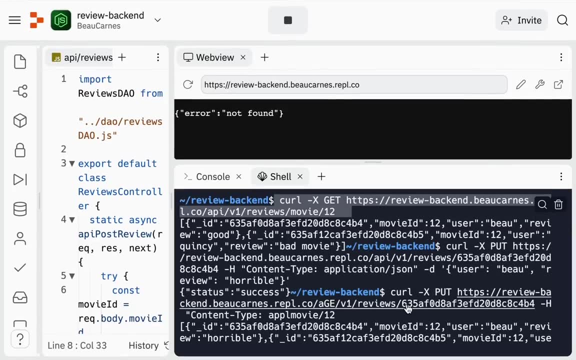 back to where we get all the reviews really quick, And this is something with replica. this is not the command. somehow it knew the correct command, but it didn't display the correct command. right, It was supposed to look like this And it I just 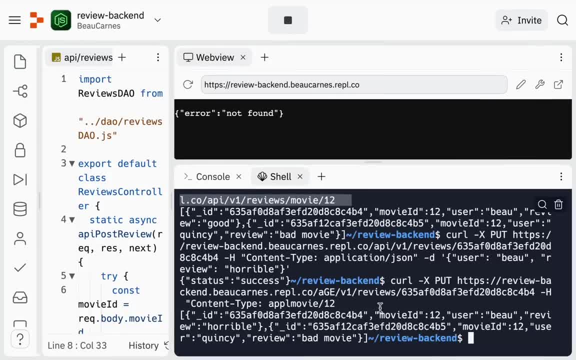 pressed up a few times to get back to the command, But it still was able to press up the correct amount of times to get to that command. And it did run that command, But for some reason it didn't look like that command in the shell. That's okay, it still gave us the correct. 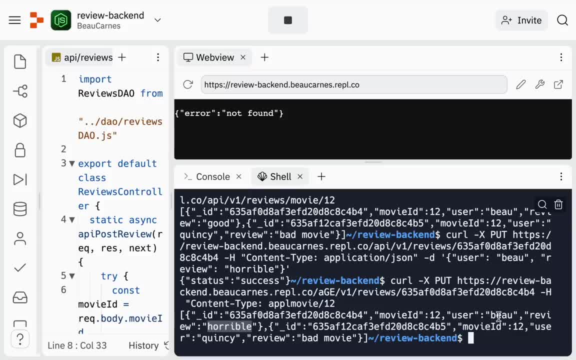 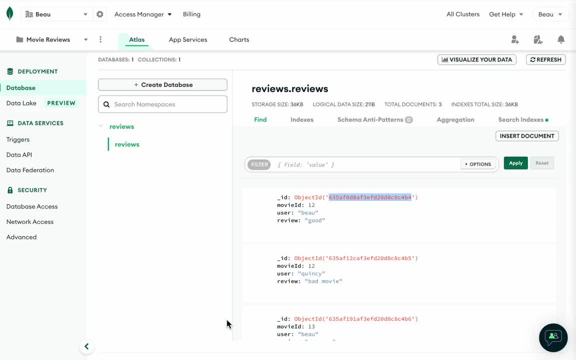 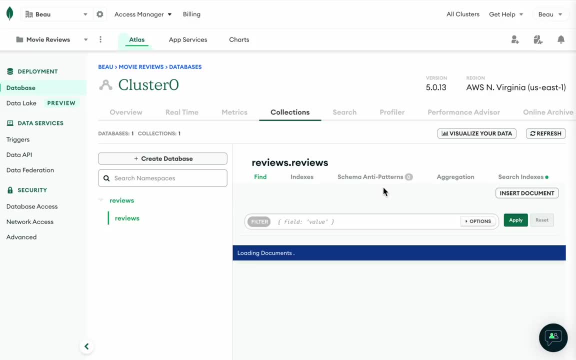 information. Look, bow review is horrible And Quincy review is bad movie, So it's changed to horrible And we can verify by just going back. going here, I'm going to refresh says good, I'll click this Where's I thought there was. Oh, here's the refresh button, here And now. 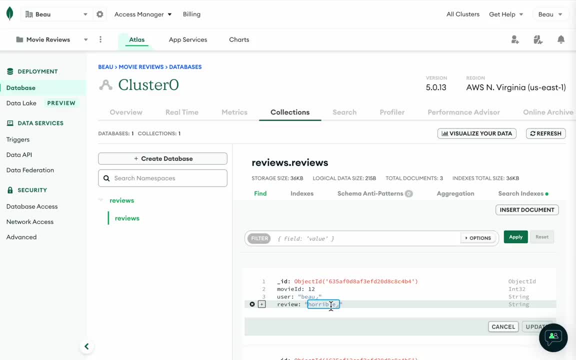 it's horrible. So we've been able to create it. we've been able to create a review, edit a review. look, get a single review, get all the reviews for a movie. Now let's just check the test, the delete one. So for delete, I can. 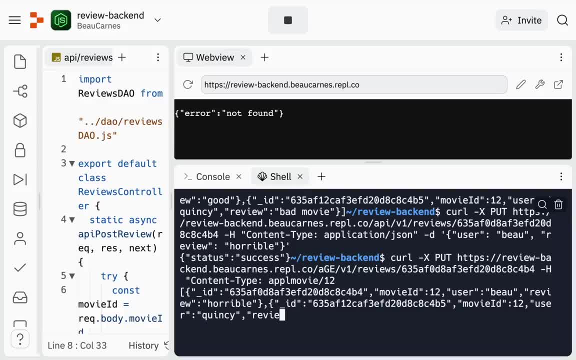 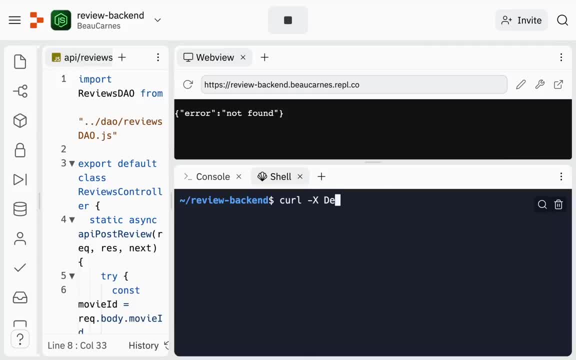 Well, let me just clear that out. So we'll do curl X, delete, And then I'll put the URL, which is that slash API, slash v1, slash reviews, slash, and then I have to get again. I'm just going to go back and just copy this of the one I want to delete: this object ID. 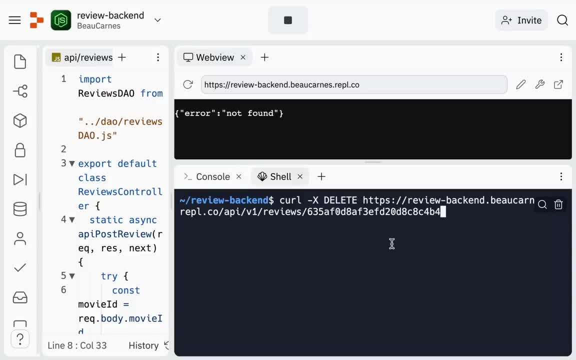 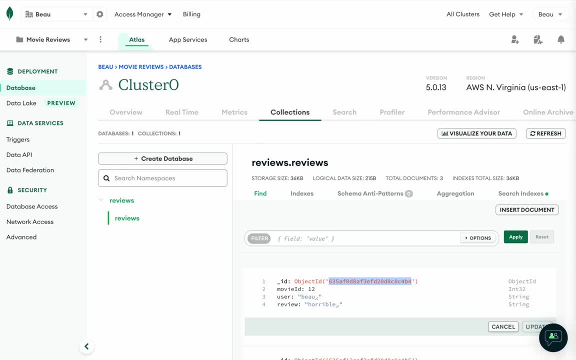 And then I put the object ID at the end And now it should delete. let's go back over there and see if the first one says bow horrible. If I refresh that it shouldn't be one that says bow horrible. See, it starts at Quincy bad movie And there's only two objects Now there used to, there used. 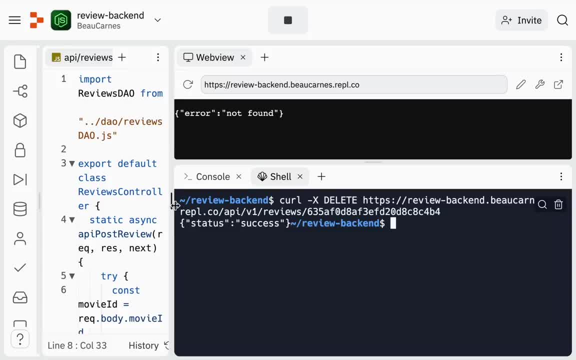 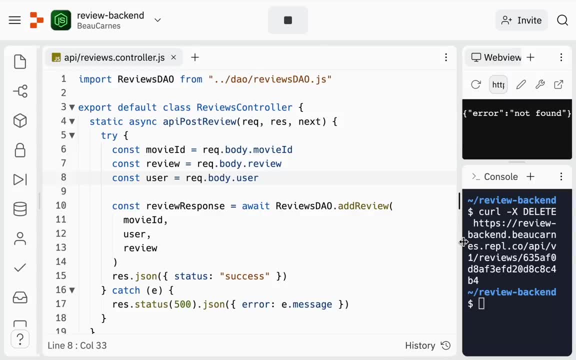 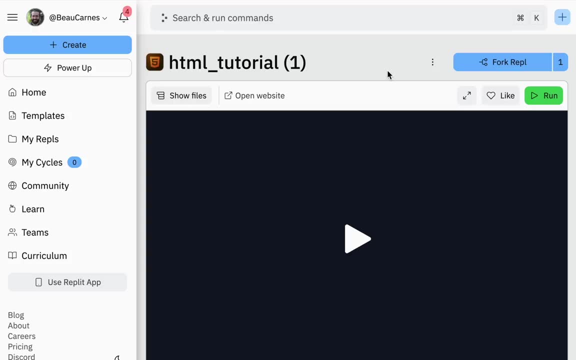 to be three. So it worked. Our entire, our API all worked. So the next step is is connecting this API with the front end. Okay, the first step in connecting the front end to the back end is to clone the front end. So this is the front end that Tomi made, And I'm just going to go. 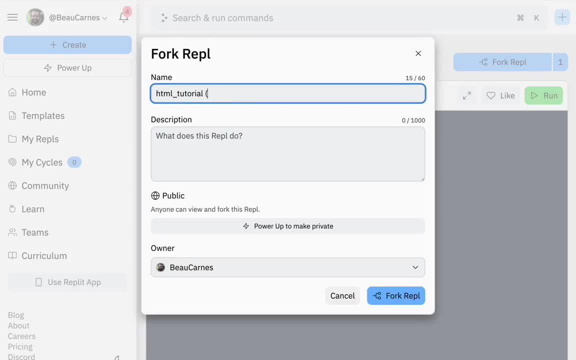 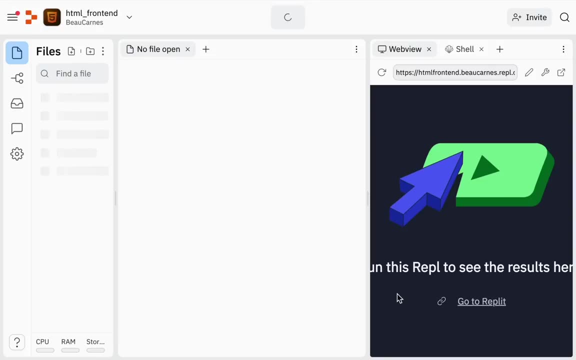 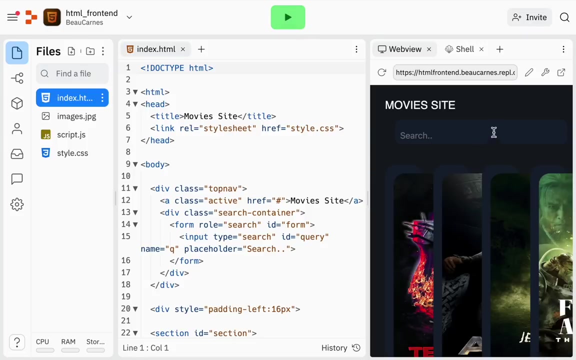 to fork repo And I'm going to call it HTML front. And that's me, my version, And now let's let it load. Okay, I'm just gonna hit the play button right here to start, so we can see what it looks like You. 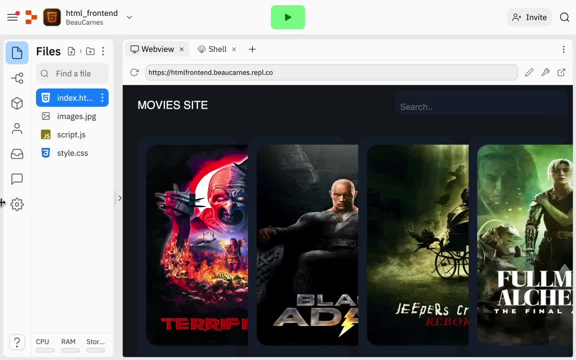 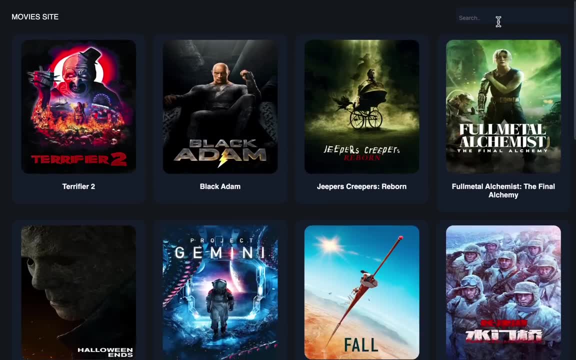 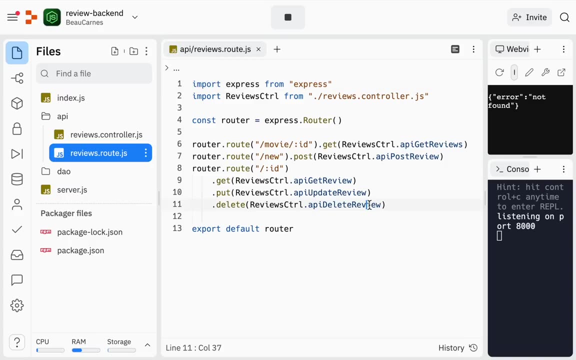 can see. if we spread out, you can see a little more. I can also open this in a new tab, So let me copy that. Okay, this is what it looks like. I can do a searching, search for things, And just how Tomi had it. So let's go back to the. Oh, that's my back end, which we are going to know why I'm here. 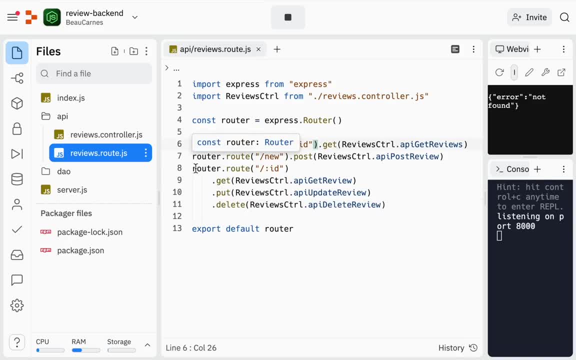 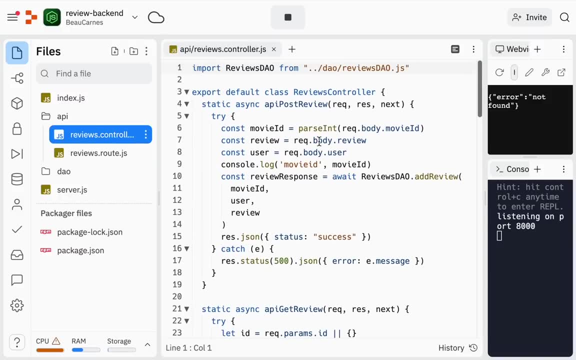 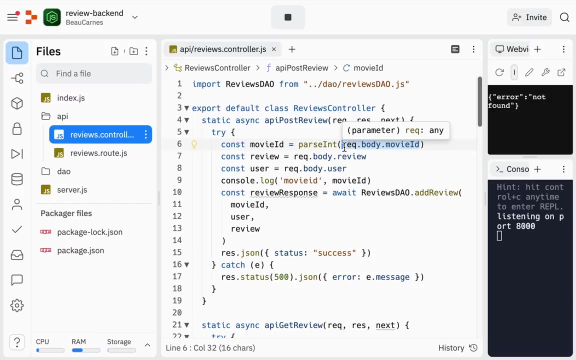 while I'm on the back end, I did make one change to the back end, which was in the what is the routes or the controllers, the movie ID, what we have? to parse it as an int because it comes. it could come in as a string or. 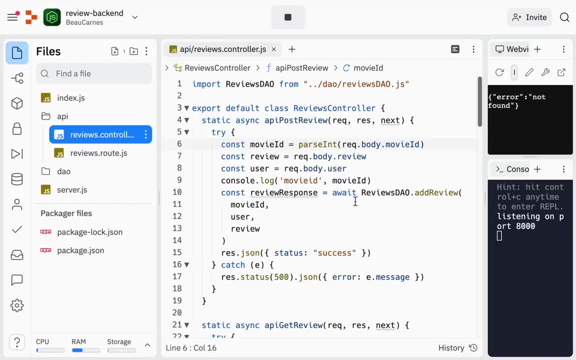 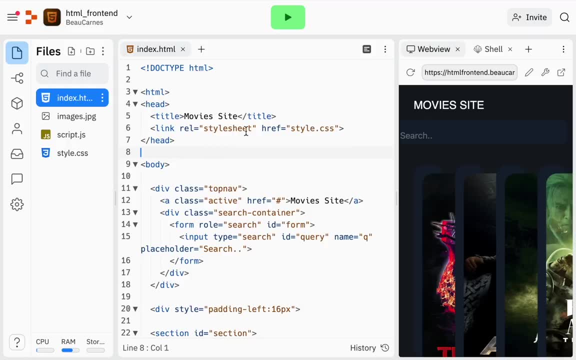 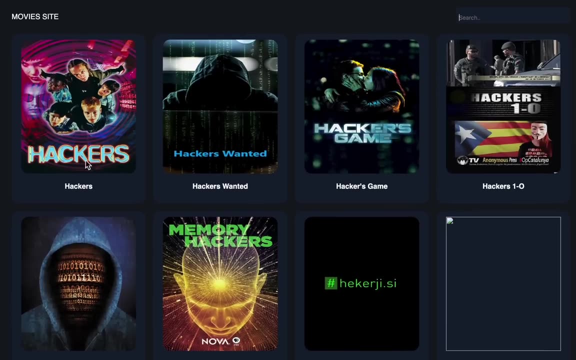 an integer, And we have to make sure it's an integer before it gets saved to the database. Okay, let's go back to the front end. So right now, there is no way to to see any reviews. it's not made up for any review, So what we want to do is make it so under each movie on here, there'll be a 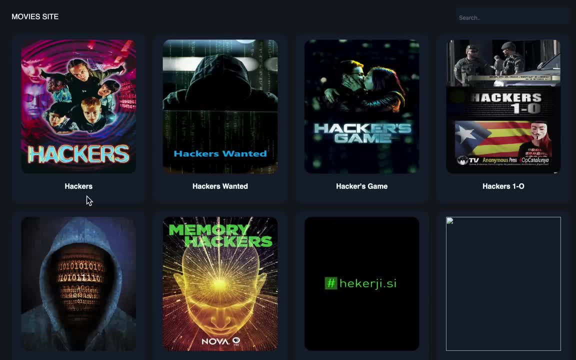 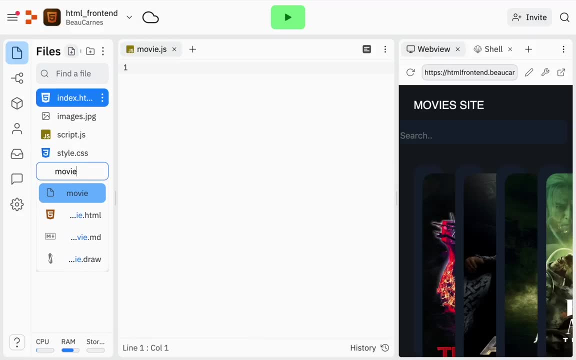 link that goes to a page of reviews. So let's make two more pages here or two more files. First I'll make a file called movie dot html, which will be the page that's just about the movie, that has all the the reviews, And then I'll make another file called movie dot j s, which will be the job. 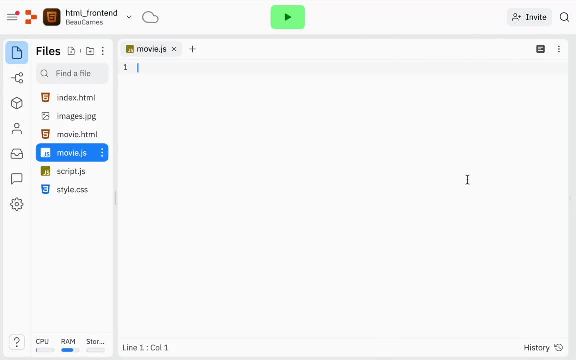 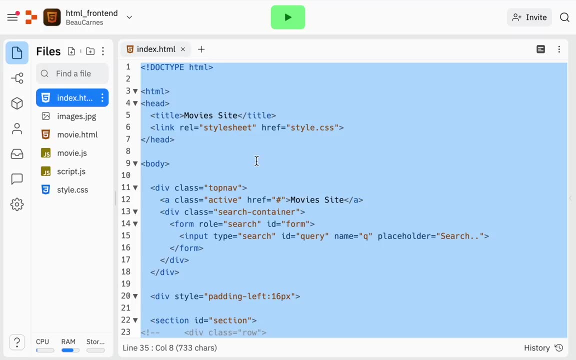 script file And let me just move that over here And to start off with, we're going to just go into the index dot html. I'm going to copy all this And then I'm just going to bring it right into the movies dot. 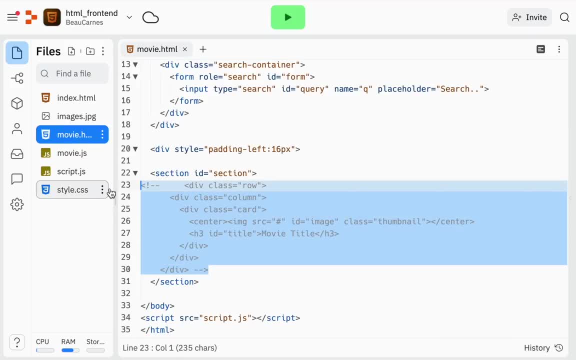 html And I'm going to make some changes, not going to have this sample code here, But. but we are going to end up the review. we're going to load the reviews kind of like the movie, So there'll be a card for each review, But I'll take that off. 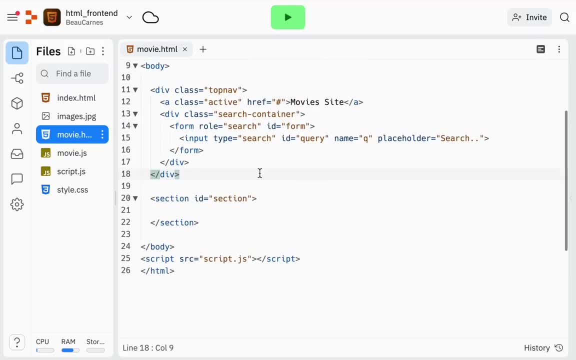 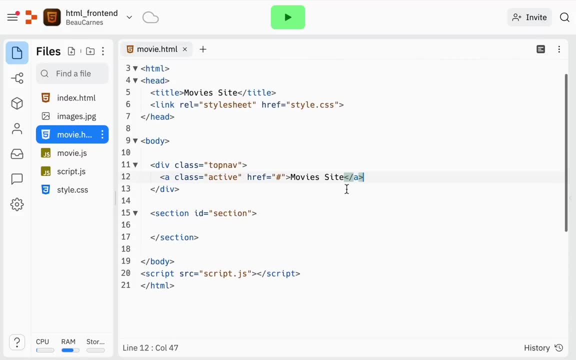 We don't need this, And what else are we not going to have? Okay, we're not going to need the search, because this is just the review, And we want to make sure that when we click the word movie site, it will go back to the index. index dot html. That's the page that Tommy made, And then we 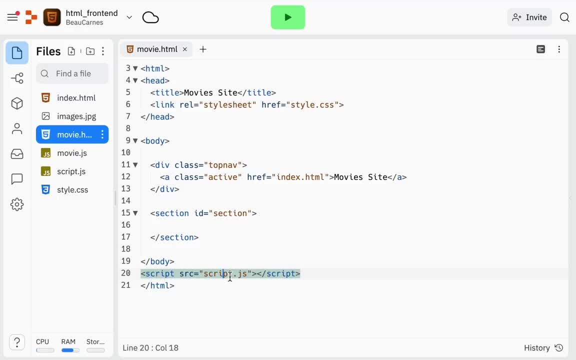 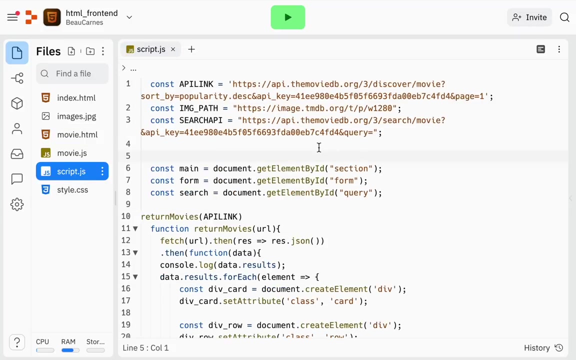 want to make sure that instead of script dot j s, we're going to make it movie dot j s, So we'll be link linking to the other JavaScript file. Okay, that looks pretty good. Now I'm going to go to the script dot j s. I'm actually going to copy all that too And bring over to a movie. 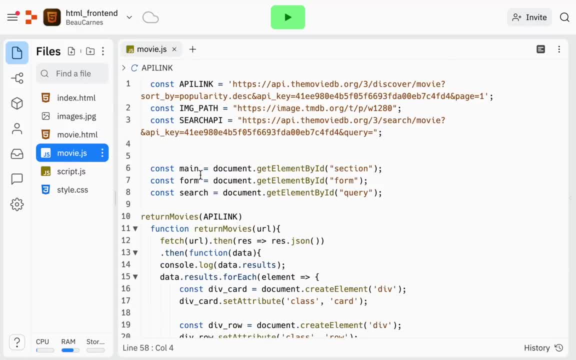 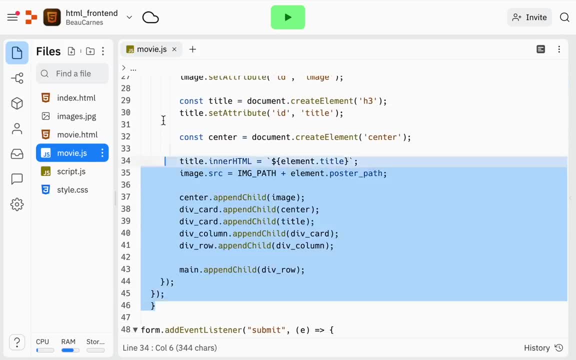 dot j s we're going to have some things are going to be kind of similar. Some of the tabbing got messed up a little here, So let me make sure we get the tabbing how we want it. So if I select everything and if I press shift, we're going to get the tabbing And then we're going to have 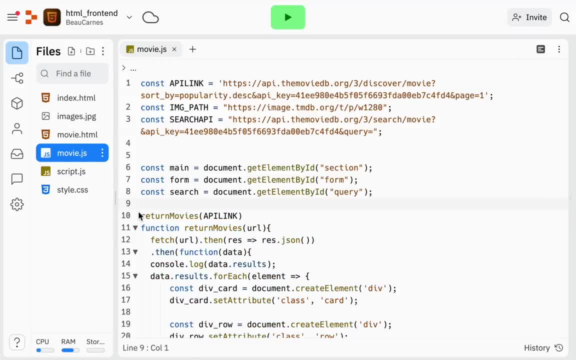 shift tab, it goes back one. Or if I do shift, or if I just do tab, it goes forward one. So what we're going to do is change. we don't need these two links, but we still need an API link. But now, 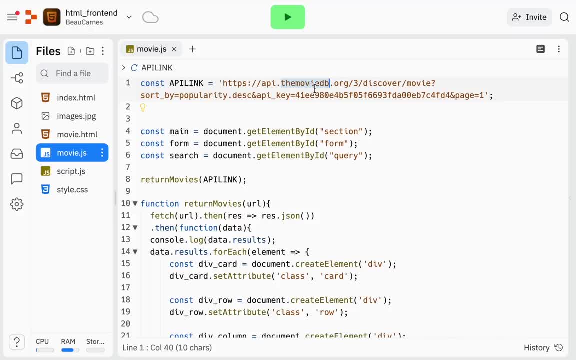 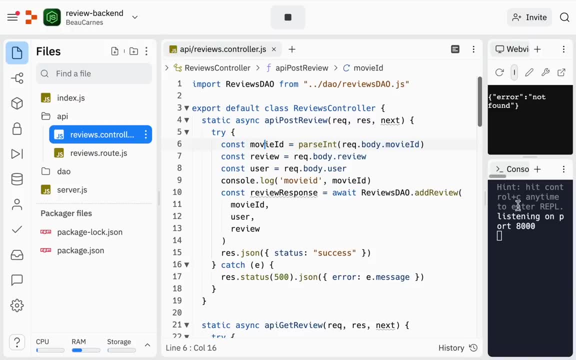 instead of using the movie DB API link, we're using the API that we created on the back end. So I'm going to go back to my back end code And we just need to get so. this is the URL. If you're following along, it could be different depending on what your 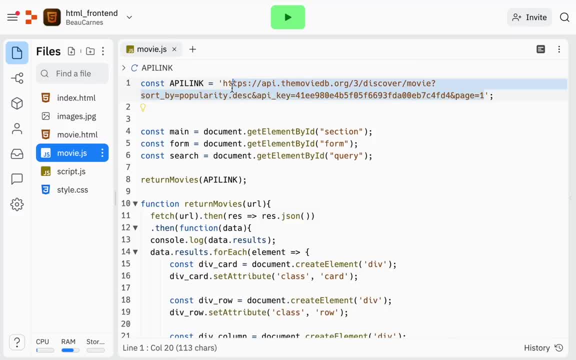 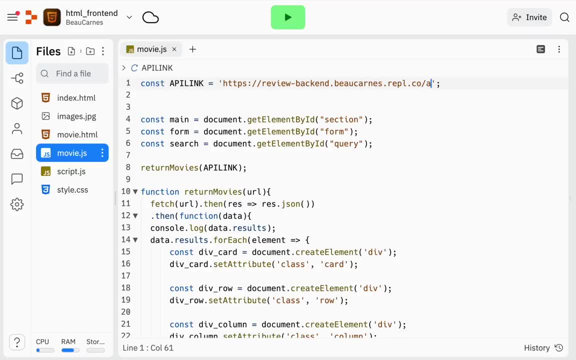 URL is, But if you're following along it could be different depending on what your URL is. we go back here and I'll just paste in this URL And then remember we have the other part of the URL, which is just what is the API: v1 slash reviews, slash, okay, and we took off the search in the 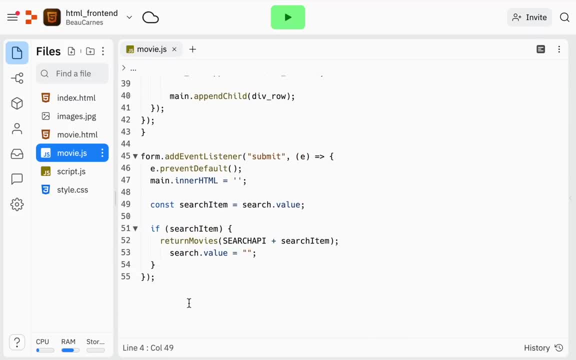 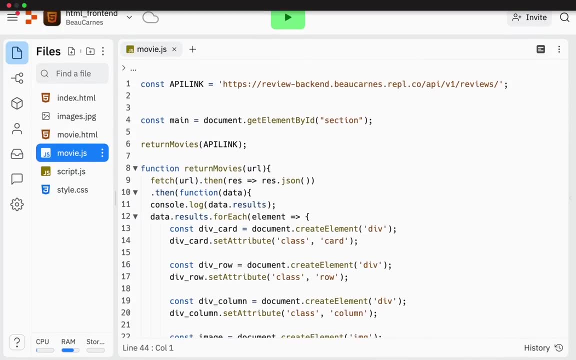 form, So we don't need that. And then we're going to delete this because we don't have that anymore. And now we're going to make some, some additional changes here. But before we make the additional changes, let's make it so a user can actually get to the movie page. So I'm going to go to the scriptjs. 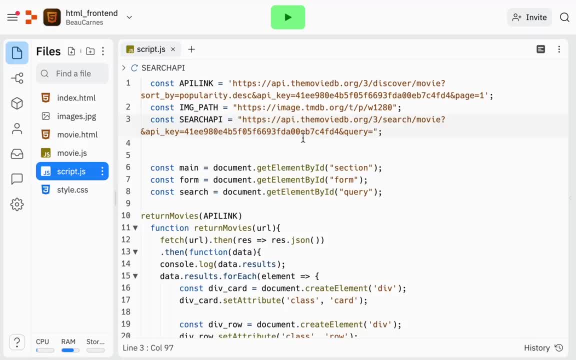 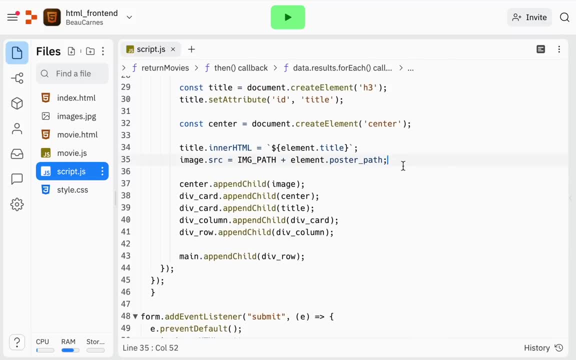 Remember, this is for our, our main root site, the one that Tommy made, and I'm gonna make some changes so we can add a link here. So what we're going to do when, on this section right here, where we update the inner HTML of the title: 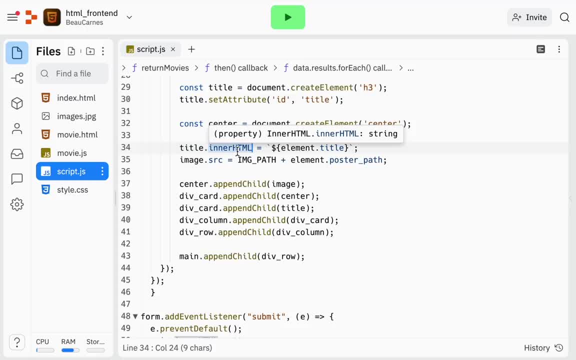 we can. since it's inner HTML, we can just add additional HTML. it just doesn't just have to be a title we can use. we can actually put any HTML in these tactics. So what I'm going to do is add a link to the review page in this HTML. So, first of all, I'm going to put a br, which means means a. 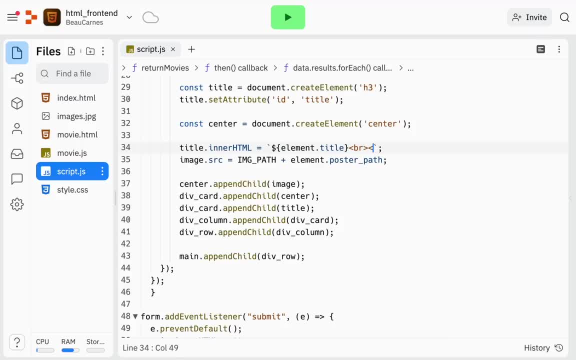 break, a line break, So we'll go to the next line And then we'll do a href. You know that's, that's an anchor tag or a link, And we just had to put the URL in there And then we're going to go to the. 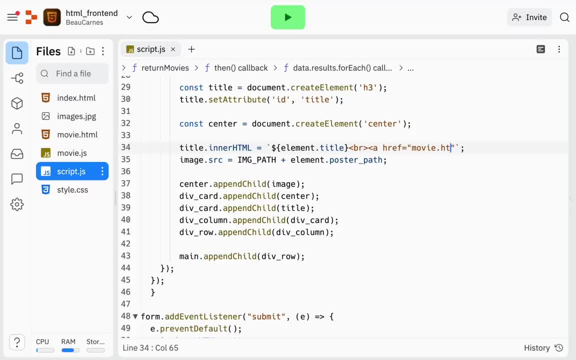 URL. So this case is this going to be movie dot HTML. But we're not just going to only put movie dot HTML, we're going to put some query parameters that we want to pass them information from the indexhtml to movie dot HTML, And we there's a few different ways to pass information between pages. 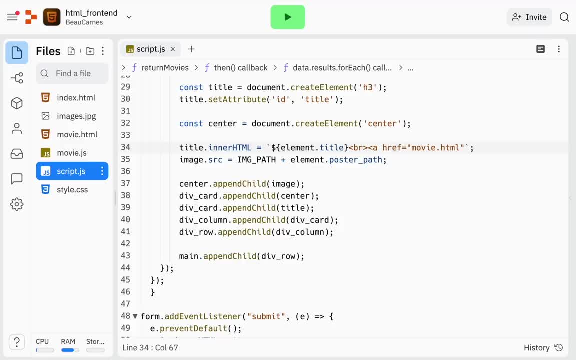 But one of the easier ones is just to use query parameters in the URL. So you've probably seen this: before a query you do the the movie HTML, we put a question mark to say that we're just about to put some query parameters. 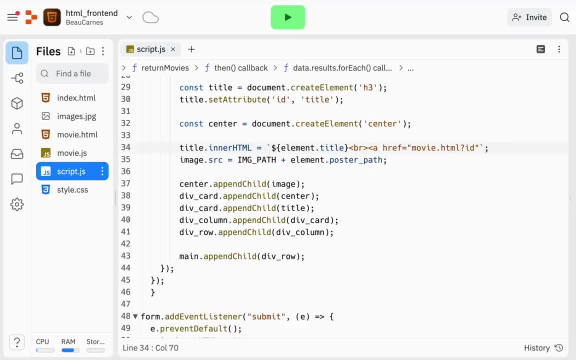 which are just basically key value pairs. So first we're going to pass in the ID, the movie ID of the movie that the person is clicking on. So we want to make sure it loads the the reviews for the right movie based on the movie ID. So I'll do ID equals and then I have to get the movie ID, Basically. 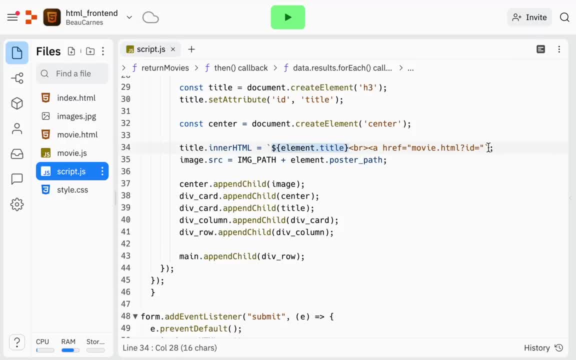 we can use this exact same way that we got the title to get the ID. So I'm just going to copy that and element that title, but instead of element title it's gonna be element ID, And then we can just put an ampersand or an and symbol to do another query parameter And it's going to 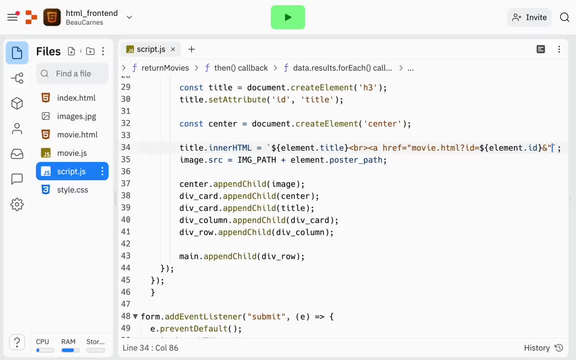 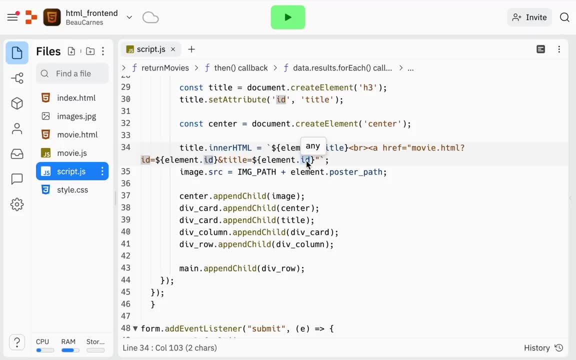 follow this same format of the ID, But instead of this time, instead of ID it's going to be title. we're going to just pass in the movie title and then we'll put title And then we have to. so this is a. we're still in this anchor tag with the link. 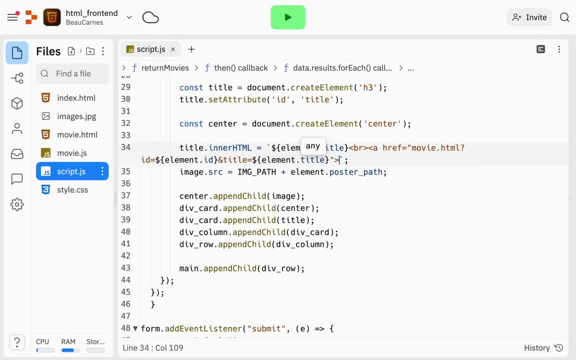 The link element. So I'm going to put what the link is going to say. it's gonna just say reviews, And then I'll put the closing tag, just like that. Okay, so now I am going to just run that And. 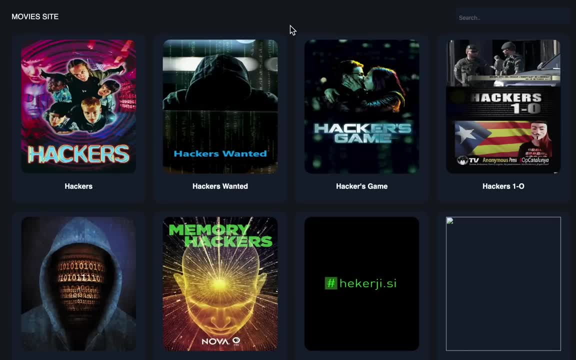 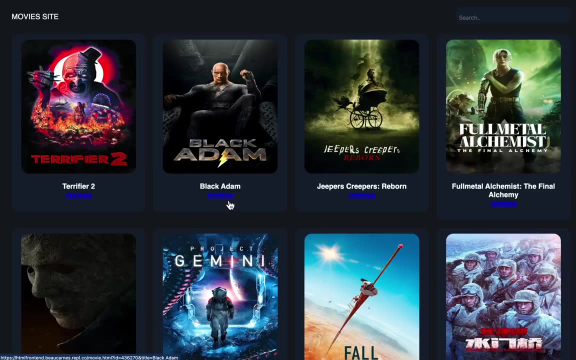 let's just test that so far. Okay, so I'm going to go back to the page I'll refresh here. Now we can see it says reviews. Now it is kind of hard to read with the blue like that And you could go into and change the CSS. I'm not going to focus so much on 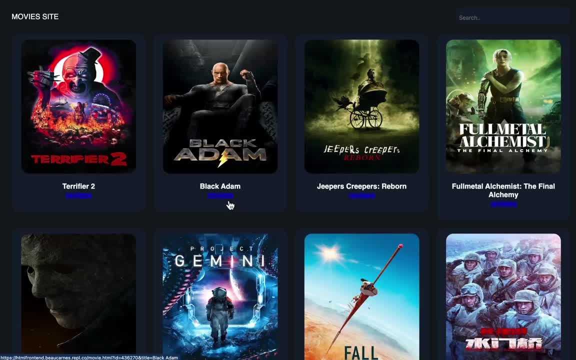 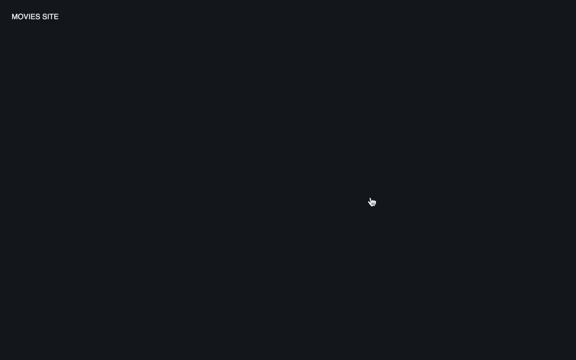 changing the CSS and styling, But that's something that you can do on your own if you want to make it look a little better. So if I just go right into this one, it doesn't show anything because we haven't loaded anything on the page yet, But we can see it definitely did load the page And we 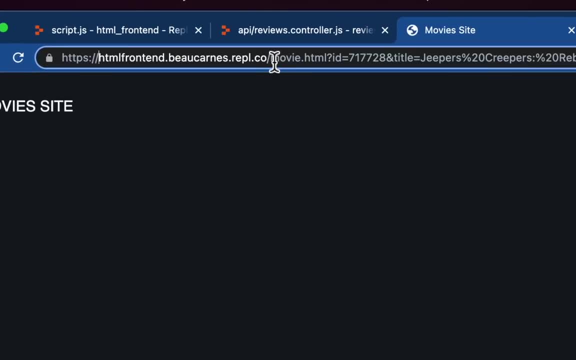 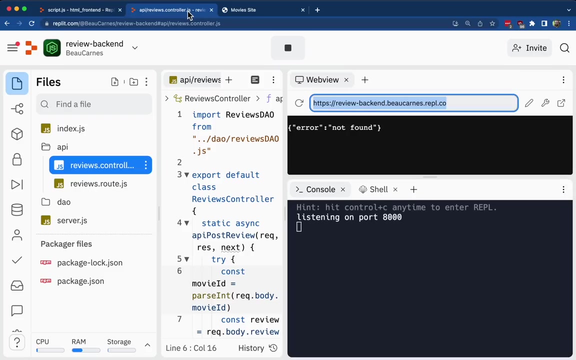 go back and see the URL bar, we can see that it's saying movie HTML, we have ID and we have the title, And then it it because there's spaces to put a space in a URL. you can't just put a space in URL, So it put the percent 20 to represent the space. Okay, let's go back over to 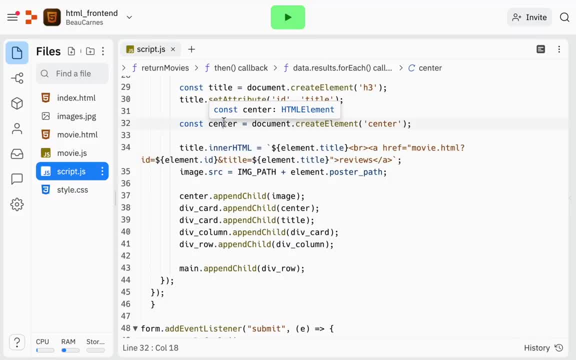 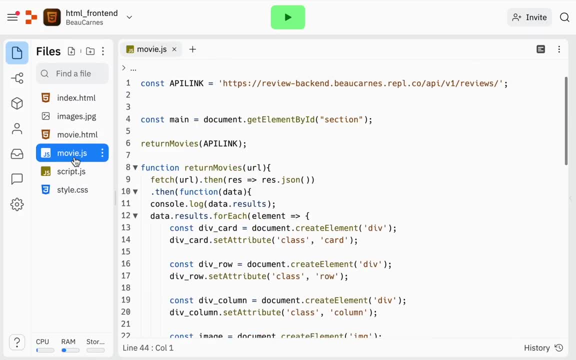 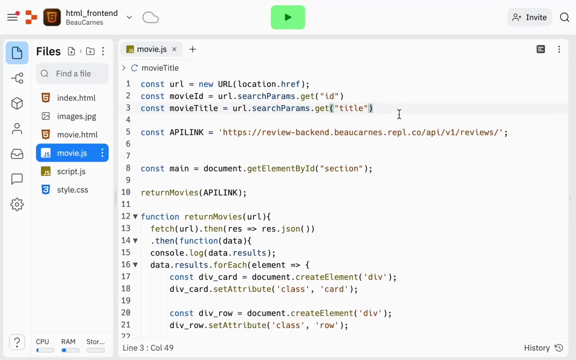 our file And now we were basically done with our updates to the, the route that each, the scriptjs and the indexhtml. Let's go back to moviejs, So I'm not going to type in everything here. sometimes I'm going to paste some things in here And so this is going to get information from our 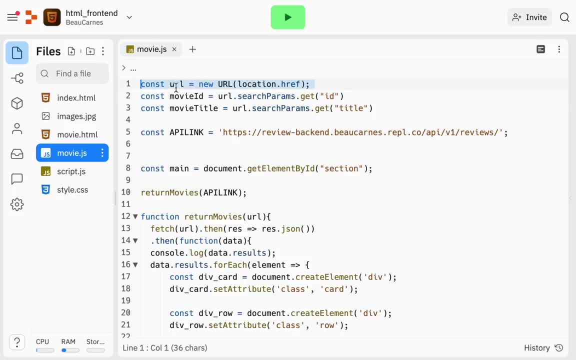 URL. So right here we, when we do a constant URL, we're making a variable called URL and we're using new URL. this is a way to basically make a URL object from the actual URL. So this is just something built into the browser, built into JavaScript. 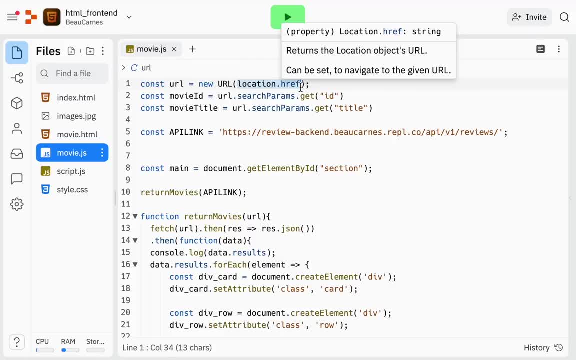 if you do location h ref, it will be a string based on the URL that the person is at And we can create a URL object like that. And once we have a URL URL object, we can access different parts of the URL. Specifically, we're trying to get the search params. So the query: 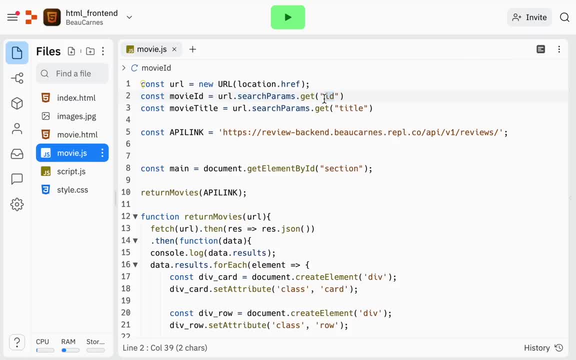 parameters. we're getting the one that has the key of ID and putting the value into movie ID and then the key of title and putting the value into movie title. So we got that. we were able to pass that information into this next page, Since we have the title. 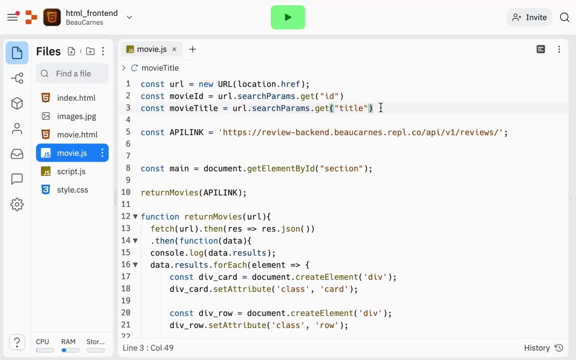 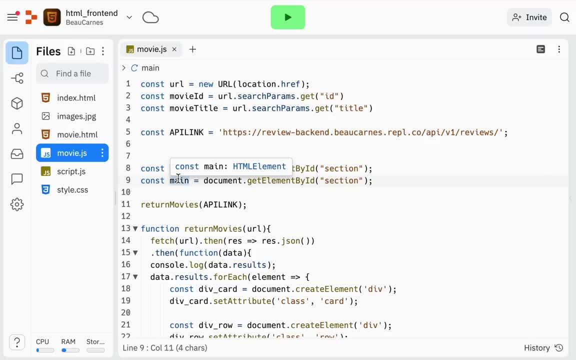 we're actually going to put in the movie title onto the page, So we already have access to the main element. I'm just going to copy that and paste that in, And now we're going to get access to the title element. If you remember, we actually don't even have a title element, So we have to. 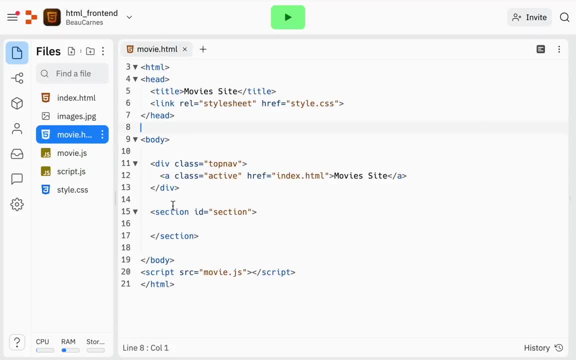 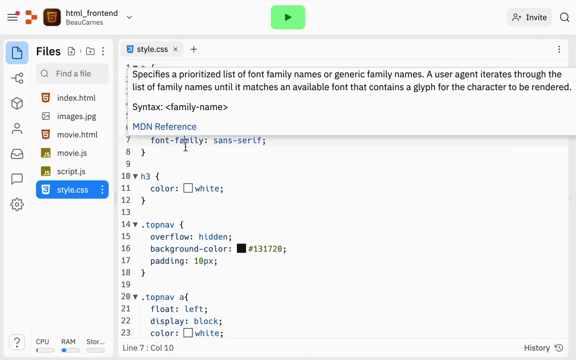 create that. So let's go over to movie HTML And then I am going to just put in some code here. reviews for movie title: Now h1, if you notice, his a dark background and right now h ones are colored black. So let me go to the style, that CSS, And I'm just going to 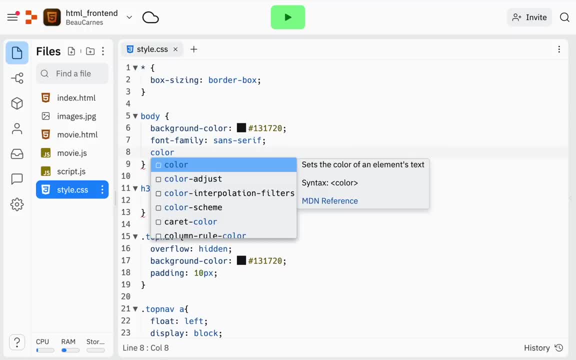 in the body. I'm just going to put color white. So now all the text color is refers to text color. So we already have the h3s are white. Now we have all the text being white, which makes sense because we have a dark background, And now we don't even need that one anymore because everything's going. 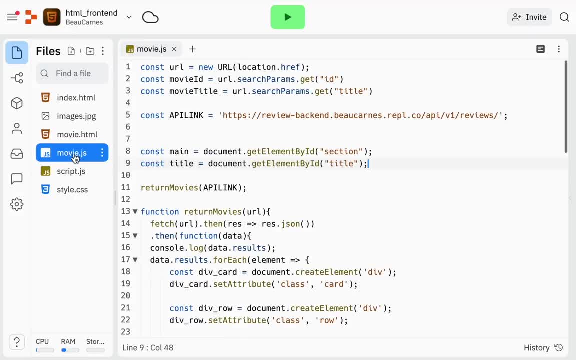 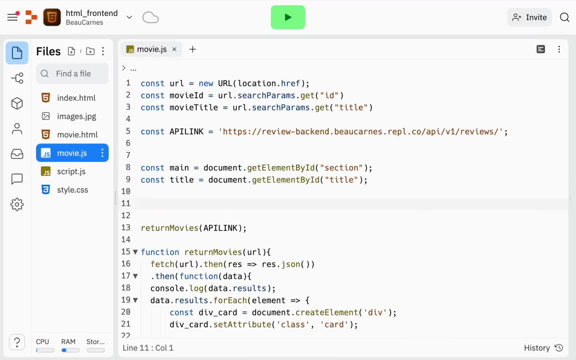 to be white. So let's just see what that looks like so far. First of all, let me just make sure everything is correct. Oh, before we see what it looks like, let's load the title into that title element that we just created. So that's just gonna be like this. It's what you've already. 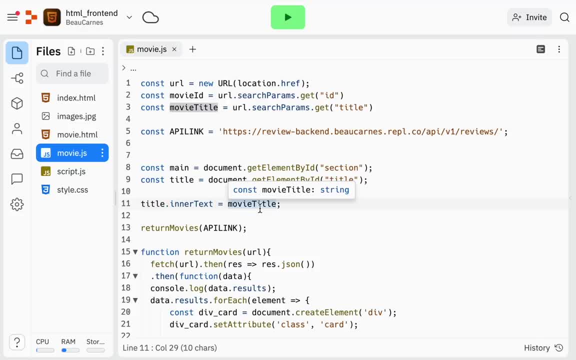 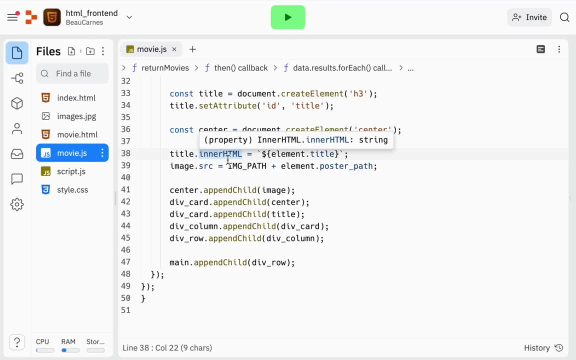 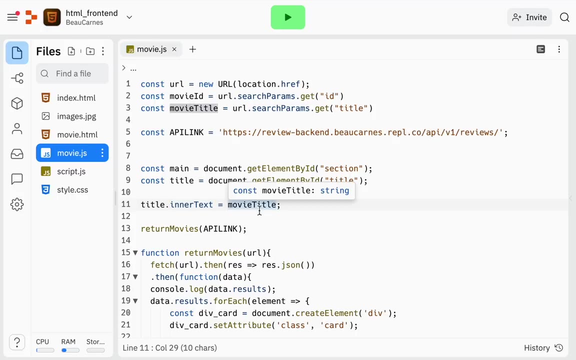 learned about title dot. inner text is going to be title. Oh, before you may have actually learned about inner HTML, think that's the inner HTML. you can put basically any any HTML. inner text is just going to focus only on changing the text. it's generally safer to use inner text. 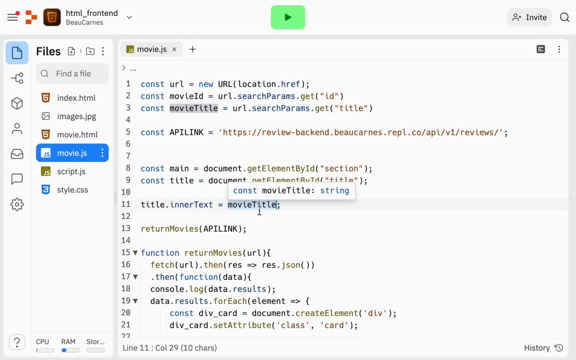 because you won't accidentally put some, some HTML that's going to just mess up everything. So if you can use inner text, but then use inner HTML if you need to, So let's just play that or run that Basically, just reload it, And then I'm going to just refresh over here. And now look. 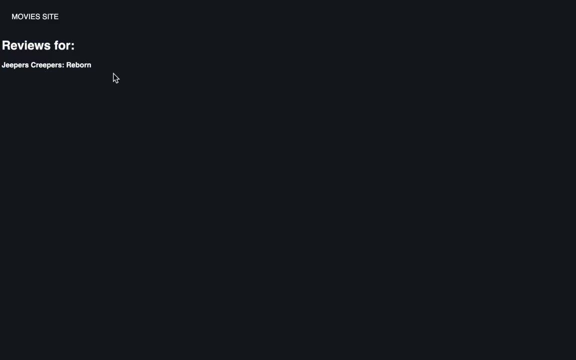 we're getting reviews for Jeepers, Creepers, reborn, that click movie site. I can go to any of these. So how about black Adam reviews for black Adam? it's kind of over onto the side here So we could go up and change the CSS, So this kind of kind of. 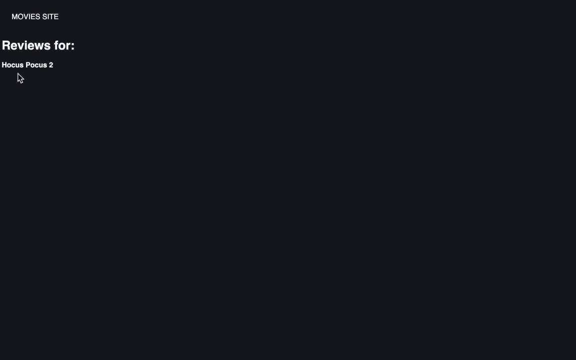 centered. I'm going to leave that as something for you to do on your own, But you can see. whatever we click on, it's gonna put the movie title right in there. Let's go to Pinocchio: reviews for Pinocchio. So now let's make it so the reviews actually show up. it doesn't actually show up, as. 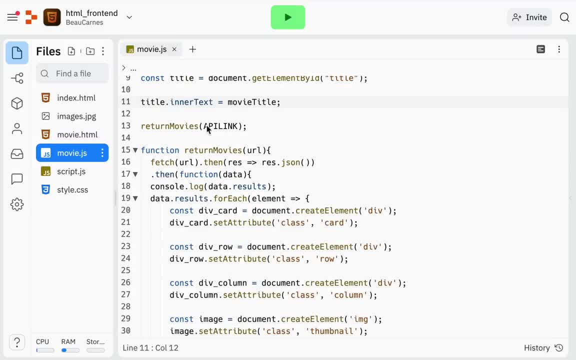 any reviews there. So we're going to change changes. So it says return movies. we actually want this to be return reviews. So I just did Command or Ctrl D to select multiple text pieces At the same time and then I can just say return reviews and I can change them both at the same. 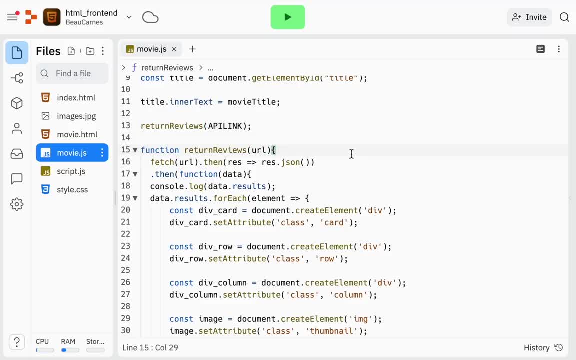 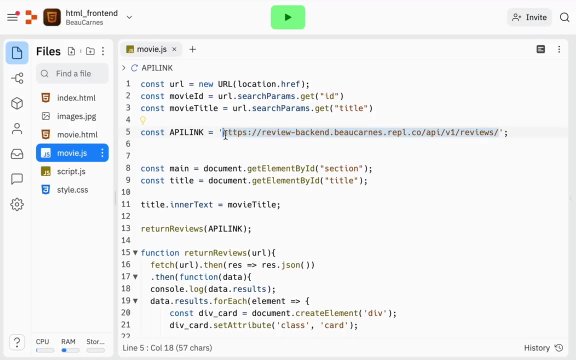 time. So then you only have to type it once it types it. we have multiple cursors to type those on. So we're going to go to the URL So, but we are going to have to change something, Because if we go up here we see the URL is this, which is slash reviews. And if you remember from our 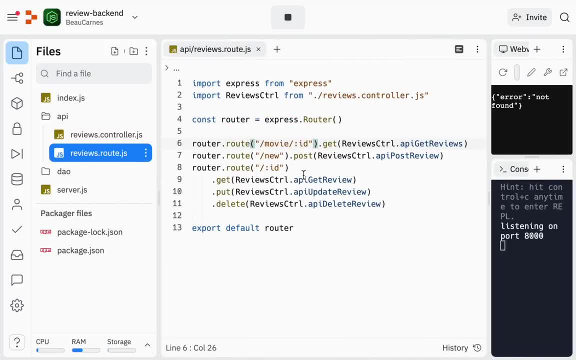 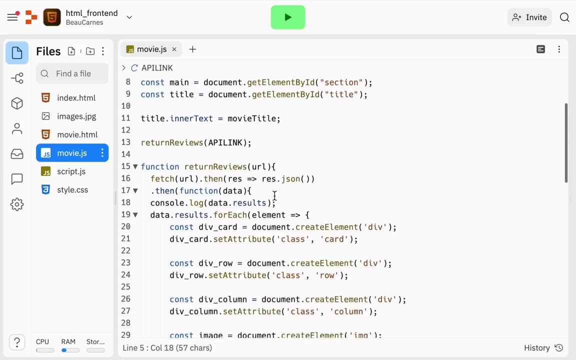 backend. here's our back end. here the route, route we actually want to go to is slash reviews, slash reviews. So, as you can see, this is what we're going to do. So if we go up here is it has slash movies, slash ID at the end. So we are going to use: keep the base URL. 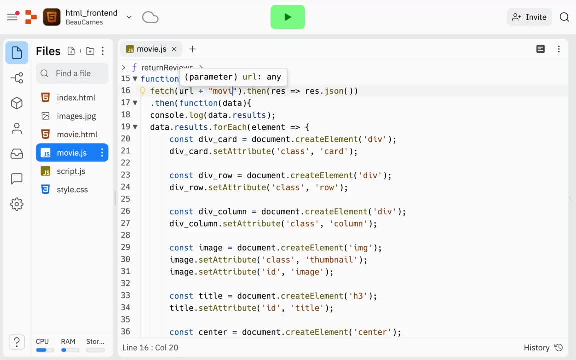 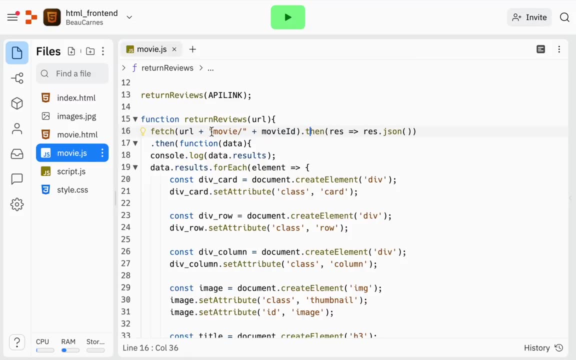 But now I'm going to say plus, movie slash, and then plus, plus, and then I'm going to put movie ID, which is what we got directly from the query parameter. Okay, now we're going to go to this newer URL, we're going to get the data And this time we don't need 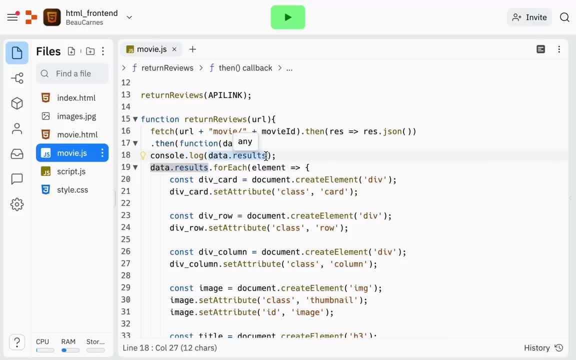 data, dot results. different. different API's work differently. So in the API for the movie page we did have to do dot results, But with the API we created it just deliver. it just gives the data directly. So I'm going to do command or Ctrl D to select every time it. 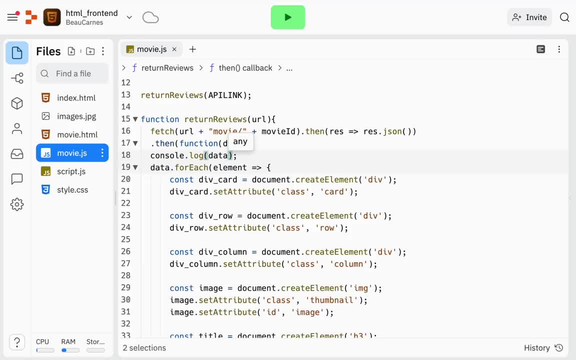 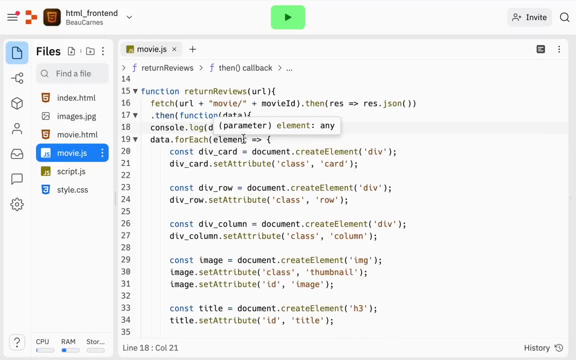 says data dot results and just get rid of that result. it's just going to be data And we can keep this console dot log here to see if anything is important. Now here there's with in programming there's just a bunch of ways to do everything. So 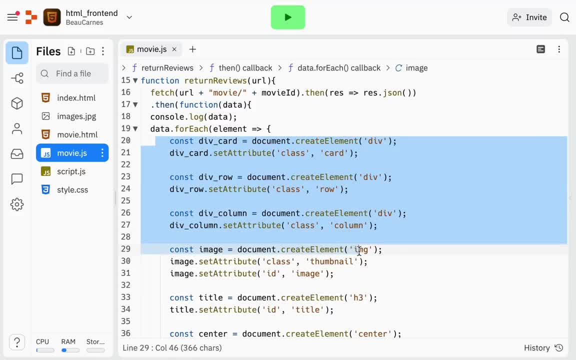 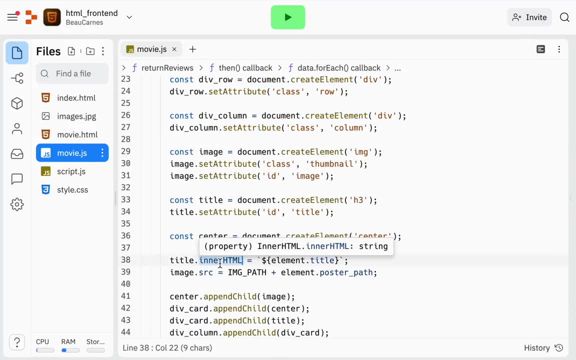 you already learned this method, But I'm going to show you now another method. So we already talked about how, with dot inner HTML, you can basically put a lot of HTML. So that's what I'm going to do, instead of creating a div. 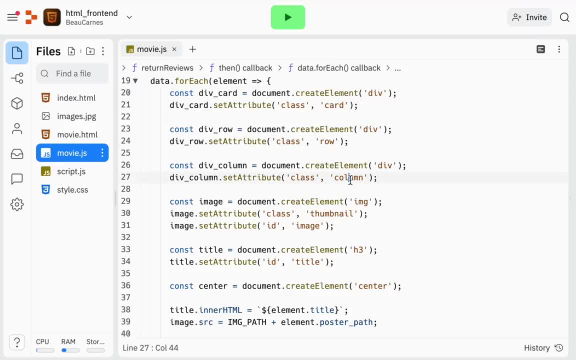 The basically the card div, the row div, the column div, all like this. I'm just going to create it as HTML. Now there's definitely there's there's definitely reasons to do it either way, And it just depends on your use case. So it's really good to know both ways of doing. 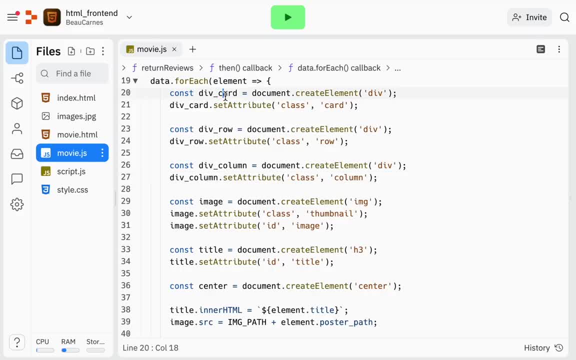 it. So I just want to teach you a new way that you can do it. So I'm going to. this is going to be called div card. I'm going to keep this the same, but I'm actually going to delete all these things, And you'll see soon what we're, how we're going to do it. 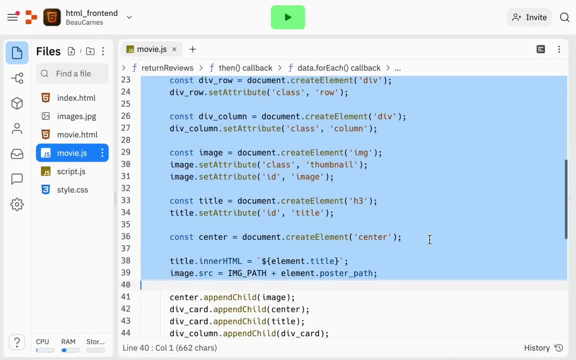 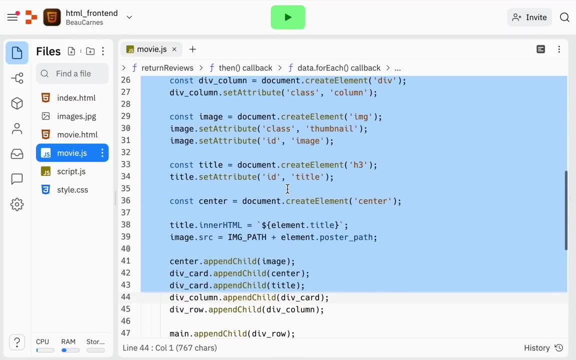 What we're, how we're going to change this And all this. actually see, all this, I'm going to show you a different way to do almost all that. we're not going to do all of it because we're not going to have the image. there's not going to be an image, we're not going. 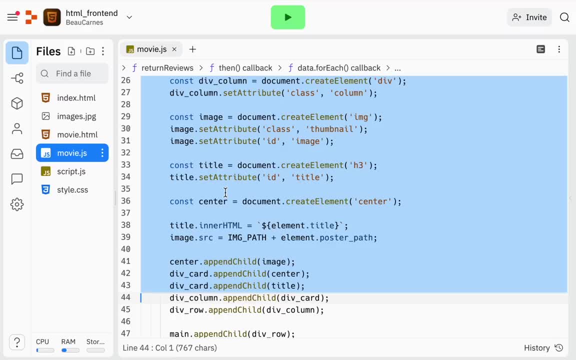 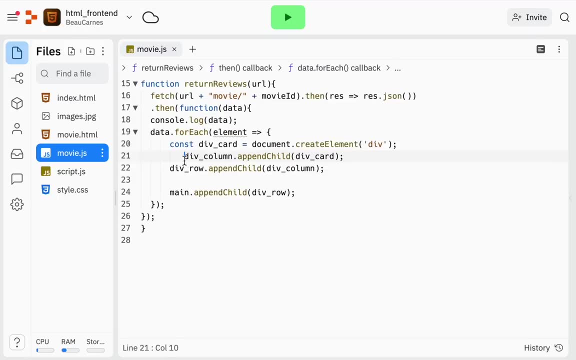 to have the. basically, that's the main thing we're not going to have. we're not going to have this, this center element. So I'm just going to delete all that And we can see that right now. Okay, we're only going to append that card, But first we have to update the card. So 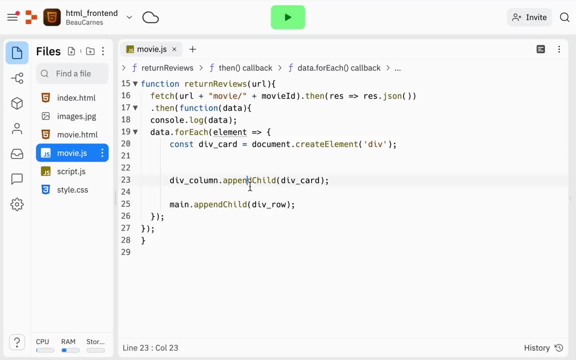 right now we've created that element and then it gets appended here. Oh, and actually, no, we don't even need to do that, Because we're just going to append this on to main div card. So I'm just going to do div card dot inner HTML, And now I'm just going to 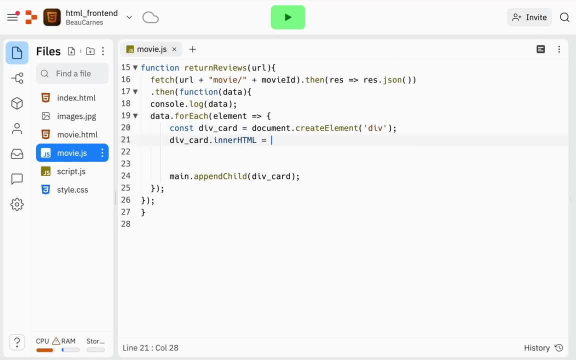 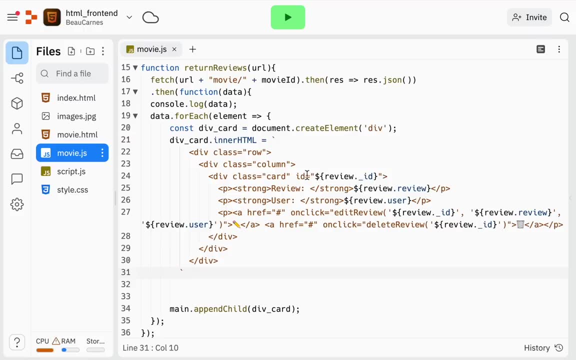 put in the actual direct HTML, instead of making everything individually like that. I'm just going to paste it in here And then we'll go over it. So you can see it's the HTML. format is very similar to before. we create the div with class row, we just create the. 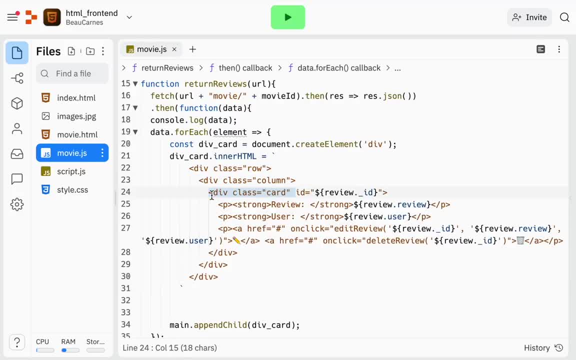 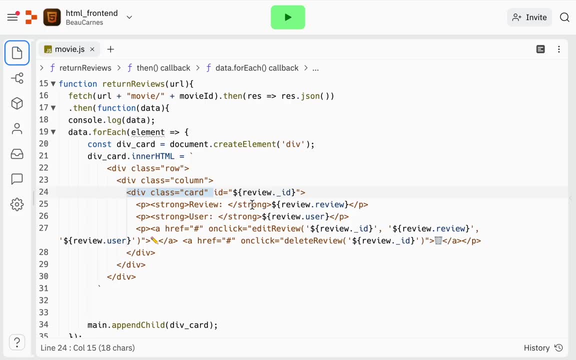 div with class column. we create the div with class card, And now it's going to be a little different Because, remember, we're doing reviews now, not movies. So let me show you what we're going to do here. If I close that here, we can see that I'm going to add an additional. 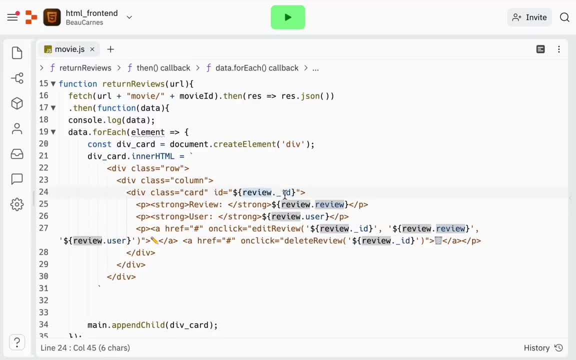 an ID that gets the review ID. the review ID is coming directly from our API because, oh, actually this needs to be changed to review. it's not element, because we're getting the data from our API And the data is basically a an array of a lot of different review elements. 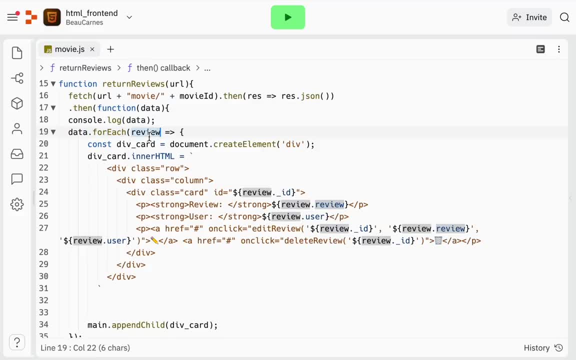 But since we're doing for each, we're doing something for each review in the returned data And each review is going to have an ID. It's going to have a review property and a user property, And we saw all that when we were talking about the back end. So we're going to create an ID for this card element. 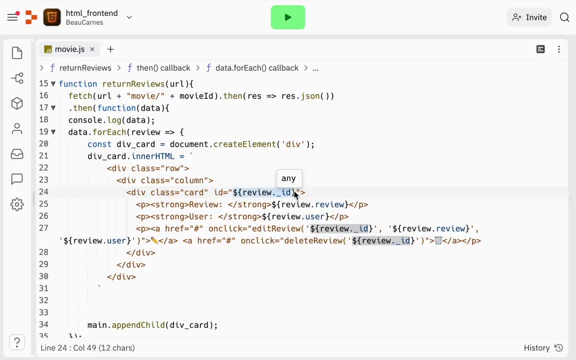 based on the review ID. The main reason is because we want it to be a, a, basically a unique ID that we can then refer to later. So we can get access to this specific element later And we know that the review ID is going to be unique. So that's why we're setting that. 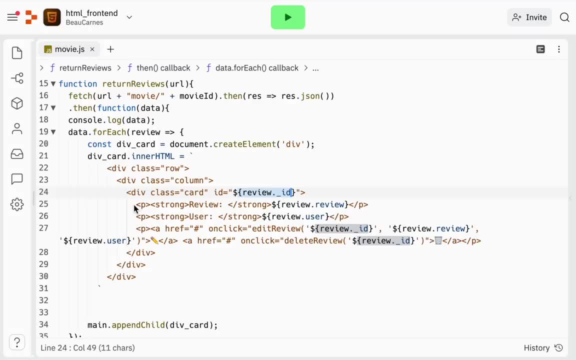 as the ID. So now we are going to create a few paragraphs. So we have three paragraph tags. the first paragraph is going to contain the review. So strong, the strong element just makes it bold. So this is going to be bold And you can see right here the review we just put. 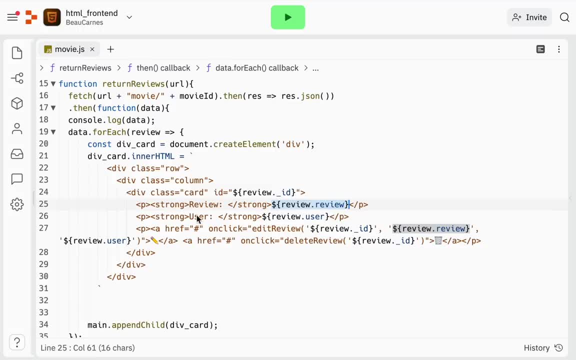 in the review that we got from the back end database, And then we get the user that we get from the back end database, And then now this is where it gets trickier here, This part right here. So there's a few different components. Basically on the screen it's: 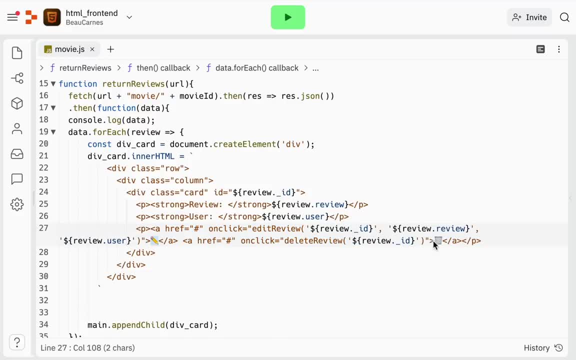 just going to look like two emojis. it's just going to look like a pencil emoji and a trash can emoji. But this is what we're doing. we're creating it as a link, but it's not going to go anywhere. That's what this, this pound sign or hash mark, me means: we're not going. 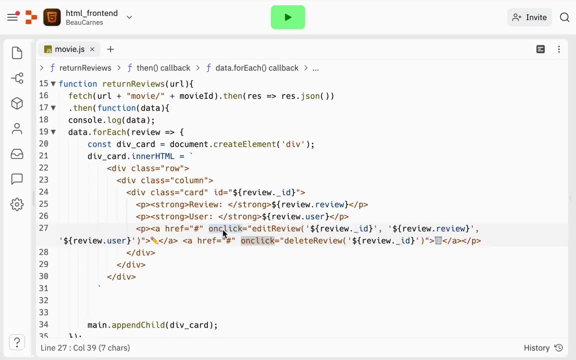 to a specific URL, because we're going to put an on click property. So when this element is clicked, which in this case is just this pencil element- it's going to call the element Edit review function, which we still have to create, And it's going to pass in three. 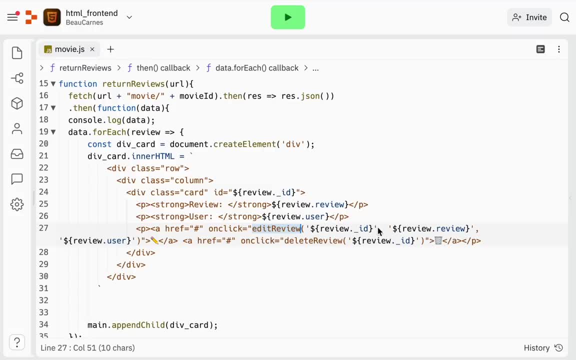 Elm, three pieces of information to the Edit review function. First it's going to pass in the review ID, then it's going to pass in the review and then it's going to pass on the user. And you can see we have these single quotes around each one because it's. 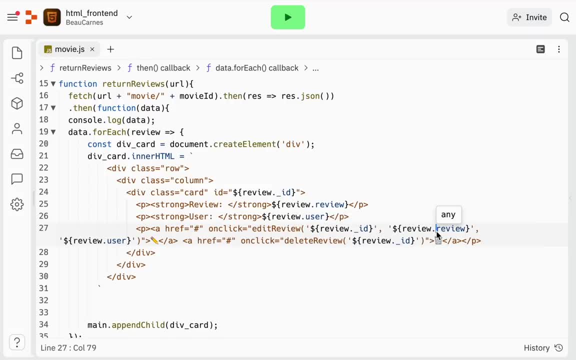 going to pass in each of those pieces of information as a string. Okay, so then that. so then when it says: when you click on this little pencil, it's going to call the Edit review function, Passing on the information, or you can click on the trashcan where it's going to call the. 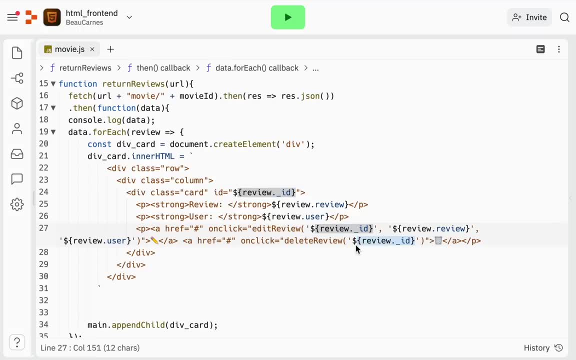 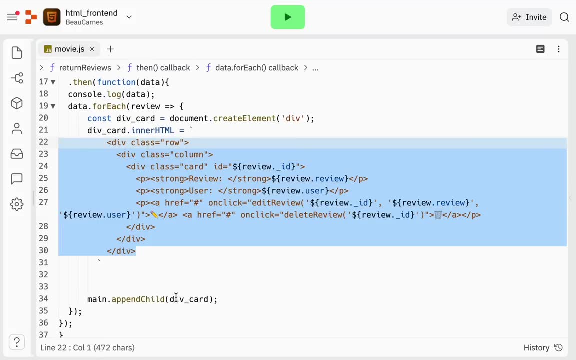 delete review function only passing in the ID, And so then it's going to append for, so that for each review it's going to put this and it's going to then append it to the main element. Okay, so let's just test it out. So far I can press that button to load. 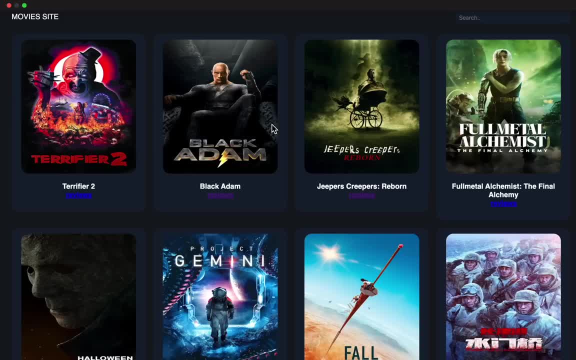 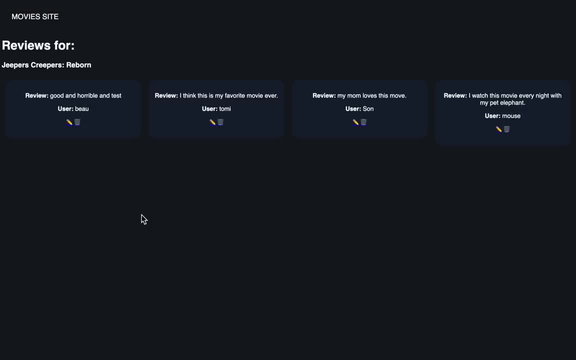 it. Okay, let's just refresh. And now I think I already I already put some reviews in this one, So let's click here and see if they show up. Okay, you can see. we have the reviews. reviews for Jeepers, Creepers reborn. So I did this off, off camera. basically, I added: 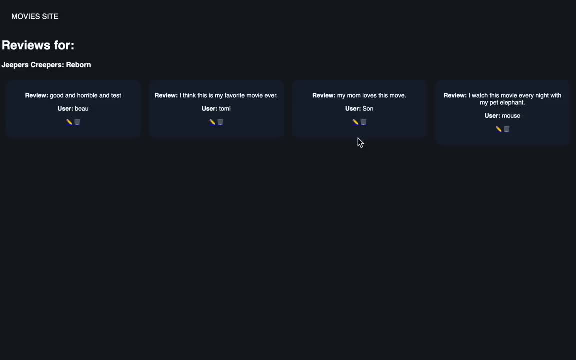 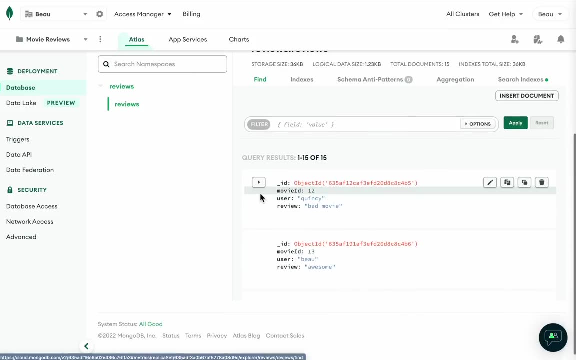 some, some reviews, so they would show up right in there. This is, they're loading right from the database. So if we go over to MongoDB Atlas, we can actually see there's 15 reviews, right, Okay, Okay, Okay. So we can see some of the ones that I previously added And you can see some of them. Some: 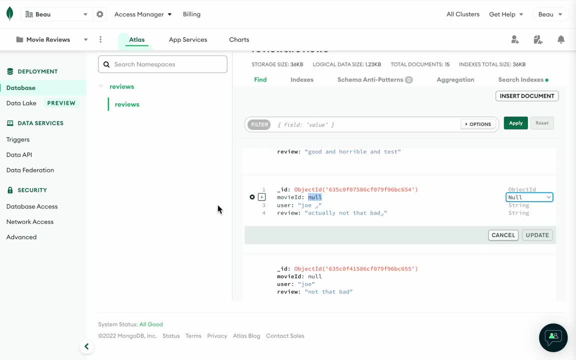 of them don't actually look correct. Oh, you see, this is null here. When you watch a tutorial, it looks like the person just has all figured out and just does it really quick. Actually, I went through and tried to figure everything out before I started recording And there 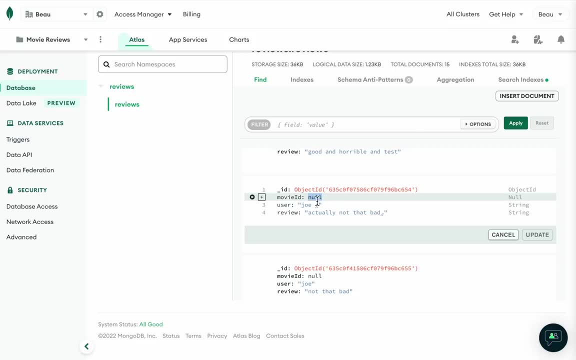 were some things that took me a while to figure out. it was saving for a while. I had something wrong, So when it saved the movie ID correctly wouldn't send it correctly, And then when I had it so it would save it as a string. That's why it has the quotation marks on. 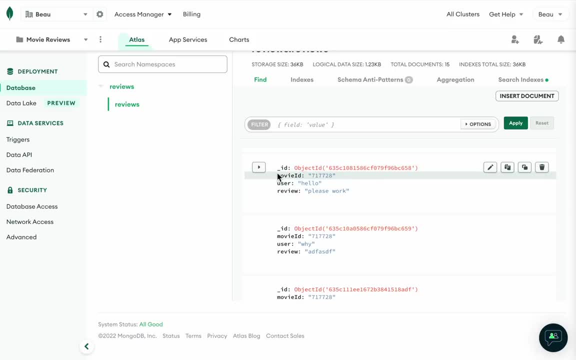 either side And that's why I showed you earlier about how I went back in to the backing code to make it do the parse into switch it to an integer. So if we go down here we can see now we're at an integer And you can see a lot of these reviews. here are the reviews. 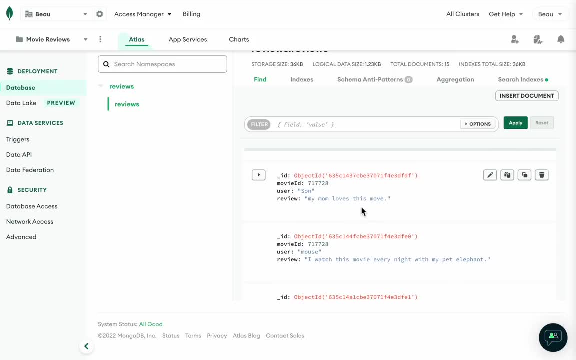 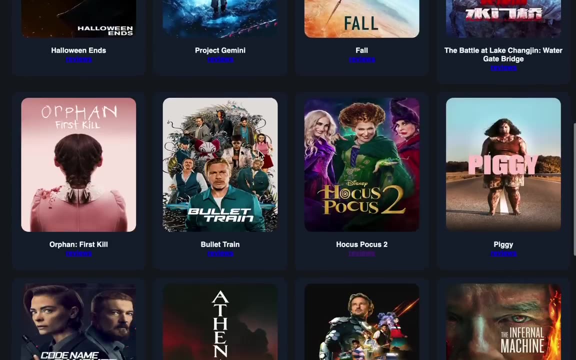 we just saw on the page, So let's go back over to that, Okay. so right now we can see these reviews And if I go here, if I go to a one that doesn't have any reviews, like here, it's not going. 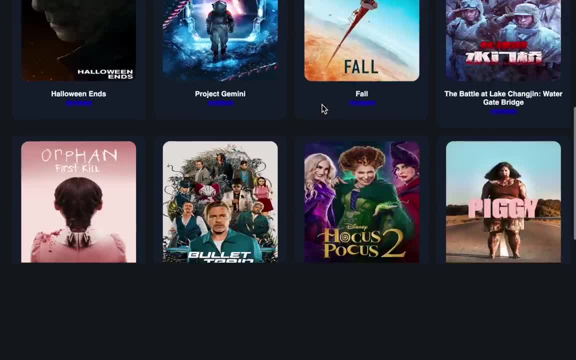 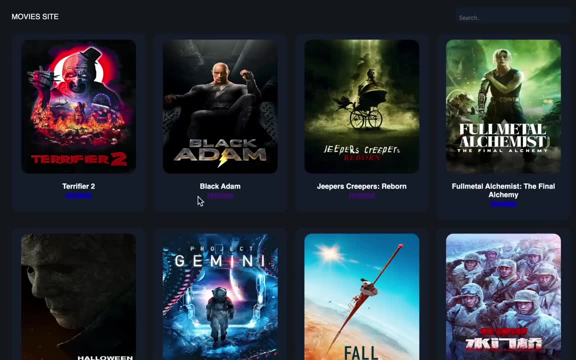 to show any reviews. there's no reviews on that one. most of the movies don't have reviews yet, So if it doesn't have a review, it's just going to basically just show like that, And right now nothing happens when I click these buttons. So it's basically just going. 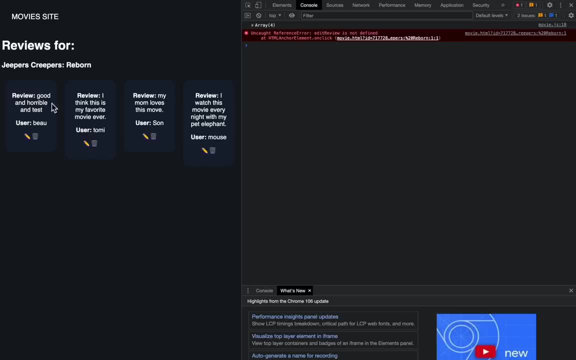 to have an error. Or if I open up the developer tools, see, whenever I click here, it's gonna say edit- review is not defined. Or if I click here, delete, review is not defined. So I'm fine, because we haven't actually created that yet. Okay, speaking of creating the other, 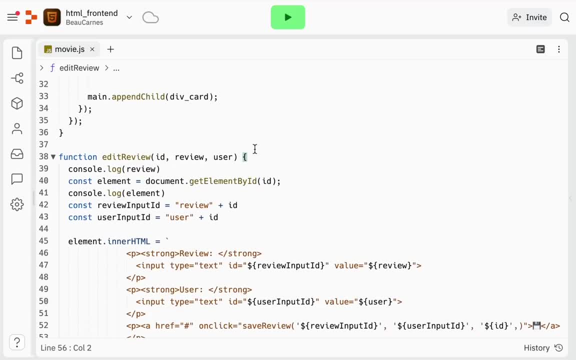 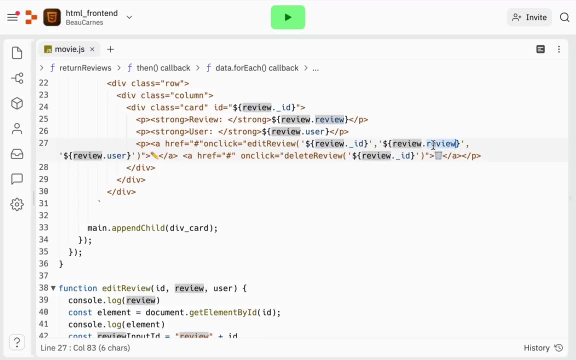 functions. I'm going to create the edit review function. I'm just going to paste this in and we'll talk about it. So, if you remember, when you call edit review, it brings in these three pieces of information: the review ID, the review and the user. So we have to accept. 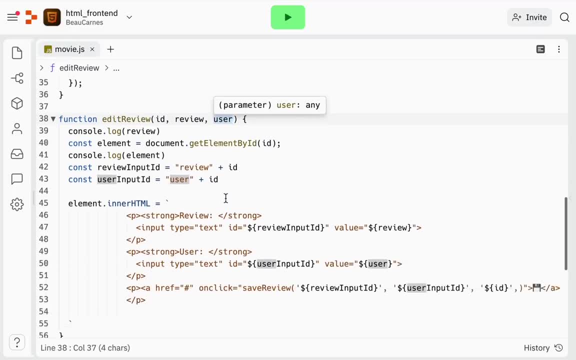 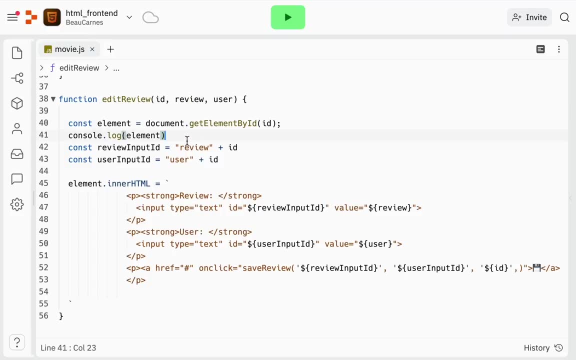 in their function. we accept the ID, the review and the user, And you don't need these, but the console that logs for just to make sure everything's working correctly. we'll get rid of them, So we can see only the important information here. So the first thing we're doing is getting. 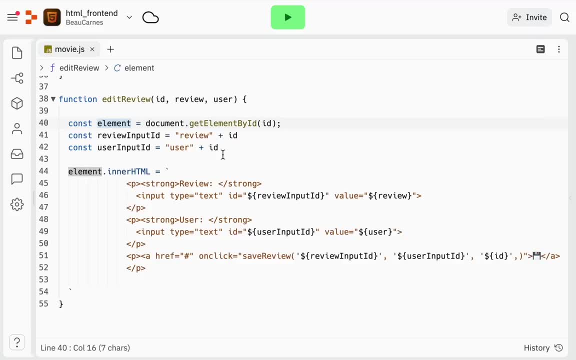 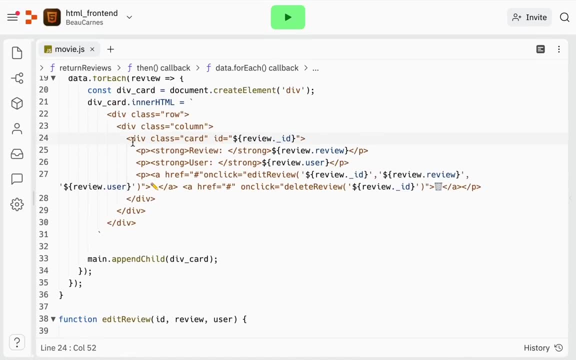 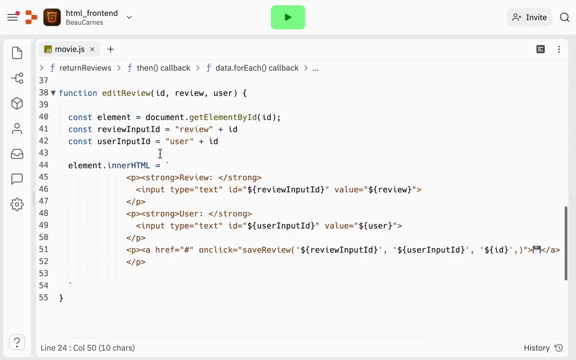 access to the element. So what element that is? so it's get element by ID And that's the ID we've passed in And if you remember, that's this element, this whole div here we created with the ID which is the review ID. So we're getting access to that whole. 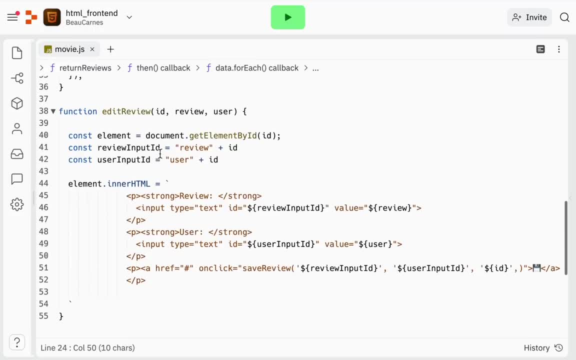 div, because we're going to replace what's in that div, And so we're getting the review. we're creating an ID that we can reuse in a few different places. So we're creating a new ID that we're going to put into our elements And when we update the HTML, so 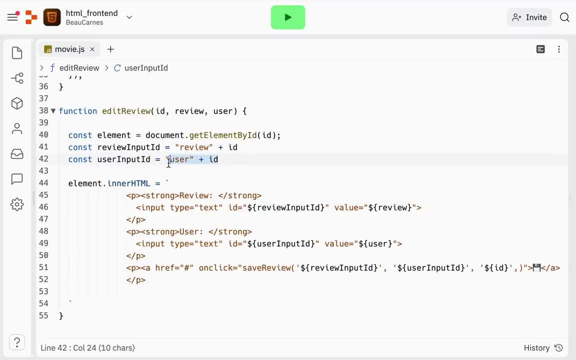 we are going to create a review ID and a user ID. The reason why we're creating an ID by using a word that's always the same plus this ID that's always different, is because we want to make unique IDs for every single element. 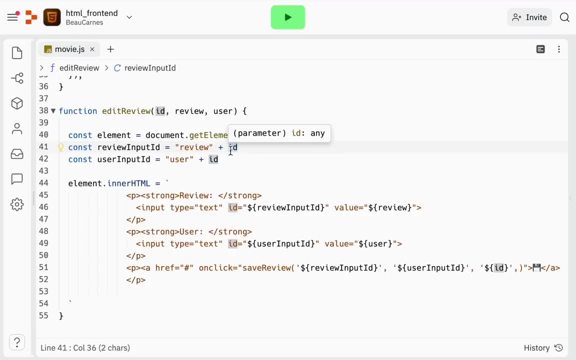 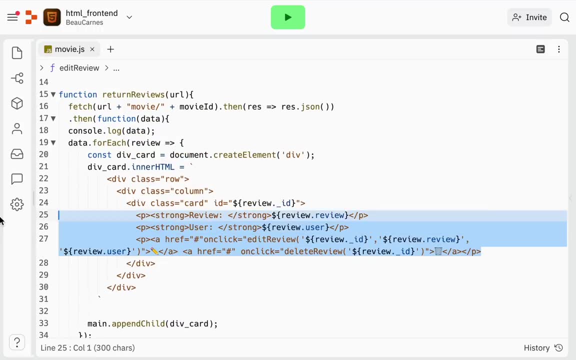 that for basically for every single review element that's on the page, and then we're just going to update the inner HTML. that means we're going to switch all the inner HTML that's already there. So this is HTML that's already there, which we're now going to switch with all this. So basically, 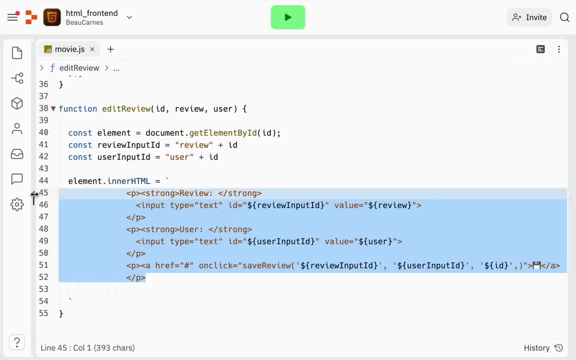 it's going to be very similar, But there's. so basically there are three paragraphs just like before, except each paragraph is taking a few different lines, But the paragraphs are a little different. Now we're using an input box, So you already learned about input boxes, even on the 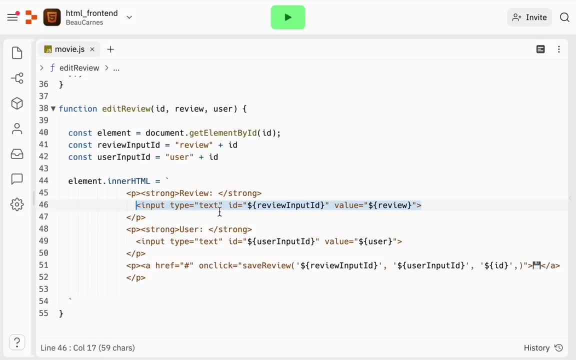 index dot. HTML. there is an input box, But this input box we are going to have the ID of the input box to be review input ID. And now look what we're doing. we're setting the value to be the review, So when you click the Edit button, the review will just switch into an input box. that 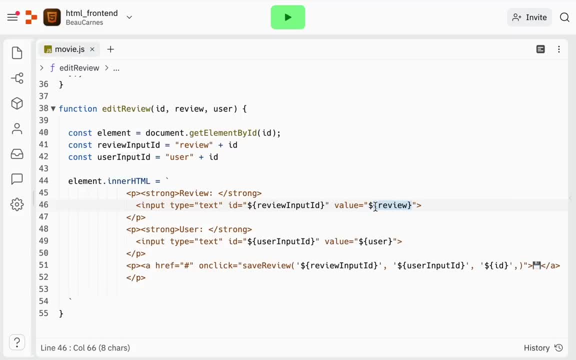 you can then edit And it's going to start with the value that it already was. So the review is going to be just how it was, But now you can edit it. we're doing the same thing for the user, where we're creating the ID of user- input ID- and then 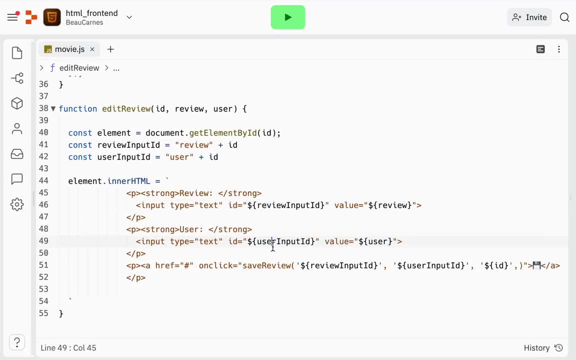 setting the value of the user. Now you'll see why soon, why we have to create these IDs just like this: because we're going to have to reference those specific elements with those specific IDs to get the value from the input box in order to send it over to our back end. So we have this. 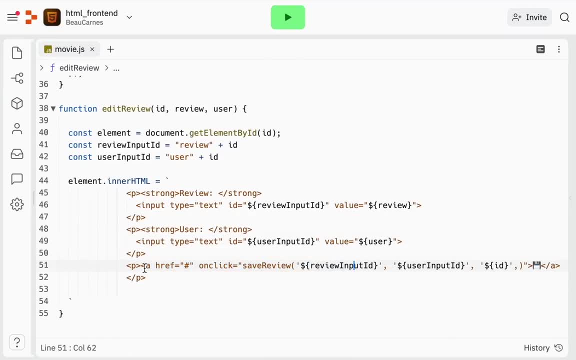 line, And then we're going to have the value of the user input ID, And then we're going to have this line here where we're now going to. before we had two buttons. now it's just one button. it's one emoji, a disk icon, which is the, which just means save. So once you click this little 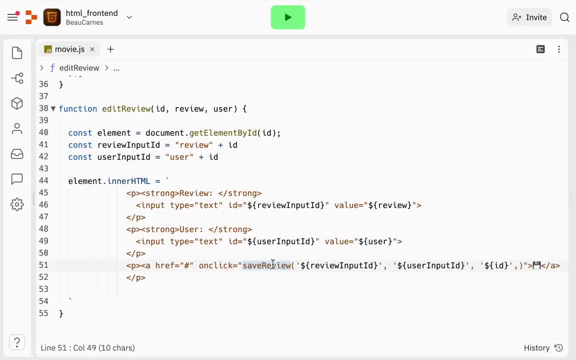 disk icon. it's going to call the save review function. it's going to pass in three things: the review input ID, the user input ID. So basically these are just the IDs of these elements, And then this ID is the review ID. That's the the review ID. 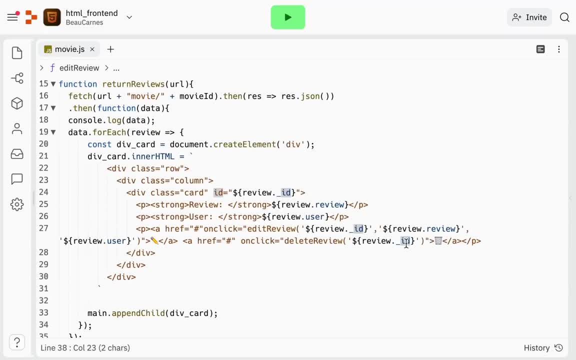 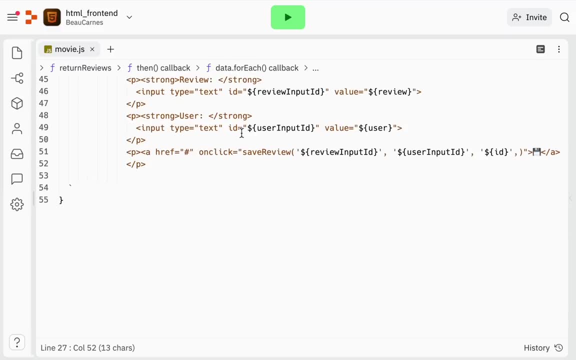 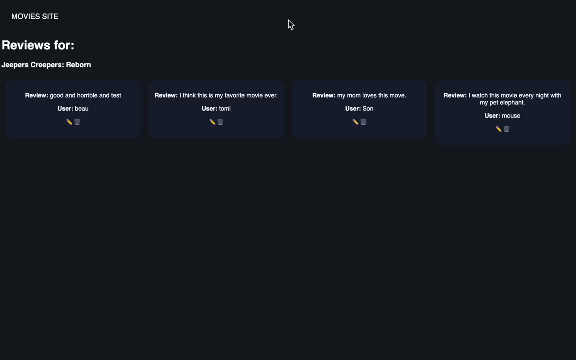 that gets passed in here, Because we're going to, if we're going to edit the review, we need to have the review ID, we need to know the ID of the review that we're going to edit. So let's see how that looks. I'm going to run that, or basically reload, And now I'm going to refresh here And now. 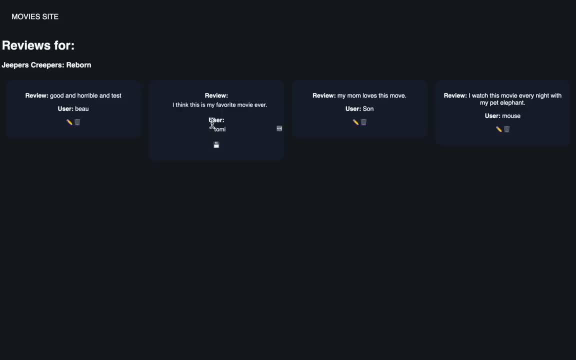 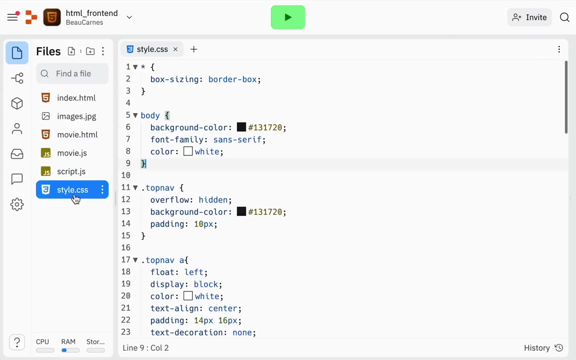 if I click here, let's see if it works. So it actually just changed into edit boxes. Now it we can't really see that they're edit boxes, mainly because of something in the CSS. So let's go back over and make a just change to the CSS. here I'm going to go into the style that. 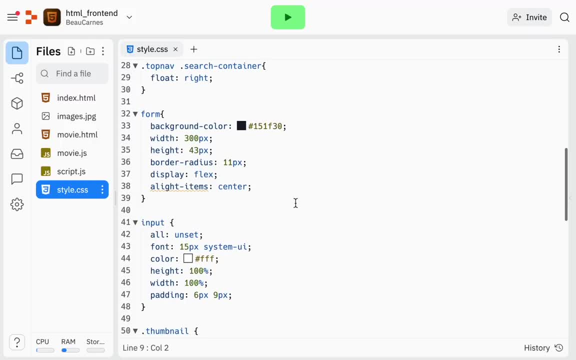 CSS And I'm going to, basically, I'm going to take off this all on set, this unset property, basically call create. causes this all the elements to inherit any inheritable values passed down from the parent element. So that's why the, the color, is not exactly what we would like. So, but we don't. 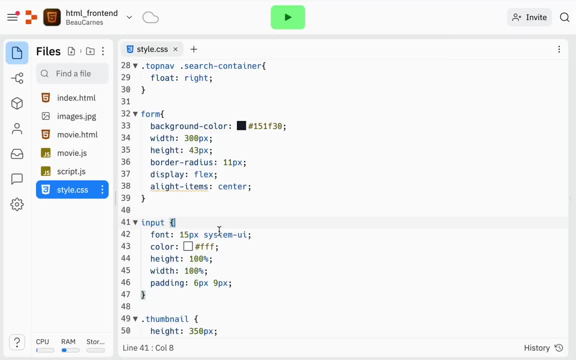 want to inherit anything. We're just going to use the, the, the normal input box color, which is a white background. And if we're having a white background, we want to make sure the foreground is black and not white. So there we go. So I mean, it's not gonna look quite as cool as how Tomi had it, But I think it'll be. 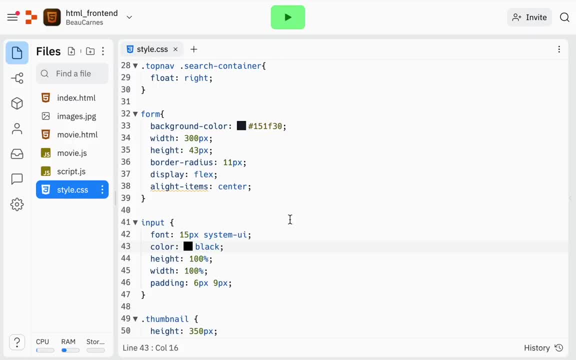 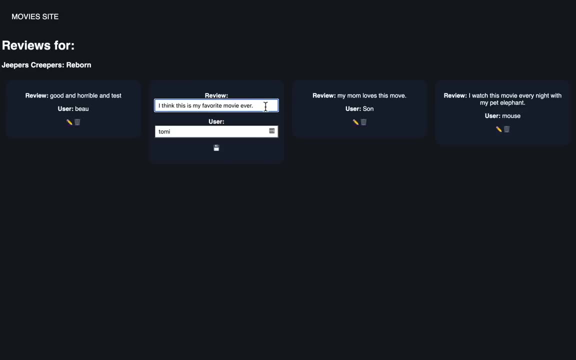 work for our purposes. If you want to customize the colors even more, you can. So let me go back over here and I will refresh. And there we go, So we can see these text boxes. I think this is my favorite movie ever, user Tommy, and you can click Save, which that's just going to do nothing. 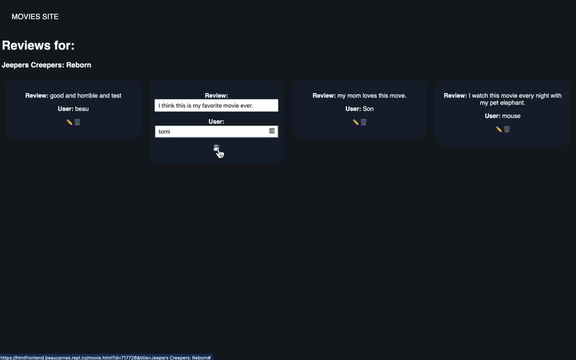 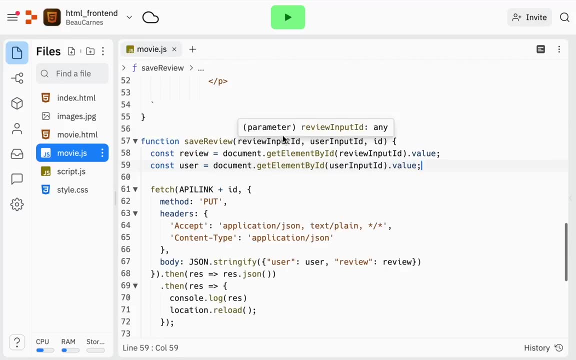 though, is in the console and show an error because we have not created the save function yet. So I think you know what we're gonna do. we're going to create the save function. Okay, here's the save review function that is called right here with the input ID, the, the review input by the. 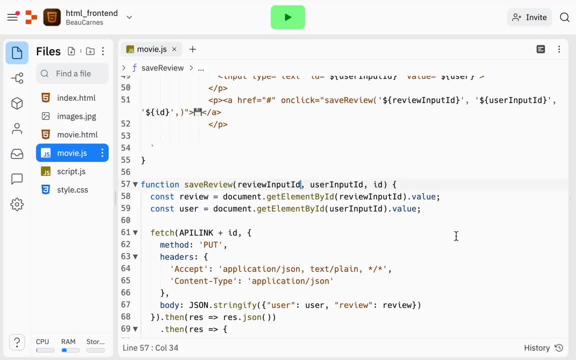 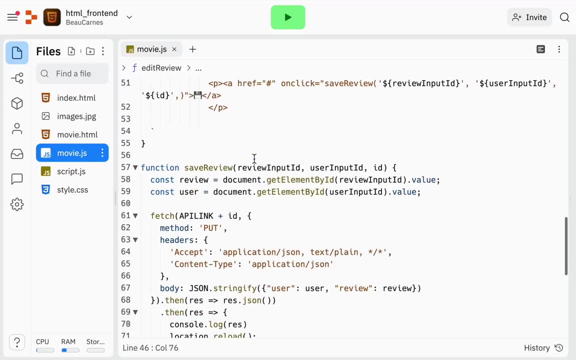 user input body and the ID. So first we're going to get access to the values of those input boxes. We do document that get element by the review input ID dot value. So that's going to get whatever value. is here the value that the person typed in for the review? it may just be the value. 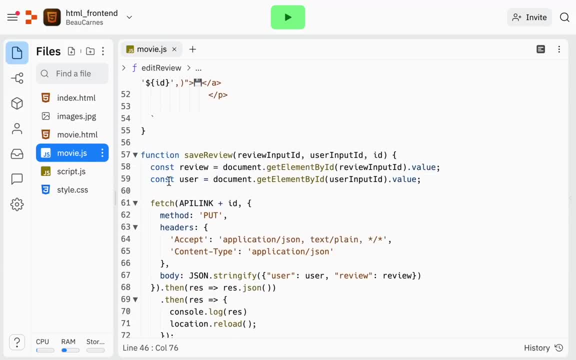 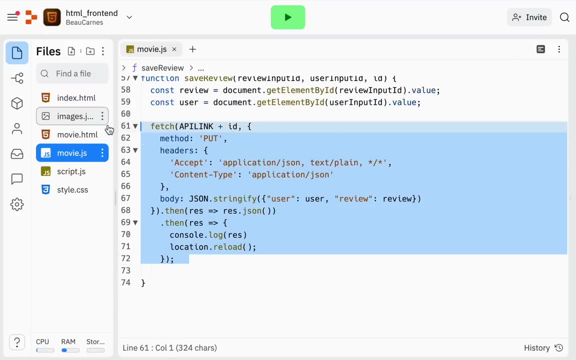 that was already there, So we also are going to get the user, so we just have to get the element dot value. Okay, now we're going to use fetch, And so I think you've already learned about fetch. fetch is basically a JavaScript command that allows us to 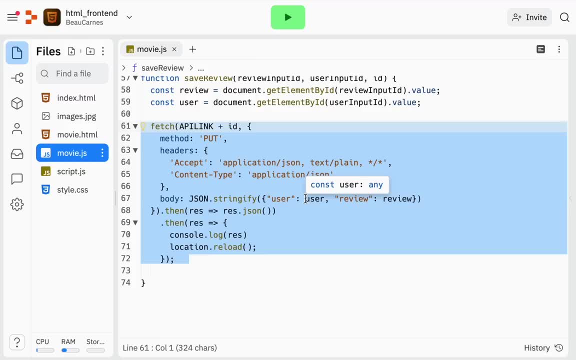 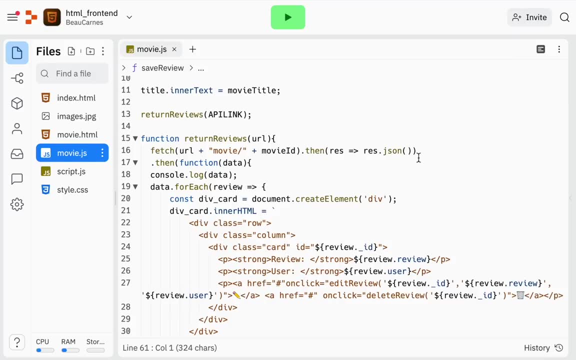 send HTTP request to a URL and get information back. So I guess, Yeah, of course we've done that, we've done tests, we've already have it up here. But here it's using it doesn't say the, the method, the HTTP method, because it just defaults to a get request. Everything, basically defaults to get. 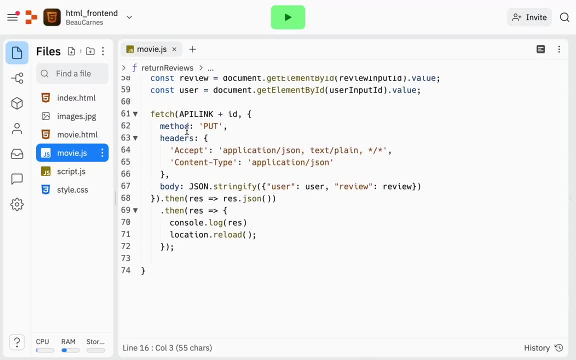 request if you don't specify. but now we're going to pass in something else, So first we're passing in the URL. So just to clarify: the URL is the root URL And you can even see it like popping up on screen. 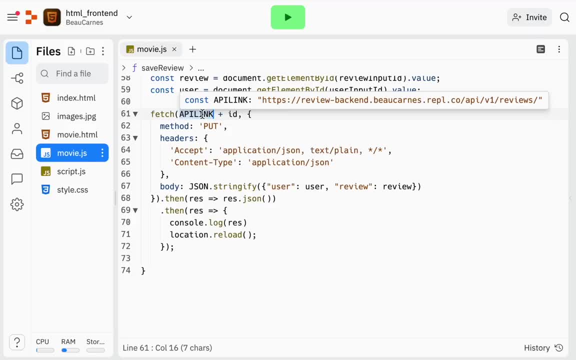 what the value of that URL is and see how it ends with slash, review, slash. then we just put the ID at the end. This is what we created the URL to be in our back end when we are going to be editing a review. So now we can. then the second we're we're passing in two things. First, we're passing 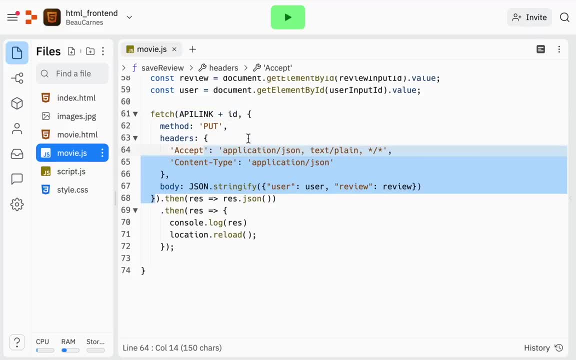 in this, then we're passing in this. So if I see, if I put my mouse on here, it highlights that it also highlights the ending curly brace. So this is the second parameter that we're passing into the fetch function And you can see this is an object that has a few different key value pairs, including the method. 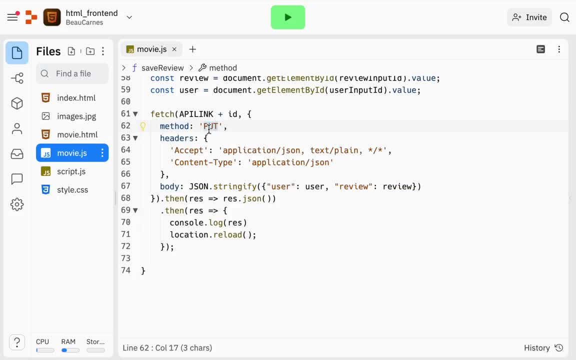 we're using put, because that's how we create our API for editing a review. we are using put and then we pass in the headers- these probably look pretty familiar to when we were using curl to do this earlier- And then we're passing in the body we set to do: JSON dot, string of i. this is a JavaScript command. 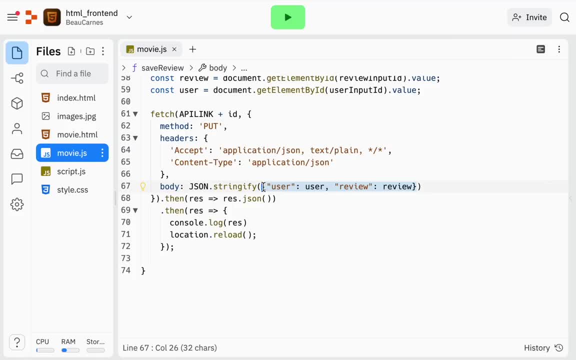 to make a string from an object And we're passing in this object And so we have the user and the review. So this is the key. this is the value which comes from our variable. this is the key. that's the value that comes from our variable. this should look kind of familiar to. 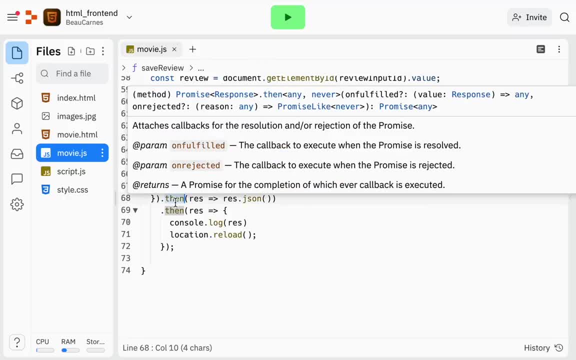 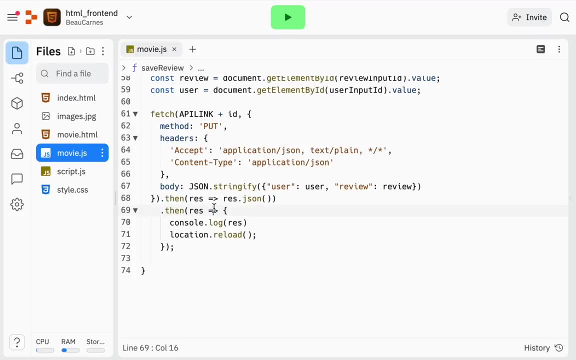 how we did it in curl then. So when we are doing a fetch, we can do dot then. dot then means after we get the data, after we get the data, then we're going to take the result And we're going to do. 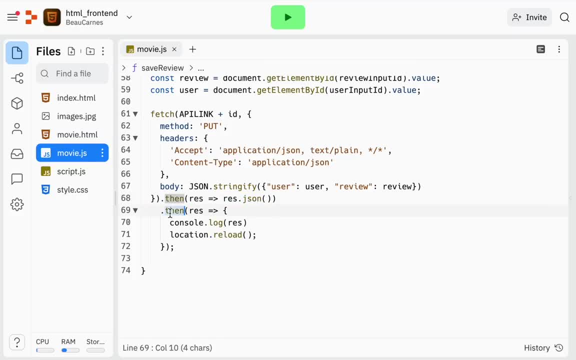 result: dot JSON. we're basically converting it to JSON, then we're going to get the result of that And we're going to log the result And then, finally, we are going to this location, dot reload. this is just the JavaScript. 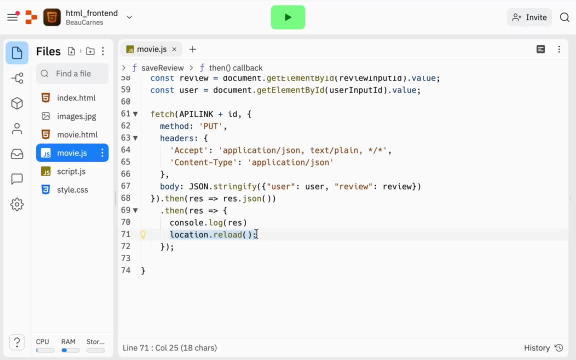 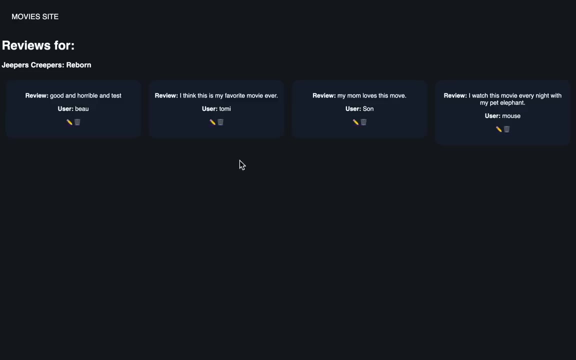 Command to reload the URL. we want to reload the website because now there's the edited data And we wanted, we want to reload everything with the new data that's been edited. Okay, let's see if it works. So I'm going to run that And I'm going to manually reload with command or Ctrl R Now. 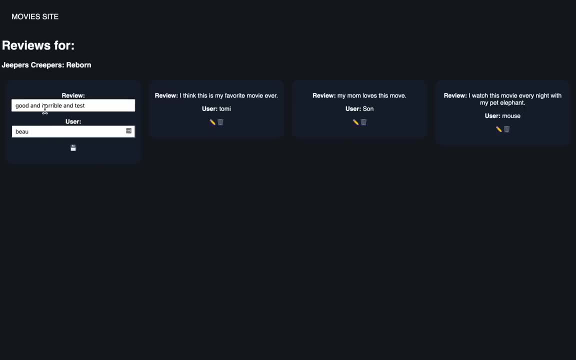 I will do this one Good and horrible and test: Well, this is good and horrible and also amazing, And then I'll see if I can change this to a capital B If I click Save, It worked. good and horrible and also amazing. 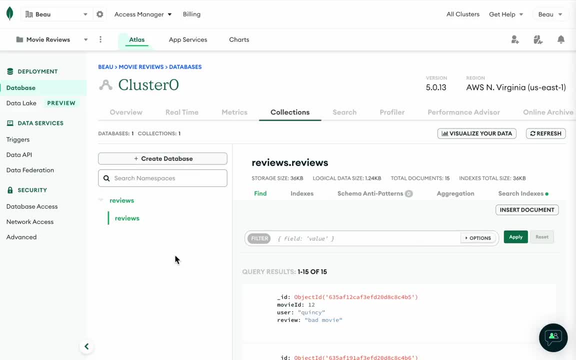 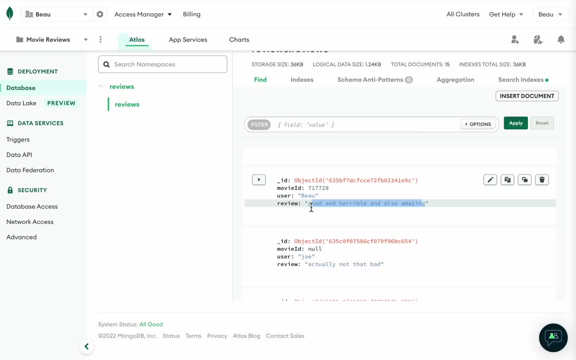 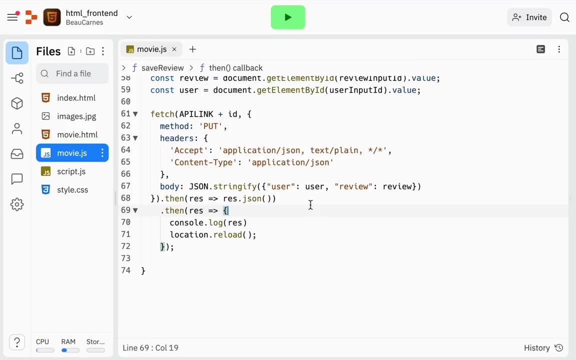 And if we go over here and refresh MongoDB Atlas, let's see if we can find that one Good and horrible and also amazing. So we successfully edited or updated our review. Okay, there's two more things we'd be able to delete a review. 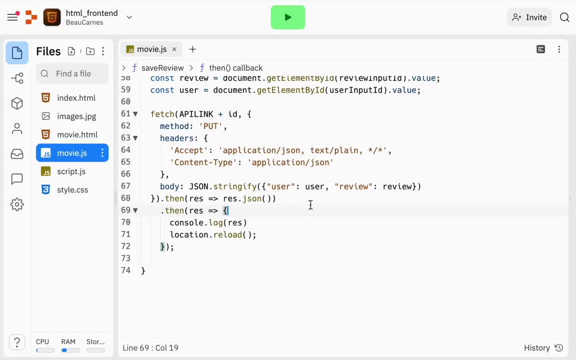 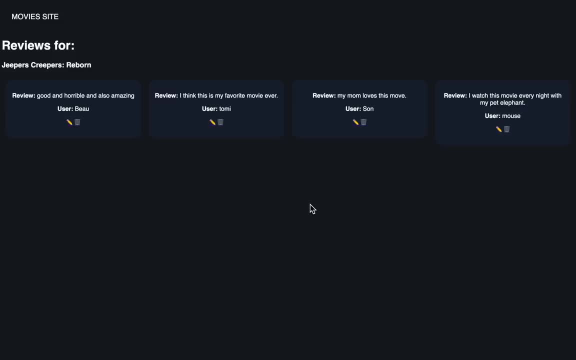 and create a new review. Let's do the create new review first And then, finally, we'll add the ability to delete a review. Now there's a bunch of different ways that we could basically visualize the Edit, the Delete, the create a new review. we could create a whole new. 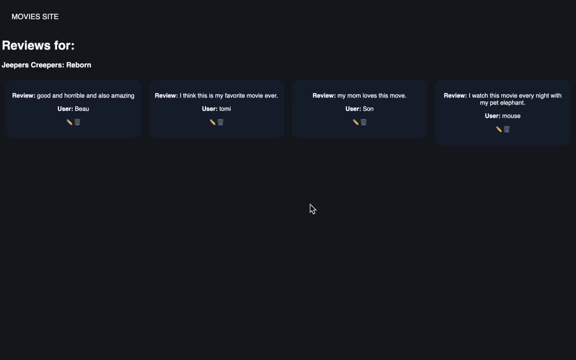 website where you create a new review. But I'm just trying to keep things simple, simple, So see how we'd have these different cards. I'm going to make it so the first card has the little form to create a new review. It may it's not the prettiest way to do it. 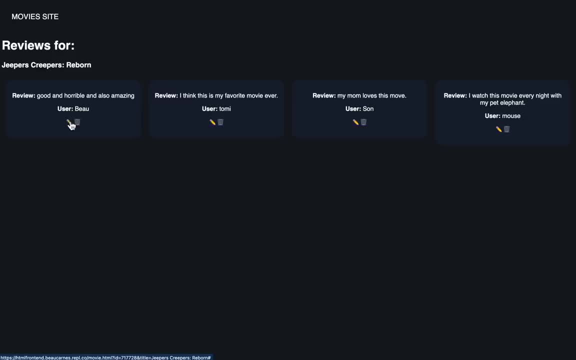 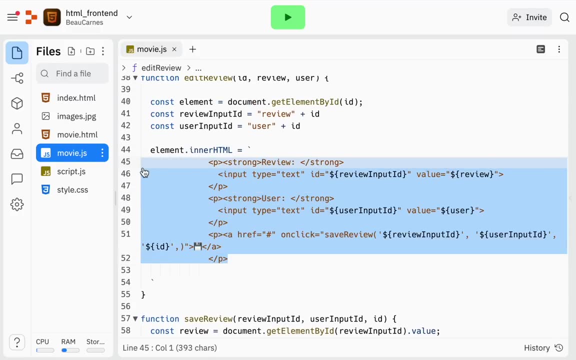 But it will get the point across and we'll show you how to how to do it, And then you can also always refactor and change things later. So we already have the code for what it's going to look like when you're editing. Well, creating a new review, it's gonna look. 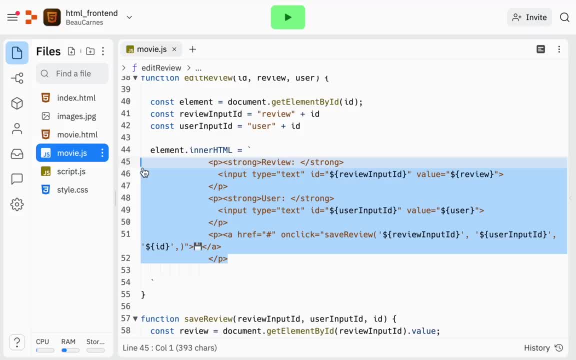 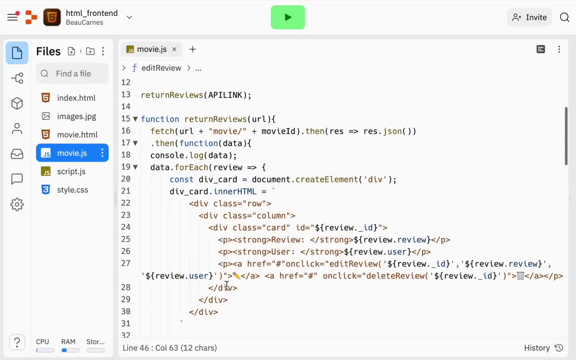 basically the same to editing a review, except this time it won't start with any value in the value here, because it will be a blank value. So what we're going to do- see how we're basically- we create all the cards for each review Before we start adding all these review. 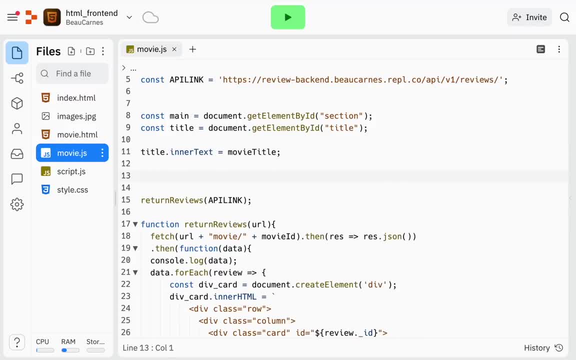 cards up here. after we create the movie title, let's create a card that will allow us to create a new review. Now, this is something we could do right Right in the HTML file, because it's not going to have that much stuff specific to. 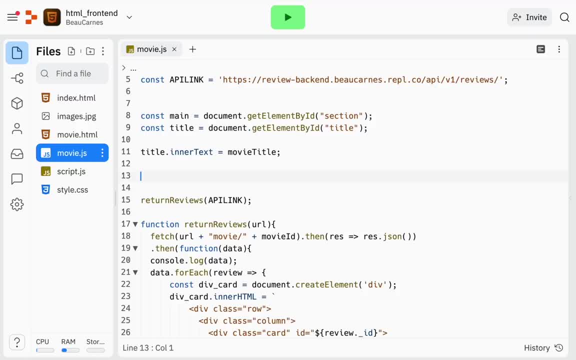 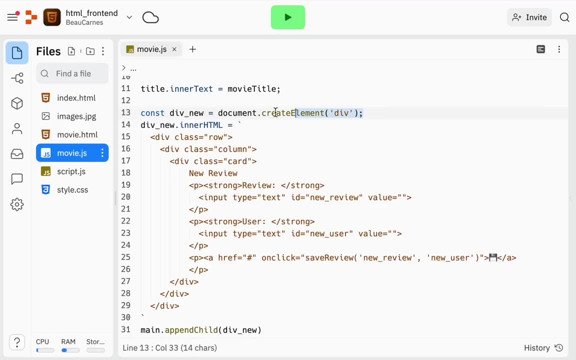 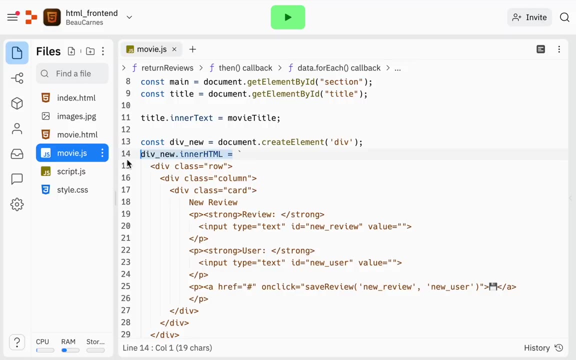 that we need JavaScript for. But just to keep things simple, Let's do just all right in the JavaScript. So you can see what I did here. So we create a new element, just like before, just like this: here, Now we're going to add inner HTML, just like we did down here, And then we're. 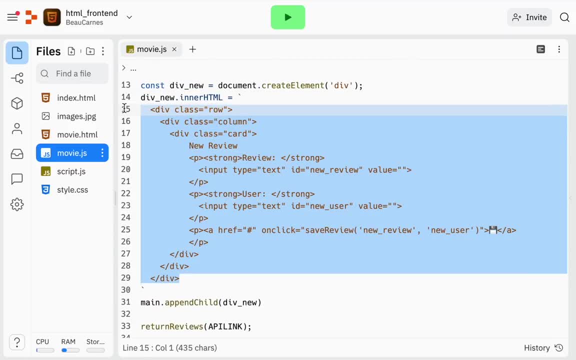 going to create all this HTML, Right? So, like I said, we could just add this to our HTML file. But we'll just do it like this. So it's it's all together here in this in the JavaScript file, But you can see we're not using any. 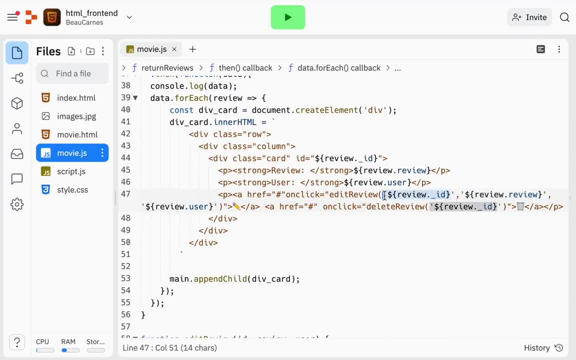 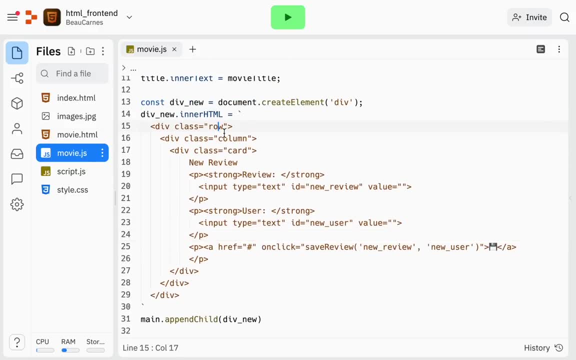 variables in here. So this is what it looks like if we're using a variable. Since we're not using the variables, that's the way we know that we could do it in the HTML. So we have the row card column. it's going to say new review. that's something new And basically. 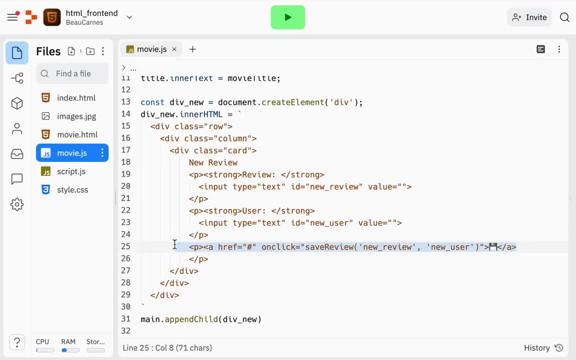 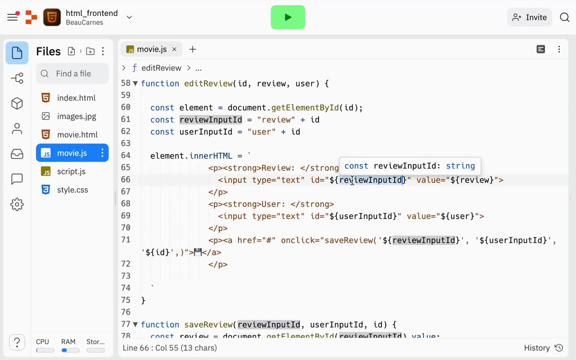 this is all exactly the same. even this is exactly the same To the Edit. the only the only thing different is that we're hard coding the IDs. we before we need to make sure we have different IDs because there could be basically an unlimited amount of reviews and every review needs a. 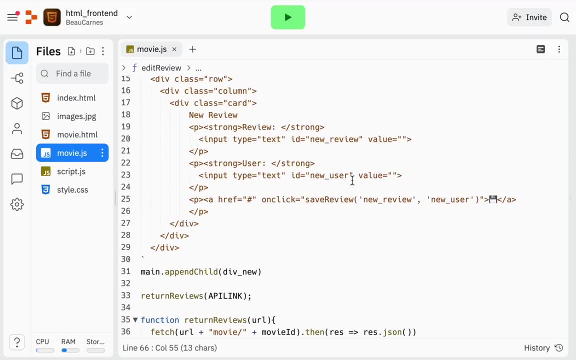 different ID, But there's only going to be one box for the new review, So we only need to. we can hard code the new, the idea of new review, new user, And then, when we save the review, this is what we're going to do. And then, when we save the review, this is what we're going to do, And then 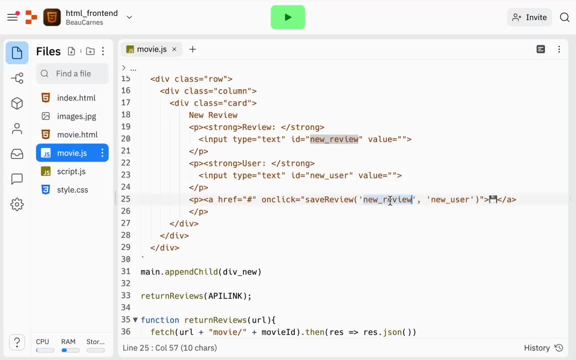 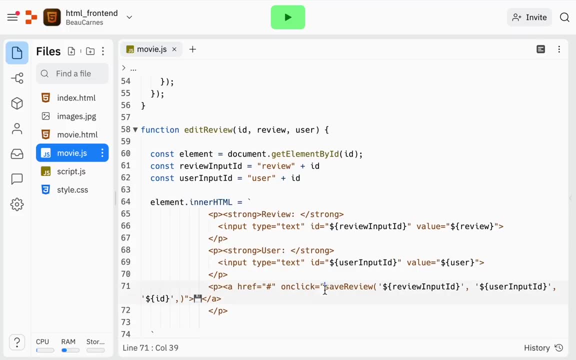 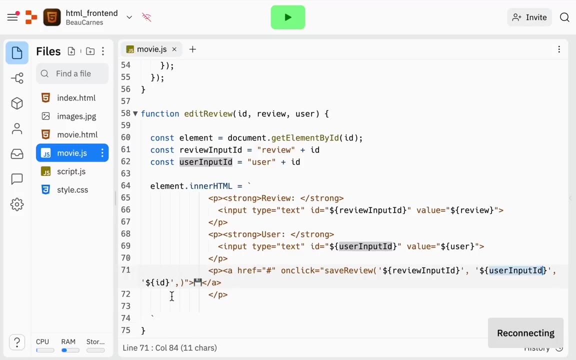 where it gets different. So we're passing in the new review, that's the idea of here, the new user, that's the idea of here. But if you remember, down here we pass in one more item. we pass in the this ID, this other ID and then the review ID. That's the third. 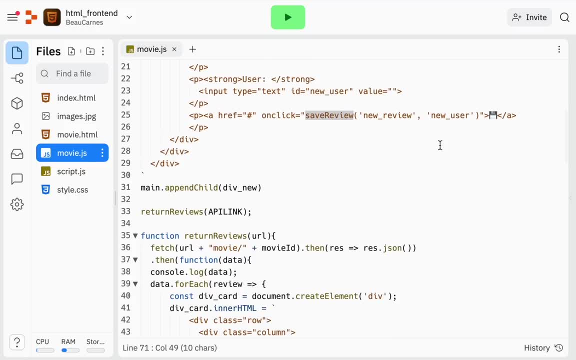 parameter we pass into the save review function. But now there is no review ID because we haven't created a review yet, So we're only going to pass in two parameters. So since we're only passing in two parameters, we're going to have to make an. 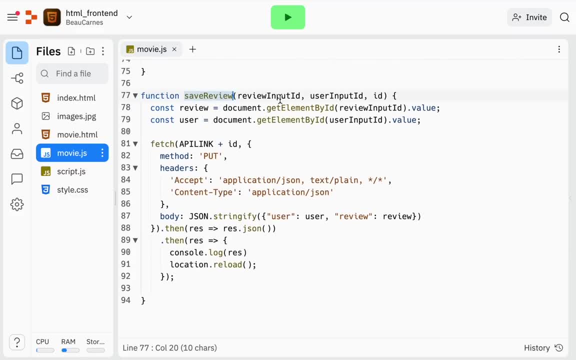 update to our save review function. So there's a way, because normally all these, all these parameters, all this information are required. there'll be an error if we don't pass in three things. there will be an error, but not for long, because I'm going to show you how to make an. 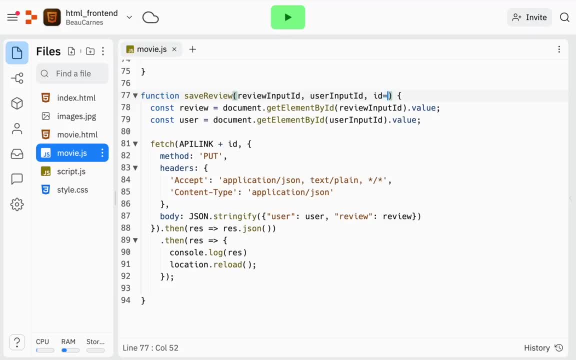 something optional. If we put equals- and then I'm just going to put what equals, we can put a default value, And right now it's just going to default to an empty string. So if you specify a default value like this, 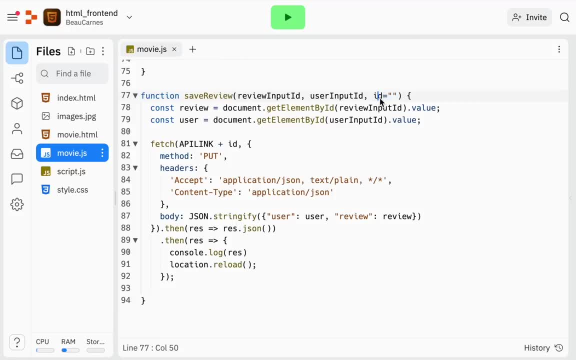 then you can pass in an ID and it will take in that information that you passed in. But you don't have to, because now, if you don't pass an ID, it will just set it to whatever the default value is, which in this case is an empty string. 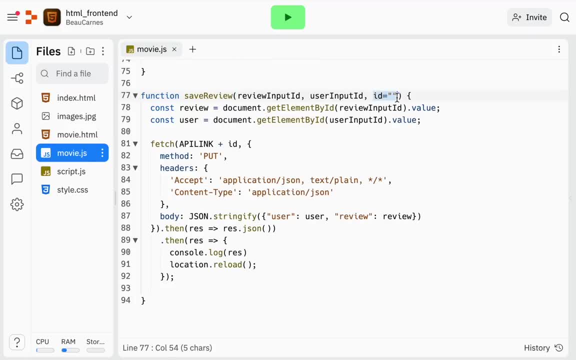 Well, since we have to make things think, things should happen differently whether there's an ID or not, because how you create a review is different than how you edit a review. So the way we're going to make it different for creating a new review or editing review is with an if statement. 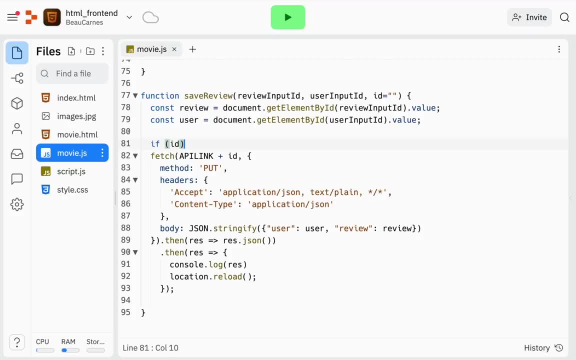 So if, and then we're just going to if ID and then I'll put the curly braces here. So if ID basically just means if it exists, this will evaluate to false, and empty string evaluates to false. But if there, if something was passed in. 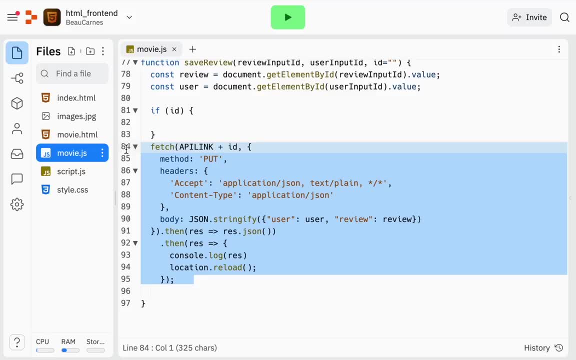 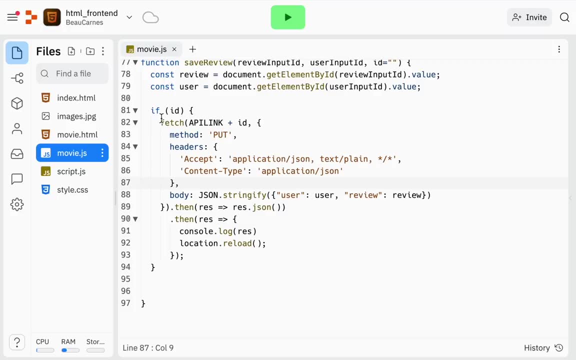 then it will evaluate to true. So it evaluates a true. we want to do all this, So let's cut that And I'll just paste it right into our if statement And let me do some tabbing So we can see that it's in this block of code. So here's our if statement, But now we will add an. 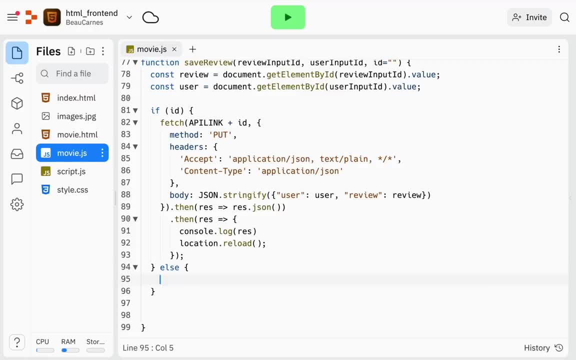 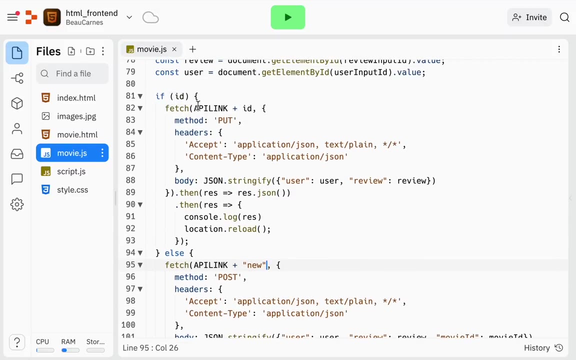 else. So else, if there is no ID that was passed into this function, that means we're creating a new review. So let me just paste in the code here And it's gonna look very similar to our edit. So for edit, we have the root URL and we have the ID at the end, But for creating a new 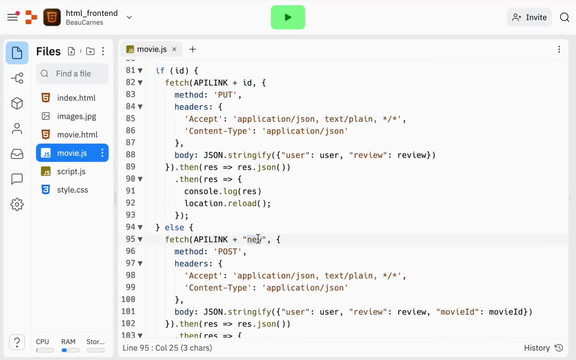 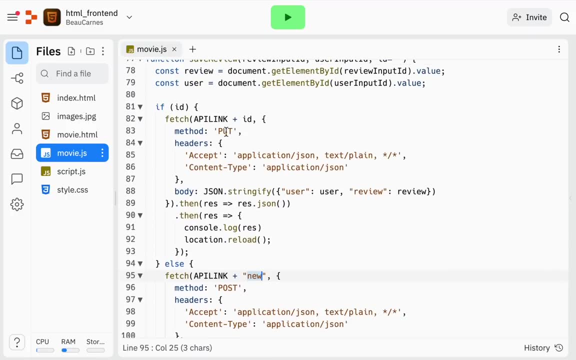 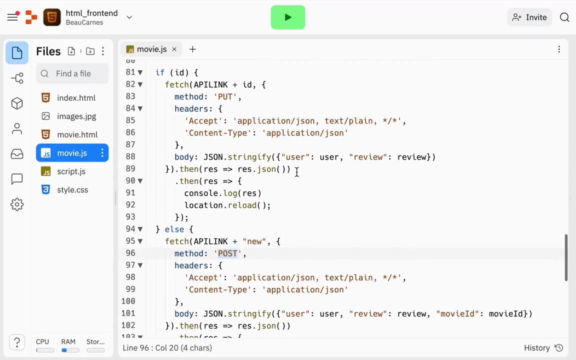 a new review. we're gonna have our root URL and it's going to be just slash new at the end, which you may remember from creating the API, And instead of a put method, put HTML method, we're using a post method, And then the only other thing that's different is now: here we pass in the user and the 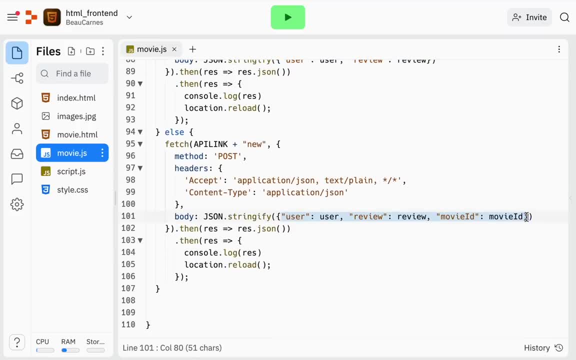 review. Now we're passing in the user, the review and the movie ID, Because we need to know what movie ID are we creating the review for, if it's a brand new review, And then this is all the same as before. So then we convert it to JSON, then we log out the results And then we do location dot. 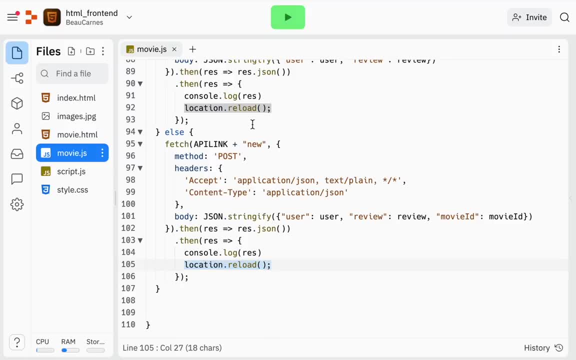 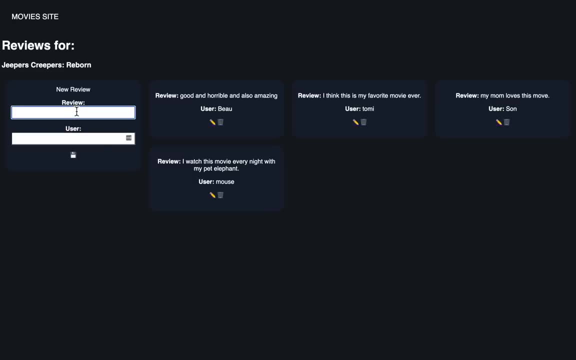 reload. Okay, let's try this. I'll load this And now I'm going to refresh, And now we can see a new review here, So I can say: this movie put me to sleep And then we can put as the user Quincy. 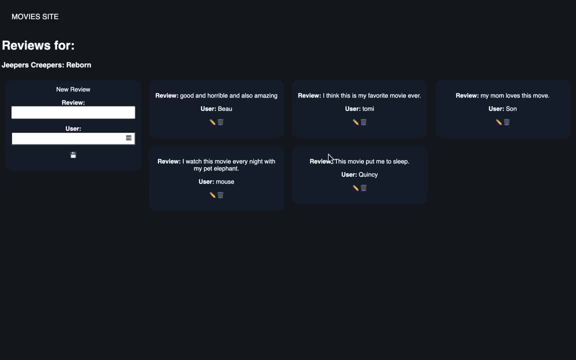 And if I hit Save, let's see if it works. And it shows up at the end of our list of reviews, So that works And let's see if we can edit that new review. This movie kept me awake And then we'll save that And it saves correctly. 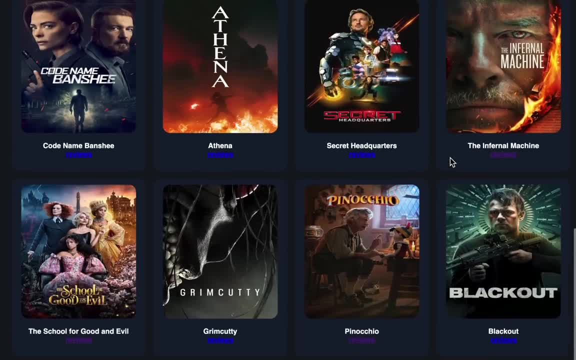 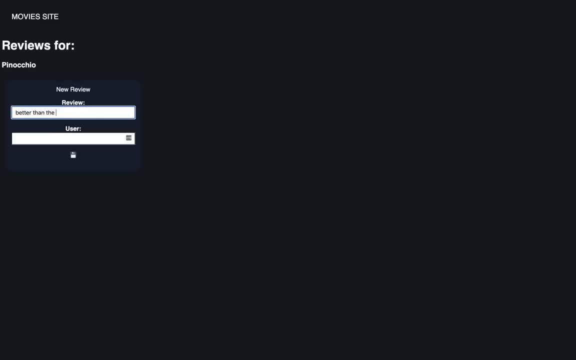 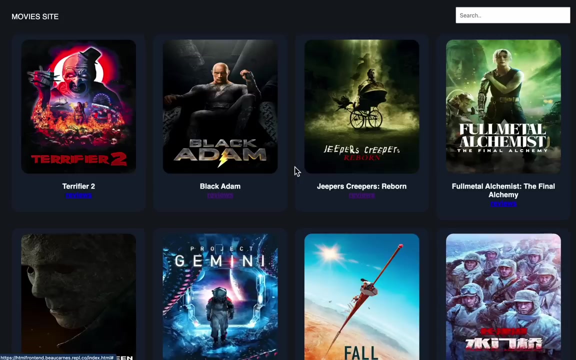 So we can even go and add a review. we can go to a whole new movie. I'll put better than the original by 2.'s 0.5%. Okay, there we go. Now we have a review for the new movie, So some are not going to have a review. 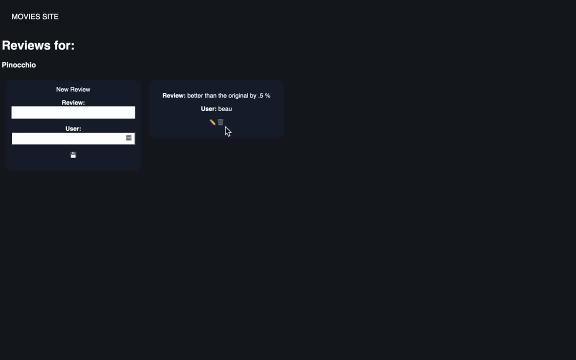 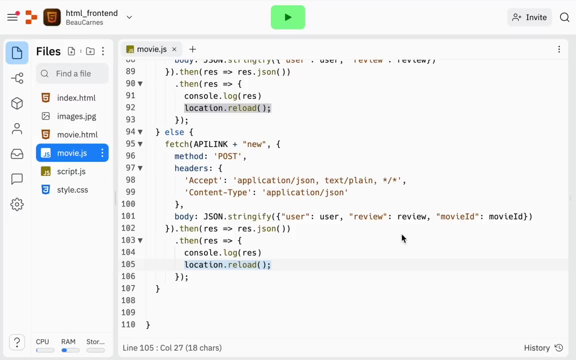 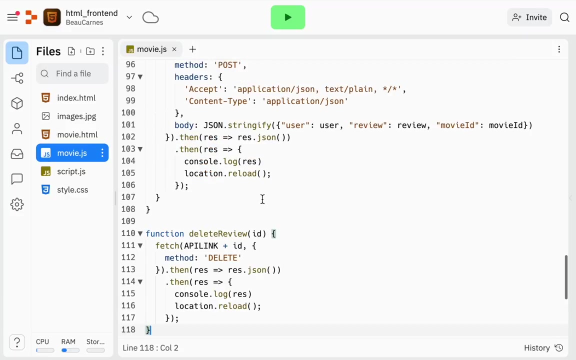 some are going to have review, but we still can't delete a review. So let's go and make it so we can delete a review. this is actually going to be one of the easiest parts, because the function to delete review is not that long. I'm just gonna paste that and it just looks like that. 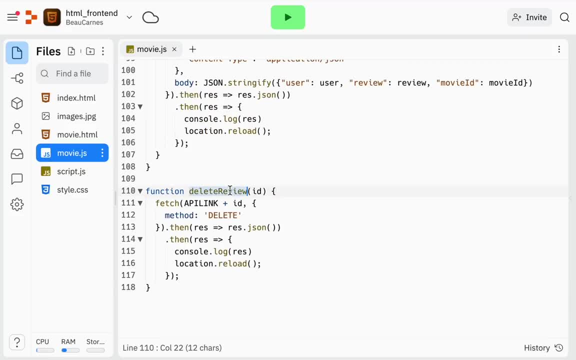 So we already have it. So you can call the delete review function and it passes in the ID. So we just go to the URL slash ID And then we use the delete method. we don't have to put in any other information, we just have to call the delete method And then everything. 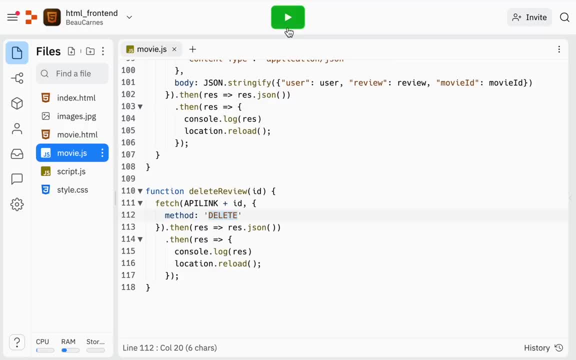 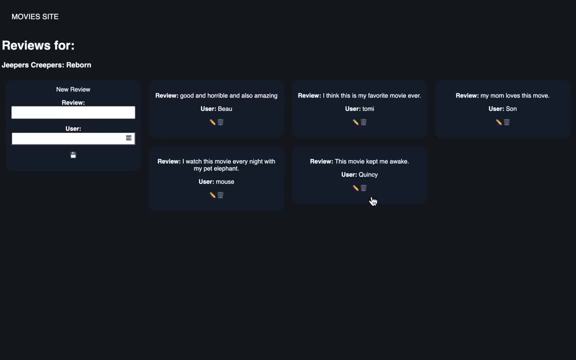 else is basically the same, So let me go here. Okay, we know we have a lot of reviews here, So let me try to delete one. How about this? I'll hit the Delete because we don't want the. anyways, this is supposed to be movie, not move. Okay, so that's a bad review. Let's 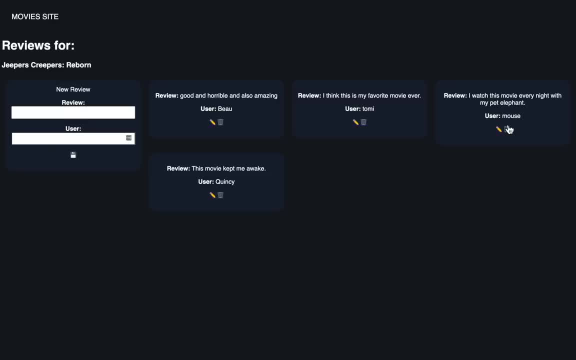 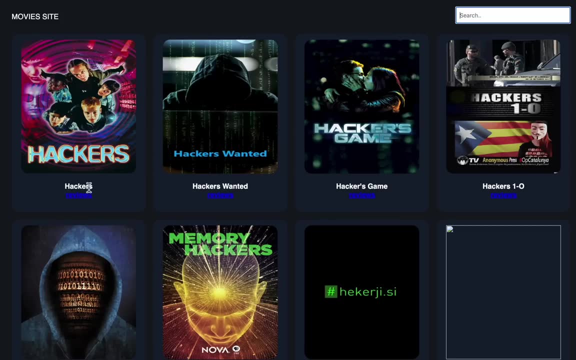 just delete that. It's gone. The- the review is gone, So we can even even search for review. Let's go to um hackers And we have one review here. Before we try to leave, let's try, let's create a. 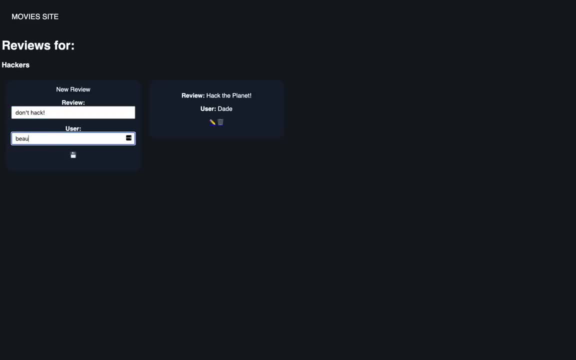 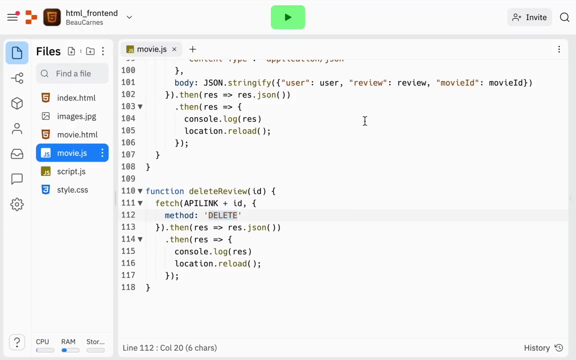 new review: Don't hack. And then it appears don't hack, which obviously is not in the spirit of this movie. This called hacker. So we're definitely deleting this review. Okay, it deletes the review. We did it. we created the. we connected the front end of. 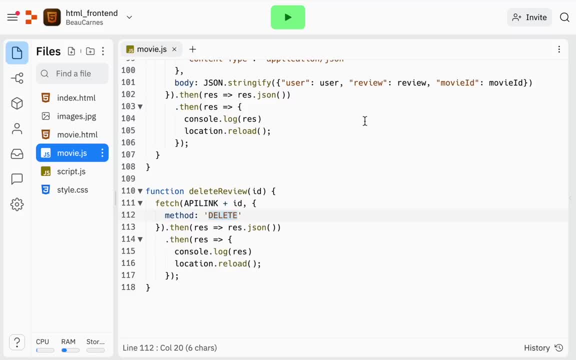 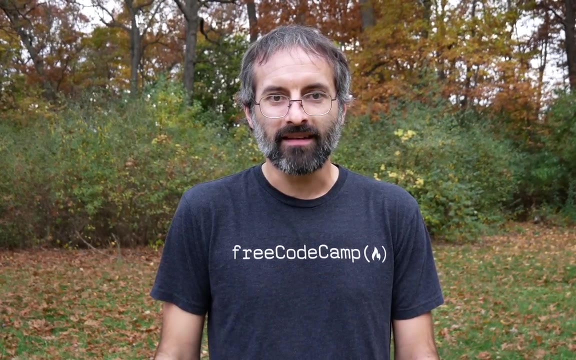 our website to our back end And it can save, update, read, delete all the CRUD operations And it does it with our MongoDB database. We've reached the end of the course. Thank you all for watching and good luck creating your own full stack websites.